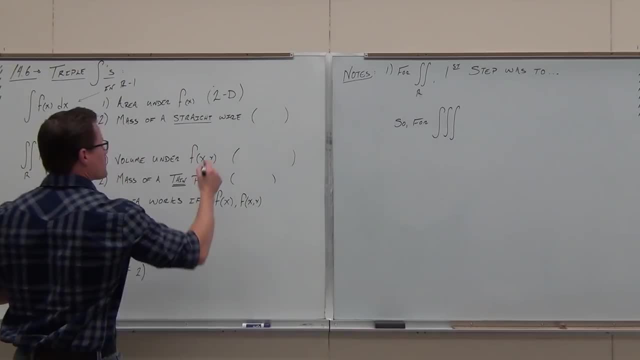 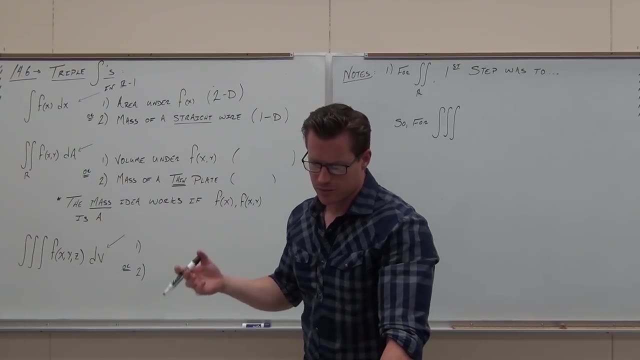 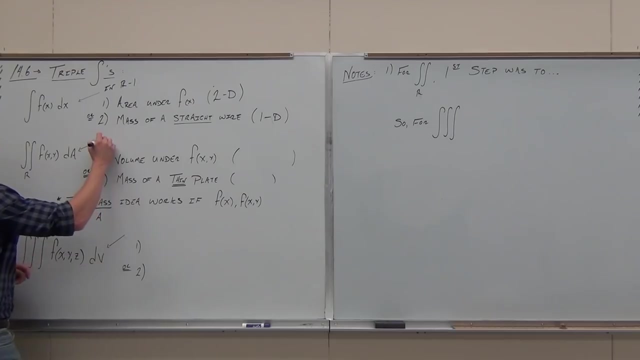 But a straight wire, that's a 1D concept. Well, and then we, then we went and we did. well, we did double integrals, And in these double integrals this DA stood for You know, dy, dx, dy or dy, dx. but the point is, you're now integrating across two axes. 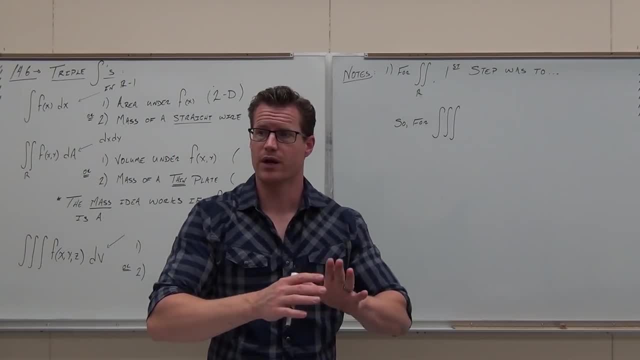 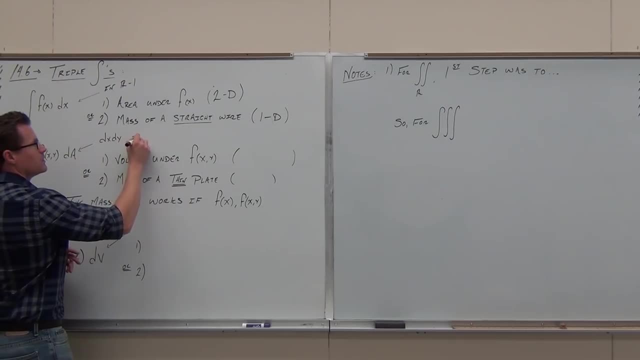 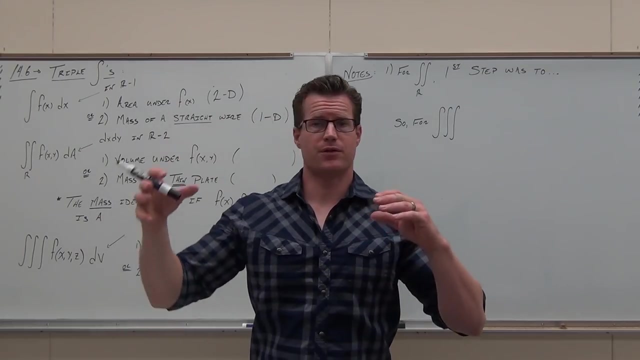 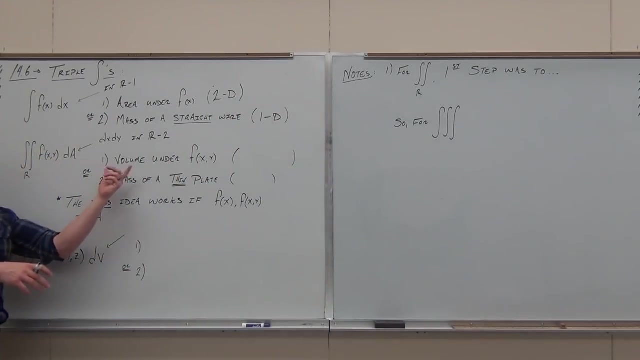 You're integrating along the x and along the y. that gave us over a region. Is this ringing a bell for you? Yes, Well, that's a 2D integration. so in R2.. And this also had two connotations. from the 14.2 and 14.3 stuff we learned that a double integral. what that represents, that is the volume. 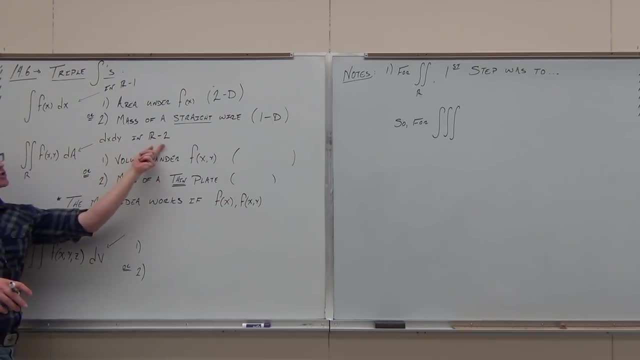 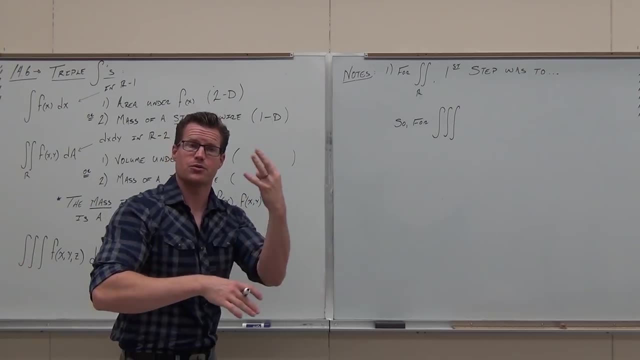 Under f of x, over that two-dimensional region, and now that you understand the concept. but it was volume. It was a volume over 2D. That was a 3D concept, But in 14.4, we had a different take on it. 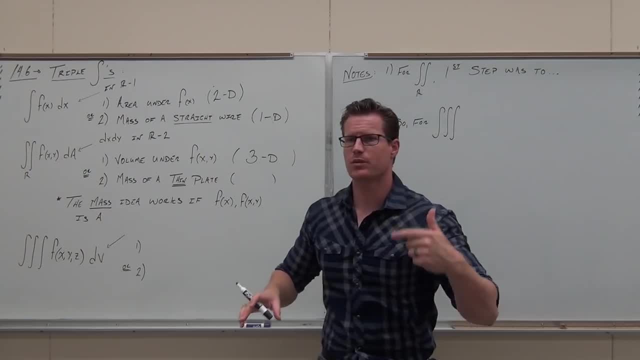 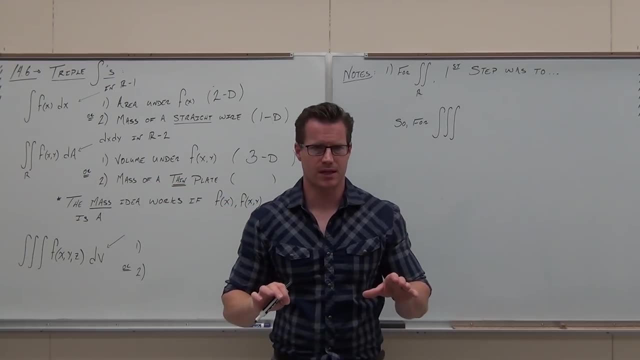 We had this take on it. We said, well, wait, wait, wait, Wait in 14.4,. we learned something else. We learned that a double integral can also represent the mass of a really thin, and when I say thin I mean like the calculus version. 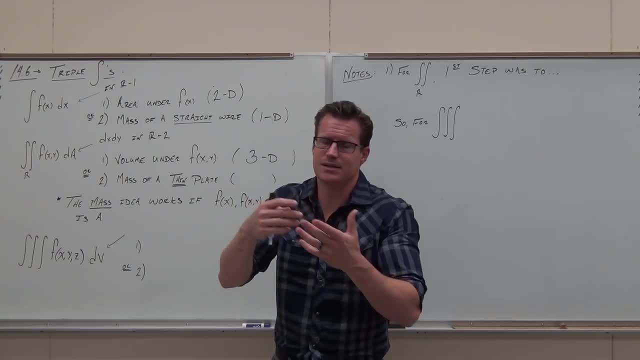 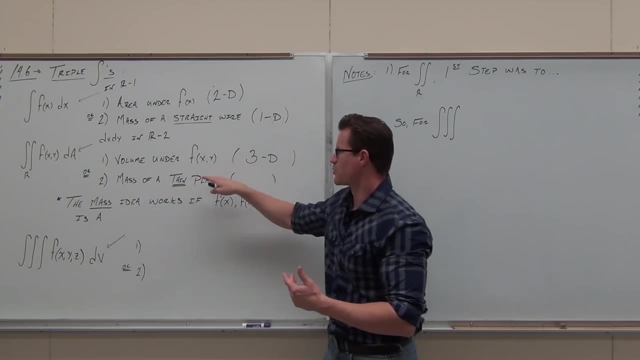 Thin like negligible thickness, like it's not measurable, like it's super thin. Does that make sense? We also learned that We said: well, okay, double integral can also represent the mass of a really thin plate. Well, if we have a plate that's really, really, really thin, is that truly a 3D concept? 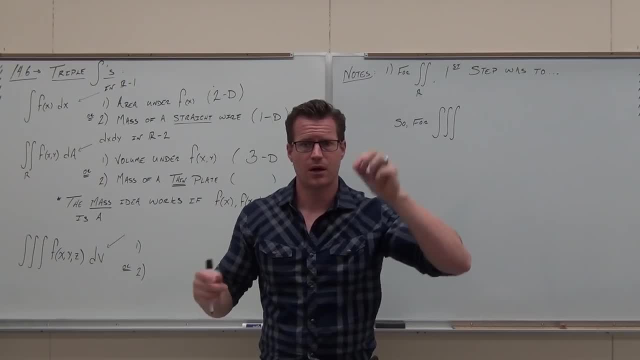 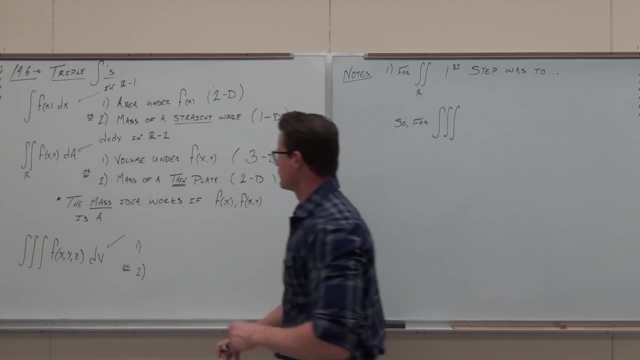 Calculus-wise, really, thin means negligible, infinitesimally thin. That means that we just have the region itself. That's a 2D concept. So let's kind of flesh this out and see what triple integrals are going to mean for us. 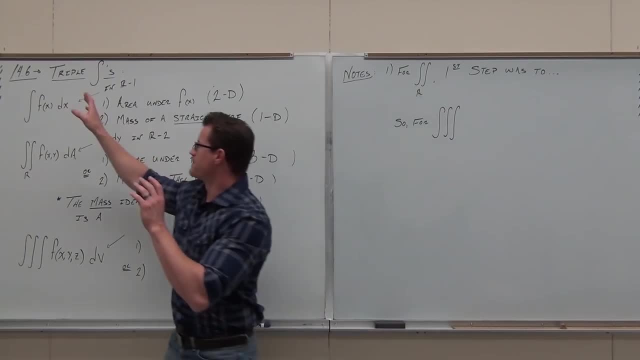 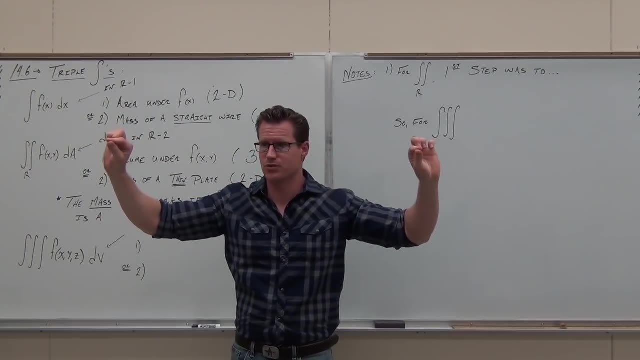 So let's think about this: Are you guys okay that for a single integral? yeah, it represents area, but it could also represent mass of a 1D creature, a 1D creation there I know that you're okay with that one. 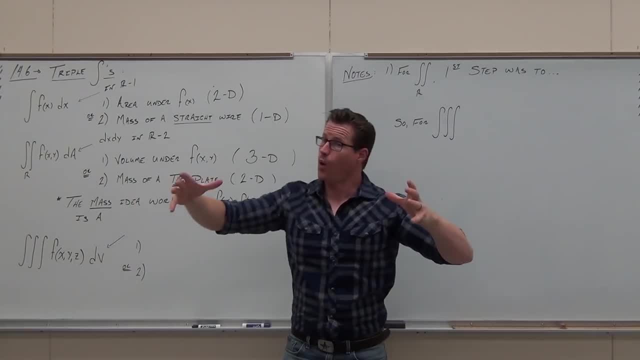 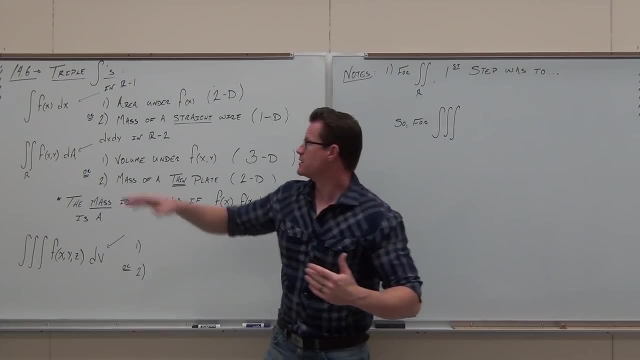 Okay, double integrals: Yeah, it could represent volume 3D or it could represent mass of something that's 2D. Do you see how it's bringing it down a dimension? Do you guys see the point? Double integrals could be a 2D idea. 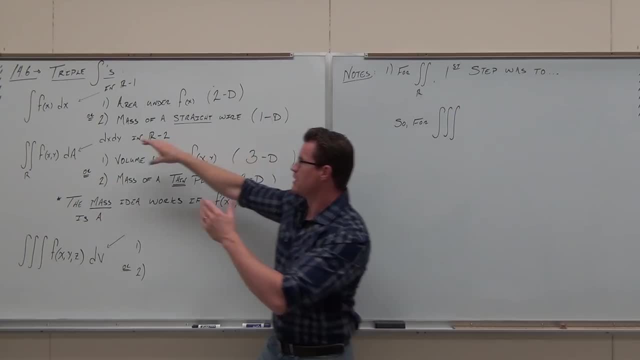 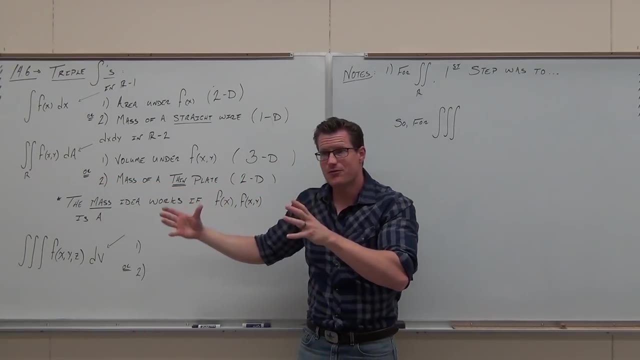 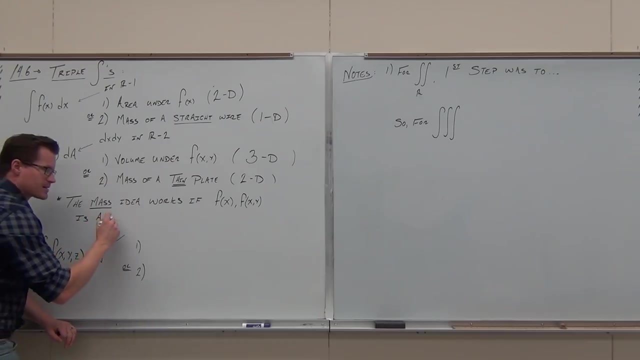 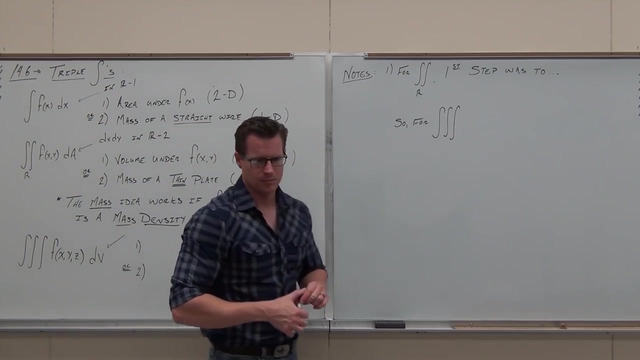 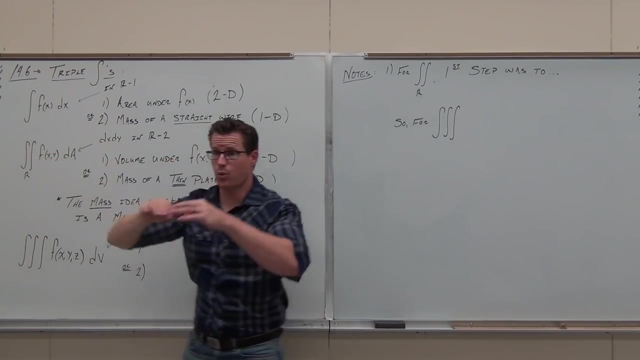 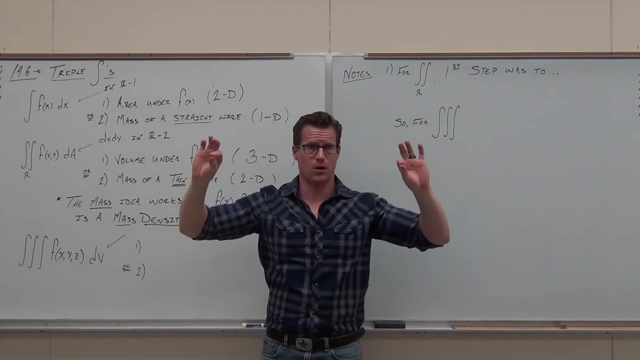 Area, or a 1D idea for mass. Double integrals could be a 3D idea for volume or a 2D idea for mass. If these things, if this is a mass density function, So if f of x is a mass density function of the wire, so imagine a straight wire, not curved straight wire, and this function tells you where the mass is along that wire. 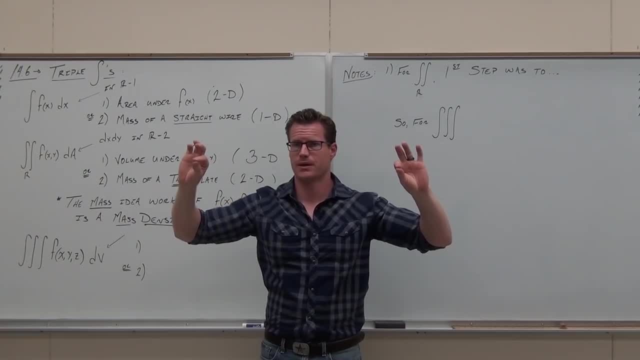 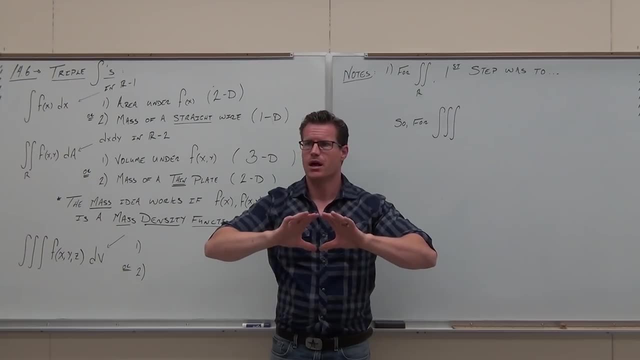 You guys getting the idea. The integral will tell you the mass of the wire. If f of x, y is a mass density function of that plate, really thin plate over a region, if it's telling you where the mass is located on that plate, 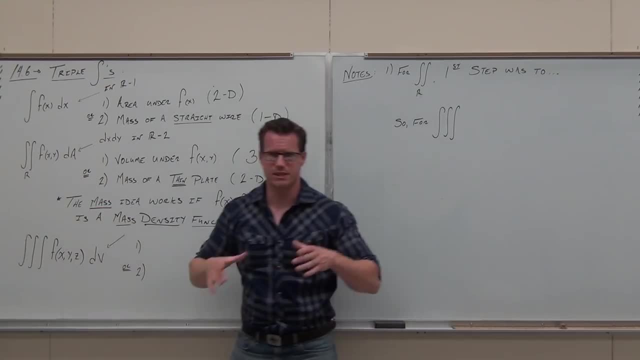 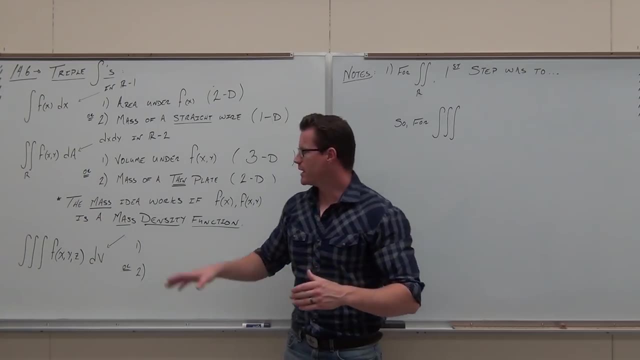 then the integral over that region of that mass density function will tell you the mass of that really thin plate. Are you guys getting the picture of that? That was that 14.4 idea. Now let's look at what a triple integral could give us. 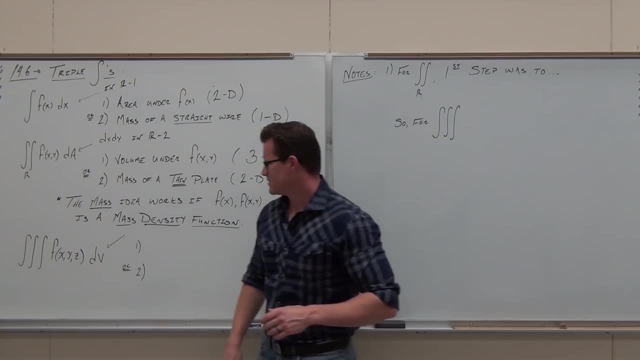 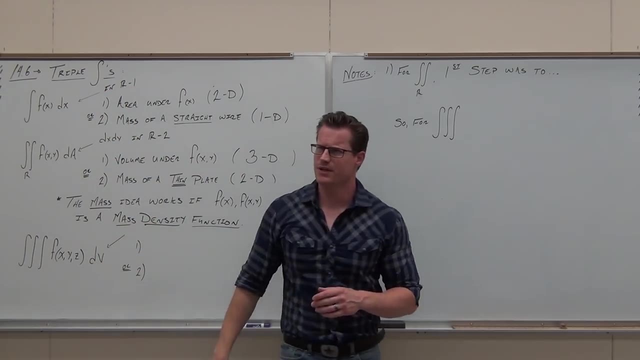 Firstly, what's dv? If this is dA, it was across two axes and this is dx across just one axis. what's dv going to? what's that going to give us? It's going to give us all three: the x, the y and the z. 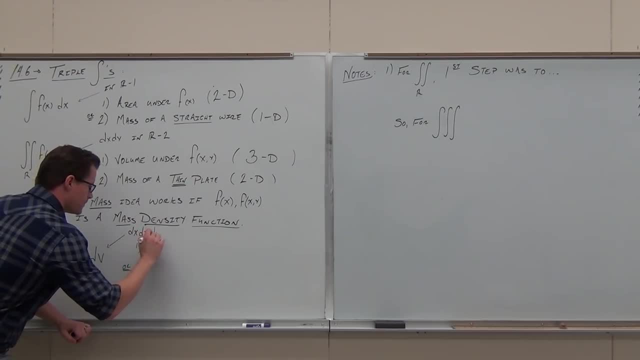 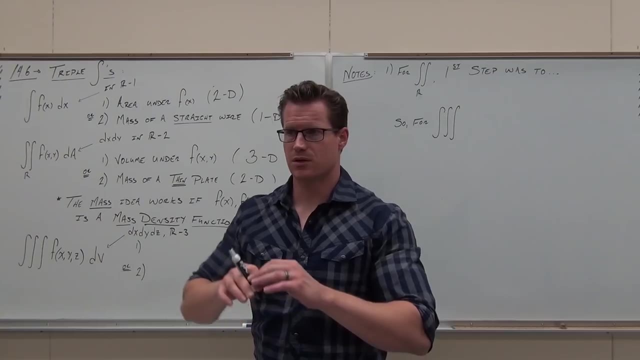 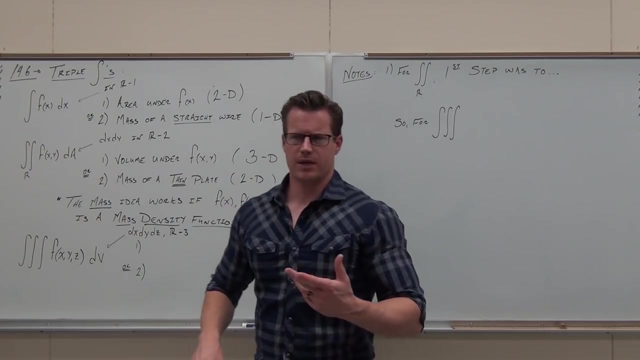 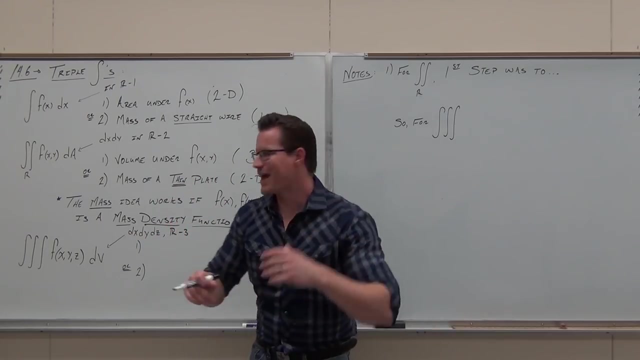 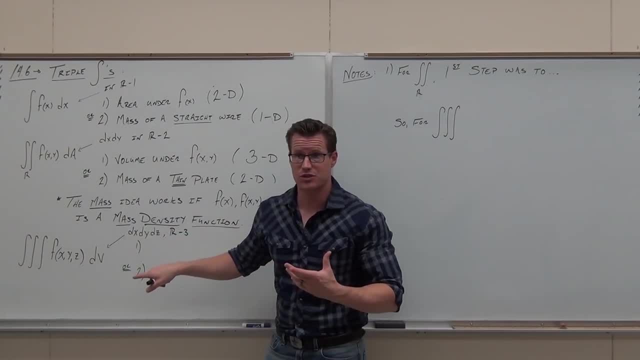 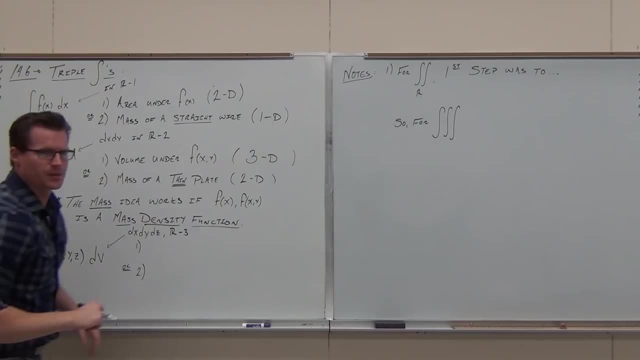 Here the region is what dimensional or three dimensional It's got to go over. some region in R3, some region in 3D. We call that region typically T to distinguish it from R. R would be a region in 2D, T would be this region in 3D or R3.. 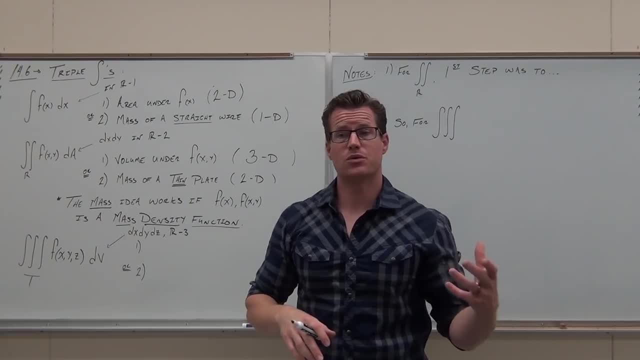 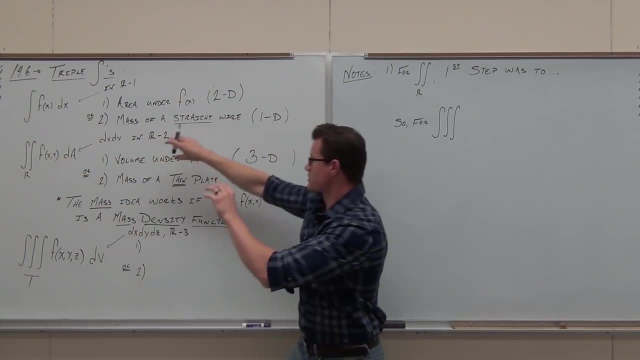 Shobhan's feel okay with that one. Well, the triple integral can still give us two things. Just like this integral can give us area, just like this double integral can give us volume, this triple integral could give us a measurement. but here's the problem. 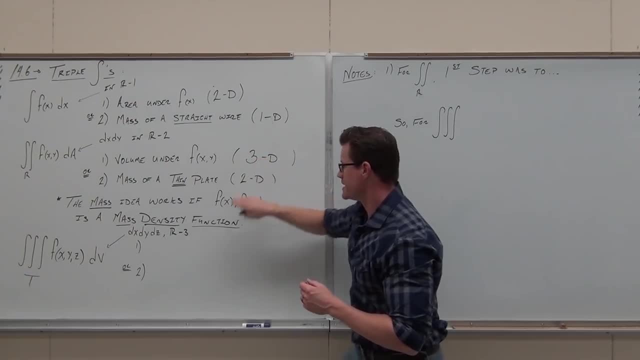 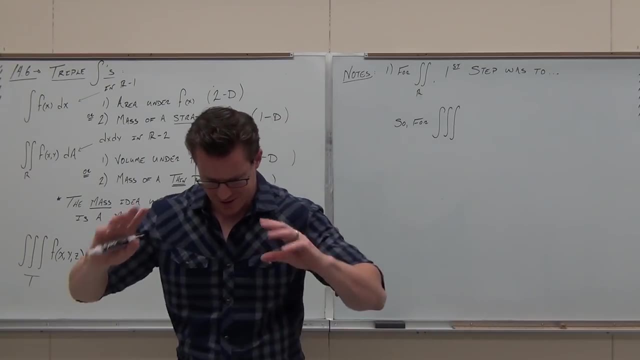 If this area is in 2D and this volume is in 3D, this measurement of region is going to be in 4D. So it could give us some measurement of this thing, this region under f of x, y, z, but it's a 4D concept. 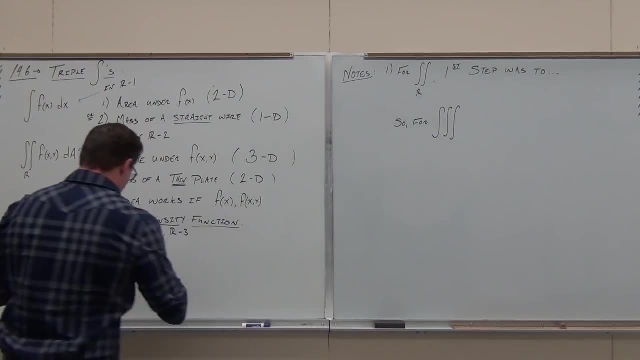 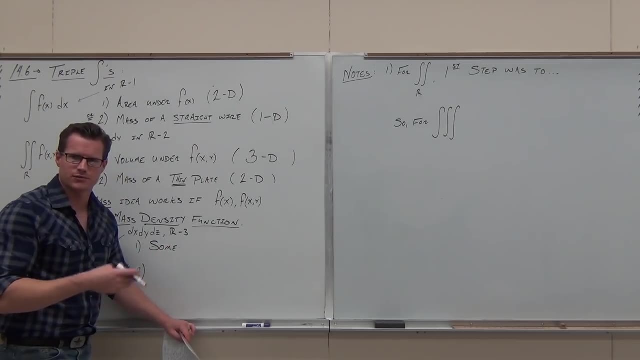 So it could give us that. So number one thing this could give us- can't quite call it volume, because volume has a connotation of 3D, but it would give us some measurement of the region under f of x, y, z. 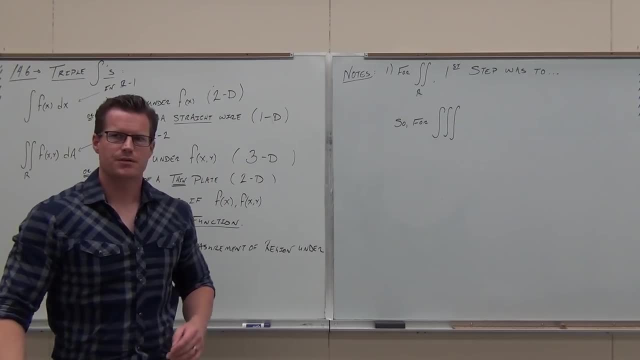 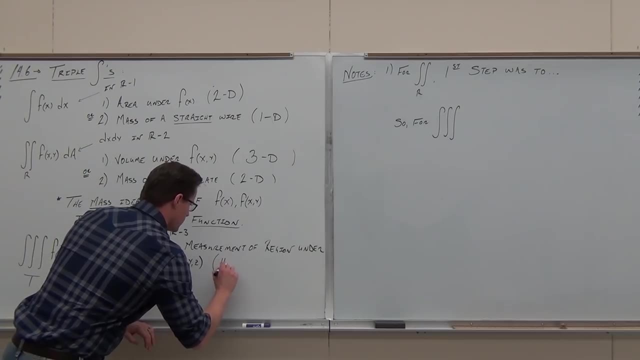 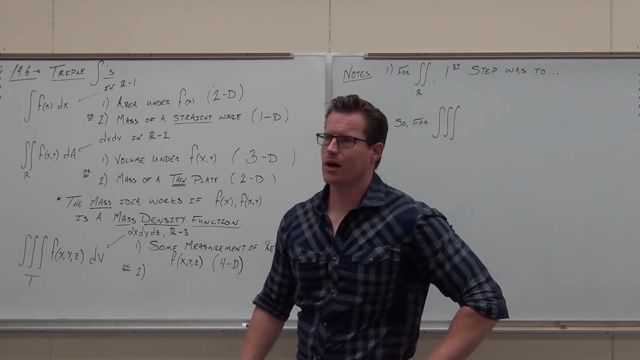 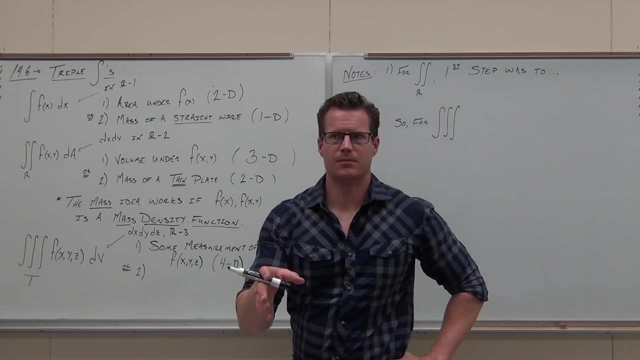 But the point is that that would be a 4D concept and that is super hard to imagine. That's one option. By the way, we don't in this class. we're not going to jump down and just go straight for integrals. 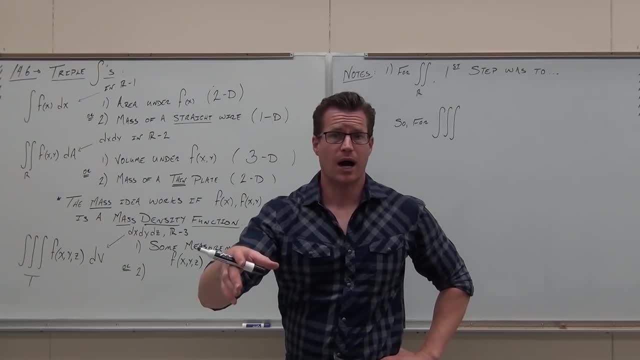 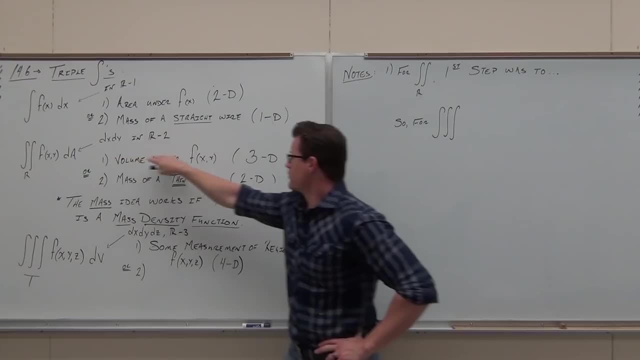 We don't do that. We learn what these things are before We start them, So I need you to actually understand this. Do you understand that? this could equal area- 2D concept. This could equal volume- 3D concept. 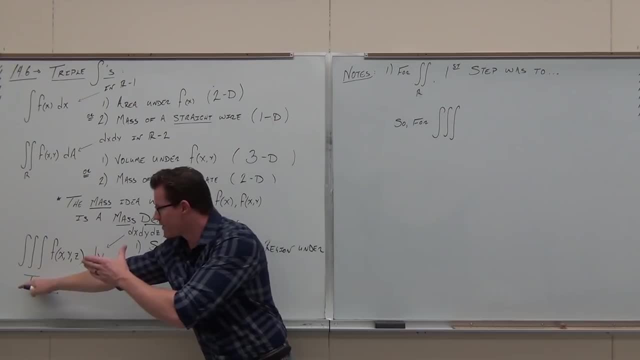 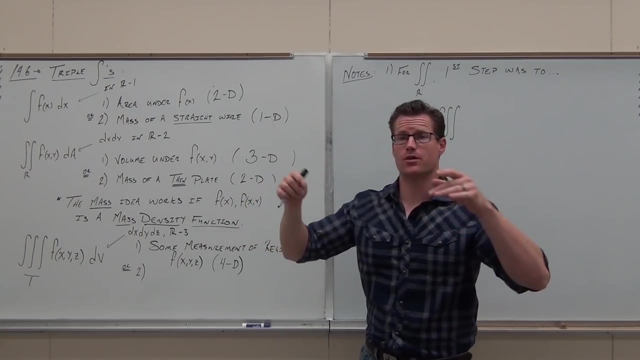 This could equal some measurement under the function over a 3D region, but it would be a 4D concept. Had not that you understand the idea. Now, that's super hard to imagine, So let's consider it the other way. 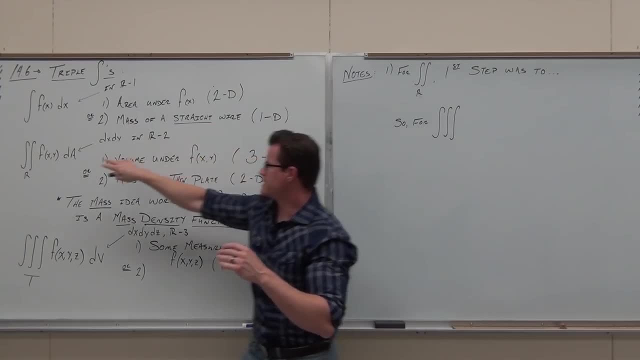 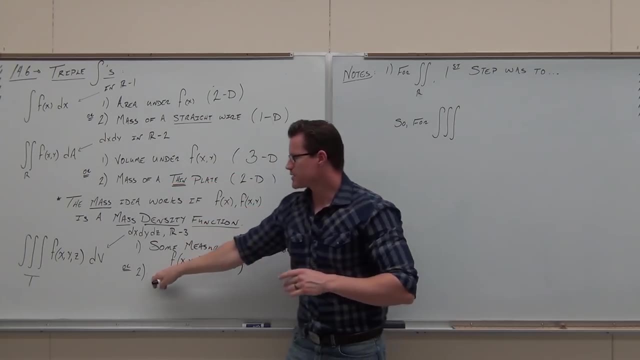 If an integral could equal the mass of straight wire, a double integral could equal the mass of a thin plate. That's a 2D, That's a 1D idea. Then this could also equal a mass idea. Do you guys get where I'm going with this thing? 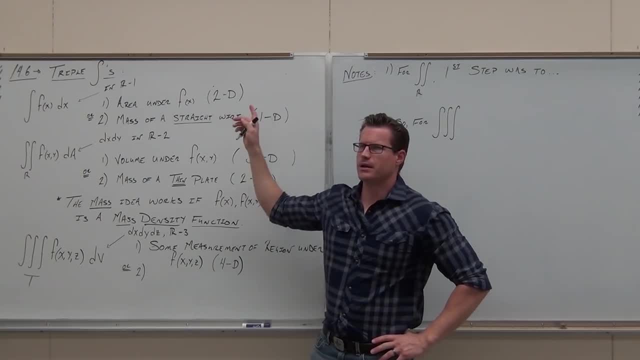 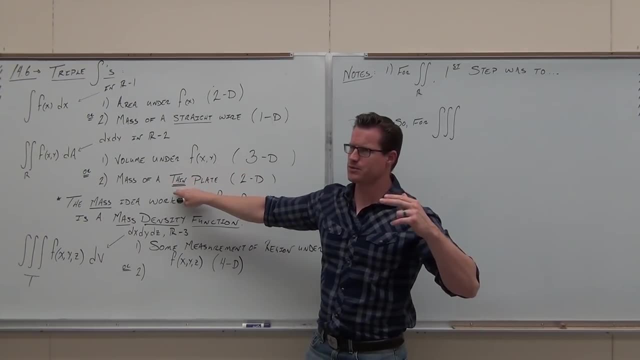 This could equal the mass of a. well, now wait a second. A super thin straight wire, that's 1D. A super thin plate, that's 2D. What would that be? Mass of a plane. Mass of a. this would be a plane. 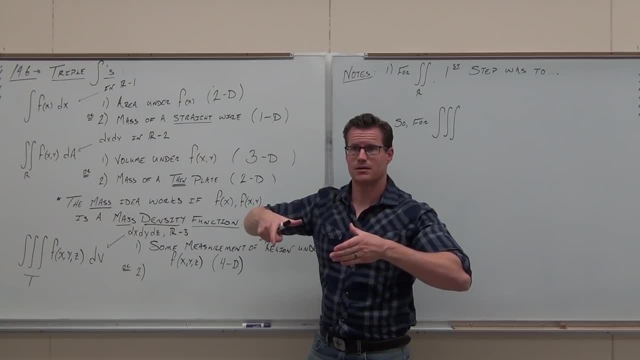 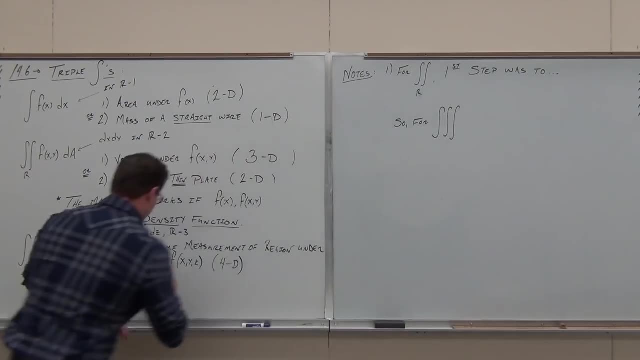 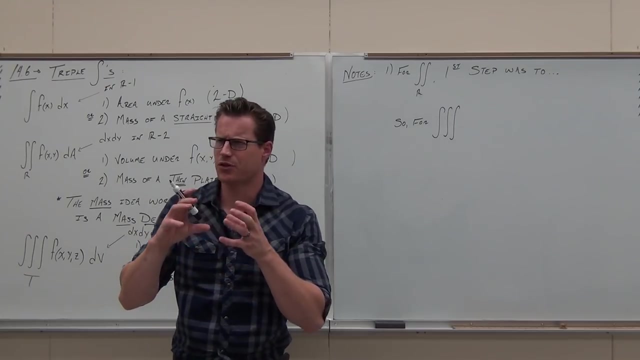 A super thin, A mass of a plate with thickness surface. That's what we're finding: Mass of a surface. Does that make sense? I'm going to call it mass of a plate with thickness. so you have this idea of a 3D region. 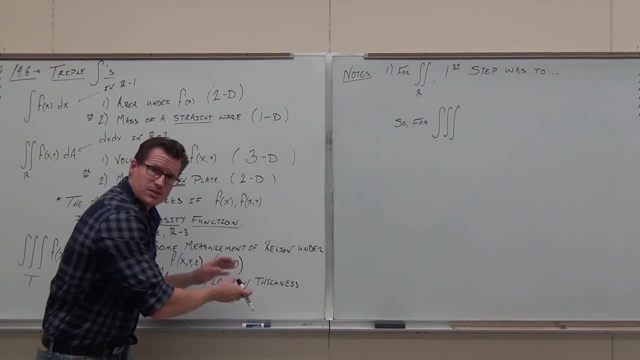 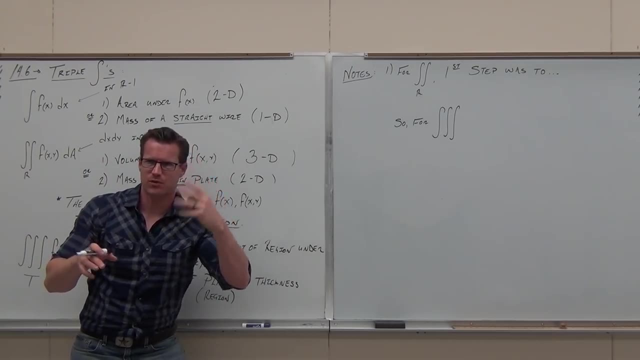 But the main point is this: If this is mass of a plate with thickness, mass of a region, what D is it? Is it 1D, Is it 2D, Is it 3D, Is it 4D? 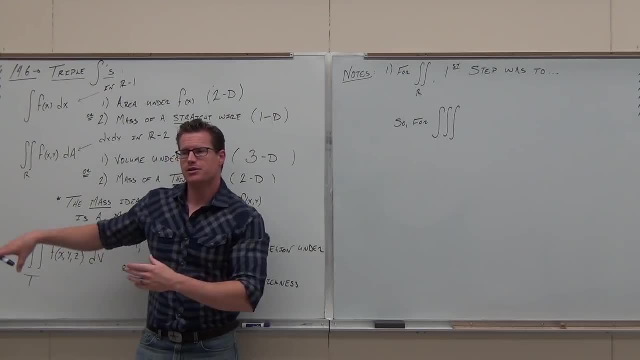 What is it? 3D, It's 3D. So basically this triple integral can represent the mass of a 3D thing. That's kind of cool, So it's something that's more real for us, Rather than imagining volume under a 4D surface. you're like. I don't even know what that means. 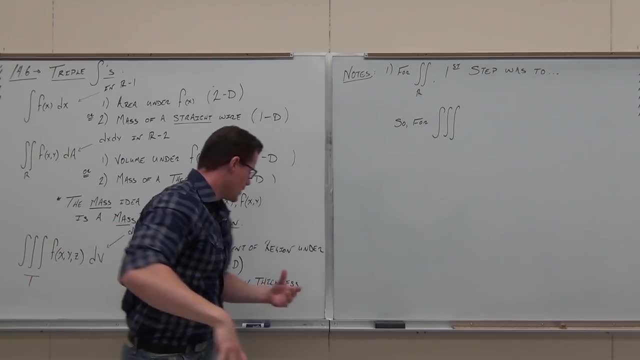 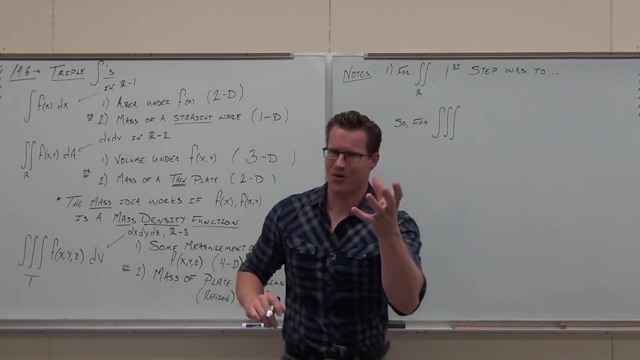 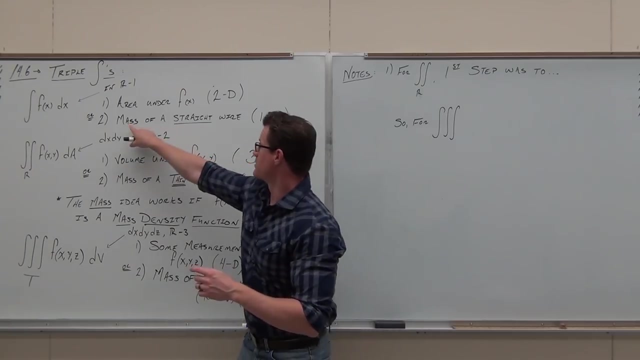 Well, if we have a triple integral, we'd also represent the mass of a plate with thickness, Some sort of region, And that's a 3D concept. But it only works if f of x, y, z represents what. This only represented the mass of a straight wire. if f of x- y was a mass density function, 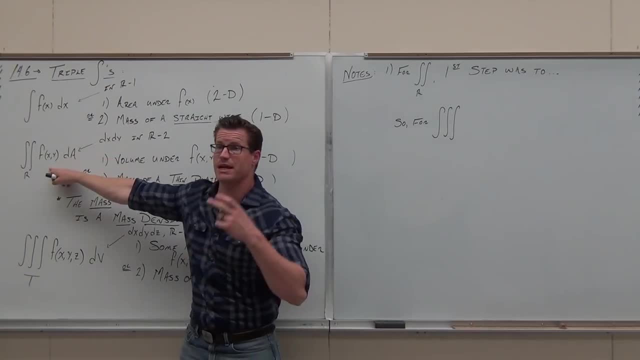 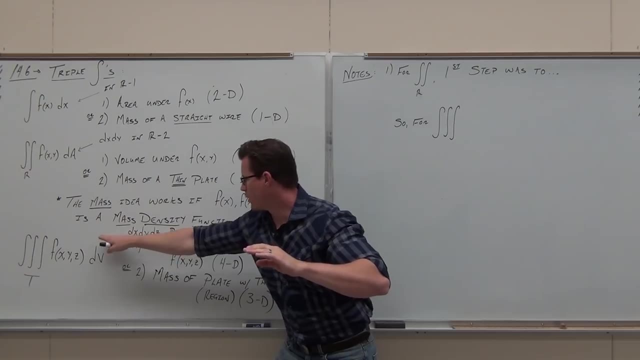 This only represented the mass of a thin plate. if f of x, y was a mass density function, Telling us the mass at any point along that thin plate, Does that make sense to you? This can only represent mass of a plate with thickness. 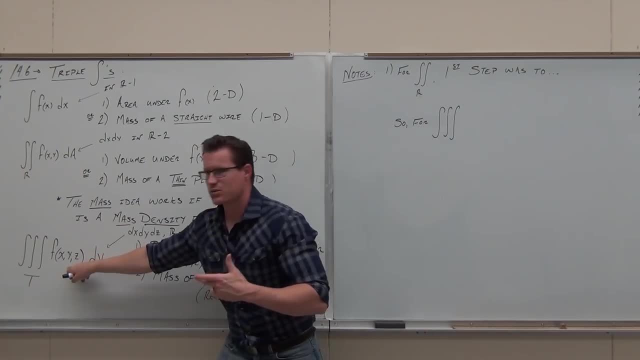 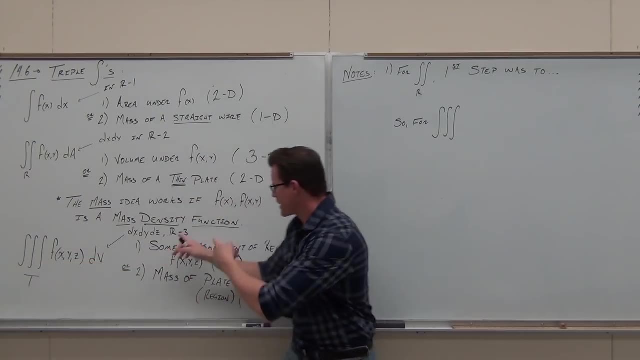 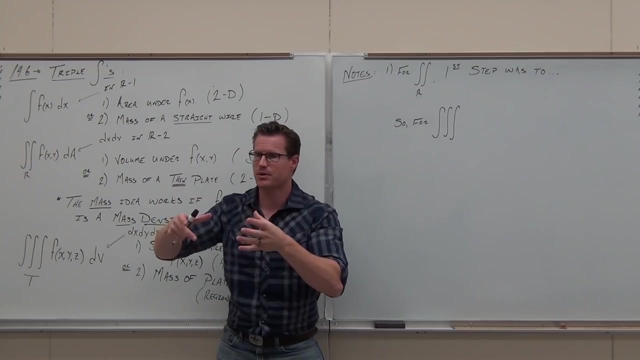 Or a region. That's a 3D concept. If f of x, y is a, what? Notice what it says: Look, look At any point in 3D space. That's why we have that R3.. At any point, f would tell us the mass of that 3D shape in space. 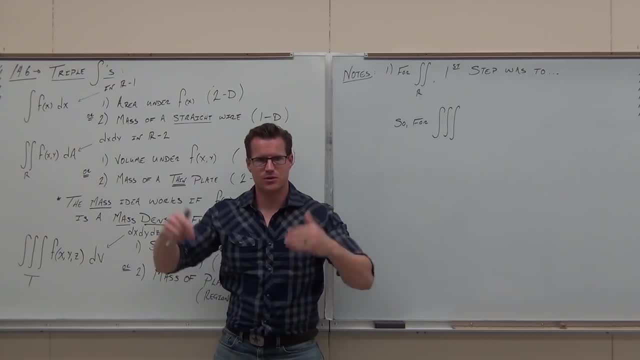 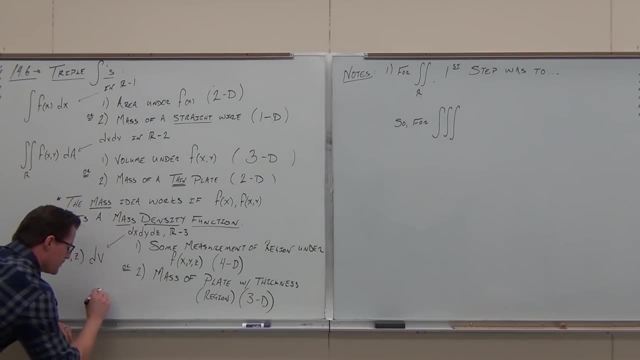 Anywhere along that 3D concept. Does that make sense? If I do the triple integral, it's basically adding up all the masses. That's what that's doing. So this works if- If that function is a mass density function. 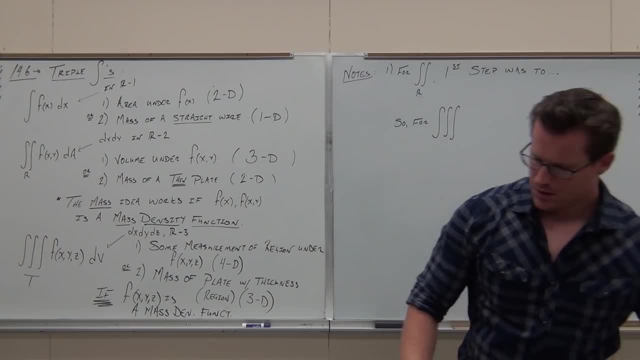 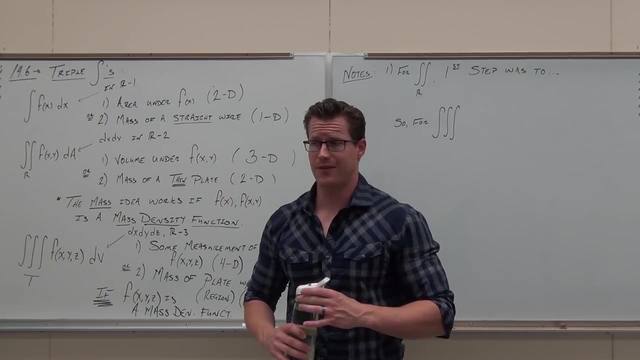 If that function is a mass density function. I'd love to just pause right there, Because- Because We're about to just get through the rest of our notes And go right into examples as fast as I can, Because I want to make it real for you. 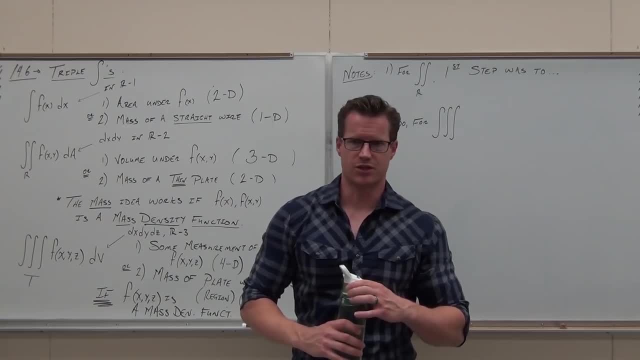 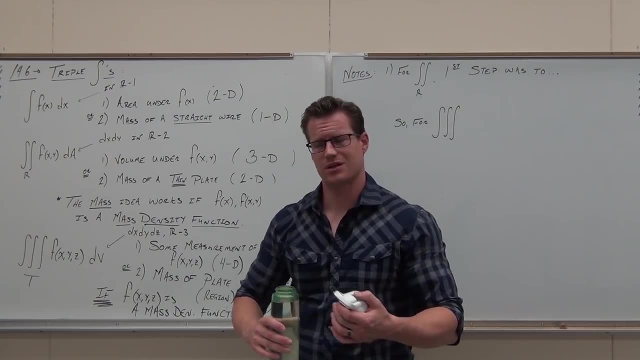 I want to show you. I want to show you more how to do it Than just explanation. I want to get right to it. It's honestly not that horrible of an idea If you understand single integrals and double integrals, triples. 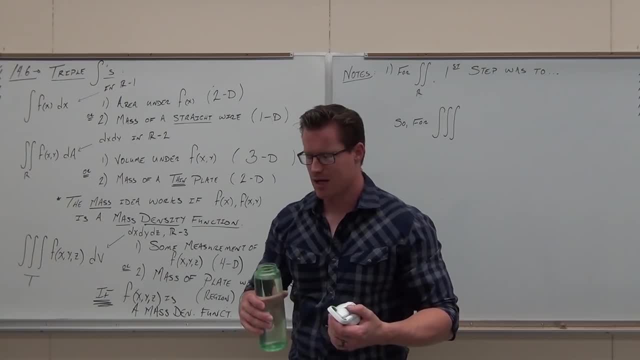 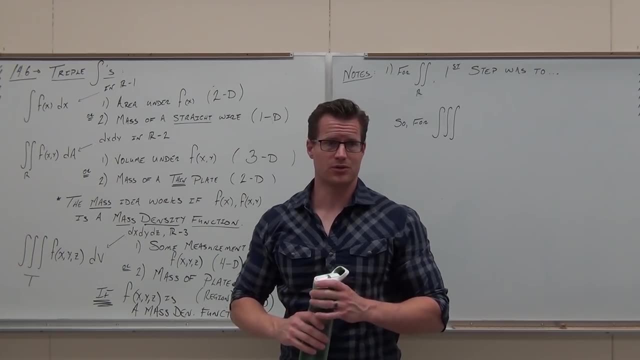 It's just one more step, But I do want to make sure you get the concept. Sometimes We, as teachers, think Y'all understand everything And we jump right into what triple integrals do And not what triple integrals represent, And that's a bad way to do math. 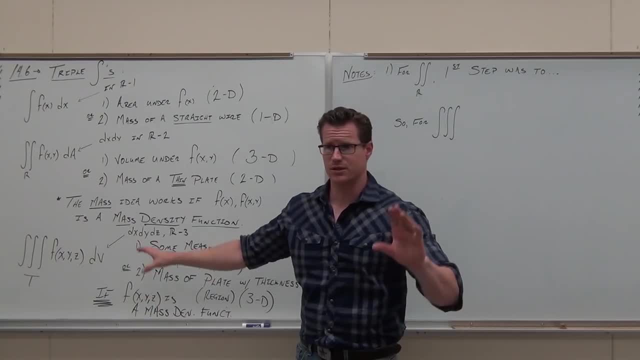 So I want to make sure that you fully understand this before we go any further. Okay, So let's go through it in like a 20 second, 30 second recap, And then we'll continue. Integrals can represent one of two things. 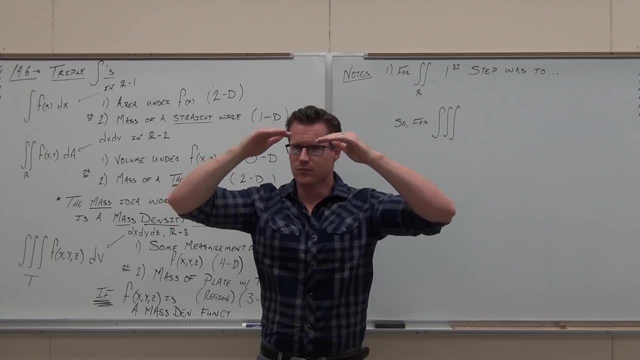 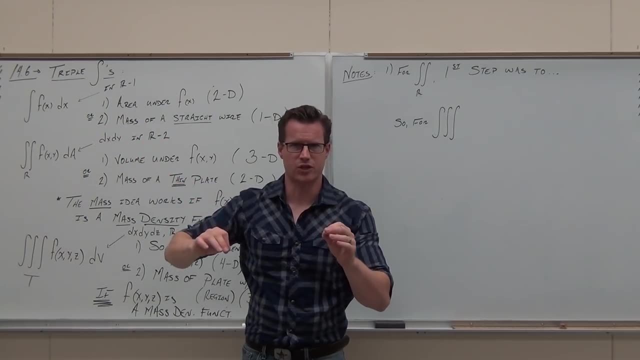 They can represent a volume area idea Or they can represent a mass idea. Every time you jump down to a mass idea, you lose a dimension. So with single integrals, area is 2D, Mass is 1D. For double integrals, volume is 3D. 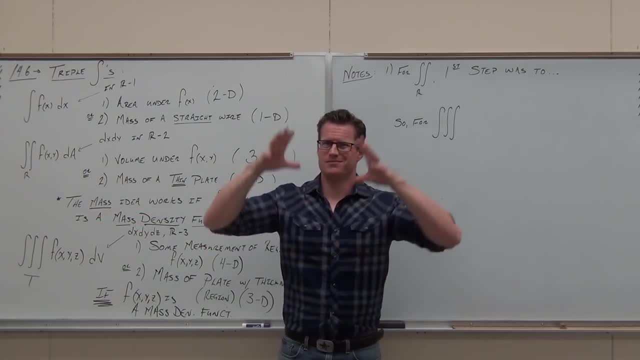 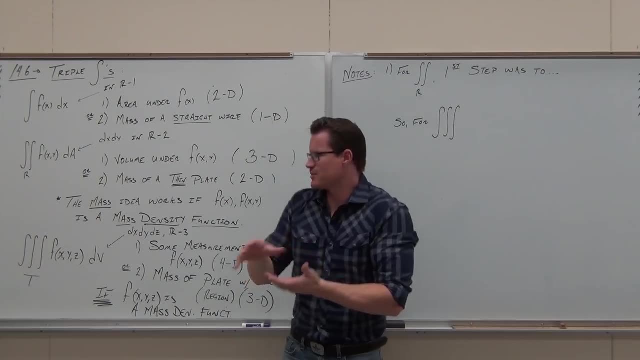 The mass would be a 2D idea For triple integrals: the volume, the measurements of 4D, the mass is 3D. Mass of 3D things makes sense. We have. it actually makes more sense than mass of 2D things. 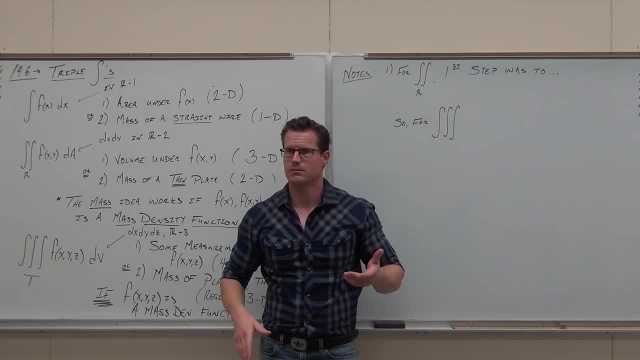 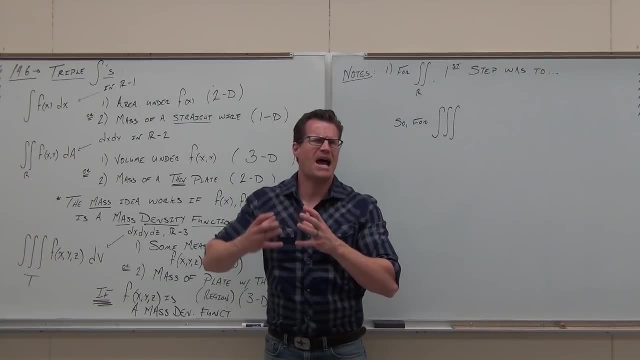 You ever seen a plate without any thickness? Neither. Now we can use it to find like charge densities and things like that, So it is very useful. But if we're talking about mass itself, mass typically comes in three dimensions, doesn't it? 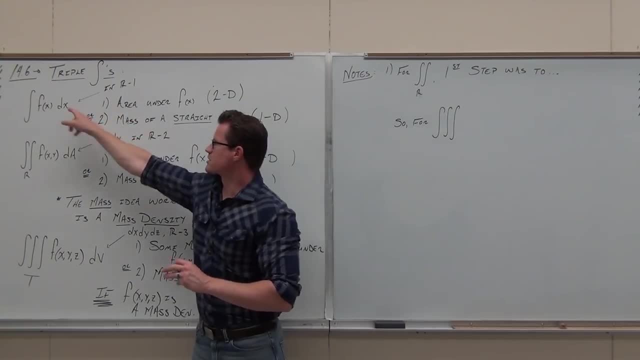 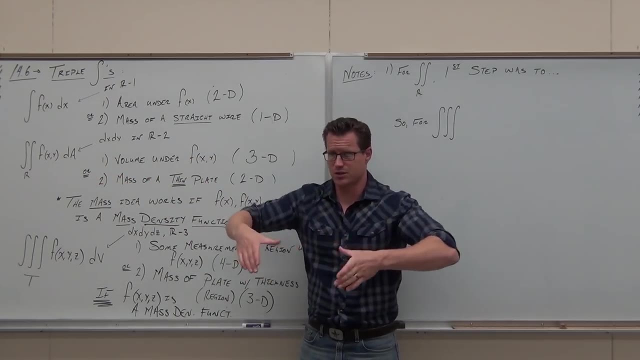 So what this says is: hey, the mass along this straight line would give us mass at every point in 1D. The mass along this thin plate would give us mass at every point along 2D. This says the mass density function would give us mass at every point. but now it's 3D. 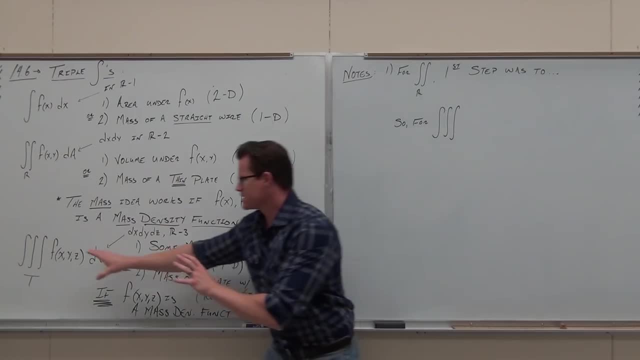 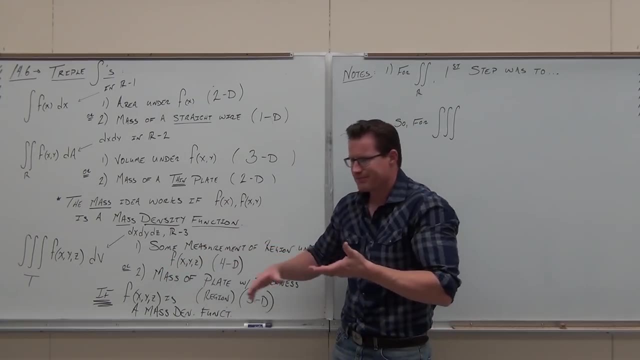 And it would add them all up and find the mass of the region in 3D. This is typically how we think of triple integrals. This is really really hard to think about The measurement of some 4D region under f, of x, y, z- we can't call it volume. 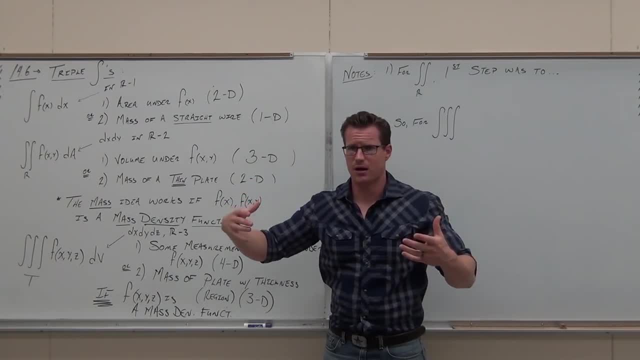 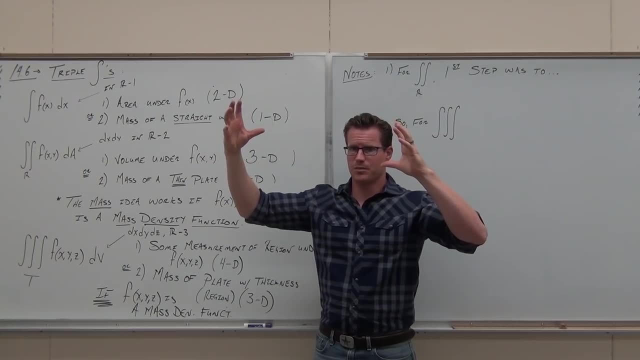 It's a dimension beyond volume. It's super hard to think about. Does that make sense? You can blow up a balloon in three dimensions and see the expansion of volume. Can you blow up a balloon in four dimensions? Well, it's hard to visualize that. 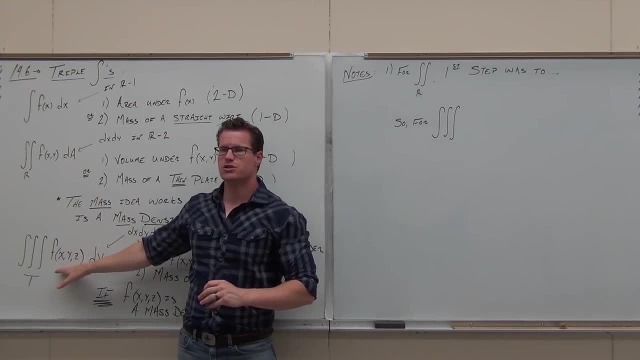 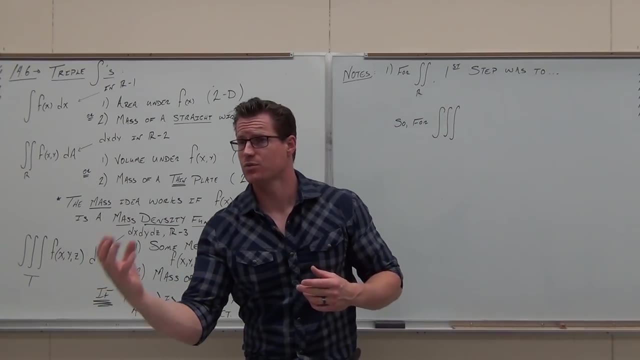 So instead we say, yeah, you know what. we're going to consider this function to be a mass density function, and so what are we going to be doing? What are we going to be doing with triple integrals? What are they going to represent for us? 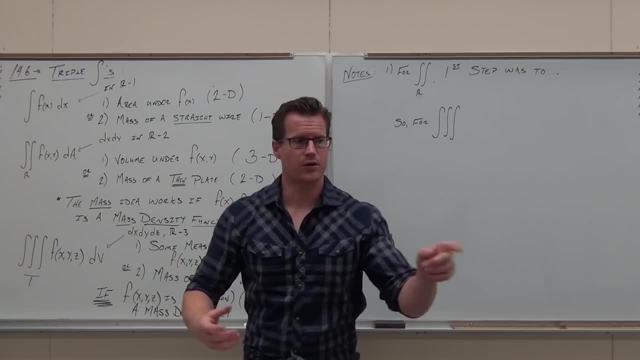 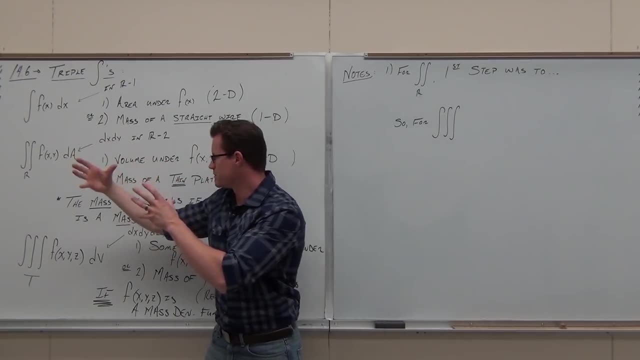 What do they represent? Mass Volume, Not volume. That would be double integrals. That's a volume idea for here. Volume under the function. The function is 3D or mass of thin plate, So we're going to think of this as a mass idea. 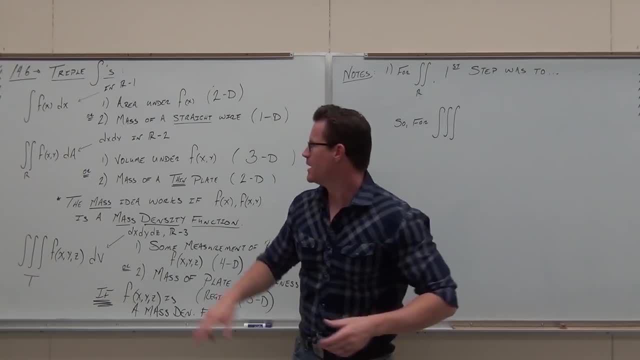 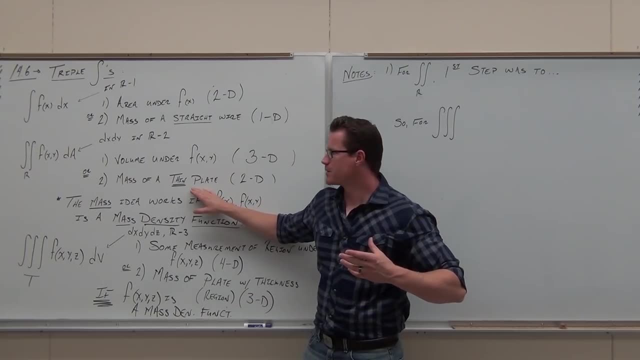 But what mass is it finding? Look carefully, I need you to get it. This is the mass of the thin plate, right? How is the thin plate defined? The thin plate is defined along that region, over that region. Look at this. 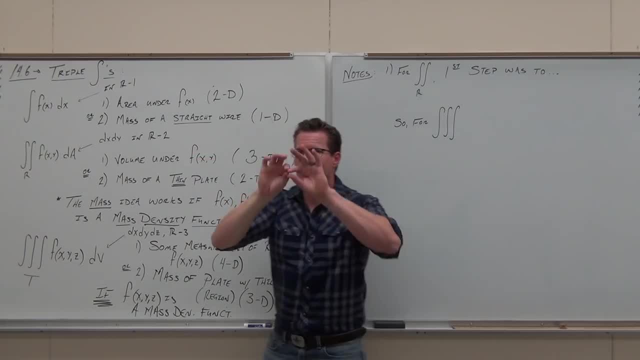 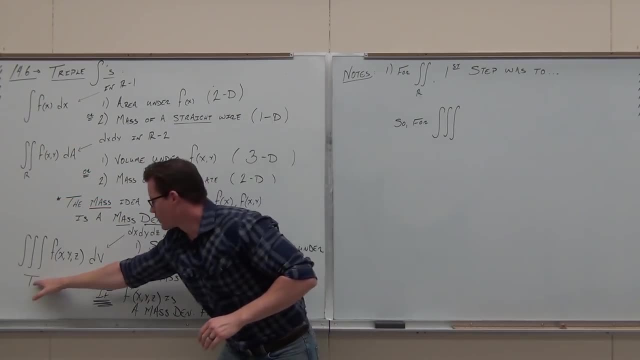 This is the mass of a straight wire. How is the straight wire defined? It's defined as a distance along the x axis, Just over a region, over a three-dimensional region. So what this is finding is going to be the mass of that region. 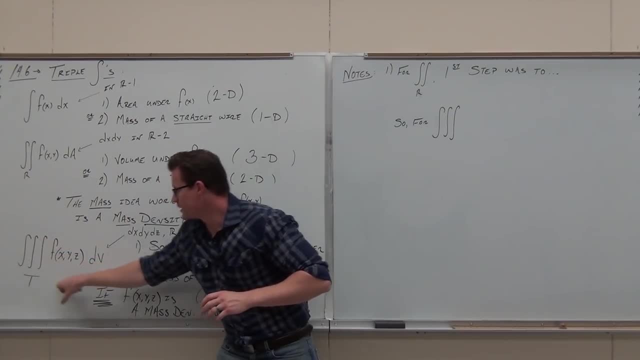 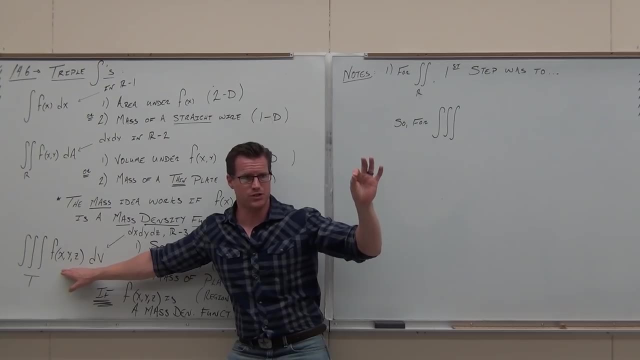 So whatever that region is defined as that 3D region, this triple integral is going to find the mass of that region, if this is giving us the mass density at every single point of that region. I know it's a weird concept, but you guys get the concept. 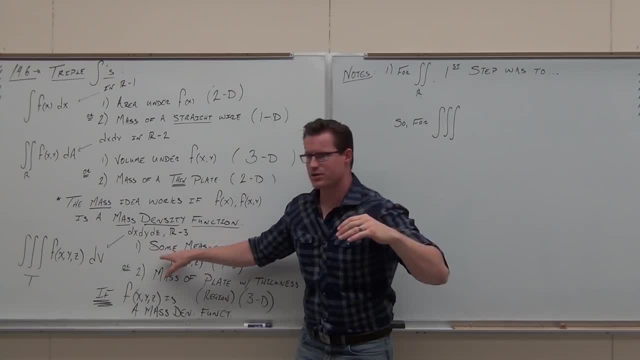 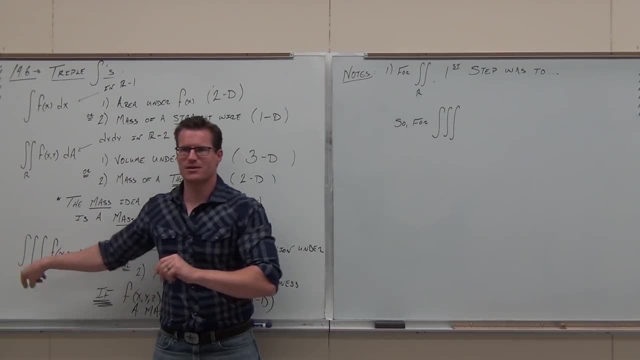 Are you sure? Do you understand the idea that this is really hard to describe, the 4D stuff, So we think of it as a 3D. If that's mass density, then what this does? it says, hey, find the 3D thing that you got. 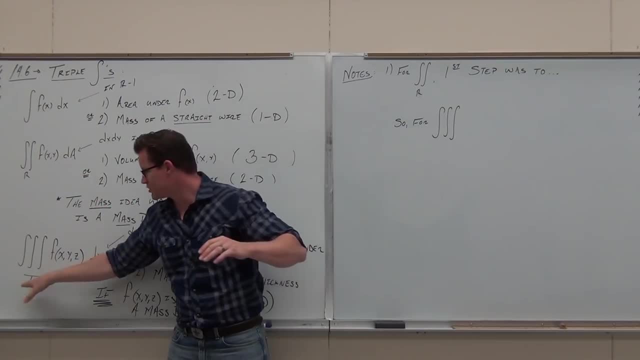 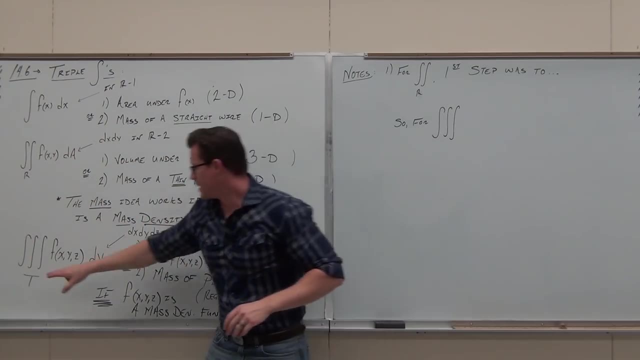 Is it 3D? Of course it is. It's x, y, z. It's going to be in 3D. This region will be in 3D, just like that's in 2D, just like that is in 1D, along the x, along xy, along x, y and z. 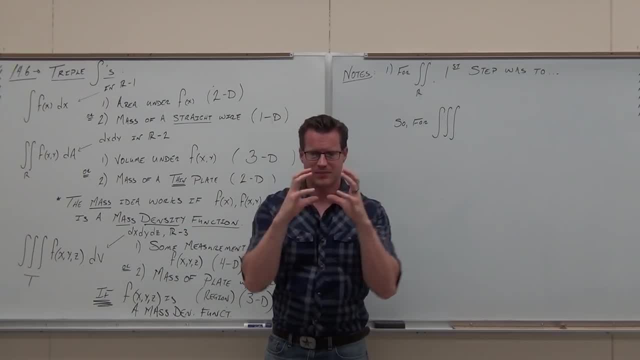 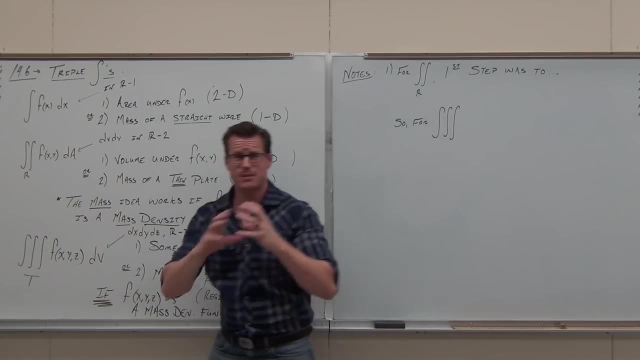 It has this shape to it, this three-dimensional shape to it, this region in 3D We call it T. What we're doing is saying: if this describes the mass density at every point in that region, then we can find the mass of that region. 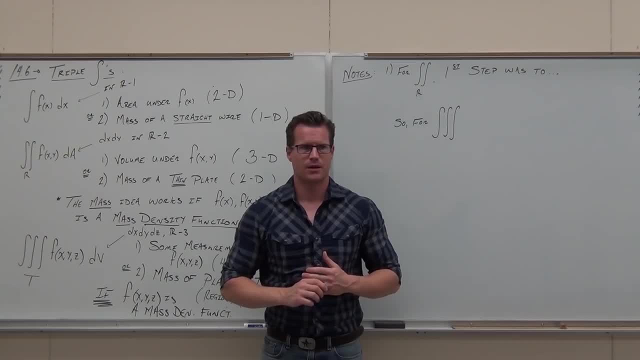 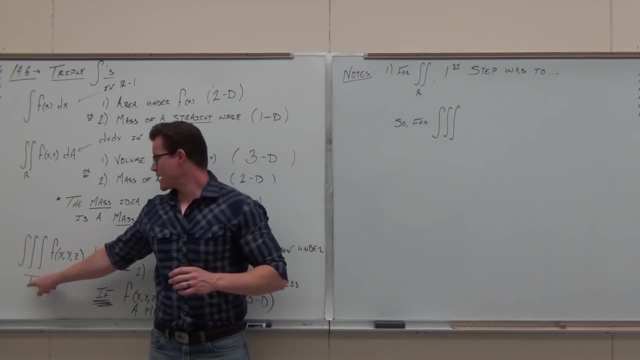 That's how we think of triple integrals. Head nod if you understand the concept there, Are you sure? So what are we finding? Mass of Whatever this region is, given that that gives us the mass density, every single point. Are you guys clear on that one? 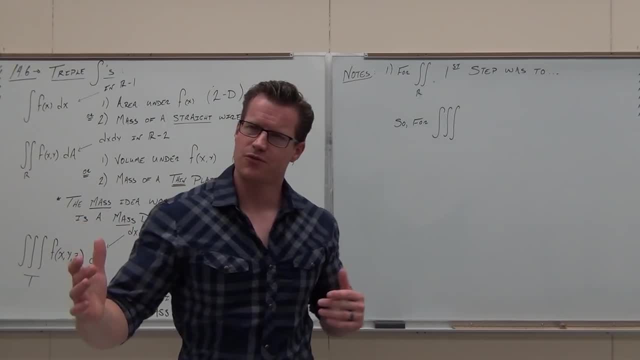 Okay, So here's some notes. We're now going to make the transition from our double integrals to our triple integrals. I'm going to make a couple of notes, I'm going to make the connections for you. So typically for double integrals, 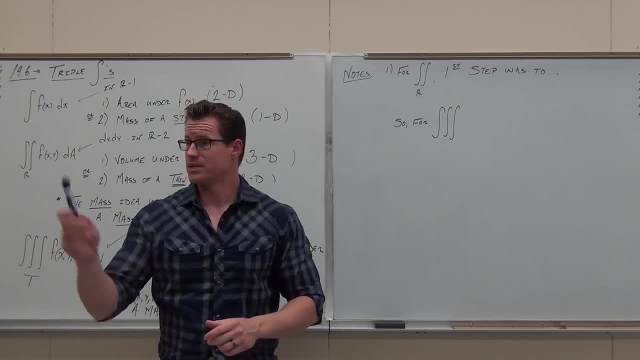 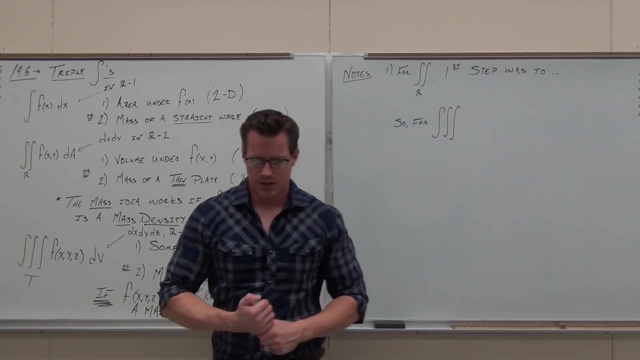 our first step was to do what We typically drew the region In 3D. we're not going to be doing that so much because it's honestly a little easier than that In 2D, or sorry for our double integrals. 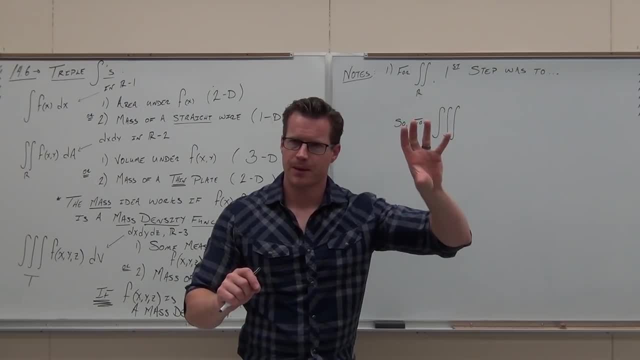 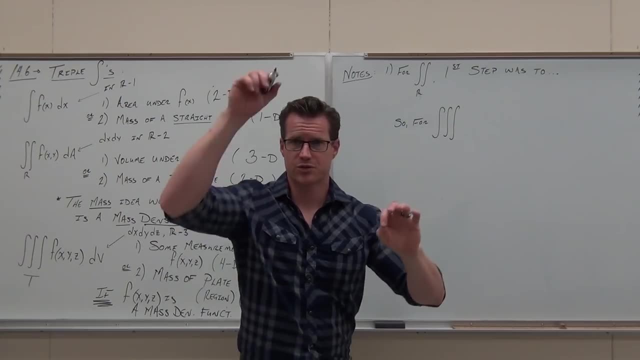 our first step was to define the region between two curves. You remember doing that. Yeah, some of you guys are going to be looking up here. okay, We defined a region, We drew our y, we drew our x and we said we're either going. 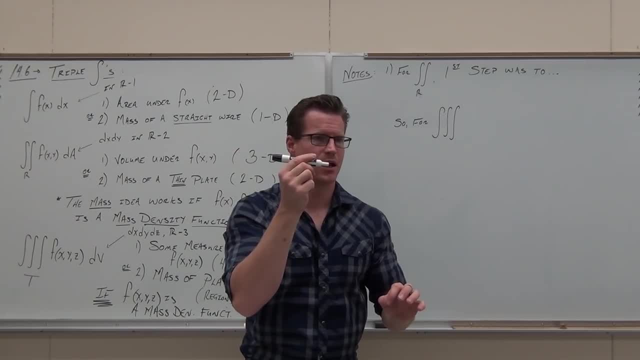 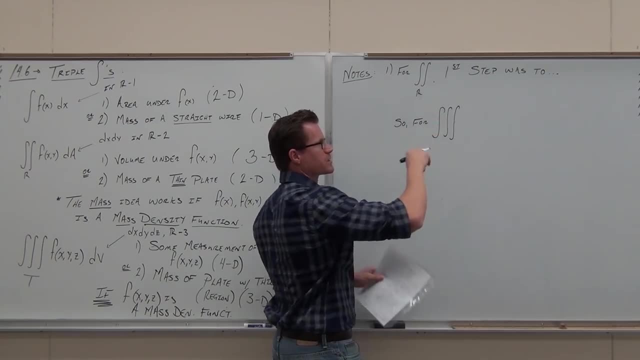 to do this or that. We're going to go along the y first, We're going to go along the x first, Remember that. But it was always between two functions, two curves. So for here, our first step was define our between two curves. 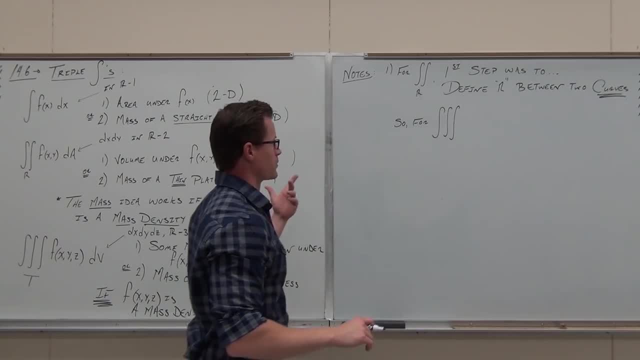 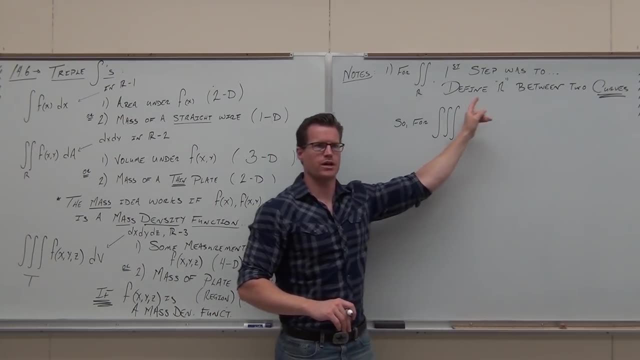 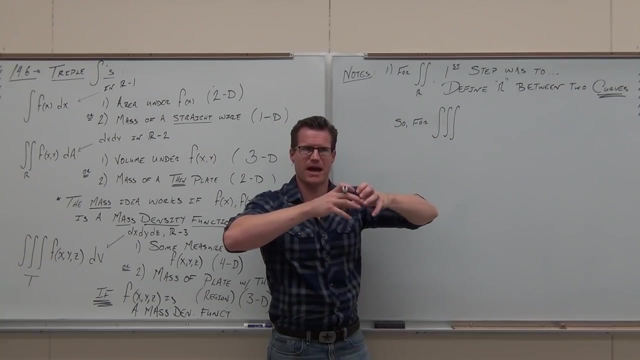 Okay, well, now for triple integrals. it's really easy to do this because your region is always on a plane. Verify that. verify that, If this is a plate and we're finding the mass of that plate, that plate was a really thin plate. 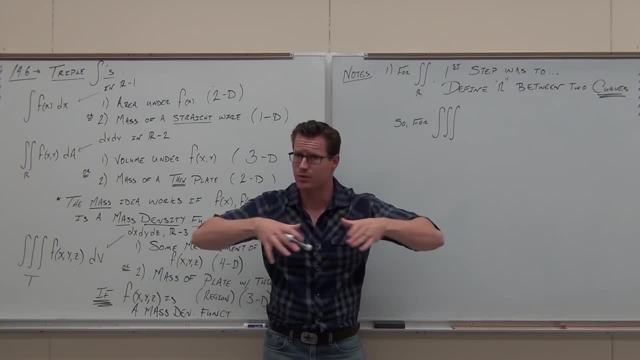 It was a 2D plate. You guys get that. It was a region that was 2D. It's really easy to define because you can draw the region on a plane. Now we have a region. We have a region that is in what's t. 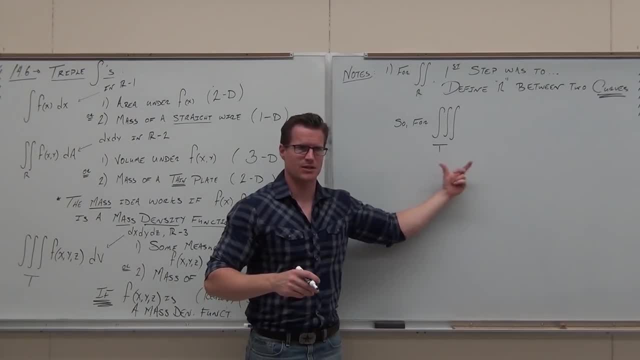 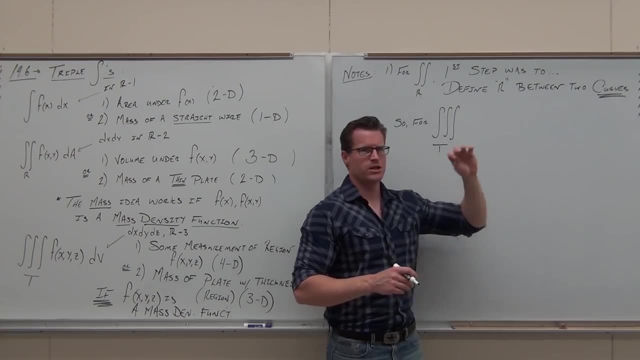 Come on, what's t? Think t equals 3D. That's what that means: That region's in 3D. So now I'm still going to define the region between two somethings, but they can't be curves. 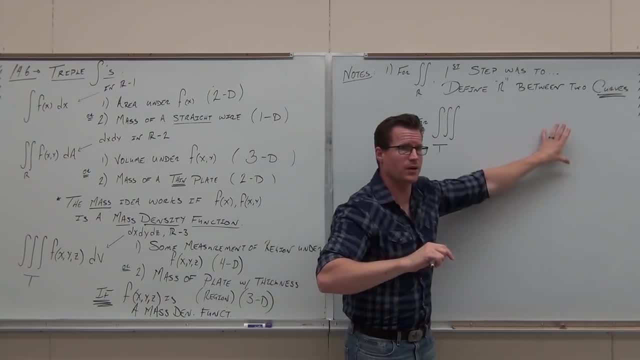 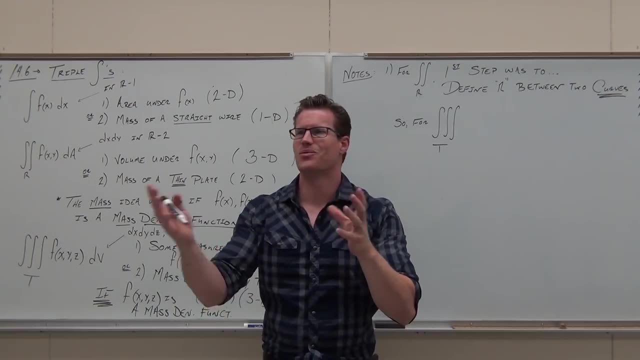 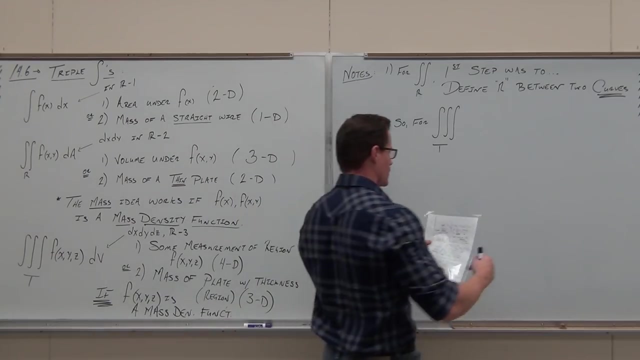 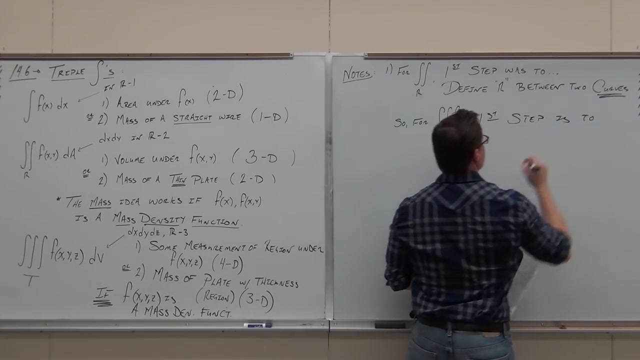 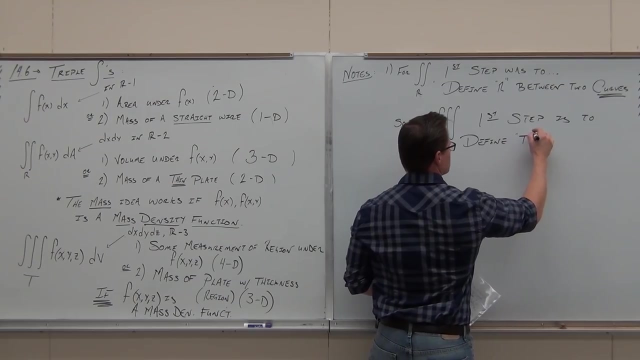 because curves are a 2D concept for us. They're on a plane. Right now, I'm going to try to define t as being between two. what Right surfaces? You're right. So that's our first step here. So now our first step is to define t between two surfaces. 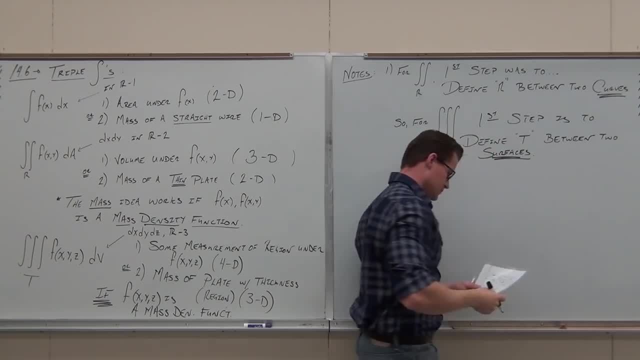 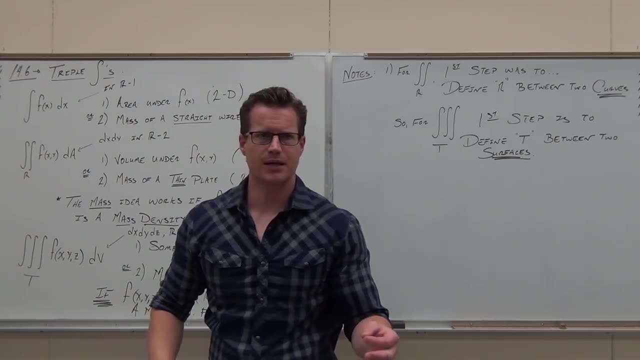 So now let's do this. You know, I hope that makes sense. I don't hope I need that to make sense to you. I need you to get the concept that when we increase an integral, like one to two to three, we're increasing a dimension. basically. 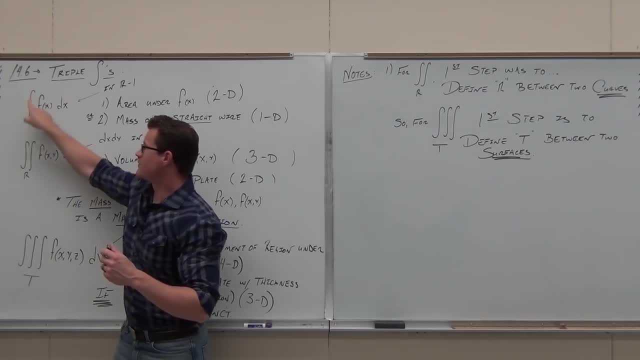 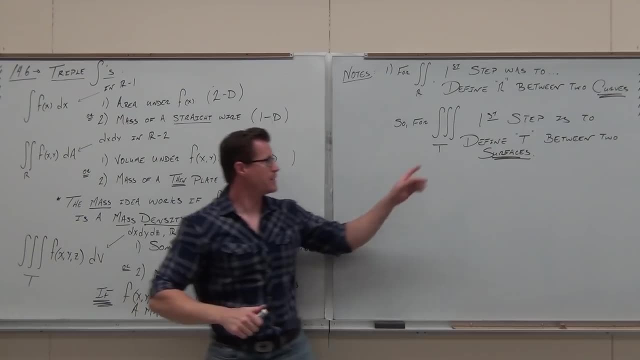 So think about this: These numbers travel along an axis, just between two numbers. This travels between two curves, along two curves. This, therefore, if I increase that, it's not going to be a 3D, It's going to be a 3D. 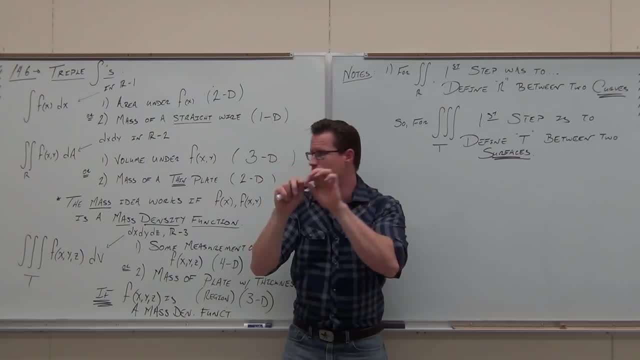 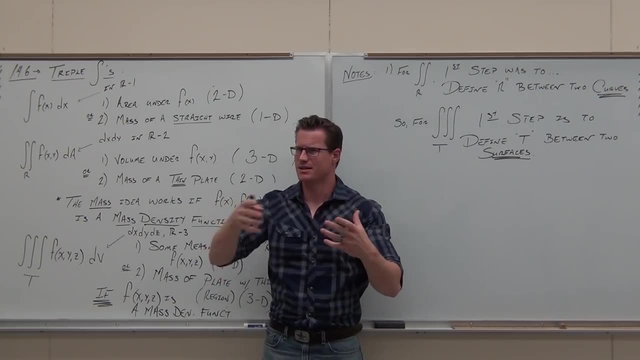 along the curves. it's now surfaces. So instead of going between two numbers, I went now between two curves on a region. Now I'm going between two surfaces somewhere in space. That's the idea. Do you guys see the extension of that concept? 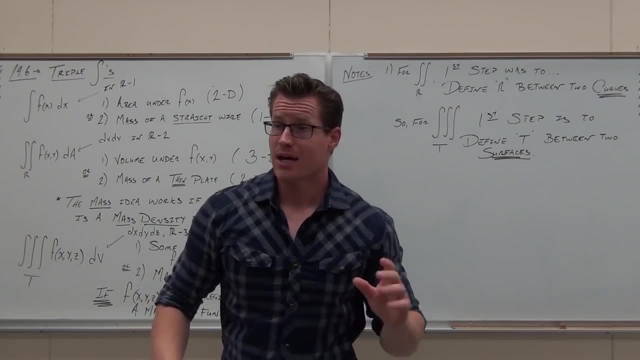 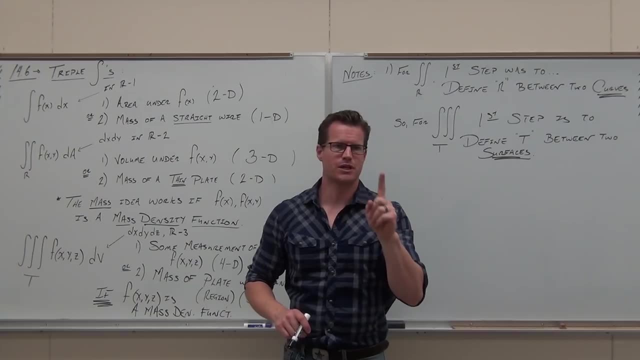 So. but there's a really nice thing about this: If you can do this, define T between two surfaces, that automatically deals with your first integral. How many do we have to deal with? Three, Three, Three. So if I take away one integral, 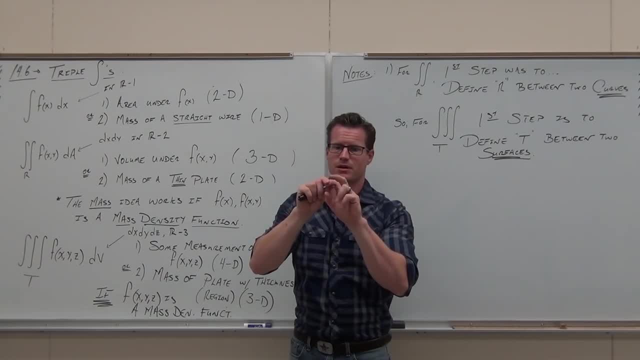 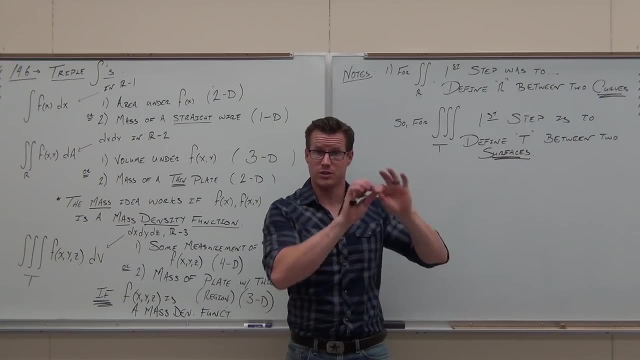 if I deal with it this way, how many other integrals are left? A double integral: Hey, do you know how to do double integrals? Yeah, So if you can define your first integral properly between two surfaces, then you're left with a double integral. 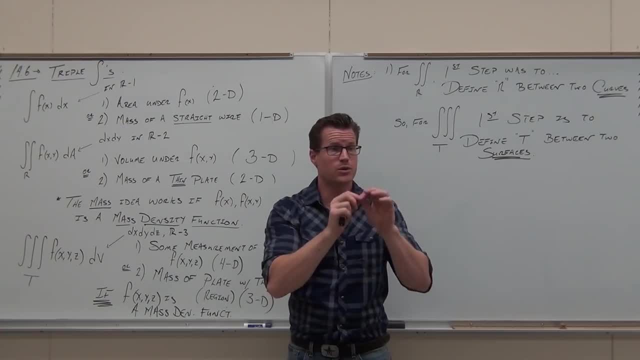 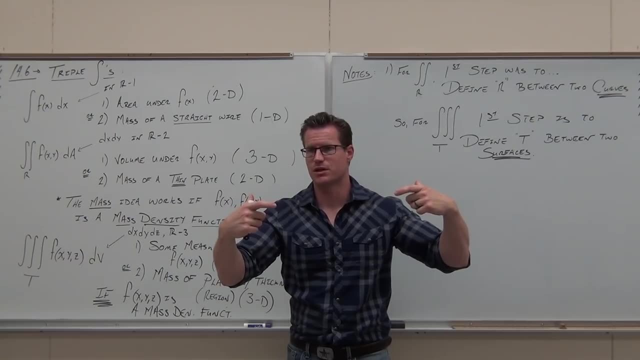 So this is literally just an extension of double integrals. Deal with your first three-dimensional region between two surfaces and then your double integral basically takes care of itself. Does that make sense to you? It won't make full sense until we do some examples. 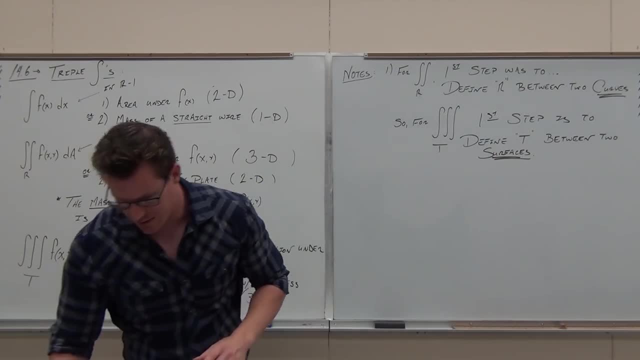 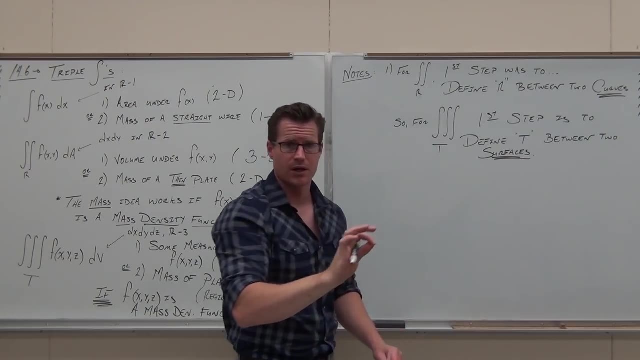 but I'm going to show you Right now. I want to write some notes out and make sure you all understand it, okay. So what this does? this lets you deal with your first inside integral first and then have a double integral to calculate, just like your. 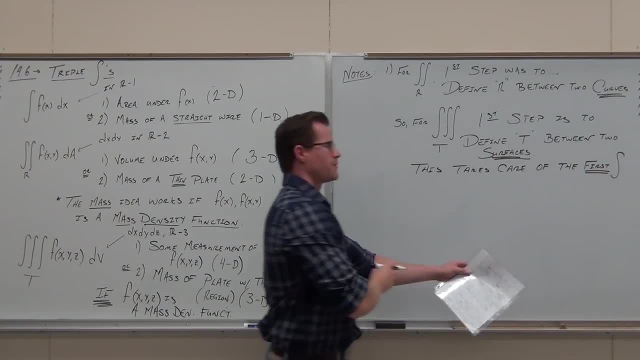 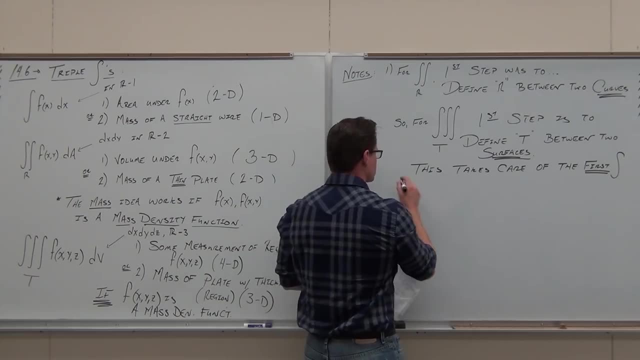 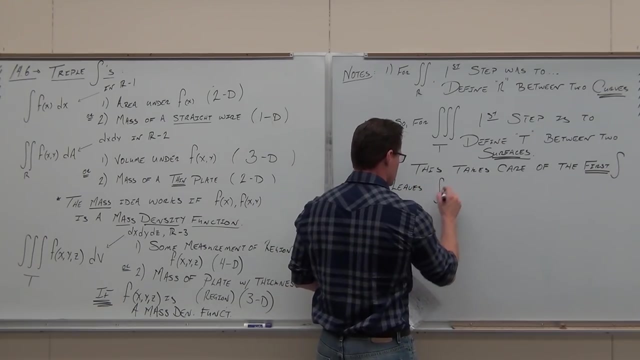 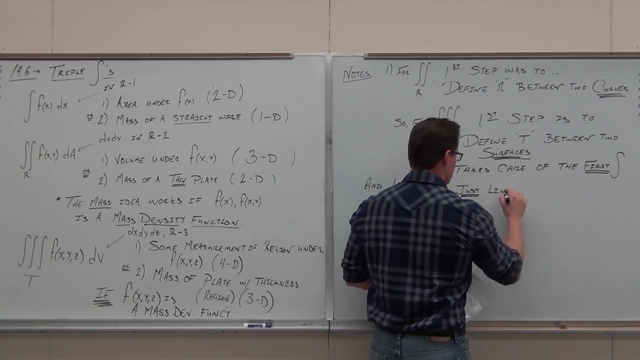 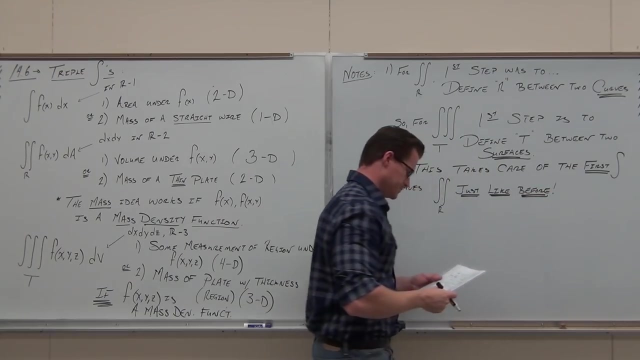 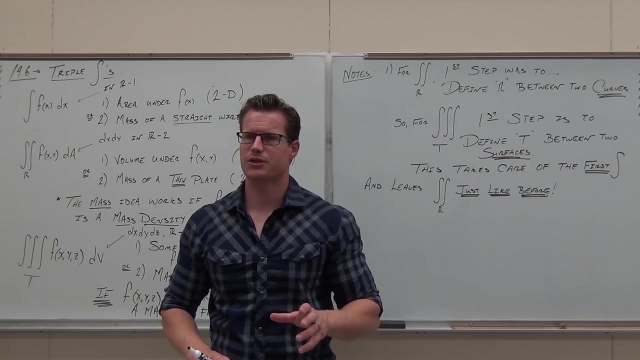 This takes care of the first integral and then it leaves a double integral over a different region, over r. There's only one issue that we are going to need to deal with. It's kind of a big issue and you guys are going to have a lot. 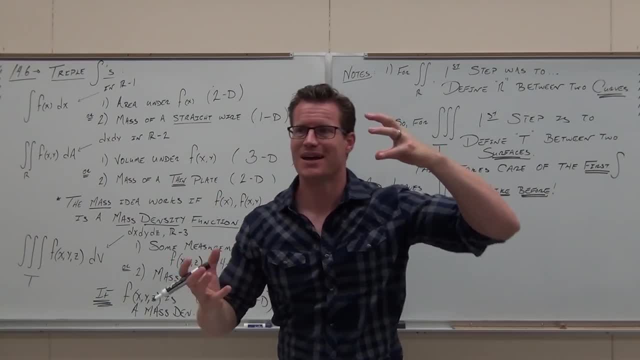 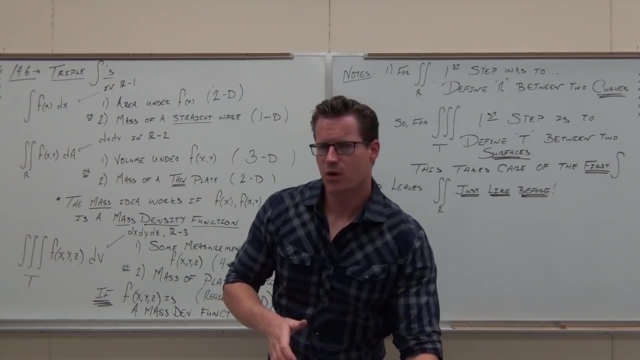 of like brain turning when you do this, but I want you to imagine this. please listen here real carefully. Please listen. With our triple integrals, if I'm going from a surface to a surface, I can choose to do that in the x direction. 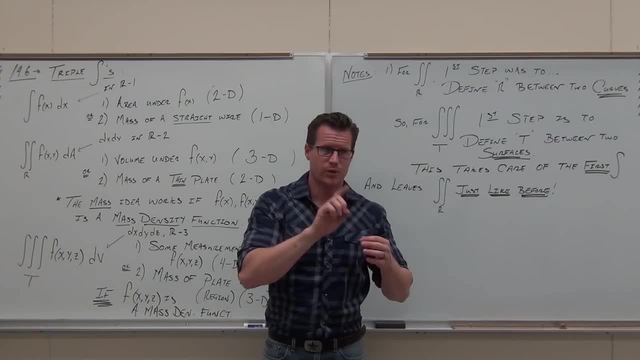 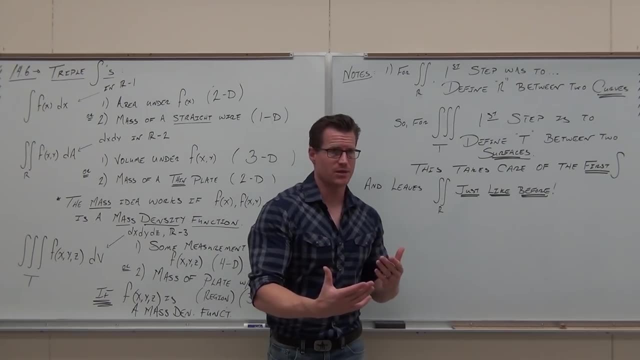 or the y direction or the z direction, Which means the double integral that I get. the region doesn't always have to be on the x? y plane We like it to be, but the region that we're going to get after we deal. 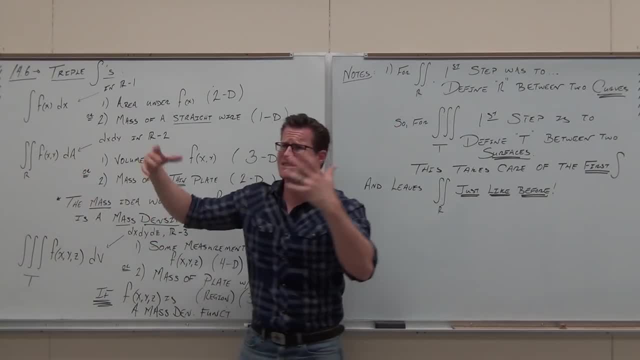 with the 3D concept, we're left with a 2D concept. Does that make sense? Just like double integrals? when you dealt with the 2D concept, you were left with the 1D concept. Do you guys remember that? 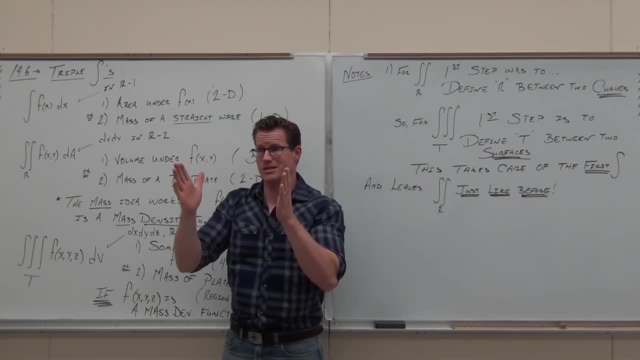 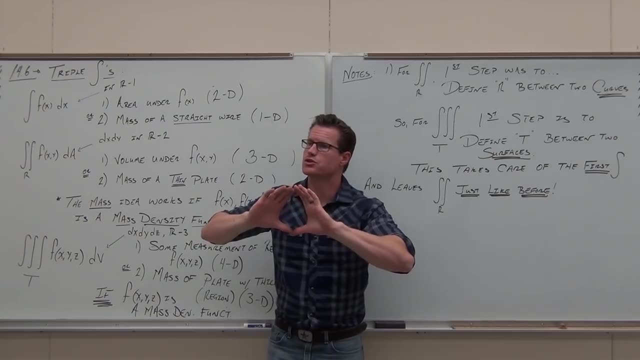 You take care of the between functions and then you're just going along an axis. That's pretty easy. Here you go between surface, then you're left with just going through a region. So we get this double integral again. Only the, the, the, the, you know. 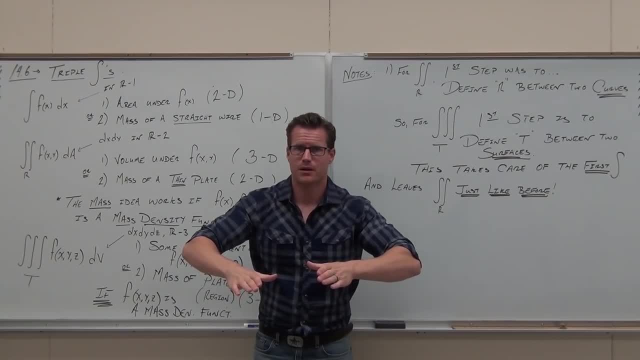 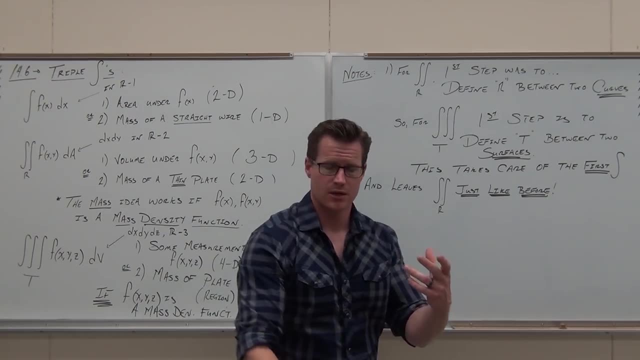 the region that we get. it could be on the x- y, It could be on the y- z or it could be on the x- z. So it could be on any one of those planes. It depends on what you pick to go across first. 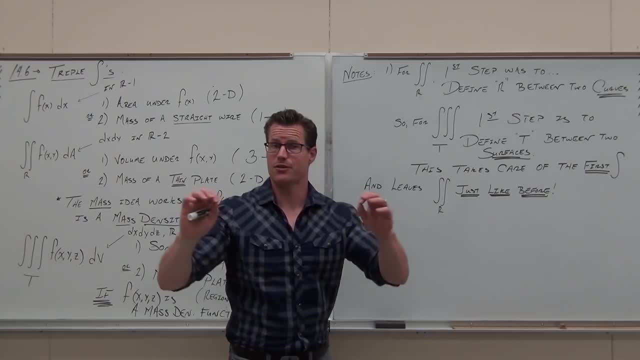 whether you do it in x direction, y direction, z direction. I know I'm throwing everything at you right now. You just have to wait until we do some examples and I will show it to you. But I need to get the ideas in your head. 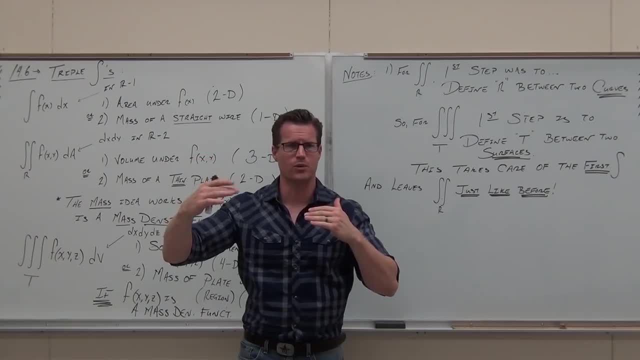 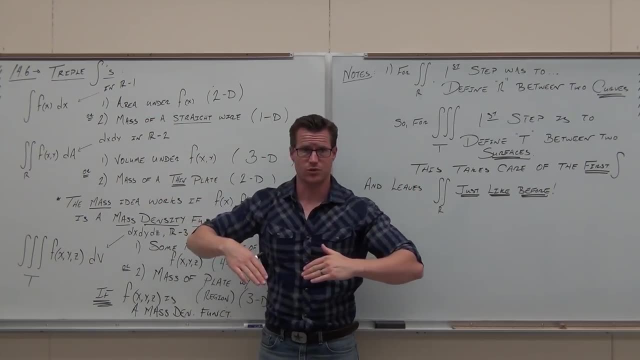 You guys understand I'm kind of front loading this. I'm trying to build an advanced organizer for you so that when we get there your schema aren't all screwed up. Okay, I need you to build these things in your head: that dimensions grow as integrals grow. 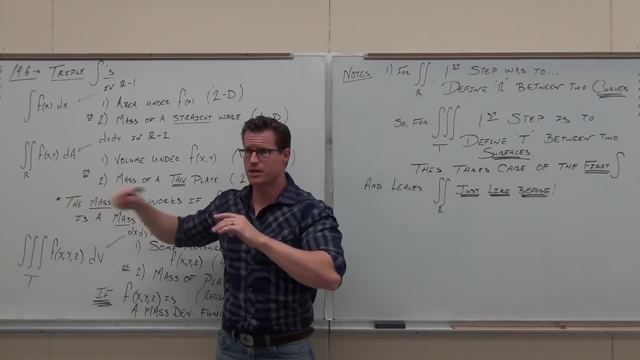 That happens. I need you to build this in your head: That in 2D you went between curves and in 3D you're first going to go between surfaces. You guys get those ideas. Well, I'm going to fill up those spaces in your mind. 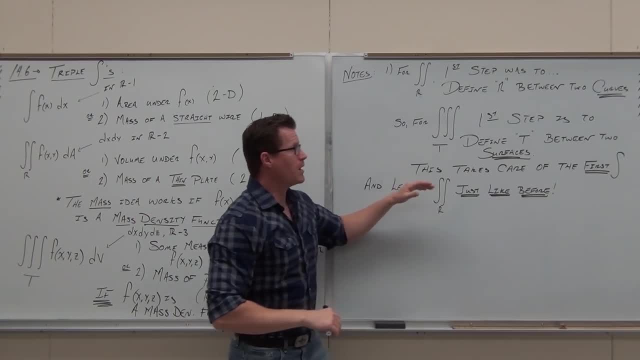 in just a little bit, Okay, So right now, I'm building you an advanced organizer. The main thing, though, is that, once I deal with the 3D concept, I'm left with a 2D concept, just like I had before. 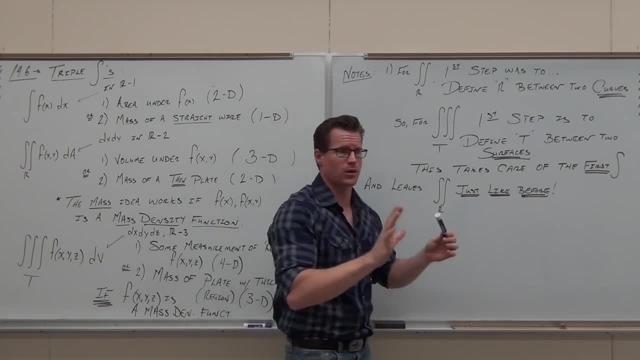 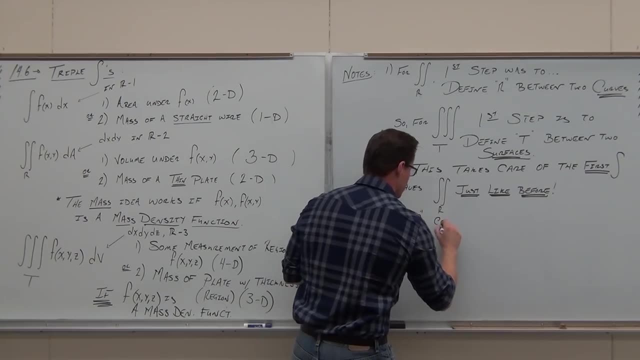 only the region could be in on any one of the three coordinate planes. So really just with a 3D model you can figure out how you want the alignment of those spaces units. So if that happens you could work it out. 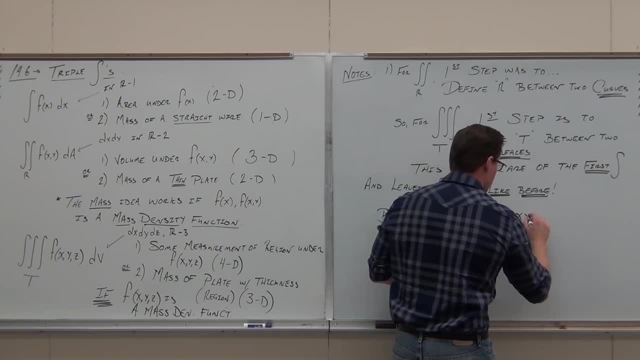 It's smart, That's cool. So this part ends here, but you think this is a nutshell? Slide it out. Alicia wanted me to stand up and tell you about this whole coworking thing you've been seeing so far. Can you imagine your whole life? 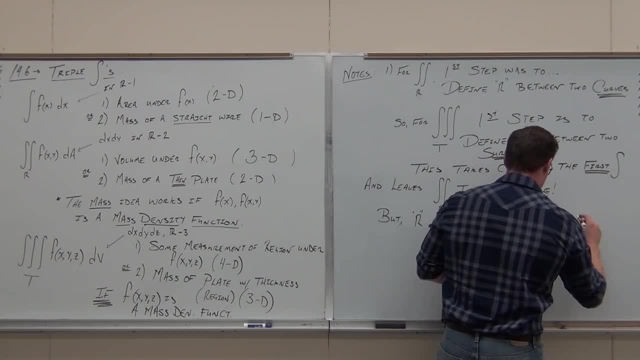 going into this book and what is that look like. So it's not easy to capture and it's daddy like me, We're always watching that. I know how that this software isn't. It's really limiting. It can be built in a way that will do better. 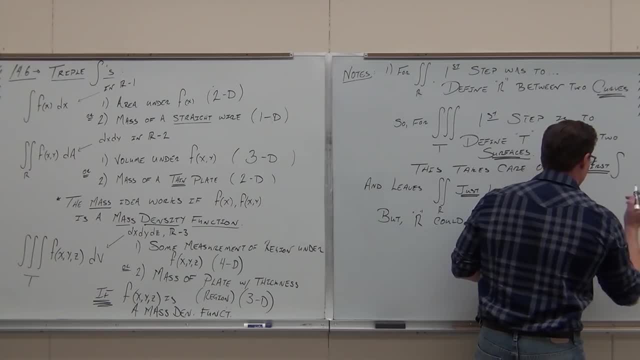 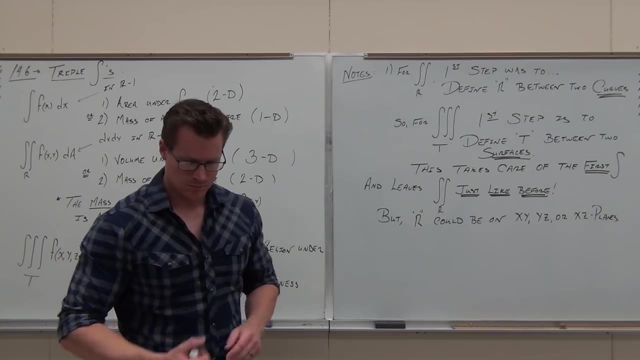 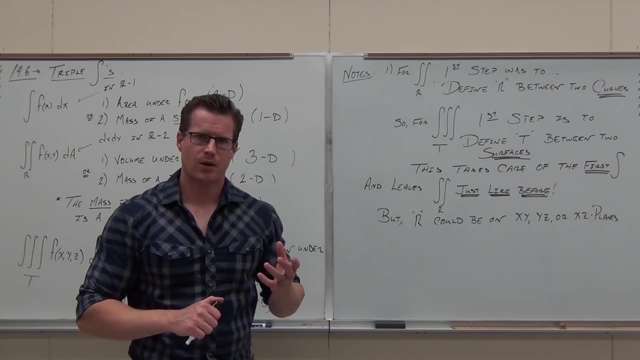 for your soon presenting experience. And these kids will never hear their kids talking down to that old teacher. So if you want it broken down into as simple as I can make it, we are left with two tasks: The task number one, two tasks and two regions. 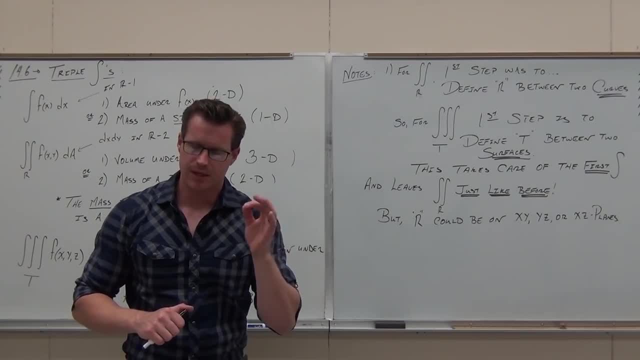 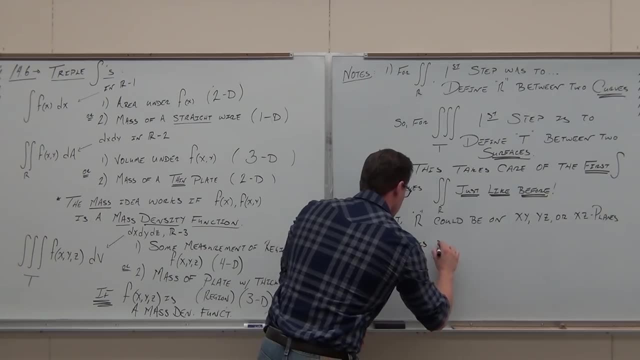 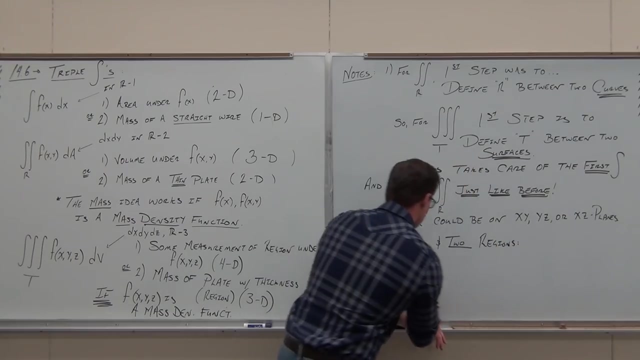 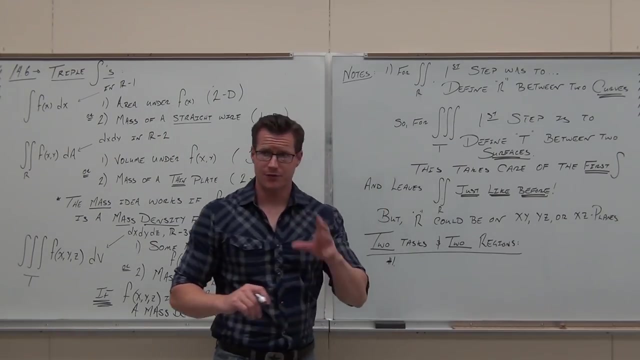 The number one task. we need to deal with a region in R3.. Okay, two tasks, two regions. Number one: you have to deal. trust me, you've got to listen to this. you've got to deal with the R3 region first. 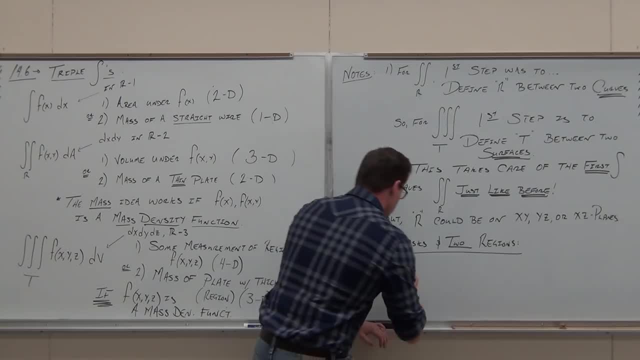 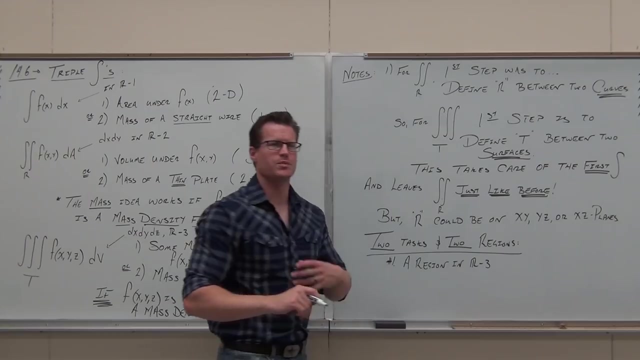 You have to go between surfaces first. So two tasks, two regions. One of them, you have to deal with the R3 region first. You've got to number one, deal with a region in R3.. That would be the one between surfaces. 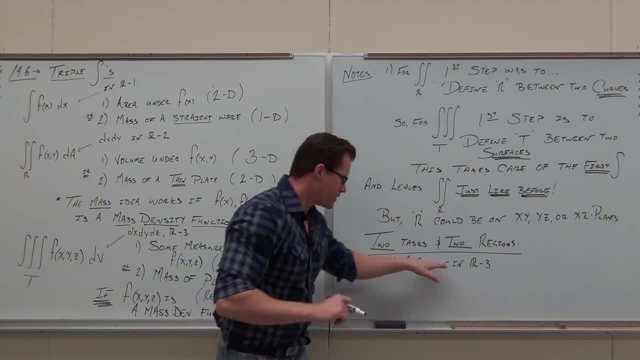 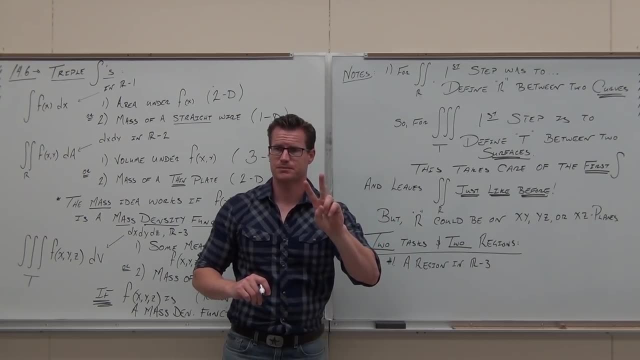 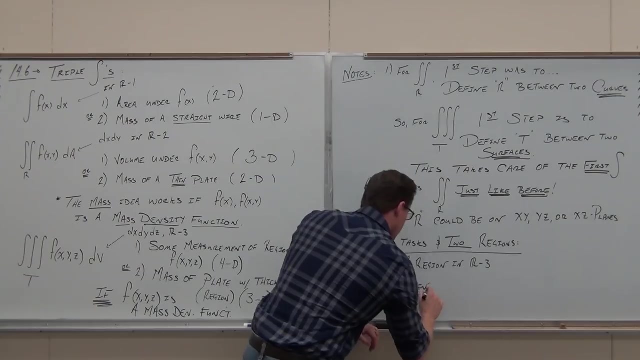 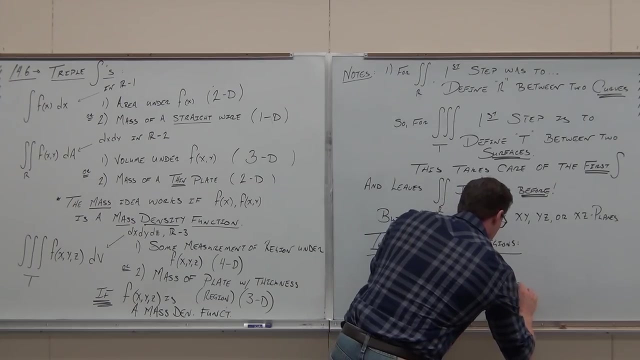 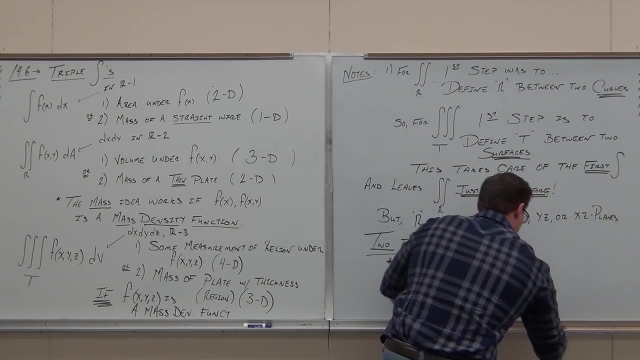 Number two. after that, after you deal with this region in R3, and I'm going to show you exactly how to do it- you'll deal with a very specific two-dimensional region on a coordinate plane. So there's- I'm going to show you the linear average solution. 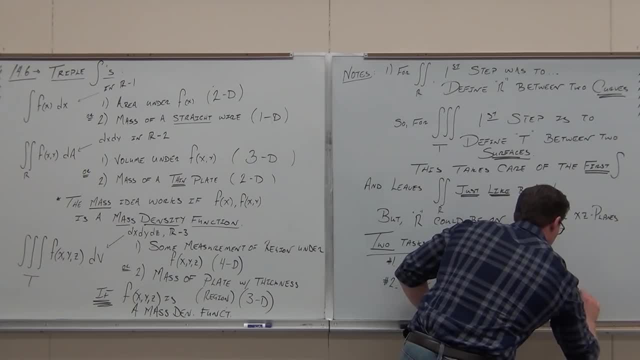 over the R3 region. You're going to have to deal with the two- two Cloud-like regions on ao and you're going to have to deal with the R3 region. All right And the less linear. that means we're dealing with a very specific line in R3,. 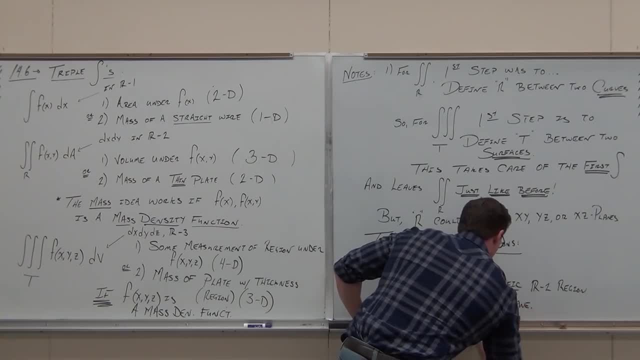 which should show you that. So the Northern 2021 distance view. Allright, you can submit in penguin. please, au, if you want. I won't leave you. I don't want to go any further. if you have any questions at all, 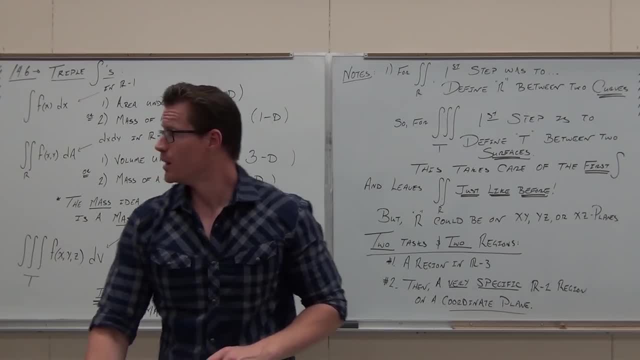 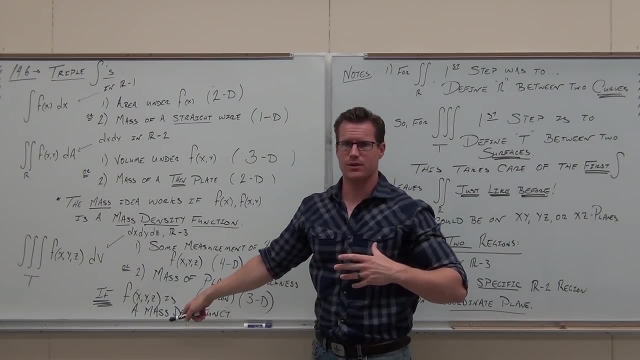 It's too important for you guys to understand this concept. So do you understand the idea of area versus mass, volume versus mass? weird 4D, volume versus mass. I don't know if you're okay with that. Do you understand? the mass idea only works. 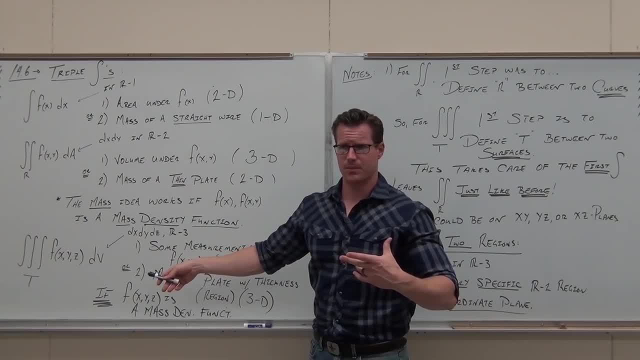 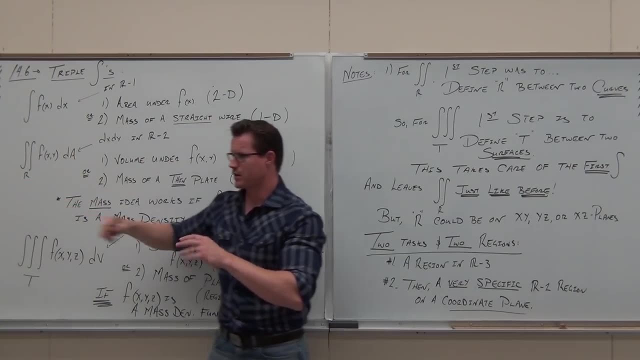 if the function is the mass density function, Hello, yes, no, Yes. And then it gives you the mass of whatever region we're integrating over It. gives you the mass of the- this is from A to B- gives you the mass of the thin plate. 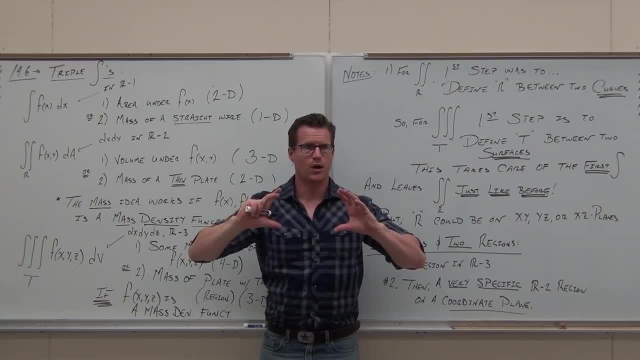 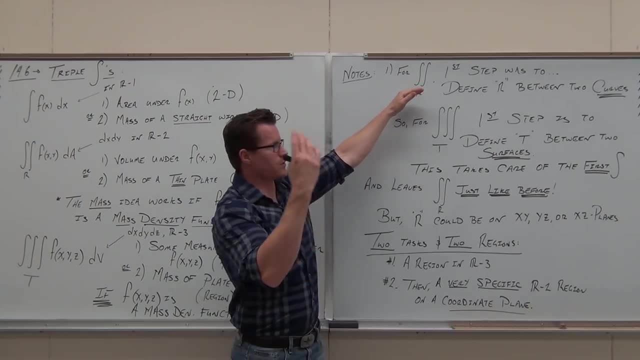 over a 2D region gives you the mass of a 3D thick plate Over a 3D region. I don't know if you're okay with that one. Main goals here deal between curves for two, for double integrals- cool. 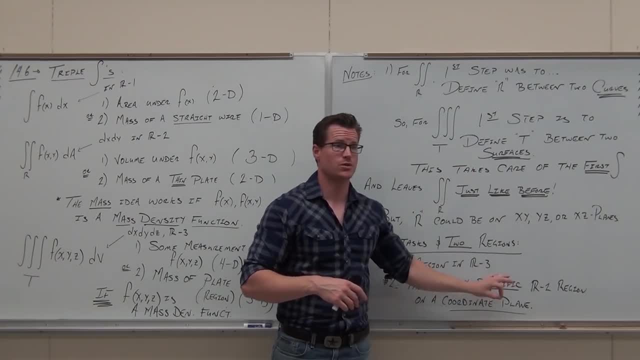 Deal between surfaces for triple integrals and then we have a region in 2D. that's the main goal. it's the main goal in life right now. right, Your goal in life. you want to write your five-year plan. 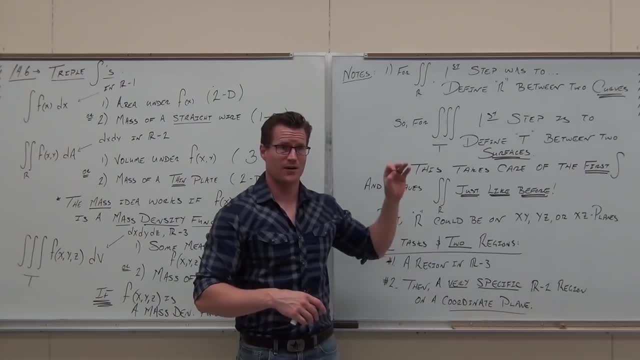 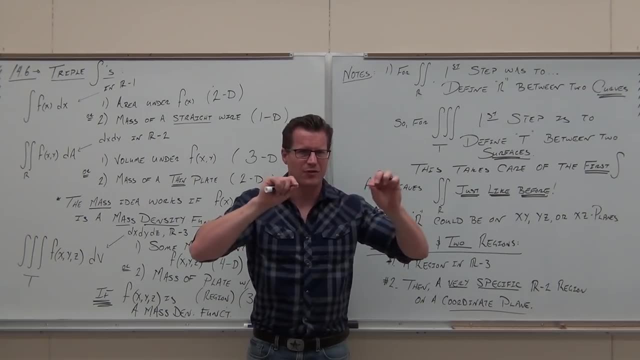 Well, this is like a five-day plan. Your five-day plan right now is figure out how to make your first distance, your first travel your first along, whatever you're going, between two surfaces Three. that's our main goal. 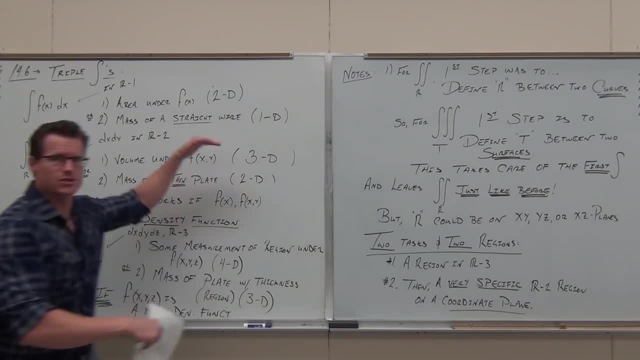 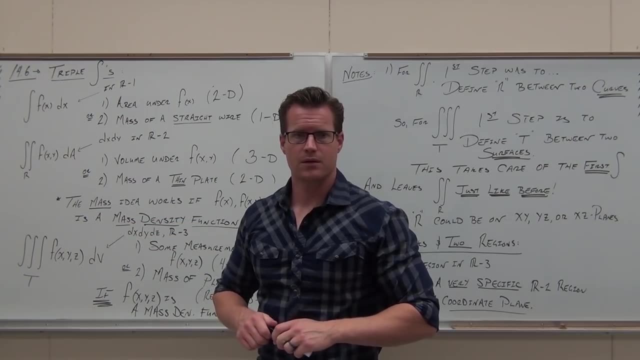 After that, a couple other notes here. Are there any questions on this one before we continue? I really want you to have it down. Are we okay with it? Yeah, Will we use. will we be using convergence of spherical, just like we were using convergence of polar for the double integrals? 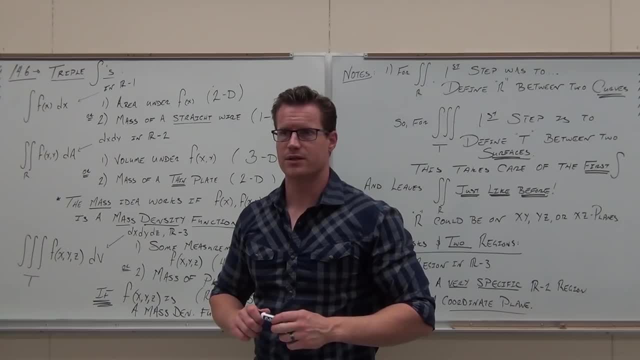 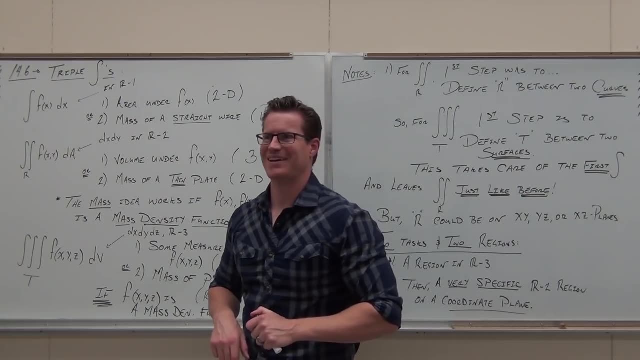 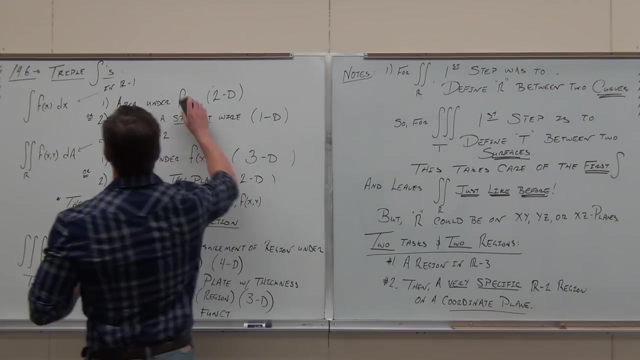 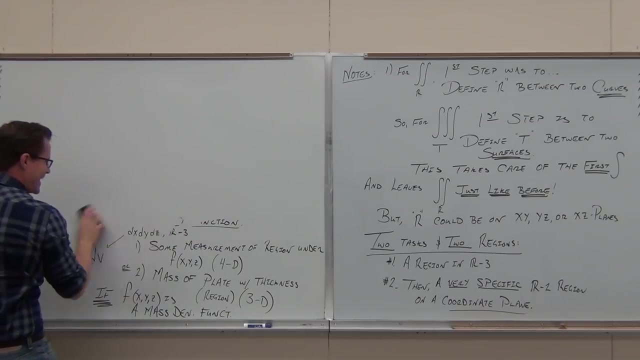 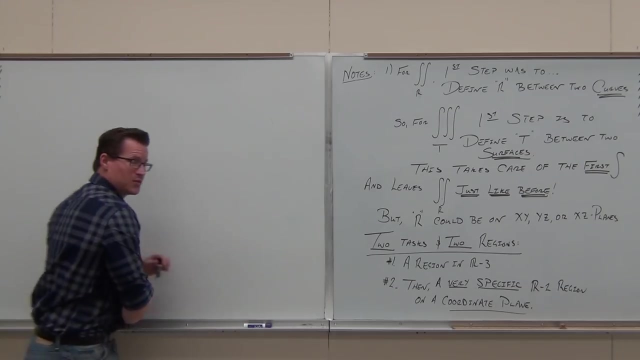 Will we be using spherical coordinates and cylindrical coordinates? Maybe, But not now. All right, Eventually- I don't want to ruin the suspense- Yeah, Yay, Then we get something called the Jacobian. You're like what? Yeah, I'll prove to you. I'll prove to you how spherical coordinates and 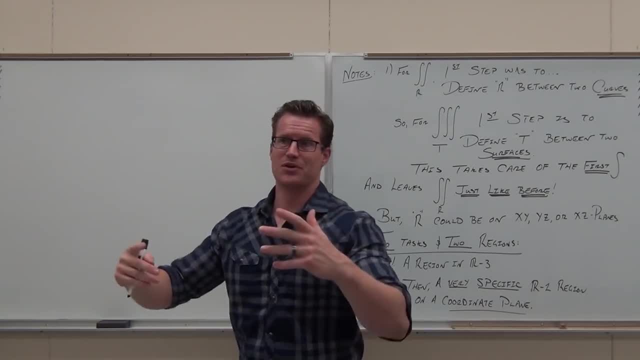 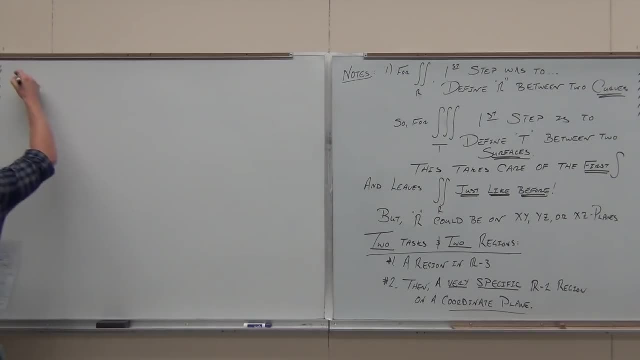 you remember the RDRD data and I kind of gave you a sort of quasi-proof. I can prove that with, like the well, we'll talk about it. So cool. The second note. so that's note number one. Note number two. 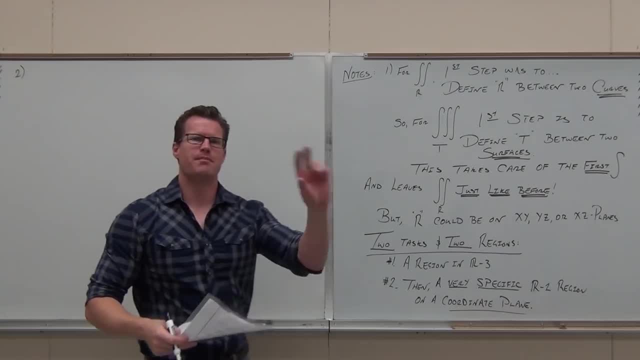 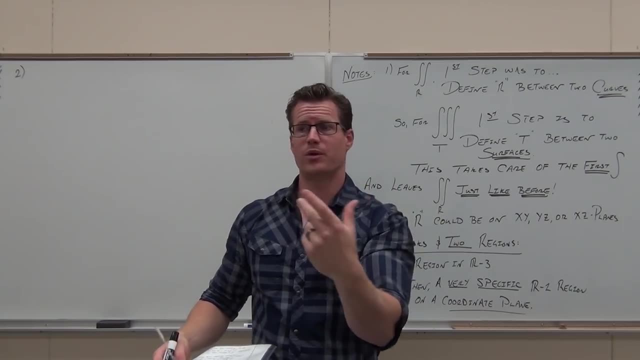 What's the second note? Just like double integrals, did it matter the order in which you integrated Dx, dy, dy, dx. did it matter? It mattered as far as the integrals hardness is concerned, but would you get the same answer? 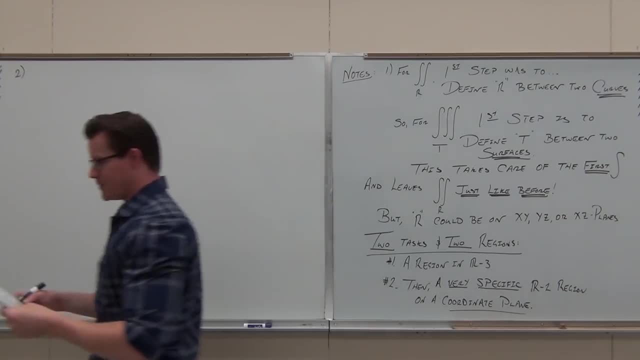 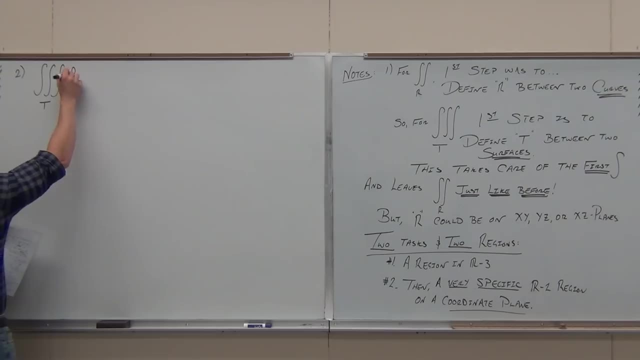 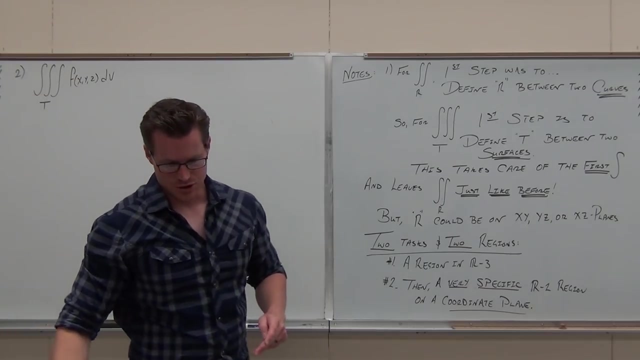 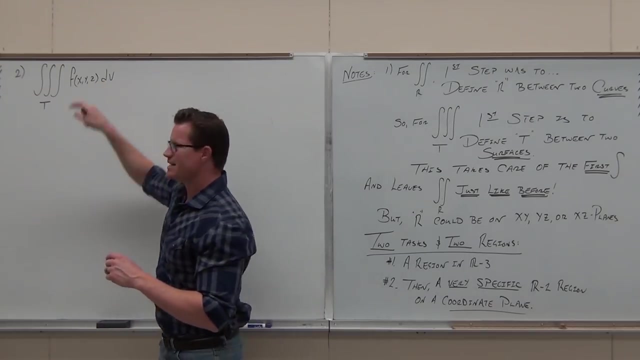 Yes, Yes, Rubini's theorem says you can switch them. Here same thing happens. Triple integrals, By the way. I do want to want you to know this Dv, just like da gave us an area, can you see that the dv is a volume concept in 3D? 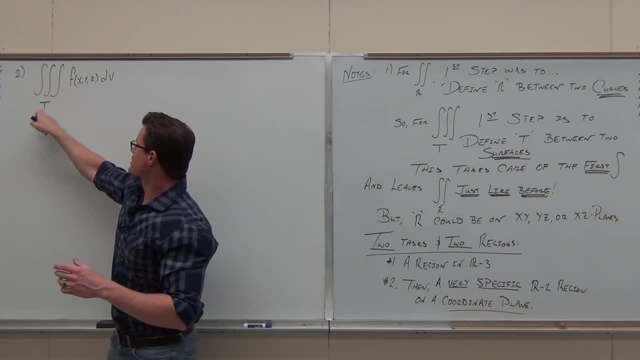 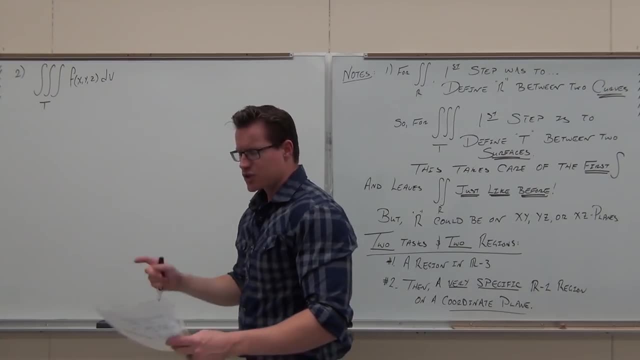 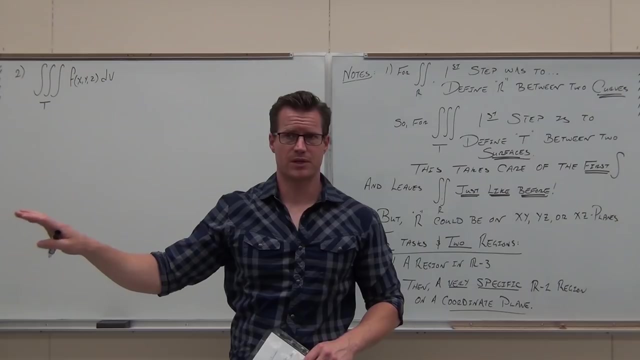 That's why we're getting the mass of the volume of that region. That's what we're getting there. if x, y, z is a mass density function, Just like double integrals, these things can be evaluated in any order. Only there are three factorial permutations. 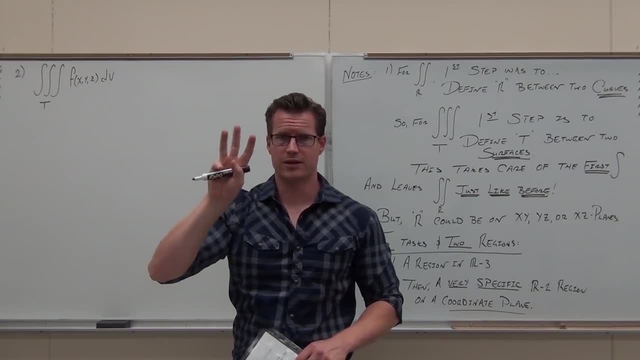 There are six ways you can do it. Because there are six ways you can do it, There are six ways to order that triple integral. You could have x y- z or x z- y, and six different ways to do that. 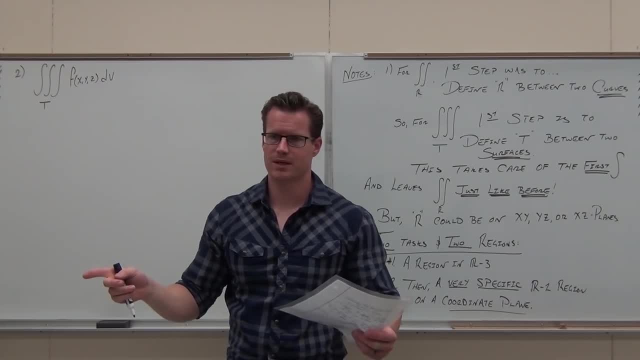 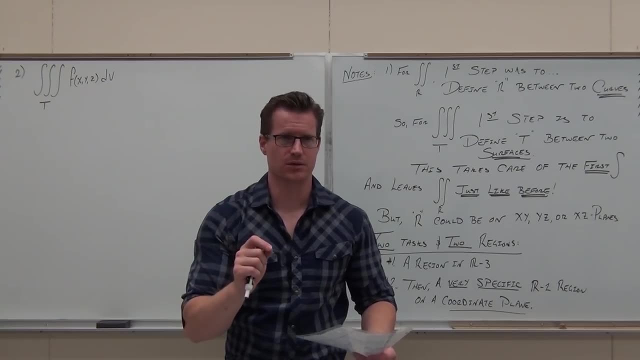 Does it matter? Well, ultimately no, Ultimately no. But I will tell you, just like double integrals, certain ways, certain orderings are way easier. Does that make sense to you? Remember that with double integrals, Sometimes dx was impossible, dy was way easier, sometimes vice versa. 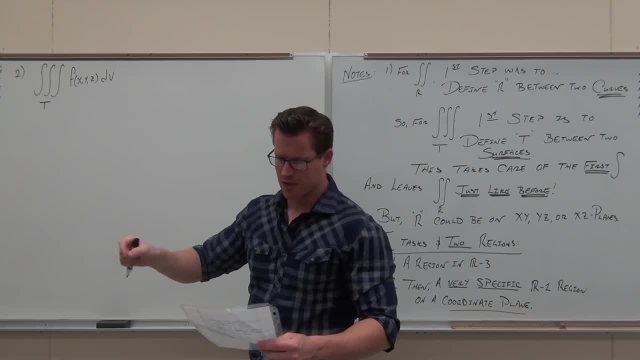 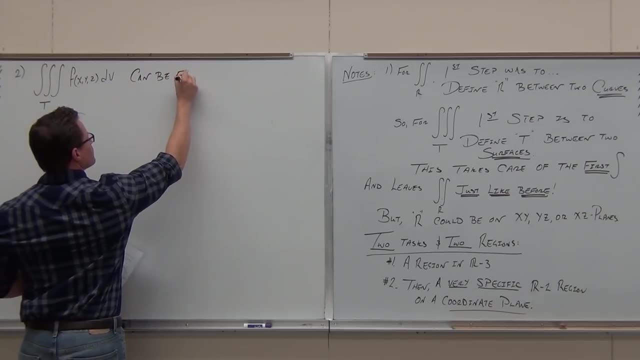 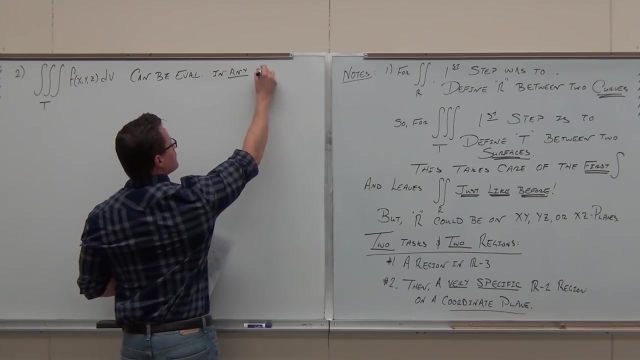 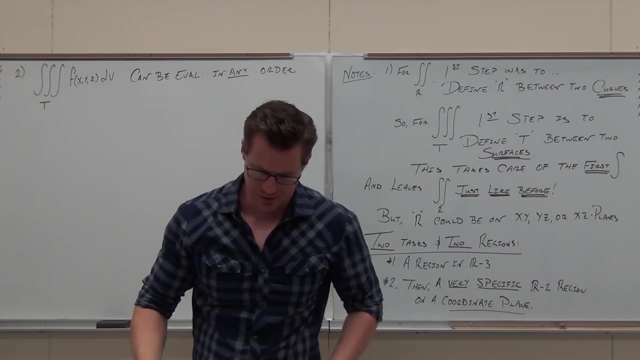 So these can be ordered, evaluated in any order, just like doubles, but there's six permutations. It can be evaluated in any order. I'll leave it like that. It's just that some are going to be much easier than others. Now let's talk about the most important thing I need to understand. 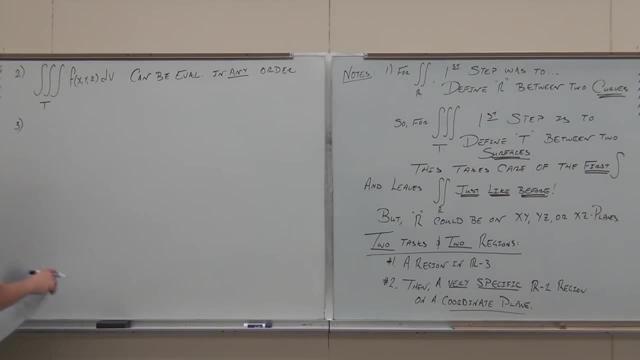 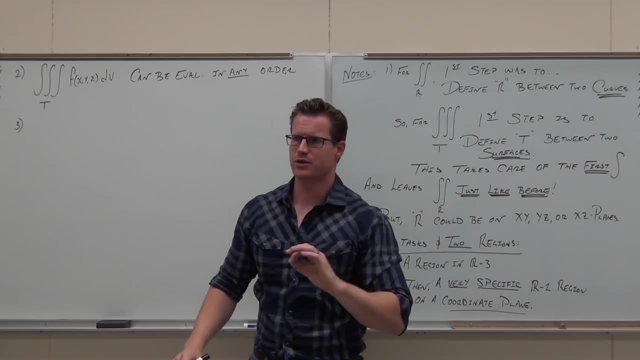 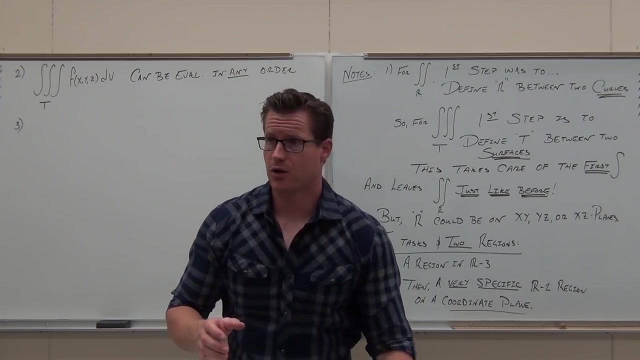 This step, How to define your triple integral between surfaces. first, If we are doing a triple integral, then we have to integrate across. well, let's see: single integrals was one axis. double integrals was x and y, that's two axes. 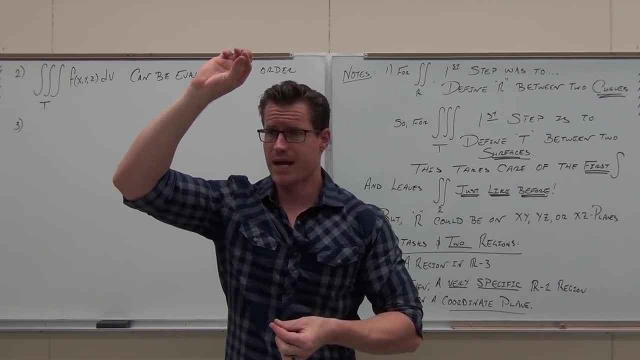 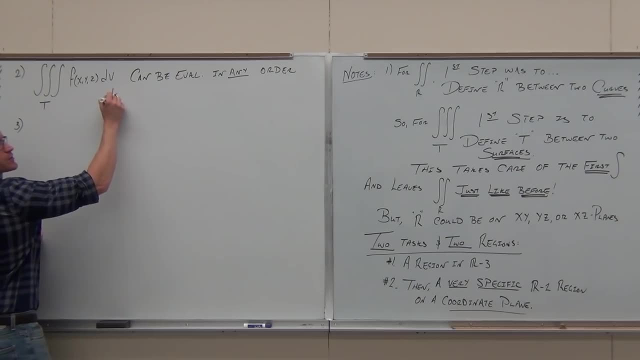 Triple integrals are going to be x and y and z. That's three axes. We have choices that we can make. We can go along x first, then y, then z Or anywhere. So you have to pick one of six permutations to do that. 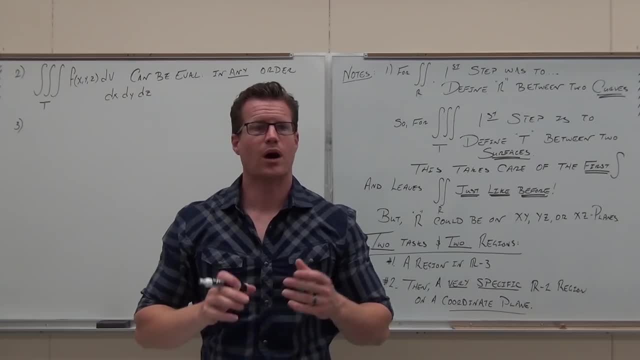 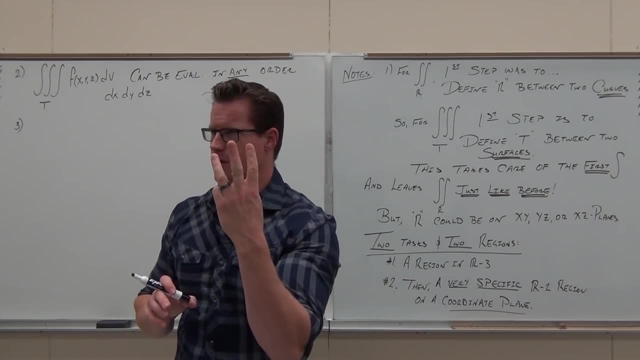 Does that make sense? You have to pick one. So I'm going to show you in our examples how to pick the appropriate choice. but we're going to have three choices here. You can only pick one thing to go first. You can pick to travel along the x. well, that's a good one. sorry, 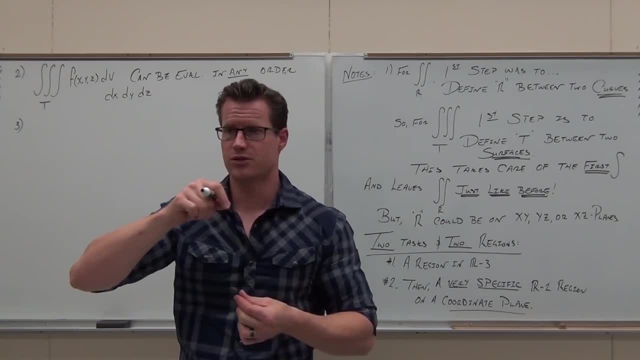 You can pick to travel along the y or you can pick to travel along the z, now that you understand that. and it's going to always go between two surfaces, So along the x between two surfaces, y between two surfaces or z between two surfaces. 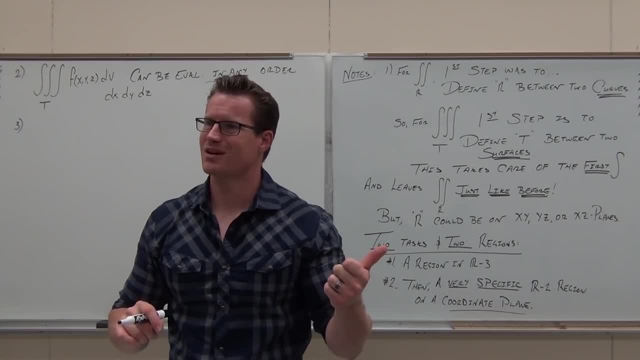 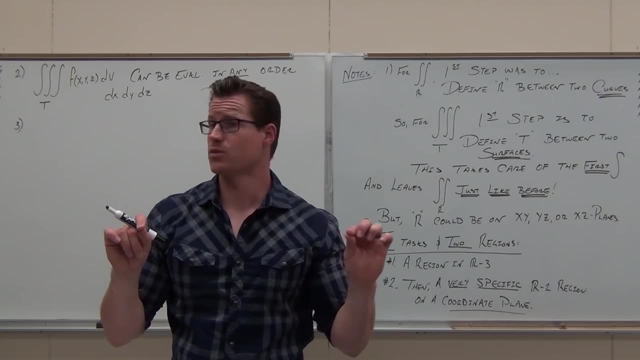 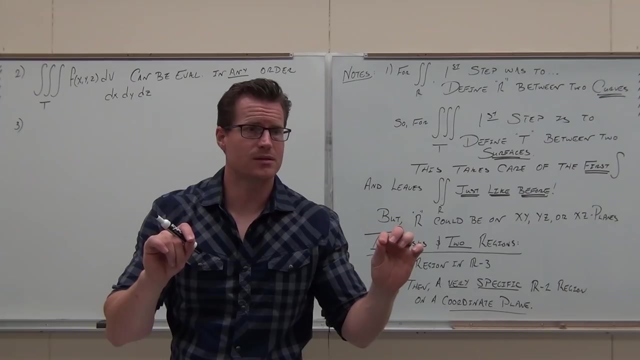 Those are called x simple. Remember the simples that we talked about. X simple would be between two functions, surfaces defined in terms of x equals, x equals y's and z's. Y simple would be between two functions: y equals x's and z's. 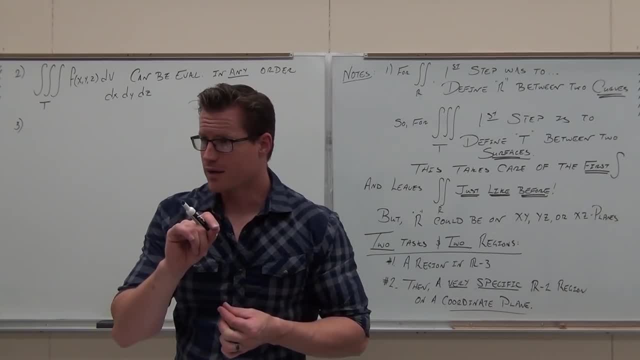 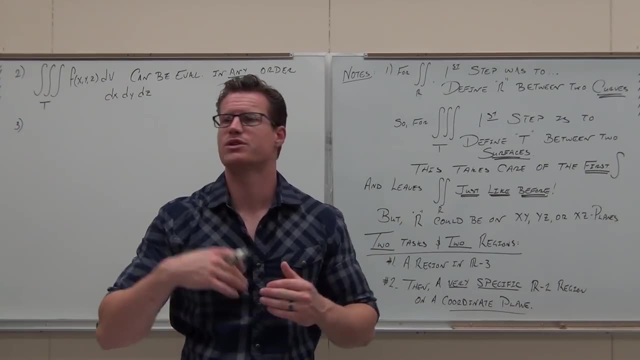 Z simple would be between two functions, x's and y's. Does that make sense? So you have a choice to make whether you want to travel along the x axis- x simple. y axis- y simple- or z axis- z- simple. first, 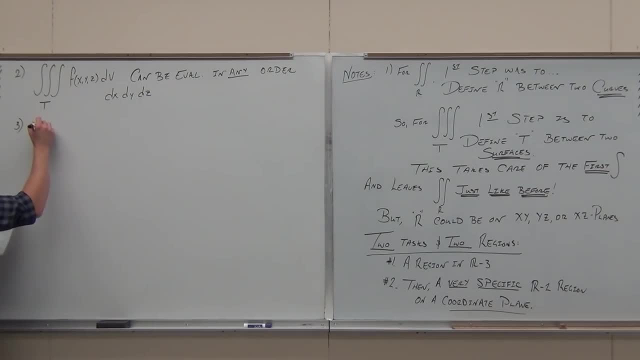 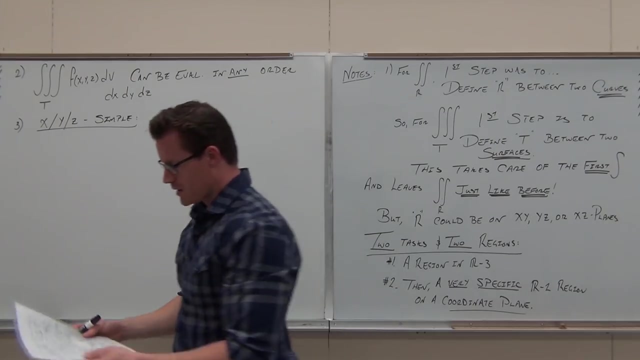 We'll talk about each one of those. Let's make it x, y, z simple. Is it simple to do Generally? yeah, it's not too bad. I'm going to show you how to make some good choices here. Let's talk about what z simple is. first, get an idea. 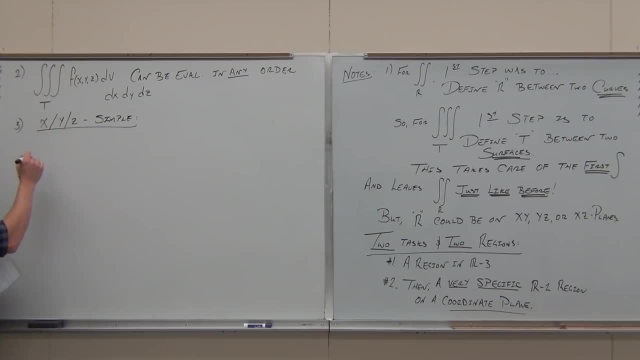 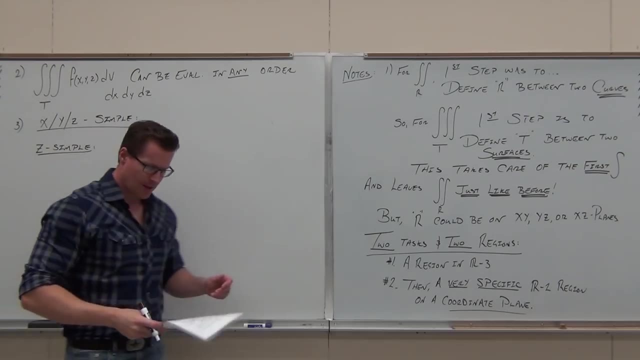 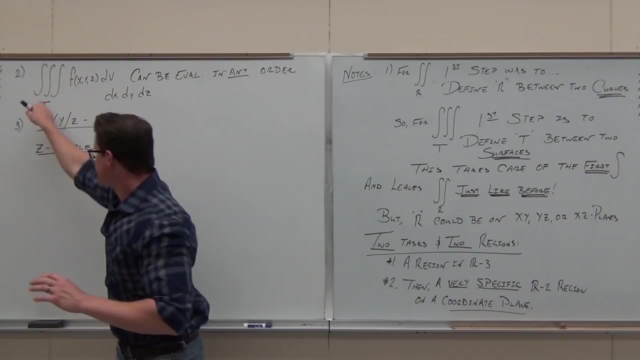 This is going to be the most common one for us. We want- we really do want- z simple. I'll start with z simple. I'll show you why. Here's what z simple means. What this means is that we're going to define our R3 region, our 3D region, RT. 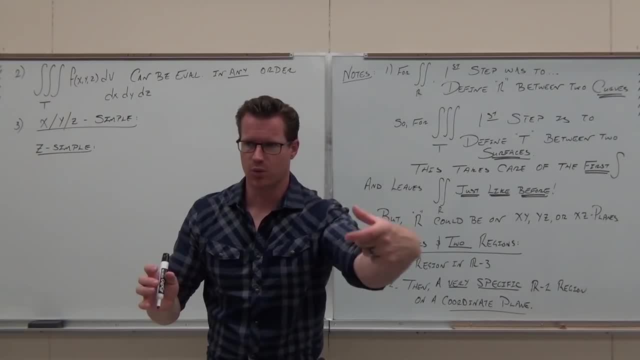 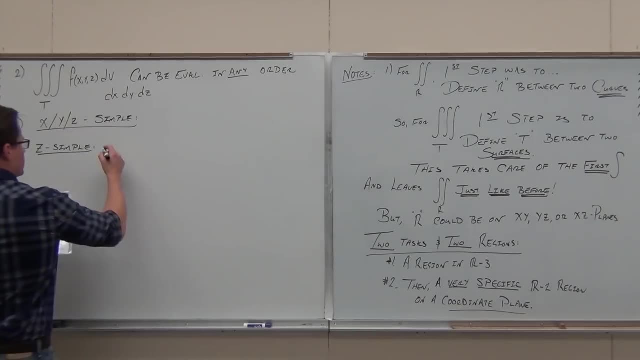 We're going to define our R3 region in terms of z equals some function that has just one of the two variables. Come on, One of the two variables, That's right. That's right. So this means that we're going to define our R3. 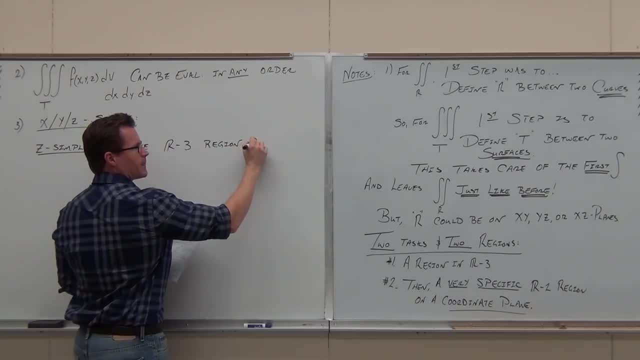 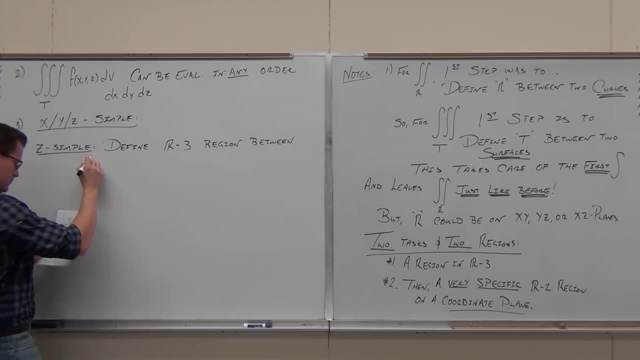 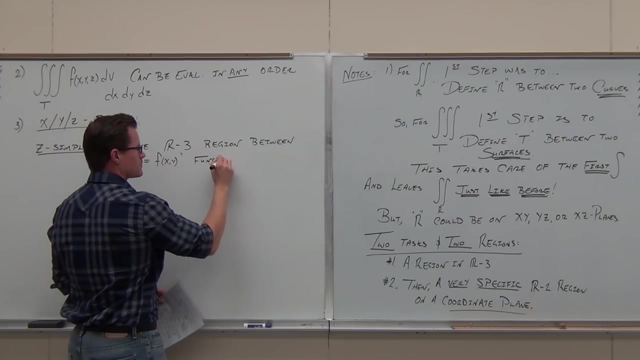 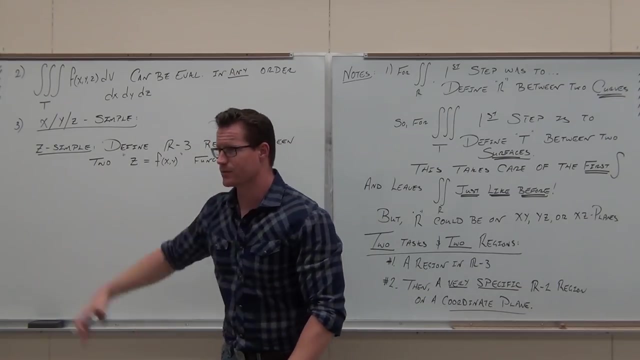 So we're going to define our R3 region between two z equals functions. I hope you're taking good notes right now, because this is going to be like an outline of how you do stuff All right from right here. this is where we start. 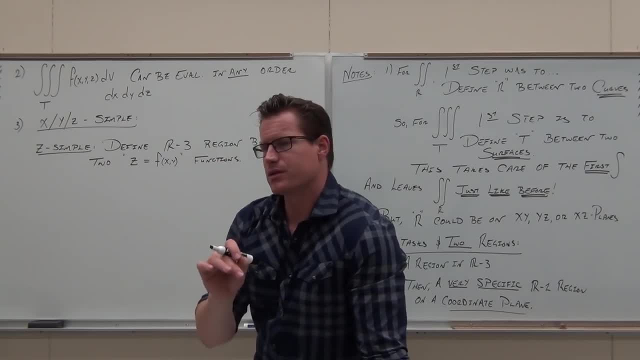 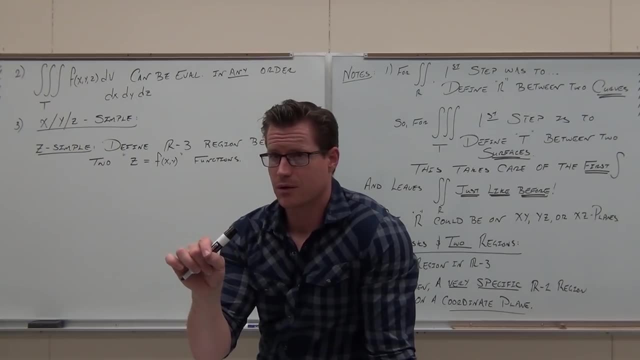 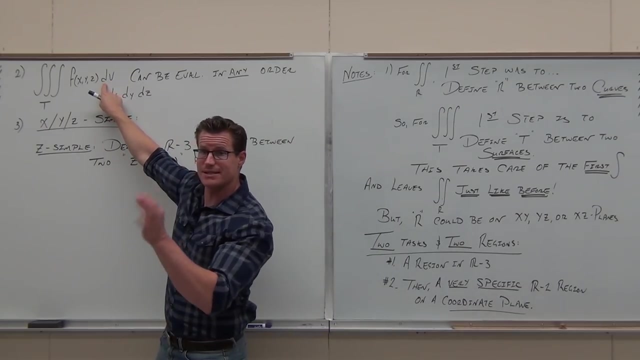 Here's the point, though This is a cool point If you make z simple. if you do z first, look at the board. Stop what you're doing. Look at the board. If you do z first, this has to be z dz first. 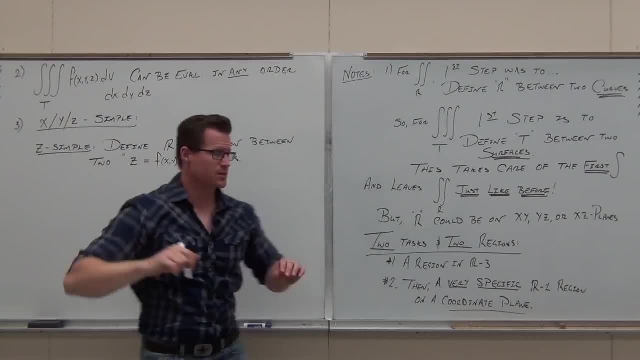 You guys get that. Are you sure you get that? If you did this, don't? you don't need to write it down. We'll do some examples to illustrate it. but if you did this, you'd have a triple integral. 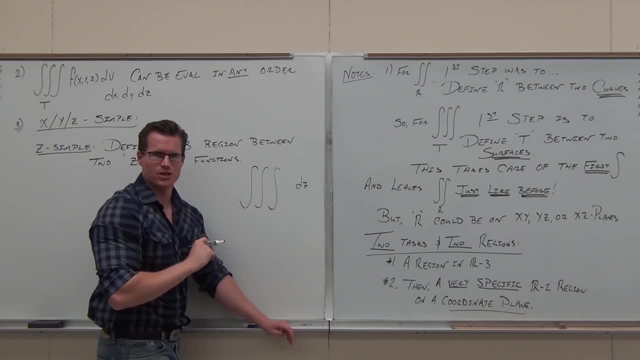 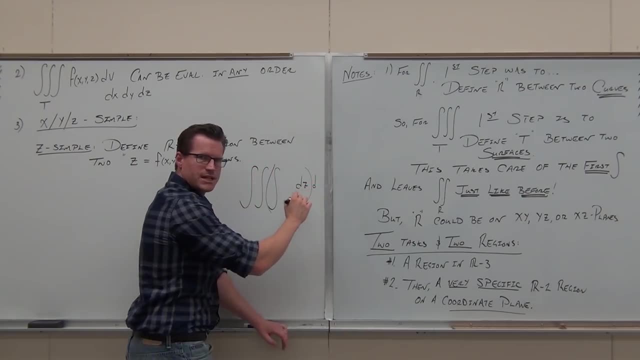 and your dz would come first. Does that make sense? Yeah Well, check this out. If you do that integral, you're going to be left with a choice of dxdy. That's da. That's a double integral over a region on the xy plane. 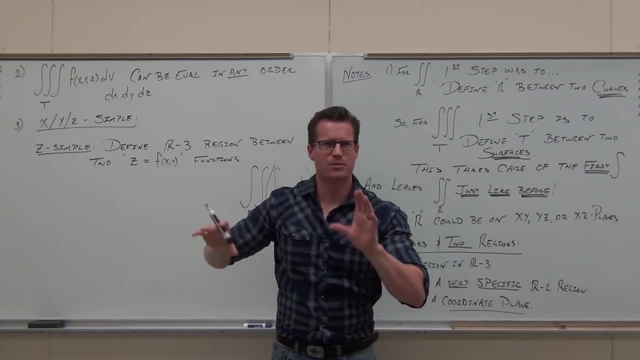 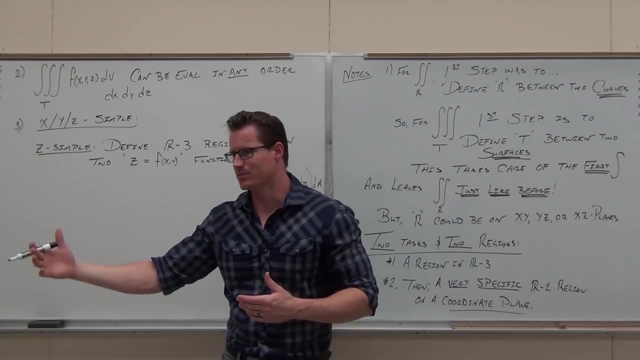 So if you choose z simple, your region will be on the xy plane. Does that make sense? The region for the double integral we're going to create is going to be on xy. That's why we like z simple, Because if you pick z simple, you're used to regions on the xy plane. 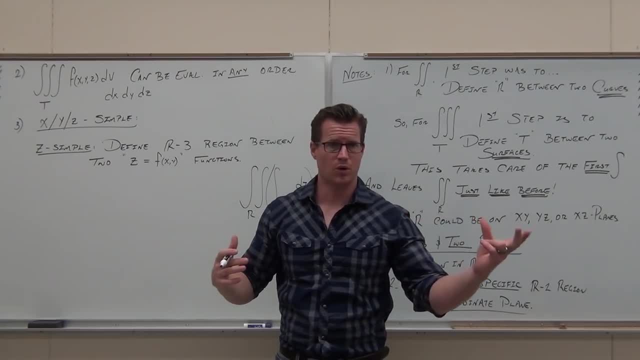 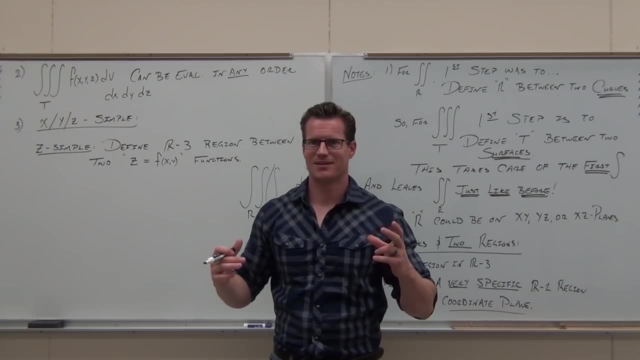 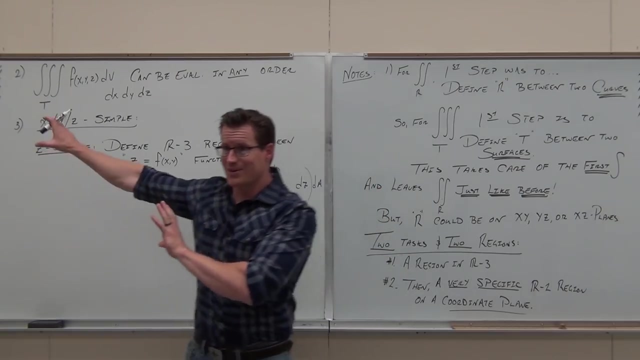 You already know how to define them. You already know how to switch them into polar. Did I just say something, Anyway, going back. so if you can do z simple, your region r the r, not the t. okay, 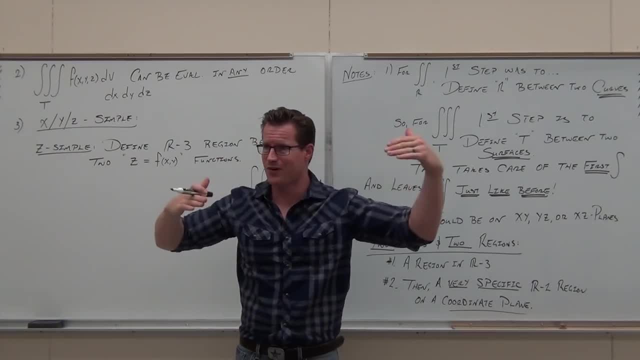 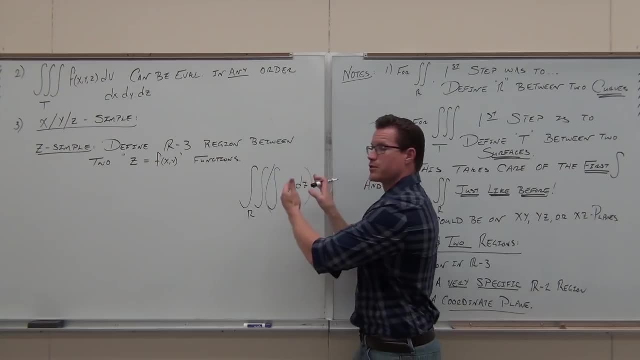 the t's in 3D. you deal with the r3 concept first between two functions, hopefully z, If it's between, z equals some crap here and z equals some other crap here some other crap, and you go between them. you've just dealt with your first integral. 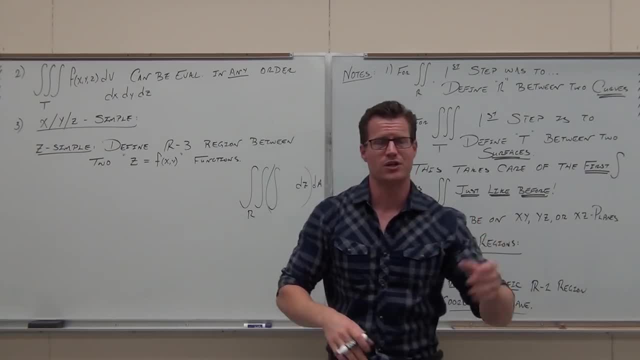 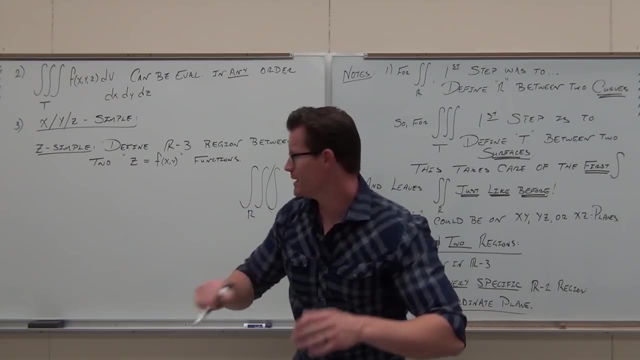 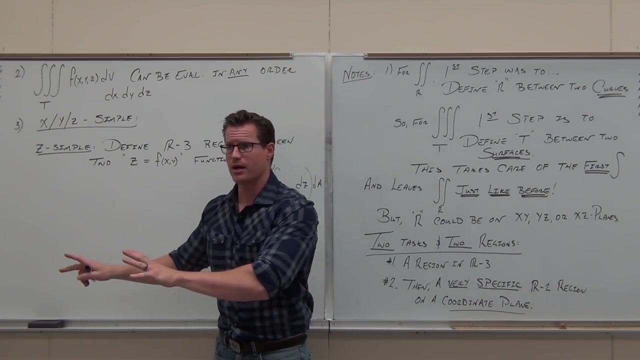 That's fantastic. You're left with a double integral over another region. What plane is that region going to be on? Whatever plane doesn't have that variable symbol. So if you go along z simple, your region is on xy. Does that make sense? 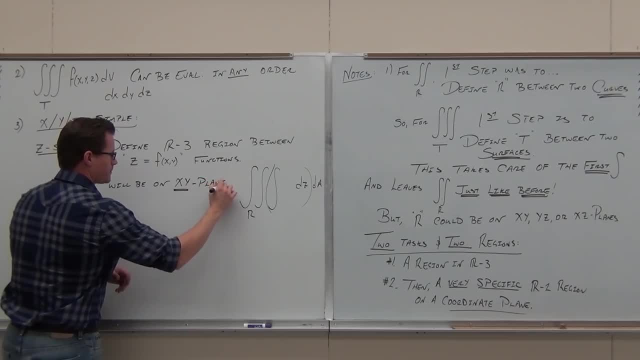 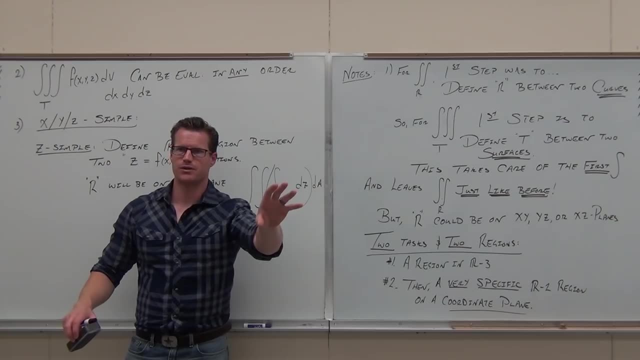 Now that's a wonderful thing because you know all about. we spent six hours. I looked at the videos. I added up the time. it's like six and a half hours, seven hours doing double integrals. Do you know that? 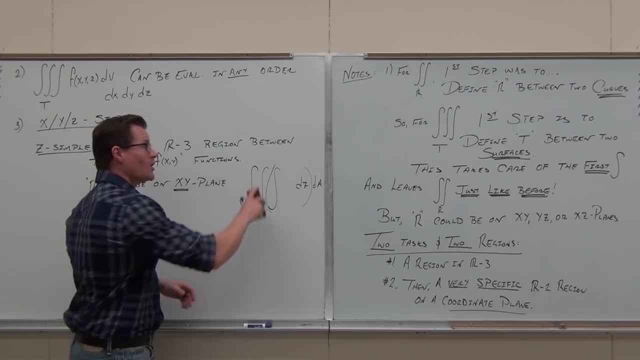 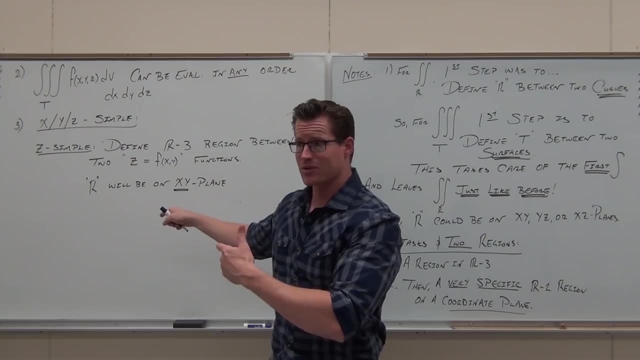 It's a freaking long time. all right, So you hopefully know all about freaking double integrals. Why do you think we spent so much time doing double integrals? Because when you get triple integrals, you automatically get double integrals. You automatically get a region. 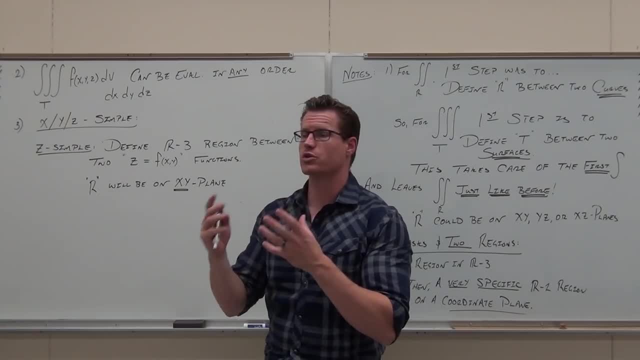 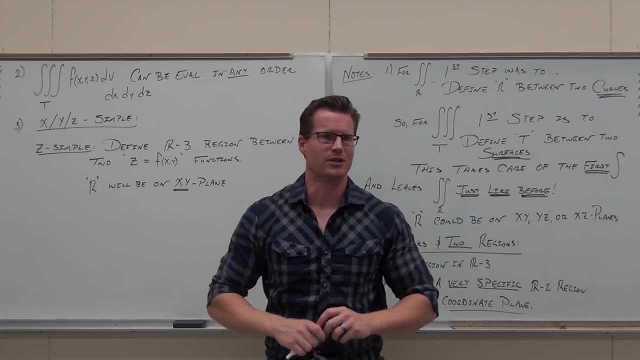 You automatically get the same exact stuff. That's why I had to have you know it so incredibly well. I couldn't just skip over double integrals to get to triple, because every triple integral automatically has a double integral in it. Did you guys get it? 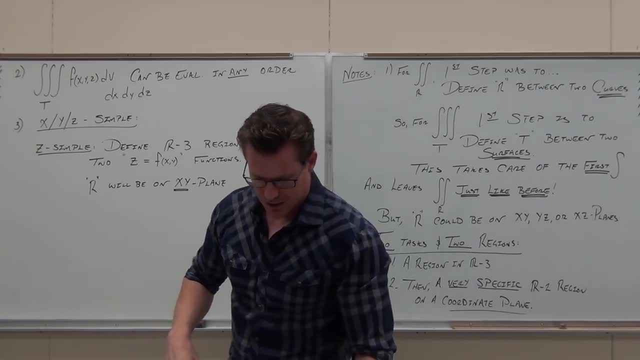 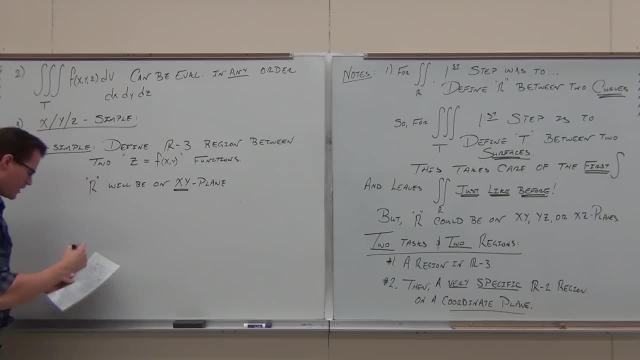 You had to know it. That's why we spent eight hours- seven to eight hours- doing it. So that's number one. Try to pick z simple. It's not always going to work out, but it's the easiest and it's the most common for us. 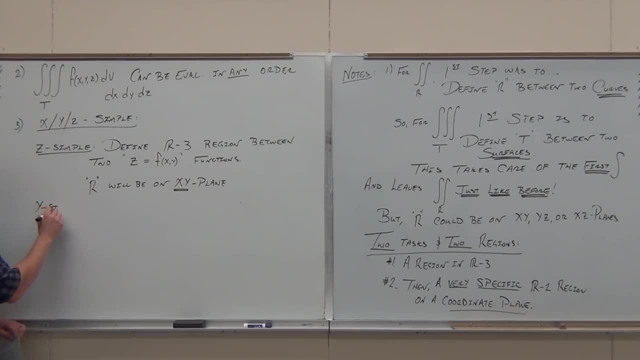 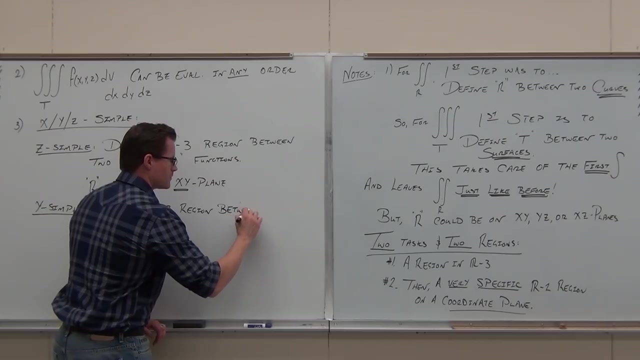 What's the? let's do y simple, You know. I'm sure you can draw some comparisons here. I'm sure you can. If this z simple defines the R3 region between two z equals functions, this is going to define the R3 region between two. what? 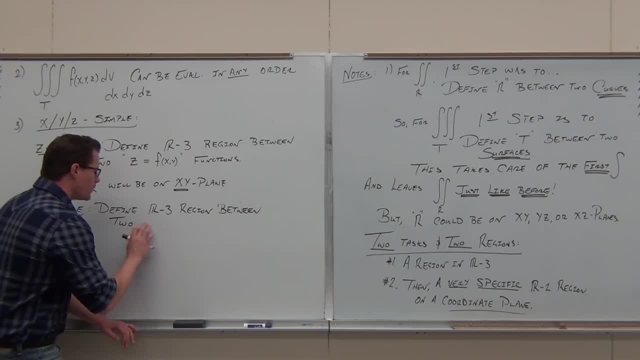 Y. Y equals a function of what. Now, wait a minute. If it's y equals, what other variables are going to be over here? Z. Now, if I had to put this after I deal with the R3 concept. 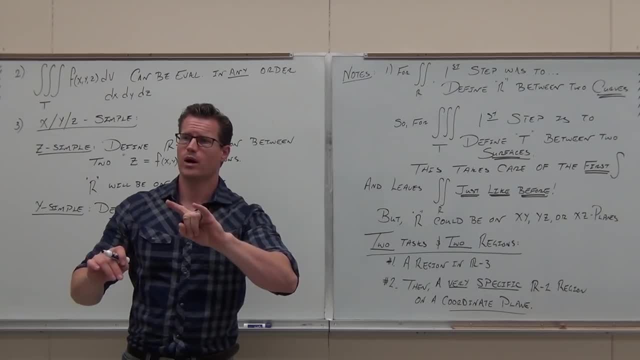 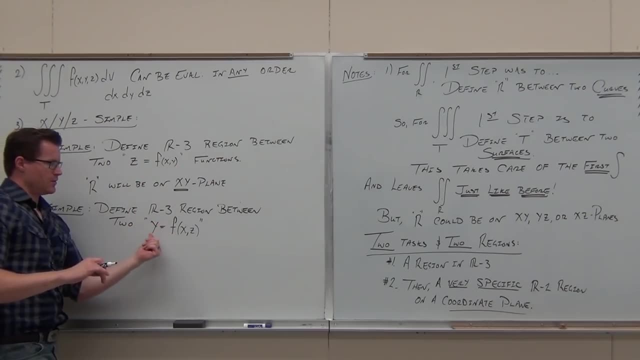 I'm going to deal with a 2D region. What plane is that 2D region going to be on? This was on the xy for our region. This is going to be on the xz for our region. Whatever variable, you do simple, you limit the variable. 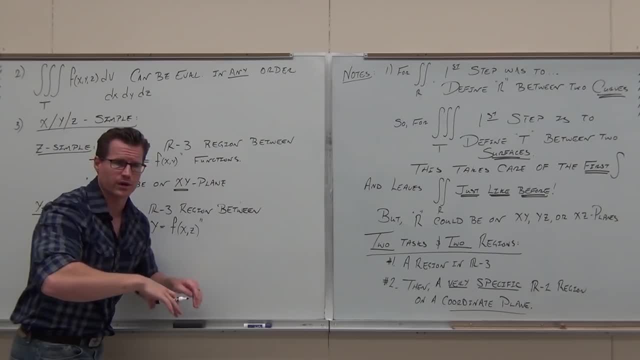 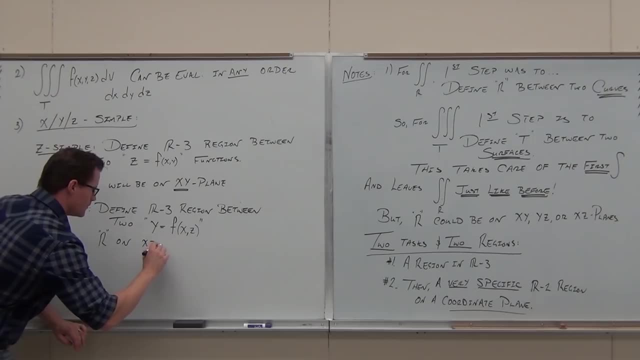 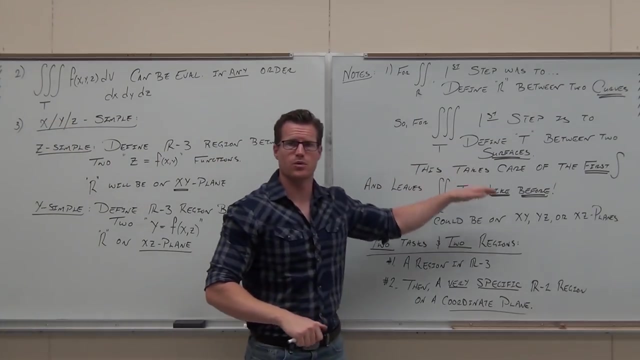 That's the whole point. Then we deal with a region on another coordinate plane there. Why don't you write out your own notes while I erase this side? Are there any questions on this side of the board? Can you write out your own notes? 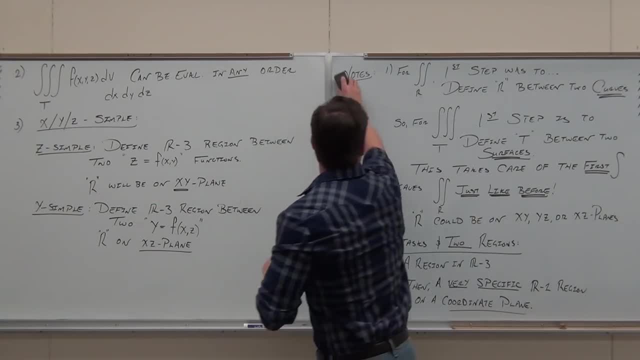 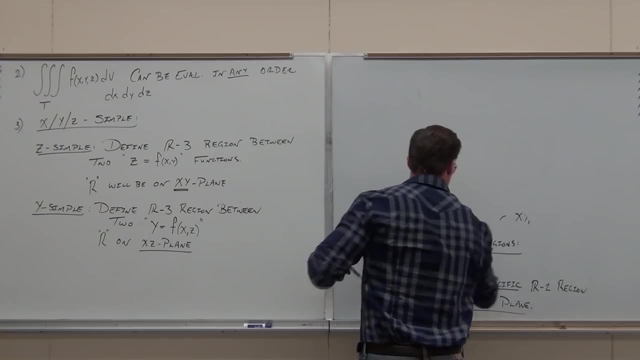 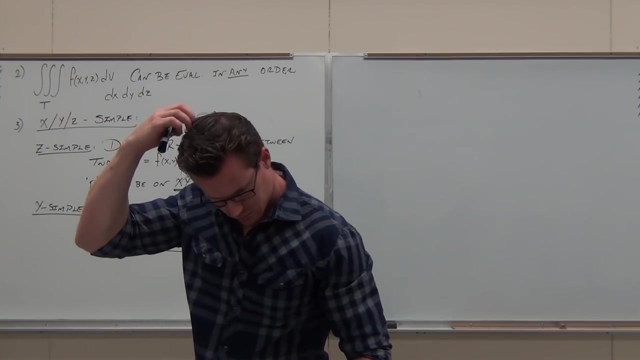 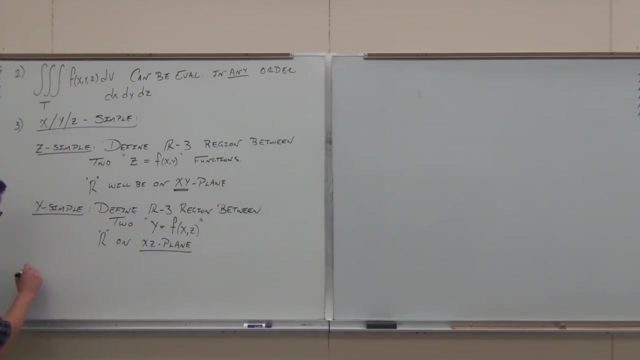 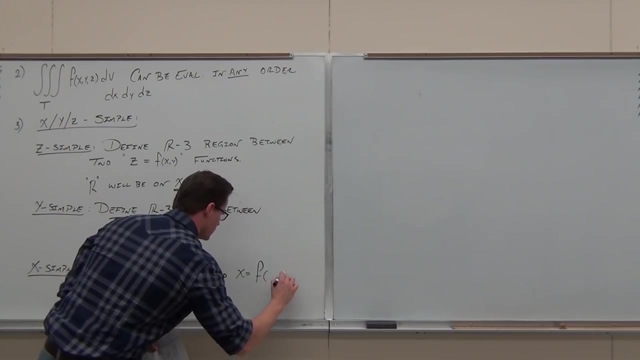 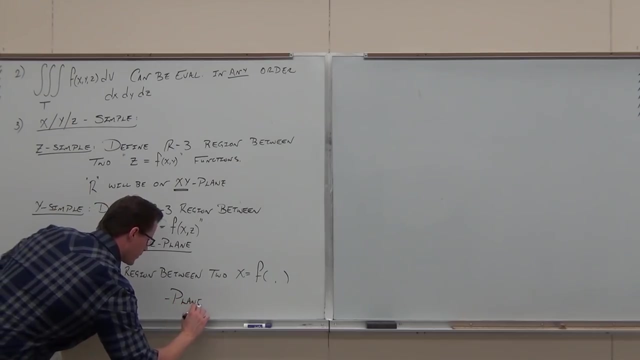 See what x simple would do. Thank you, If we want to do X simple, we would have X equals. what two variables would it be over here, please? Y, Perfect, And so the region. once we dealt with the 3D concept, we have a 2D concept to deal with. 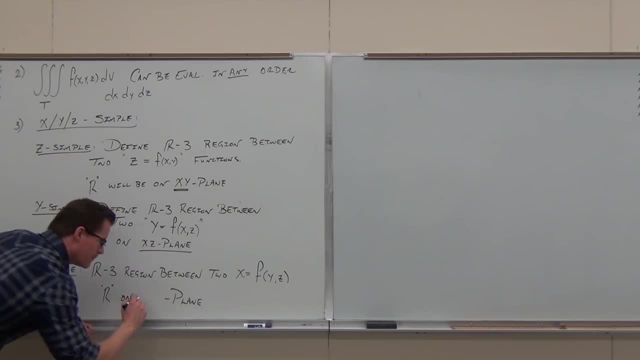 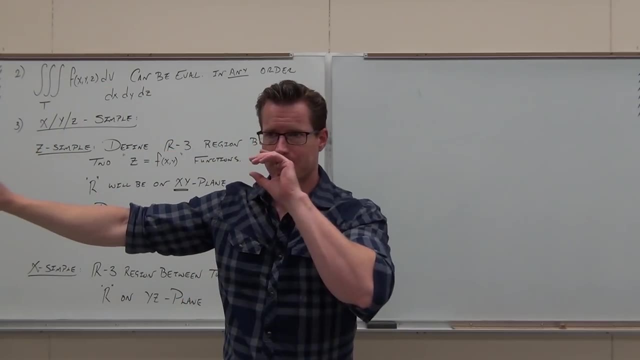 That's why we get a double integral Out of every single one of these triple integrals. what would it be on Y Beautiful? So if fans feel okay with the concept, Am I starting to flesh out the idea? You're starting to see double integrals at work and triple integrals. 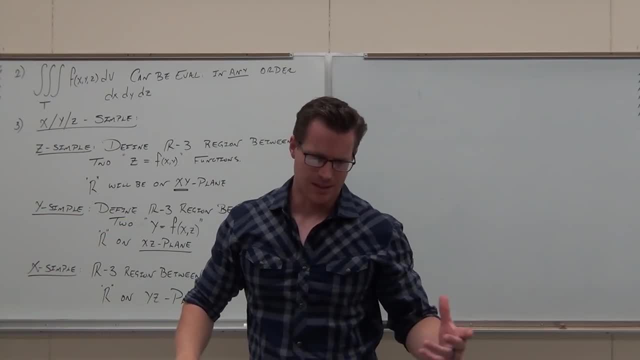 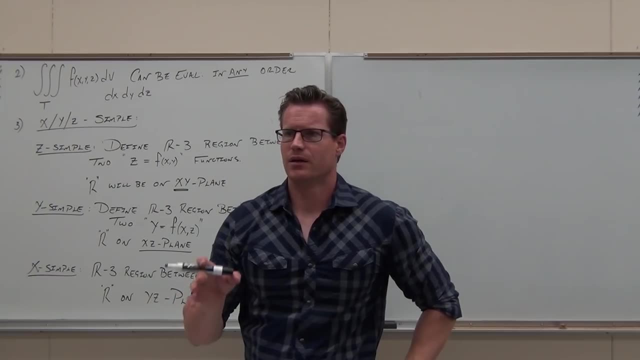 Okay, The fourth note. I'm not going to write it down, but it doesn't go without saying, because I'm saying it But it's redundant. Defining the region is the hardest part of any double or triple integral: Defining the region. 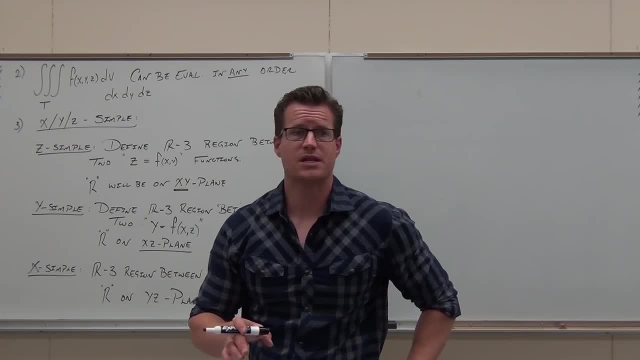 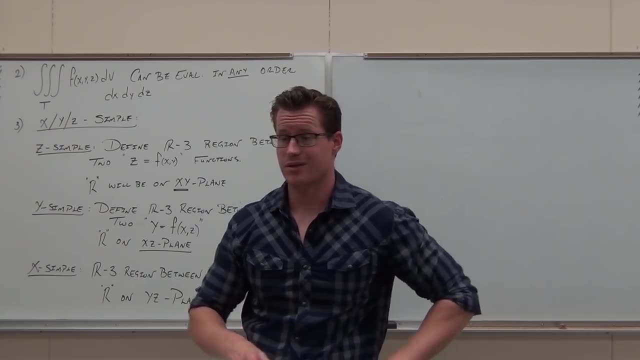 You guys knew that from double integrals- right, They can get very difficult. Same thing here. They're not super difficult, but you have to know what you're doing, especially with the double integrals. So I'm going to show you how to do it. 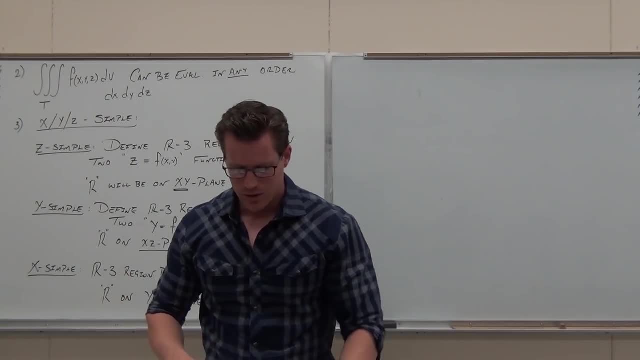 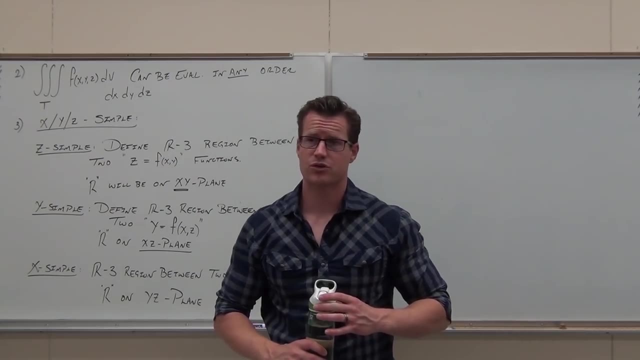 There's another variable floating around. We've got to deal with that thing Right now. what's going to happen is we're going to do two very, very quick examples where the triple integrals are already set up for you. I just want to get you used to seeing them for right now. 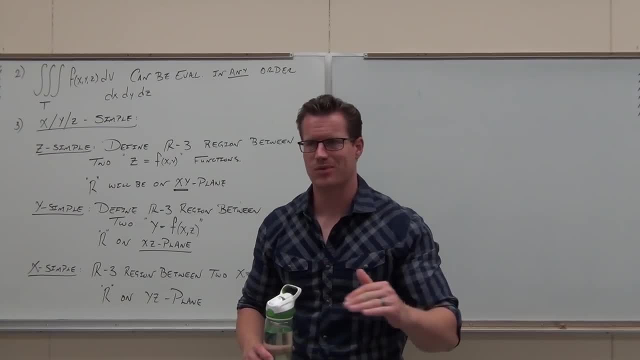 Does that make sense? So, really quick, I'll show you how they work- There's not going to be any surprises at all- And then we'll start setting them up from scratch. That's the hard part. What am I going to give you on a test? 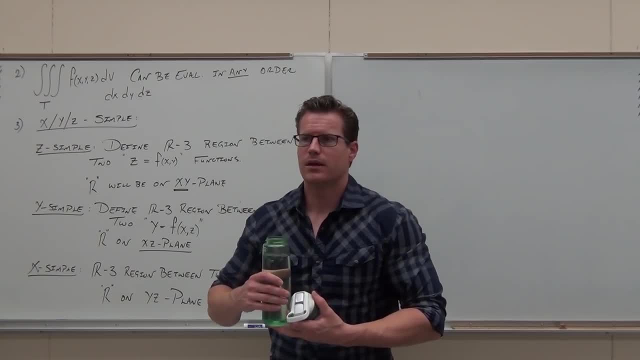 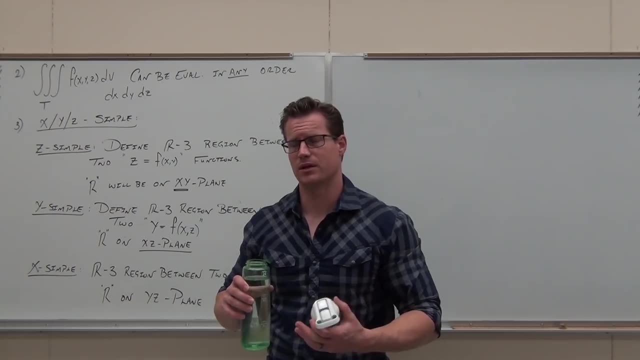 Set up ones or ones you have to set up. Which one do you have to set up? Yeah, It's really pointless for someone to give you an integral that's already set up on a test. It doesn't show that you know anything besides how to plug in numbers. 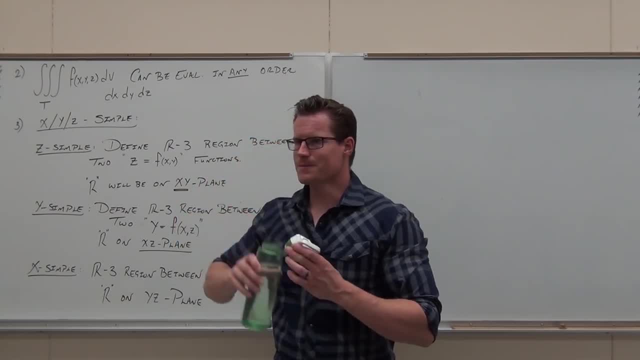 That's not going to happen here. I think you guys are better than that. I think you actually know. No, I'm not. I'm not better than that. I want to set up. Please, I'm not going to do that man. 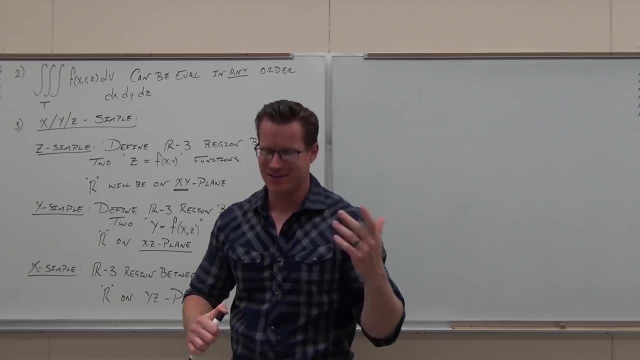 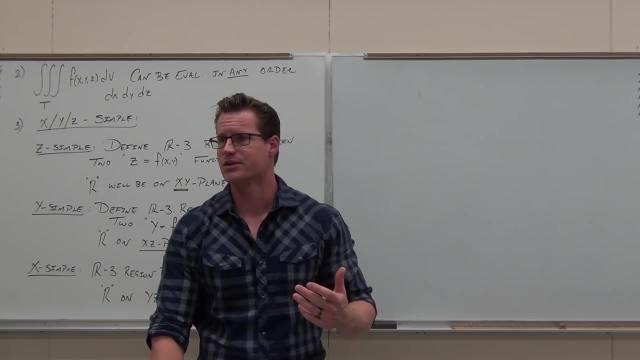 I trust that you guys can learn this stuff really well. I know that you can. You did excellent on your last test, So that's what's going to happen. I'm going to show you how you actually set up triple integrals, so that way you don't get lost in the hard stuff. 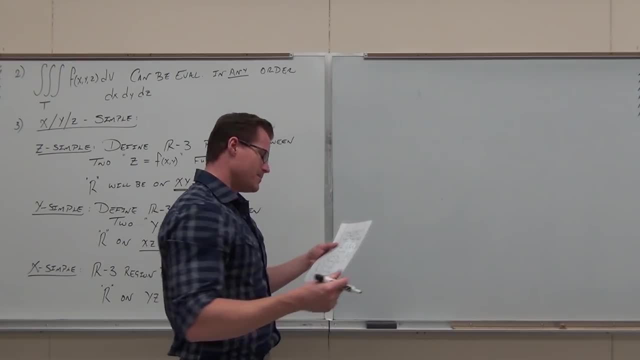 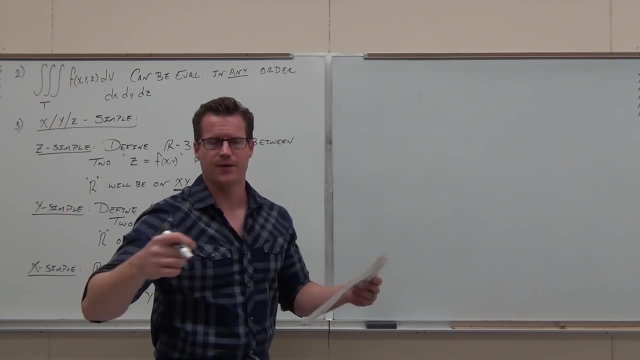 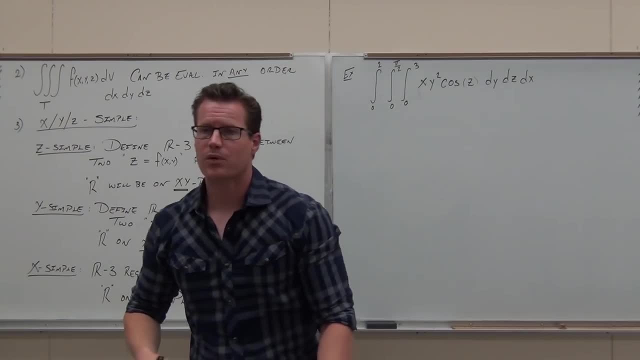 No, No, No, No, No, No. Okay, obviously there's a lot more to write down, There's a lot more to keep track of. That's one of the big things right there is keeping track of what's going on. 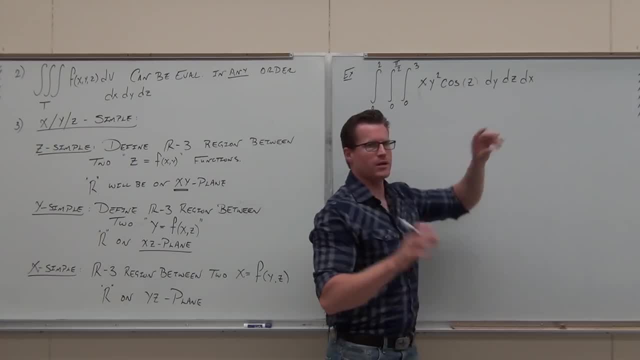 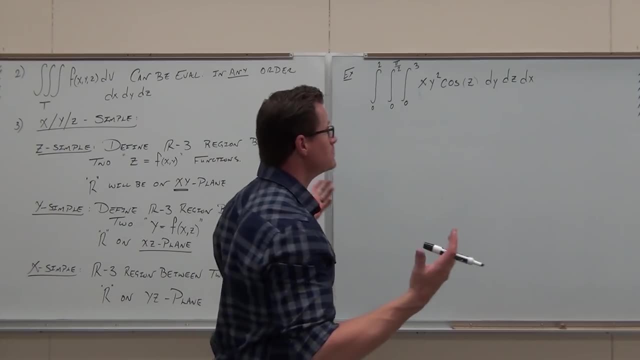 So first, let's kind of look at this thing. Could I start reordering these things, these integrals? Answer is yeah, it doesn't matter how you order them. Sometimes we get a lot easier integrals when we do reorder. 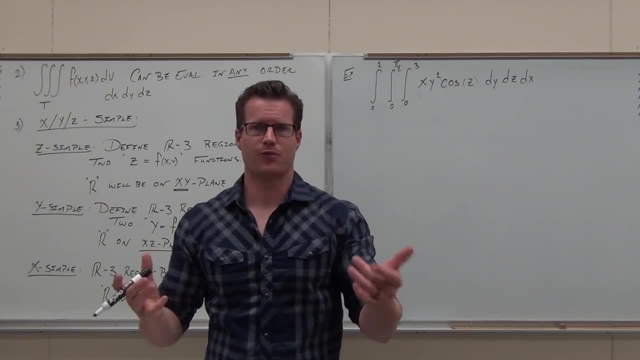 Sometimes it's easiest the way they are. My advice to you is: if one's set up for you, try it first. Don't try to reorder it right off the bat. Just try it first and see if it works. It wastes a lot of time reordering things that you don't have to. 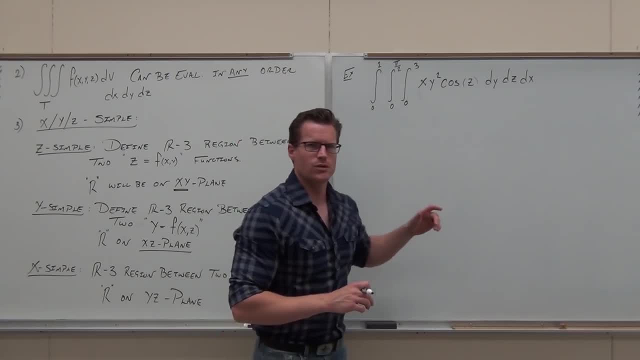 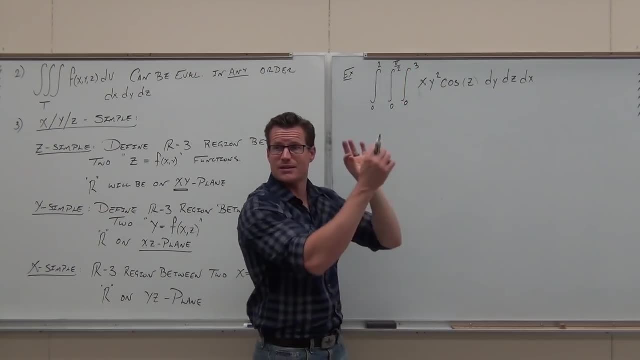 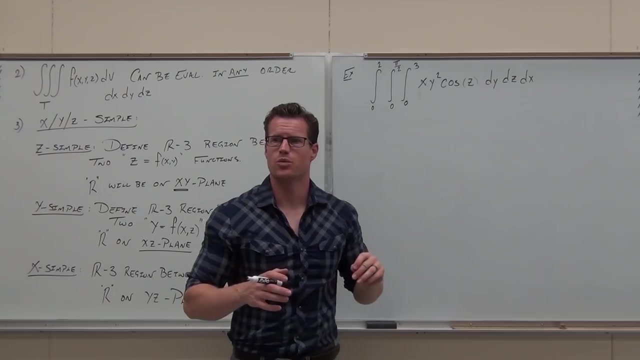 Make sense, So let's try it first. What variables would these numbers be in terms of Y? Good, Do you see how they still have to match up? What variable for these ones Z And these X? What's my first integral tell us to do with respect to what variable? 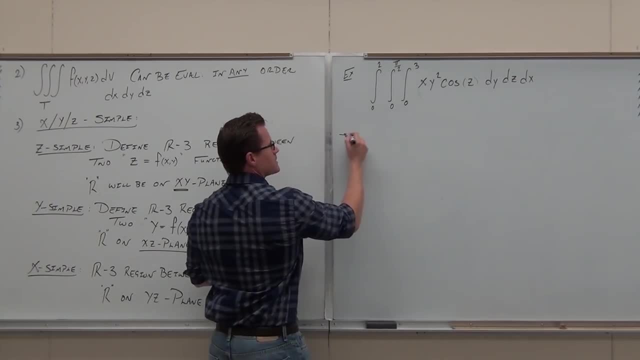 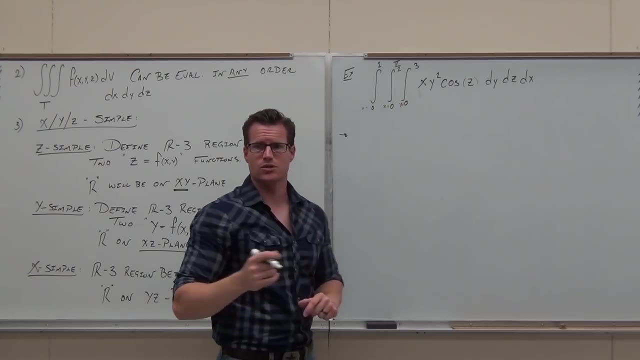 Y, So everything else is held constant. So this integral says: let's keep. and you can write out: X equals Z equals NY. If that helps you, like I showed you last time, you can do that. You can still do it. 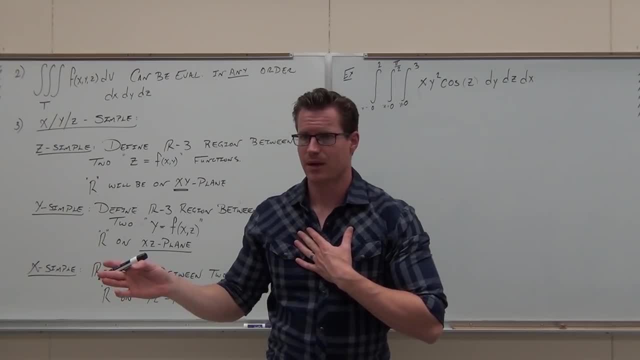 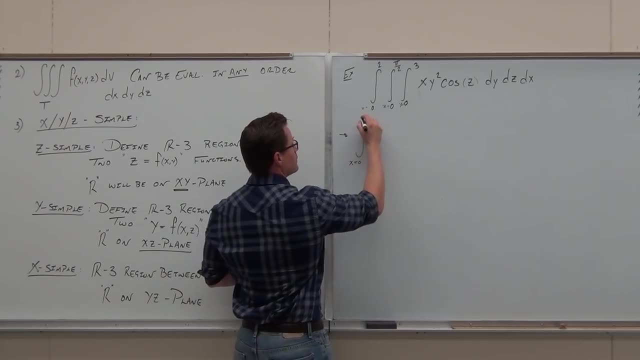 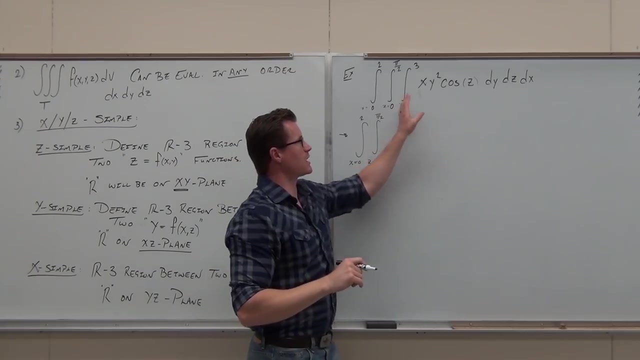 I don't care For me. it's very helpful. I like doing that, But that's up to you. Maybe even just on one of them. Also, make sure you're only touching the correct variable when we're integrating here. So if I integrate this with respect to Y, which it says, do that first. 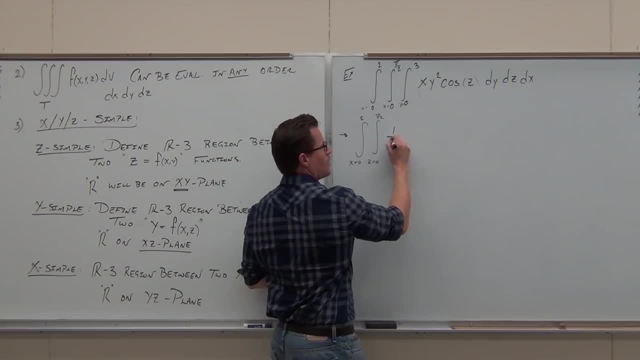 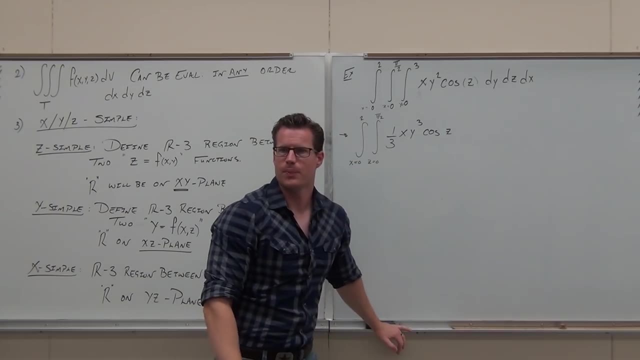 we do it with the first inside integral. first it says that we're going to get this One-third X, Y, Q, cosine Z, And now that you're okay with that one, Yes, no. Now what do we do? 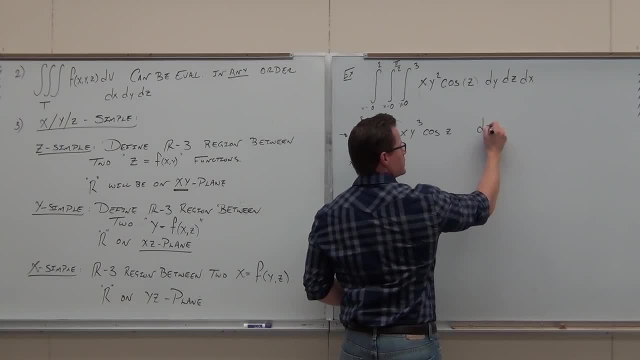 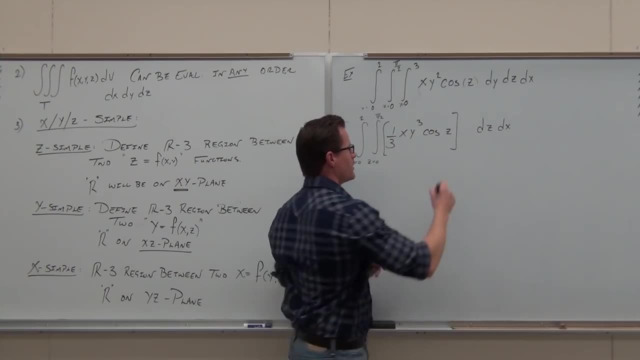 Immediately before we start doing the other integrals. what do we do? So we're going to evaluate it. What variable is getting evaluated? That's why we write this stuff. That's why we're doing this in order of Y. I know Y equals 0 to Y equals 3.. 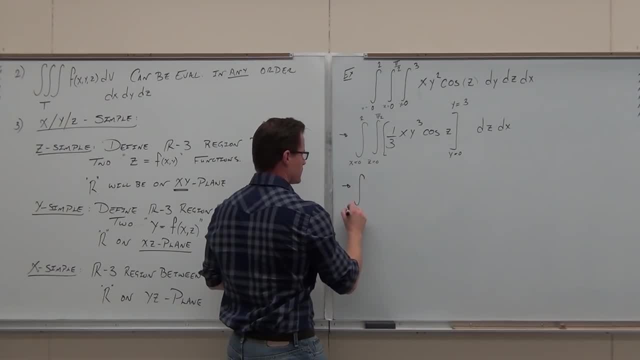 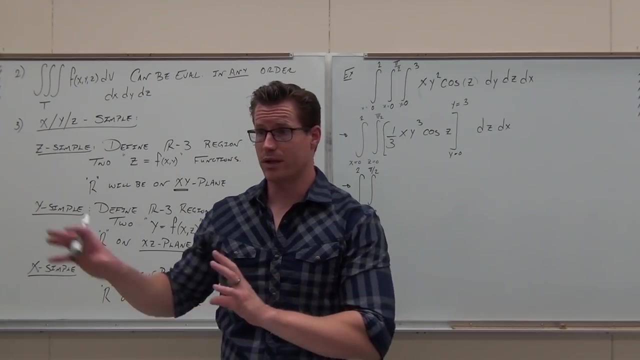 We plug in the 3 first. You can speed through these. However, my goal here is not to get you to show me as many steps as possible on triple integrals. My goal at the end of this lesson is to get you to set. 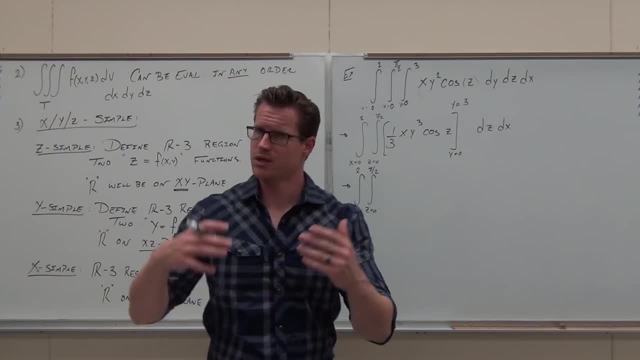 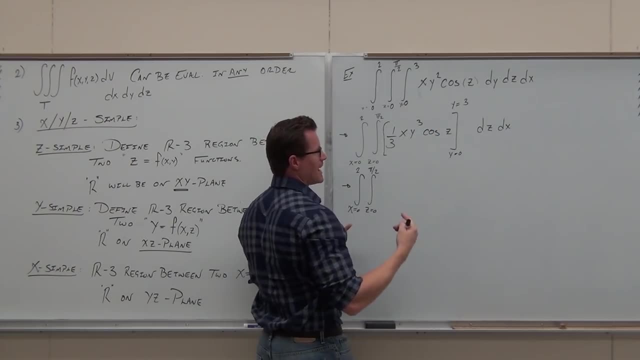 up triple integrals flawlessly. That's my goal. Okay, Your integration techniques. you know those. There's no more for us. So here we get this: 27 divided by 3. It looks like we get 9XY cubed. sorry, 9X cosines 8.. 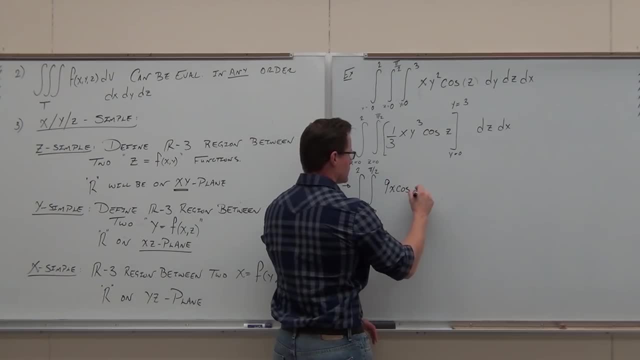 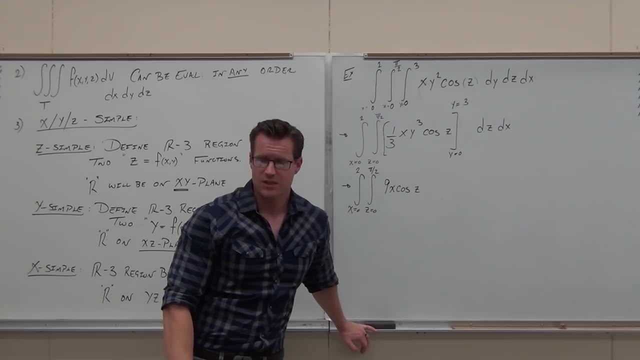 Cosines 8.. The Y equals 0,. that's completely gone. It already looks a whole lot better. Still okay with it. And then we do have to keep this in order, though. It's got to always match up our variables. 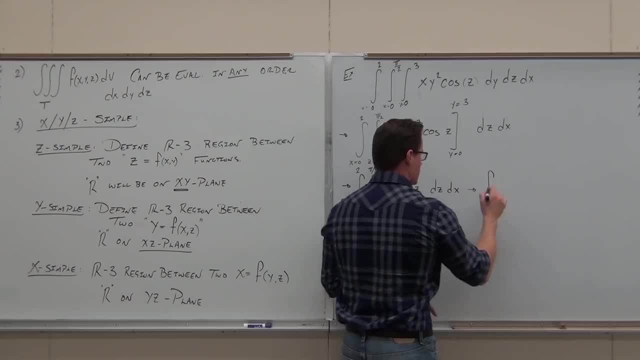 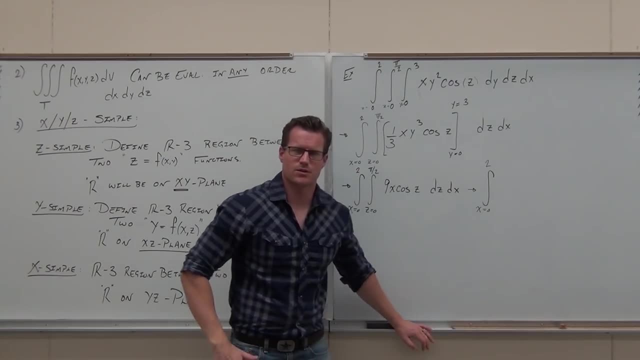 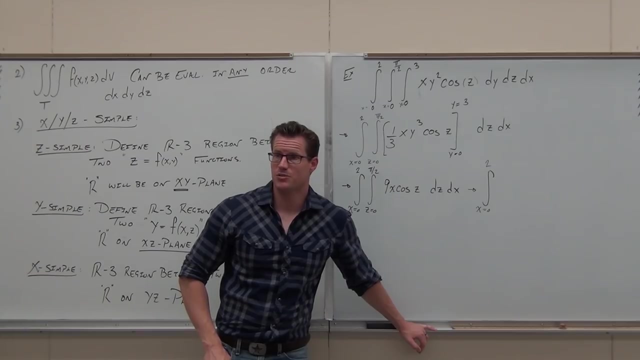 So Zs have to go next. Hey, what's the integral of 9X cosines Z, 9X, 9X, I'm sorry, Negative or positive, Positive, Positive, Positive. Be careful, That's the most often mistake in probably Calc 3 when dealing. 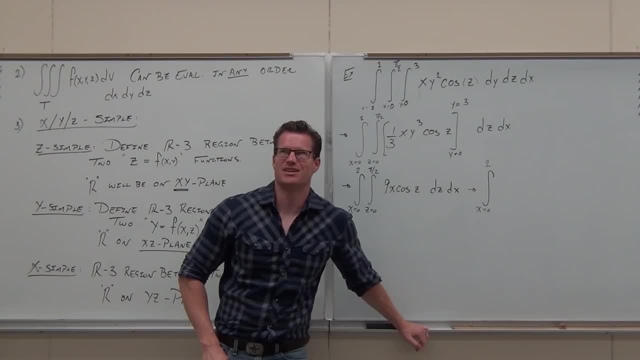 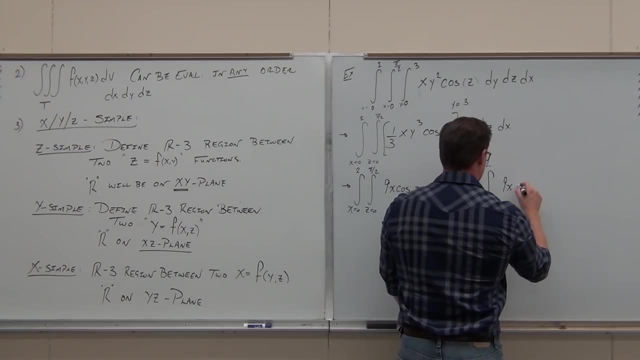 with treatment is we do integral of cosines, negative sine, because I love it, And you go: no, no, that's derivative. You go to opposite, Sine, Sine. And before we continue, before we do our last little integral, 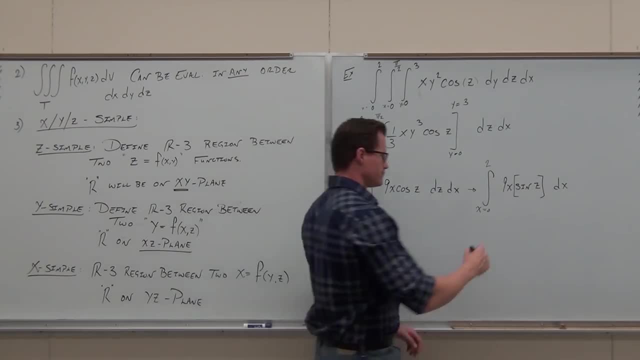 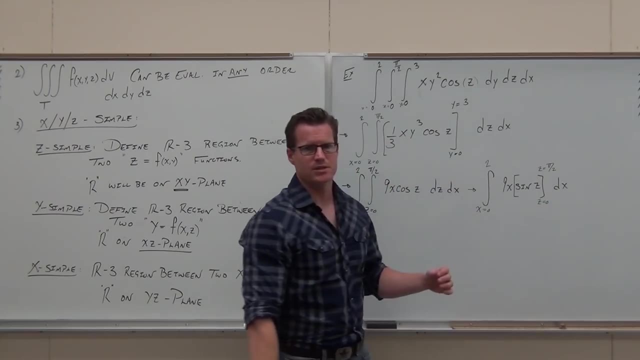 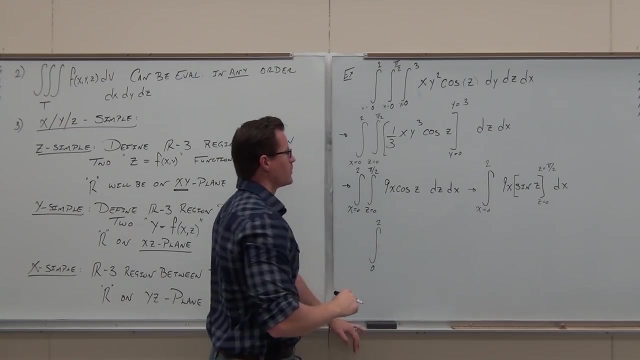 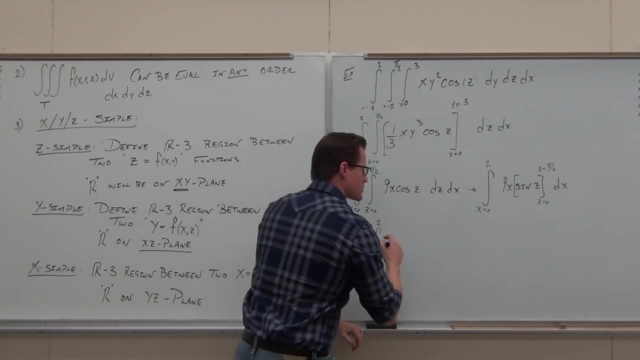 here, sine of 0 is 0, I love when that happens. Sine of pi over 2 is 1.. So this gives us integral from 0 to 2L. you know what We went from 3D to 2D to? we went from triple double single works, works great. 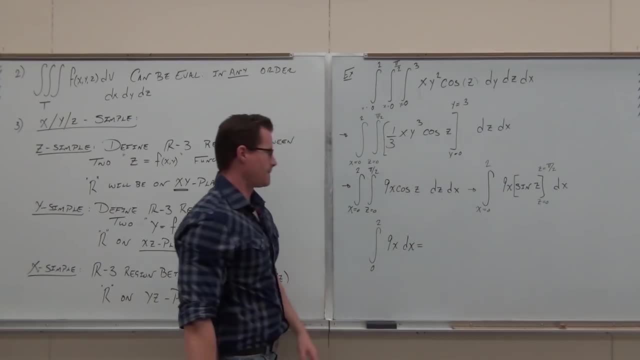 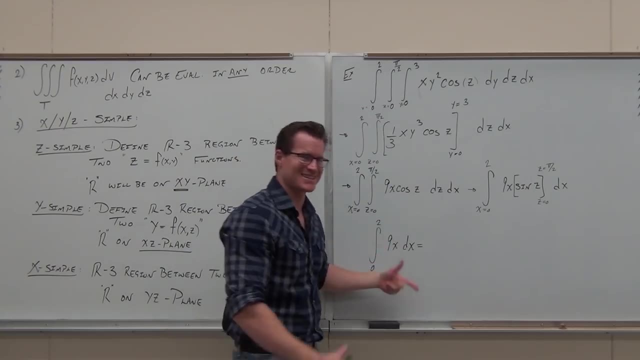 Matt, we haven't had one like that in a while. Yeah, Yeah, We haven't had one like that in a long time. I love this class. Don't you love this class? That's crazy. This is easy, I love that. 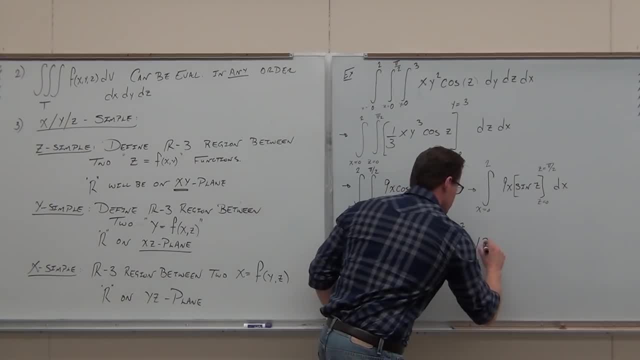 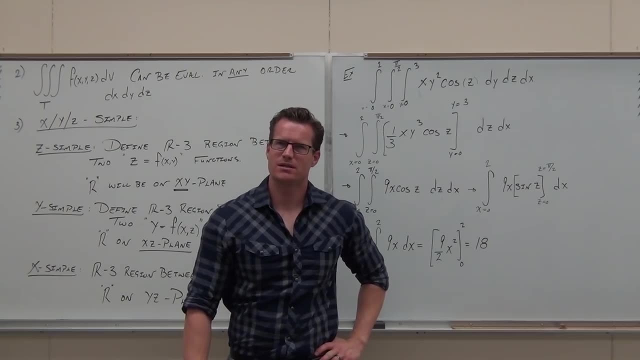 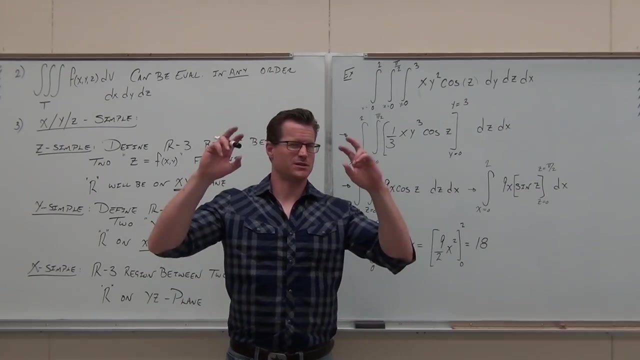 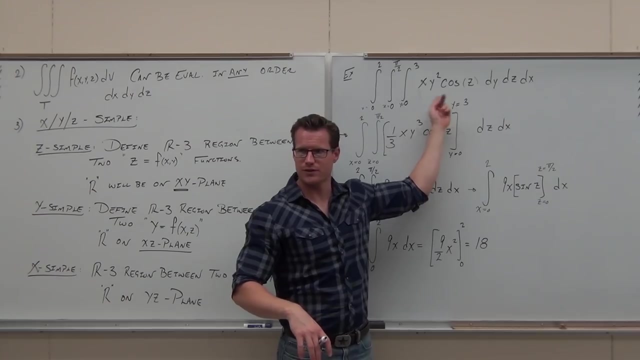 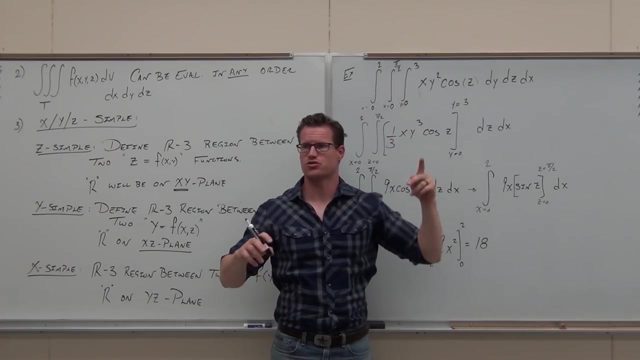 What do you get? 18.. 18. What's it mean? What's it mean? Well, it depends. It's either the volume measurement under that verify 4D, 4D surface here. this is either the volume for 4D over that 3D region, which is extremely hard to think about, or, if that's, 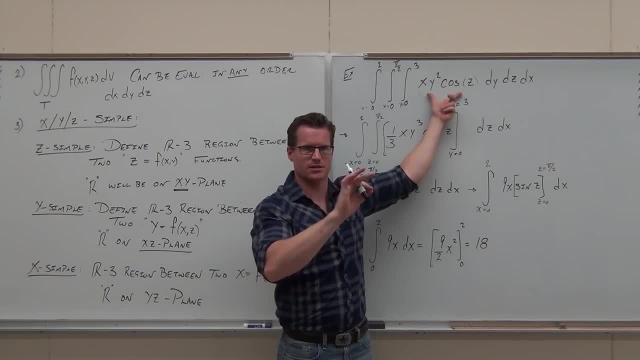 the mass density function that tells you where the mass is, the mass density are located on this 3D image. Notice: this is 3D, This region, this T is 3D. This would be the mass of that 3D region if that is the mass density function. 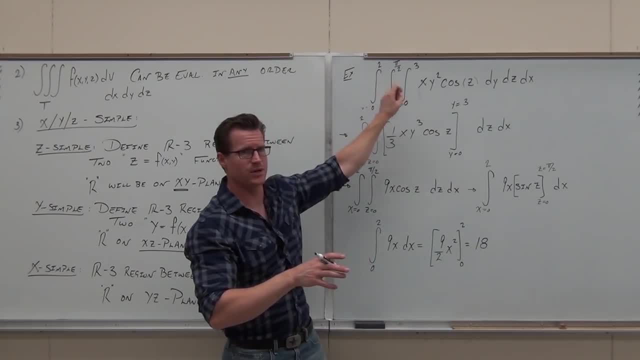 That's what that represents. That's typically how we think of it, So you may feel okay with that one. Okay, Tell you what I want you to start. one more, Little more challenging, but it's honestly the same idea, Just something interesting happens there. 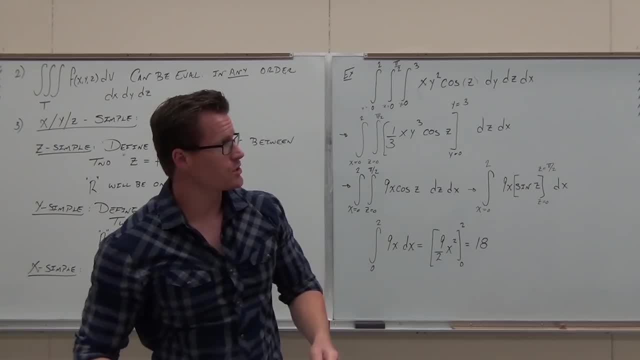 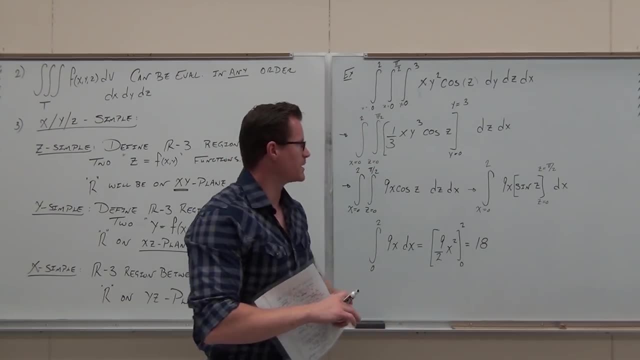 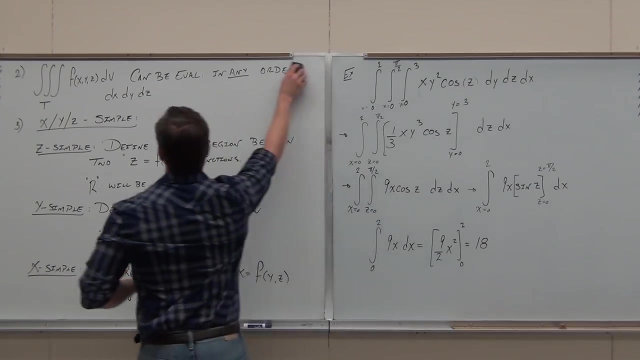 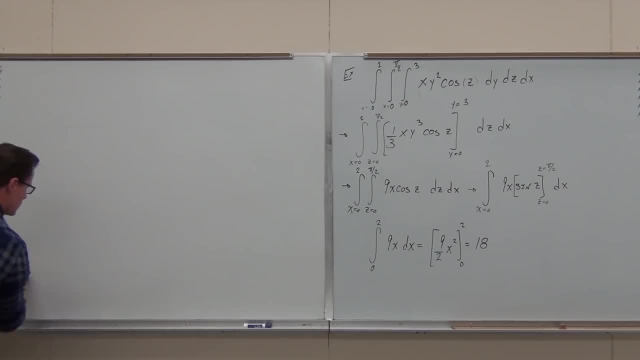 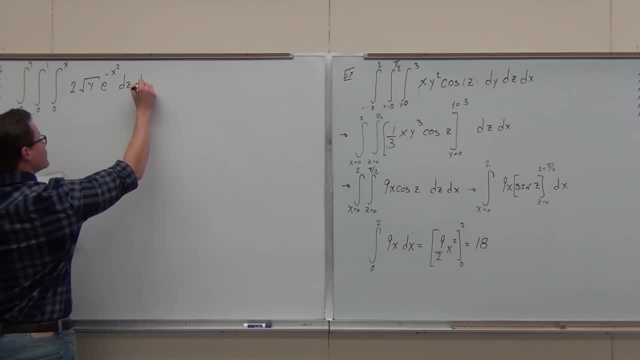 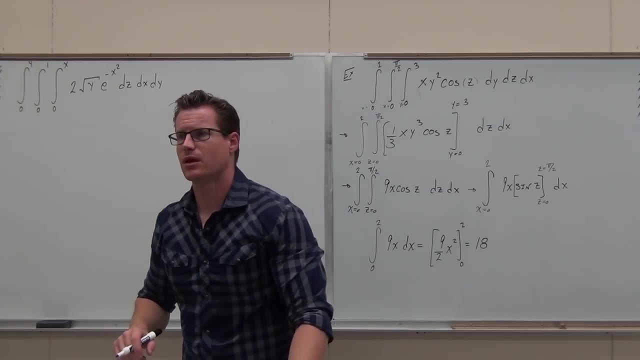 Okay, Okay, I want you just to do the first step. That's all I want right now, just the first step, and then we're going to run through the rest of it real quick. Maybe write out what the bounds of integration mean. 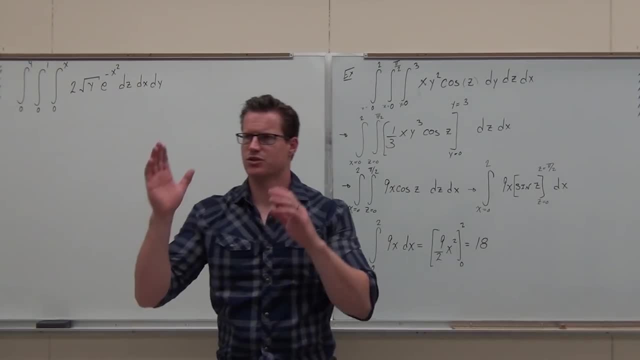 what variables those are related to. That's the first thing I always do. I look and make sure that I have x's with x's, y's with y's, z's with z's, to make sure I'm not plugging in the wrong things to the wrong variables. 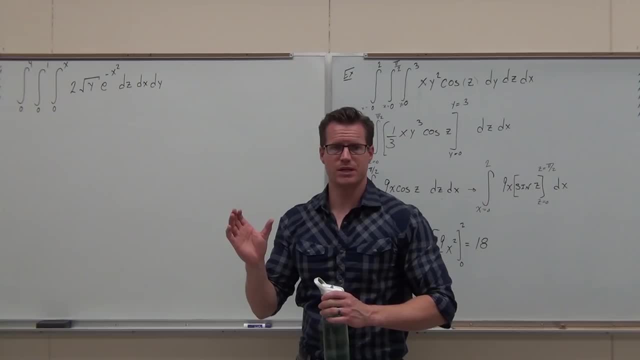 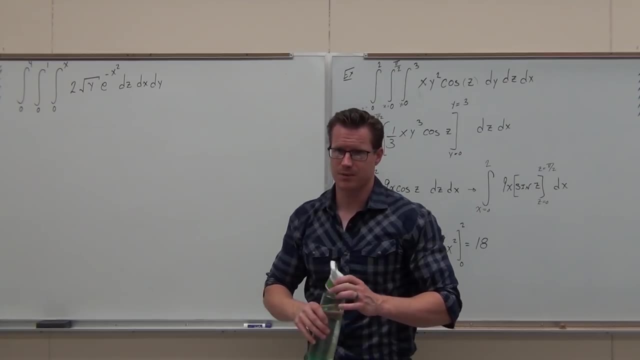 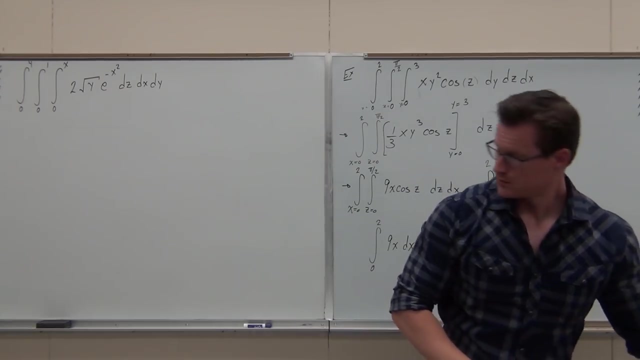 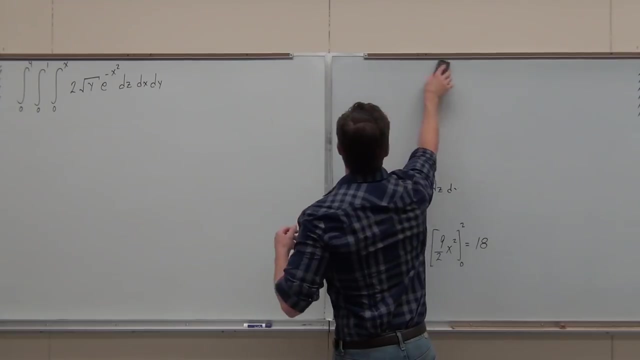 The problem here with 3D is you have a lot of choices. With 2D it was easier because you- only you- know that you have only one option for your other variable. Here you get a couple. Okay, be careful. Hey, what's your first independent variable? 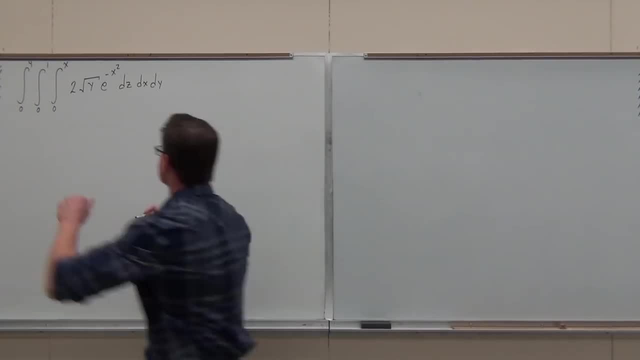 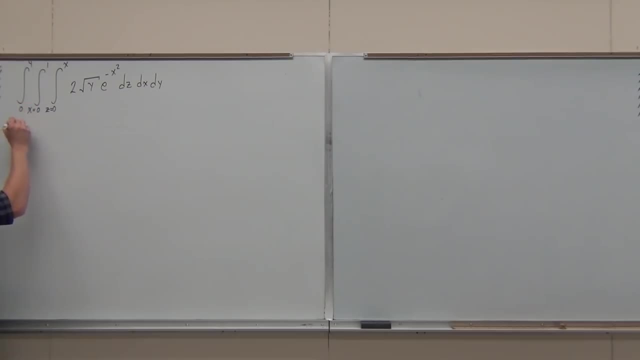 What's the first thing you integrate with respect to What is that Z? Okay, that means that These first two numbers are z numbers and these next ones are- Oh, thanks for the help on that one. guys appreciate that. and y. 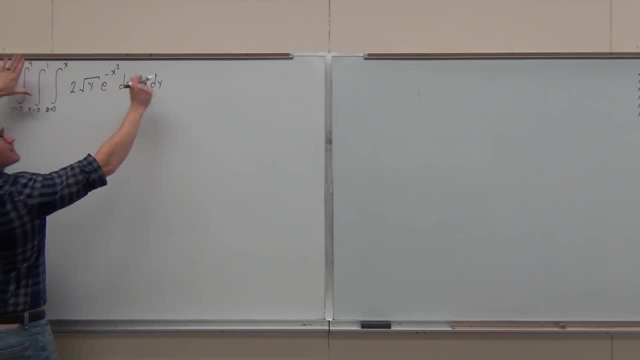 So when I look at my first integral, just this guy. I leave the rest alone. All I care about is this: That's it. So when we do that, we're still going to have this: y from 0 to 4, x from 0 to 4,. 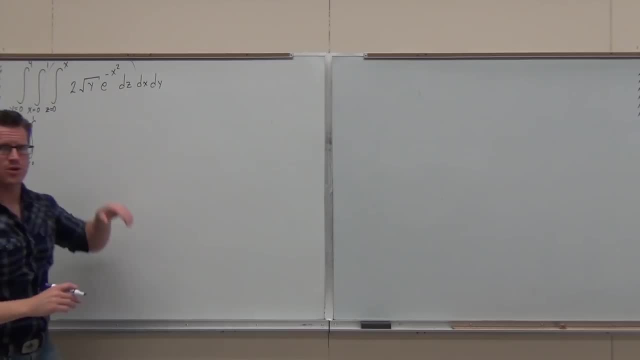 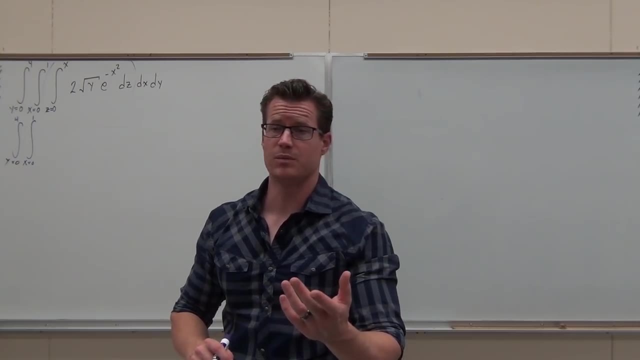 and y from 0 to 4.. So we're still going to have this y from 0 to 1, I'm just focused here. You can tell probably why they set this up as dz first, because the x would be impossible, the y would be nasty and the z would be easy. 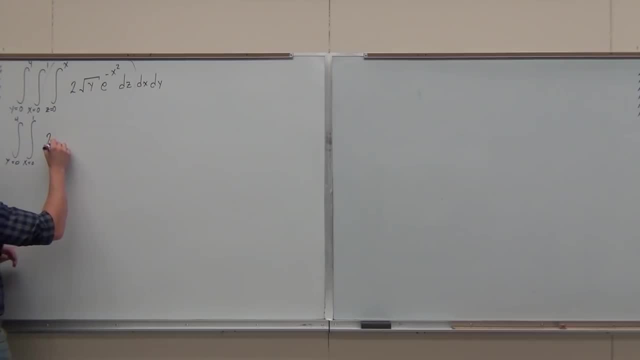 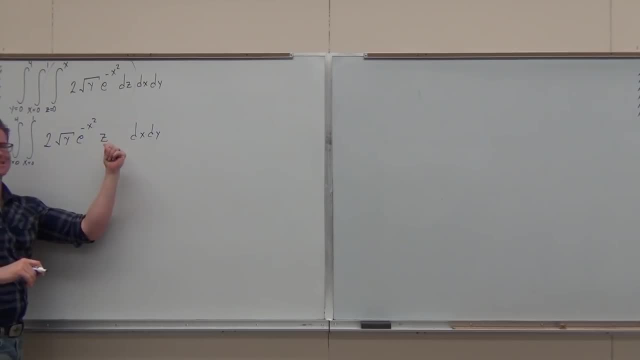 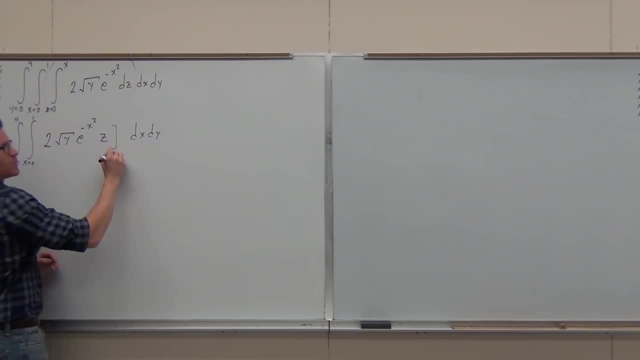 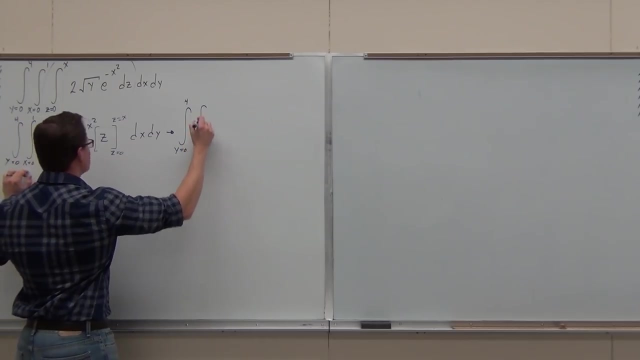 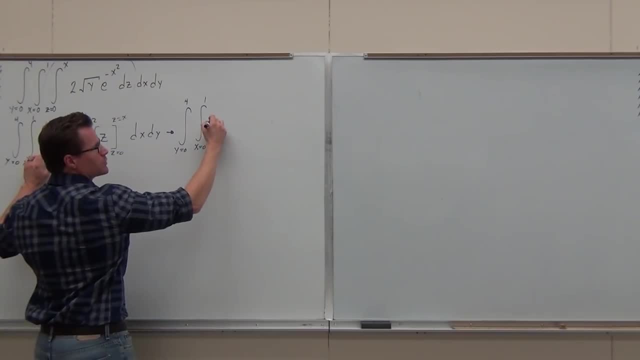 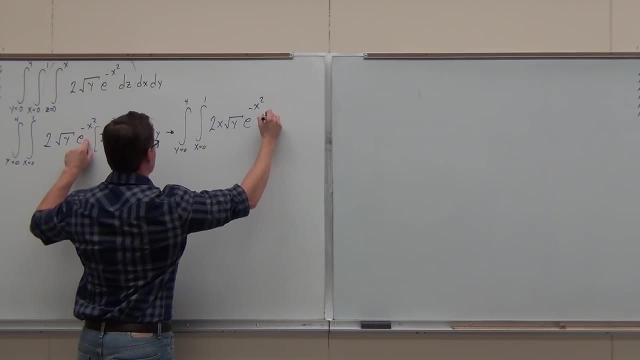 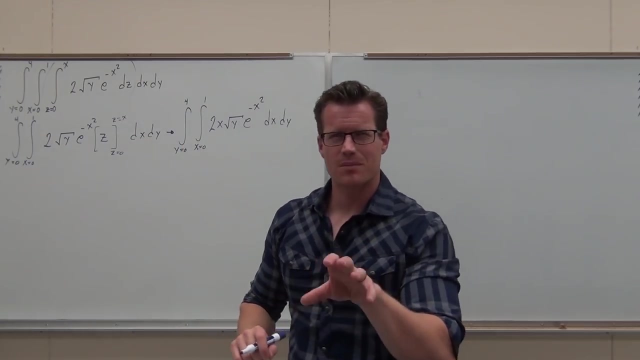 Plug in zero, we get zero. You're just getting an added x in here. Well, multiply it Now. is it a problem that we're going to do dx Next? X should be my next independent variable, And it's just a double integral. 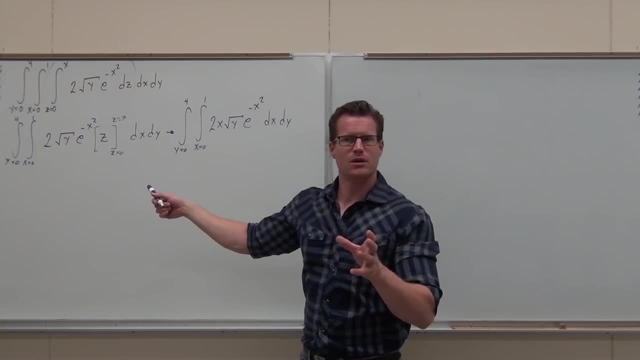 Is that going to be a problem? No, What would you use? Try the use of. Try the use of Go for it. I'm going to do it on the board as you're doing it, but I want you all to try it. 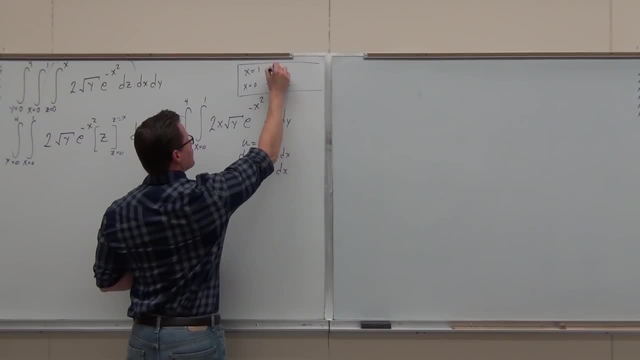 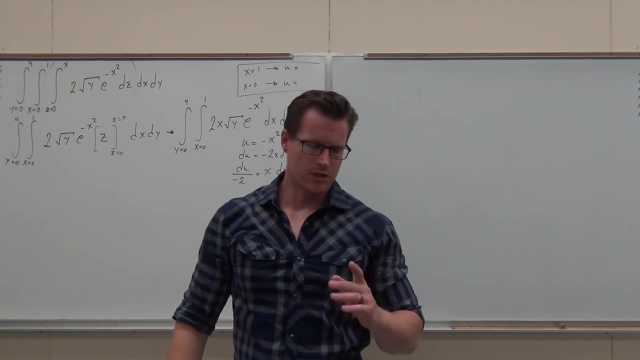 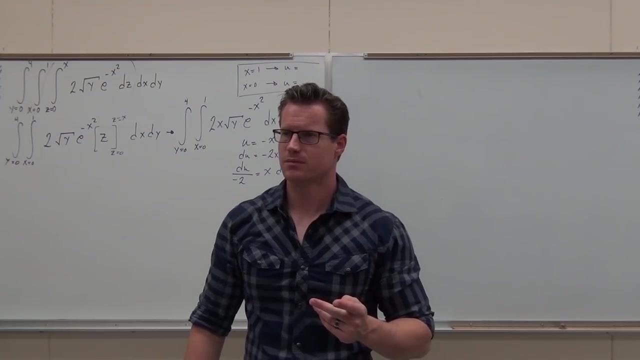 I just got through telling my count one students that we do use subs and changing bounds on practically every single one of these. Have you noticed that It happens an awful lot? Change your bounds. I tell them all the time: change your bounds. 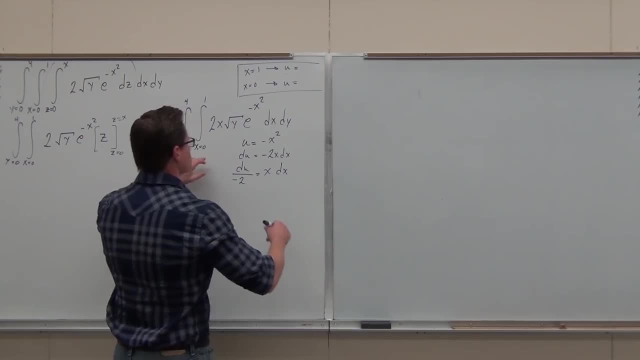 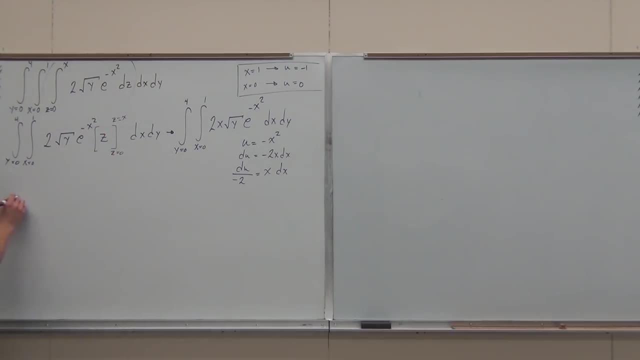 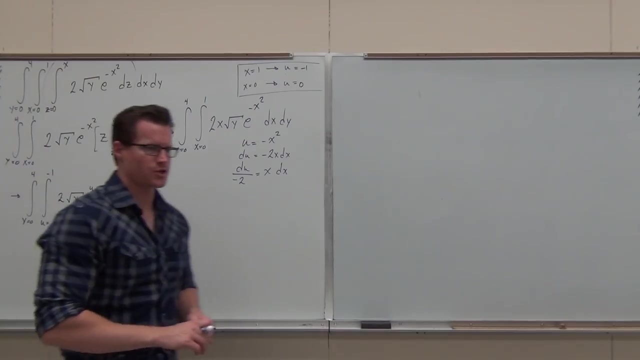 It makes your life easier. so you don't forget anything later, Change your bounds. I want to pause you here real quick to make sure we're on the right track. We're on the same page. If we pick u as negative, x squared. 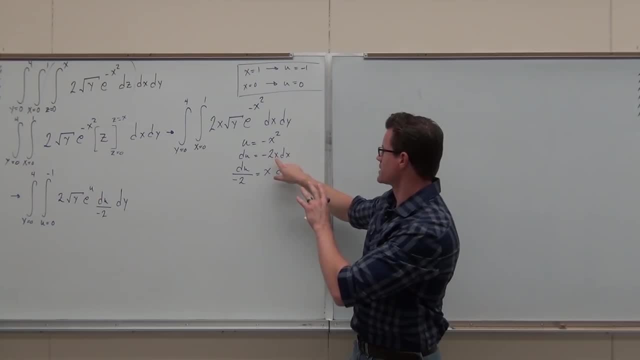 which is the correct choice. we're going to get this negative 2xdx. You can substitute right from there if you'd like. That's fine. I always solve for du over the coefficient. That's the way I do it Most of the time. I'll solve even with the variable over there. 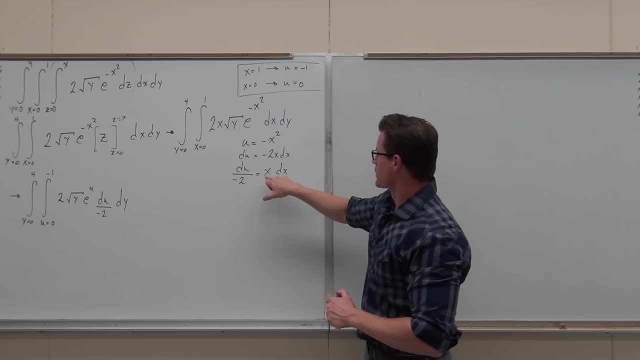 and cross this out. It just depends on the technique. I don't care. Here we go. Okay, The xdx. this is going to get replaced with du over negative 2.. And I'll get you with me on that one. 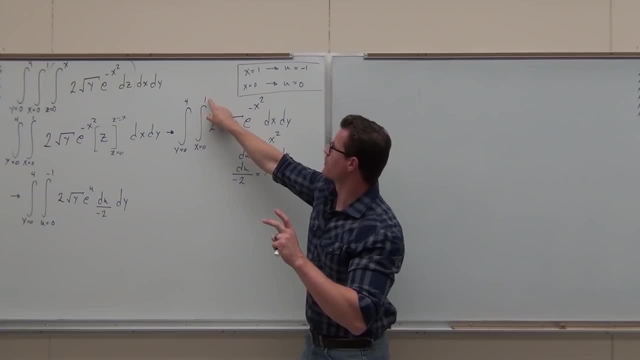 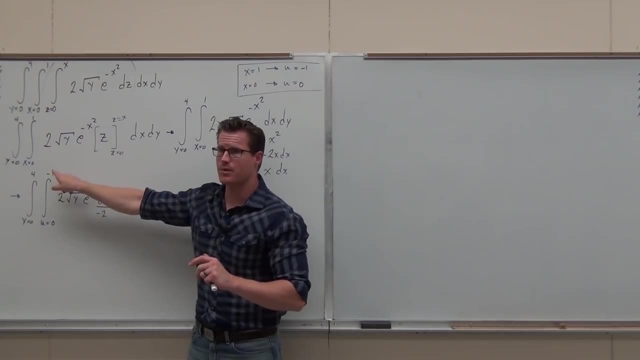 If you change bounds, though, you have to make sure that where the xdx is going to be, all this x values mapped remains in the same place. So if I map 1 to negative 1, negative 1 is on the top. 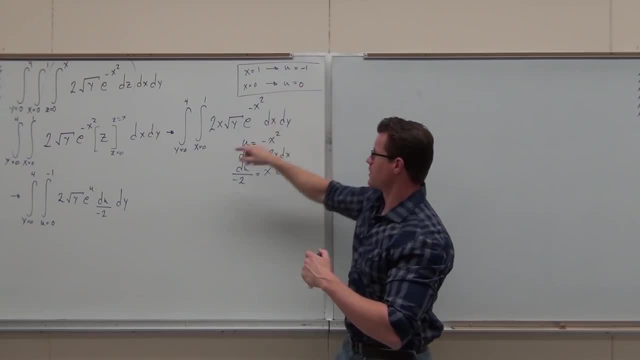 You can't just arbitrarily switch those every time you want. 0 got mapped to 0. That's still on the bottom. So if you can just feel, okay with that one Now there is a problem with this. What's the problem with that? 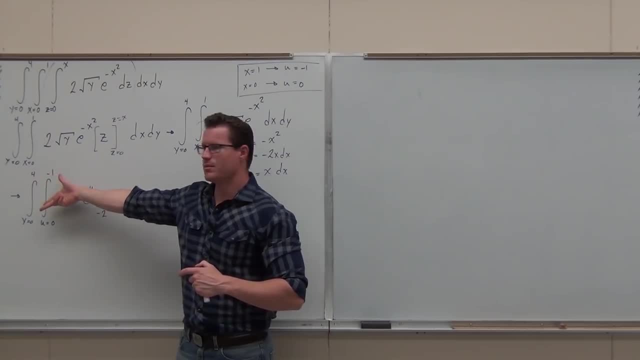 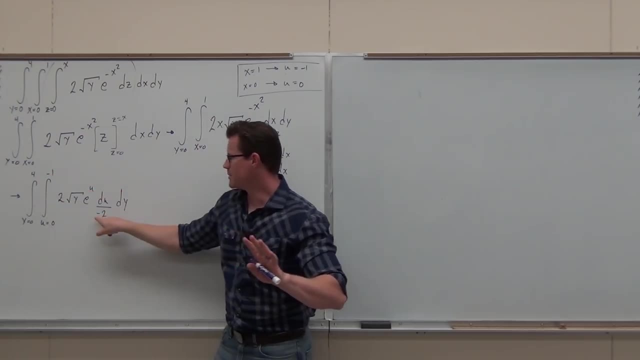 Negative 1 smaller than 0.. So if I switch them, what's going to happen? Change the sign. So here's what I'm going to do. Don't get lost, You're going to miss it. I'm going to switch these around, but I'm going to eliminate that sign. 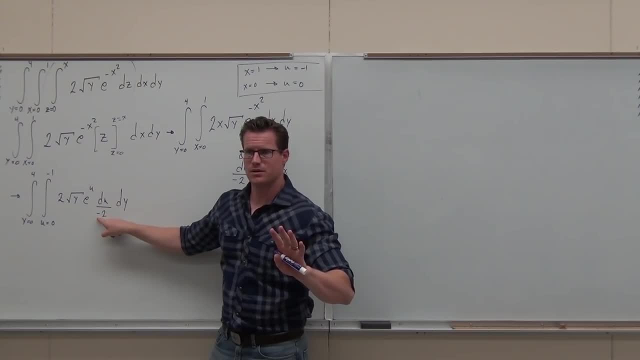 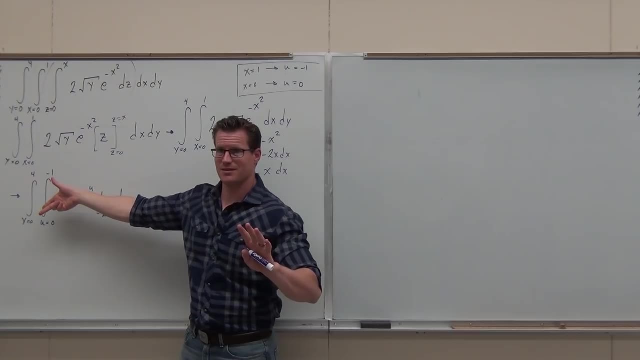 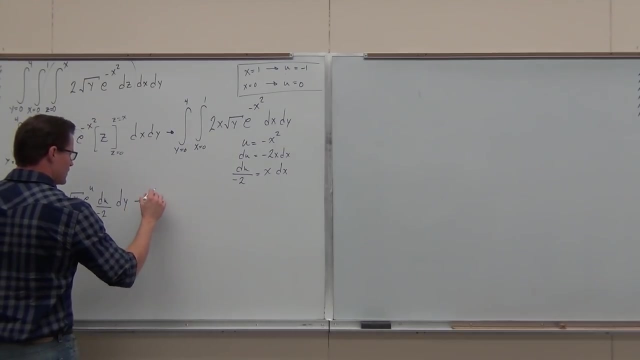 You guys see that. Okay, Yes, no, Say it again. Switcheroo changes the sign. No, Say it again. Is it 2 on the square root of y together? Does that answer your question? I love it when that happens. 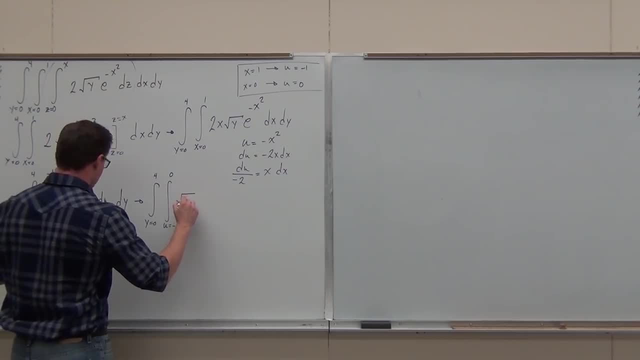 I love crossing stuff out. Okay, if you want to know the whole shebang, here's the whole shebang. You ready for it? Watch, Watch. That negative would get moved right there And you have parentheses, Just like that. 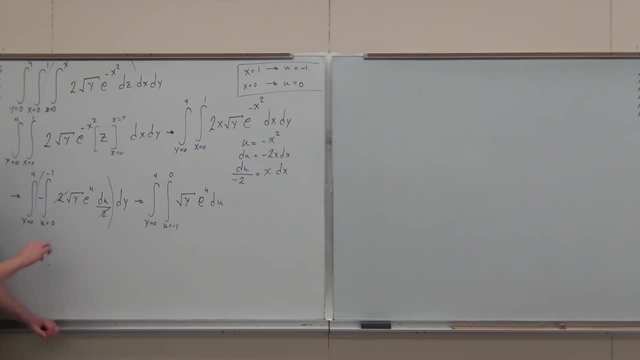 Can you follow that? Look at the board. please Stop what you're doing. Look at the board. That negative that was here would move right there, Not in front. Right there, Are you clear? When I switch bounds of integration, it changes the sign of integral. 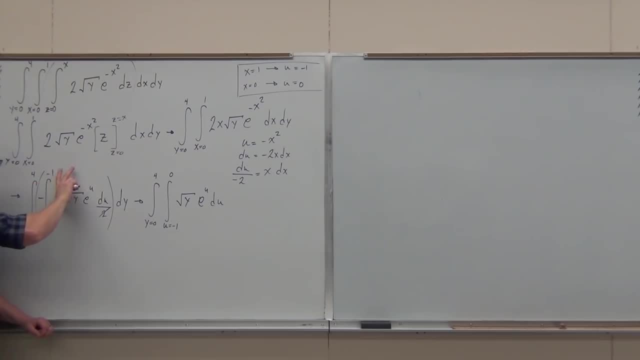 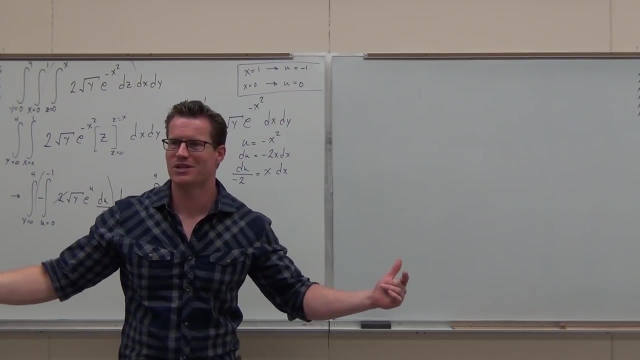 So if I have a negative integral with wrong bounds, if I switch the bounds it becomes a positive of that integral. Does that make sense to you now? You basically have two wrongs making a right. That's the way the real world works anyway. 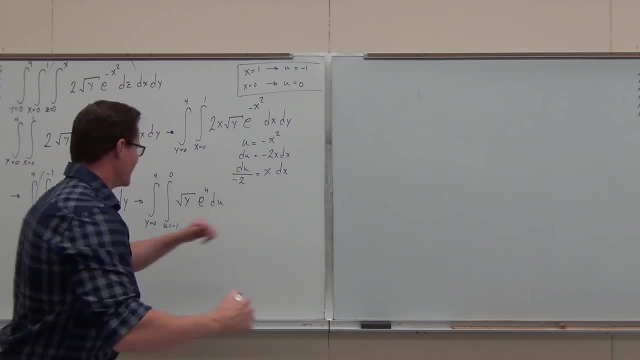 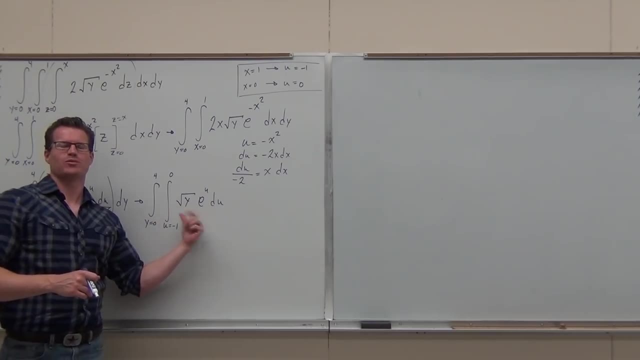 Right, Am I right? Yes, Not right, Wrong, Wrong, But in this case it does. Two negatives make a positive, So we got that From here. Hey, I love that. What's the integral? So we have this guy now. 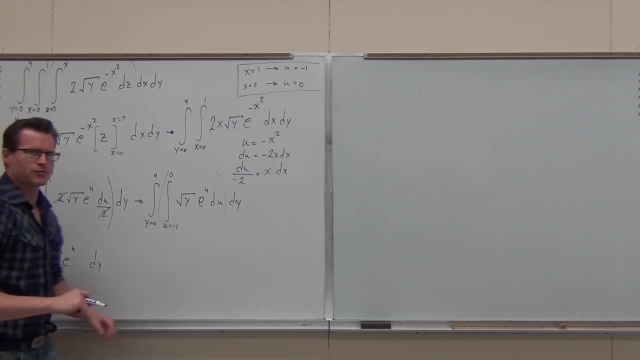 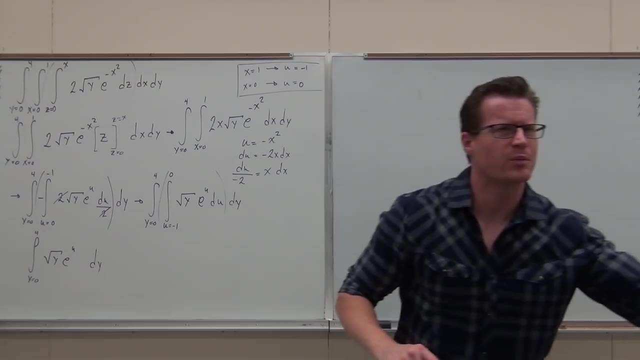 Before we do the final integral with respect to this integral, with respect to y, everyone in class right now, tell me what you must do. What must you do? Plug in, You've got to plug in. for what? What variable would we plug in for? 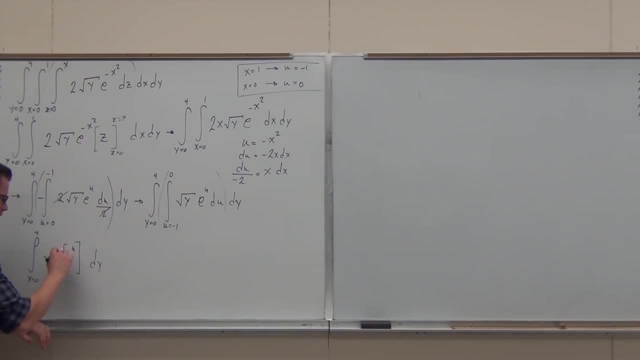 U. So here we would get from what, Which means we have this integral from y equals 0 to y equals 4, and we'd have the square root of y, And in here we get something kind of awkward: We get 1.. 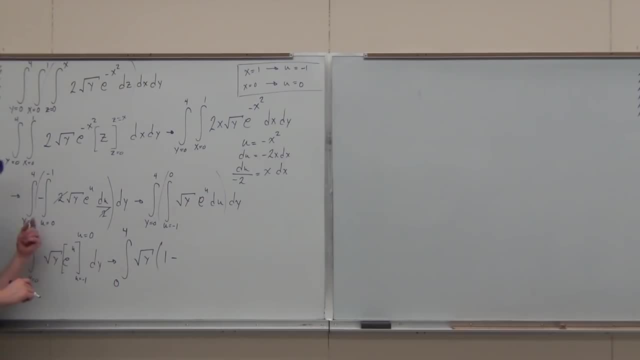 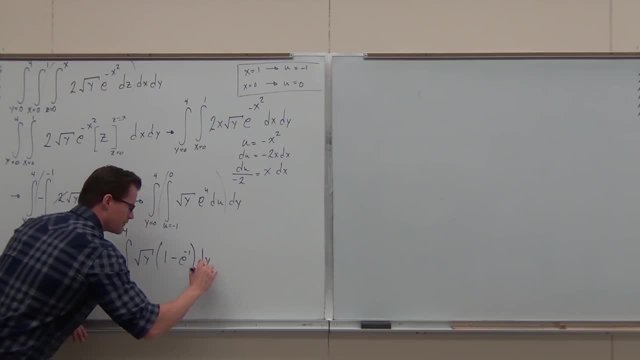 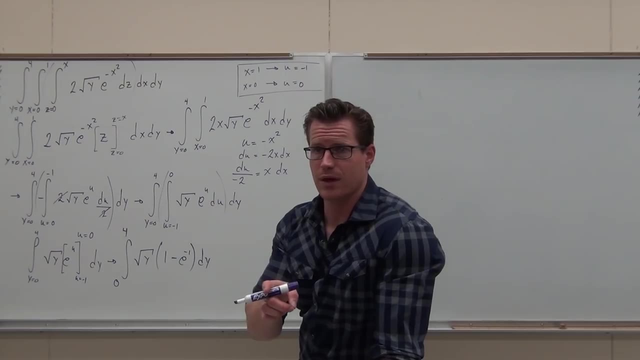 Or you could put 1 over e. It doesn't matter Whatever you want to do, But it's definitely dy. I would love to know if that makes sense to you. Can you follow that one Now? after that, is it possible to integrate that? 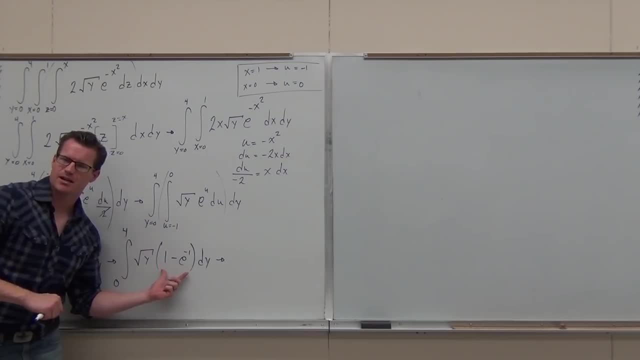 Yes, This looks crazy, but you all tell me what that is. What is that? It's constant. It's just a number. You can even pull this out front. So that's a square root of y. So we're going to get that. 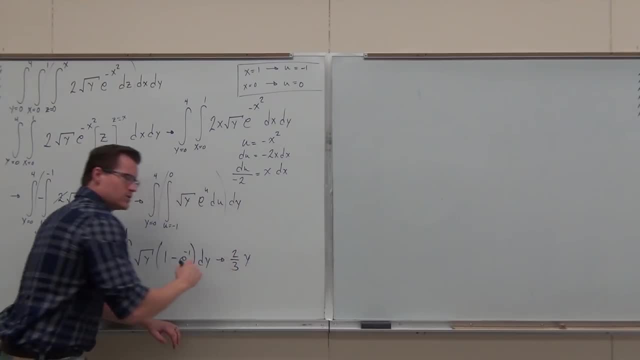 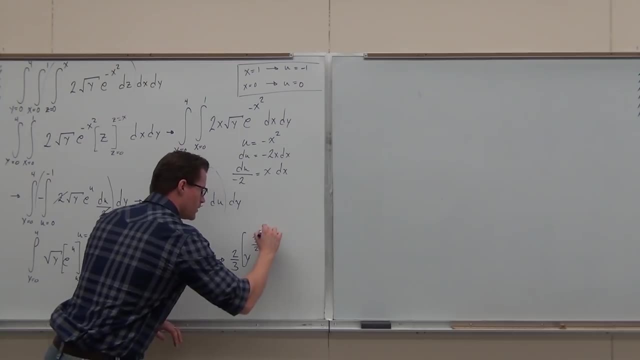 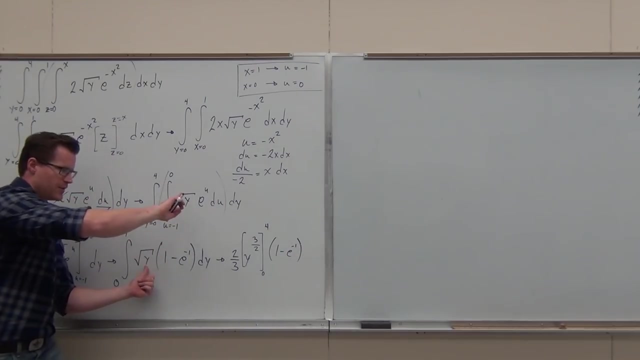 that two-thirds y to the three-halves evaluated from zero to four, and then we'll multiply by that constant. Add one, you get three-halves. Divide by the new exponent, you get three-halves but two-thirds. 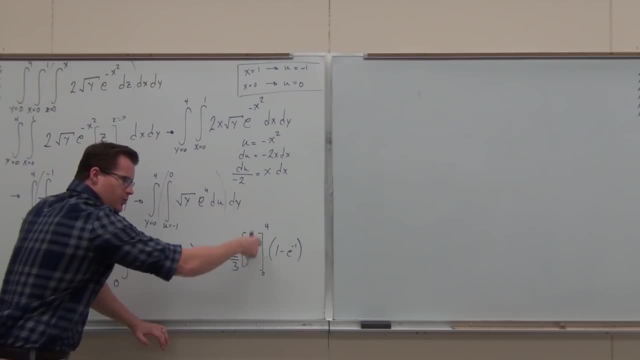 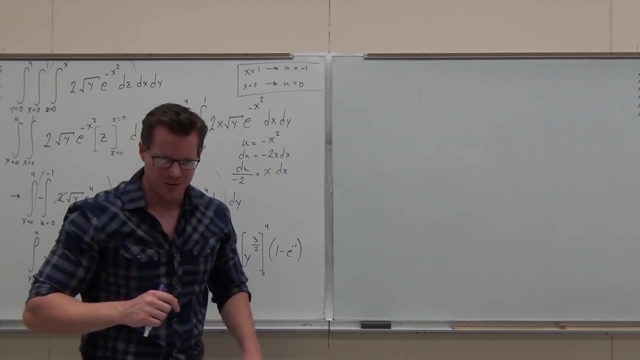 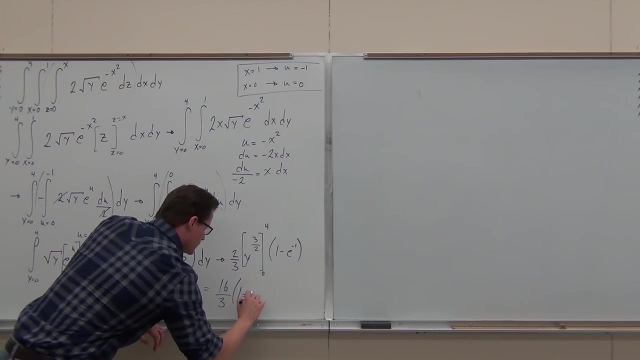 and then evaluate from four to zero. Plug in the four, plug in the zero. the square root of four gives you two to the third. power is eight times two is 16-thirds, and then we have that constant. It's nasty, but that's the answer. 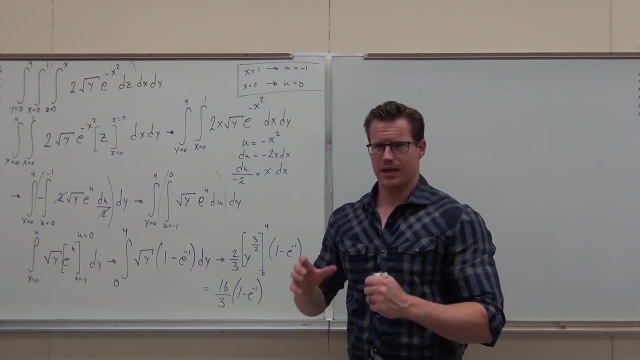 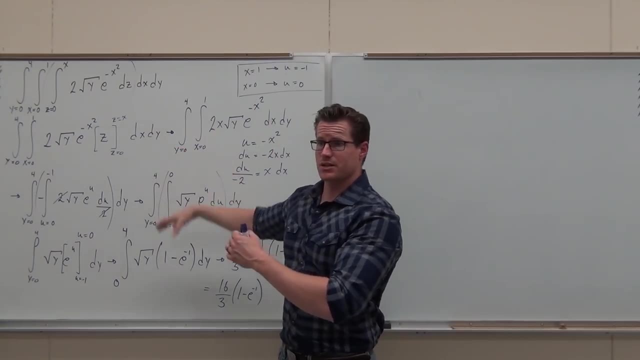 I know that was pretty quick, but I understand it's quick. I'm doing this quickly to not get you to repeat your knowledge of integrals, but just to get us down to the final answer and show you how all this stuff works. So here's our little recap. 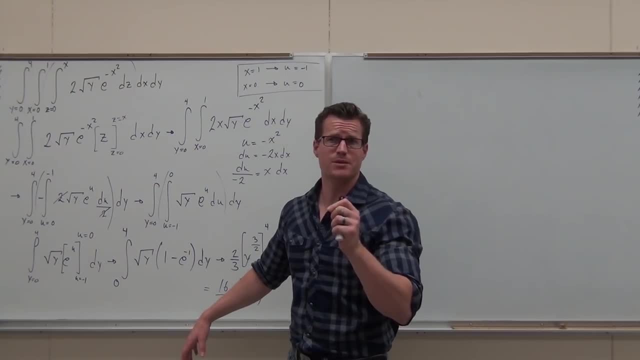 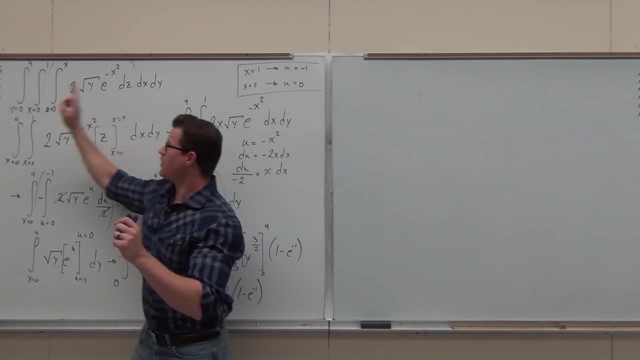 Do you feel confident? Do you feel confident about understanding what your first independent variable is? Do you feel confident about matching up this with these numbers all the time, yes or no? So when you set up your own integrals, you keep that in mind. 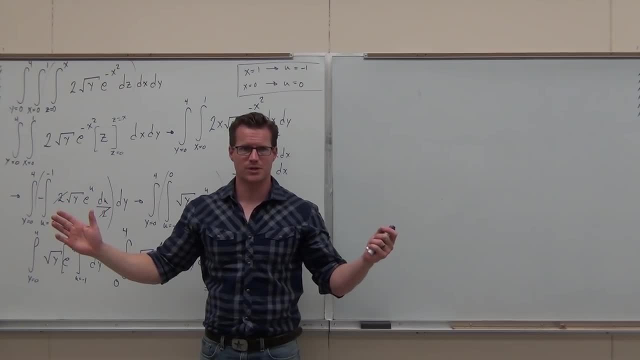 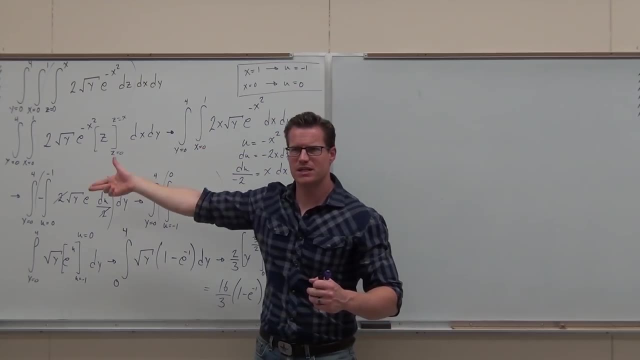 You have to match those up. Order doesn't matter, but you've got to match them up. You guys clear on that one Did you catch? the only reason we really worked this out is to catch the whole bounds shifting, bounds switching and the sign change. 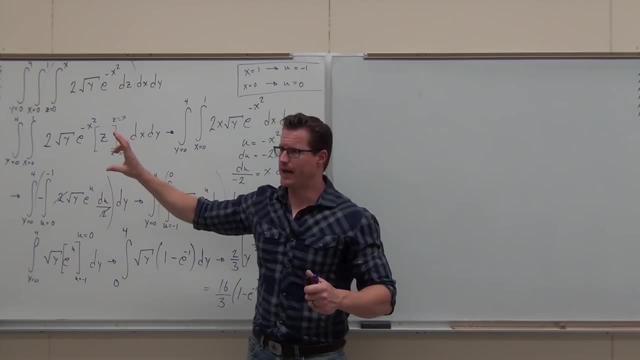 That's a big deal. Did you guys catch that? Change your bounds. That helps a lot. So you don't have to worry about that. You don't have to worry about that. You don't have to redo in here. plug your stuff back in. 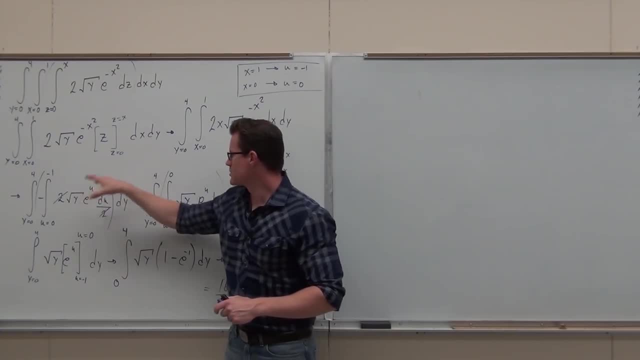 And then keep in mind what we're integrating the spec to. If we still have DUs, man don't change Ys here, Don't plug in for Ys here. Do that at the very end, whatever you have at the very end. 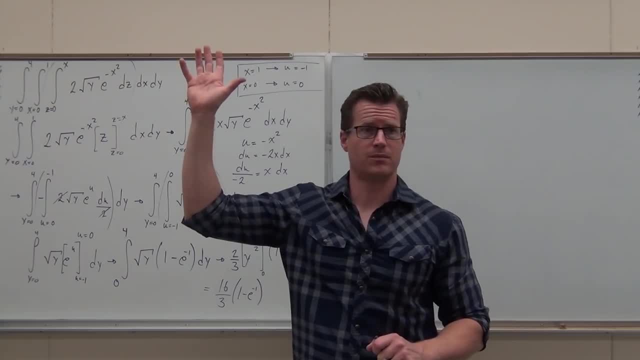 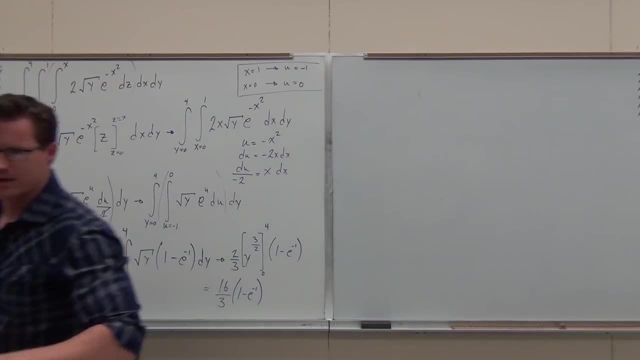 of your integrals is the last thing you plug in for Should have answered with okay, it's for real Comments. questions at all From here. do you feel like you know what to do? Okay, We're going to pause here and come back. 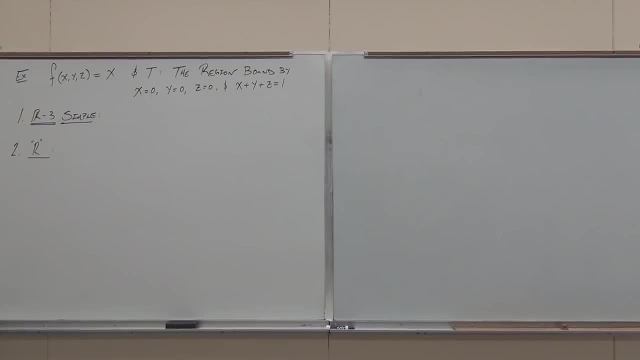 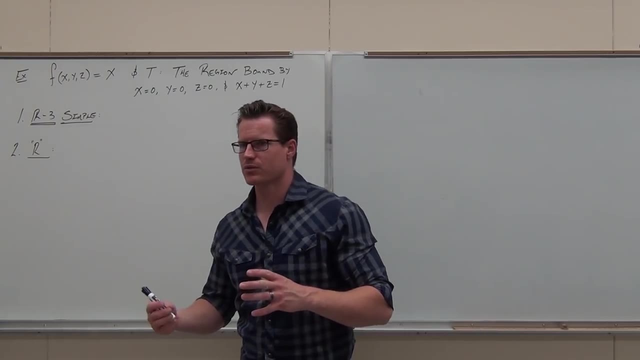 and do some real stuff, set up our own. Okay, so here we go. We're going to get to the real stuff. This is the big stuff: how to actually set up your triple integrals appropriately. The number one thing that I want you to get to know is how to set. 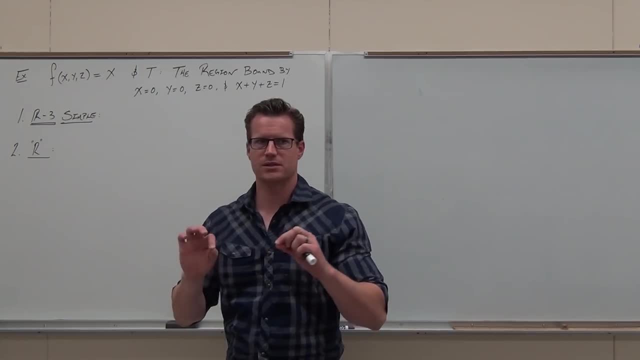 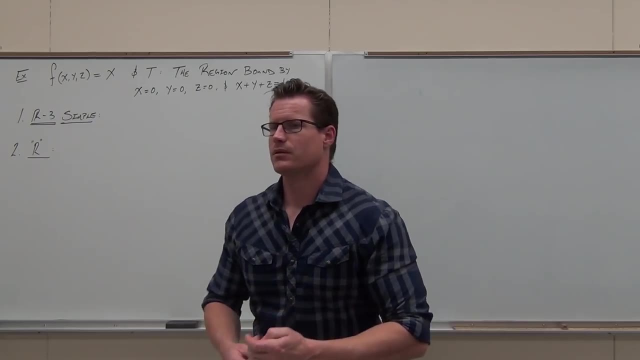 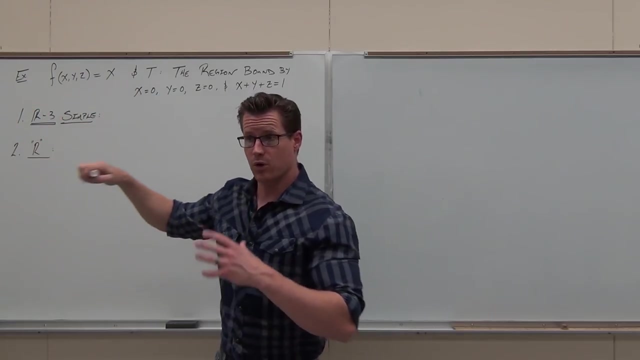 up the integral across the R3 region first. That's number one. So what we call that? we call that R3 symbol. Now, this right here has nothing to do with your region. That is not what we're talking about. What we're talking about is how the region is defined over here. 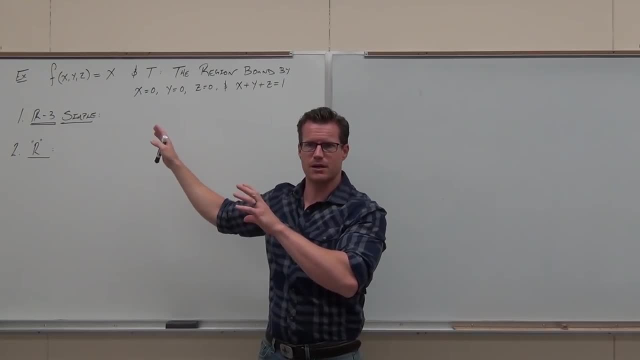 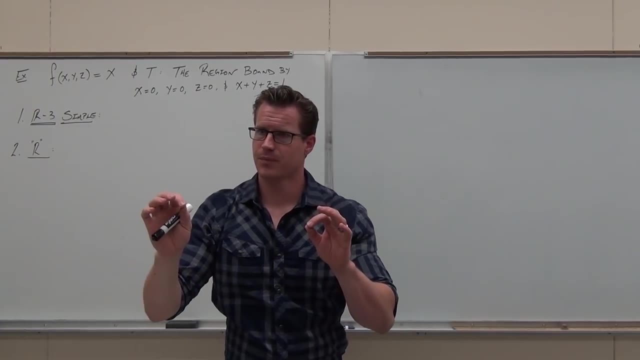 This is what we choose to go across first, And now that you understand what I'm talking about, That's the first thing we do. So we have to choose to go between two functions of z, two functions of y or two functions of x. 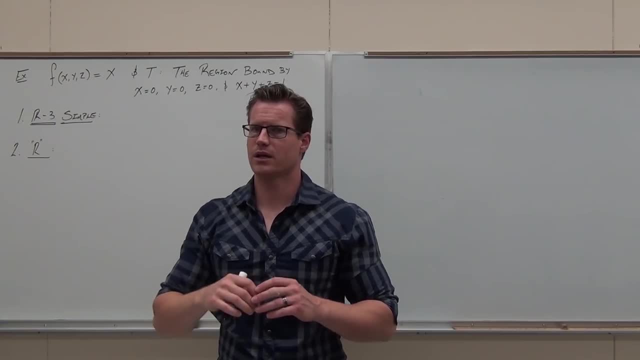 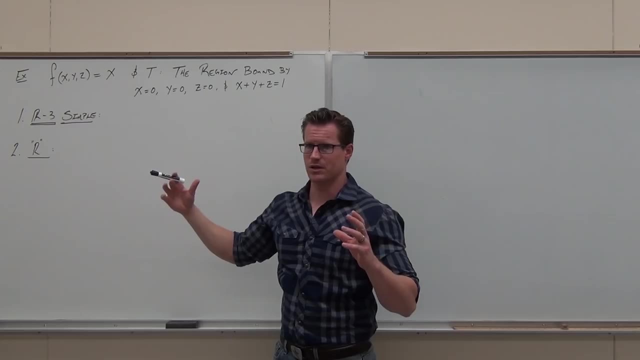 My advice to you is: pick z simple. if you can Try to go across the z first. In this case, I want you to look at something. I got x and y and z, all equal to zero. That's not telling me anything. 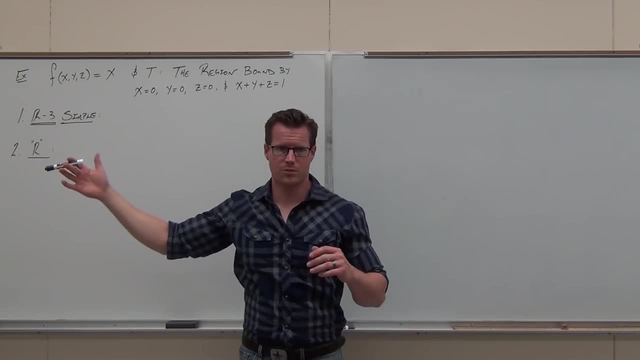 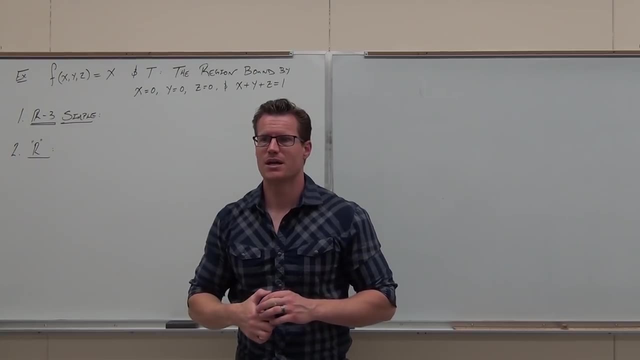 I got this: x plus y plus z equals 1.. These are all four planes, But I can solve any of these for x or y or z and have a pretty easy time doing it. Does that make sense? If that's the case, if it doesn't matter, pick z simple. 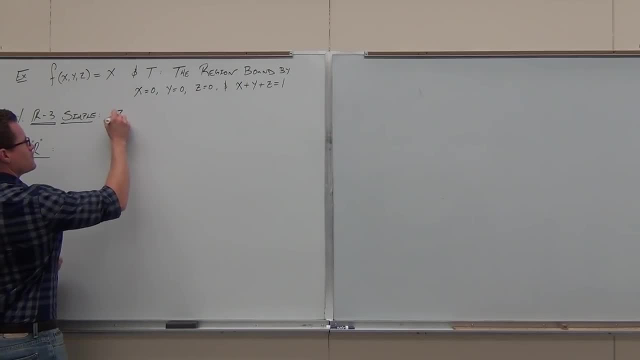 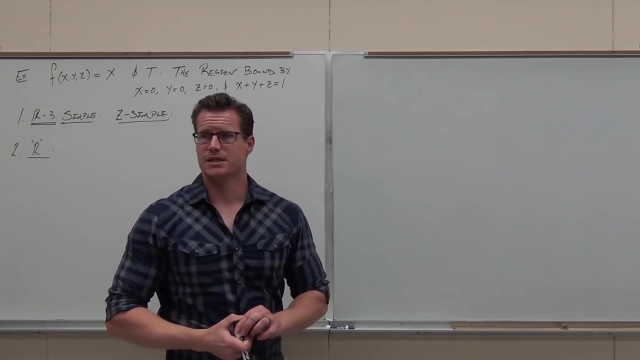 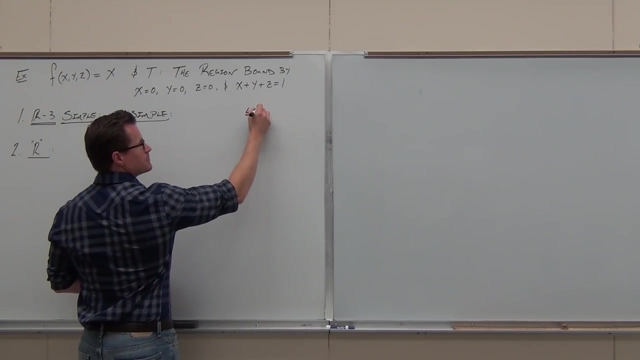 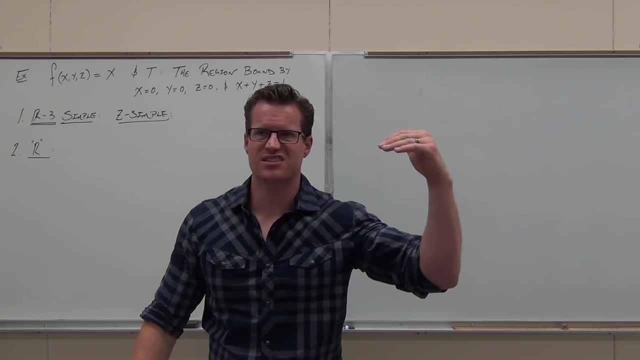 Try that. So we're going to do z simple. If you pick z simple, what has to happen is we're going to have z, We're going to have z between two functions. So I want you to take all the stuff that says z in it. 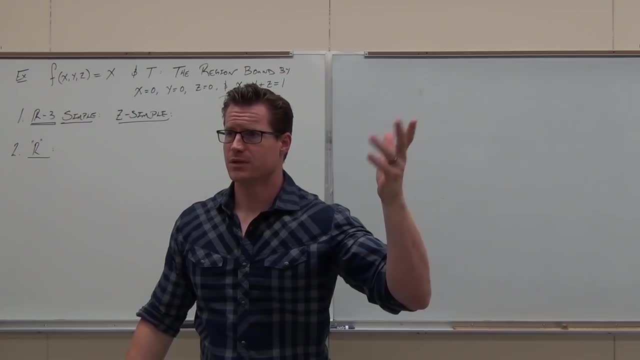 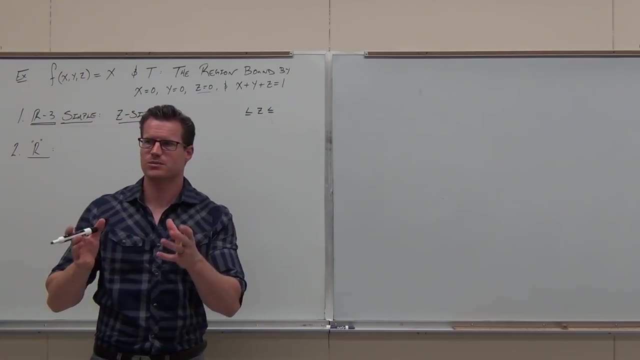 if you're choosing z, simple and solve it for z. So, for instance, I've already got 1 right here. I got z equals zero. That's pretty fantastic, That hopefully you understand. that's going to be our lower bound for z. 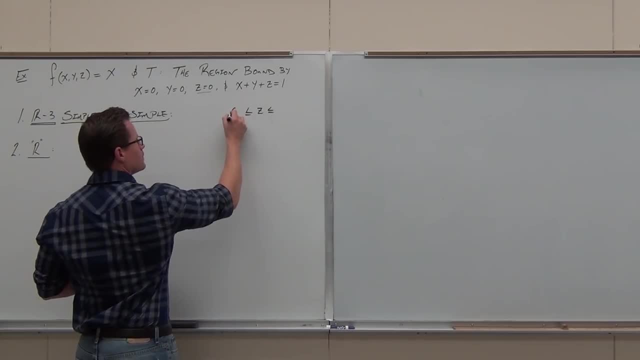 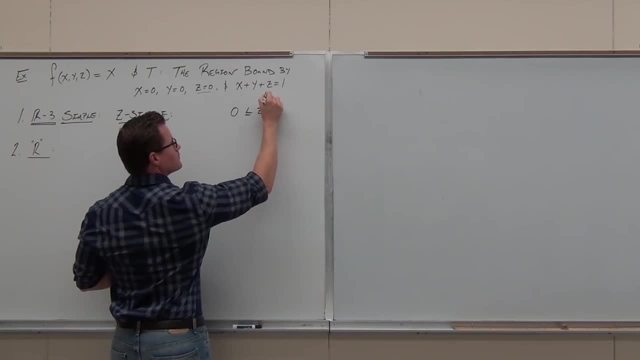 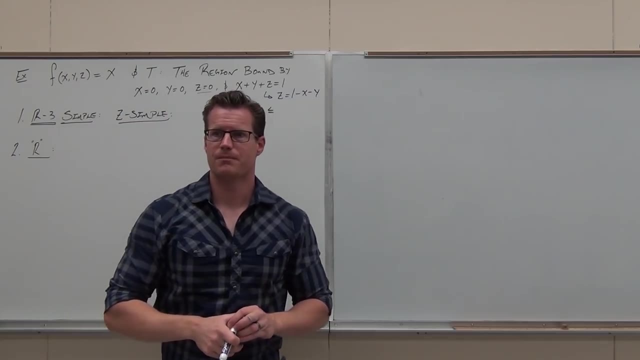 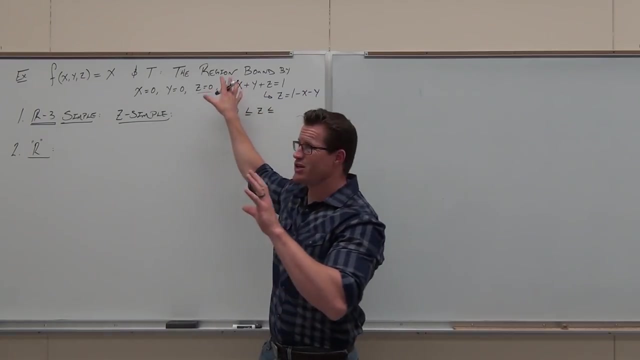 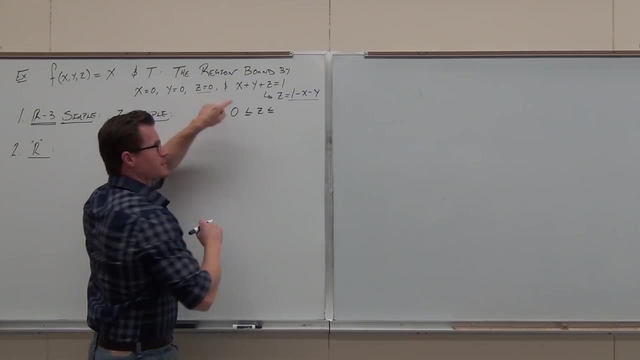 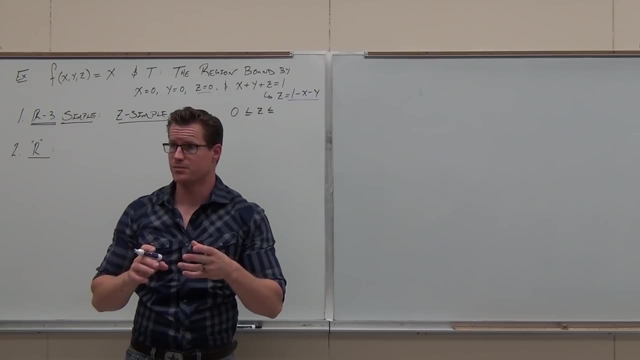 Z equals zero is the first one, and z equals 1 minus x minus y is the second one, And it's between those two functions. Hey, Don, are you okay with that? Are you sure That's the biggest idea that I can get you to understand? 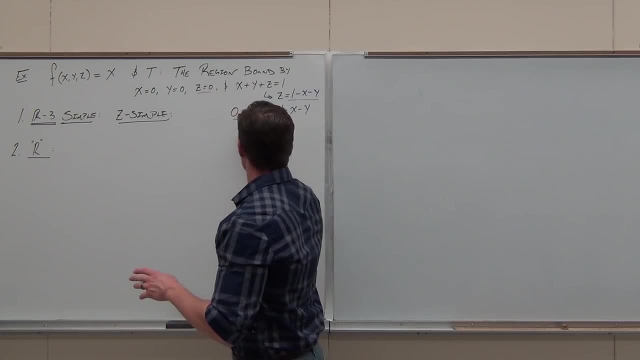 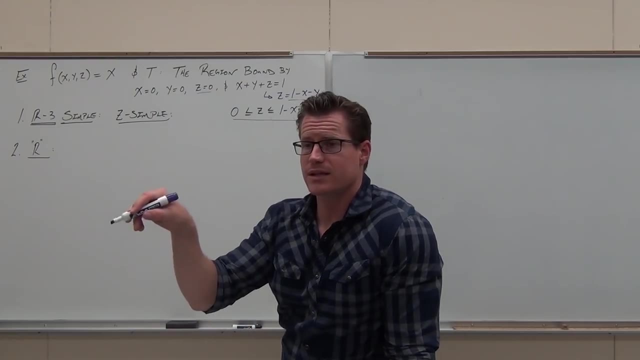 So we're going to hang onto that in the back of our head. We're going to keep this. That's a big deal. Now here's what this also means. If we chose z, simple, that's going to let us take care. 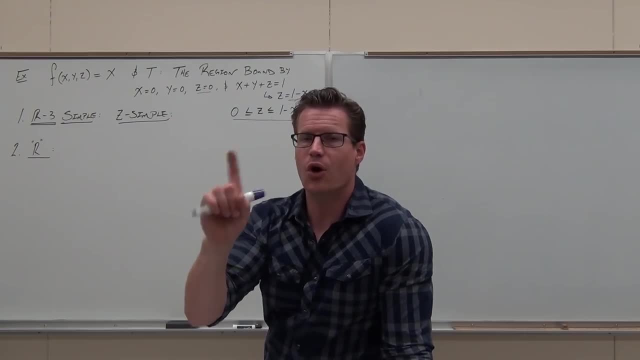 of the first integral. Our first integral is basically done. I know what it's going to go across. first I'm going to have what dxd1.. dxd2.. dy, dz, What's first? dz is first because I'm doing z simple first. 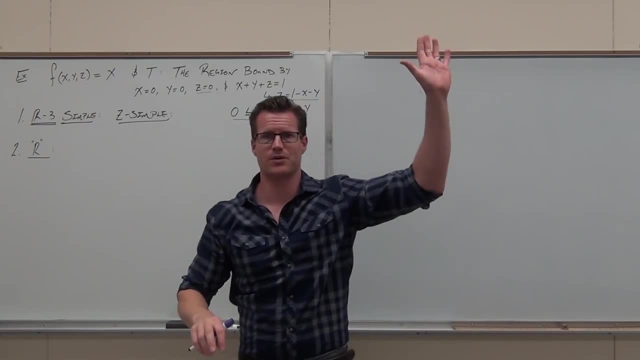 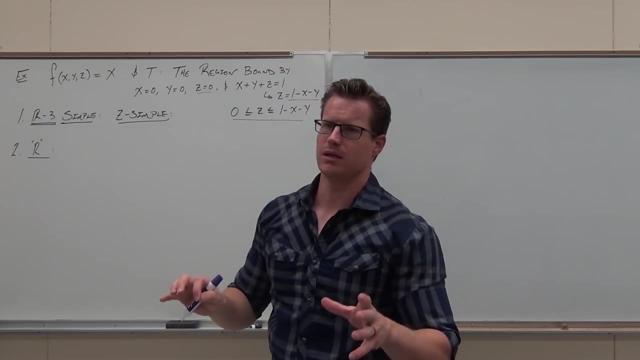 and it's between two functions, z equals and z equals, So I'm going to have to be okay with that one. I also know something else: If I did z simple, my r is going to be on what coordinate plane? Perfect. 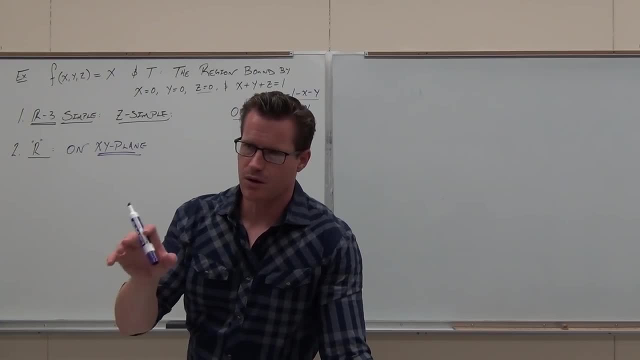 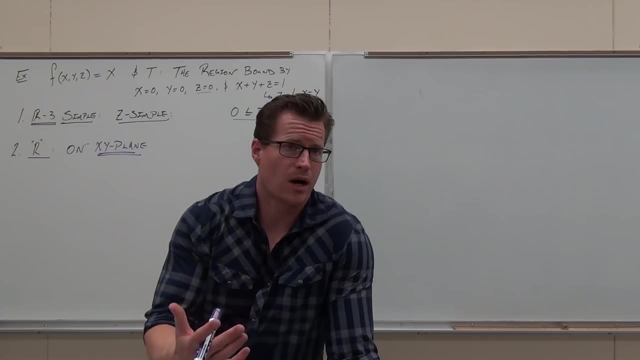 So this is- This is always our first step: Do the r3 simple first and then draw your region, Because you're going to get a r, a region, on some coordinate plane. Hopefully it's xy, but it doesn't have to be. 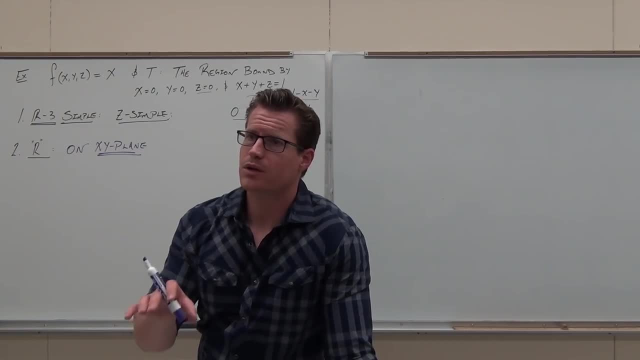 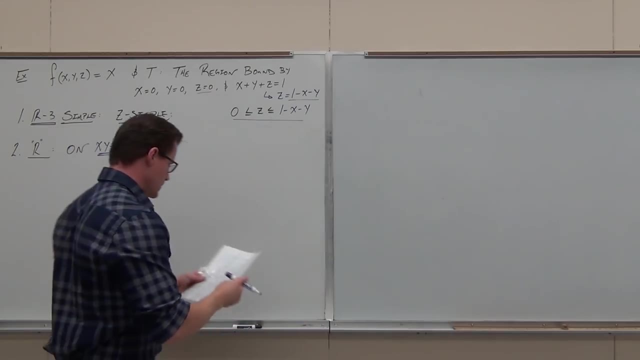 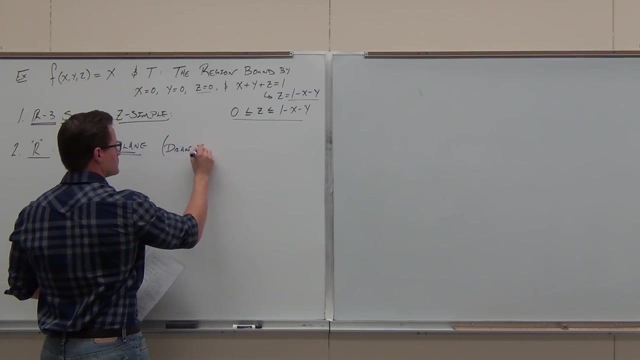 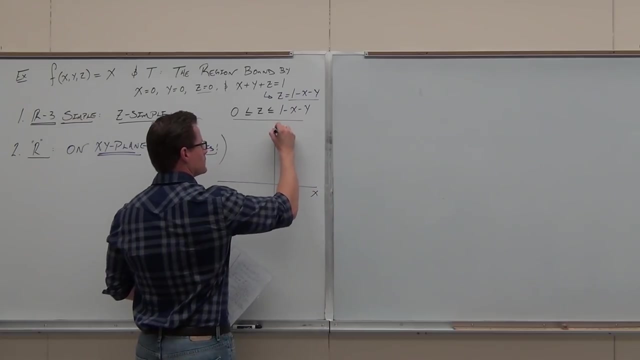 It could be xz, yz, one of those coordinate planes Now we're going to take, and all this information is going to get put on the xy plane. Let's draw this. Okay, make sure you label it too, because it's not always xy. 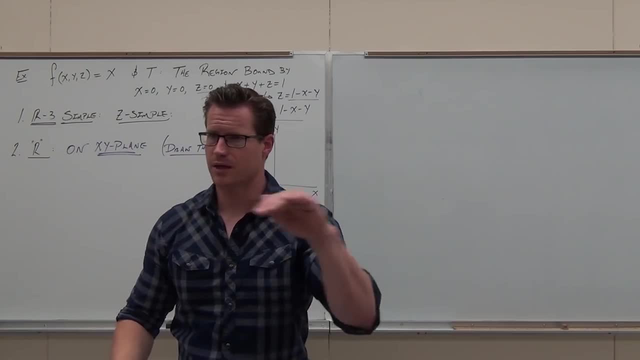 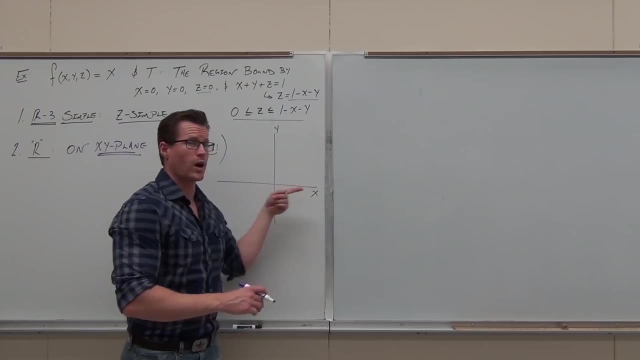 If you chose y, simple it would be xz. You've got to label this stuff. We have x, always the horizontal for us, if we can, and then z If it's not x. if you had like the yz, you'd put y horizontal. 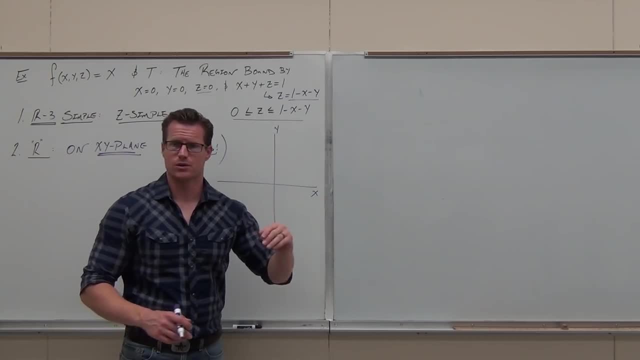 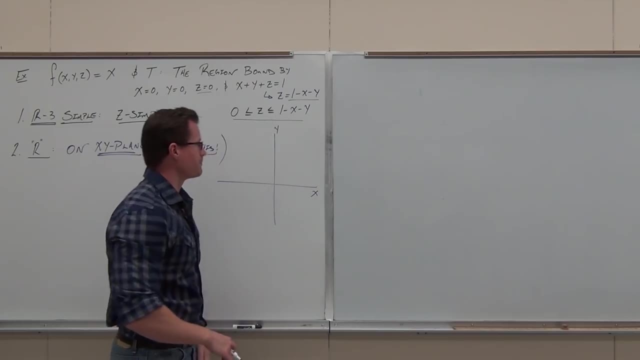 Z is always our vertical one. okay, It's never our horizontal. So x horizontal, y, horizontal z is always the vertical. Make sense xy. Now we're kind of looking down at it, So let's graph them. Hey, can you graph? x equals 0 on the xy plane. 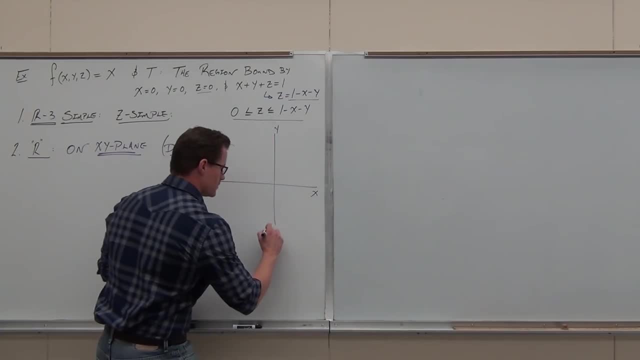 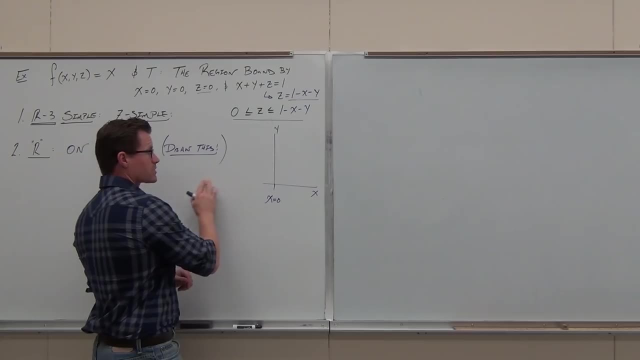 What type of line does it give us Y, That's it. It's right here. I don't even need that much, So we got that one. We also have y equals 0.. Now what's z equals 0?? 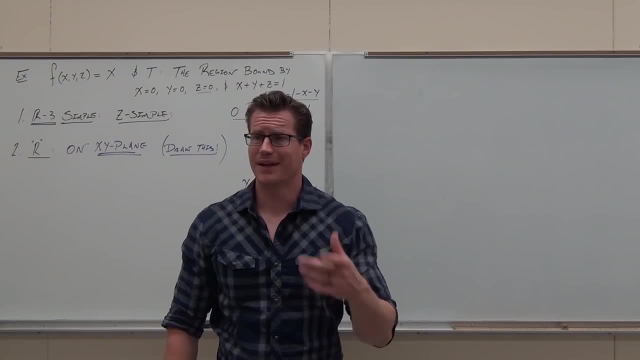 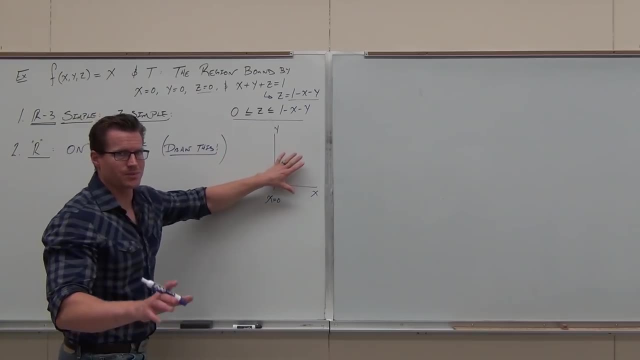 Is that somewhere on the xy plane? It is, That is the xy plane, So that's the same. We're on the xy plane. Okay, that makes sense. Now, on the xy plane, notice something. Notice, if we're on the xy plane, z is in fact equal to 0.. 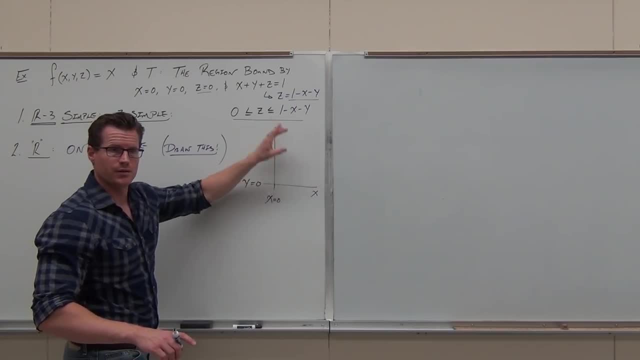 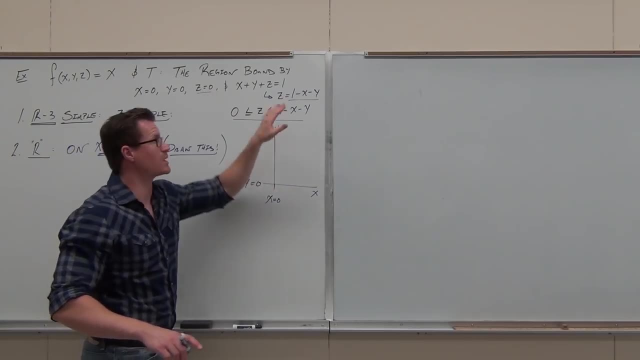 Does that make sense? That means that any function that has z's in it, replace the z with 0, and you'll be on that plane. That will give you the intersection of whatever this is with that plane. So it makes me look good with that concept. 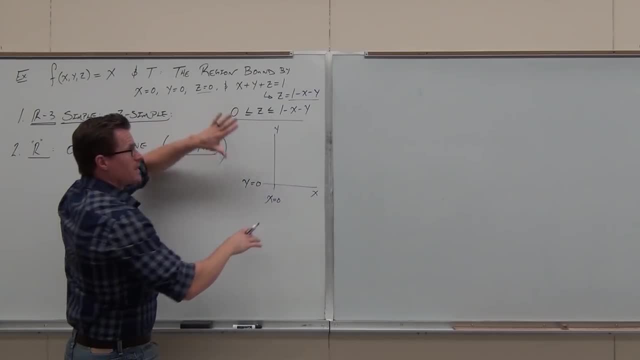 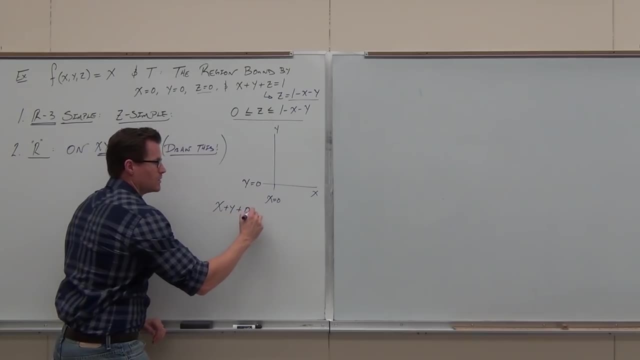 So x equals 0, great, Y equals 0, great If we're on the xy plane. z is also equal to 0.. Okay, That means that we get x plus y plus 0 equals 1.. That's stemming from the x plus y plus z equals 1.. 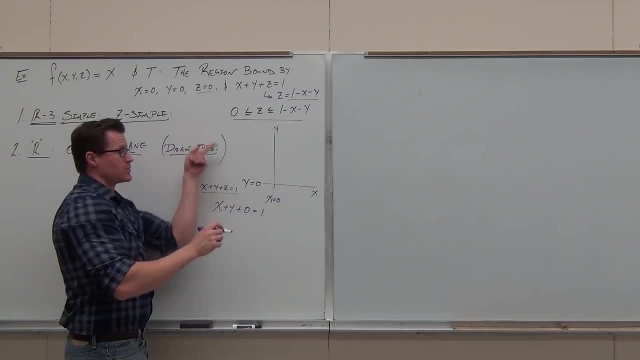 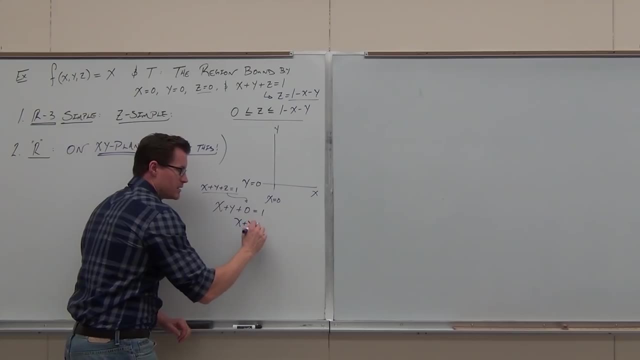 But if we're on the xy plane, then z equals 0.. If we're on the xy plane, z equals 0, and we get x plus y equals 1.. Hey, everyone in class right now, what is? x plus y equals 1?. 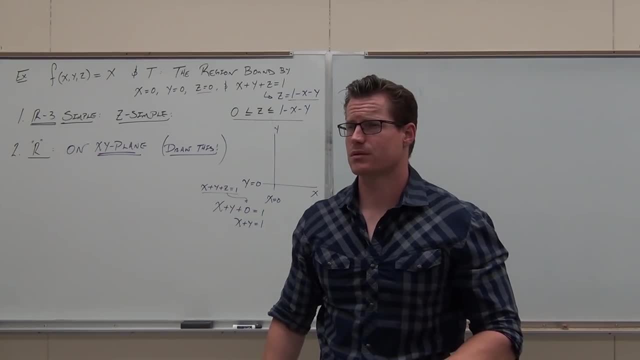 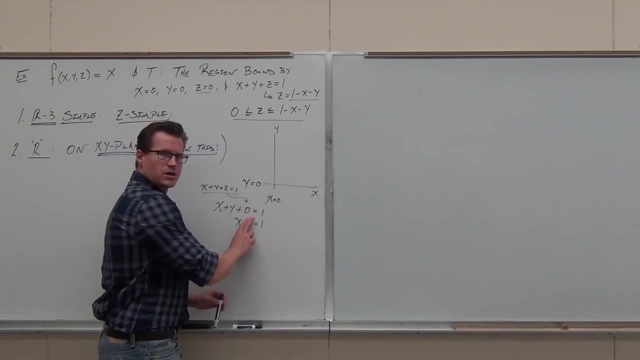 What's it? give you A line. What's my two intercepts? Have you ever seen this before? Cover it up. If I cover up the y- x equals 1.. Cover up the x- y equals 1.. Those are my two intercepts. 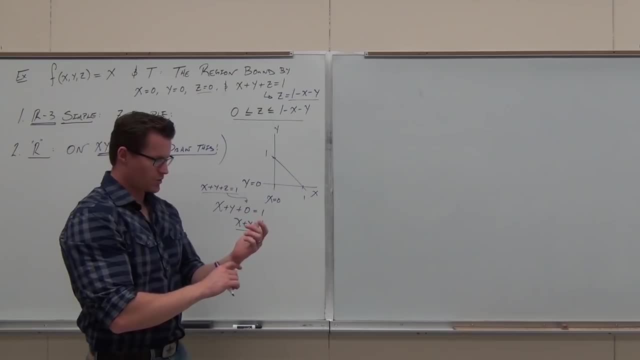 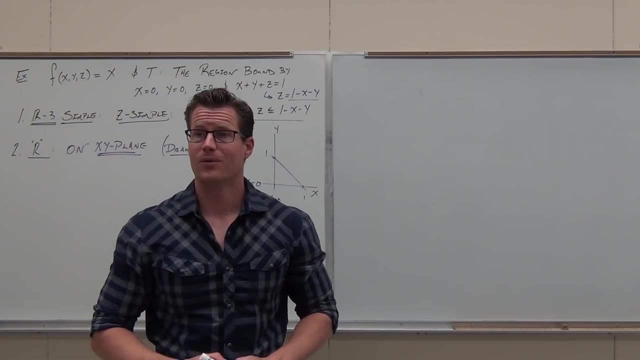 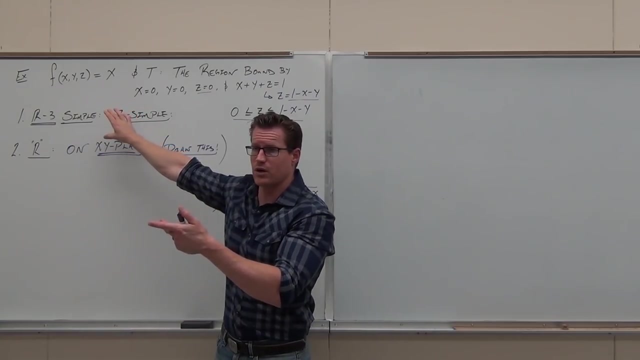 So that's the line x plus y equals 1.. Now, this was the whole point. If you have picked R3, simple X, y, z, whatever, you're going to be left with a 2D region, It's good. 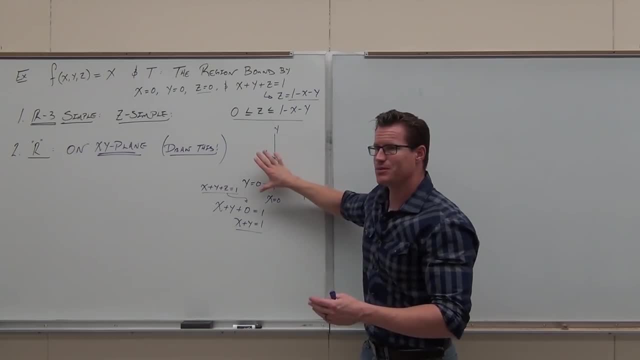 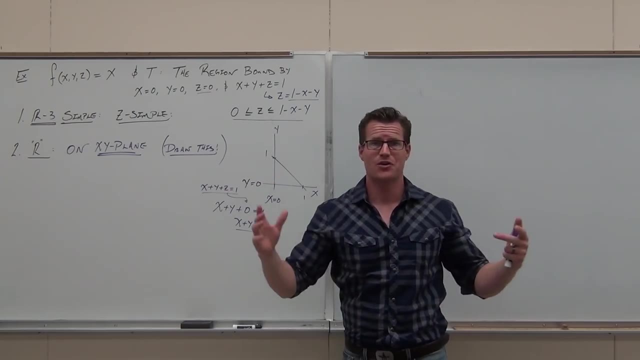 Listen. if it's on a coordinate plane it's got to be 2D. That's now a 2D region. Does it look familiar? Can you identify that region as a double integral? Because if you can, you're practically done. 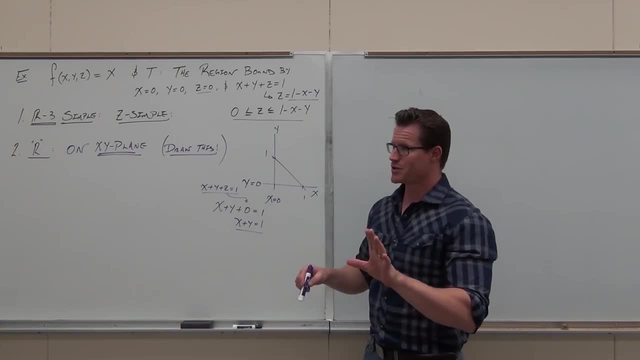 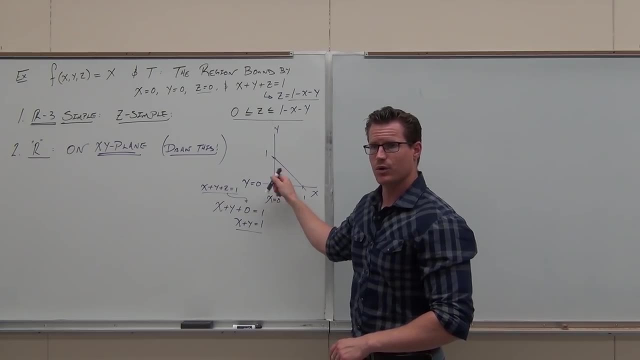 If you're with me Now, you've got a choice. You can, for your double integral, think back to double integral days. You can choose to go along the y first dy or along the x first dx. Which do you want to choose? 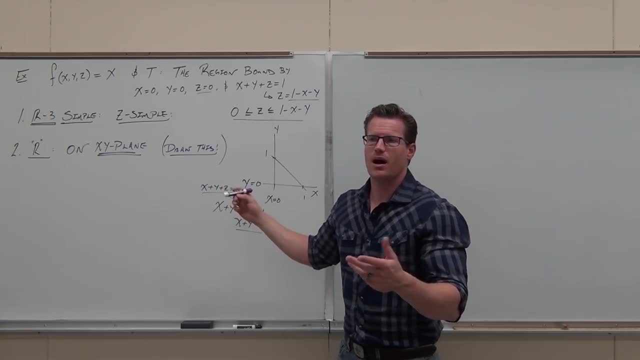 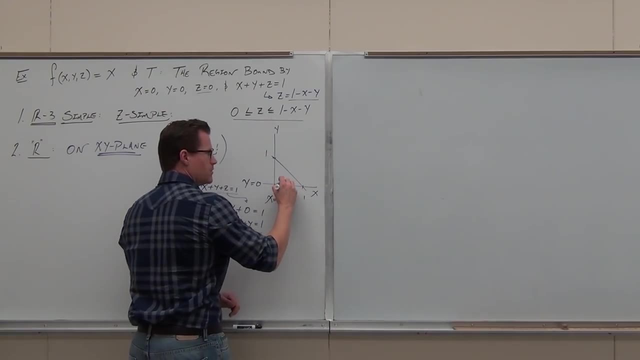 It doesn't matter, As long as you say it, As long as you set it up, I don't care. It doesn't matter. I like going along the y first, because I like y equals functions. Does that make sense? So I'm going to choose to go along this first. 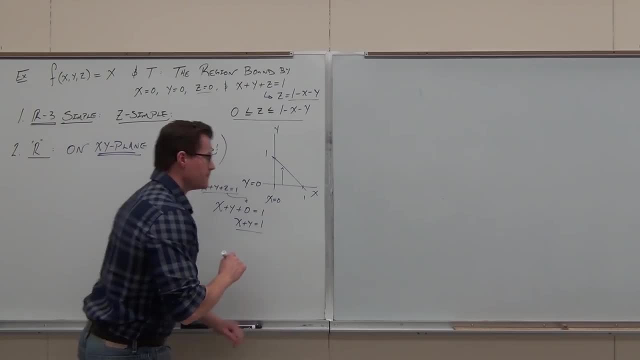 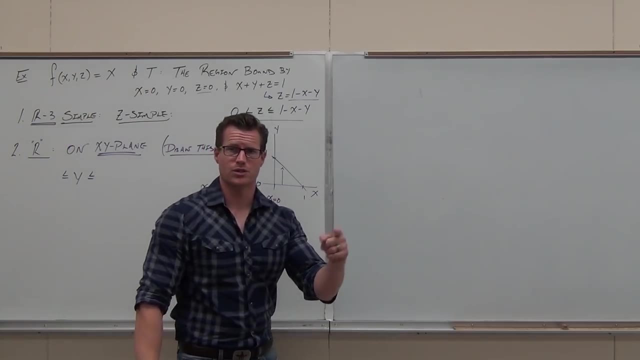 If I choose to go along this, first I need y. So for my R I need y to be between two functions of y equals The first one. The first one. The first one is y equals 0.. I'm between one function: y equals 0.. 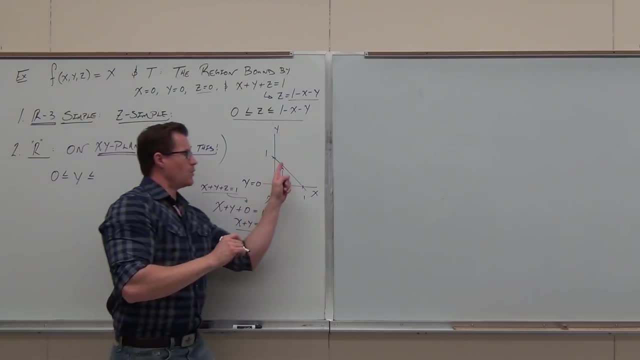 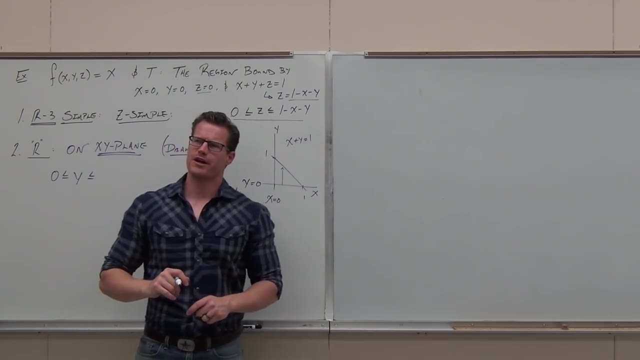 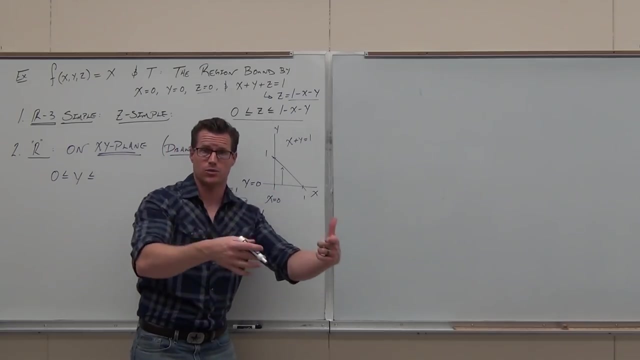 Do you guys see that? The second one: Well, if this line is x plus y equals 1, what variable would you want to solve? for if I'm going along the dy, the y axis first, I want dy- y equals. 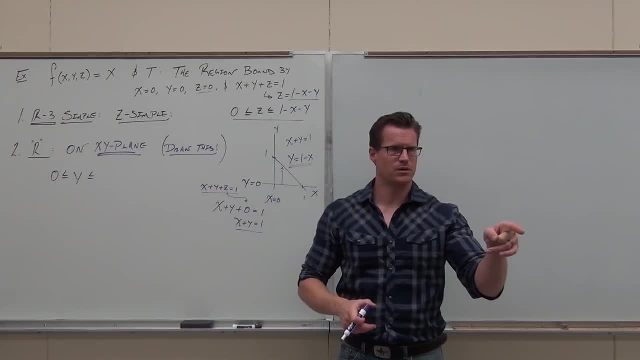 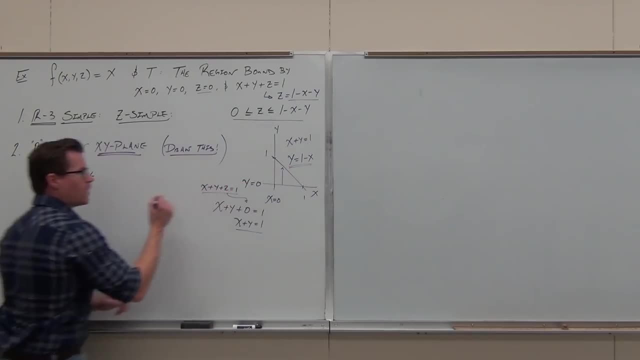 I don't know if you're okay with that. You guys over here, yes or no? So if I go along the dy, the y axis, I'm going from y equals 0 to y equals 1.. 1 minus x. 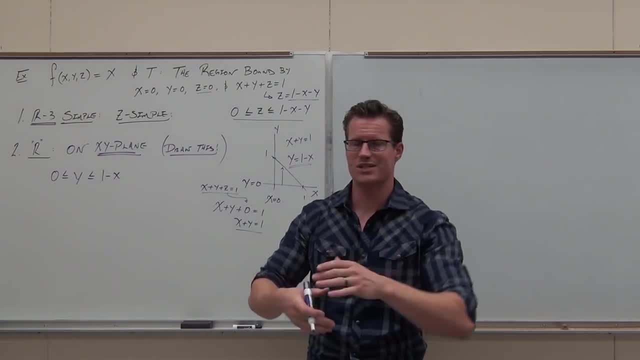 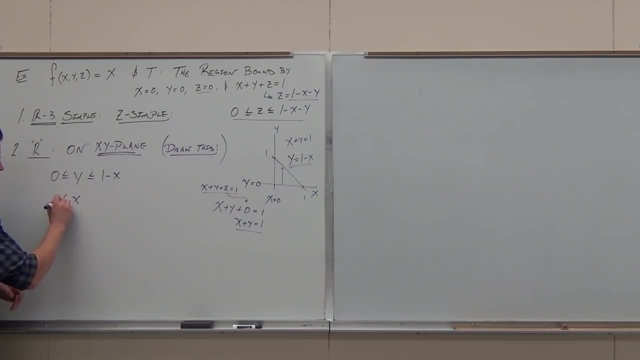 You can even see it. You can see what's the larger and what's the smaller function by drawing the region. That's why we practice so much of that. Now the last one. I also need my final variable. Hey, how about this? 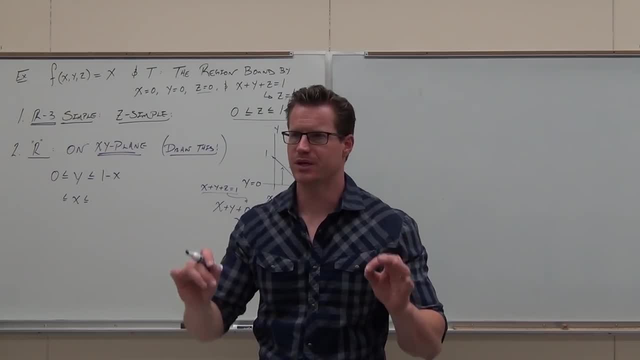 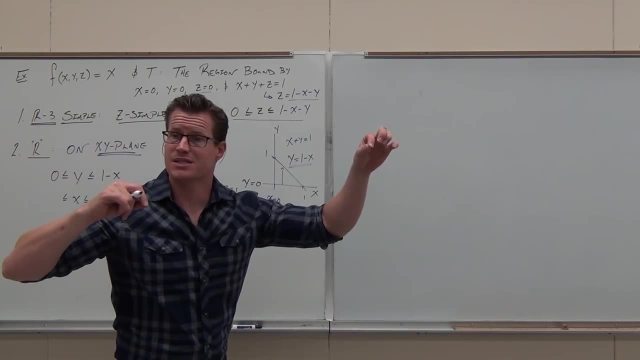 What does the final variable always have to be between Constants? Has to. So make sure that happens. First one between functions R3.. Second one between functions in R2.. Last one between functions in R1.. That's numbers, That's just numbers. 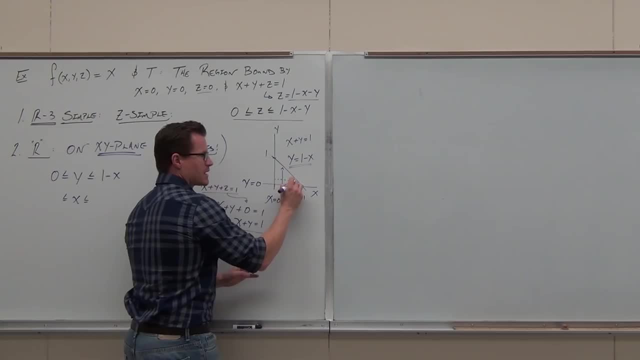 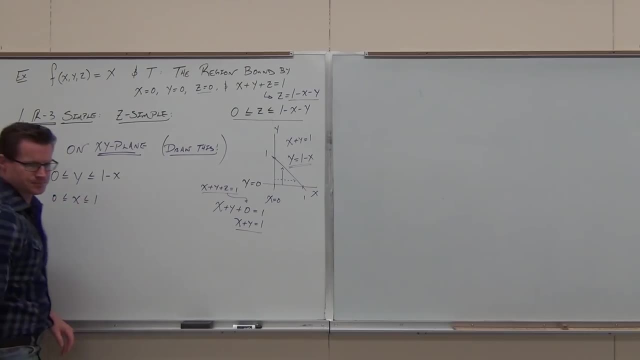 So we went along: the y first, dy, The x comes second. Go between the largest constants that bind that region. What are they? 0 and 1.. Perfect, That's perfect. Ladies and gentlemen, this is the biggest idea. 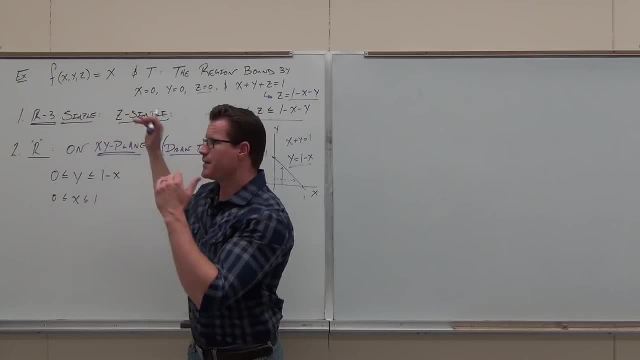 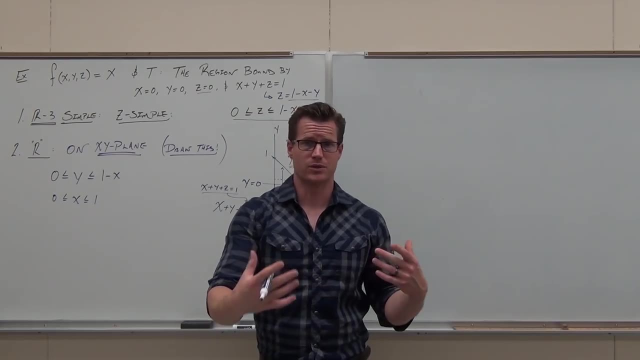 The biggest idea is getting the R3 symbol first and then drawing the region. Why? Because then you have a double integral after that. Have I explained this? I really need to explain this well enough. If not, I can do it again. 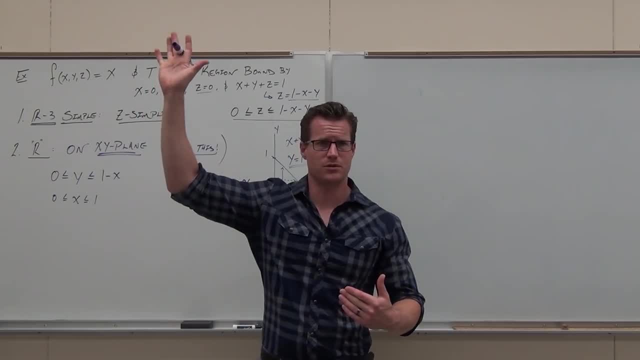 But I want to. I want to make sure that I've explained it well enough for you guys to understand this setup. Show of hands, if I have, You actually get it. That was like half of us Guys over here in the back left. are you sure that you're okay with it? 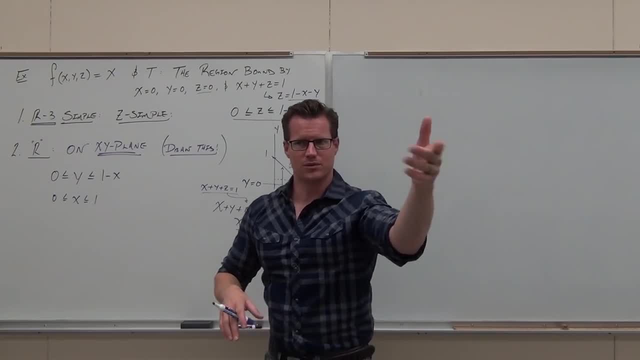 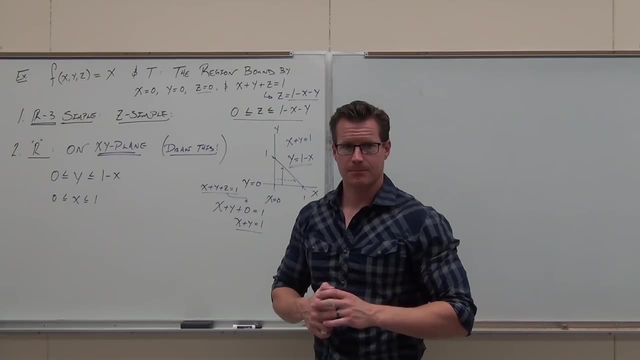 I don't want to leave you hanging. Are you all right or not? You sure So the yes. So if you had like z equals 1, you would not cancel out the z in that first x plus y plus z equation. you would fill in with a 1 and then solve. 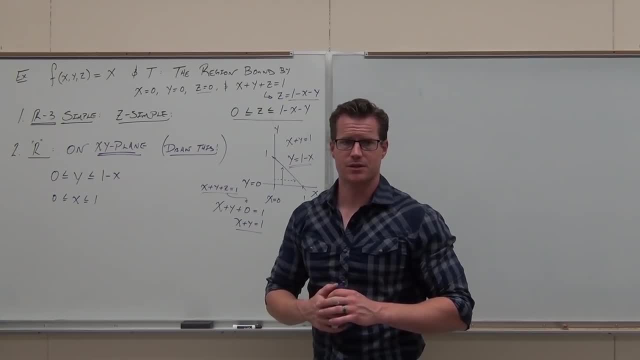 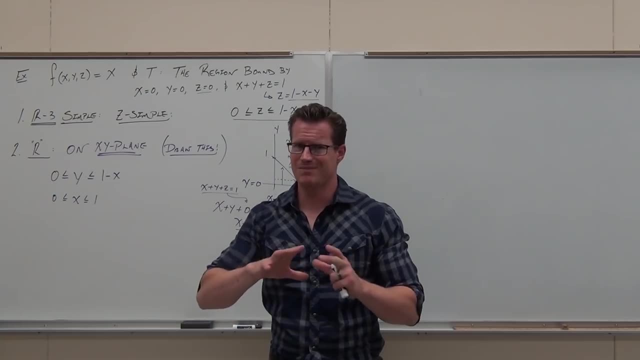 Correct, You'd have to find the level curve of those z functions. Okay, If you did that I might have. if it was z equals 1, I might have chosen to go y-simple or something. Right, You can always. you can always make it different if it's not suiting you. 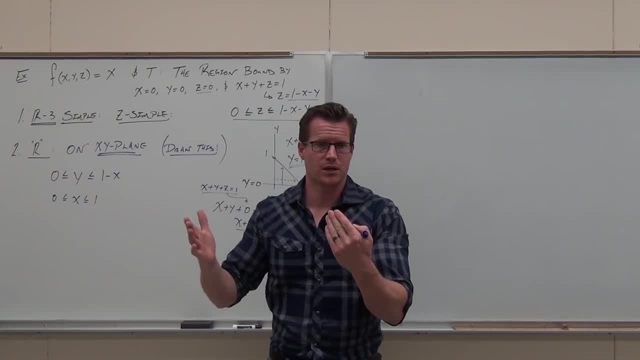 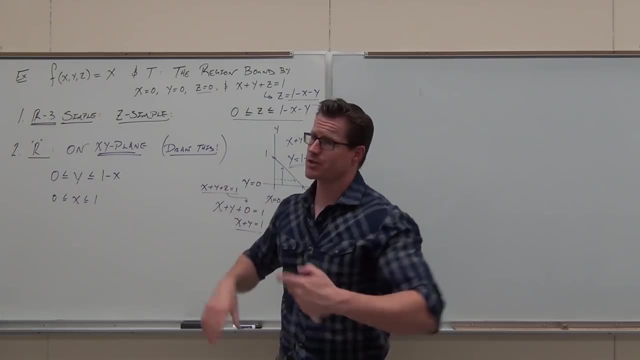 You can always change it. They're in six different orderings. if you want, So choose the r3-simple. that's the easiest to deal with. Since these were all the same. I chose z-simple because I wanted r on the xy-plane. 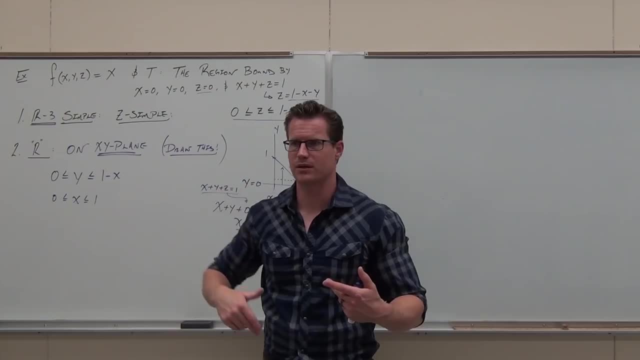 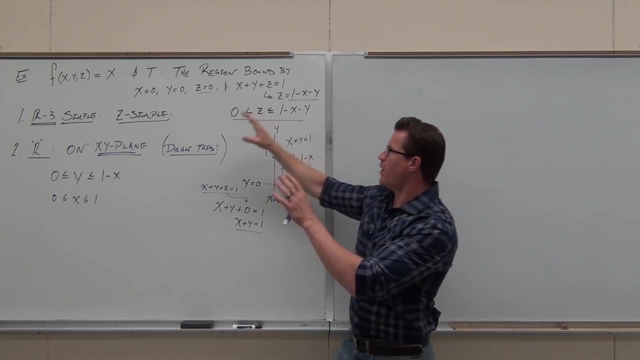 Because that's, that's nice. We're, we're used to that, We're used to drawing xy-plane. Make sense, So z-simple. yeah, I needed to go between 0 and solve for z. Got it. R's got to be on the xy-plane. 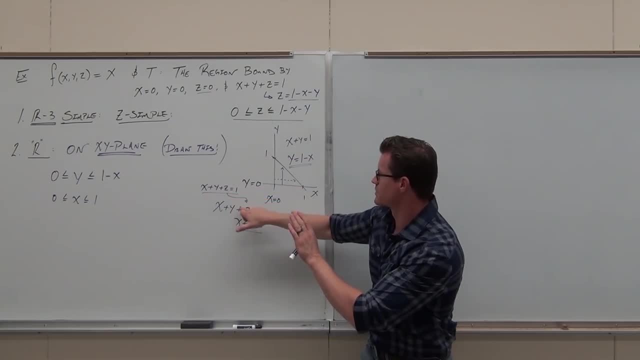 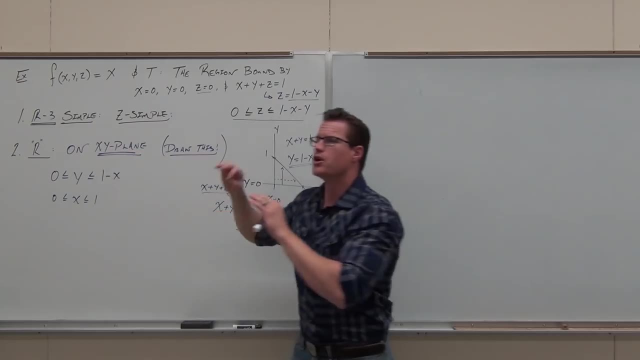 xy-plane has z equals 0.. Okay, So xy-plane has z equals 0.. Draw the line, draw the line. draw the line. everything that's on the coordinate plane that this is referencing, that this refers to for r, draw them all. 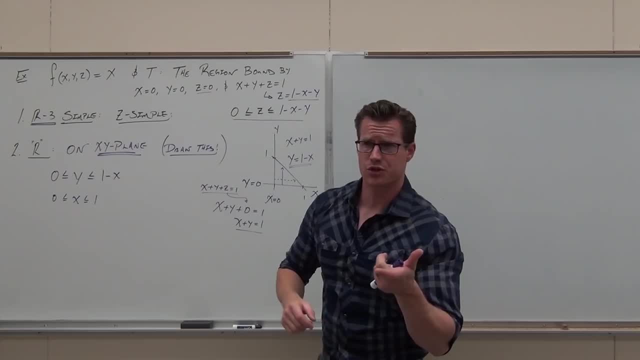 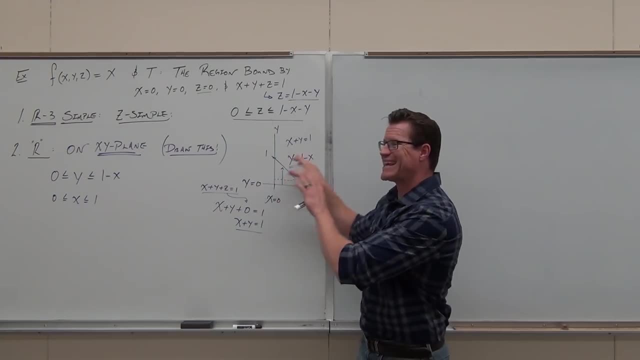 It's going to create a region for you. You get to choose how you want to define that region. Go between two functions of y or between two functions of x. I went between two functions of y first, 0 and y equals. That's what that's giving us. 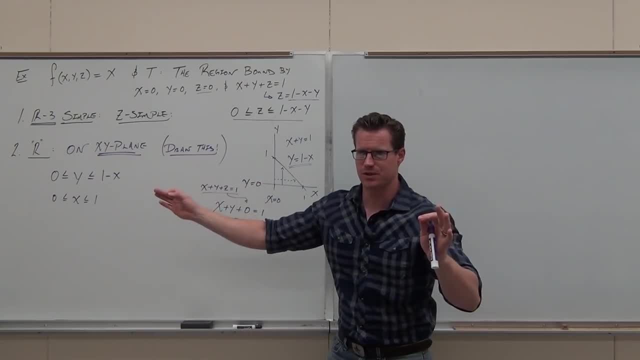 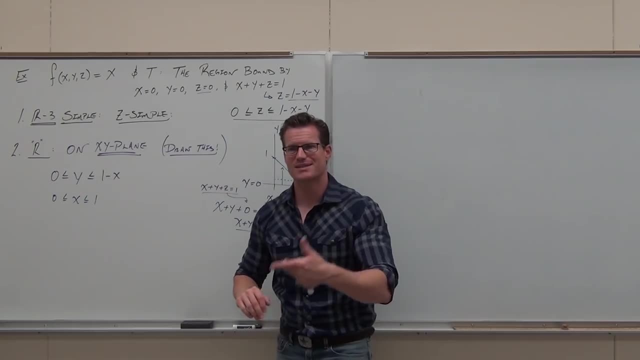 Then we go between constants On the. the only axis you have left should be constants x equals 0 to x equals 1.. For real, you guys? okay with it? Now, this will always set up your triple integral. Here's how triple integrals always work. 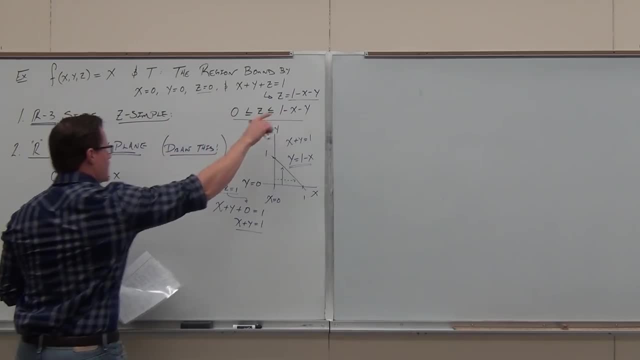 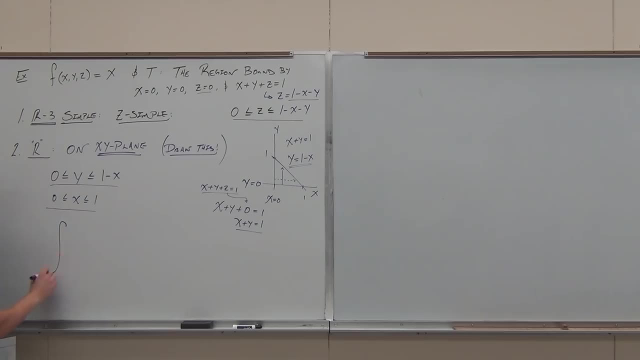 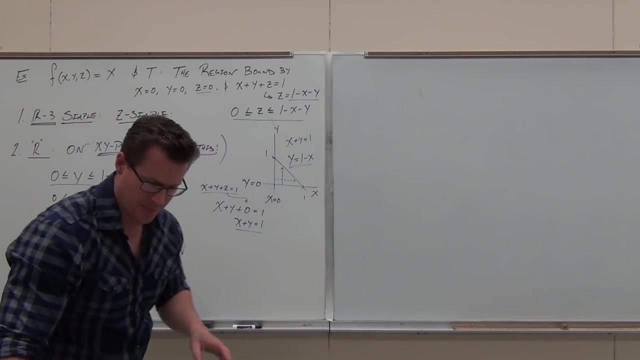 Okay, Here's how you set them up: After you find the z-simple and you find the next 2d-simple and you find the 1d-constants, triple integrals work this way. We put our function in the middle, We have dv. it's going to be dx, dy, dz or any any permutation of that. 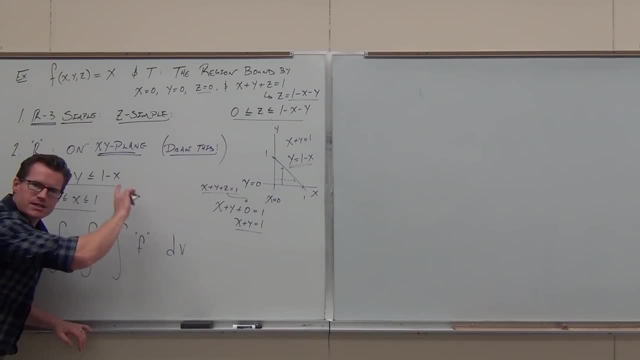 Here's what you do: Whatever you found for the r3-simple goes here. We call that maybe t-simple as well, r3-simple or t-simple. Then we do the 2d or the r2-simple That would be for our, our region, so r-simple. and then here is always constants. 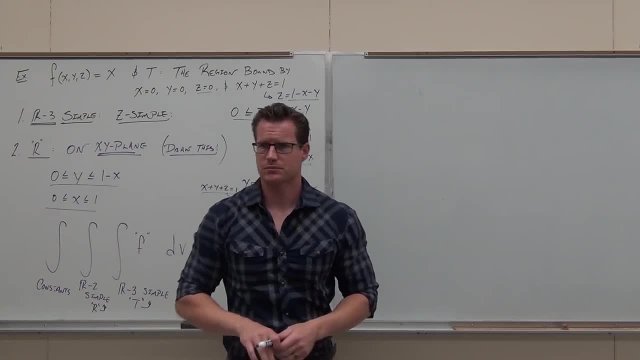 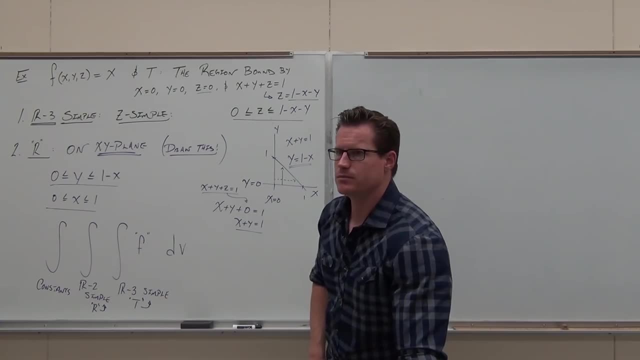 If you're not having your constants on your most outside integral, you're going to do something wrong. That's got to be there Now let's put it together. Do you guys think that you guys, you could put it together if I asked you to do it? 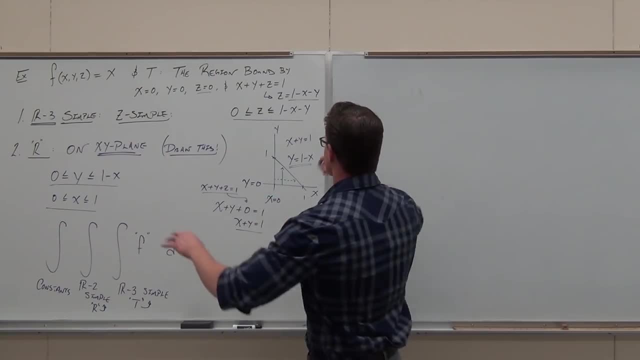 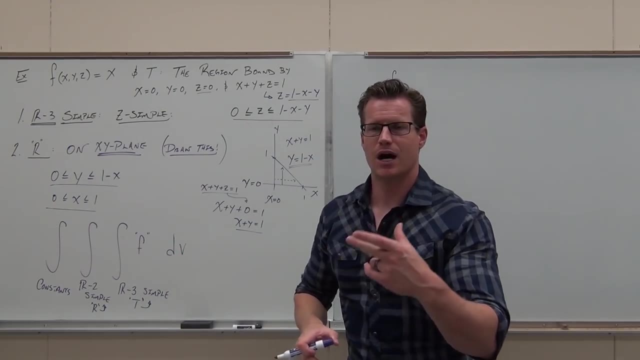 Yeah, Let's start with the inside. We always work inside out with these. So if I'm going to set this up, I want an integral, that's, the r3-simple, first. Hey, what axis did we go along for? the r3-simple, x, y or z? 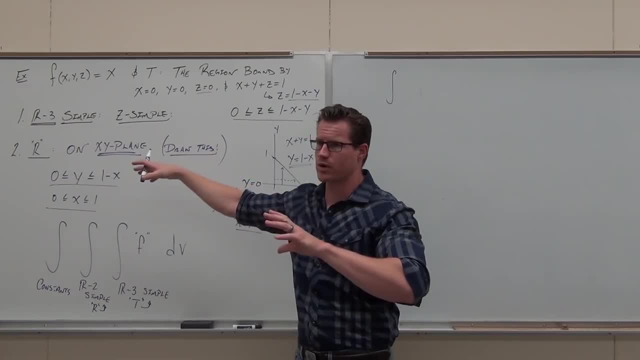 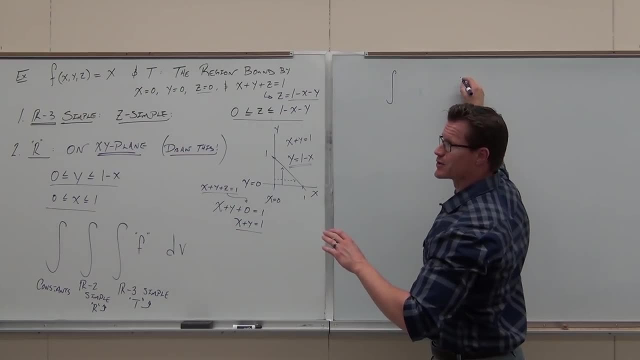 Z. That's why we write this stuff down. Write down everything I've written. Keep your work organized. It's too easy to get lost. So if I went along the z first z-simple, I should have d what first? 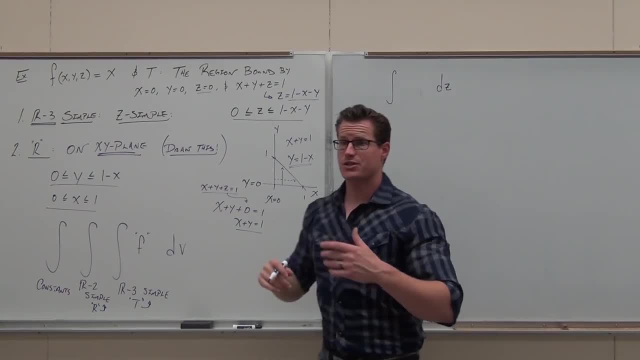 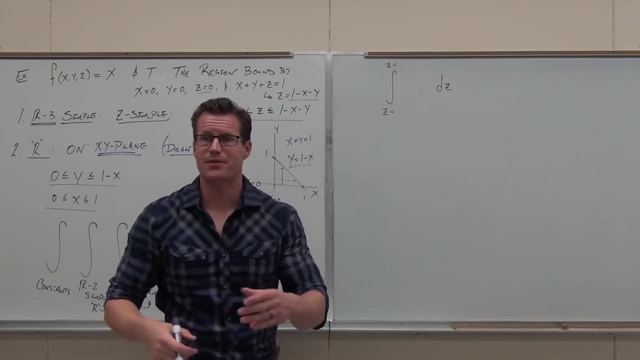 Z And then we're going to match that up. So if I went dz, I've got to have z equals something and z equals something. That's why I took that. I taught you that method to match up the dz with the z equals. 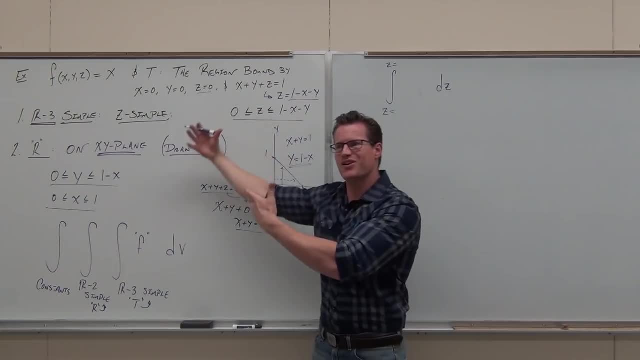 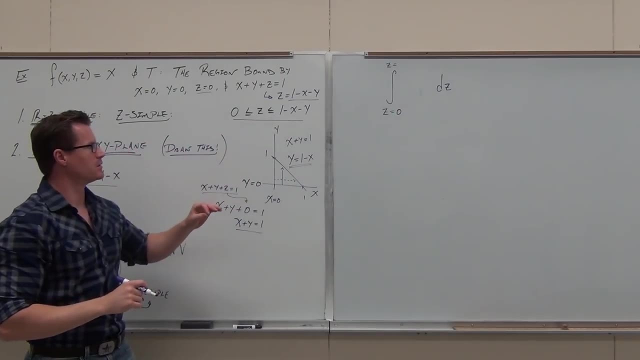 That's why we did z-simple and between two z equals functions. That's the whole plan here. What's the smallest z function that we're going between? What is it? Two? what One minus x minus? Yeah, if you write that, it makes it pretty clear. 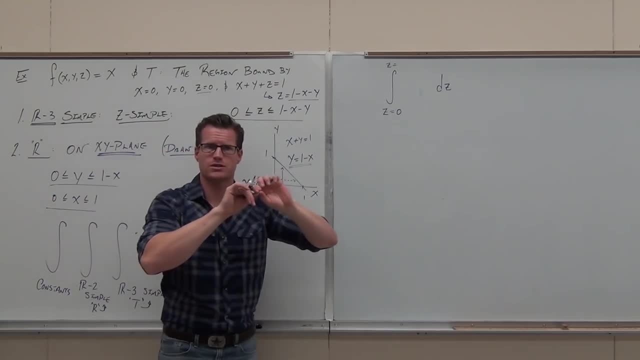 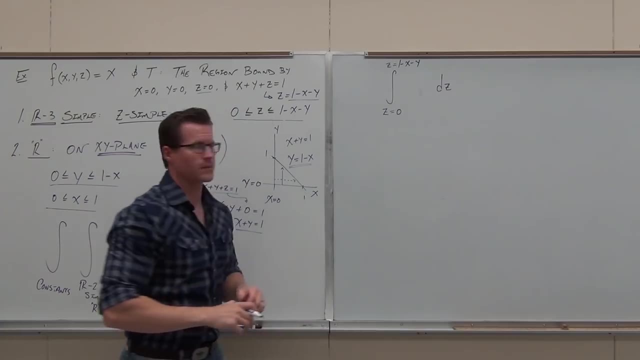 It says we're going between z equals zero and this- Those are two functions in r3- between z equals And now, if you're okay with that one, Now let's build this. Let's build our way out. I want left side, only, you guys. 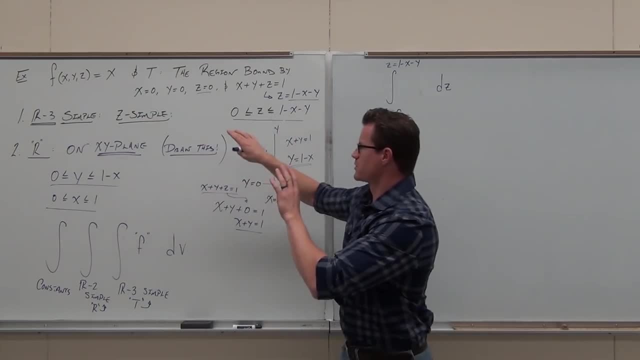 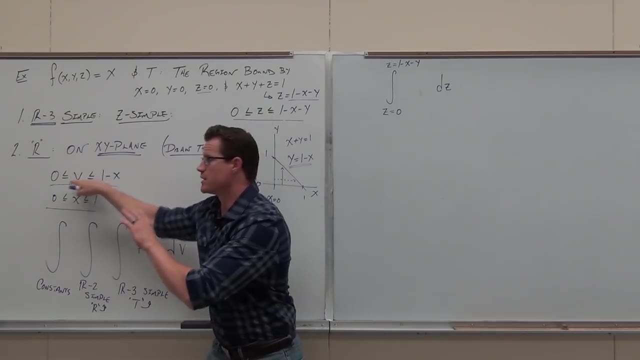 According to my region, I went z-simple first, cool. According to this, did I go x-simple or y-simple? What did I do? Y-simple because that's the one that's between two functions. The x would be the constants. 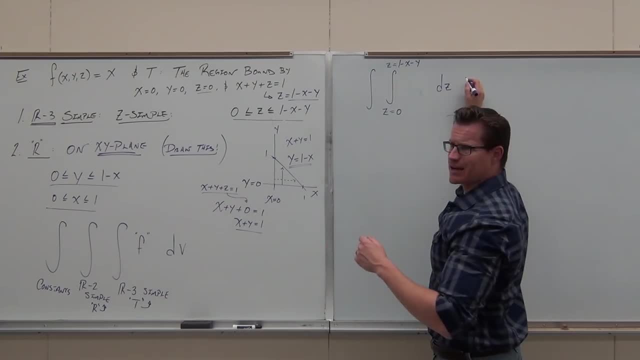 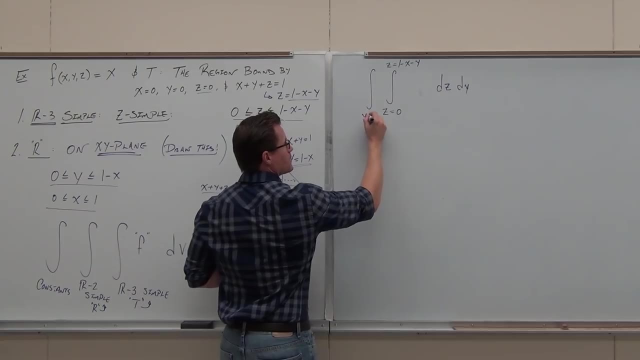 So the next integral I do would be dx or dy. Perfect, That means right-siders, you guys. I have to have y equals something and y equals something. What's going to go right here, please? So we write all this stuff down. 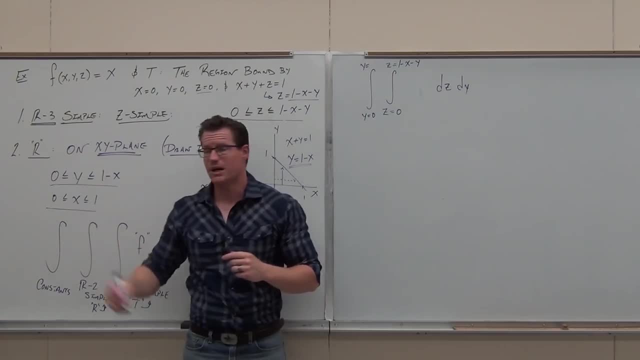 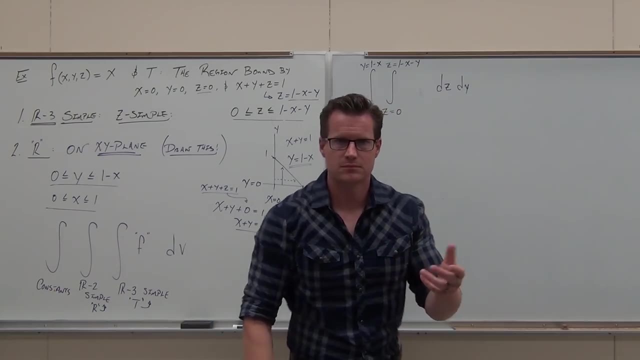 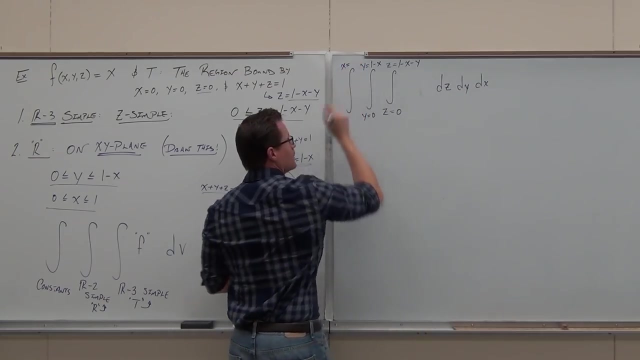 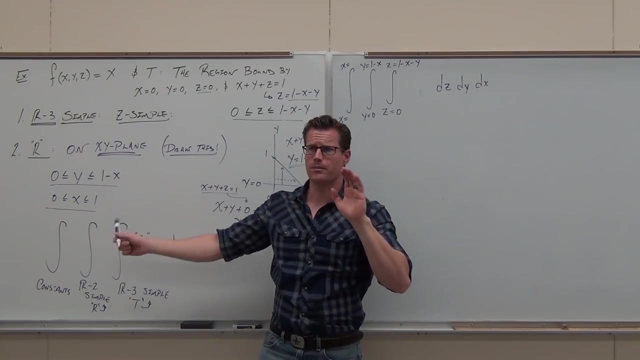 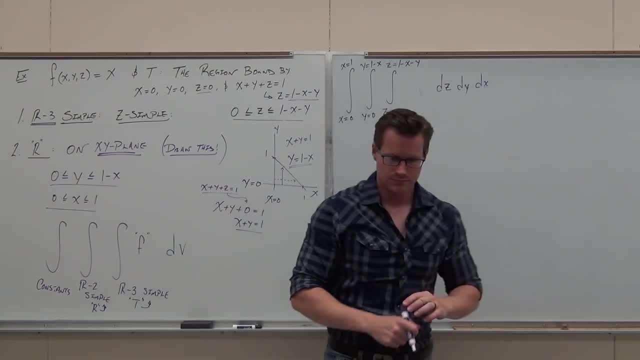 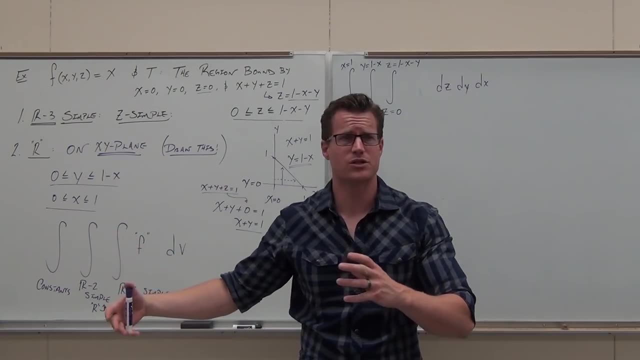 Zero, Zero, Zero, Zero, Zero, Zero Zero. That's almost it, Almost, But that's the hard part. The hard part is the setup. This is a really basic integral, but I want to make sure that you actually get it. 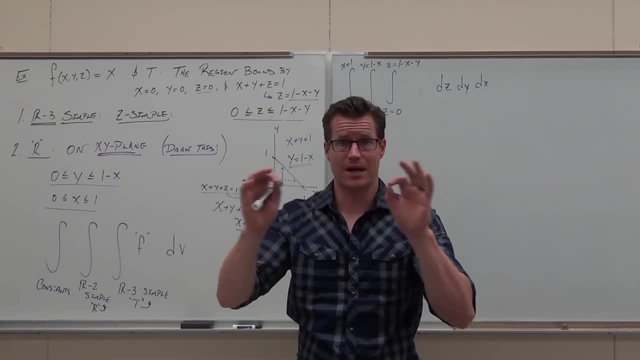 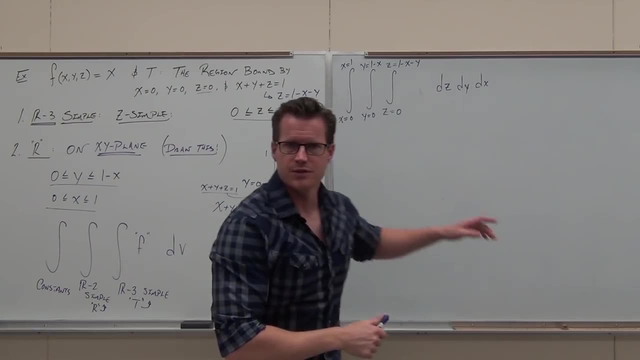 Do you understand? the z first, then the y, then the x, and that's why we have an order between the functions, that we have them in Show of hands. if you do Also, the stuff matches up. still, This variable still matches this variable. 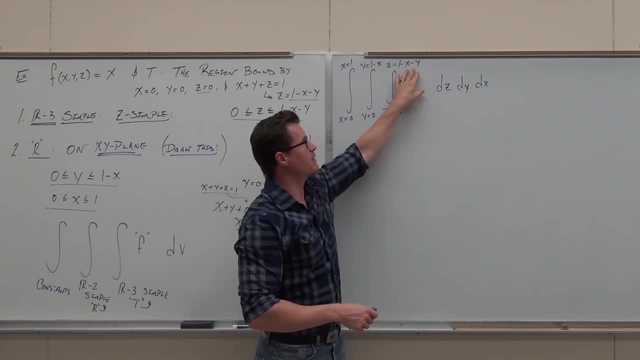 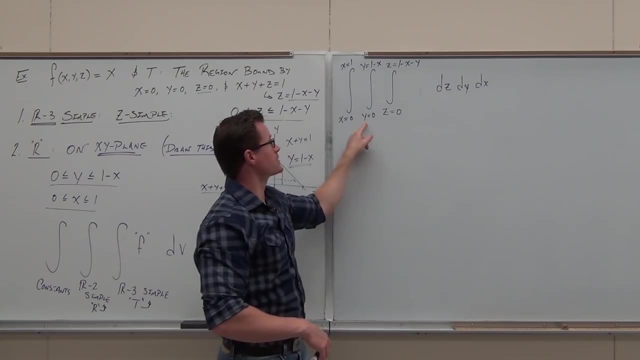 And look at this: The remaining variables will be these two remaining variables. They have to be, or else you're going to do it wrong. It won't work out for you. This variable matches up with the next one and the only remaining variables here have: 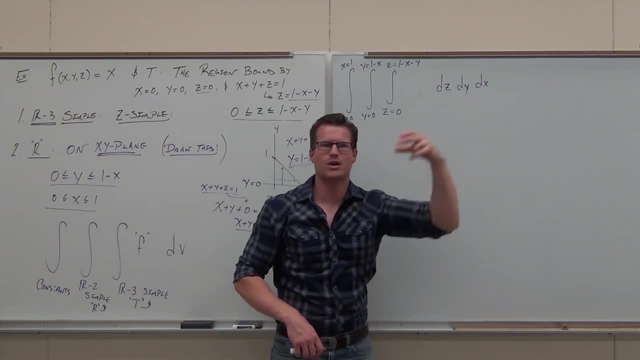 to be the final variable. Do you remember doing that? matching up what it's equal to to what's next, what it's equal to to what's next. That always has to work for us. We are missing one thing that's really common. 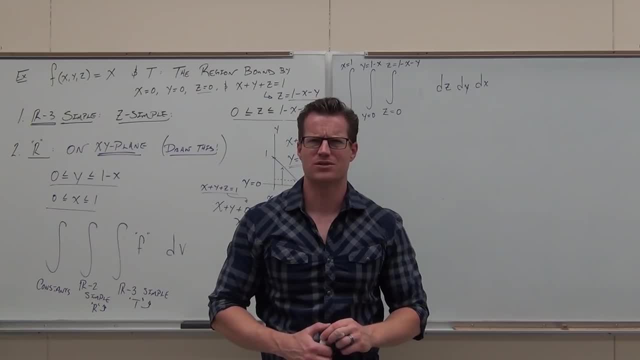 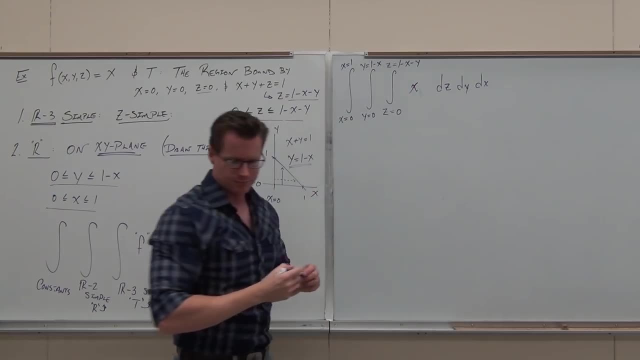 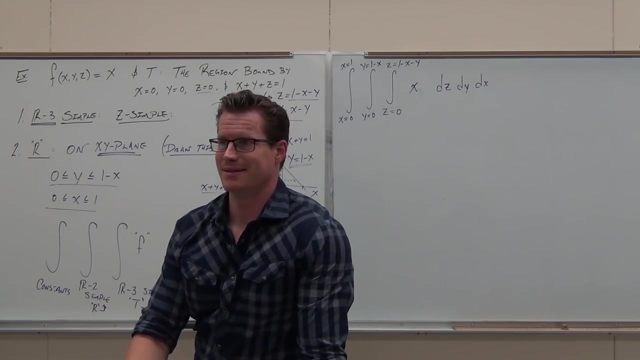 When we get going we get all caught up in the region. We miss out this one major thing. What is it? Tell you what I've got to be honest with you here. You are going to be distributing like crazy in this section. 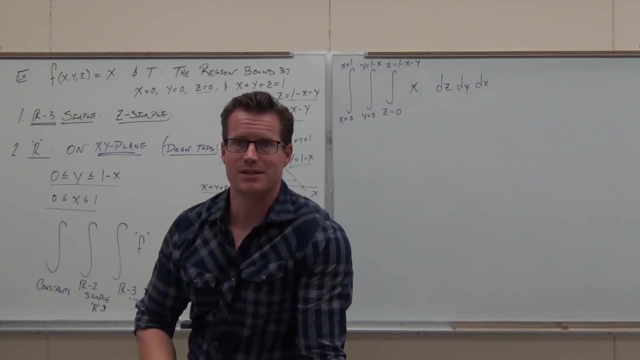 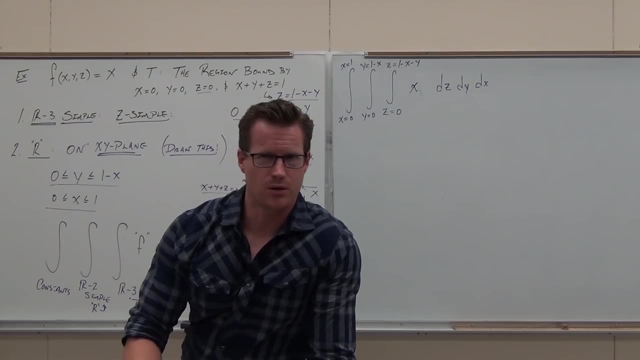 with some rectangular triple integrals. It's crazy because there's a lot of stuff that happens. I'm going to basically fly through this to give you the outline of it, but I want to know, if I give this to you right now, if you could start it. 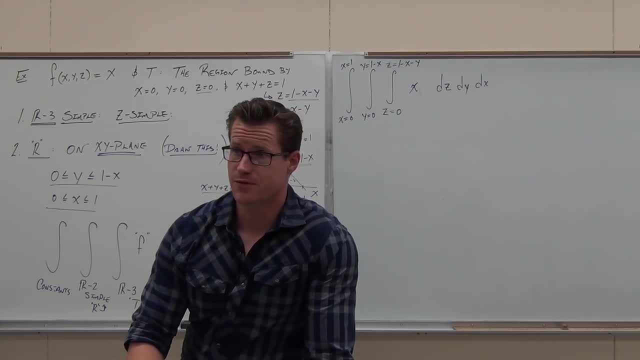 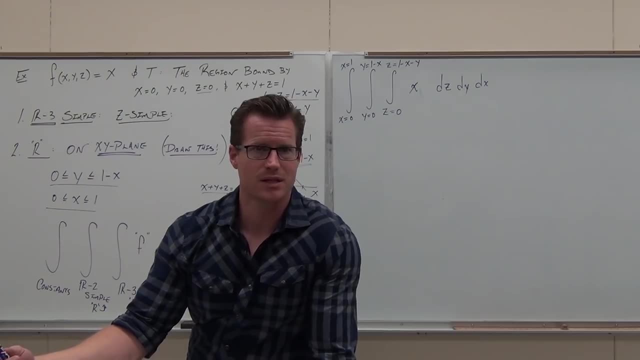 what would you integrate with respect to first, And then you plug in for the z variable, Then you integrate with respect to and you plug in for the y variable, then you integrate with respect to x and you plug in constants. Does that make sense? 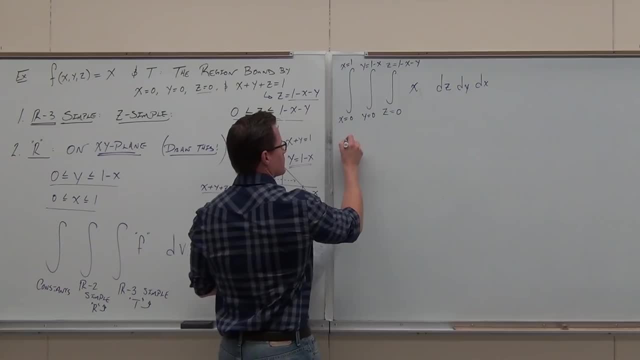 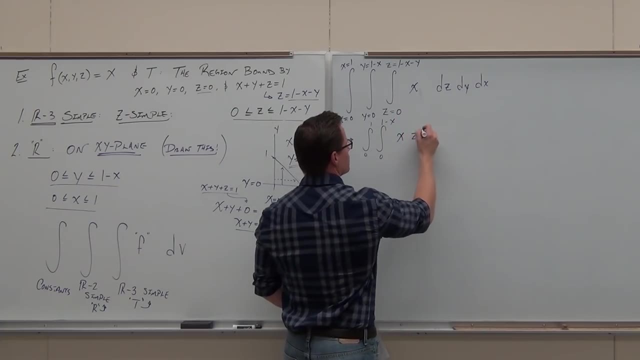 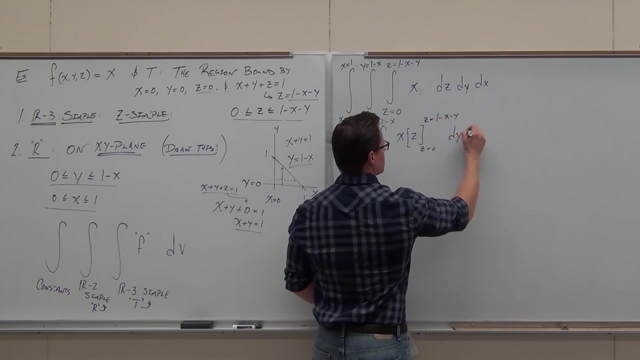 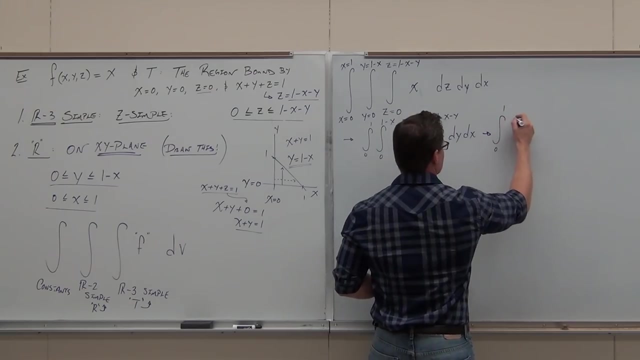 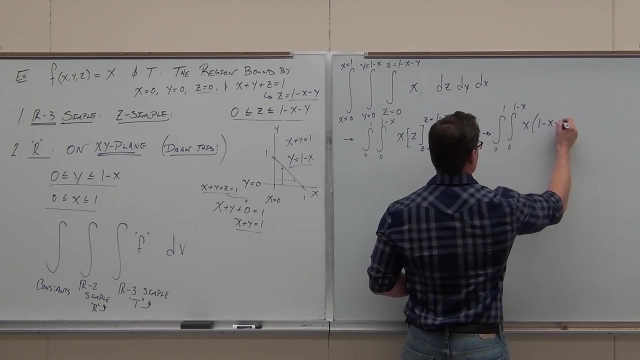 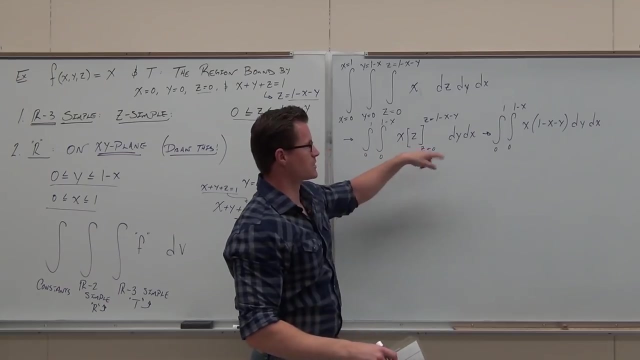 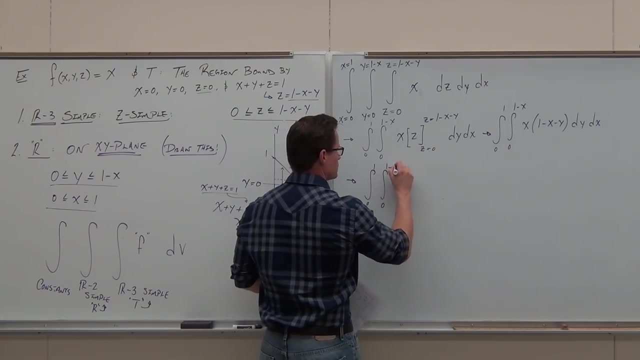 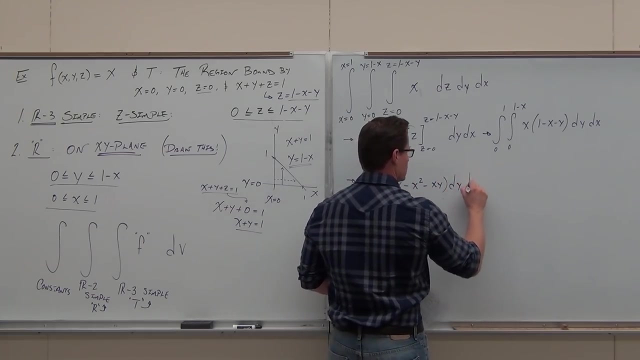 So here's the idea really quick: We integrate with respect to z. We get a z, We plug in for z. Z equals zero, no problem, We distribute. We're now forced to integrate with respect to y. Don't jump to the x. 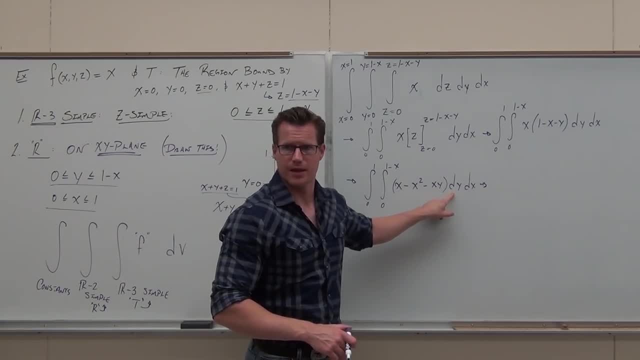 You're now forced to integrate with respect to y. Do you guys see what I'm talking about? You have to do that. It's in that order. That's the way we set it up. You can't just switch them around now. 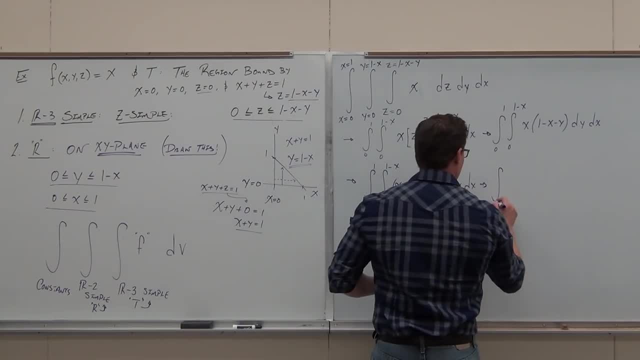 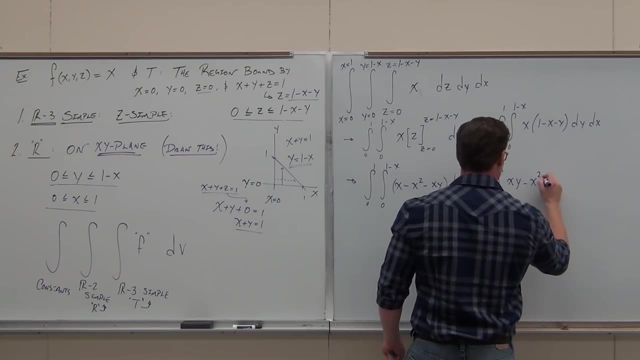 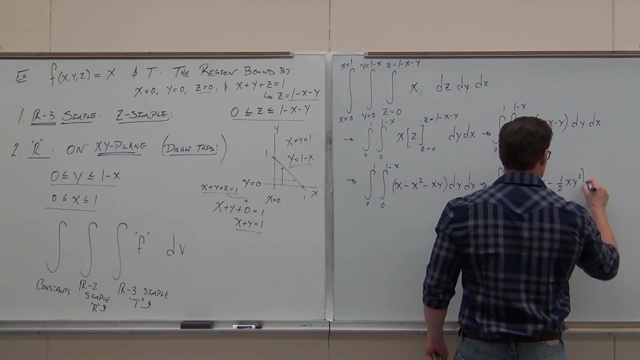 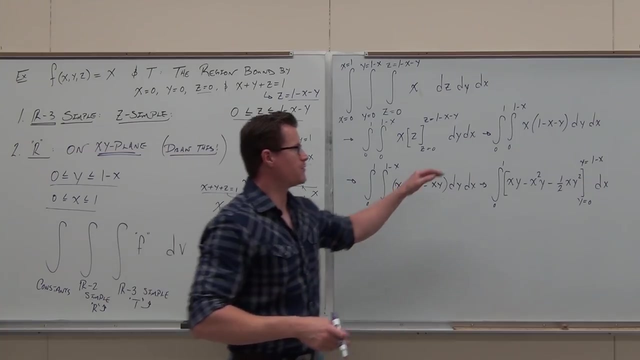 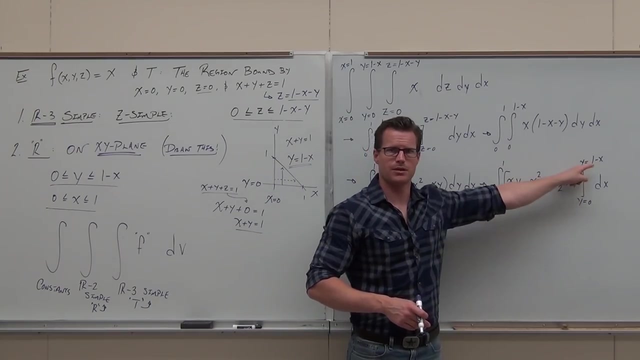 Otherwise you've got to redefine your graph. Don't do that. I'm hoping you can follow down the basic integration with respect to y and the fact that right now I've got a whole bunch of y's and I'm going to plug in this for all of them. 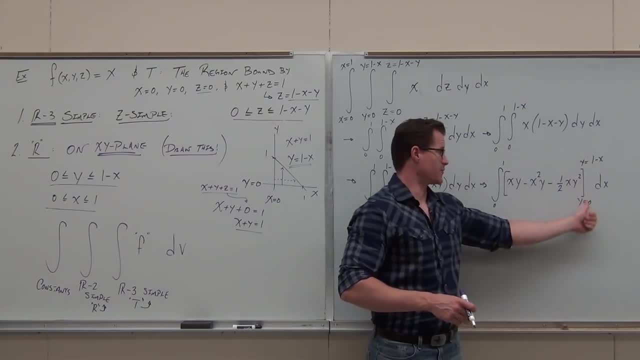 Do you guys see that? So this is going to be x times 1 minus. unfortunately, the y is zero. I love that, but I'm going to get this and all three of these places, and this one's got to be squared. 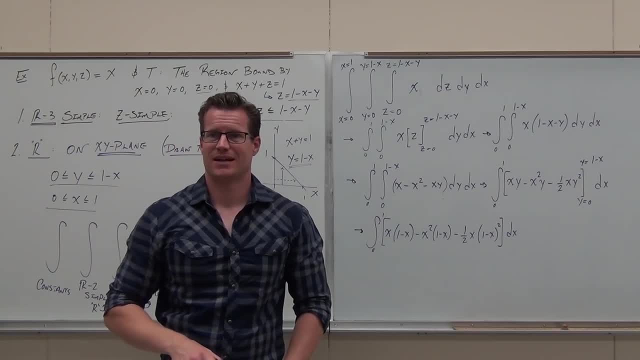 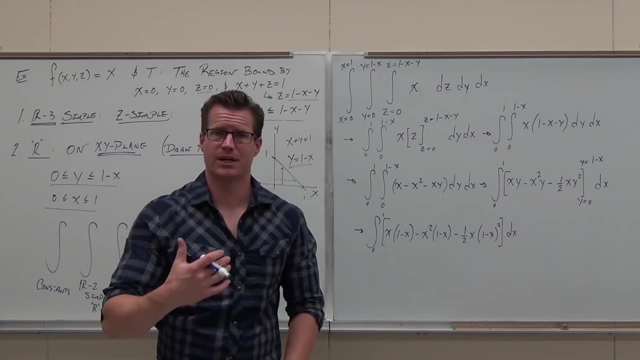 Now what? It looks crazy, but do you see that that's calc 1?? It's actually a basic calc 1.. It's a lot of distribution and combine like terms, but it's no u subs, It's just a basic calc 1 integral. 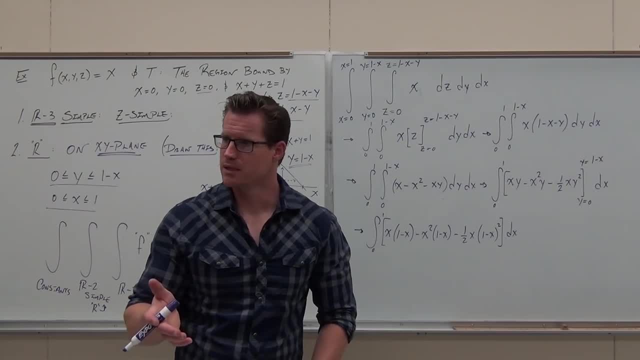 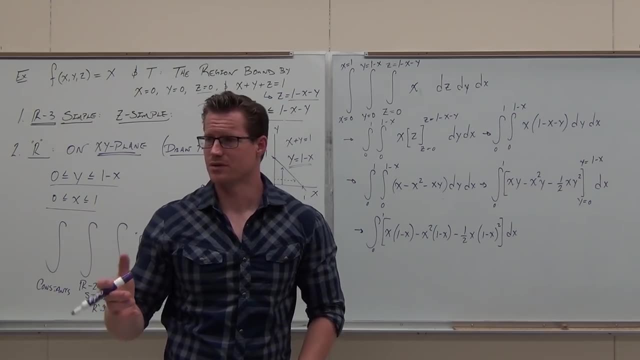 For real. some of these integrals are really easy because sometimes you can't do them and they take too long. So a lot of times you're dealt. the setup is hard, but the integration itself. tedious maybe, but not horrible. 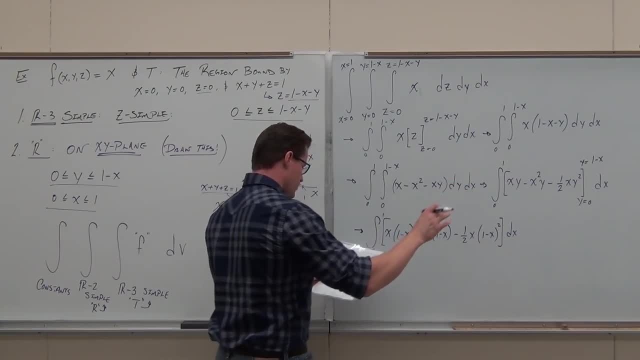 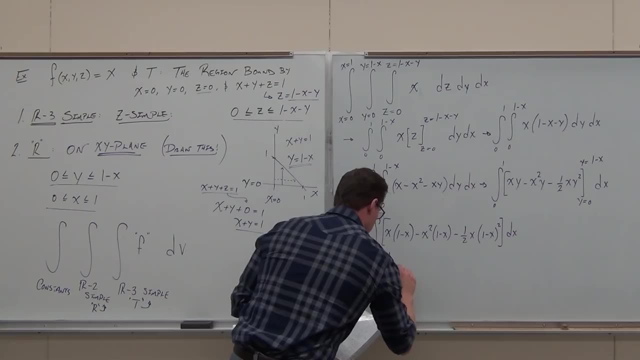 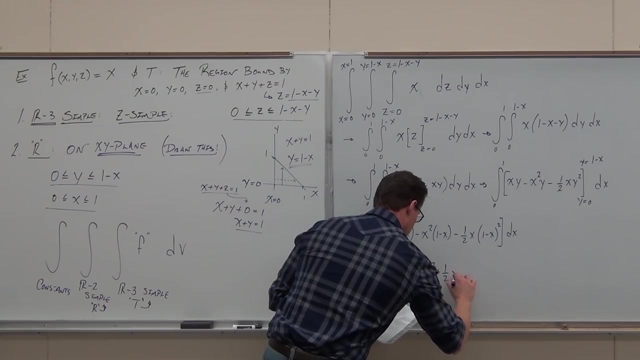 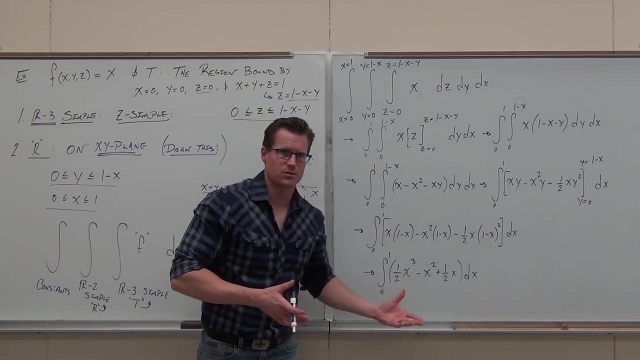 So here you can distribute by yourself. you can trust me This all I'm guessing that all of you are going to trust me. This all works down to this. Here's my question to you. Are you going to be okay if I just give you the answer to stuff like this? 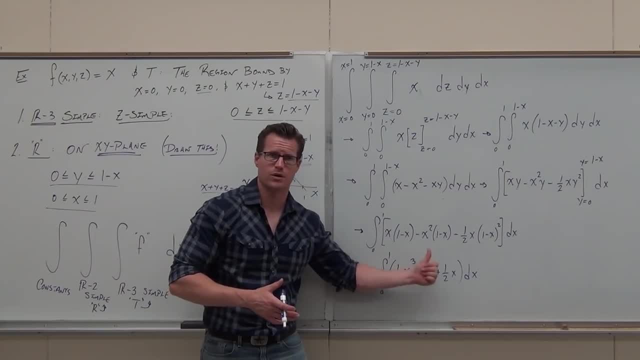 I don't really want to waste your time Integrating. you know what this is going to be. You're going to add 1, divide by 4.. You're going to add 1, divide by 3.. You're going to add 1, divide by 2.. 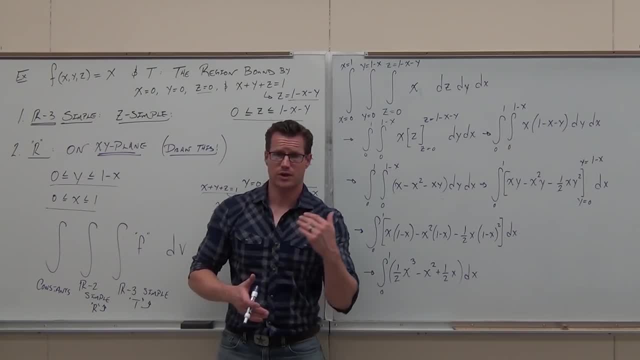 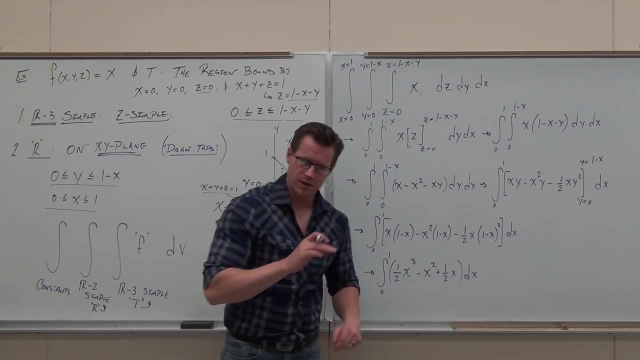 You guys see the idea there. Yeah, Are you sure? Yeah, Then you plug in 1,, you plug in 0. I'd like you to do it to make sure you still- you know, get this down. but the answer here is 1 over 24.. 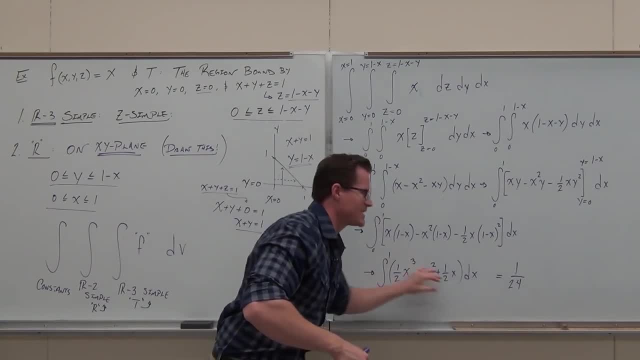 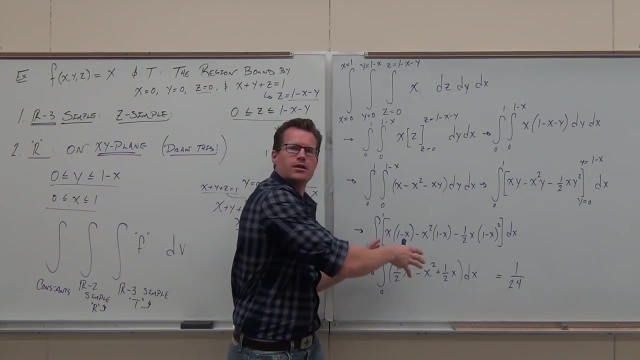 Again, my goal is not to just reiterate how to do basic integrals. It's to do the setup and do the first few steps so that you're learning. You're learning this and then relying on your old knowledge to do this. I don't want to be the type of teacher who goes well. 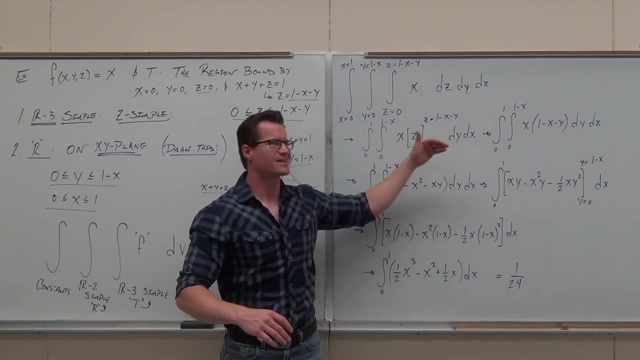 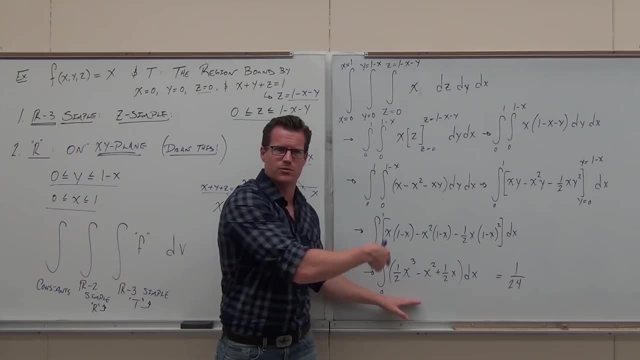 you guys are supposed to know this. so from here you're good? No, that's not quite true, But from here, yeah, I mean you need to be good from here. Is that fair enough to ask you to be okay from here? 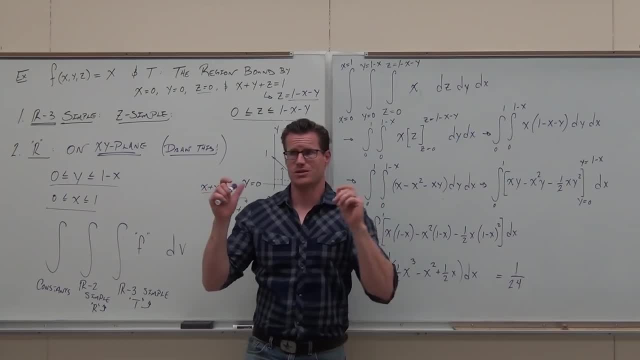 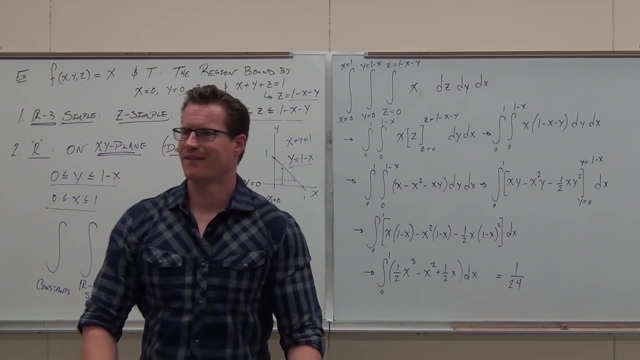 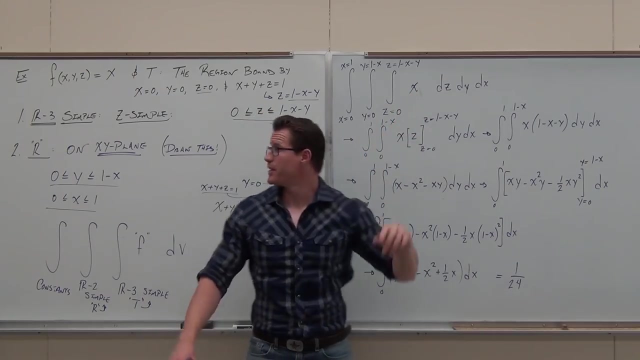 Okay, so you integrate, plug in 1,, plug in 0, subtract them and you're golden. I know that you're okay with it. Now, what is that? What is that? It depends, If that is the mass density function of this region, that we have 3D, 3D region. 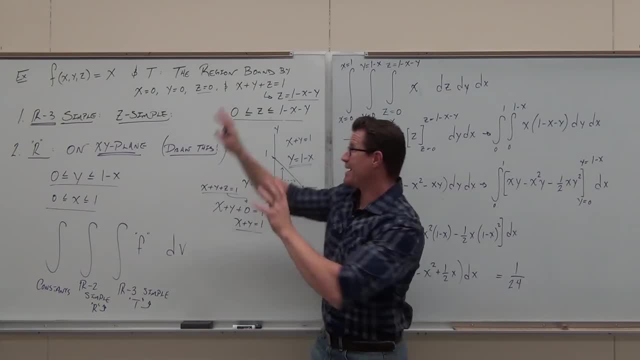 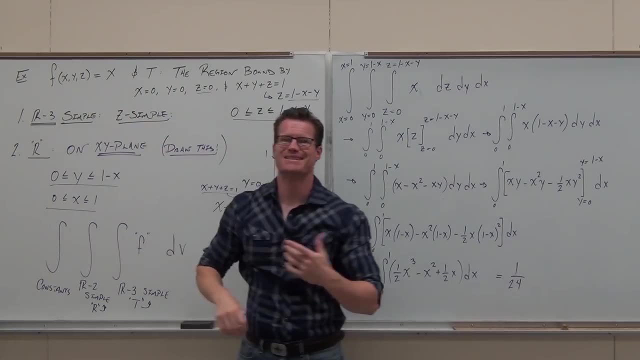 if that's the mass density function of that region. we just found the mass of that region Make sense. It doesn't have to do with that as far as the region is concerned. It has to do with that as far as the mass density is concerned. 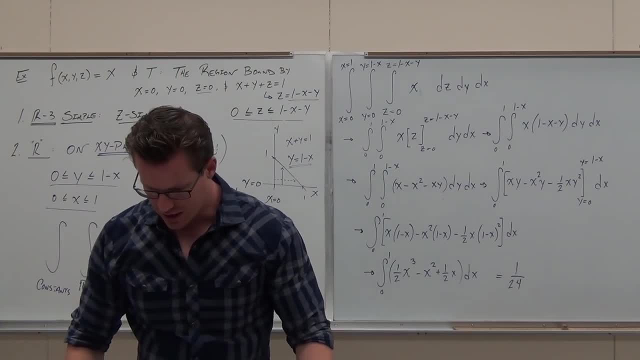 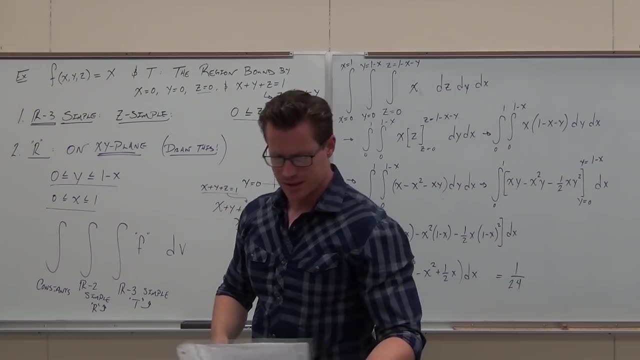 So it depends. if you understand the concept there, That's pretty cool. Now we're going to do a couple more Honestly, as many as we have time. we're just. it's all about the practice of the setup, So let's get to it. 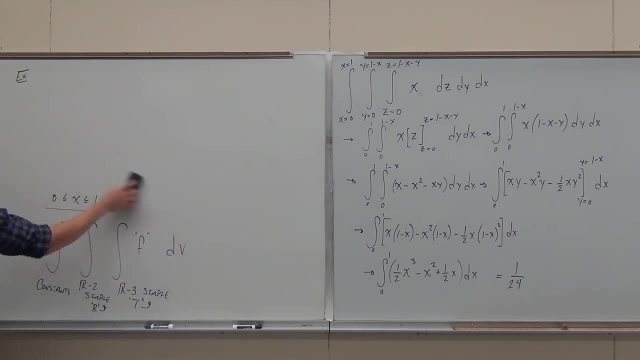 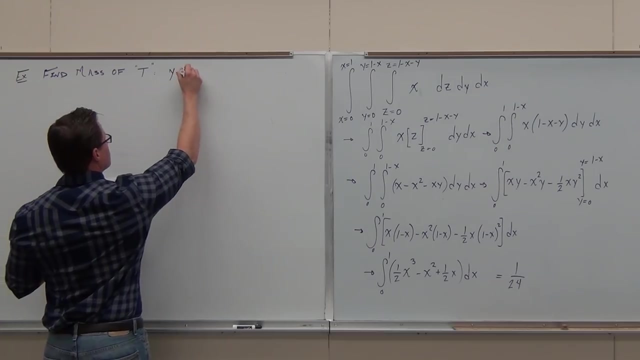 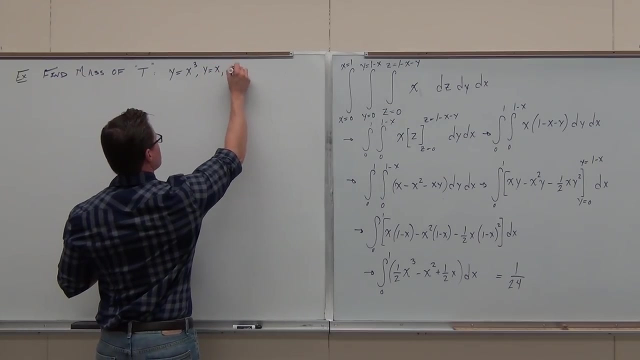 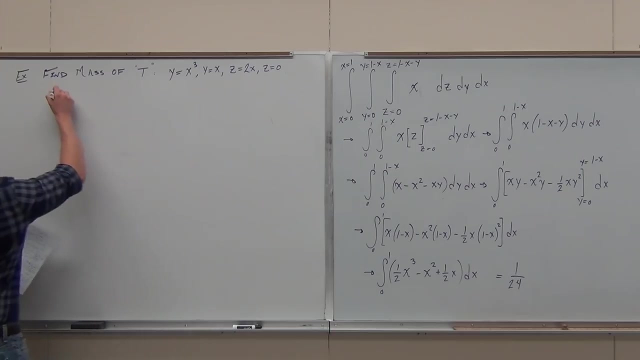 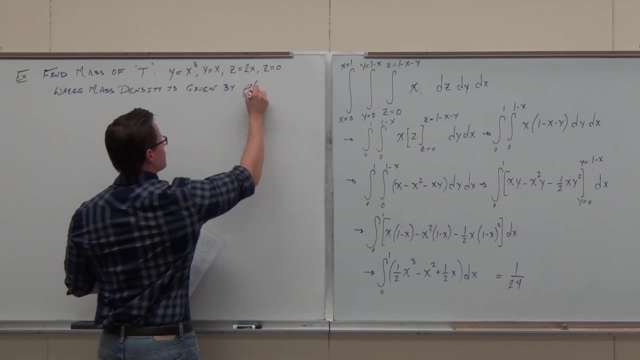 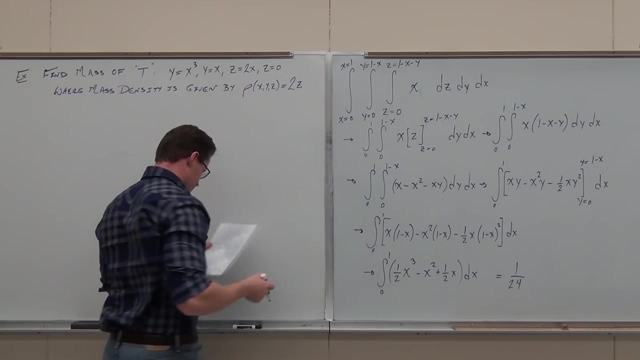 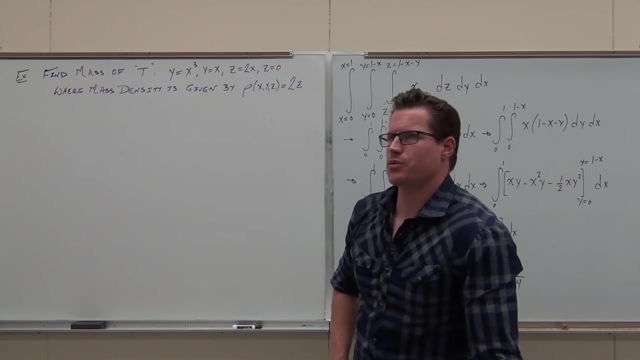 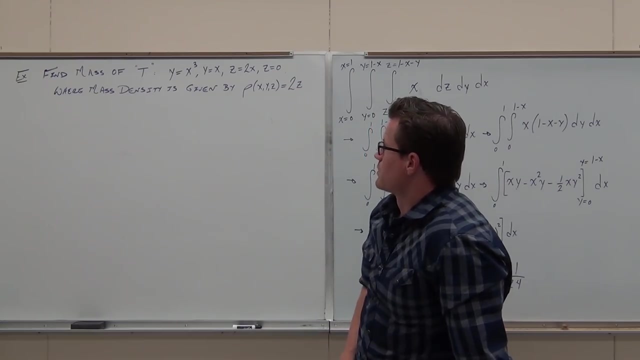 Okay, Thank you. So find the mass of the region T. where the region T is given by that thing, y equals x, cubed y equals x, z equals 2x and z equals 0.. So notice, if you were to graph all that stuff, 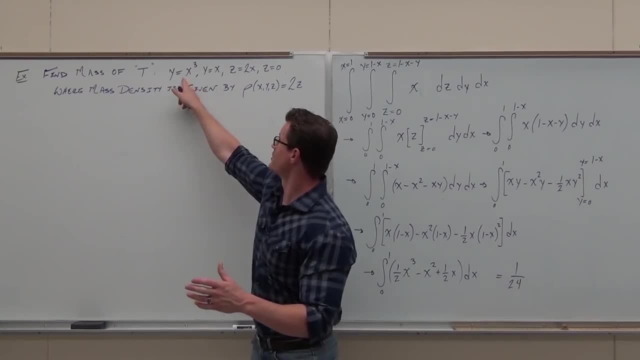 it is going to be in 3D. Do you guys see that that's going to be in 3D? You've got a cylinder, you've got a plane, you've got another plane and you've got another plane, And when they all cross each other, 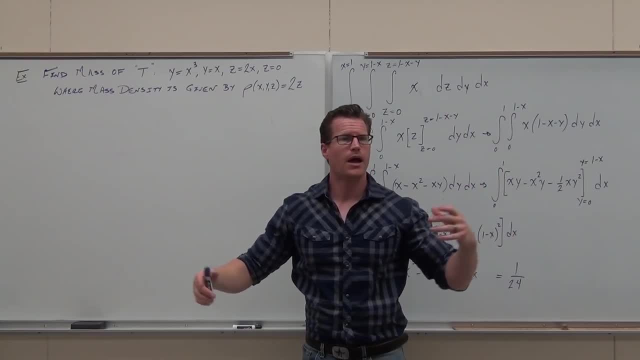 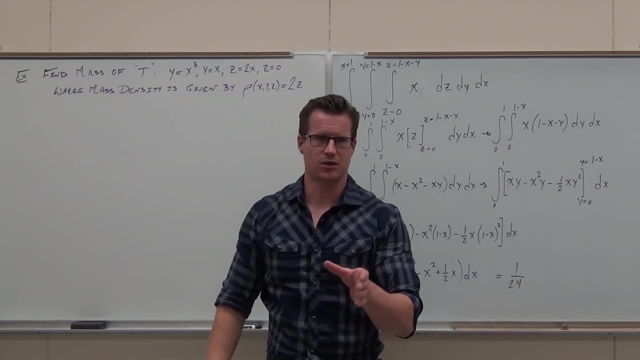 you get this three-dimensional region. That's what we're dealing with here, And I'm telling you. the mass density of that region is given by 2z. And now, if you understand the problem here, this is how your test is going to look. 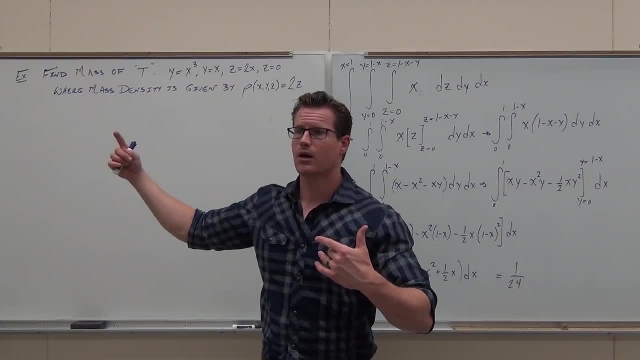 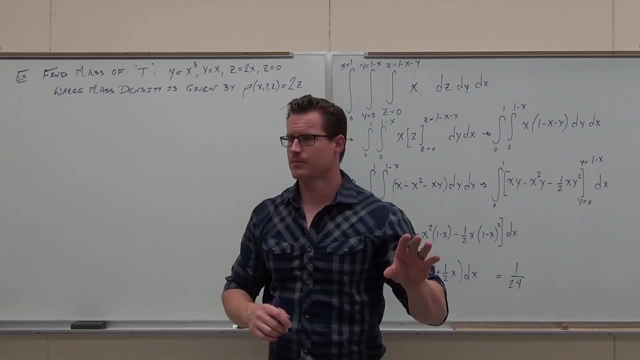 I'm going to say: I want you to find the mass of the region. This is what this looks like. What's your first, first step? Say that again: R3 simple, R3 simple. So we're going to choose. 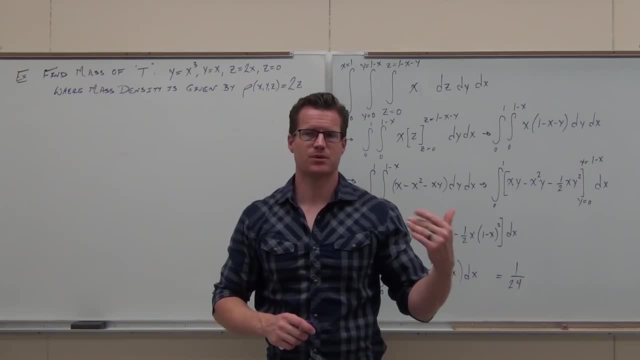 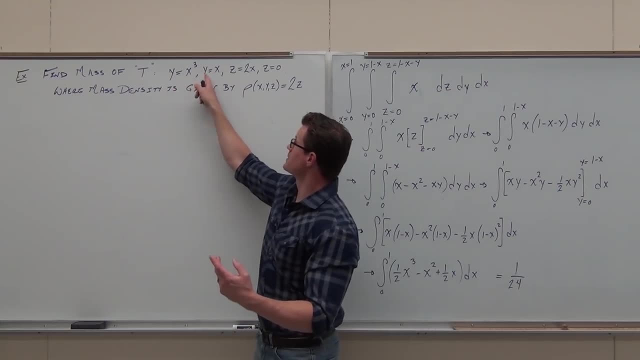 well, we've got three variables to choose from. We're going to choose x simple, y simple or z simple. Now, what's the best choice? It's between two of them. You're either going to choose y simple or z simple. 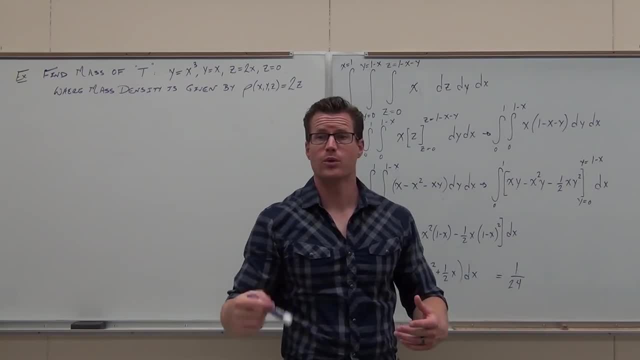 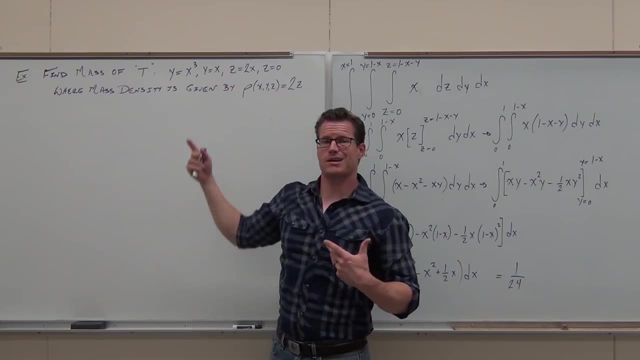 How do we know? Well, choose the ones where the variables are already solved for, So you have to do less work. So y simple, maybe Z simple, maybe Two options. What am I going to pick? I'm going to pick z simple. 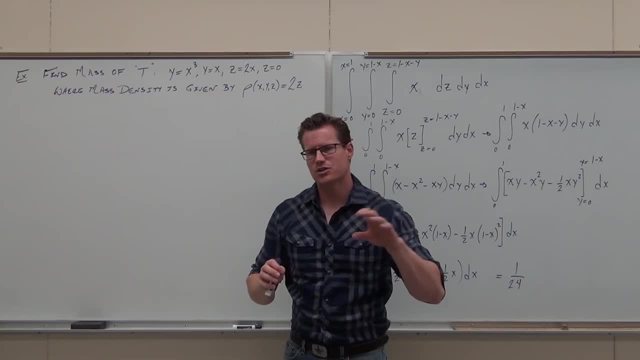 It probably doesn't matter, But I'm going to pick z simple because I like to draw my regions on the xy plane, because I'm used to it. I make less mistakes that way. Does that make sense? So, even though we have two choices here, I'm going to pick z simple, as often. 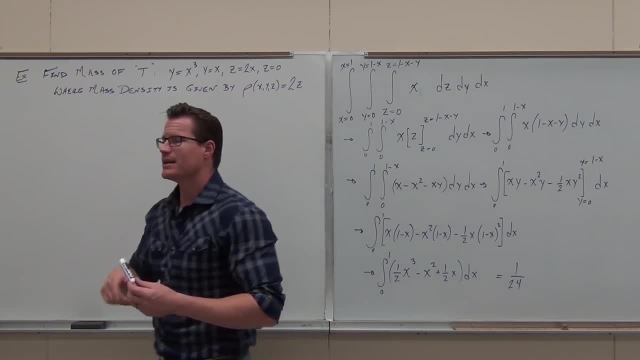 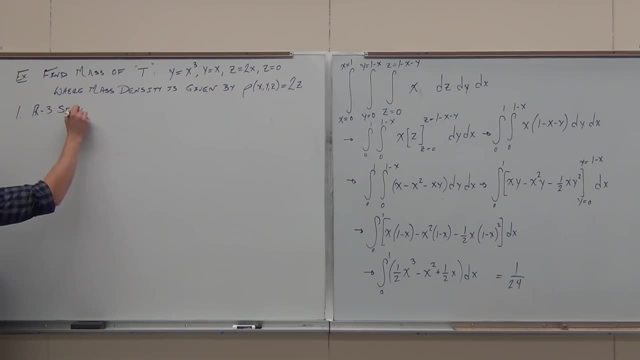 as I can, provided the integrals are still easy. So let's go ahead. Let's set that up. Step one is R3 simple, So we're going to write that down. You're going to tell me what your choice is. 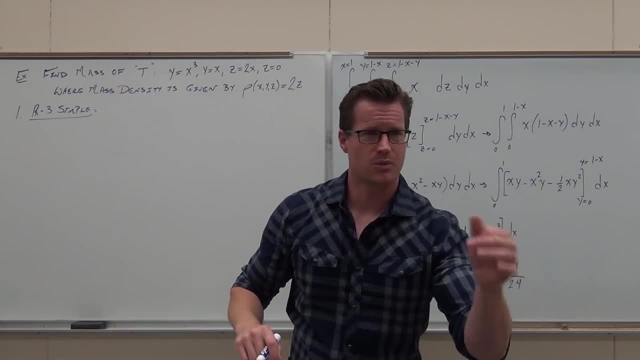 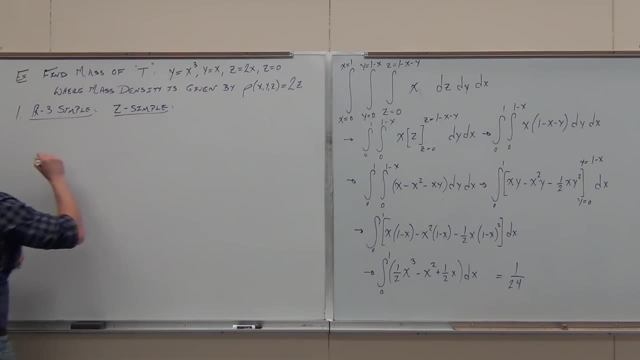 You're going to tell me what you're choosing right now. What are we choosing? R3 simple, What are we choosing? So write down z simple And let's go ahead. If we're choosing z simple, then the first thing we do is we have to make sure. 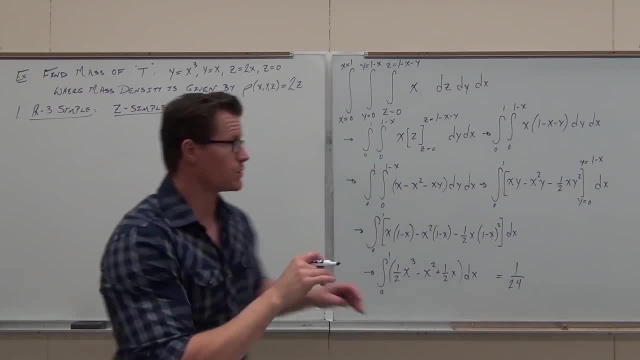 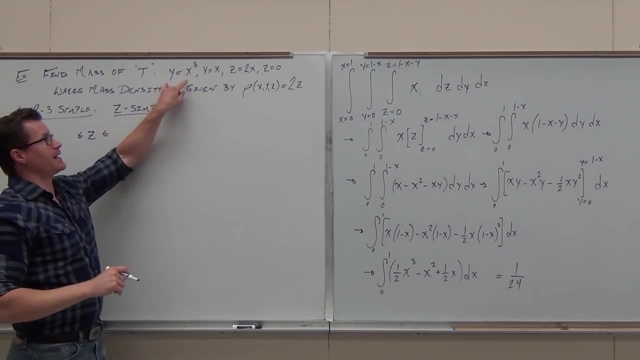 that z is bound between two functions of z equals. So here, since we already got it equal to two functions, we're going to have z between. well, let's look at it, That ain't got no z's. That ain't got no z's. 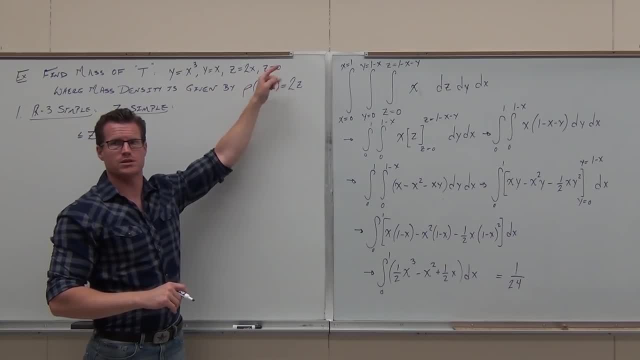 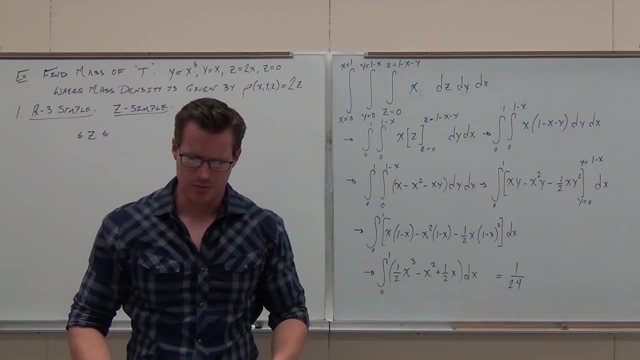 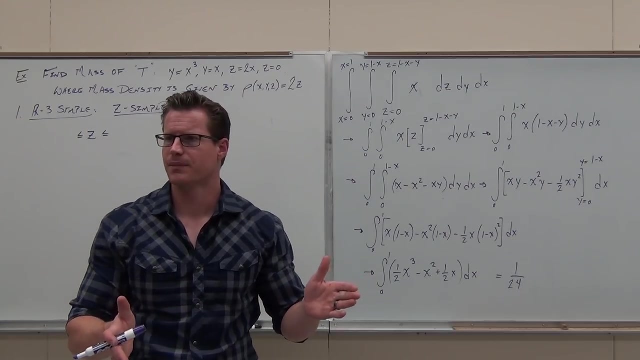 That's got some z's And that's got some z's, So what's the smallest value for z that we have? Yeah, I do got to tell you a lot of times. textbooks do not tell you this, but oftentimes we try to restrict where these graphs are to the first quadrant. 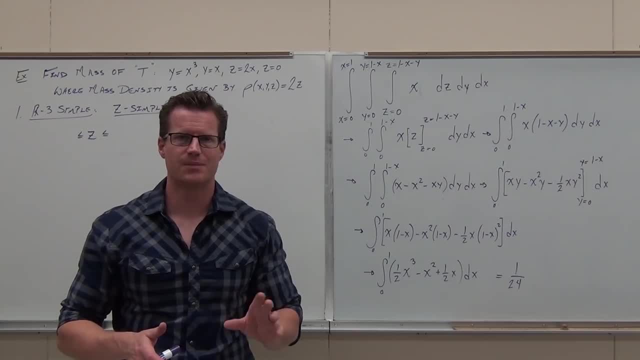 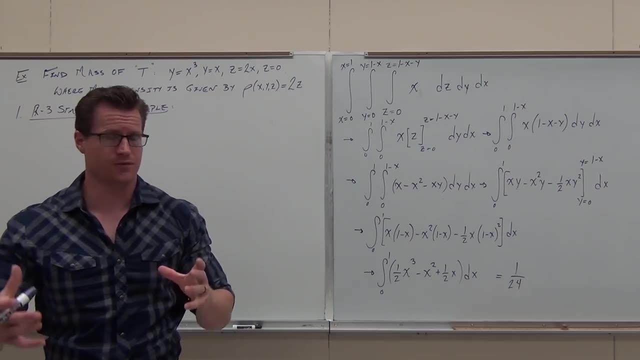 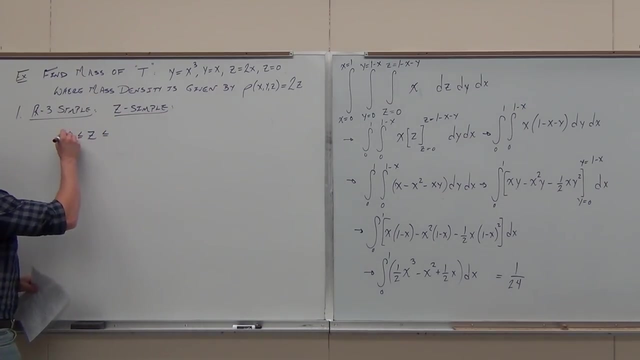 of whatever coordinate plane you have. So typically that's the case here, Because when we start graphing this, this does go down to the third quadrant rather than just the first, but oftentimes we restrict it to the first quadrant. So if that's the case, then x is growing positive and we'd have z between 0 and 2x. 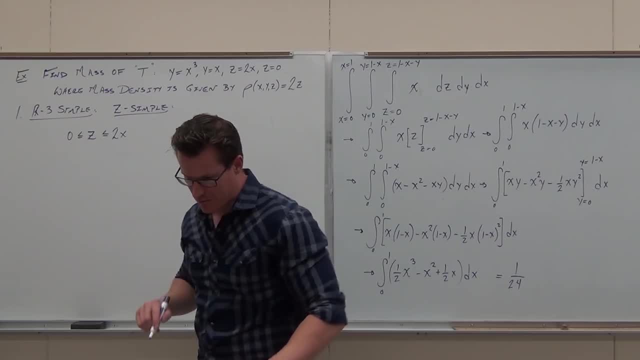 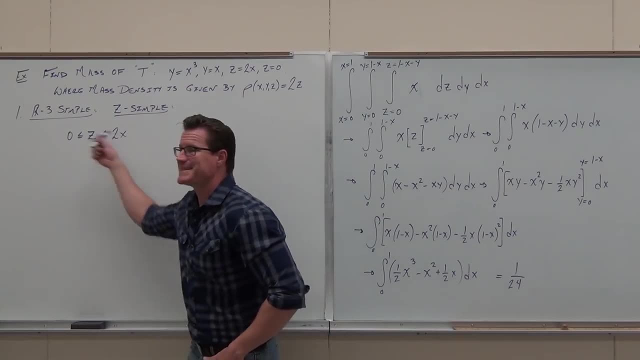 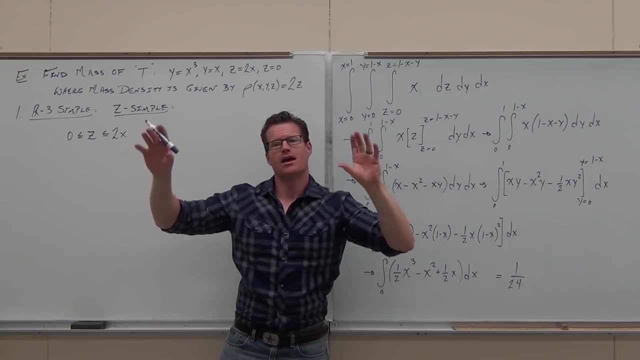 Is that clear enough for you? That's what that does. Now, if I chose z, simple, we're practically done. Do you guys realize that we've already done this? right now, We just got that. That's the hardest part is getting that and then making double integral. 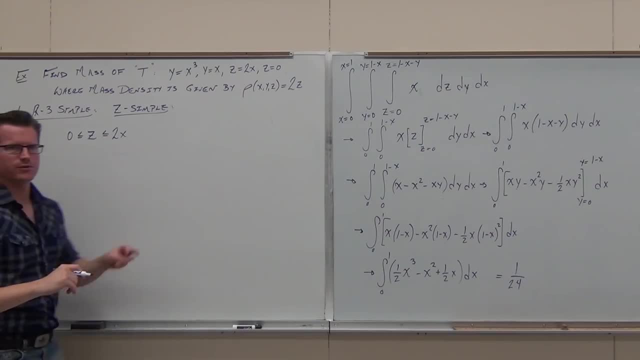 Okay, Let's make a double integral. How do we do it? Well, the next thing we do after you've picked z- you pick z simple- is determine what The region for our double integral. So let's talk about r, the region for our double integral. 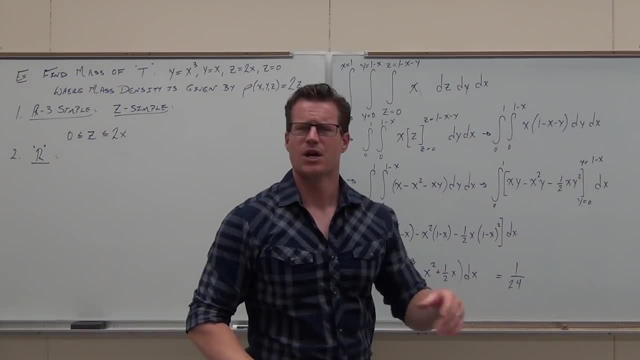 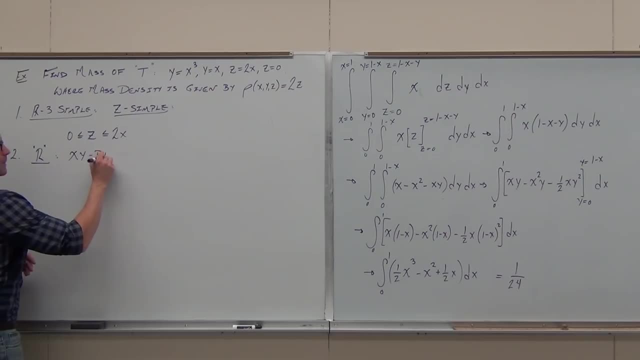 Can you please describe for me- and you should be writing this down every time you do these problems- what plane is the region for our double integral going to be on xy? That means that right now you should be drawing me an xy plane. 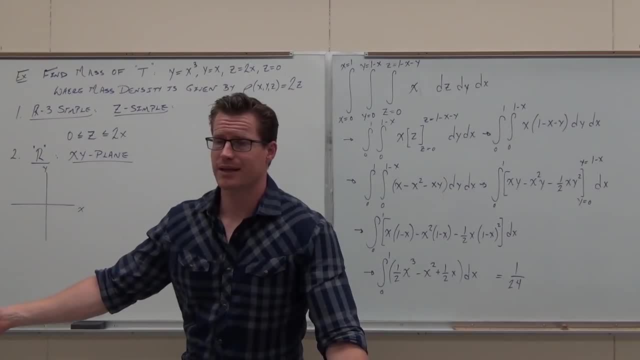 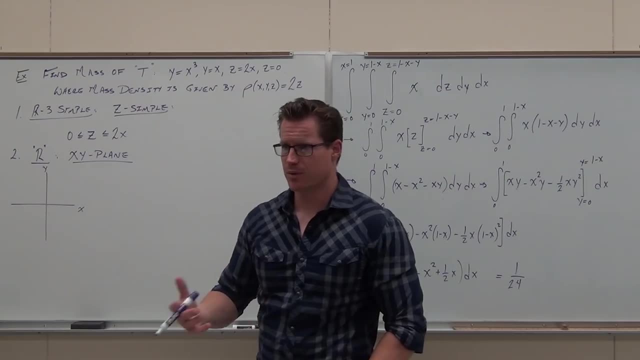 We always draw the, just like in double integrals. you always draw the xy plane If you drew the region- unless you had like rectangular numbers, and it was pretty easy if it was given to you here- we're always going to be drawing the region to set up our double integrals. 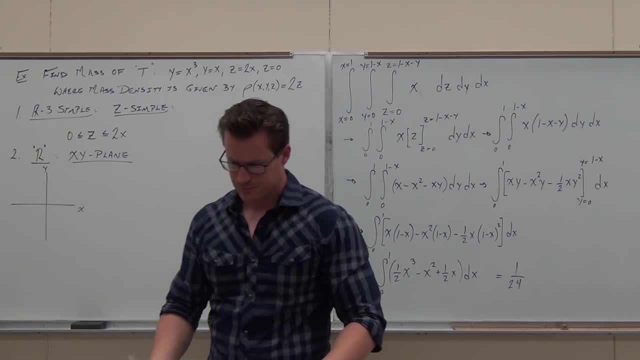 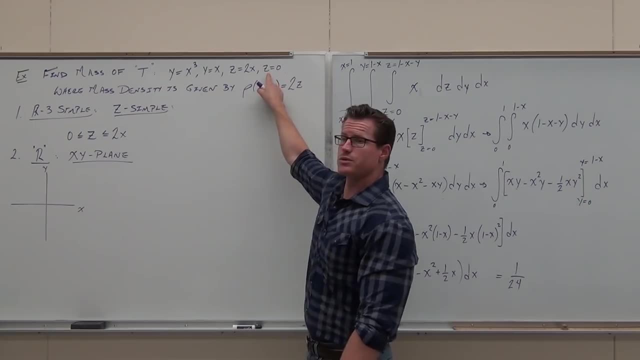 because they're always going to be between functions. Now, oh my gosh, can you draw this stuff? Well, let's see. Do you need to draw z equals 0?? Well, no, because that's literally the xy. Do you need to draw z equals 2x? 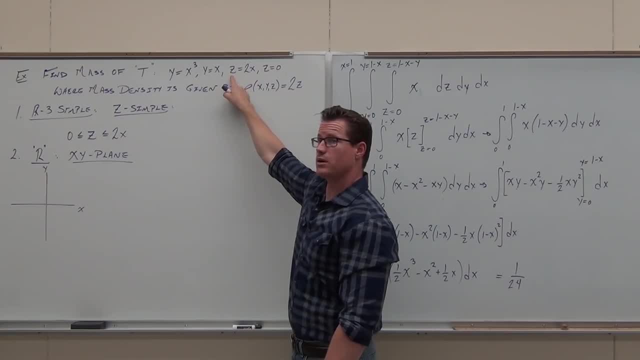 It does give you something, though. It says that if z equals 2x, it's going to be 2x. If z equals 0, then x equals 0.. Do you see it? It's giving you the x equals 0 line. 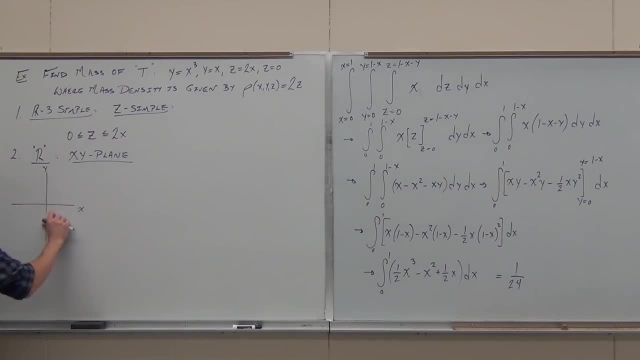 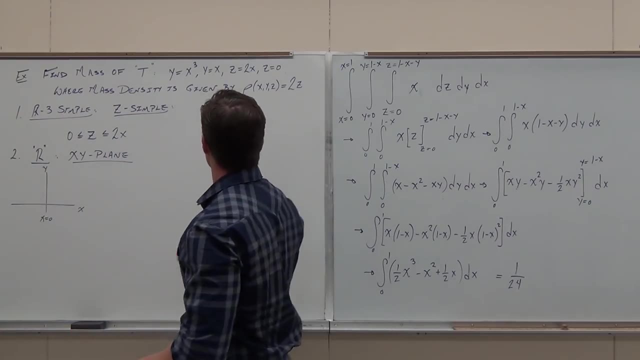 You can actually use that. So x equals 0,. I know that that's part of my boundary. just the y axis. Okay, Can you draw? y equals x on the xy plane. So use the pieces that are relevant. Let's draw that. 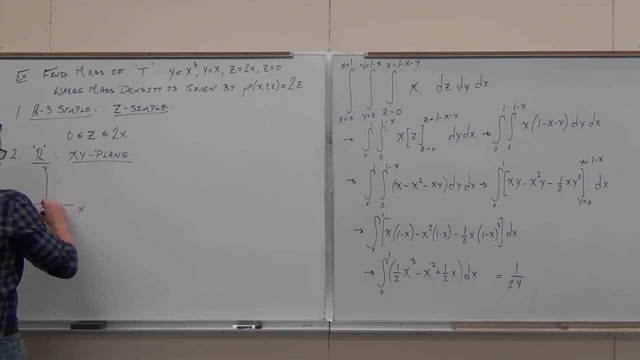 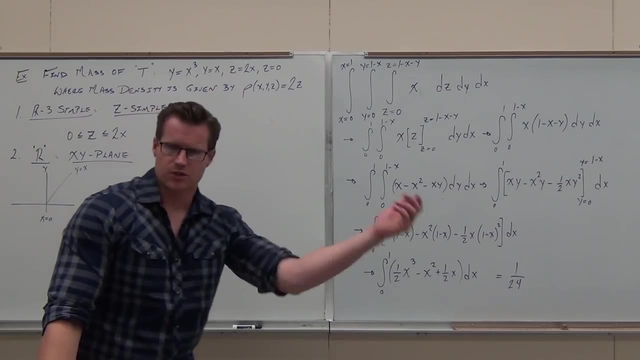 What's that? give you A line, of course, a diagonal line. What else can you draw? What else should you be drawing right now? right, Cyrus, Can you draw that one? Yes, You can just sketch it, It's fine. 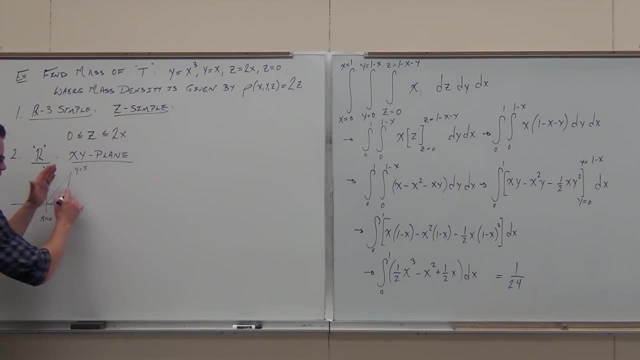 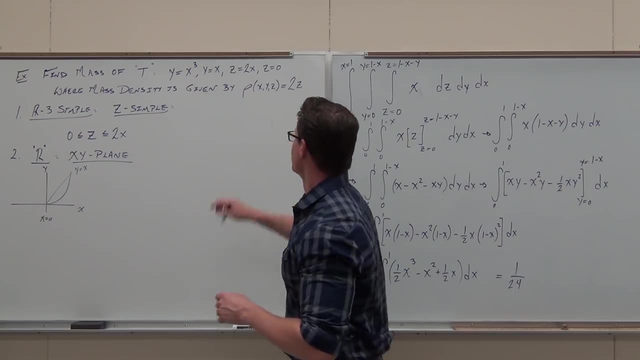 This is why we normally consider the region to be here, because these are both traveling down the third coordinate. also, We're not going to consider that, We're just going to consider the positive. That z equals 0 also tells us that, so we want to consider. 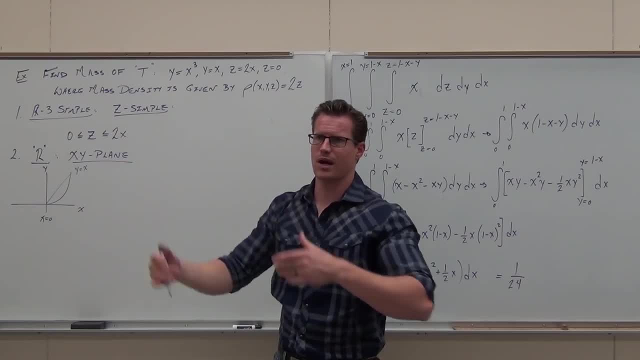 that to be our bottom here. It's bound in the upper part of our graph. We tend to do that. We typically do it, even if it's unsaid, We typically do that. I know it can be a little bit weird, but 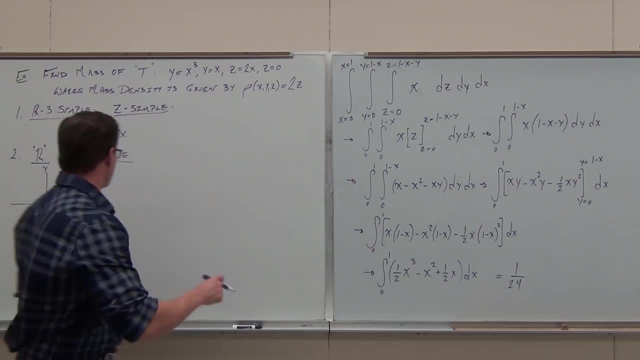 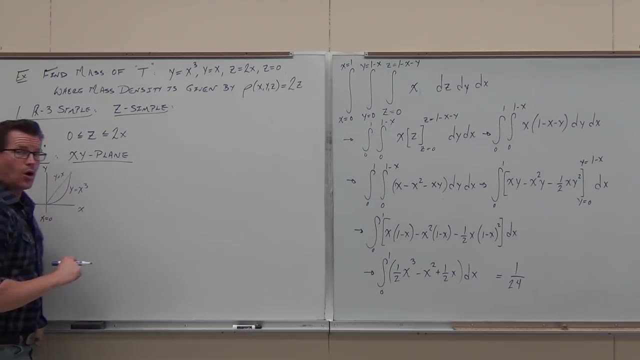 Now, now, in order to do this really correctly, we need to outline what these functions are. I know this is y equals x. I know this is y equals x- cubed, but you also need to know what the intersections are. Why do you need to know what the intersections are? 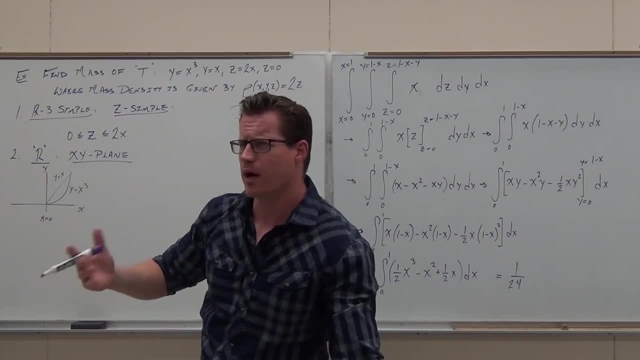 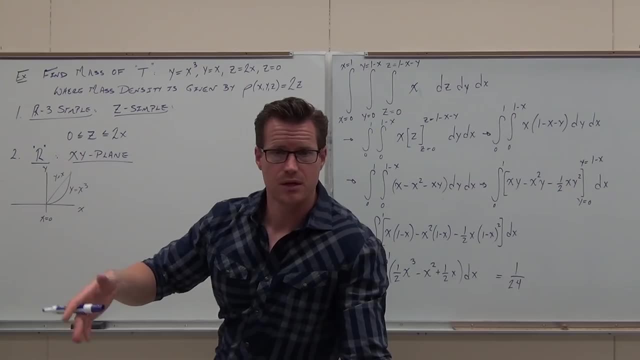 Think about what you would do for your last, most outside integral. It goes between what Constants. Constants are the points, So you need to know what your intersections are so you can draw them, Evaluate for your constants. Does that make sense? So how well? how do we do it? 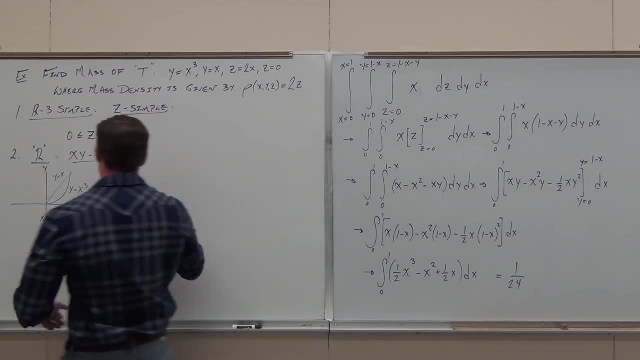 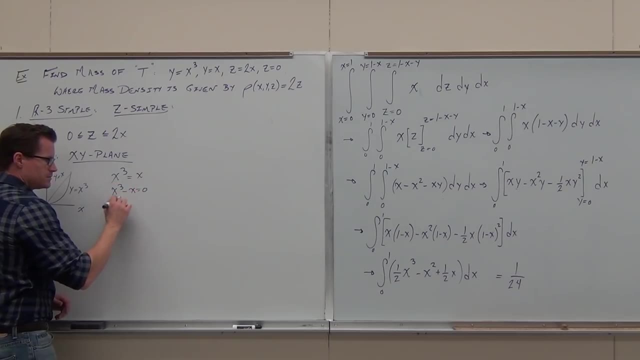 How do you always find out where things intersect? You might do that X cubed equals x. Set these equal to find the intersection X cubed minus x equals 0. We get x equals 0, x equals 1, and x equals negative 1.. 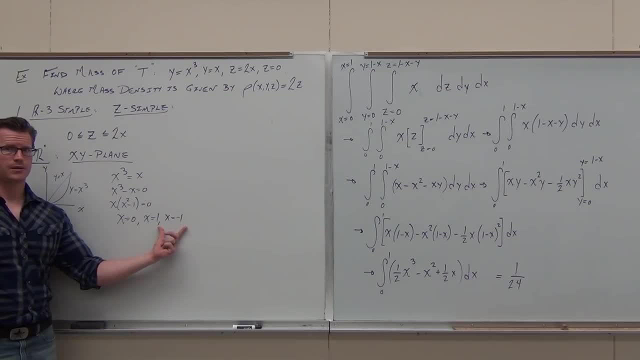 Now I'll tell you right now that x equals negative 1.. If I close this, it's going to be negative 1.. If I plug in negative 1, I get something that's outside of that region that we defined. 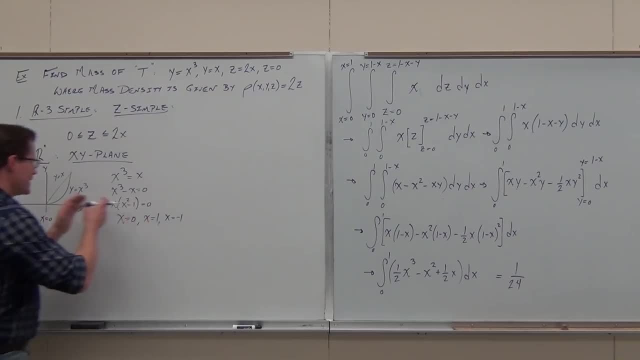 That's also how we tell that this was just in this quadrant and not in the bottom quadrant. Does that make sense to you? That would fail our constraint for our R3, how we define that. So this guy- no, that one not. 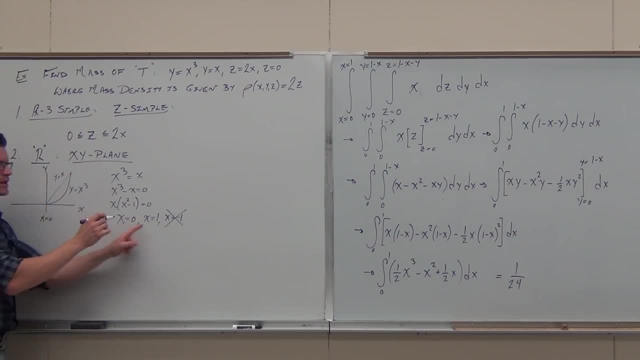 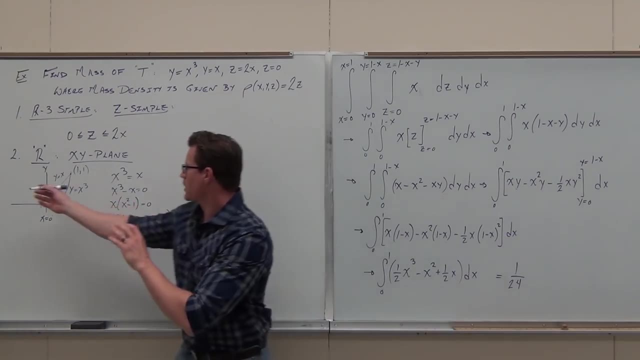 But now I do know that x equals 0, and if I plug in 1,, I know that's the point 1, 1.. Listen, write these as points That way, if you do go along the x first and you go along the y. 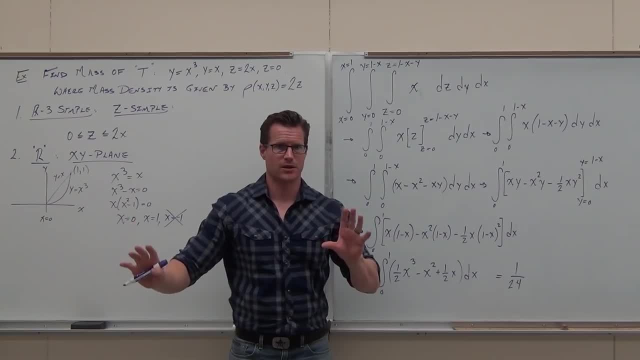 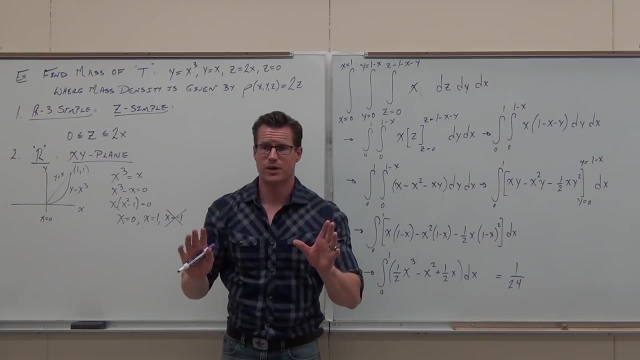 second or whatever you're going to get a point: If you go along the y first, x second, you have both values there. You don't have to just know along one axis. Does that make sense to you? So we're going 0, 0 to 1, 1,. no matter whether we do x or y. 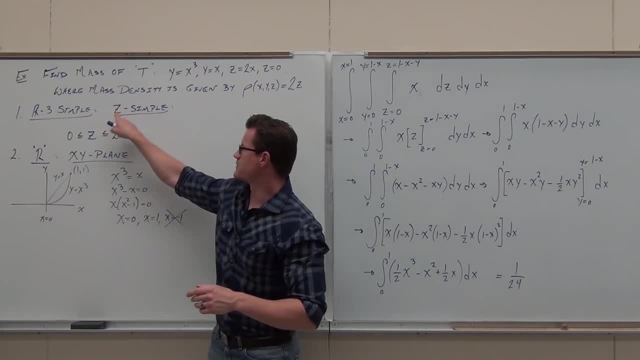 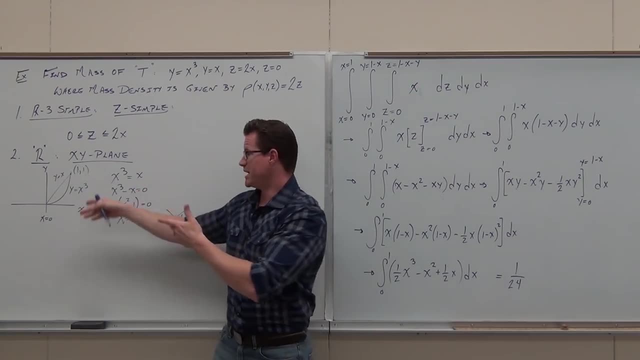 Now let's see if you're with me. Are you guys okay on the choice of z, simple and 0 to 2x over r, Perfect. Are you guys okay that the r is going to be on the xy plane? I know you're okay with graphing them. 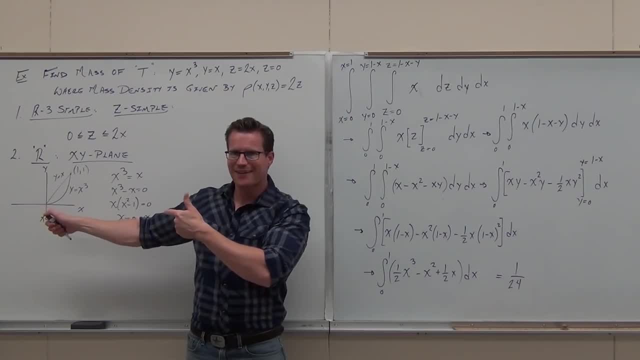 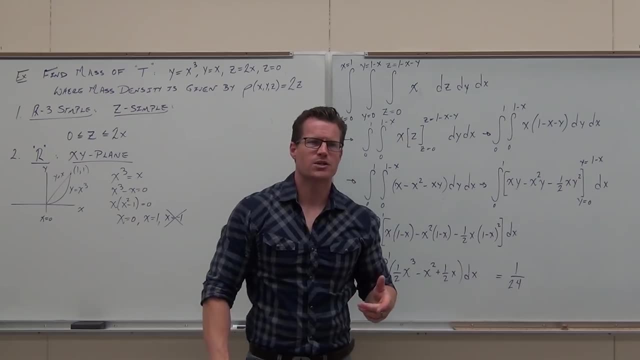 We've done that a lot for double integrals. I don't know if you're okay, Are you okay with graphing them? You're okay on finding it? You're okay on finding the intersection? Now, what right-siders would be the good choice to do next? 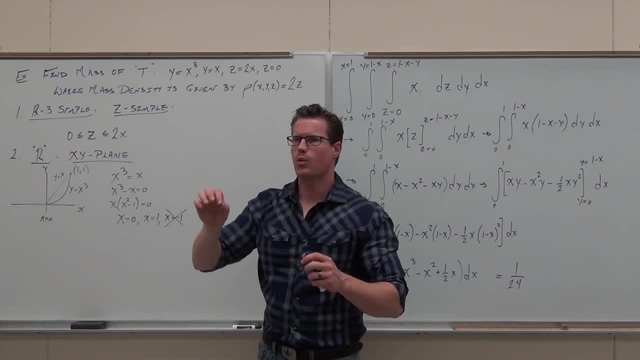 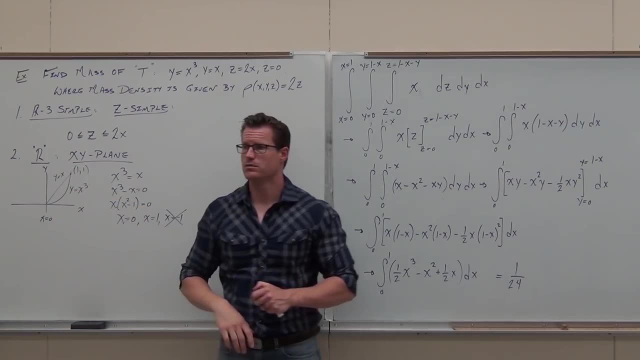 We already went along the z, I'm going to have dz first. What's the next best choice? Would you go along the y or along the x? Given how we've written our, given that it doesn't even matter, I can go along either one I want. 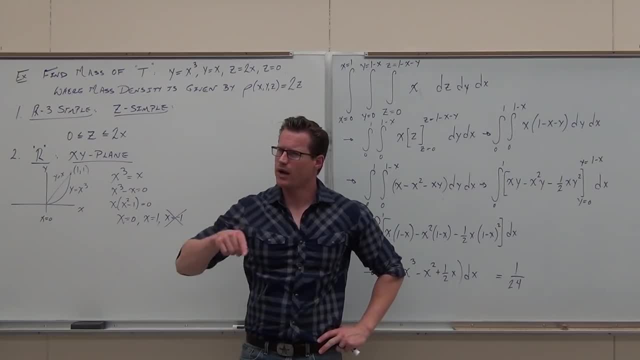 But, given how we've written our functions, what's the best thing to do? A dy or a dx? What do you think A dy? Why? Because it's already in terms of y, That's a, that's yeah. that's exactly right. 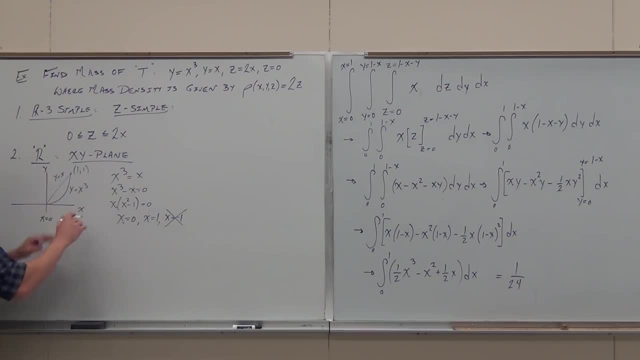 So let's do that. So I want to set up my region. I'm going to do dy first, which means I want to go along the y first. That means that y is the guy that we've got to have between two functions. 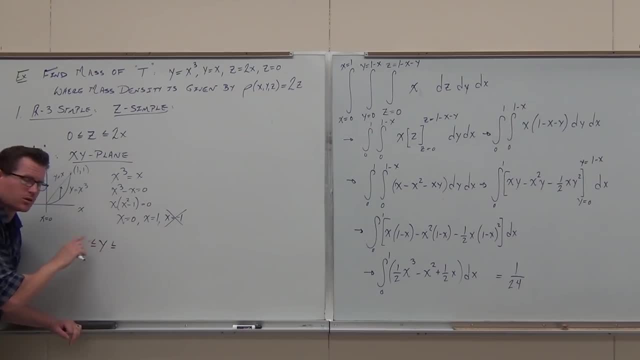 Now use your region appropriately. What's the smaller when I get to that? what's the smaller of the functions here? Excuse me, And then I ultimately reach. Yeah, Ladies and gentlemen, is that is that clear for you? 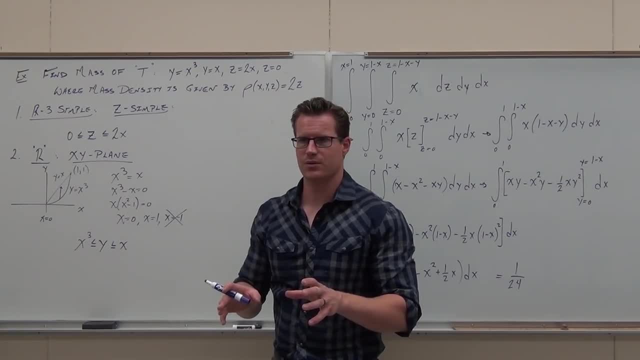 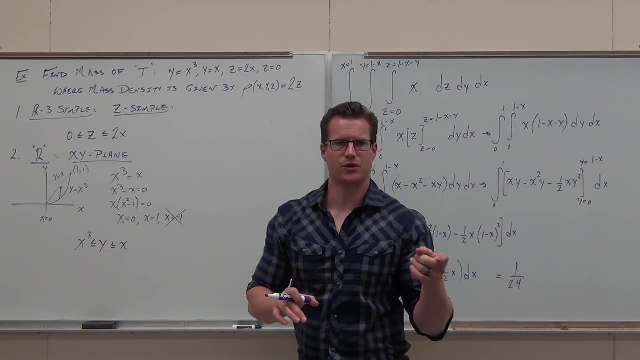 I don't want to lose you now. You've learned too much from me to lose you now. Are you guys okay with that one? Yeah, Question: Explain why we went along the y axis. The question was: why did we go along the y? 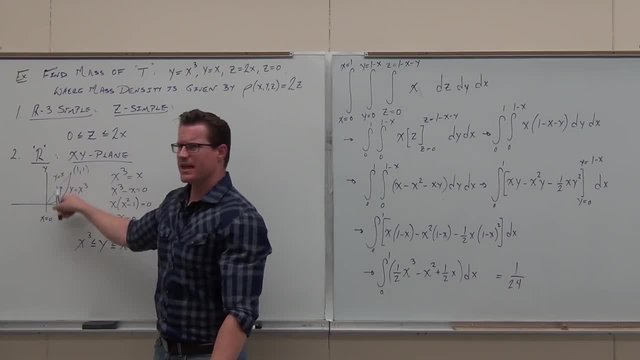 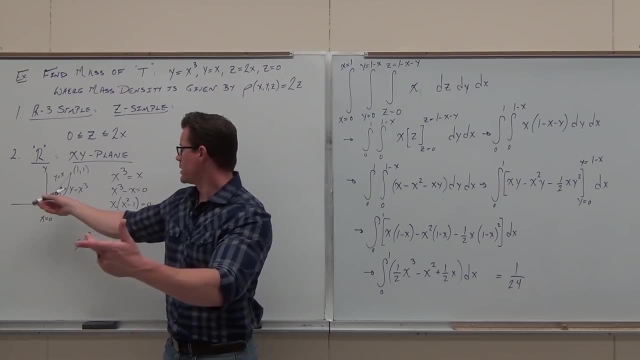 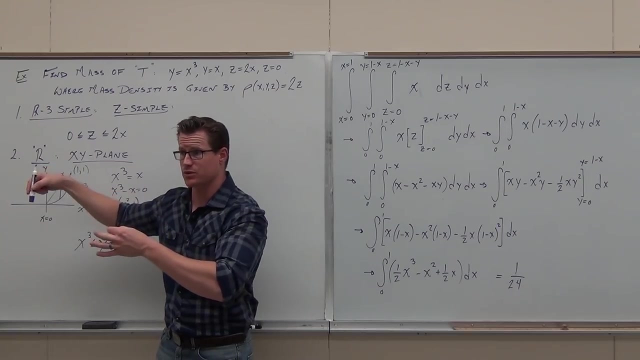 Why? why did we do this? Why not that? The answer is: Say what now We would If we went along this way? we'd have to have x equals functions. That's the question. Does that make sense? Along the y between y equals. 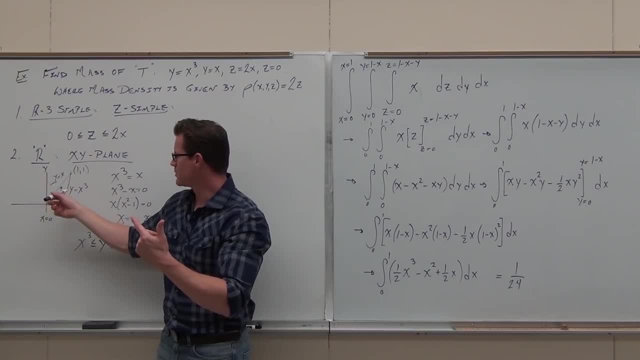 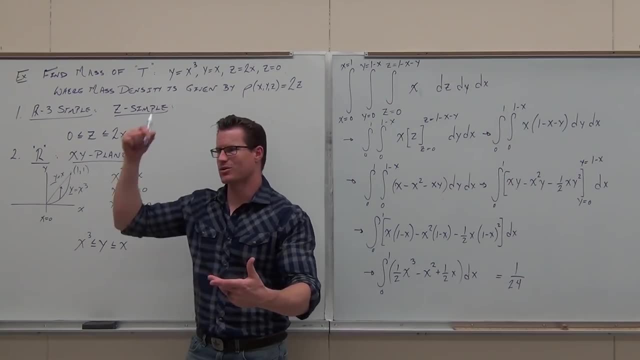 Along the x between x equals, Since these are already defined as y equals and y equals. that's the easier choice. Does it matter? No, No, But because it's already set up that way, it's nice to go along the y. 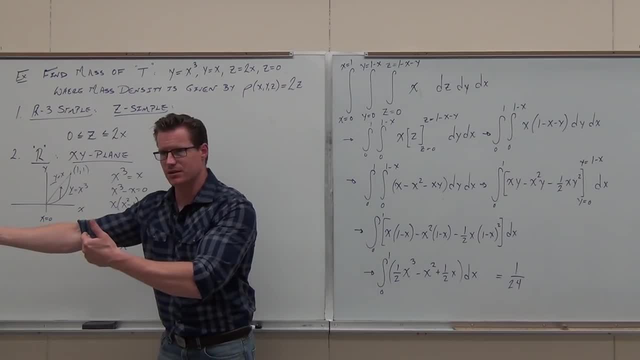 Because now I'm between two functions of y equals. That's the. that's the point. That's why we did that. Is that? is that clear enough? Now the bottom. it's important, you know, the bottom of the top one. 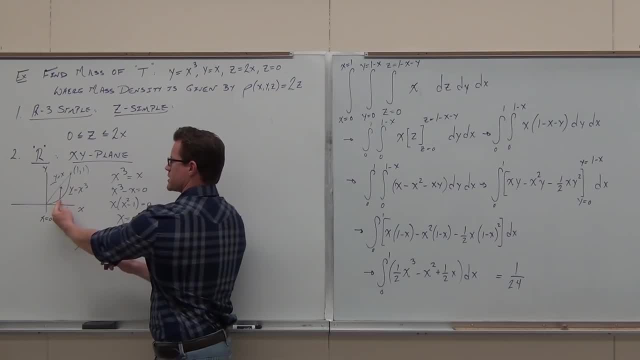 So, along our region, along the y, from smallest to largest, we first get into this region by hitting y equals Y equals x, cubed, That's why it's small. And then, ultimately, by hitting y equals x, that's why it's a larger bound. 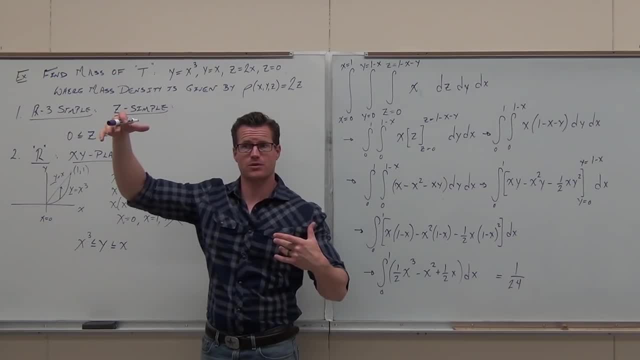 So basically we're good with that one. Okay, That's set up the first of our double integrals. Now we set up the last part. It's the easiest part, It's always constants. Now we're going to go along the x. 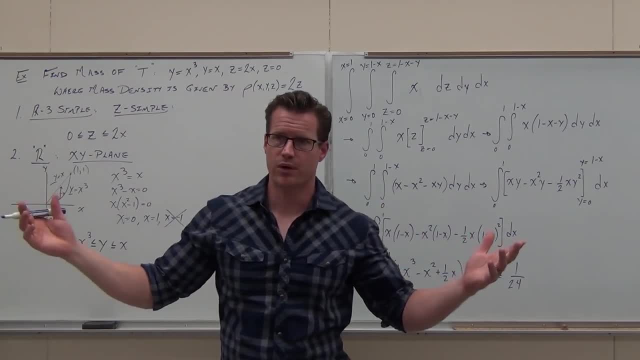 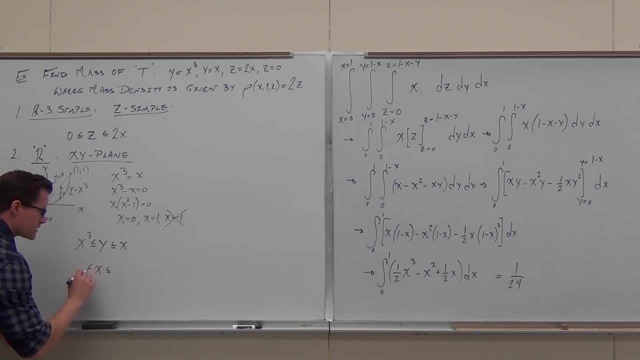 It should look very familiar, because it's everything we've done in section 14.2 and 3.. It's just double integrals and you practiced the heck out of that. So I do need x to be bound between constants. What are the constants, please? 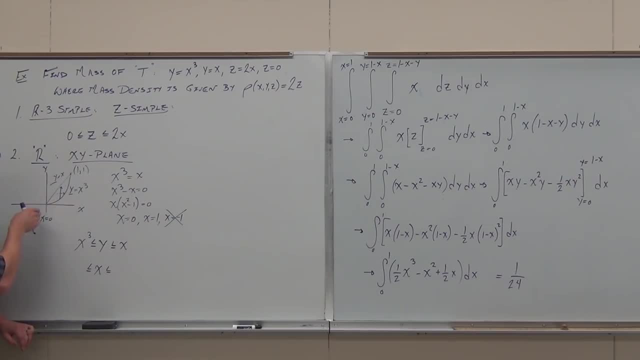 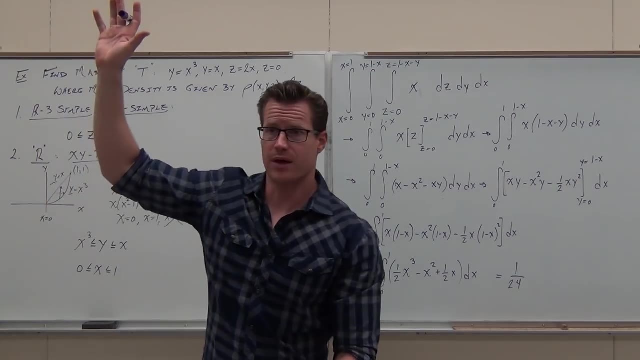 Zero, Zero. It's why you write the point here, so you know to go from point to point, but only along one final axis. zero to one Show: the fans. you've got to understand the concept for that one. That's a big deal. 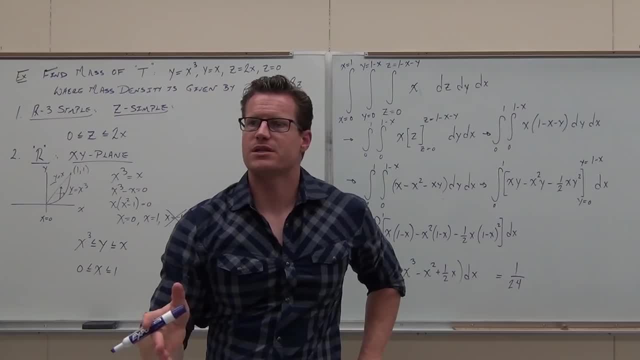 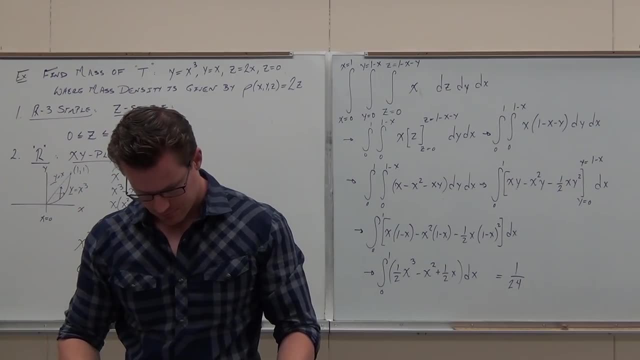 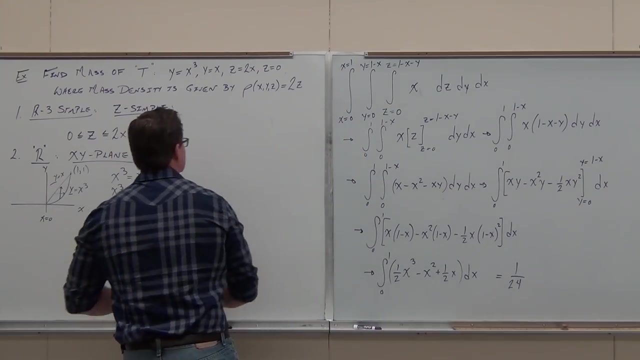 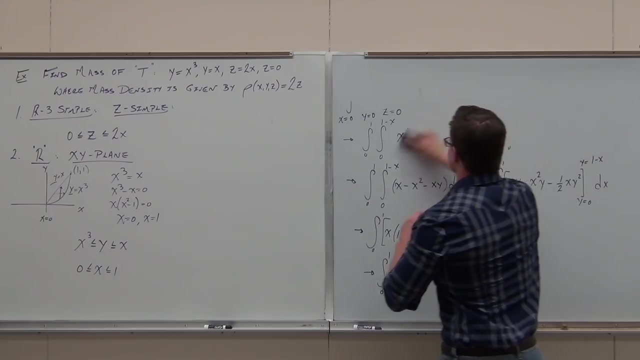 I want you to try right now, take about 30 seconds, and I want you to set up the triple integral. See what you've done. Do you understand? Yes, So then we've got our first part and then we've got our second part. 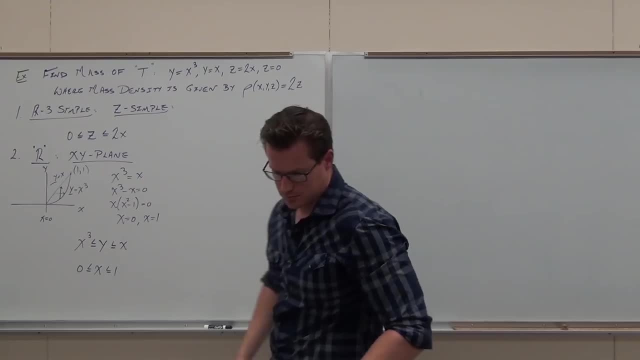 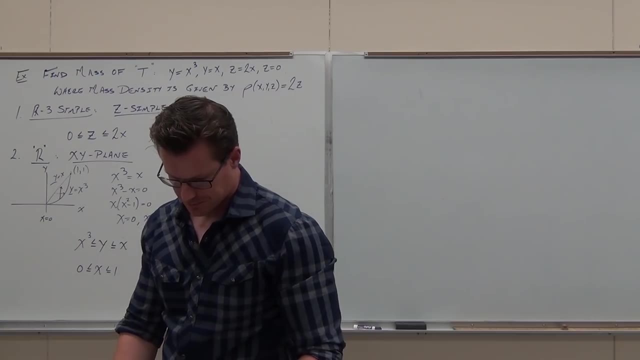 So every 3,, 4,, 5,, 6,, 7,, 8,, 9,, 10,, 11,, 12,, 13,, 14,, 15,, 16,, 17,, 18,, 19, 20.. 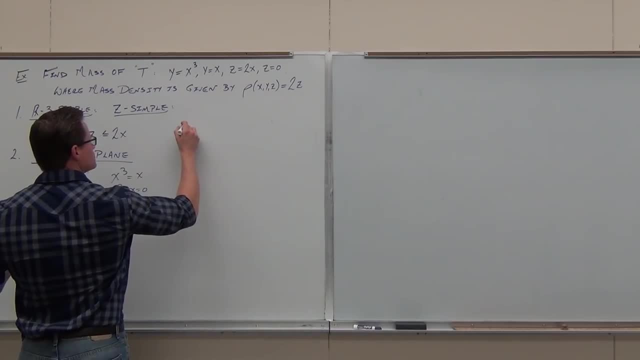 I've got this one, but I'm going to give you another example. So this is number, in this case Number three, Number three, Number 3.. Number 4.. Number 5.. Number 6.. Number 7.. Number 4.. 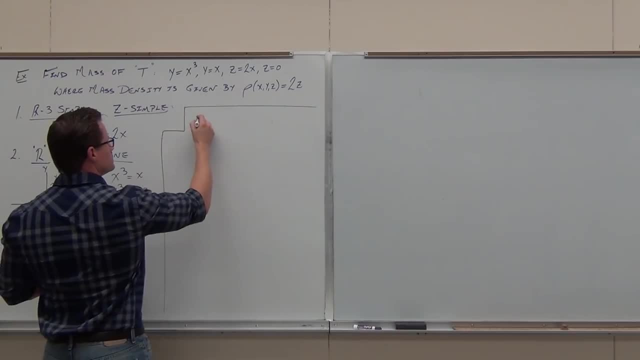 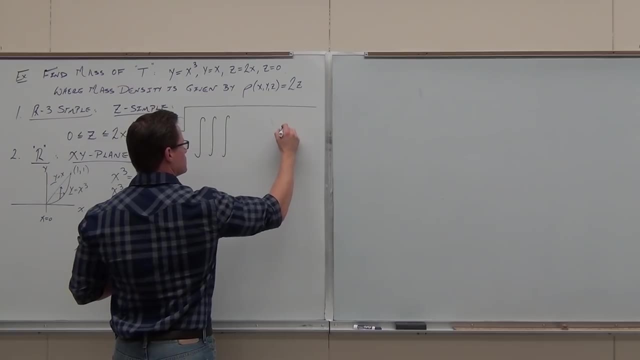 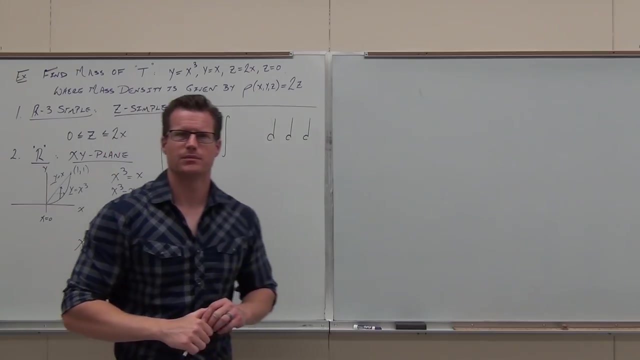 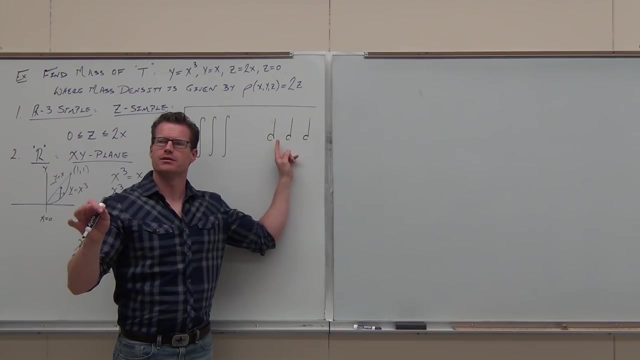 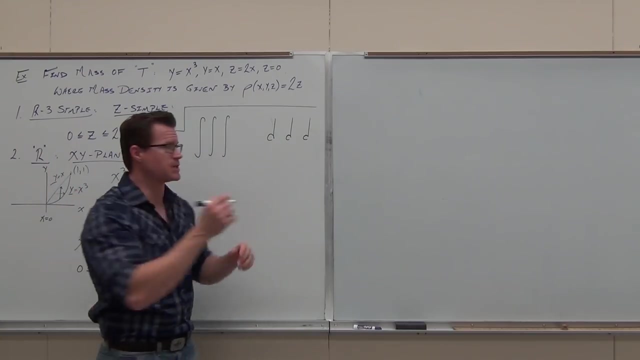 Number 6.. Did you get to it, At least the setup? Yeah, What's the first? what's the first? D, what should we have? D, Y, Y, D, Z, R, simple, R, simple with Z simple along the Z axis. first, between two functions of Z, Z, simple. 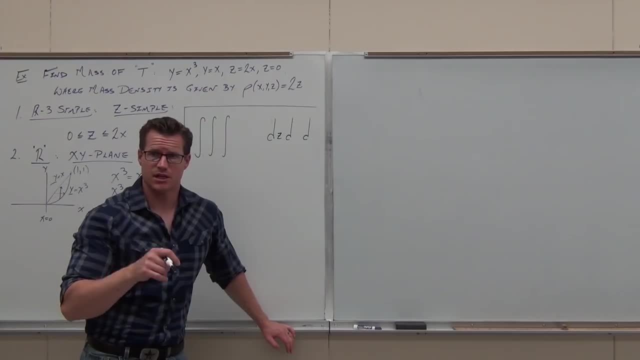 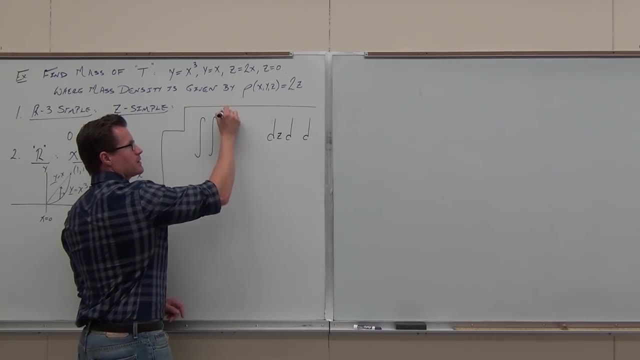 I hope you recognize the way that touchy double integral still stands. You do the setup first, then you worry about the functions. All about the setup. If I do Z, then I match up the variable here, and here Z equals hey, what's the bottom? 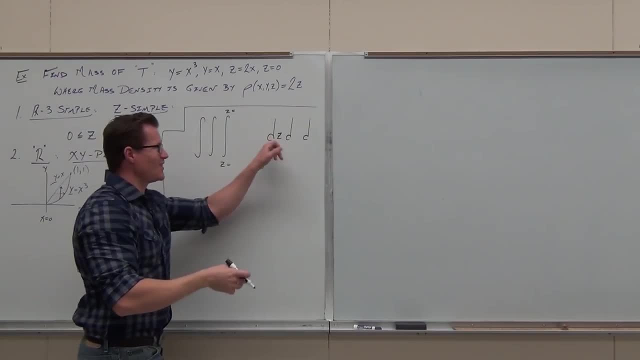 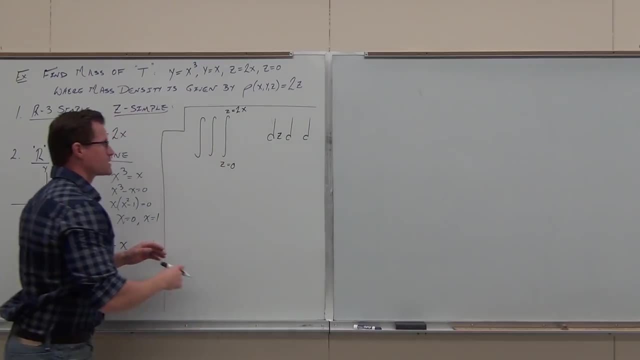 Zero. That's why we write it this way. It makes it so nice. You go along the Z. That's where I'm going along. the Z Zero to 2X, That's pretty painless. Then we go: okay, well, what's the next one? I went along. 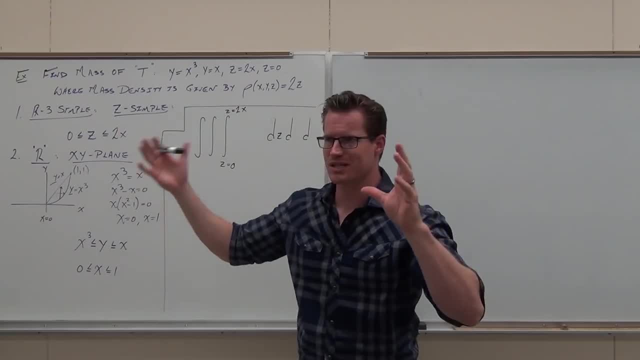 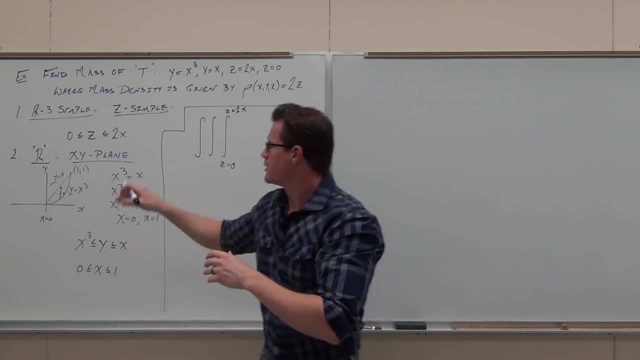 That's where you look at your region. You don't have to draw a 3D region to do Z simple or X simple or R3 simple in general. You just got to know what variable you want to solve, for That's practically it. 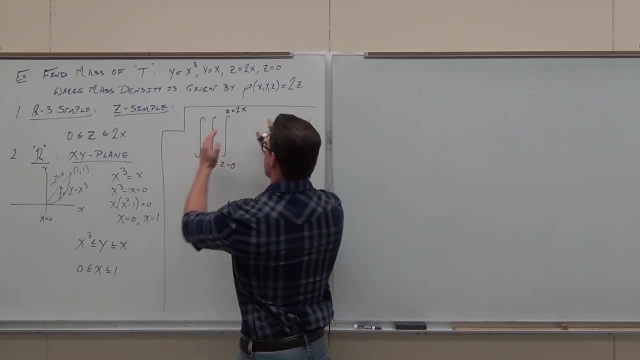 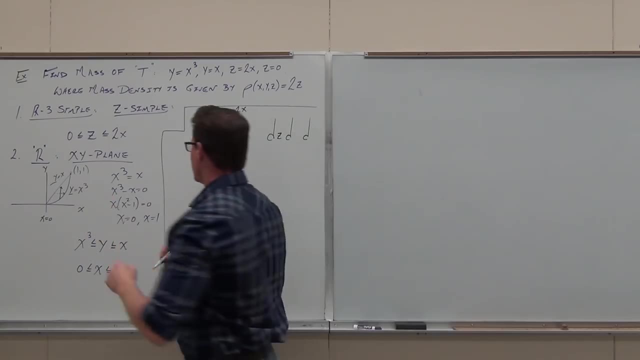 You do draw your R and this gives you everything else you need to know for the double integral that we're left with. We went along what axis after the Z? So we went Z first, Then we went R, Then we went along the Y. 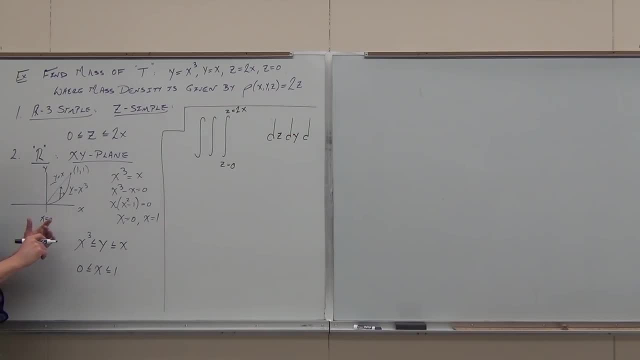 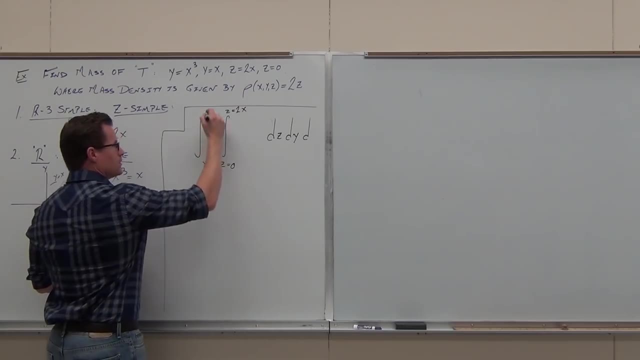 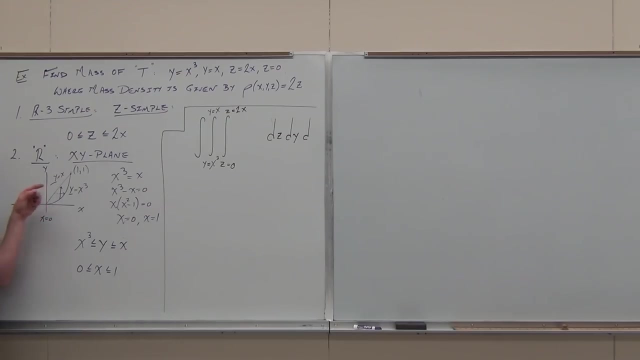 And we went so along the Y. We went between two functions of Y, It's Y. we write them down: Y equals 2X. And lastly, the dotted line said we went along the X axis, That's DX. 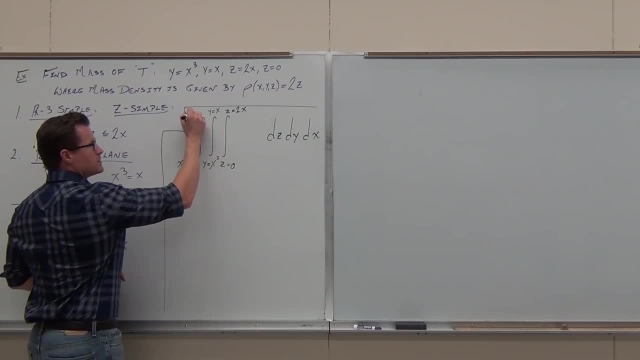 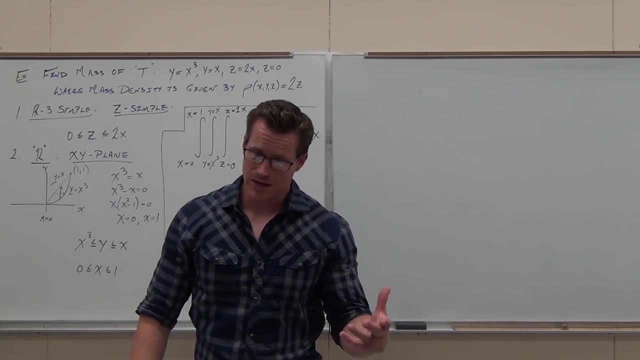 That says we went from X equals zero to X equals one. Did you get the same set up? That's fantastic, That's man, you. it's integration after this, which, yeah, you can screw it up, But honestly, that that lends itself to a really successful test question. 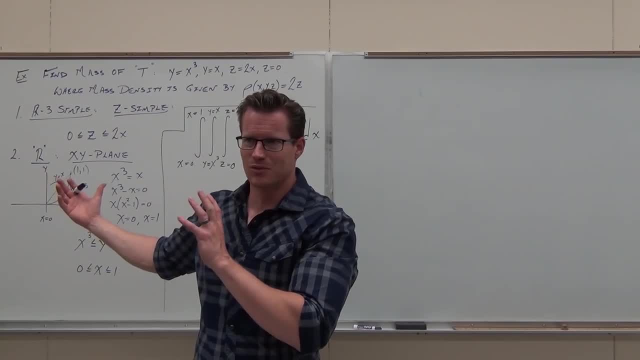 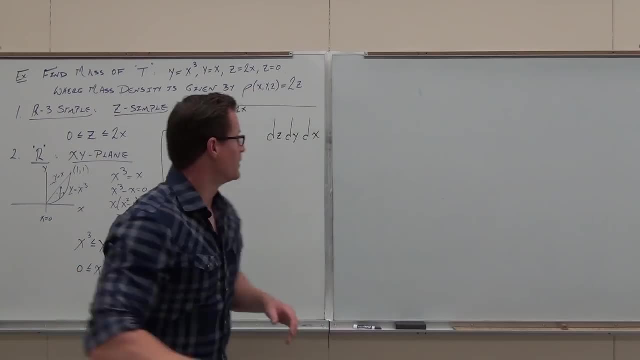 Well, if you, if you, if you complete one more, one more thing, There's one thing that we've left out: Yeah, the mass density function. So don't forget that. Yeah, there's one way you can screw it up. 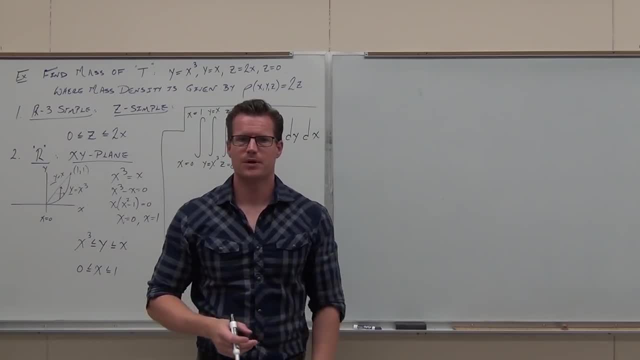 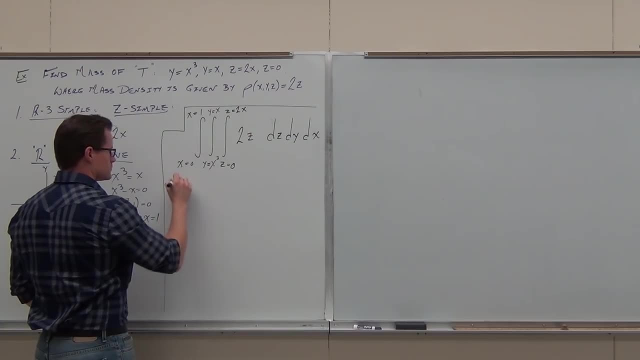 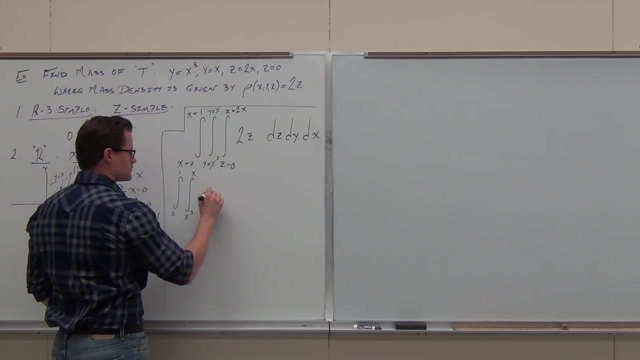 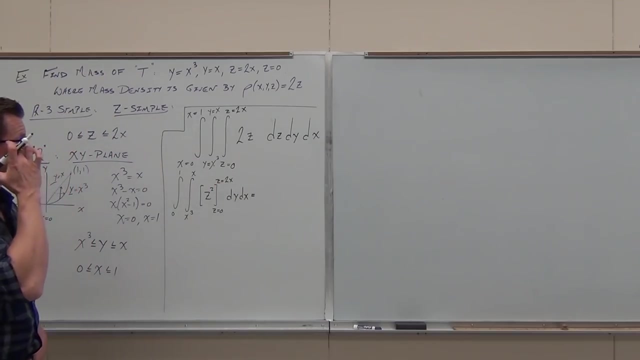 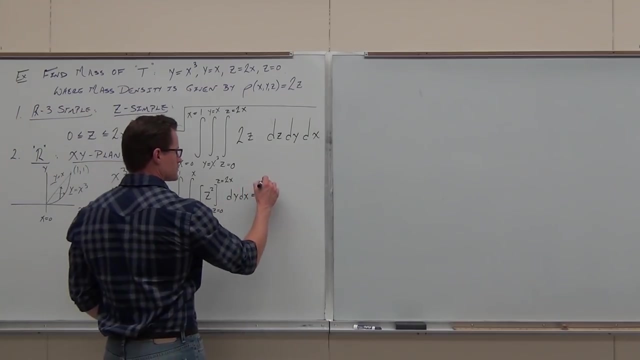 Now can you work on it? Why don't you try it? I'm going to put up a step about every 10 seconds. Let's see if you get the same thing. Okay, here we go. Okay, here we go, And. 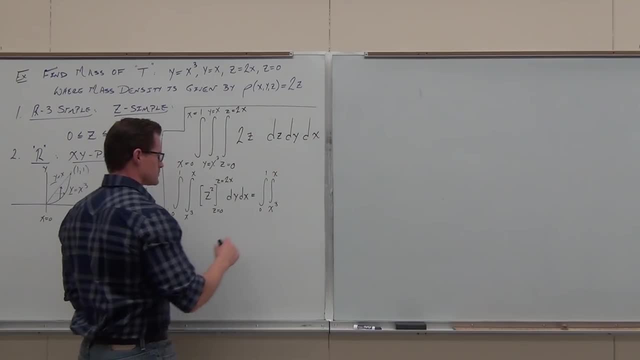 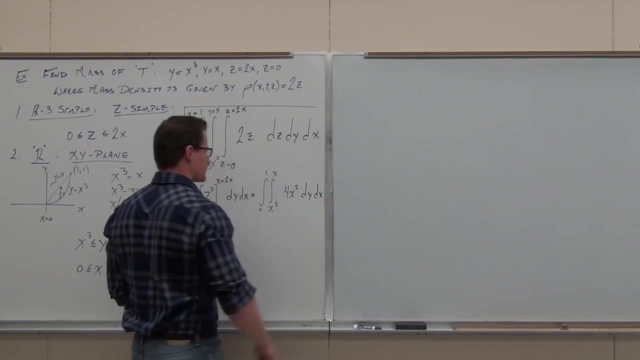 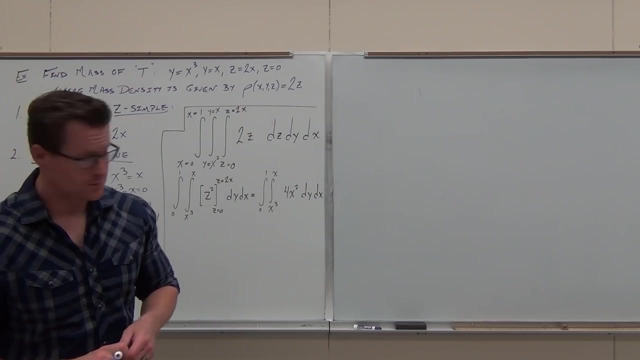 Yeah, I mean it should work. So what I've got, I've got not really got an answer. so I'm going to say: don't worry about that, That's it. Okay, There we go. Thank you, All right. 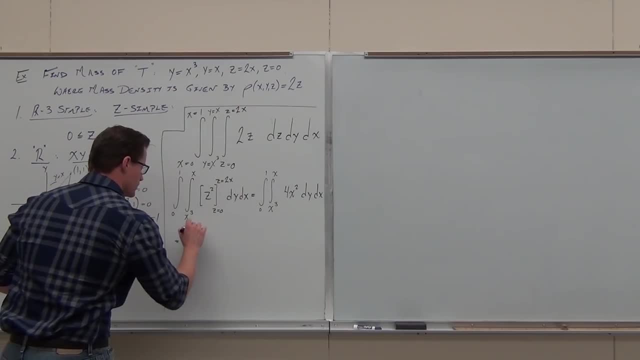 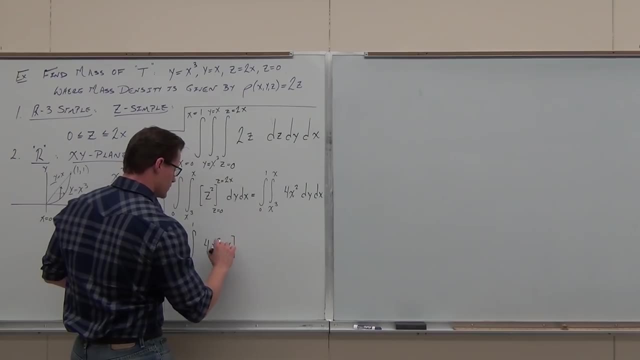 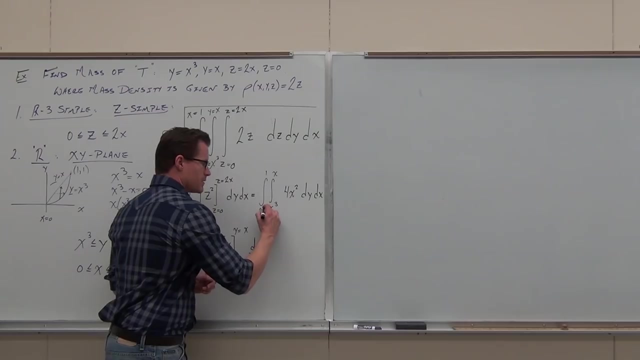 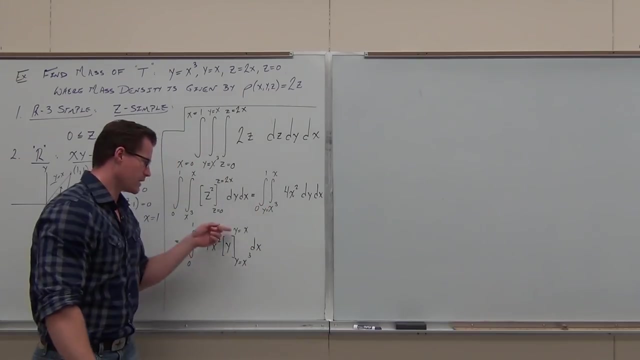 You know I've been doing this a long time but I still write y equals here sometimes just to make sure I know I'm not messing with the wrong variable. I still do that. I still write it here just to make sure that I have everything in line. 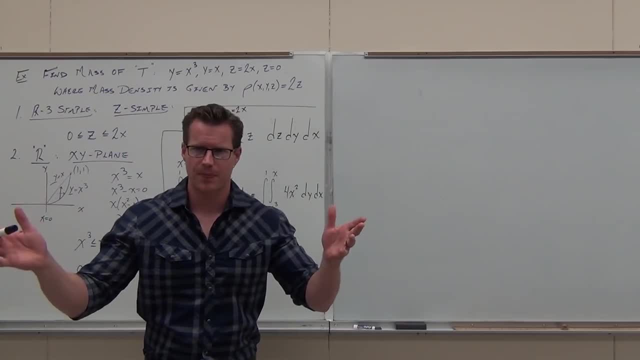 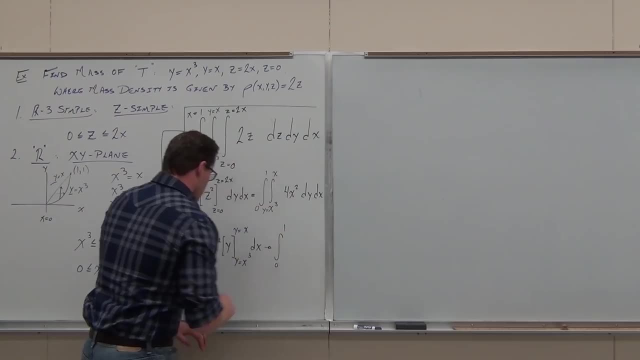 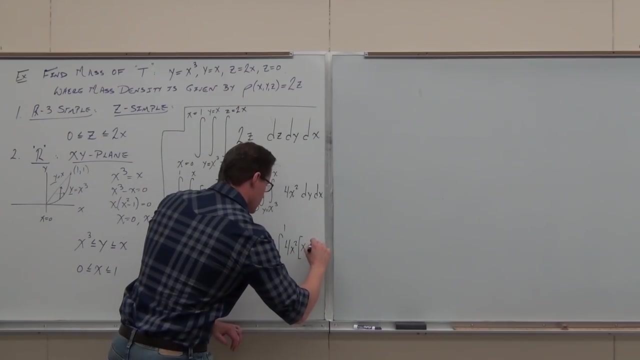 It's just good practice. It's good practice Even if you guys are really smart. you are really smart If you know what you're doing. still write it. It's too easy to make mistakes here. That's an X, Sorry. 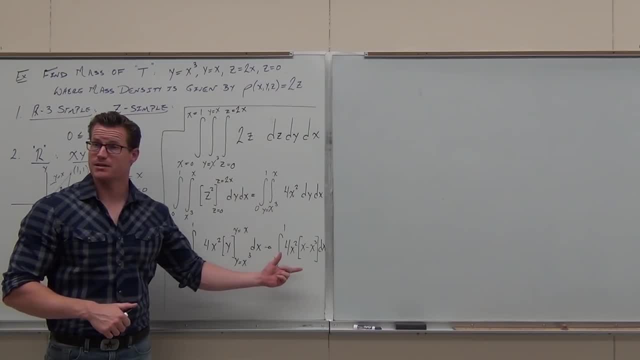 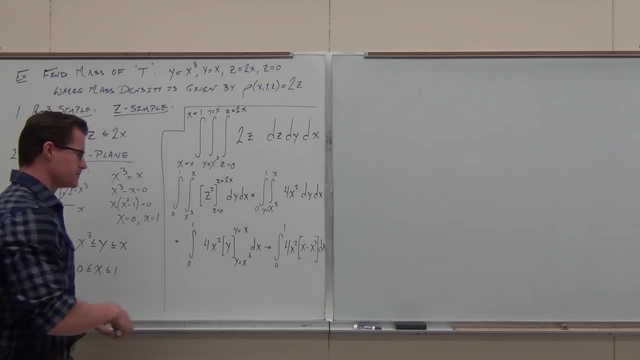 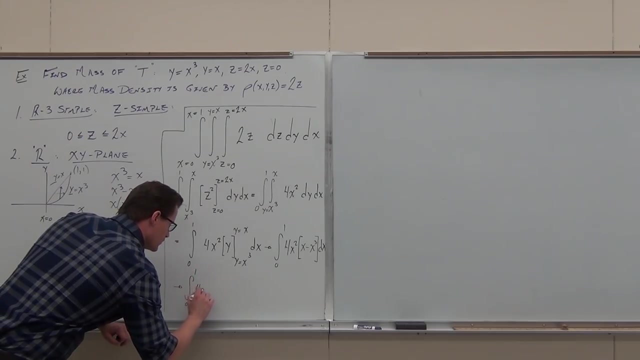 Did you make it that far with the 4X squared and the X minus X cubed? It's got to be that order. Did you get the X minus X cubed? What would your next step be? Keep on going. 1, 2, 3, 4,, 5,, 6,, 7,, 8, 9,, 10,, 12,, 11,, 12,, 13,, 14,, 15,, 16,, 18,, 19,, 20,, 21,, 22,, 23,, 24,, 25,, 26,, 27,, 28,, 29,, 30,, 32,, 33,, 34,, 35,, 37,, 38,, 38,, 39,, 40,, 42,. marriage of kids. love is recipe. 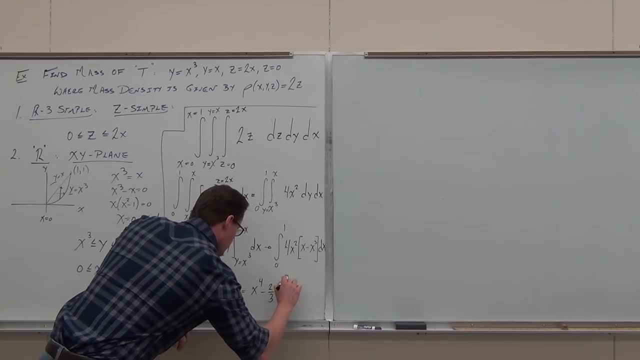 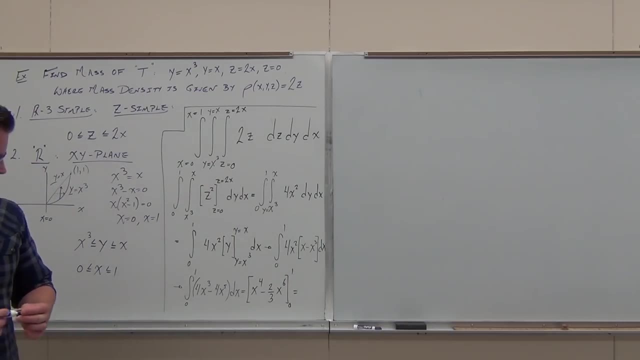 Very easy, That's going to be good. Very easy to master, Absolutely easy to master: marijuana b immorality, no control. divorce is Qin ailed to tetrapalpy right toI nf a problem with promising of benefits to money dear. 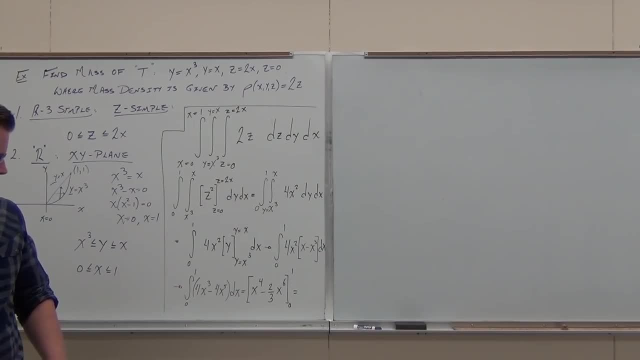 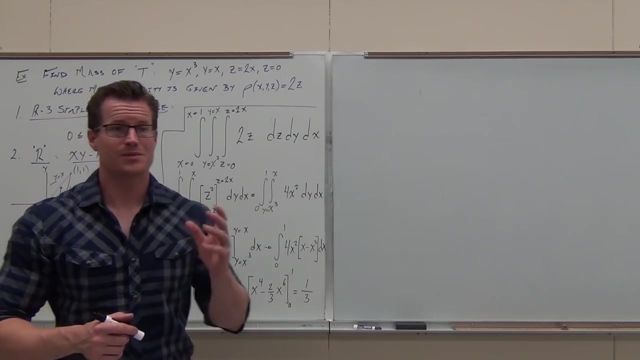 discipline, trans, educate ethical PP and resign the ay ex. see you, potsy, Did you get one-third Yes? What's it mean? It's the mass, Since this literally is the mass density function of this three-dimensional region. this thing with volume. 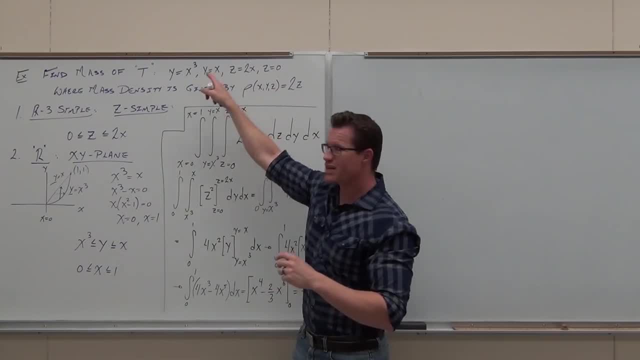 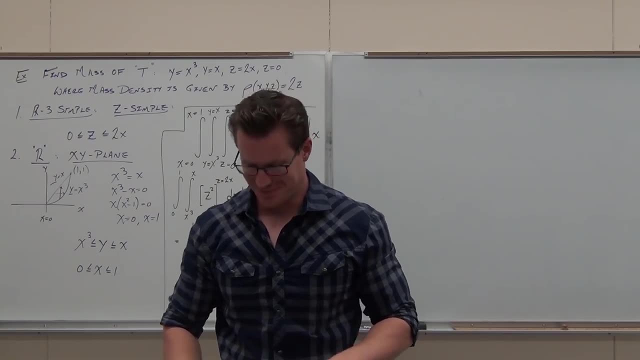 this three space. the mass of this region is one-third, whatever units, It's kind of cool, right? Kind of cool. Tell you what we're going to do: one more and then we're going to call it good for today. 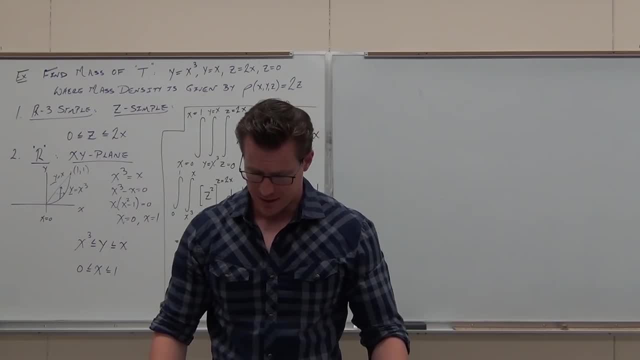 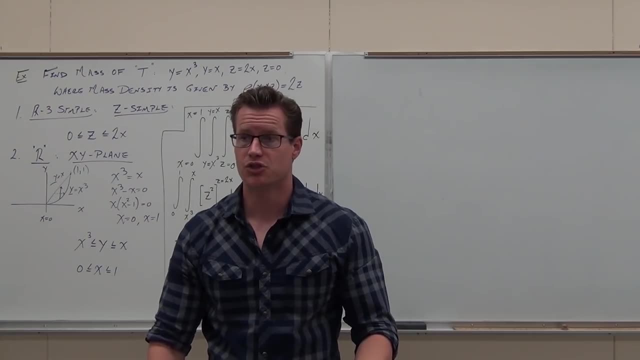 I need to make this connection for you before we leave. I've got to have you know this. After that, you can probably do most of the homework. There's some other ones that we're going to practice with some just crazy setups, just so we can set them up. 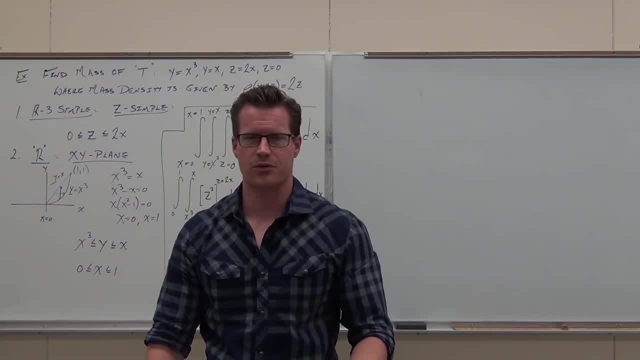 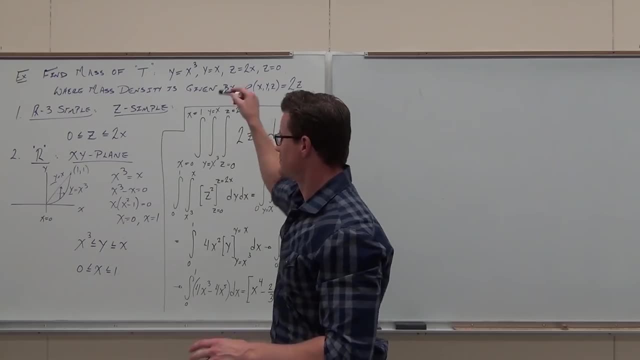 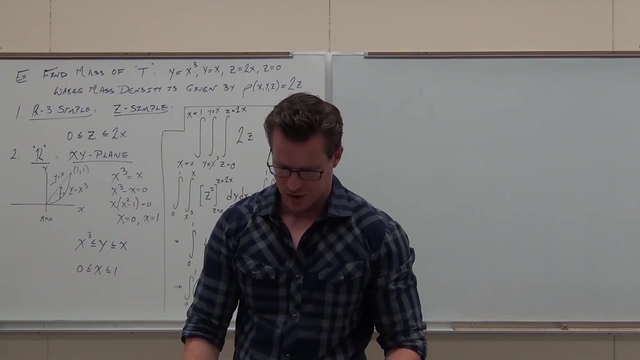 But as far as the idea of triple integrals, we're almost about through with triple integrals. the way we do them, It's nice because they're very similar double integrals. just we need the R3 sample. So last one we're going to do and then we'll stop for now. 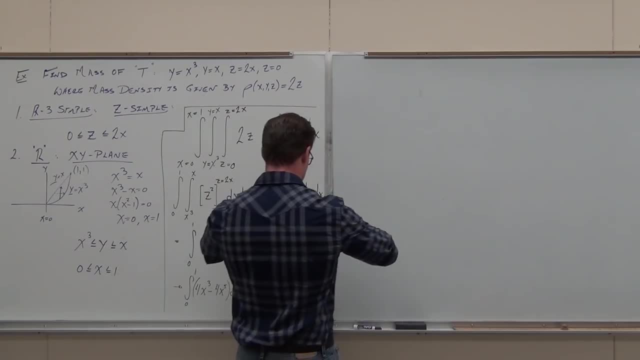 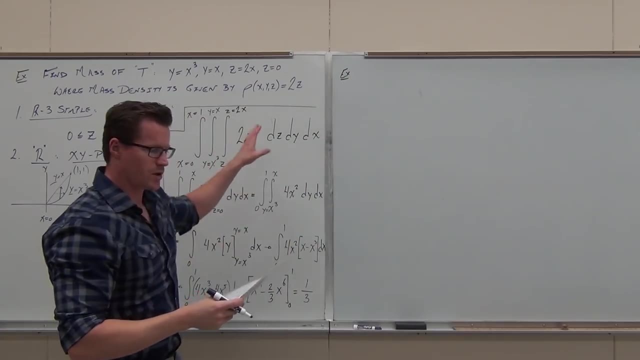 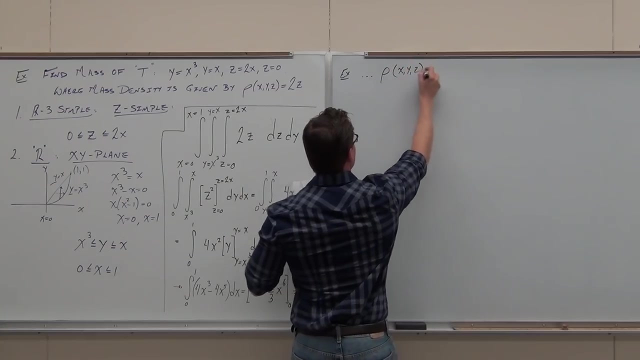 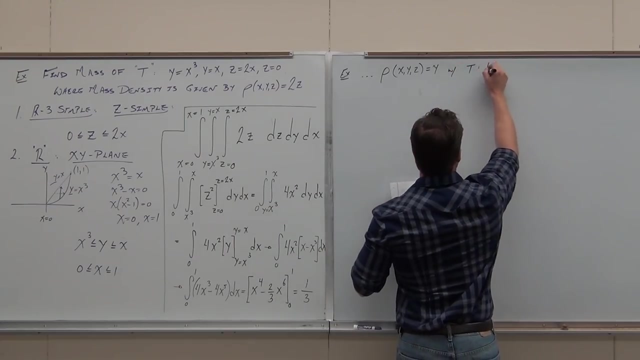 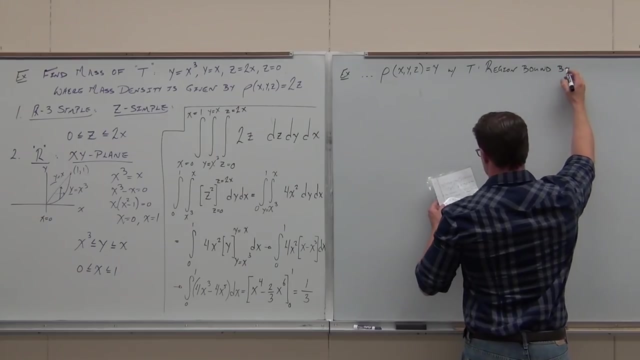 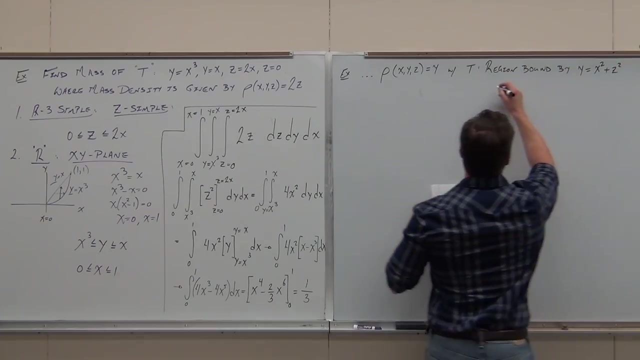 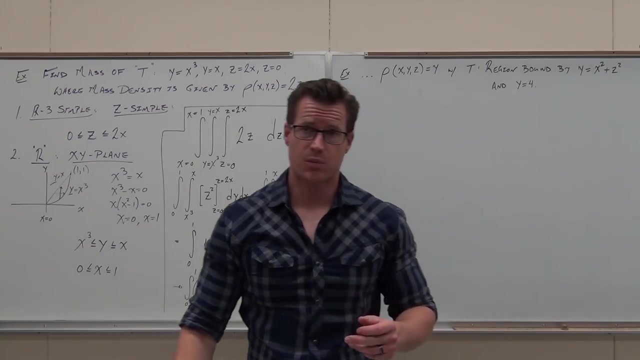 come back and do some setups and see what we can do next. So same question as before. All right, But this is important. This is a good one, Man. I hope I haven't bored you enough that you are not paying attention any longer. 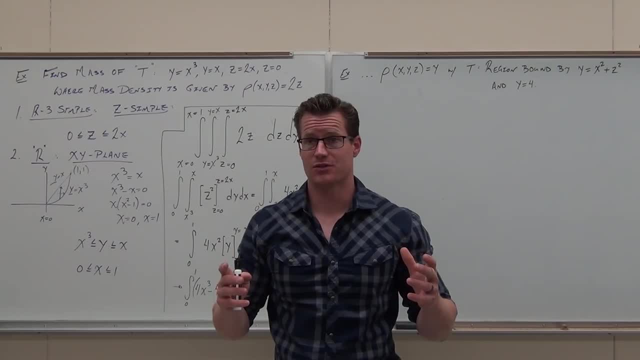 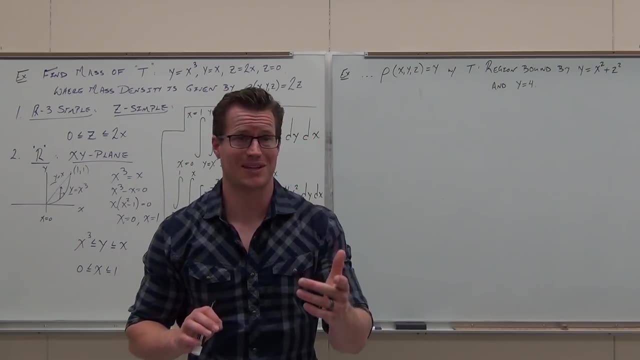 because what this is going to do, this is going to make a connection for your next section. I'm going to kind of prove- well, not really prove, but show you something here that should be really interesting. It's going to be so cool. 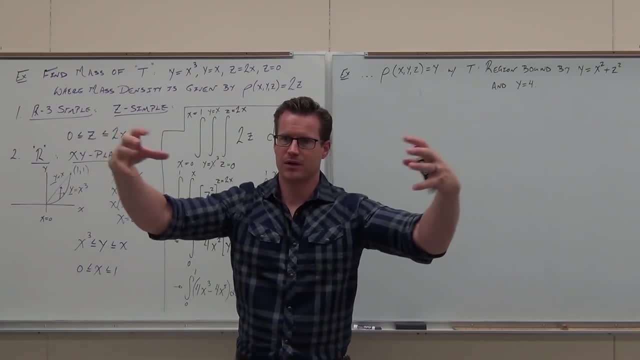 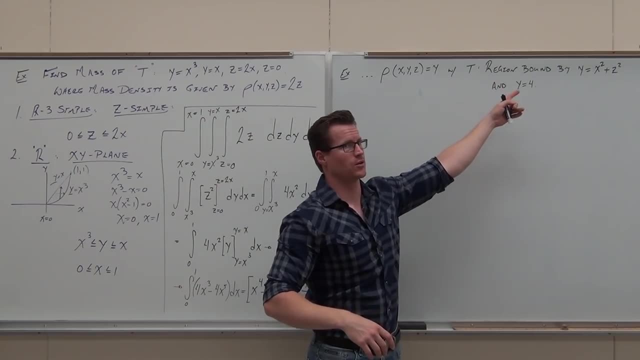 You guys ready for it? I'm going to connect all of chapter 14 that we've done so far. It's all going to get connected. We're talking. We're talking mass, We're talking. We're talking double integrals. 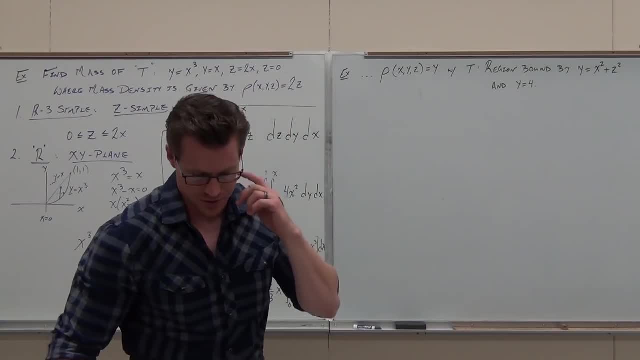 We're talking how to switch these things, We're talking triple integrals, So the whole thing is going to come together in this problem and then we're going to run with that. So, number one, the first thing that you do, first thing you do for any triple integral is what? 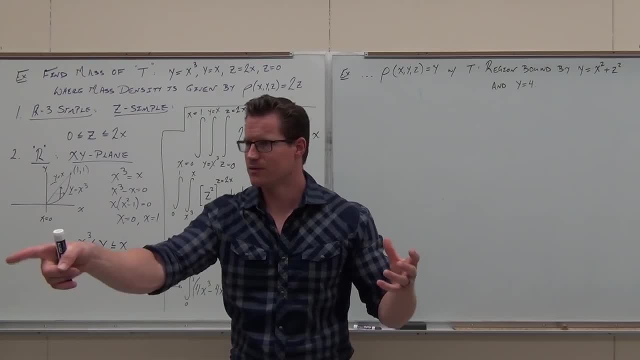 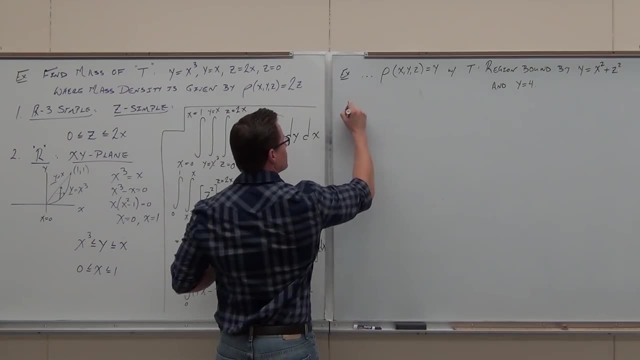 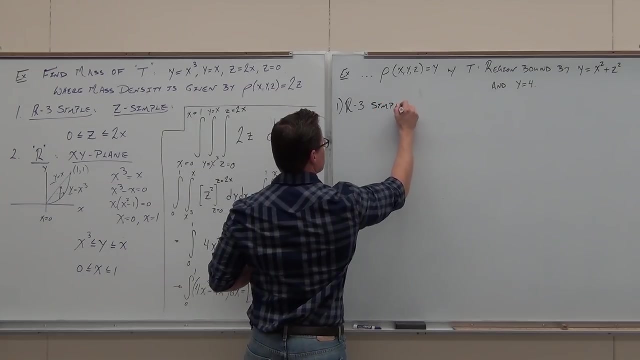 Say the? oh, I heard it was, I'm sorry. What now? R3 simple, R3 simple. Yes, Let's do the R3 simple. Let's write that down. Write down R3 simple. Organization is pretty key here. 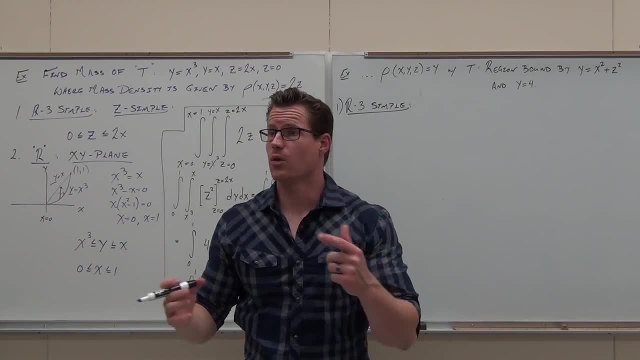 You don't want to get disorganized, You're going to lose some stuff. Don't lose your stuff. So R3, simple. What Now? what would you choose? Would you choose to do Z simple, Y simple, X simple? 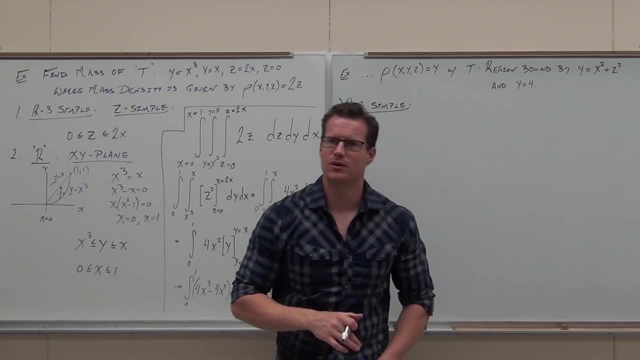 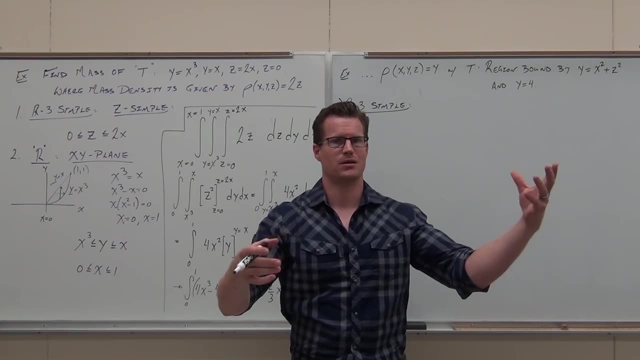 What would you choose? Y, simple, Y. Why would you choose Y simple? Look at what it's solved for. That makes it so nice. If it's solved for two functions of Y, already man choose Y simple. This is one of those cases. 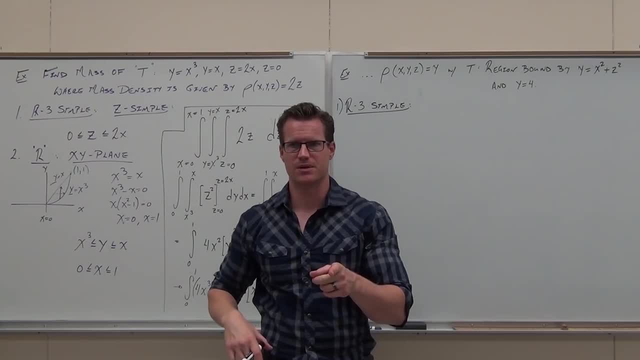 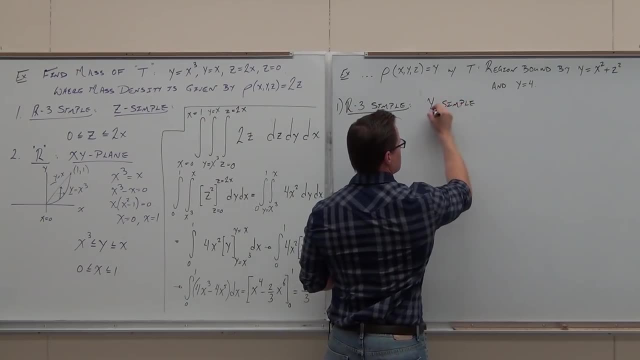 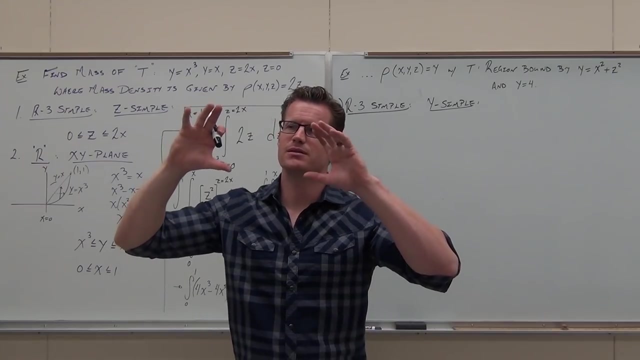 where you wouldn't have Z simple and it would not be logical to solve for it. Does that make sense? It'd be hard. So here for sure, Y simple Head nod if you're okay with that one. Now, what that means is that's our most inside integral. 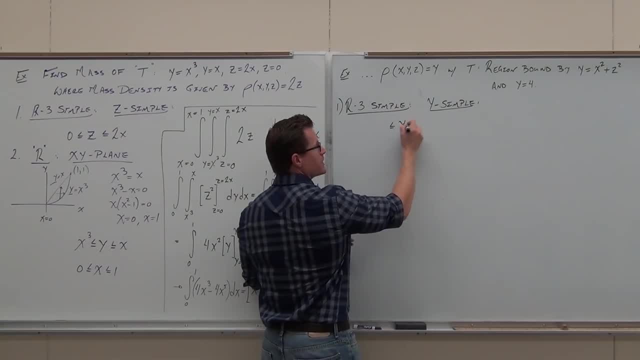 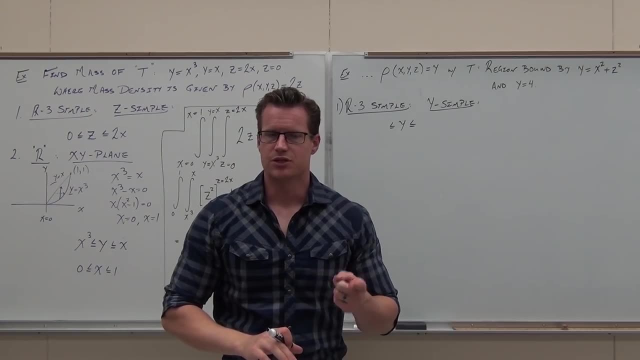 That means that we're going to have to get something Y between two functions. Are you guys okay with what I'm talking about? Well, what that means is you need to know what the bigger one is and what the smaller one is. Now, a lot of times, it's really easy to see. 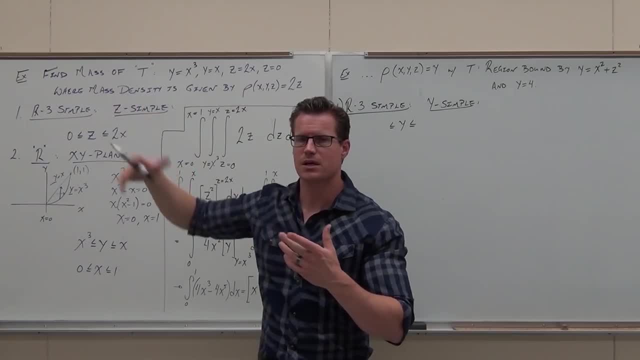 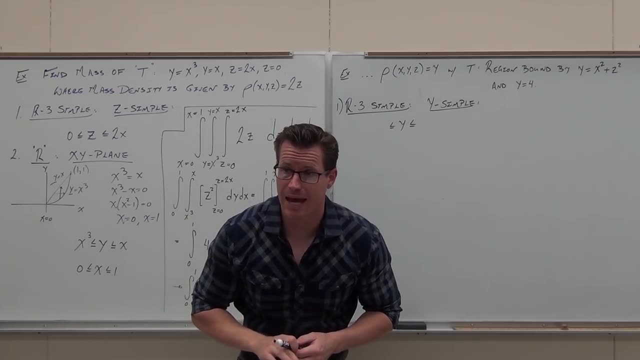 If you have a zero, you're probably climbing. Yeah, that makes sense. But if you don't have that zero, you might have to think intuitively, or you might have to wait for just half a second until you draw your R. I'm going to show you both ways. 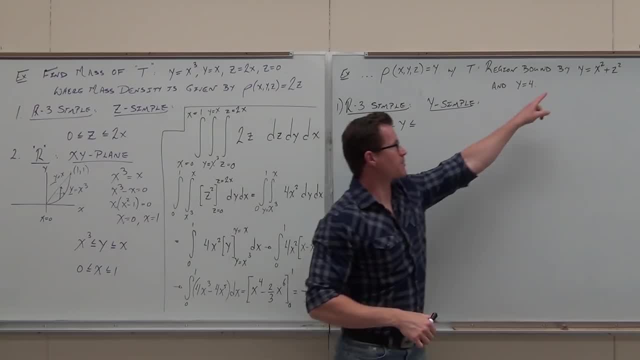 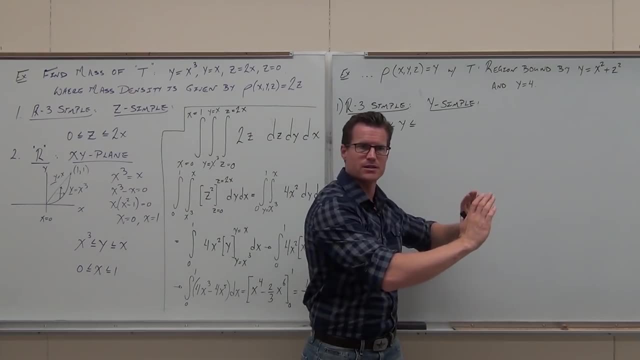 Intuitively speaking, that right there is a paraboloid. That paraboloid is traveling along the Y axis. Do you see it? Origin along the Y axis. If you learned anything about your surfaces- some of you- it's doing this. 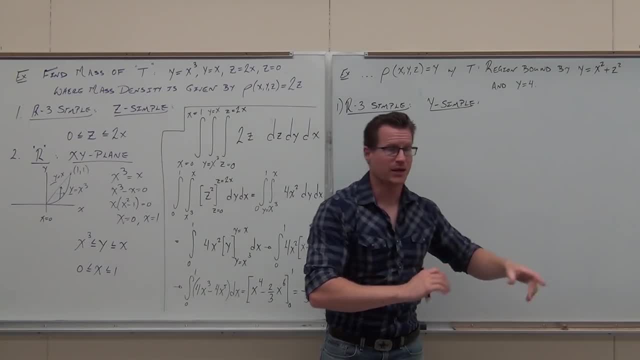 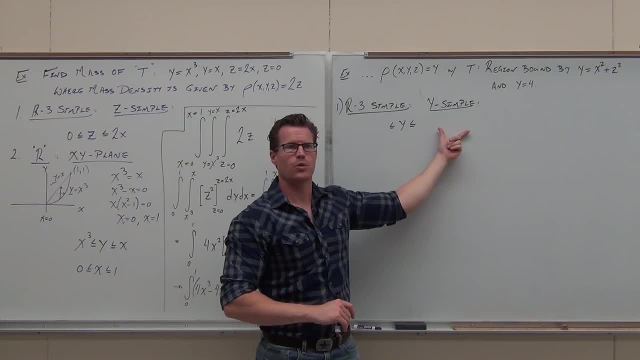 That's a plane. It's going like this until it hits the plane That is the small one, For sure. I know that that's going to be X squared plus Z squared and 4.. If that works for you, awesome. If you're like, I don't know what that is. 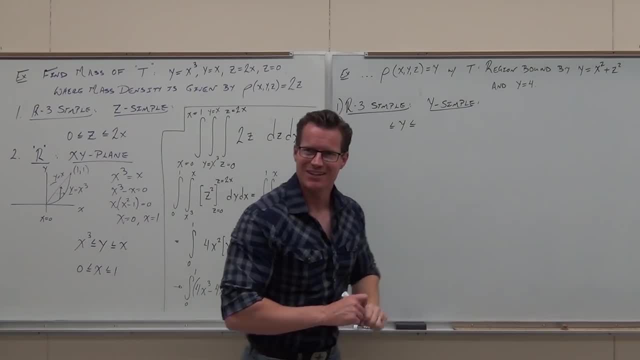 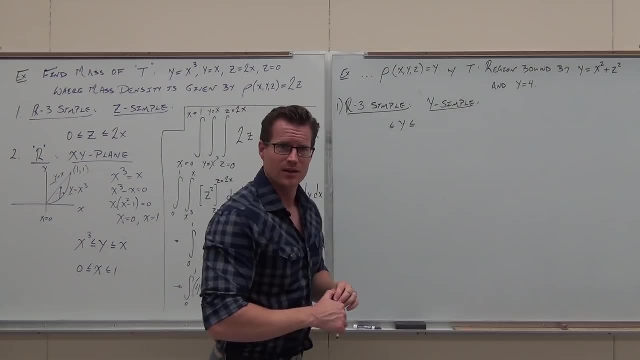 You just talked about it. then you wait and you go, okay, okay, Well, you're not speaking my language. Here's the other language. If that was Greek, then this is Roman English. What are we speaking now? You should translate. 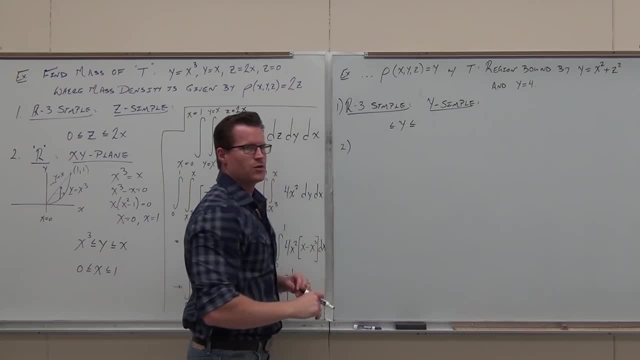 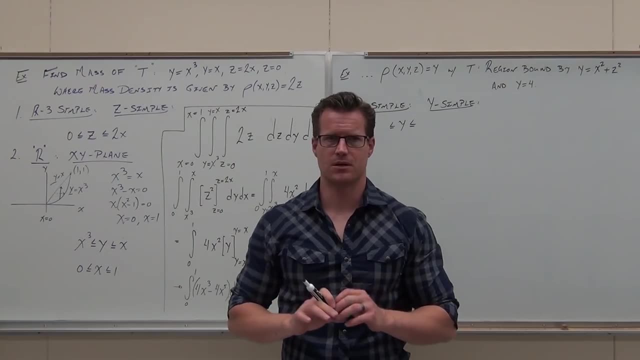 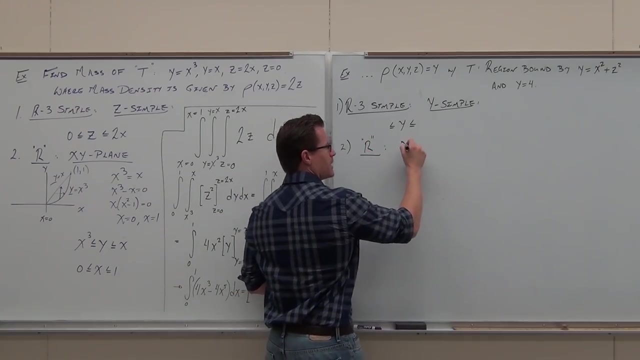 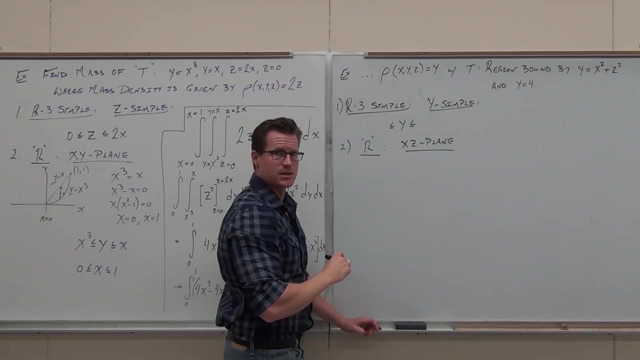 All right, If you have chosen Y, simple, where will the region for your double integral have to be? on What coordinate plane? So the R is going to be on the XZ plane. Right now you should be drawing me the XZ plane. from what I told you earlier. 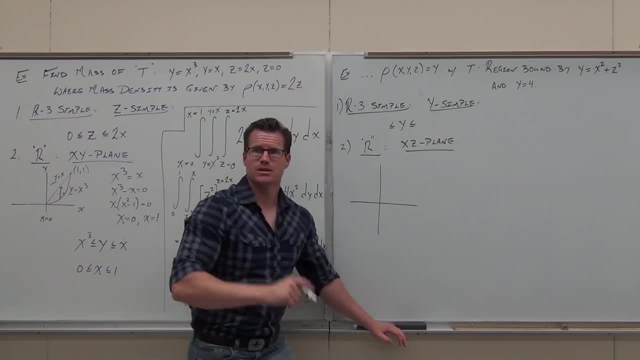 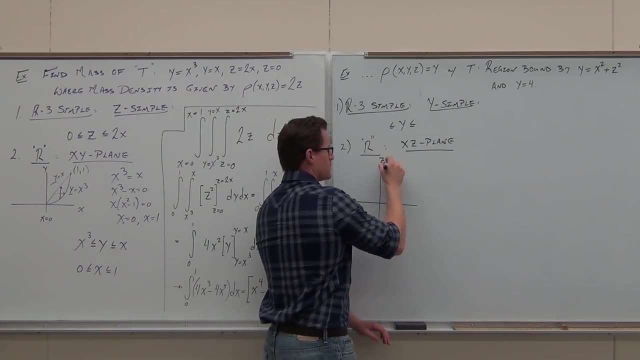 If you have a Z in it, it's always the vertical. X and Y are always the one of those is the horizontal. okay, So this is Z, this is X. You're on the XZ plane. Does that make sense to you? 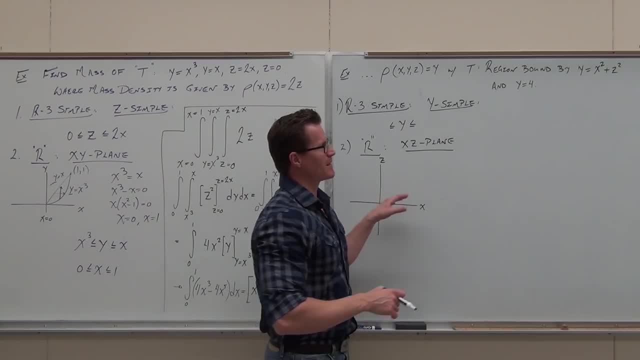 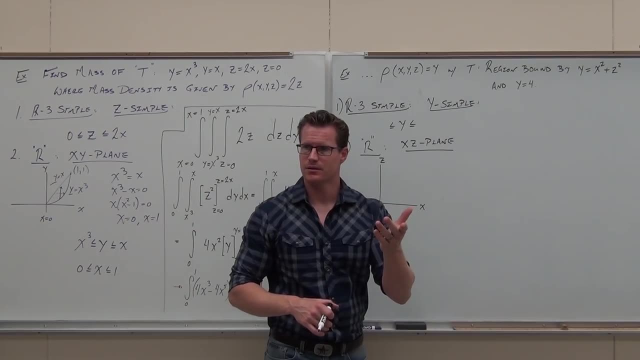 Now, how about this? How about this? On the XZ plane. on the XZ plane. on the XZ plane Y has a value of what? No, on the XZ plane, on a coordinate plane. on the XZ plane Y has a value of what? 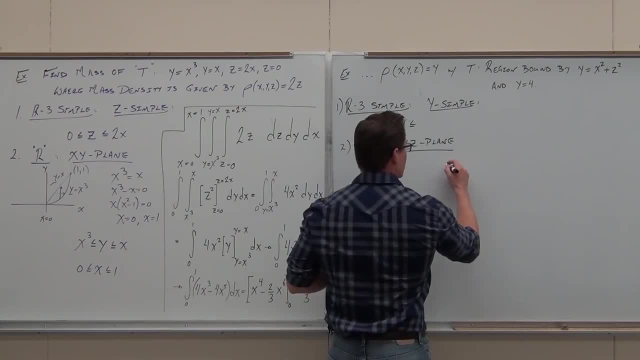 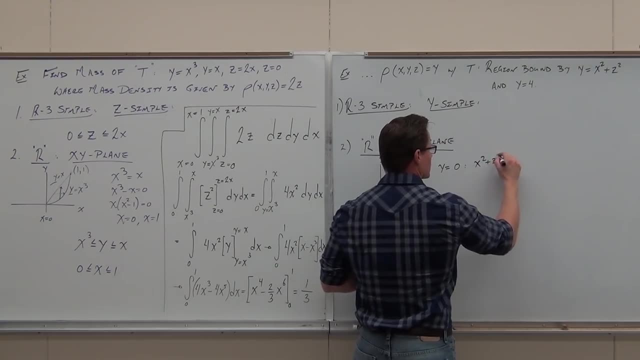 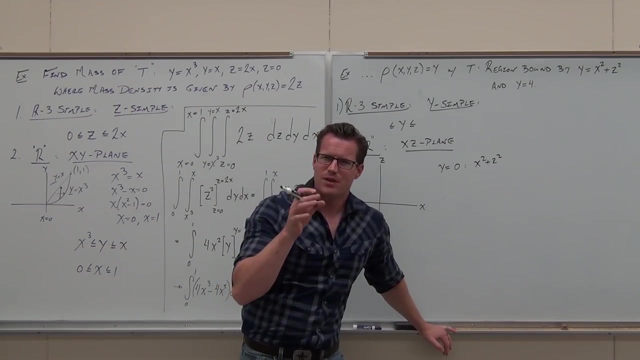 Zero. Okay, If I did that, though, would that give you anything? No, This goes back to that one idea. when you find your region, Do you remember that you do the intersection of your surfaces, and it creates for you a new region? 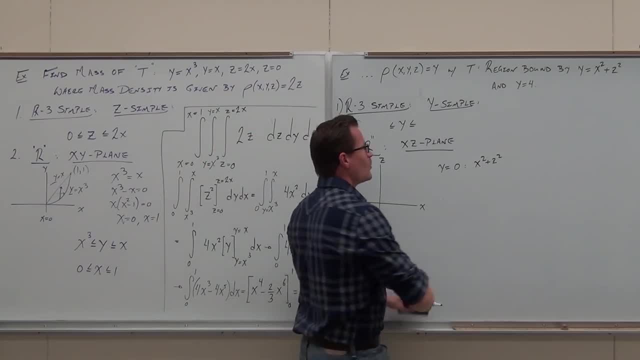 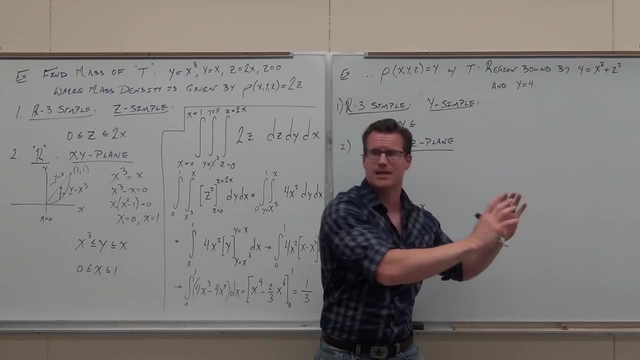 It's a level curve. Do you remember that? You go, hey, where do these things intersect? Well, these things intersect. We talked about it. That's a paraboloid doing this, That's a plane doing this. They will intersect. 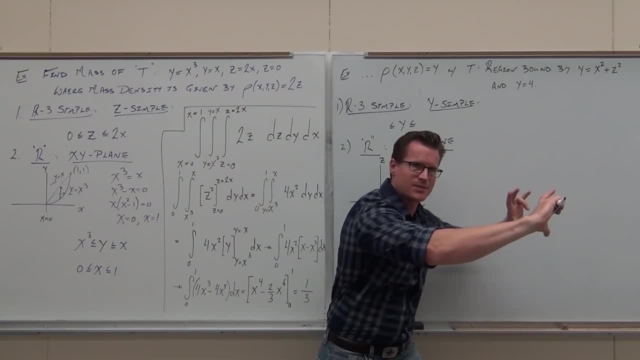 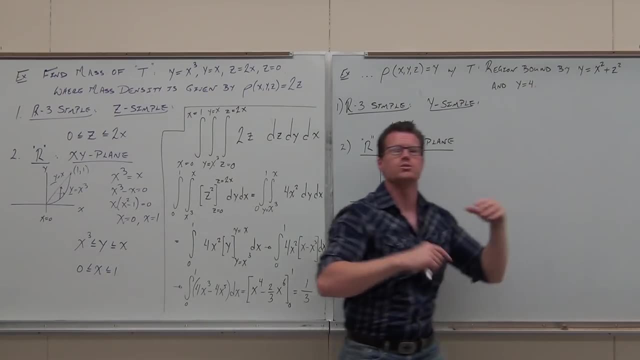 It's going to be a circle and that circle has a projection as a level curve onto the XZ plane. Does that make sense? So you don't just get to plug in zero for this all the time. You do find where to intersect. 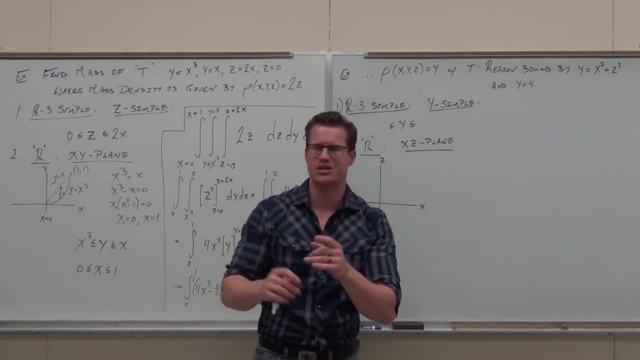 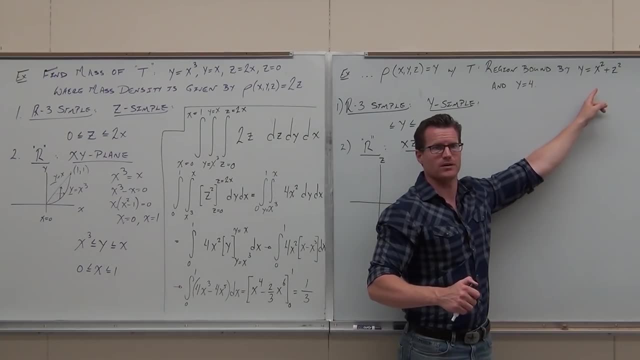 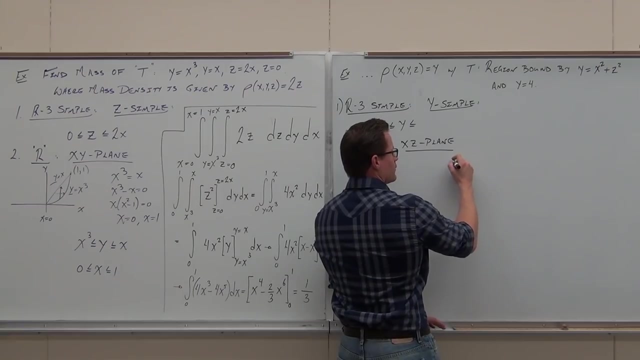 You do find the level curve over the intersect That creates your region. It's just like any of the double integral. It says, hey, Can you tell me where those two things intersect? Yes, Where, When they equal each other. Okay, Well, at the intersection you go. hey, then, if Y equals 4, 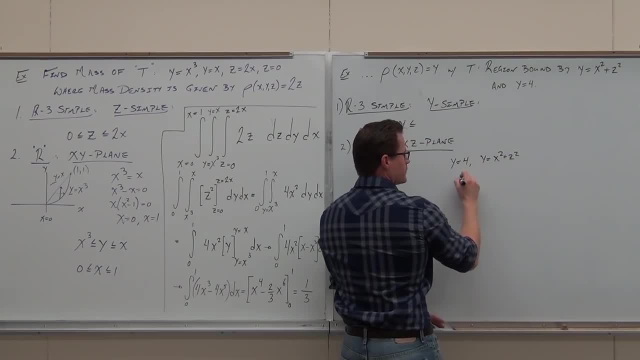 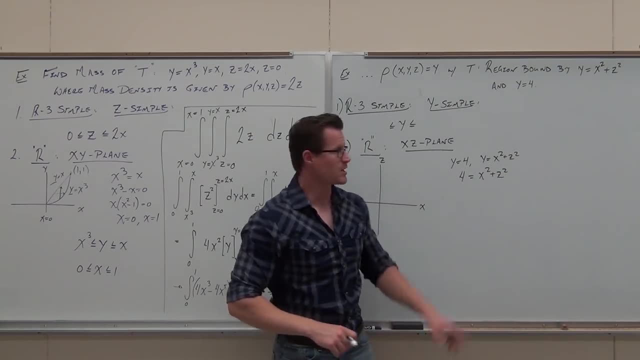 and Y equals X squared plus Z squared, then 4 equals X squared plus Z squared. If you want the common sense approach to doing this, eliminate the variable that you just solved for Y. simple, Just get rid of it. So solve somehow to eliminate that variable. 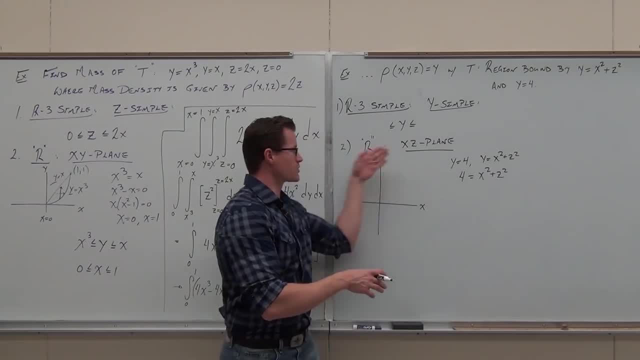 Maybe you should be left alone. Maybe you should be left with just Xs and Zs, or just whatever two variables. you're on on the coordinate plane and not be okay with that one. So what we've done here, we've set them equal. 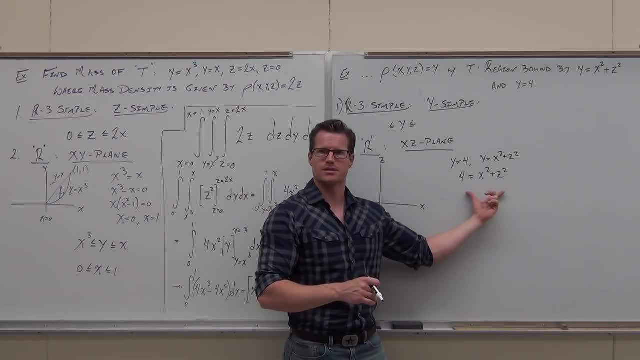 You go: hey, can you now graph this on your XZ plane? Come on, people, Help me out. What's that make on your XZ plane? Circle, Circle, Radius, Circle, Radius of what? 2, 2.. 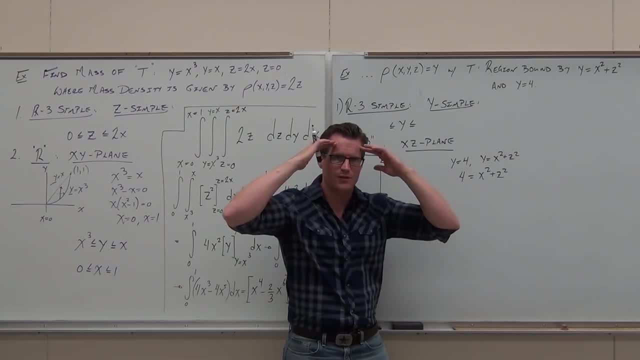 Centered at the Point. Think about the picture. I know if you don't, even if you don't know the picture you're like- I don't know the picture, You can still do it. Set them equal to each other. 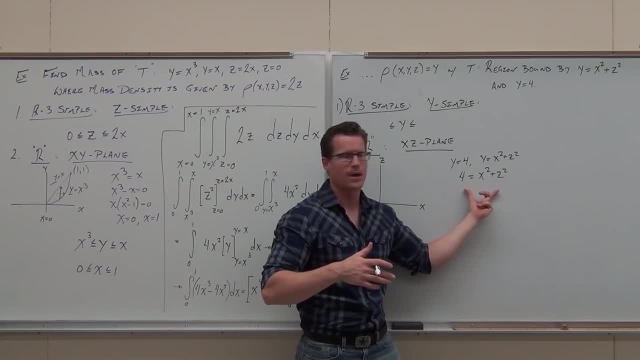 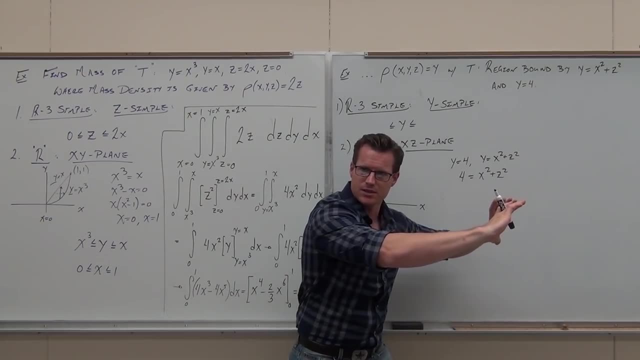 Set those equal to each other. It's going to give you this. You do need to know that's a circle, But that's a paraboloid. It's intersecting a plane, It's making a circle, That circle. listen, listen. I want you to get the concept. 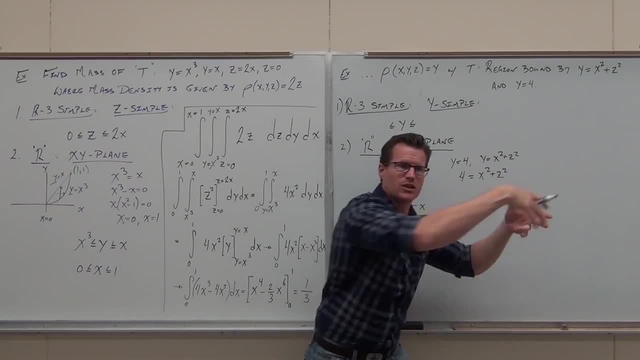 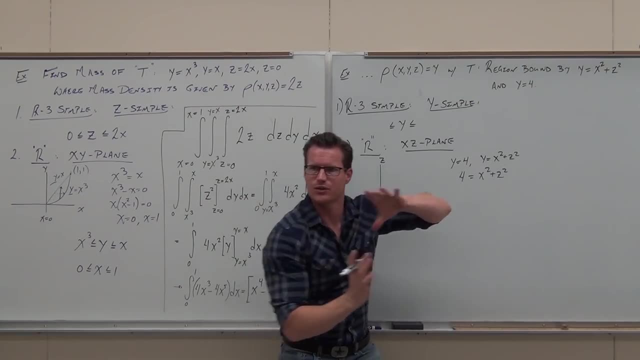 That circle is out in space, but the projection of it, the level curve of it, is on the XZ plane. That's the region, That's the idea of making a cylinder subtracting big volume by a small volume. that's a double integral idea. 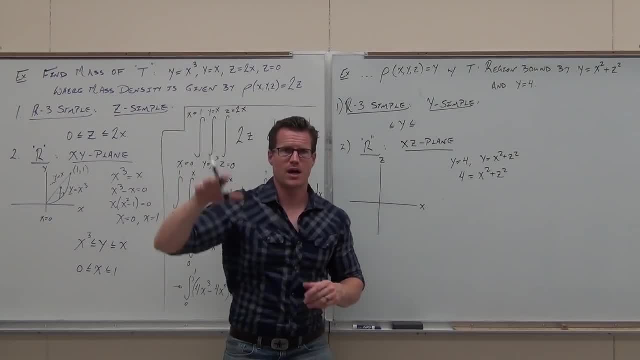 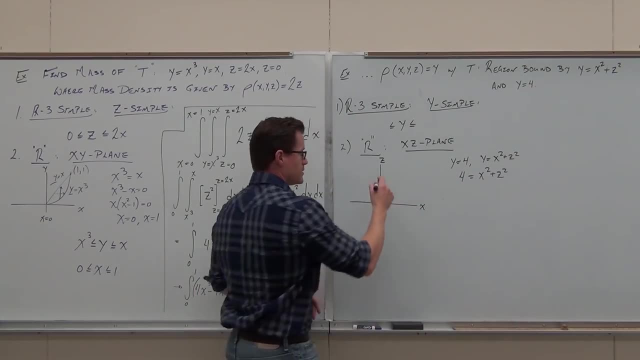 That is what I want you to graph: Show fans, if you know where that's coming from. So if you're not given specific numbers, planes whatever. if you do find the intersection, you draw an appropriate coordinate plane. If I do, then I got this nice little circle. 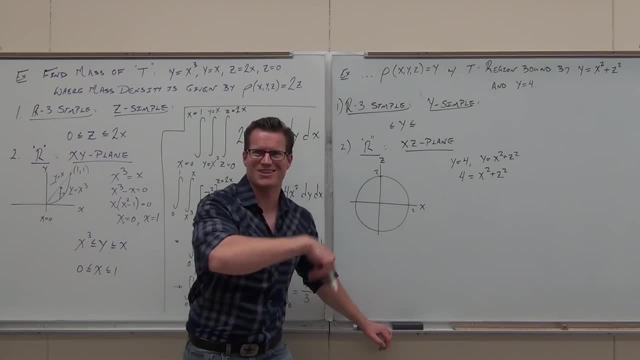 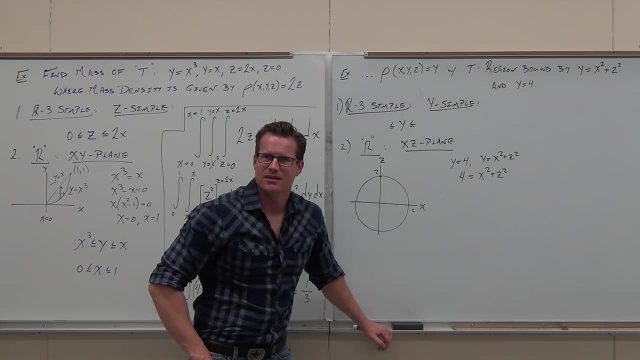 Probably the best circle I've ever drawn. It's on video too. I can draw circles. Whoo, I love drawing circles when they work out good. Let me tell you about that professor. I had that one guy, Drew, perfect circles. 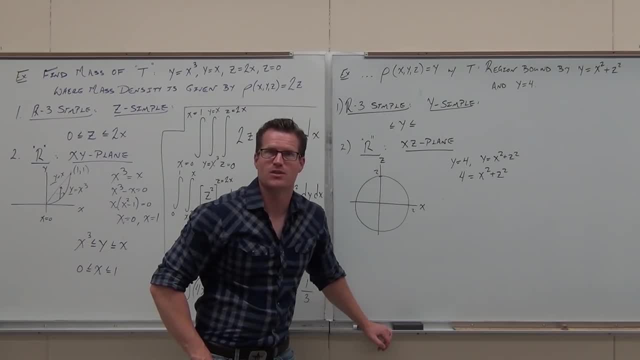 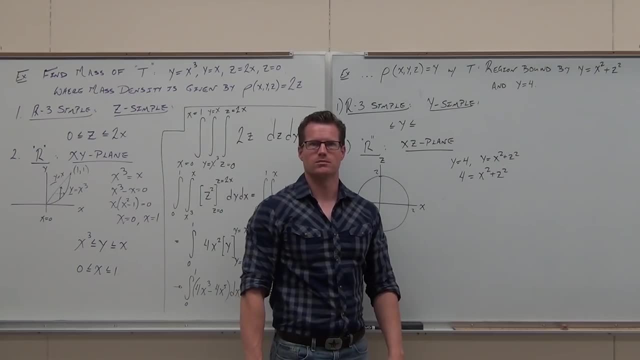 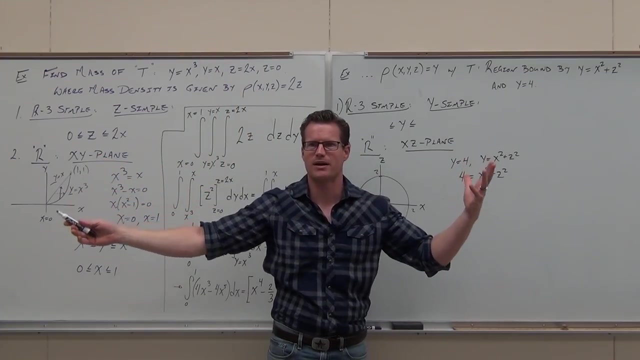 I never told you that Worst professor in the world, Uncannily bad at teaching anything besides freaking circles. I swear this guy could stand there and just go perfect circle. It's as if his arm moved independent from his body. 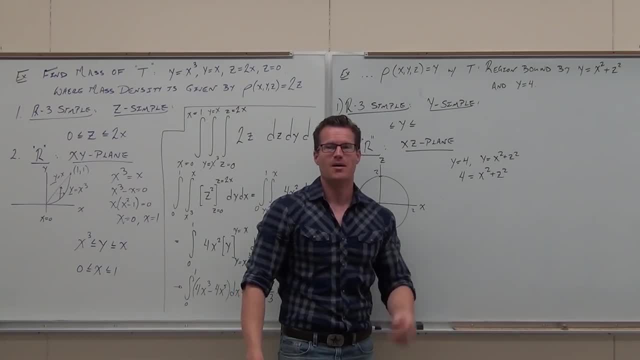 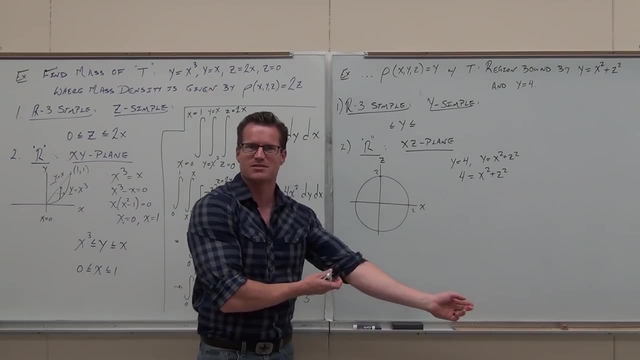 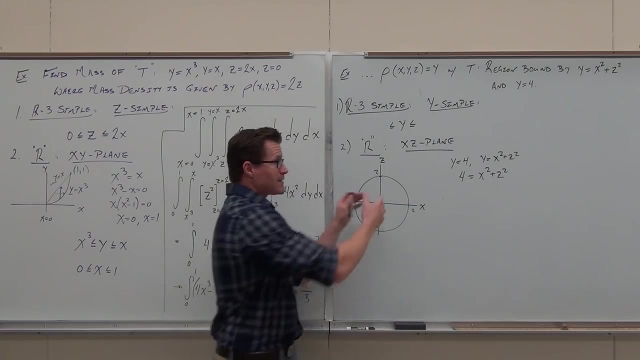 That's amazing. But you suck at teaching, sir. But his circles- mind blowing- Unbelievable- Taught physics. Well, I know nothing about physics. Thanks, professor, Awesome professor, Circle sucker guy Anyway. So that's the circle. 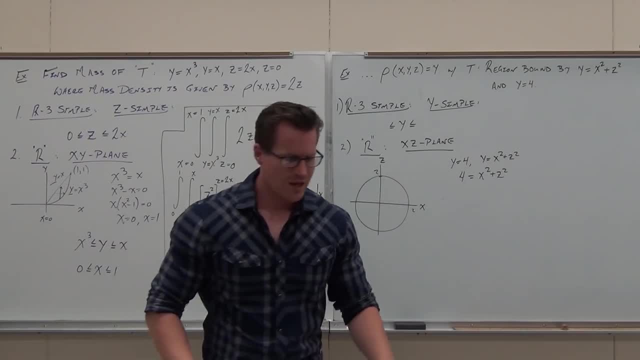 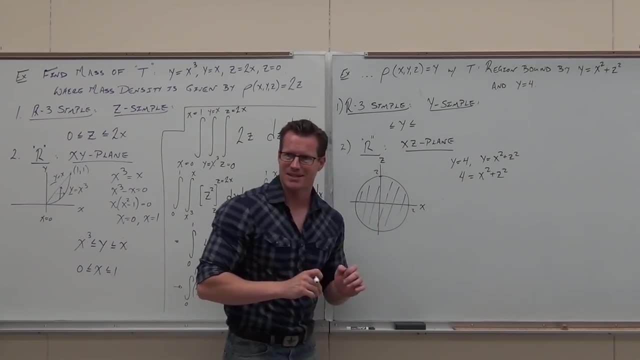 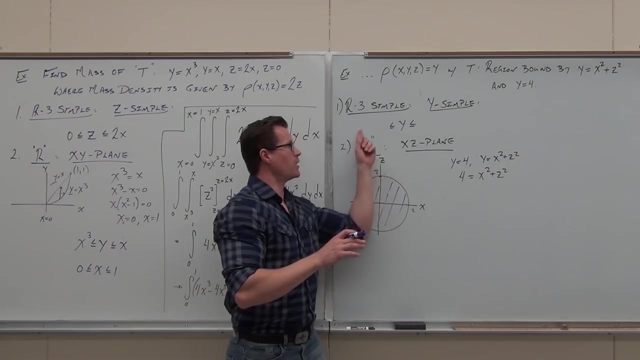 Now wait, Now wait a second. So if that's the circle, this right here creates for you the region, for your double integral, Does that make sense? This thing is above that region, Does that make sense? Here's how you determine what goes here and here. 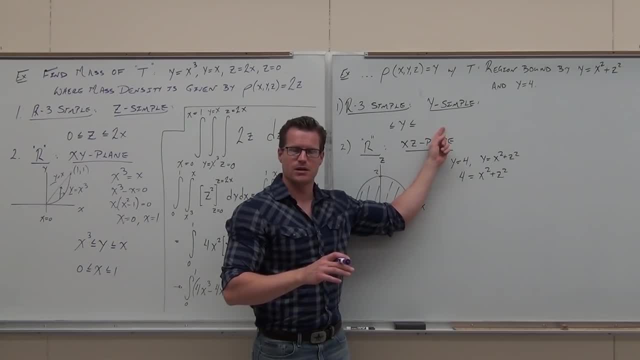 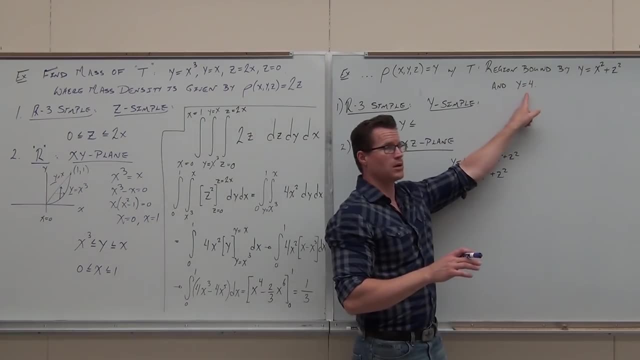 if you can't picture it in your head. Are you listening? Take some point on the region. Give me a good point on the region. Zero, zero, zero, Plug it in here and plug it in here and see which one's bigger. 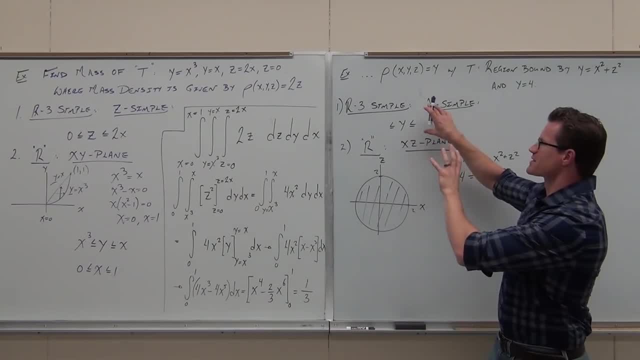 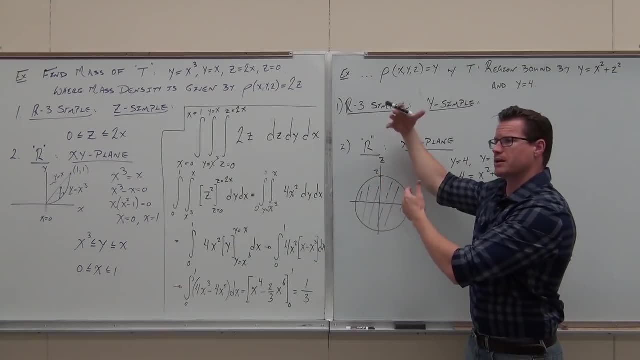 But it's got to be on the region. Do you get it? So you can kind of skip this. whatever's in order-ness so far. Do your region first, So skip down. Do your region first and then go back to it. 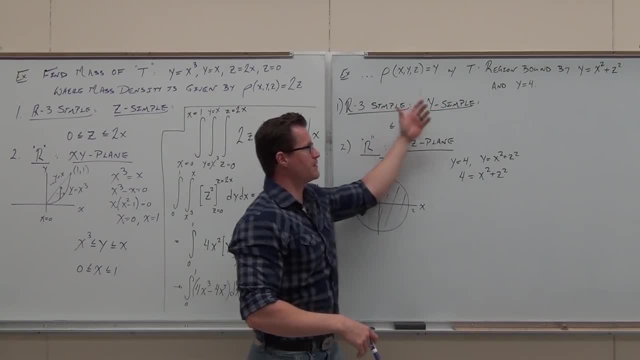 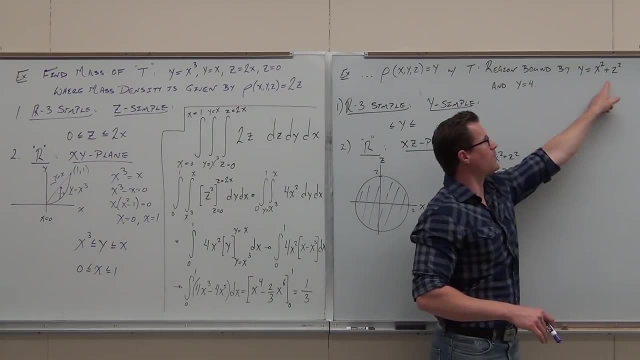 So if I don't know how to put them in order from here, then I find my level curve, I put it on the plane, my coordinate plane, just like we always do, And then you plug in a point. If I plug in zero, zero, y would equal what? 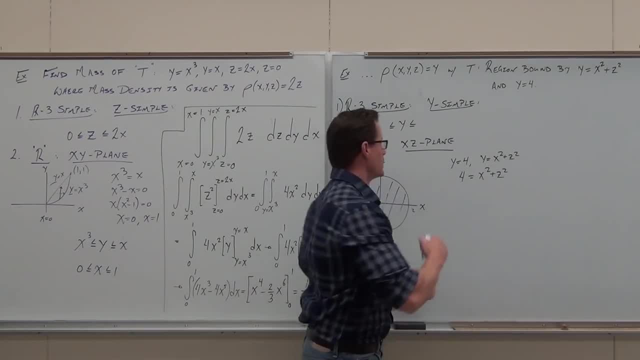 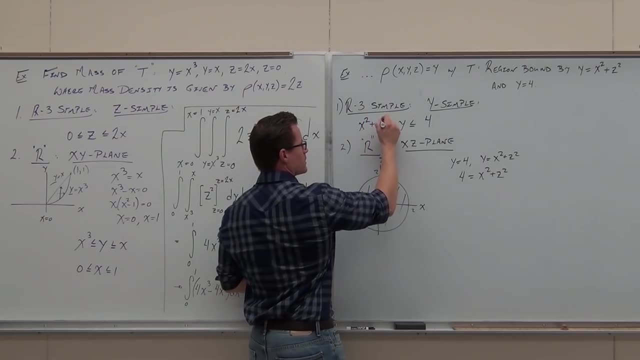 And y would equal which one's bigger. Either way you do it, the four is the bigger y equals function. The x squared plus z squared is the smaller y equals function. Head nod. if you're going to give me that one, Hey, we're pretty much, we're getting there. 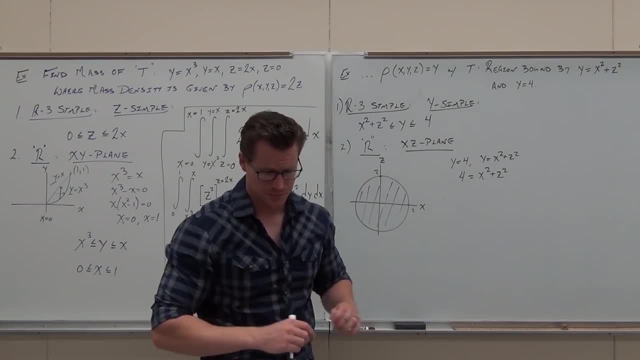 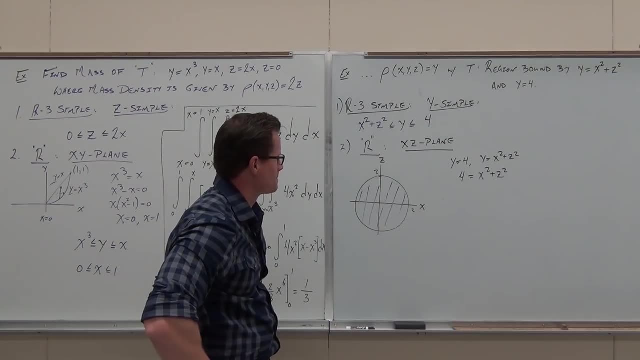 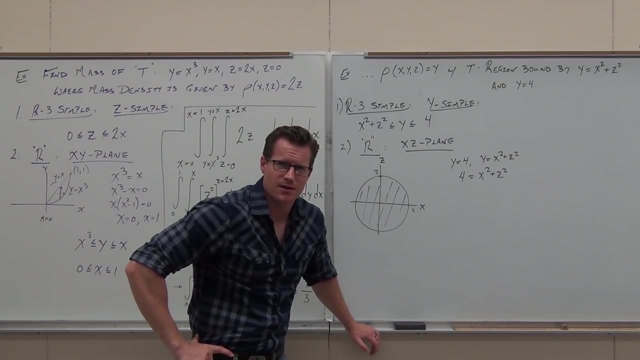 We're pretty close Now. now, Wow, What type of region Do you have here? What do you use for circular regions, for double integrals, Polar, Polar? I'm going to shake your head. That's awesome. You trust me. 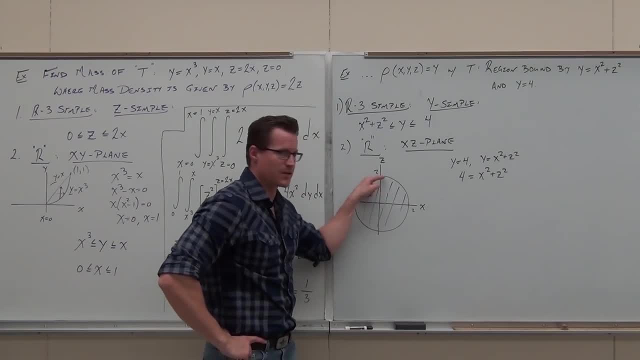 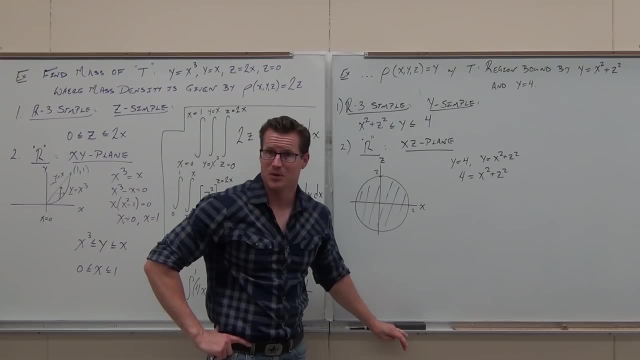 You will not want to do this with a rectangular because you have to go from here to here, that's, across two functions and then constants. would be easy, But you would not want to do that. Trust the lender. Polar is your absolute best friend of this problem because your region is a circle. 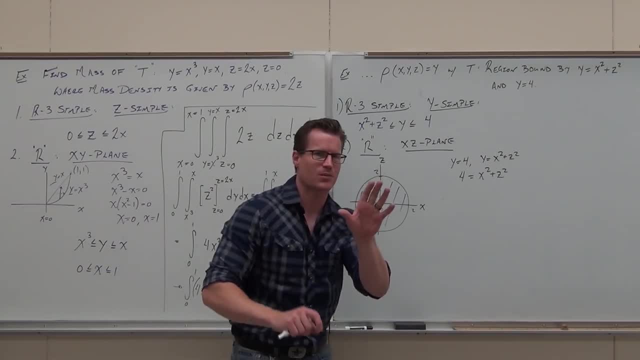 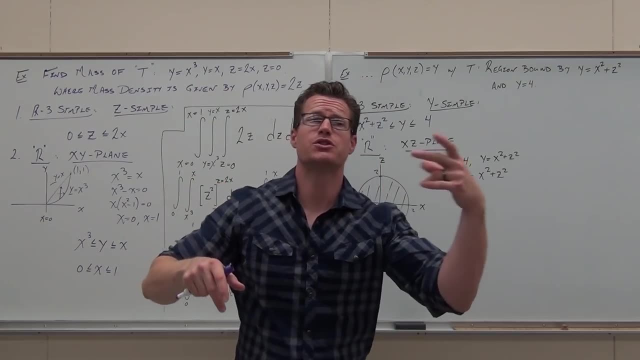 and circles are really nice, But there's one. There's one thing. There's one thing you've got to realize: Whatever coordinate plane that you're on, that is what determines your polar coordinates. So you are used to doing x squared plus y squared. 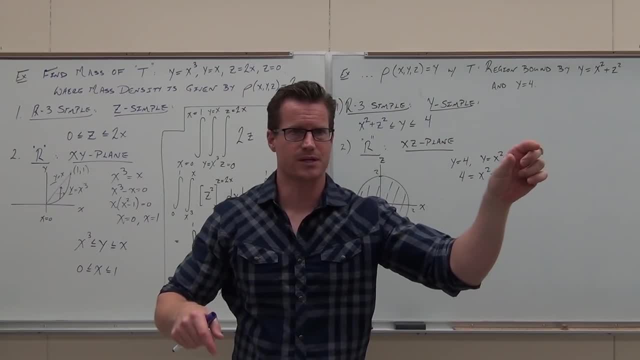 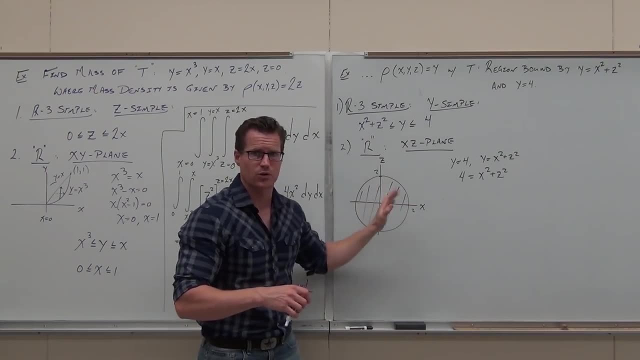 I hope you're listening. You're used to doing x squared plus y squared equals r squared. Does that make sense? Now listen, The reason why we draw these always in the same orientation, where x is horizontal and y is horizontal and z is vertical, is so that you always have the same type of idea. 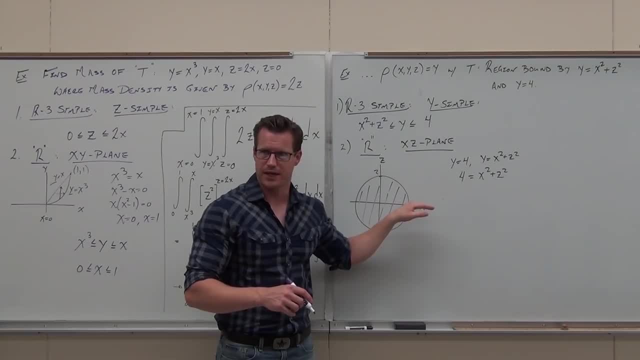 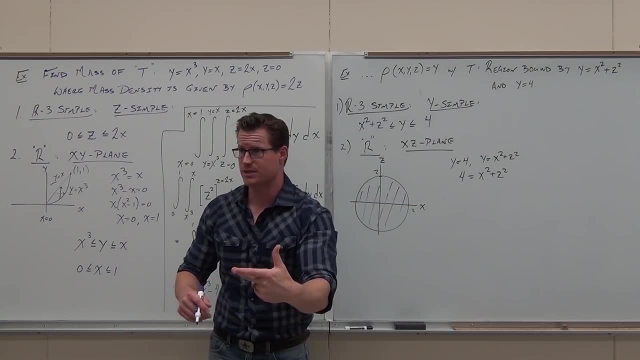 X is going to be your r cosine theta, But y is a cosine. It's not going to be your r sine theta. What is Z? Z takes the place of y here. Does that make sense? Z takes the place of y. 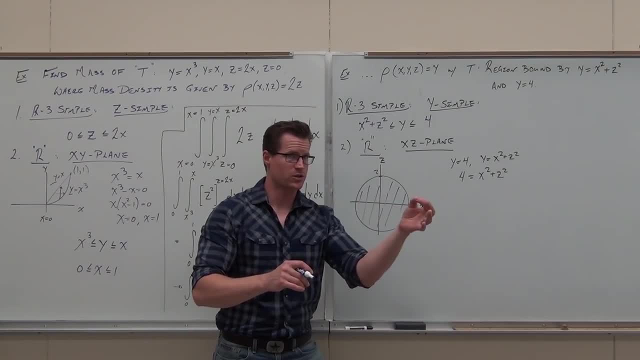 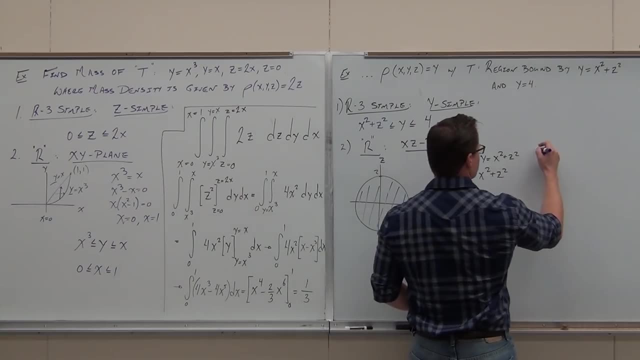 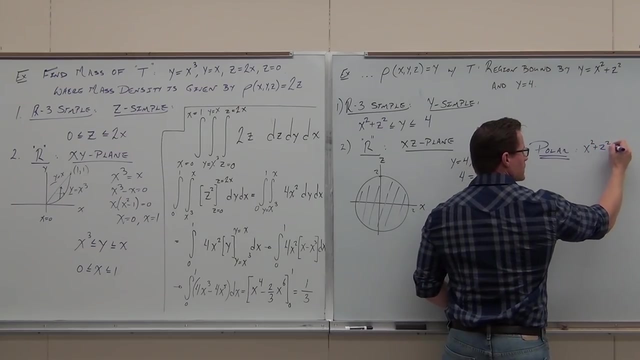 Which means that it's not x squared plus y squared equals r squared, It's x squared plus Z squared, Yes. So this looks a whole lot like polar. Yes, But x squared plus z squared equals r squared. Well, that's not going to be your r sine theta. 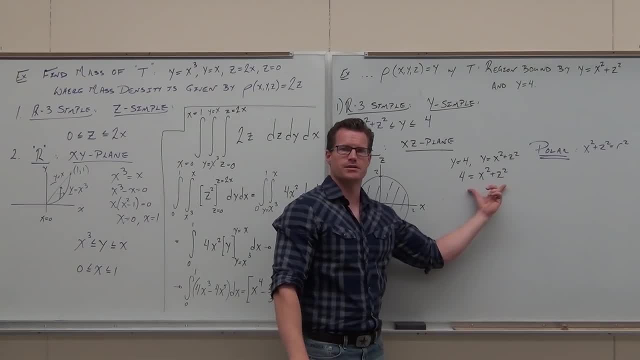 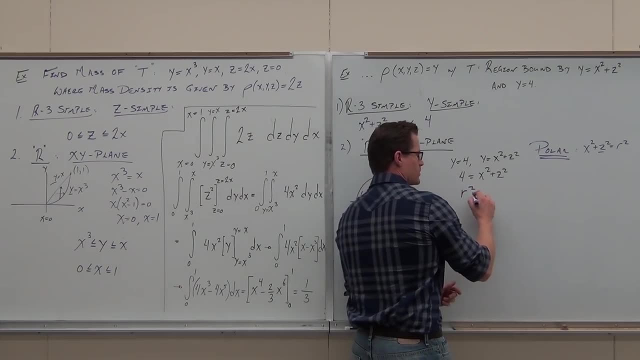 It's not going to be your r sine theta. That's pretty darn nice, because now I can start translating this, since it's z squared- Hey, how much is all this stuff right here? r squared, So that would be. r squared equals 4.. 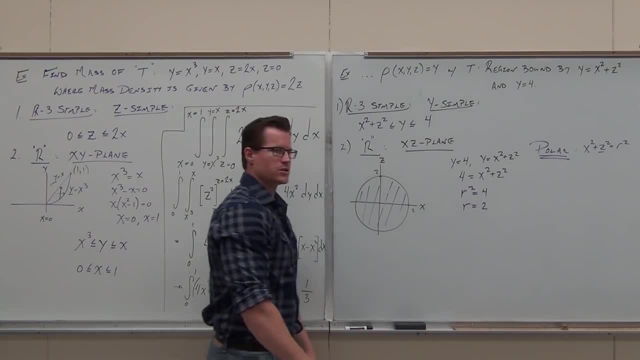 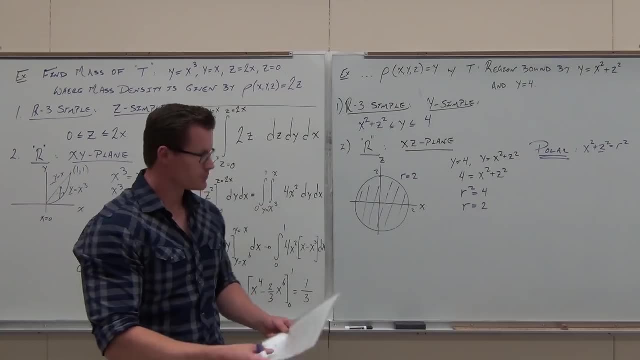 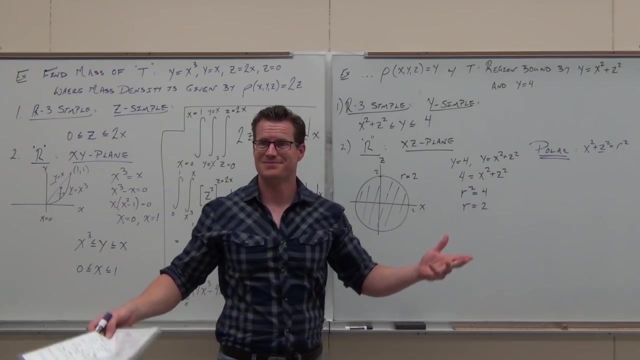 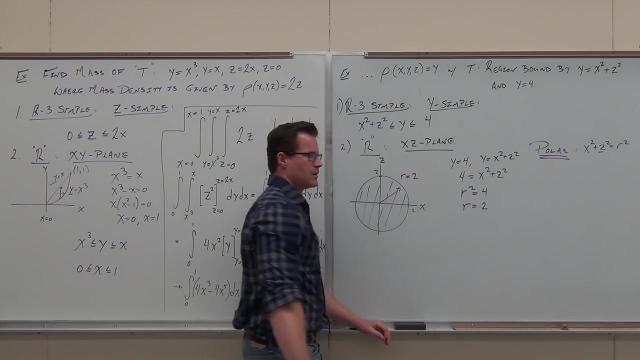 r equals how much, ladies and gentlemen. 2. r equals 2. r equals 2.. Yeah, Pretty neat. So from here to here, if you remember, for double integrals, which one do we do first? Do we do the r first or the theta first? 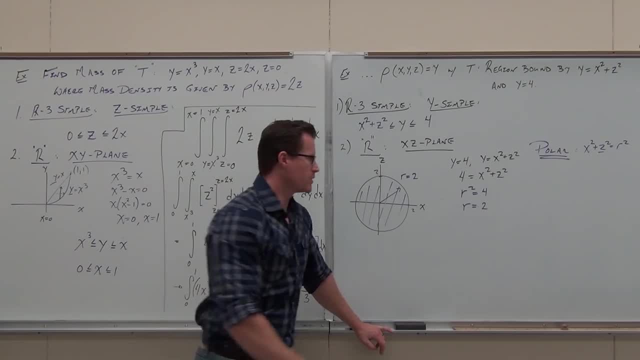 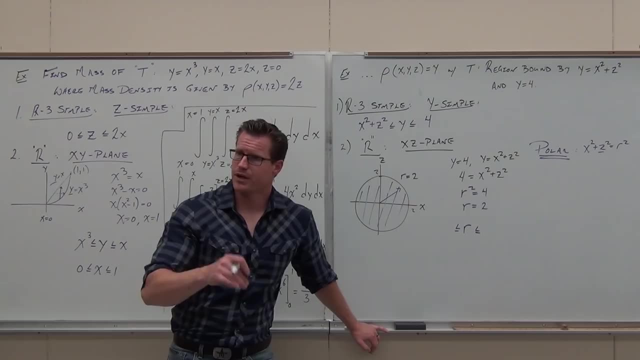 R All the time, All the time, Which means that I want to start with r between two functions of r, And then I want theta between two functions of theta. So let's try to get this together. What's the small value for r? 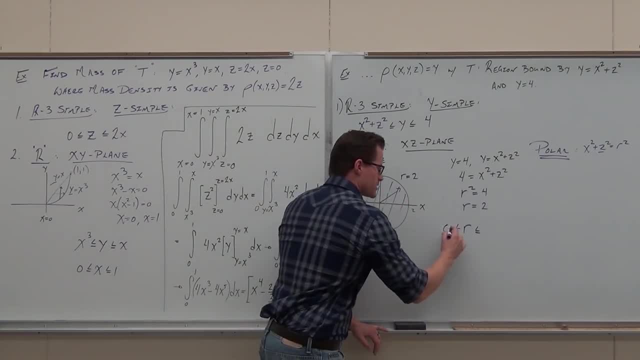 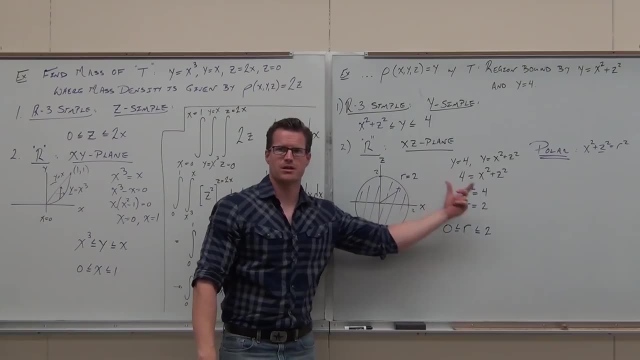 Think back to polar Zero. Zero. Start the region immediately zero. What's the large value? Wherever you get your function, it's the large value Two. I love constants Two. If that had been like r cosine theta, you'd put r cosine theta. 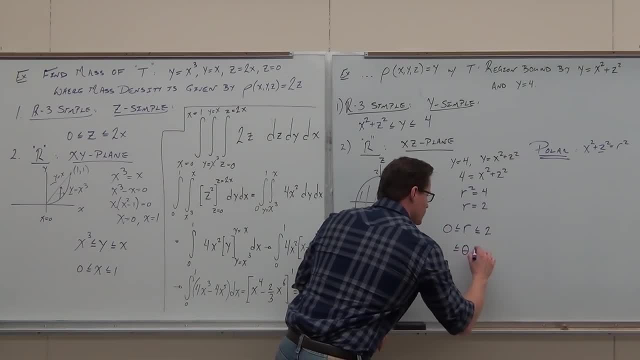 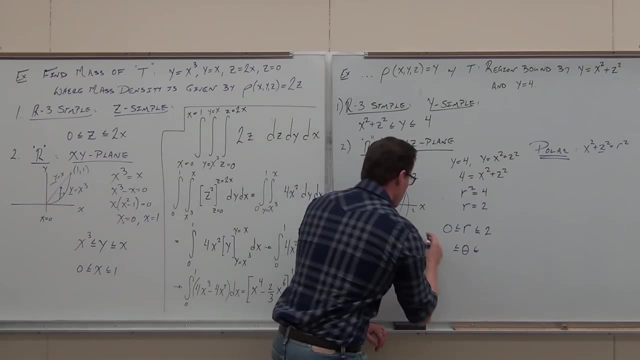 Now, how about the theta? That would be my last little piece here. What's the small value for theta? Where's the star? Zero, Zero. It's the full circle. normal circle Doesn't move too fast, too slow. 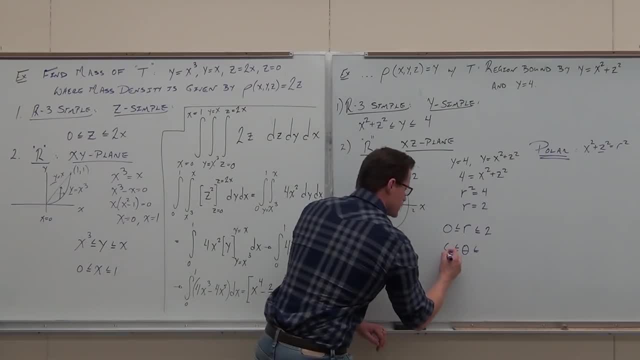 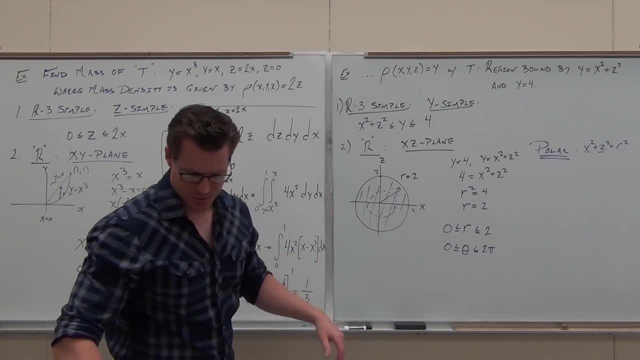 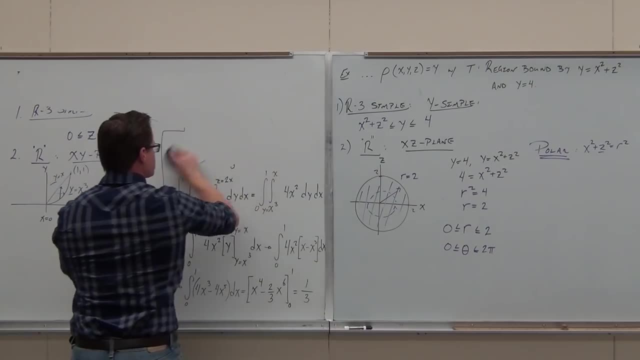 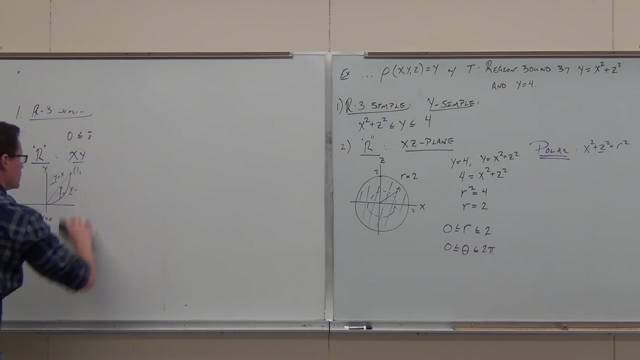 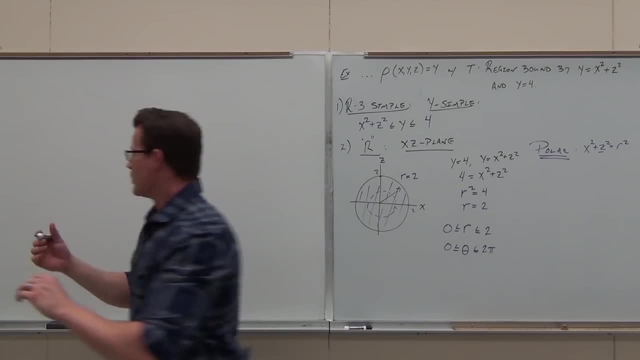 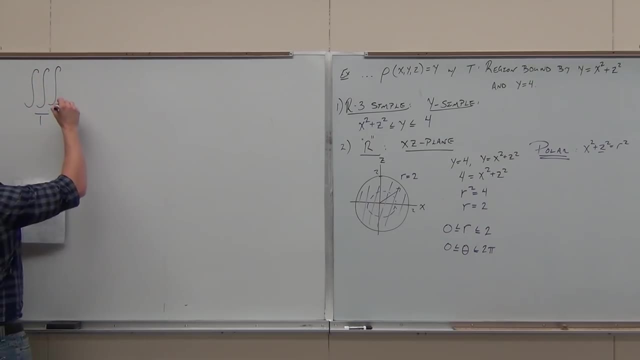 unless you want just really really good notes. Here's what we've done. What we've taken is we've taken the normal idea of a triple integral over a region and we've said: you know what? no, let's think about this. 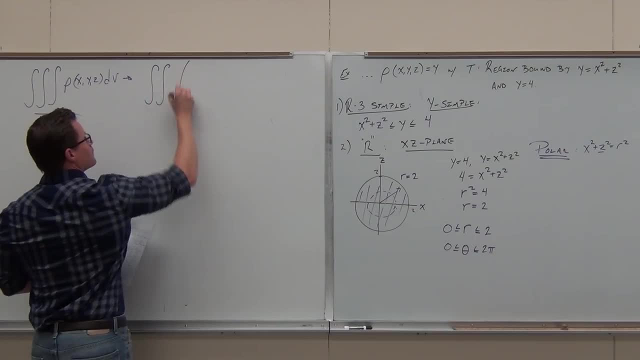 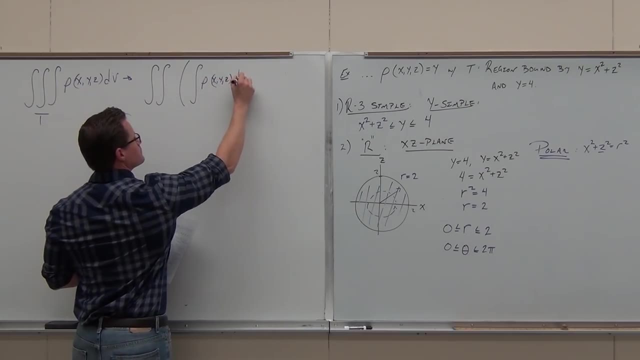 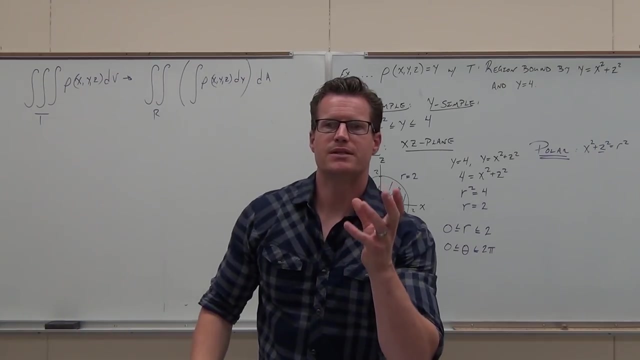 Let's think about this as a first integral, dy, and then another integral. that's a double integral outside of it, But you can do that double integral however you want. So the first one, man, that's always between two functions. 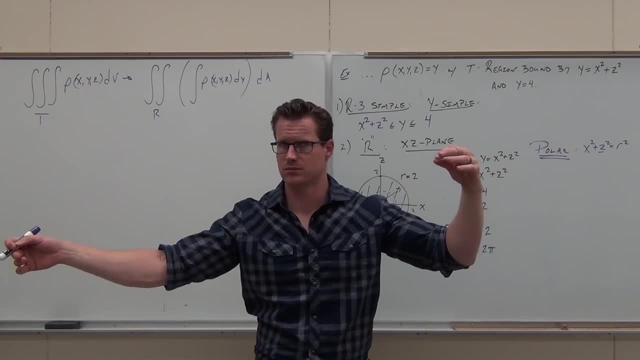 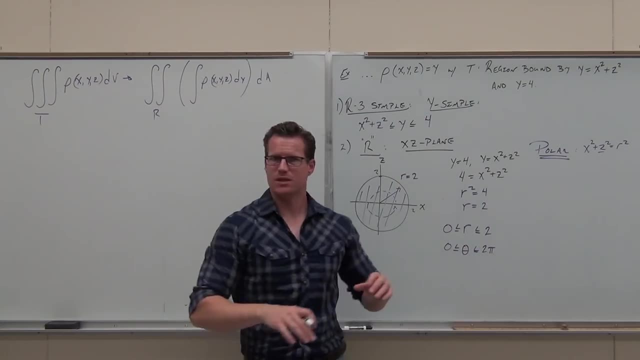 x, y or z, always for us, unless we start talking about spherical. that's later, But it's always between two functions: x, y or z. After that you get a double integral. If you get a region, that's circular, goodness. 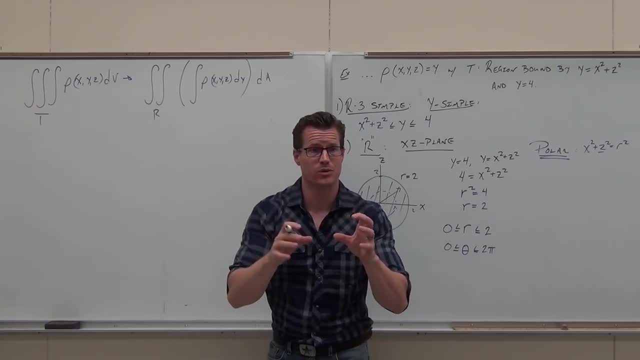 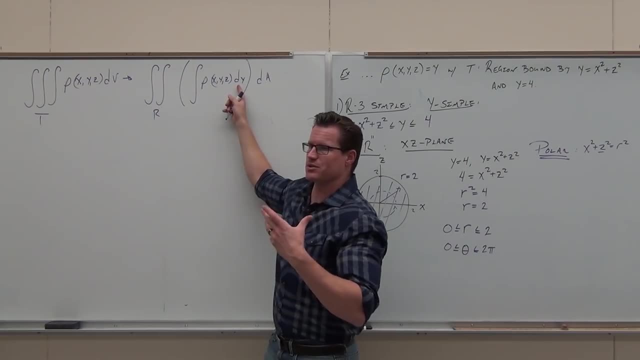 change that double integral into polar? Are you guys starting to see the connection between why we did polar and how that relates to this stuff? Inside one you're always speaking x, y or z, But if I have a y or an x or a z, I'm left with any other. 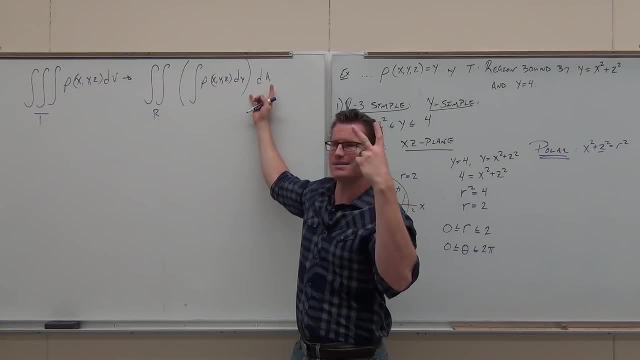 two variables: x, z, x, y, y, z. That creates a coordinate plane. That creates a region on a coordinate plane. That creates possibly a circular region on a coordinate plane. I can change that and go well, let's consider my region. 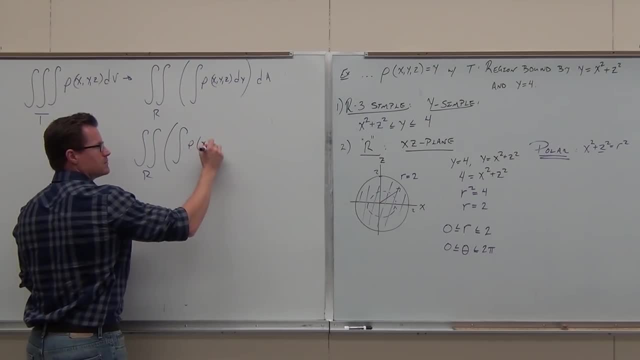 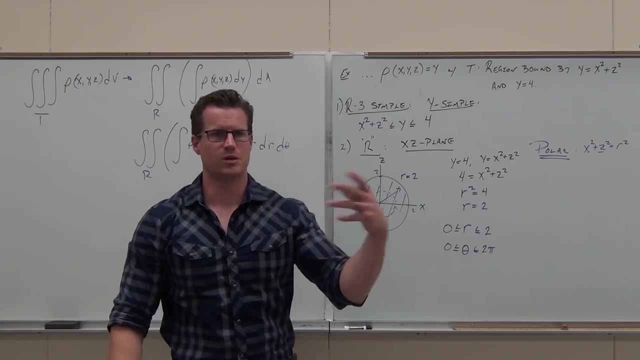 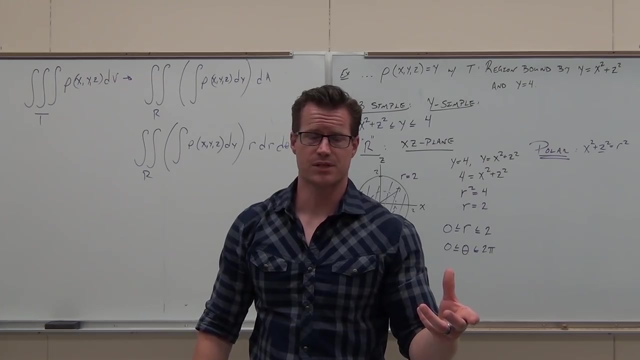 to be same stuff inside r, d, r d theta. Let's consider circular regions to be polar for that double integral. Does that make sense? I know we're learning a lot. There's a lot of stuff and we're going to stop after this example. 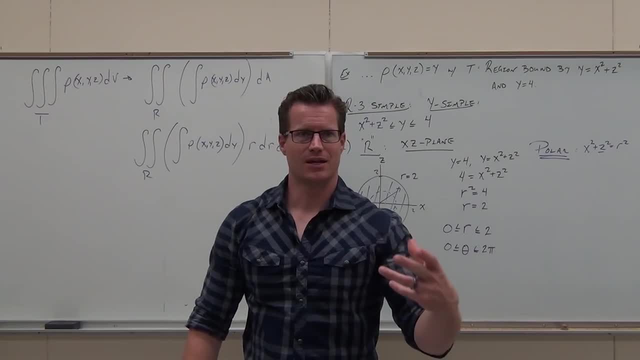 because your brains are going to be fried after this one. But are you getting the connections? Do you feel like you've learned a lot today so far? Are you ready to put it together? Yes, It's not going to be that hard. 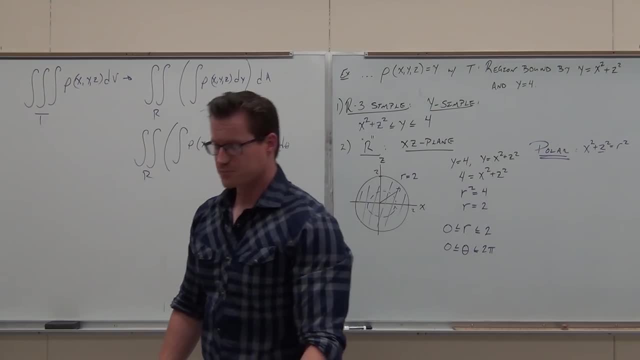 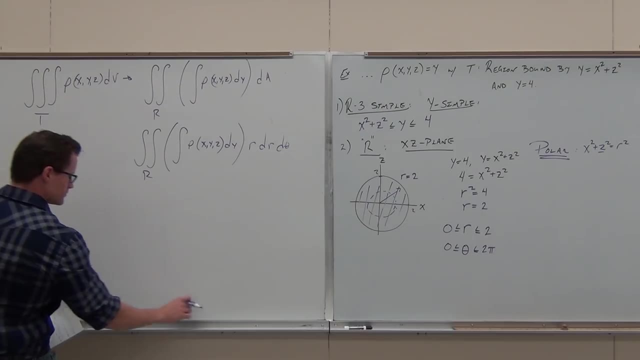 There's just one more thing we got to do. There's one more thing When we start setting this up. so here's our setup here. When we start setting this up, what's the first? what did we do? What simple, r3 simple did we do first? 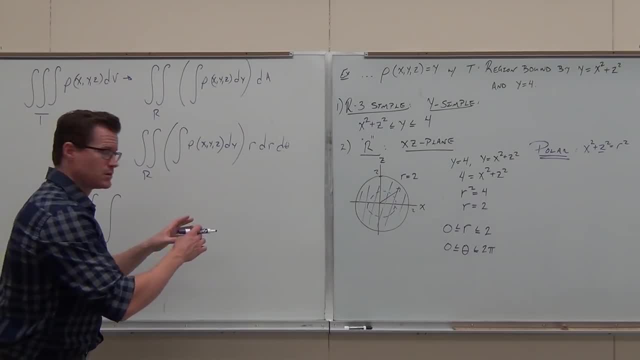 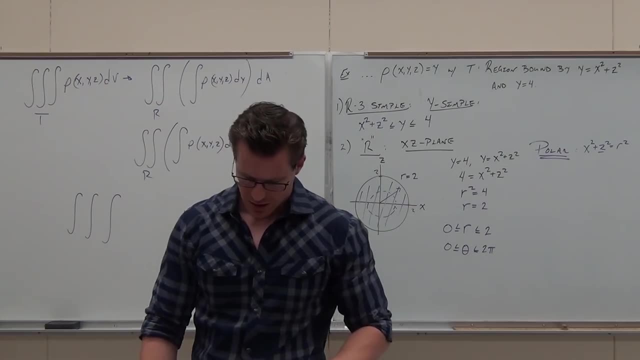 I'm going to need a d. I'm going to need that first. I'm going to need a dy first. Now, if I need the dy first and I'm going to need a dy first, I'm going to need a dy first. 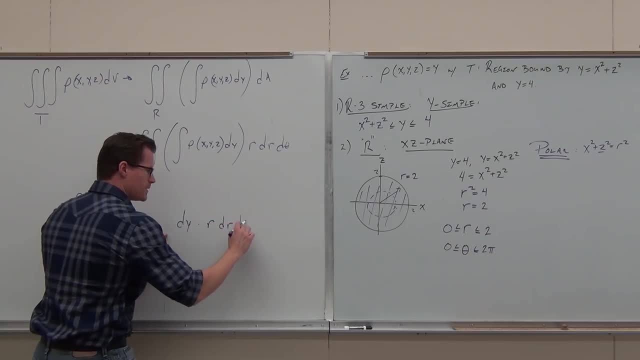 And I'm going to do r, dr d theta, Do you see where that comes from? Here's our first integral. Here's our double integral, switching to polar. The problem is this: Look at the problem. I need you to look at the problem. 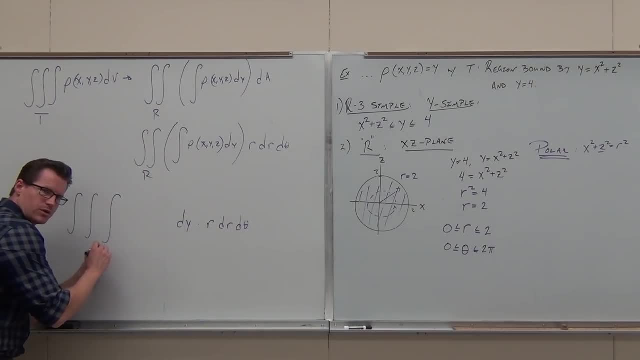 The problem is: yes, I'm certainly going to have what variable equals? what variable I'm going for? I'm going to have y equals and I'm going to have y equals. Does that make sense? I'm going to have to have that because I'm still integrating. 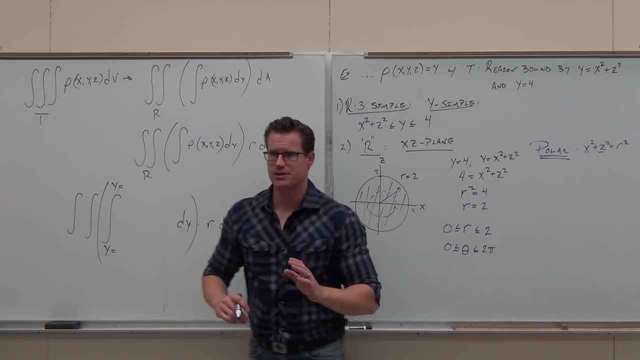 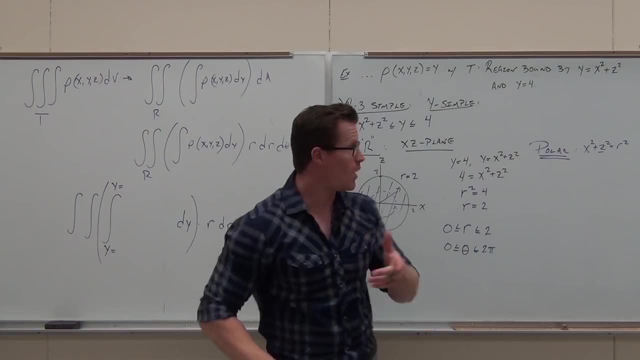 with respect to y first. Now that you understand the concept, That does not change. That's why, simple, first, I'm going between two functions of y. I'm going to integrate with respect to y, Just like we've said. Does that make sense? 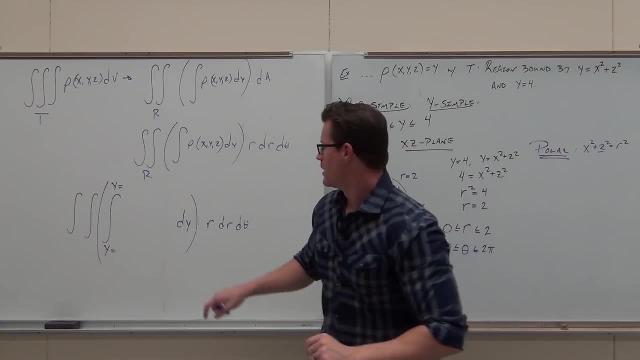 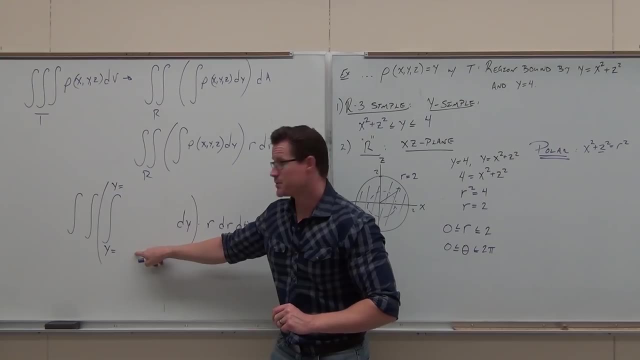 However, we also talked about this. Don't lose me here. Don't miss this thing. Whatever this equals, and whatever this equals, the way I've taught you must match up to the next variables that you're doing. Does that make sense? 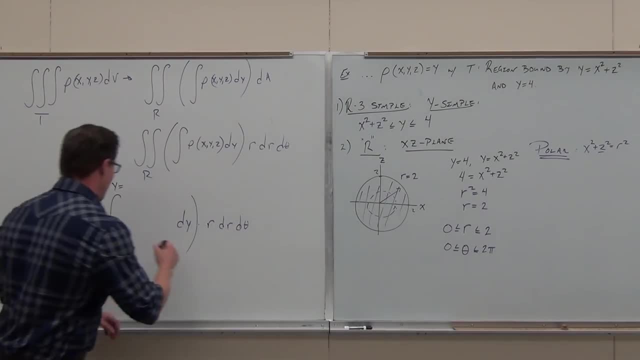 They've got to be in terms of r. So when we look over here, I can't just put x squared plus z squared. I don't see no x's and I don't see any z's over there either. Does that make sense? 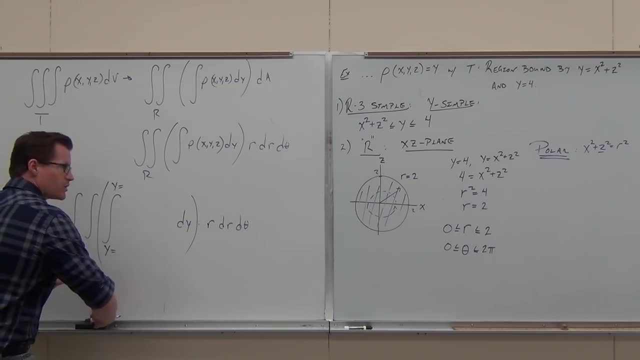 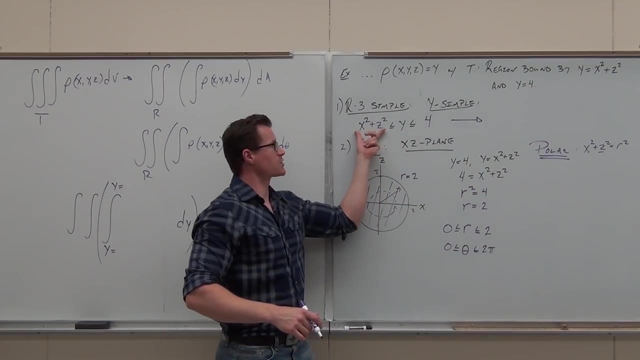 You've got to change it. So let's change this. So, if we're going to use polar for our region, we're going to change this now. But we already have the math. Hey, you tell me How much is x squared plus z squared according? 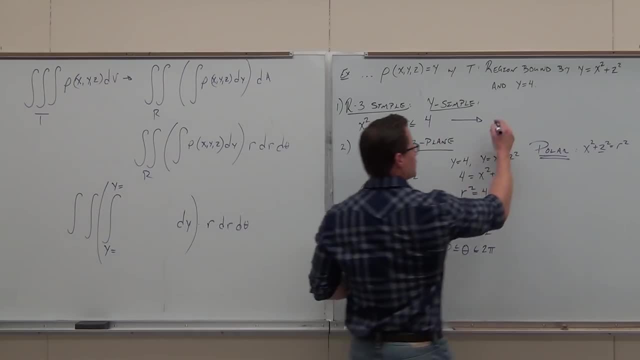 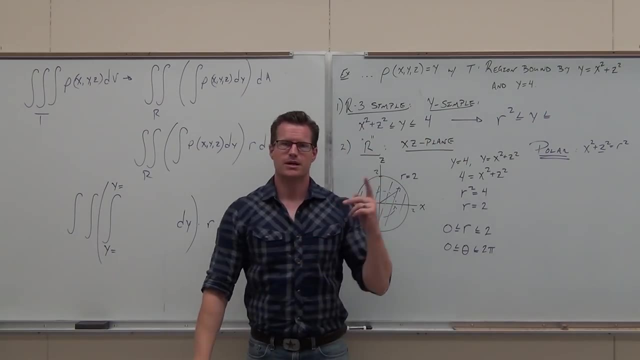 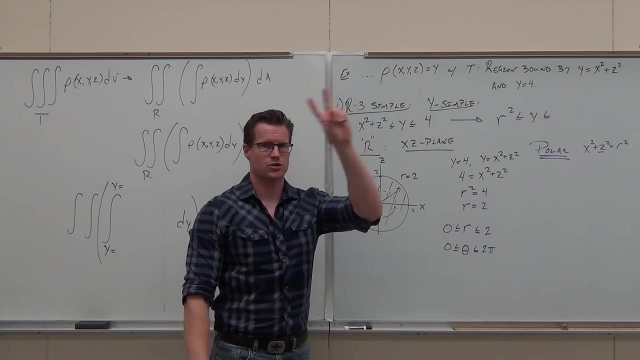 to our polar region. What are we going to change it to? So r squared is less than or equal to, y is less than or equal to. oh, be careful, Be very careful, Be careful here. Is it still 4?? No, It's 2.. 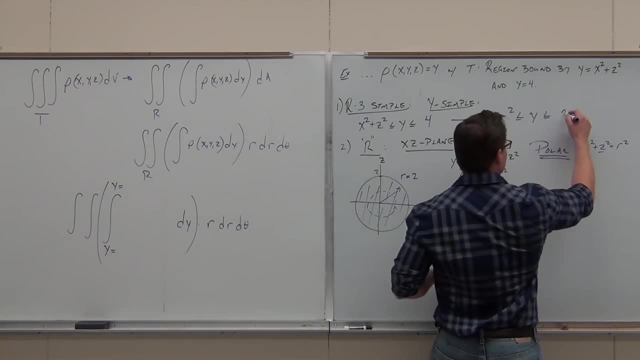 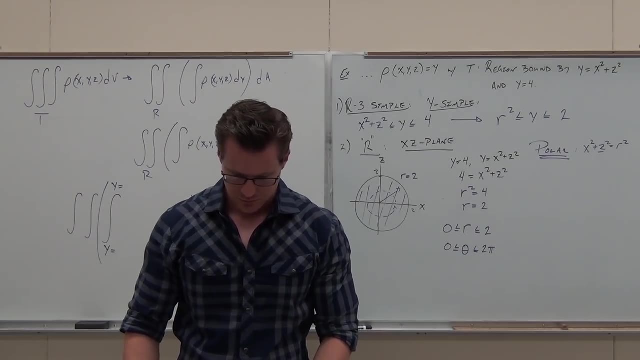 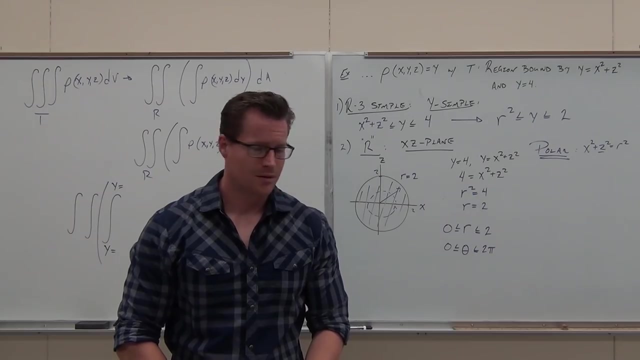 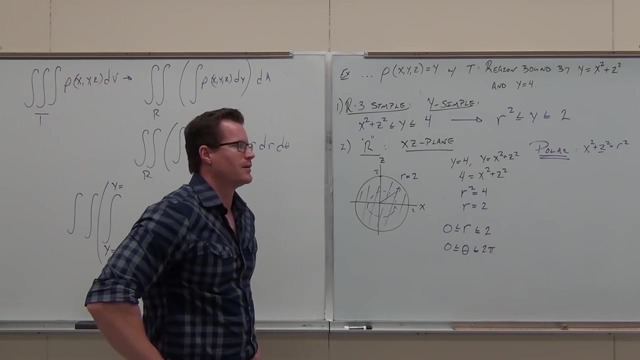 Do you see why it's 2?? Wait, no, Oops, Okay, I got thrown off. No, I'm sorry, I got to read it back. I heard him rather than round right back there and I lost my train of thought and I think I made a mistake. 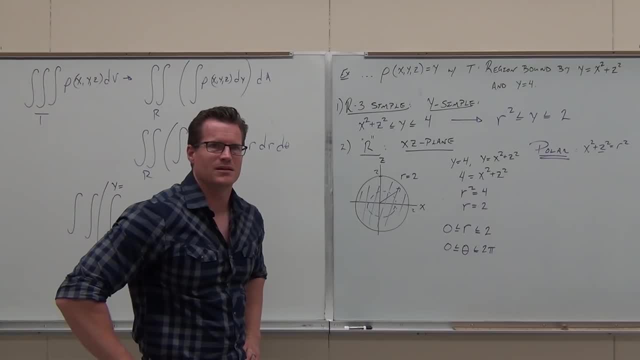 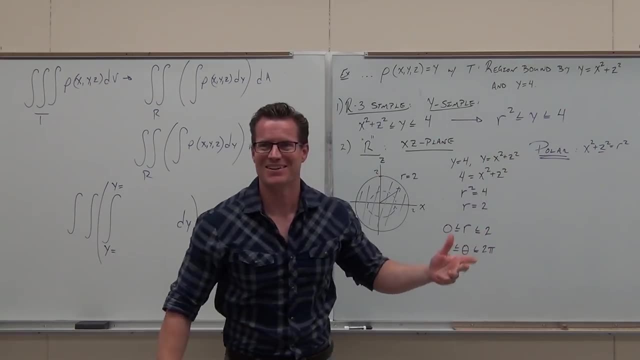 I'm not going to erase the whole thing. I'm going to erase this number, though, if that's still 4.. I got, I'm sorry. The janitor came in and was like fuck crazy. Did he freak you out too? 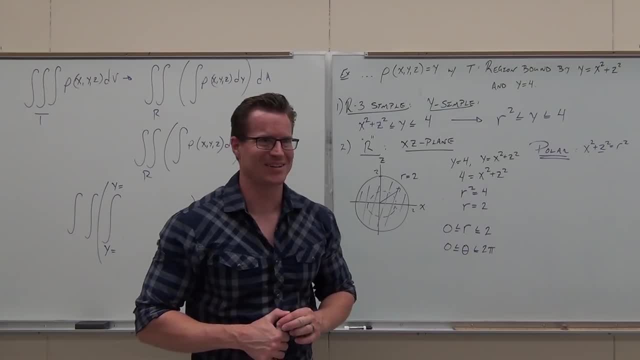 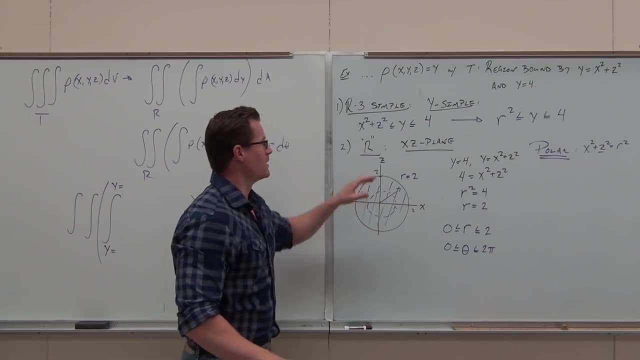 Yeah, He's going to jump out again. He's going to get me. It's so fast, Look. look. I made a mistake there. I apologize. I don't want to catch my mistake here. That part is polar, but this is still a y equals function. 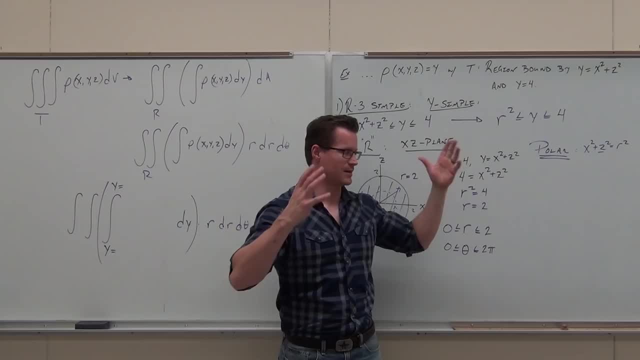 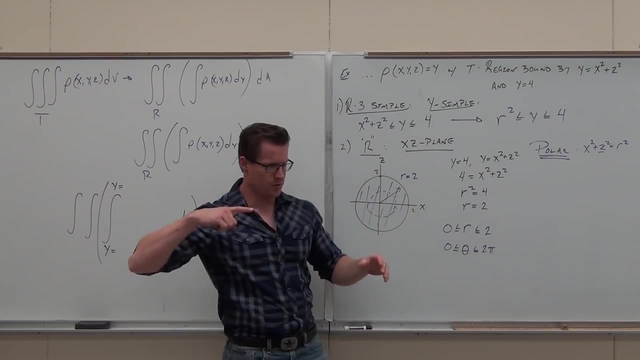 I made a mistake. I started thinking the region and I got confused myself. I started thinking the region, that we're over here and that's not what we're doing. What we're doing is we're going through 3 space between the paraboloid and between the plane. 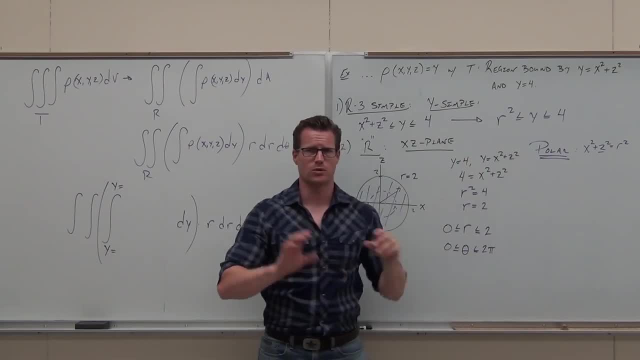 and we're just redefining the paraboloid in terms of something polar. That's what we're doing. I apologize for the confusion there. if I confused you, but I want to make sure we're all clear on that. Don't change the 4.. 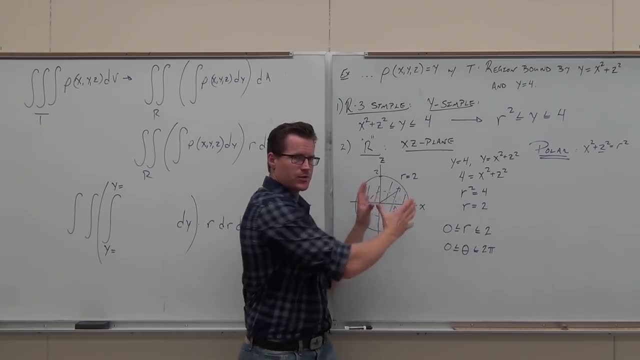 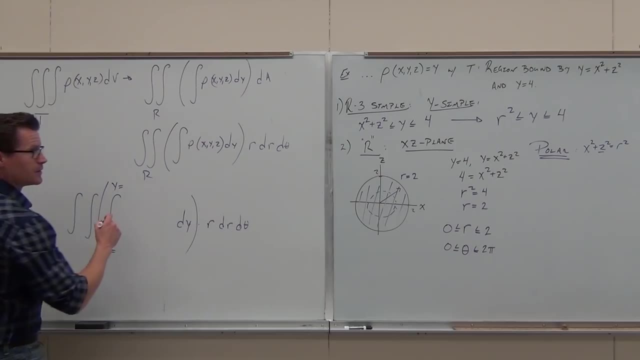 That's my bad. I got confused between the 3D idea and the region idea. Do you guys understand my confusion And get it straight here? So it's not 2. It's 4. My bad, So we're going to go yes, along y simple. 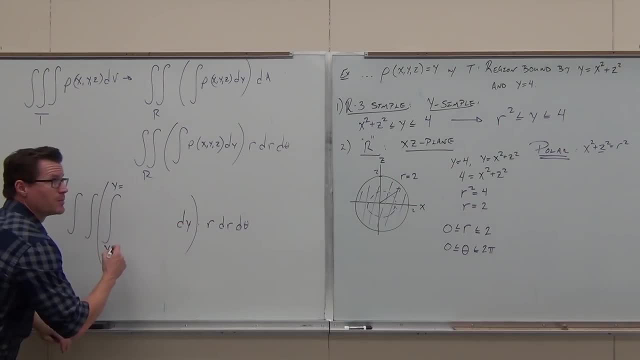 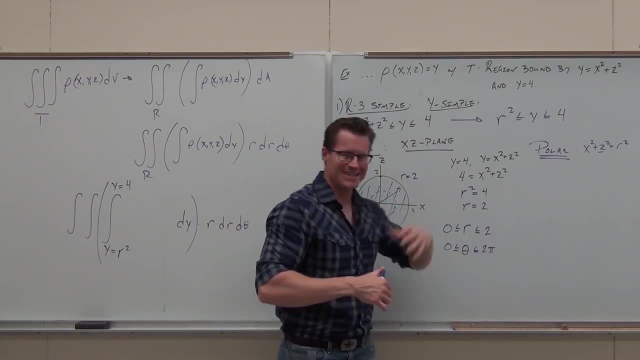 We just changed the function in terms of r, so that way it matches up, but this is still r squared and this is 4.. It just: you cannot have this in terms of x's and z's if we have r's and theta's any longer. 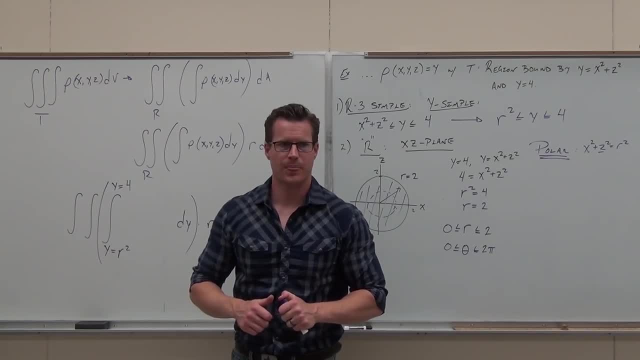 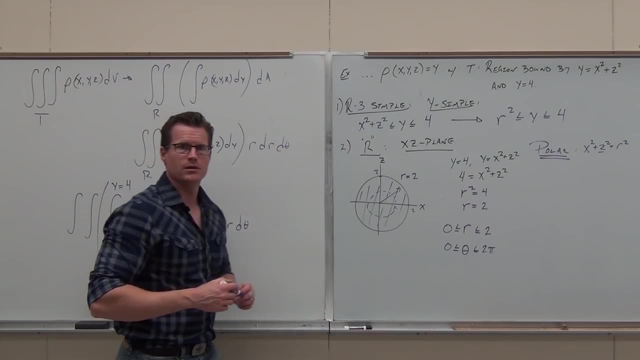 I did not do okay with that one. For real, Yes, no. Okay, Now let's wrap up the rest of it. I know the r dr d theta. Yes, You can't just put in: r is less than or equal to y. 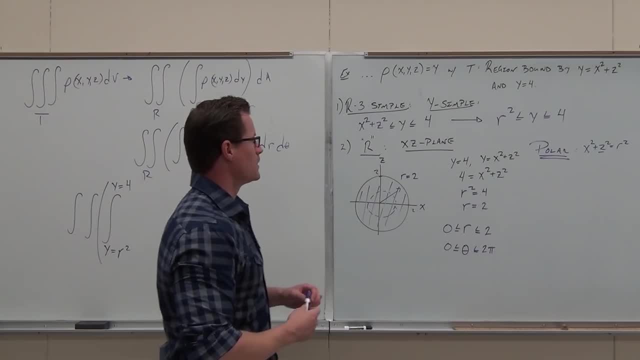 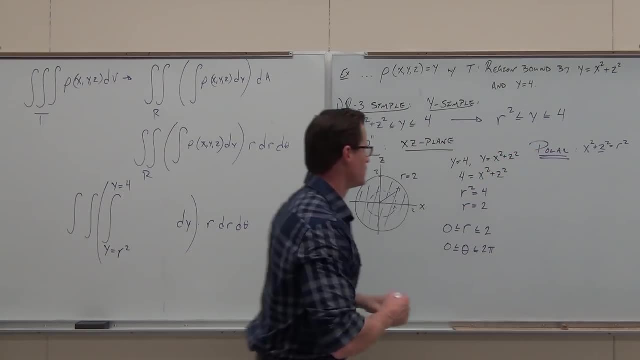 which is less than or equal to 2.. Or you could do that. You mean like square root, all of it. Yeah, Because then you have square root of y. I don't want to do that Now. let's wrap the rest of it up. 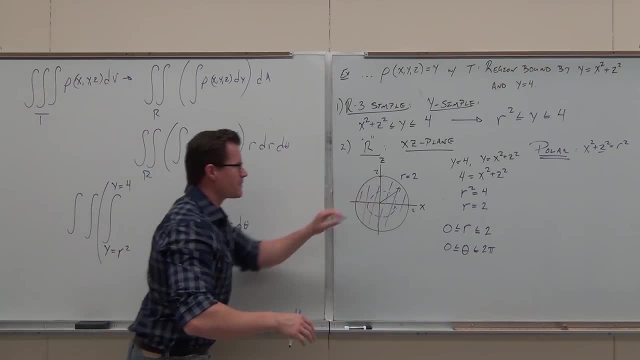 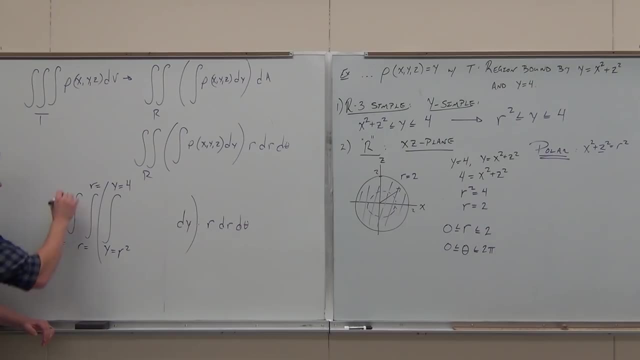 Now, as long as we've done r simple first, we've done our y simple, now we've got this region, that's polar. We have dr d theta. We always go. We go along r first and then we go along theta second. 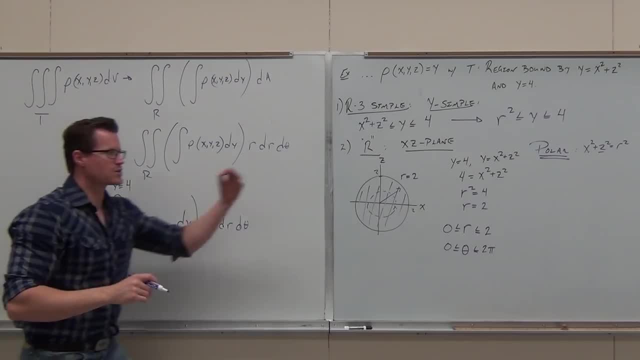 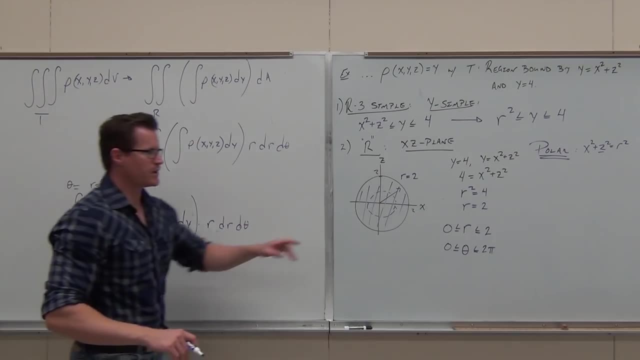 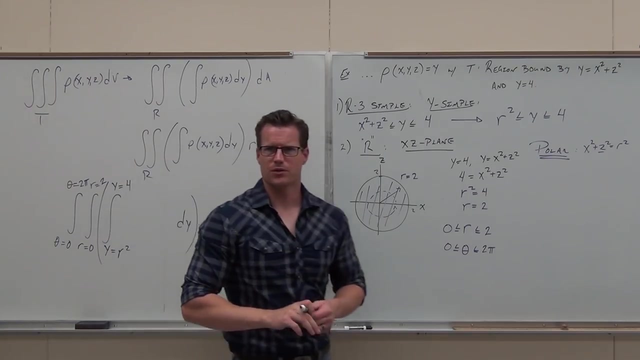 but we've already determined these things. r equals what to what? for our polar region, From where to where, Zero to 2 pi, Beautiful. And then for our theta, we already got it: Zero to 2 pi. And now, if you're okay with that, 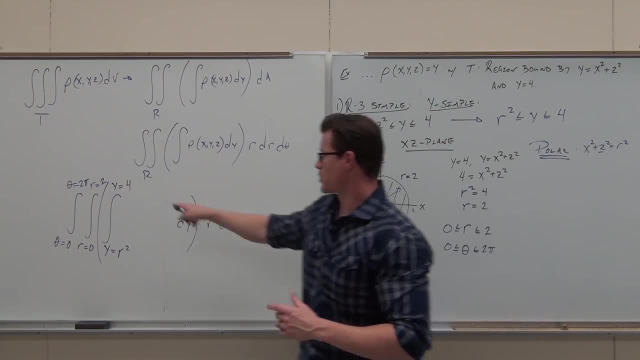 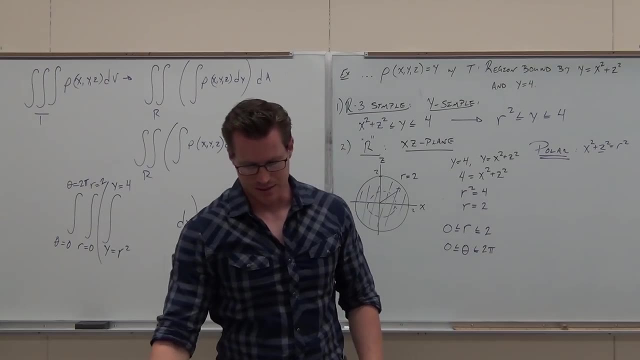 Yes, no, Yes, yes, yes. Okay, Hopefully I didn't totally screw that up for you guys, so you understand that I made a mistake And that's supposed to be four. Now I'm going to tell you something. 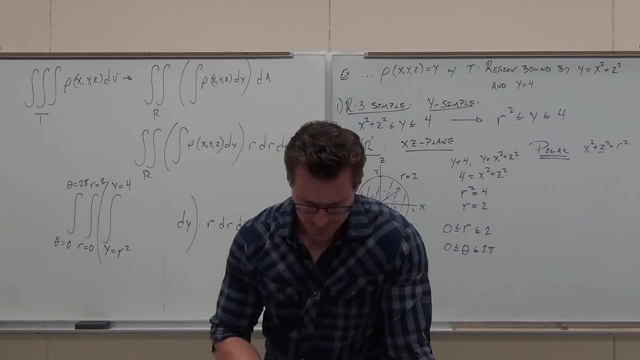 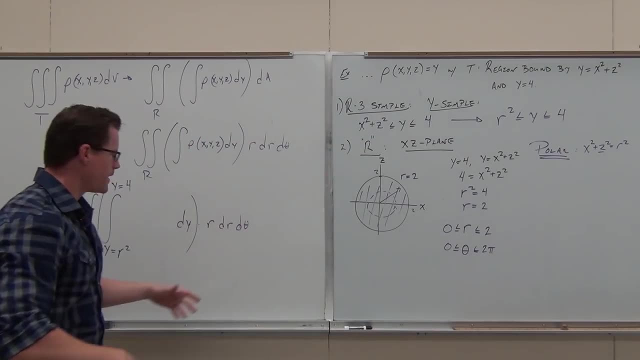 Some books have it different. They're a little wrong. Please, please, even though some of you might want to, We're missing one thing. You know what that thing is. What are we missing? Missing the mass density function. That mass density function is what. 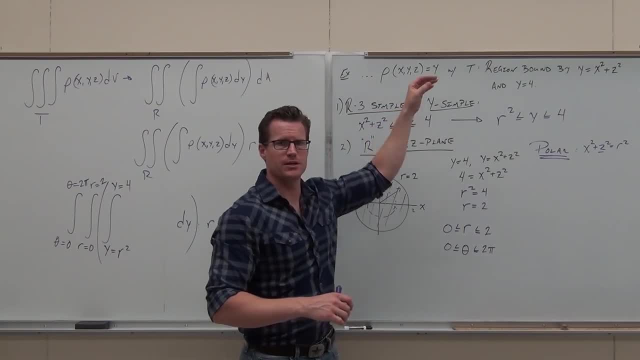 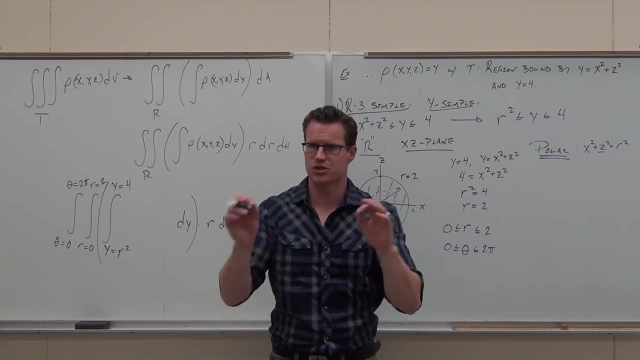 Y. Please don't start changing that into like r sine r cosine. Please don't change that, Because that right don't you, even if it was like x's and z's. some books change it ahead of time. They shouldn't. 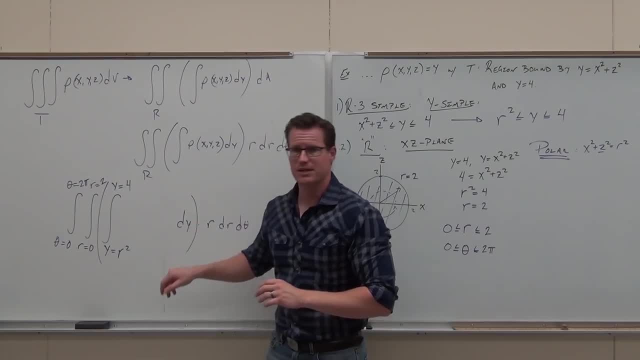 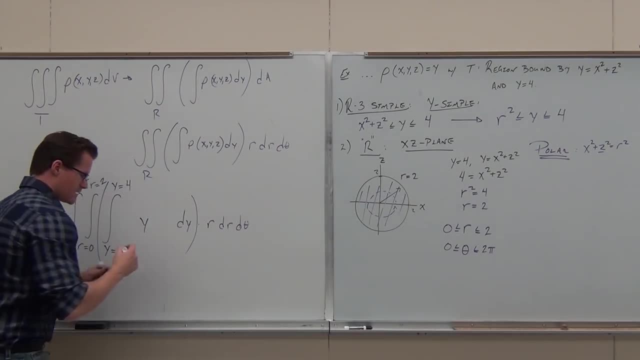 Because if that has a variable like this, you have to integrate with respect to that variable. Don't worry, I got more. Does that make sense? I got lots more, So you leave this. Look, it's going to be fine. 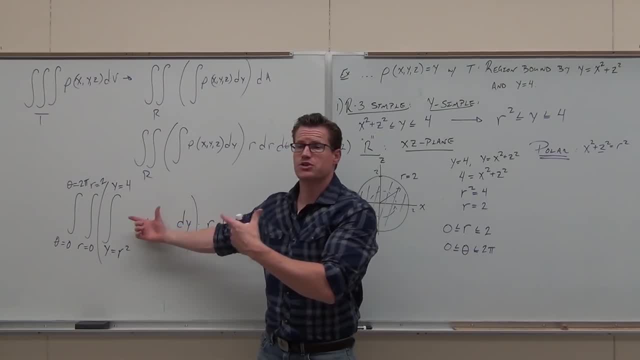 Even if, even if that doesn't have y's in it and you integrate, you'd be able to change it later. in terms of these things, The only thing we got to make sure that we we match up Y equals with y equals. 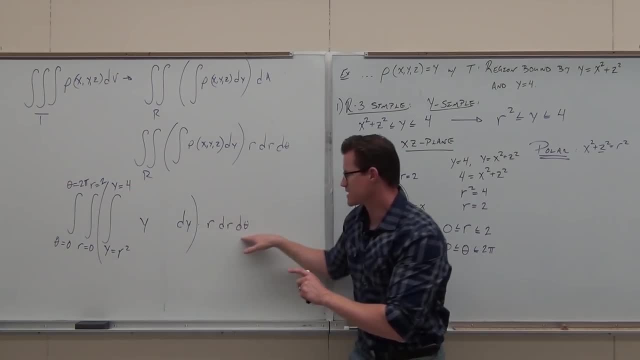 Don't change this, Let's do it again. But then what the y equals has to match up with the rest of your variables. Whatever this is has to match up with these things. So if it's really okay with that one, Can you try to do the first step? 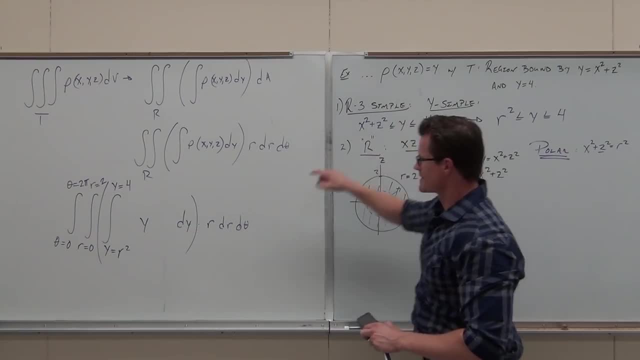 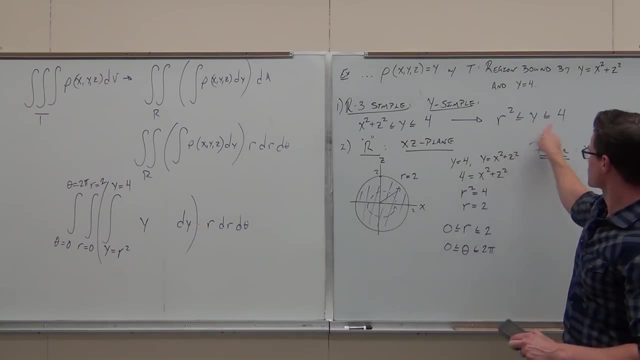 Y, simple, y simple. mass density. mass density Change to polar. So we got to change that to polar Polar. to match: We got: okay, r squared to 4, r squared to 4.. We got, dr, r is matching between 0 and 2.. 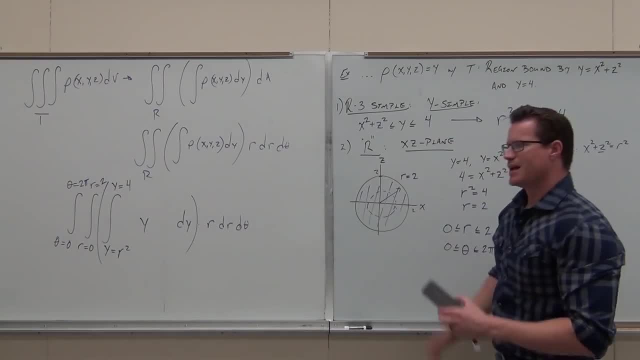 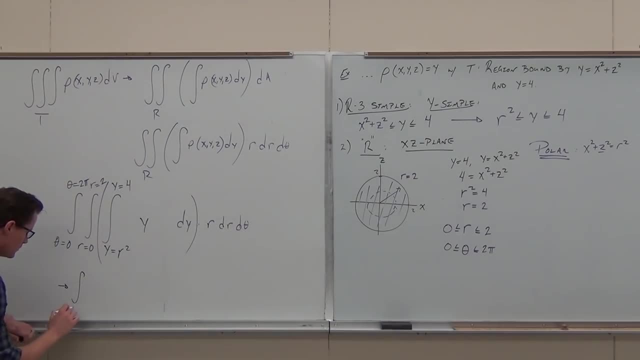 That's what we got: Theta between 0 and 2 pi. That's what we got. Basic integration. Do you see how you have to leave that variable? To integrate that It's with respect to y. You need to leave those variables because if you have any, 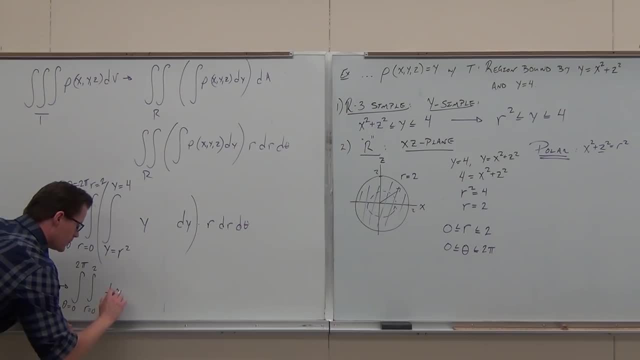 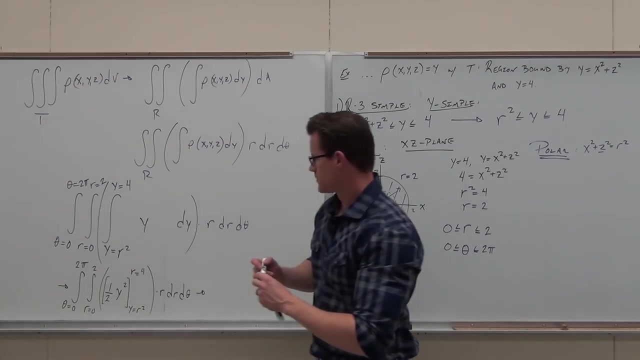 of that variable. it's got to have something to integrate. Okay, You're still going 0 and 2 pi, You're still going 0 and 2.. Did you all get the 1 half y squared? and then r goes from. 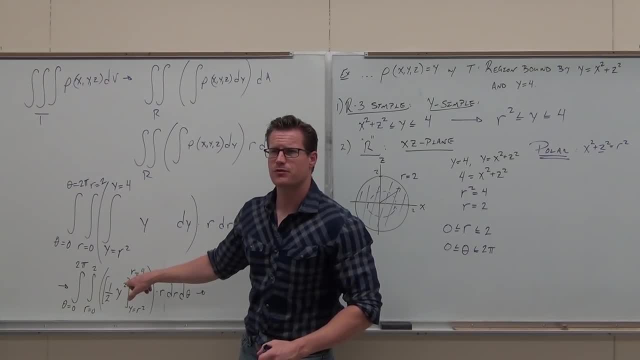 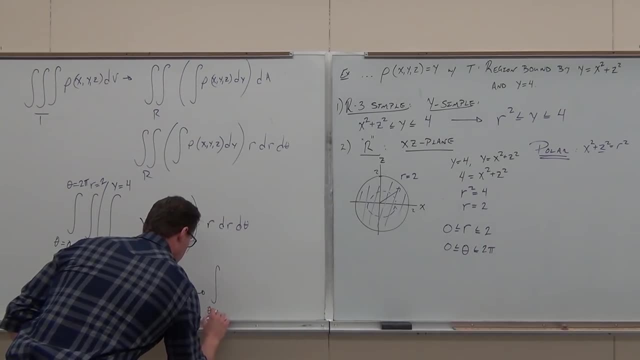 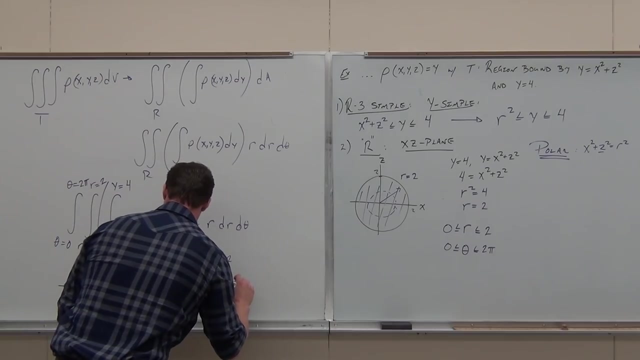 sorry, y goes from r squared to 4.. Did you all make it that far? Which one do we plug in first? the 4 or the r squared? The 4. The 4.. Okay, I think I get that. 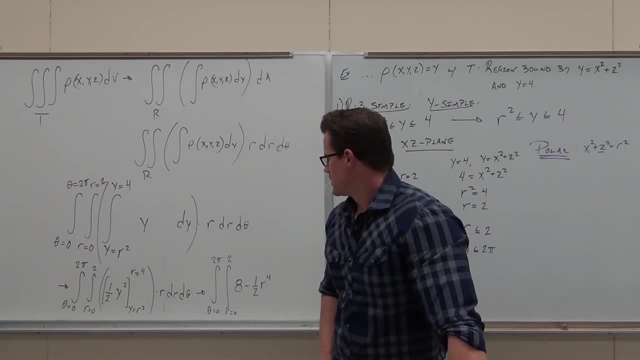 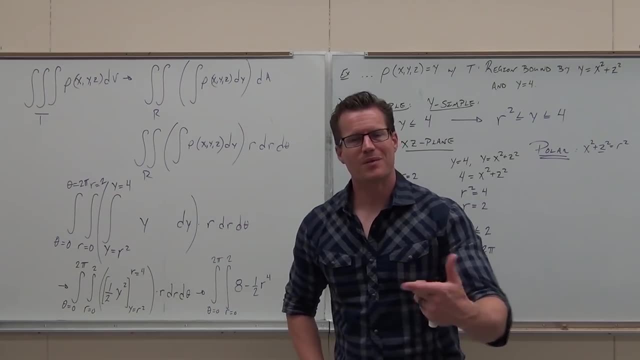 Did you get that 8 minus 1 half r squared, Or, oh sorry, the 4.. Tell me what's the next thing you should be writing: r, The r, The r. Did you remember how I told you the r is one? 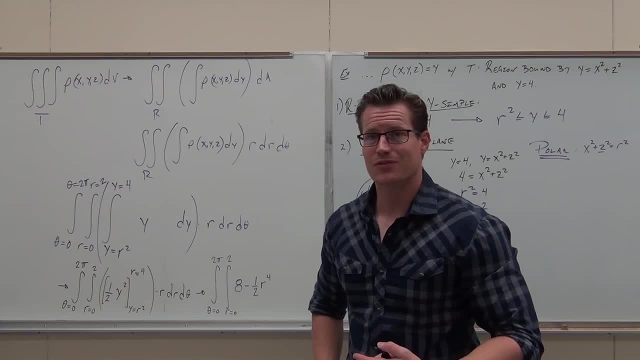 of the easiest things to forget about. Have you forgotten it yet? No, Good, Good for you, Because I made such a big deal of it. I said: don't forget the r. I'm mad at you. Yeah well, you'll get mad at you because you get the. 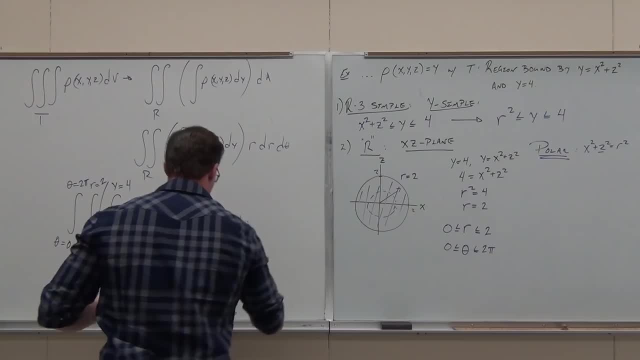 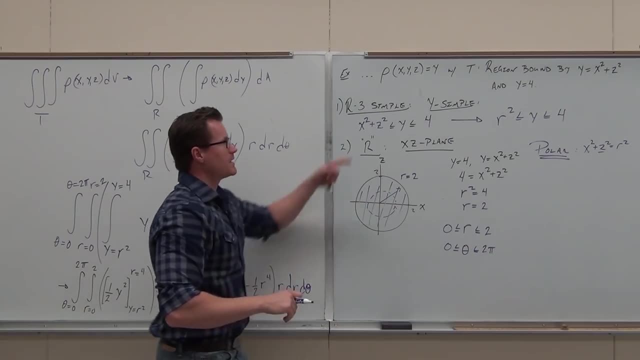 and you go. oh my gosh, I'm going to forget the r And it's just such a pain. But that r, that's r's got to be there. r dr d theta. Any comments? questions about this whole thing? 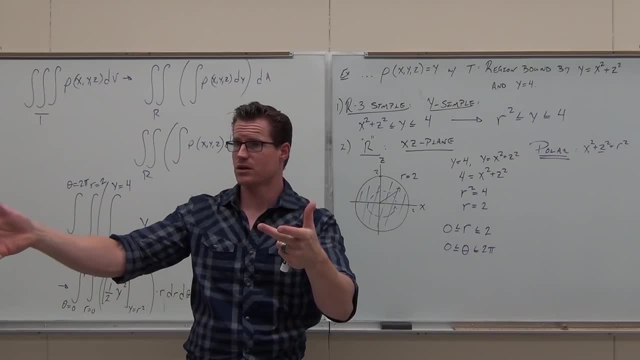 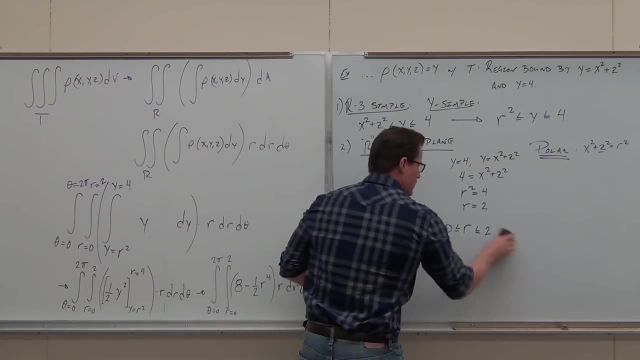 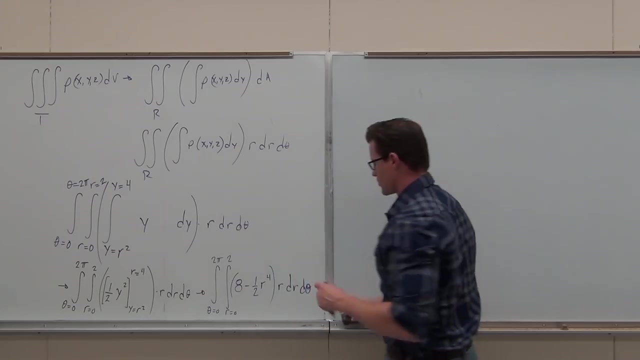 So r simple: the region you feel confident doing the polar regions these days, Even if they're not xy, you can do xz, whatever. Just change the way you're defining your polar functions. You can do any of those things now that you're coming up. 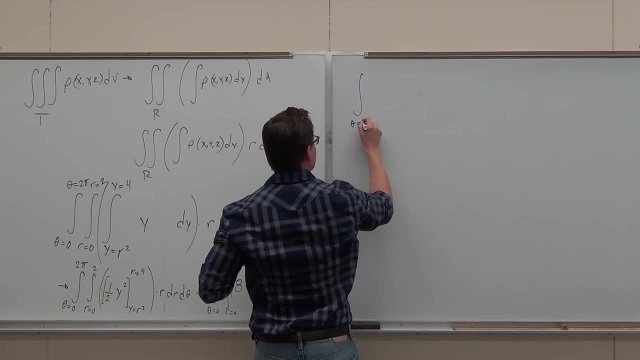 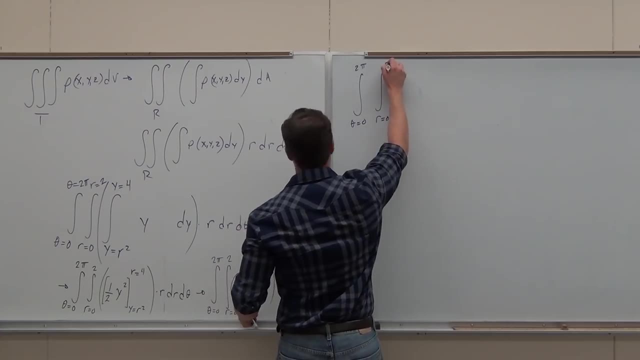 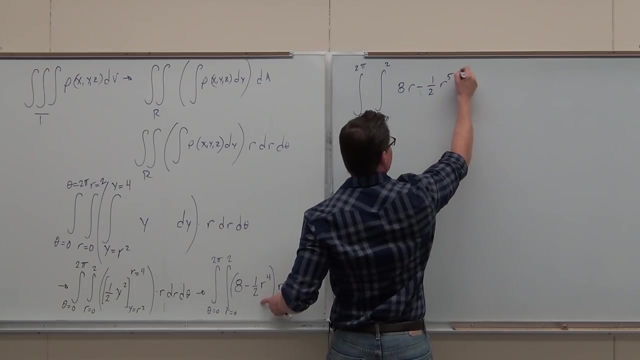 you just can't. We're all going to be in the same group. Let me crash an integral, OK. well, this is theta equals 0 to 2, pi 0 to 2. for our r, I know that's going to be 8r minus 1 half r to the fifth, dr d. 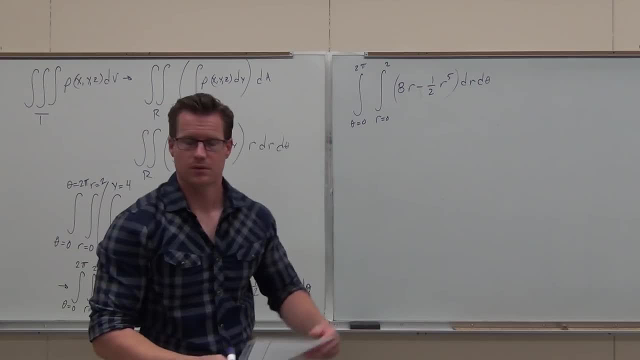 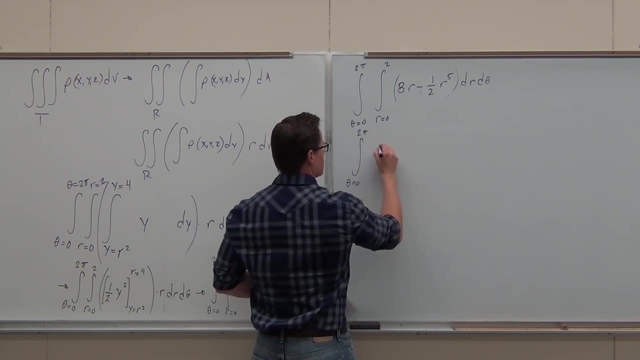 theta. Still so far, so good. y'all know That's our first idea. OK, OK, Thanks, so much Thanks, Let's know. okay, So that is 4r squared minus 1. twelfth r to the sixth. 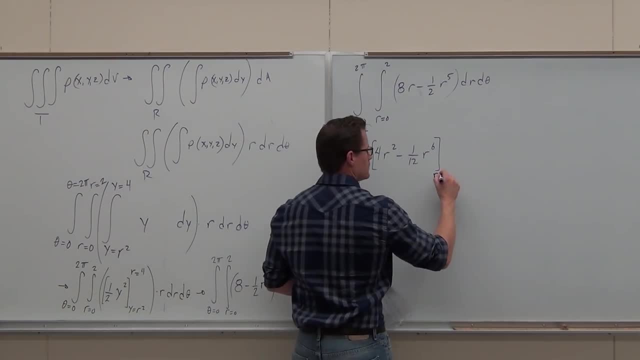 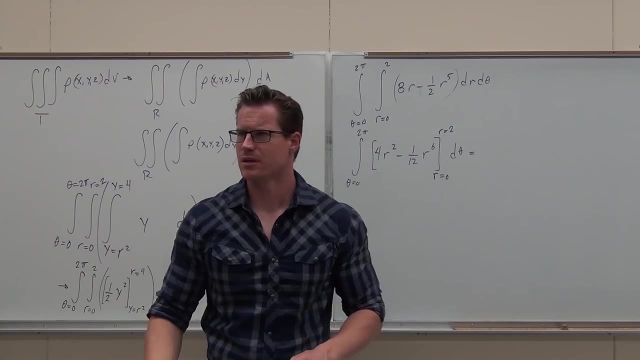 and then we're going to plug in, for You know, I love it when that happens, when there's no other thetas or anything, and you just get all r's and you plug in, for r equals a number and zero, you're going to get left with a constant. 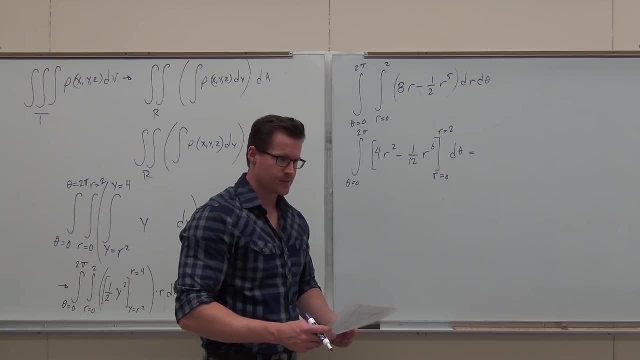 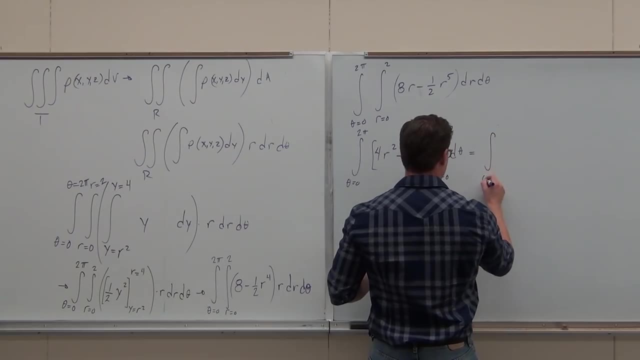 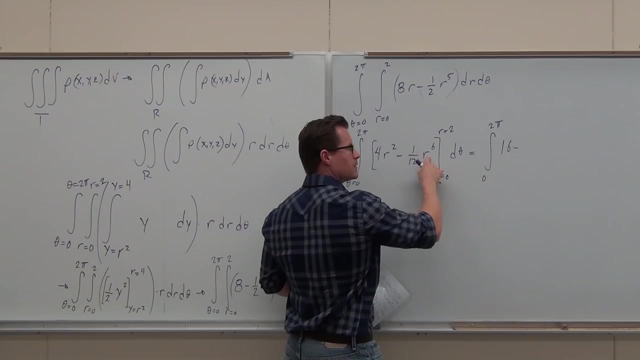 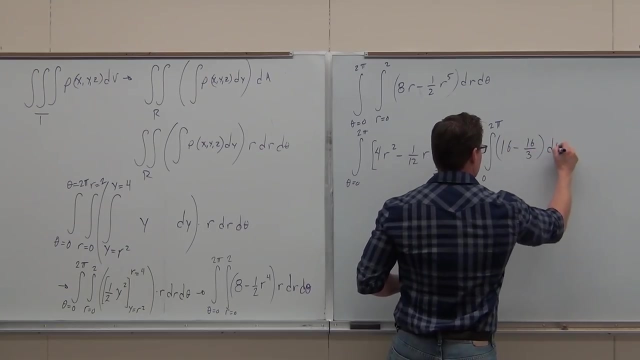 That constant, if I've done my math right, is 32 over 3.. I don't remember, I'll do it again. That's 64 divided by 12. 16 thirds. Can you correct me if I have a mistake? 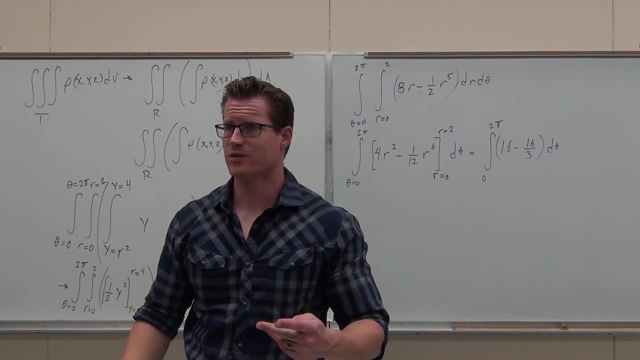 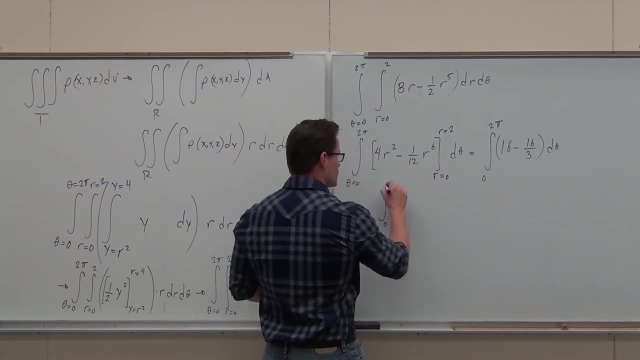 Did you get the same thing? Yeah, Did you bust out your fraction button in your calculator? 48 minus 16 is 32.. So we get zero to 2 pi 32 over 3.. Yes, no, Did you make it that far? 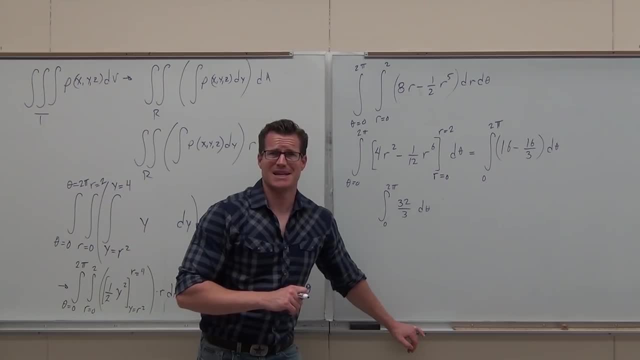 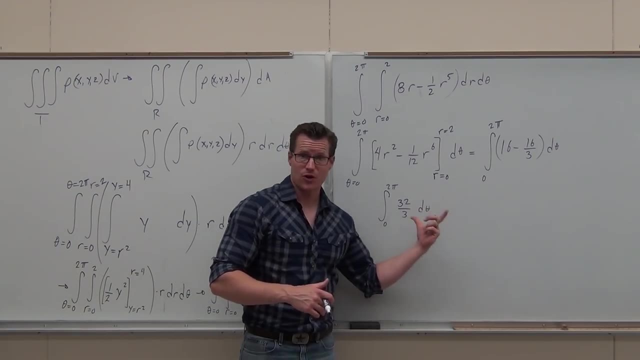 Yeah, What's your last step Over here? Easy step, You know easy step, but we make some mistakes on this. When you're integrating a constant d, whatever, the whatever is important, It's telling what your variable is. 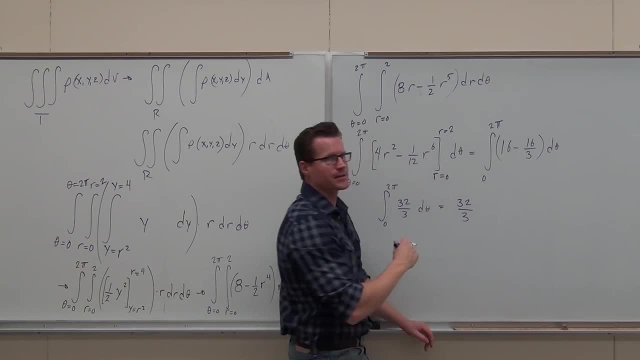 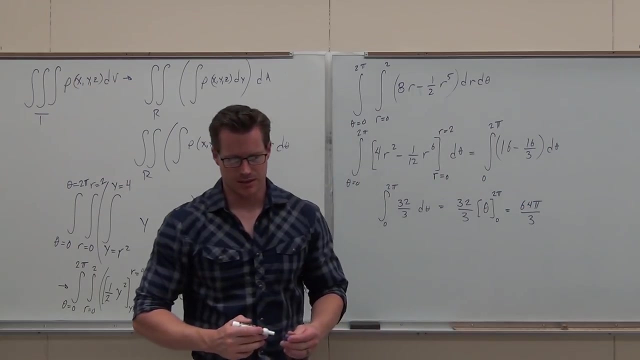 So this needs to give you 32 over 3. what Theta, Theta, yeah, And that theta is being taken from zero to 2 pi. So we're going to get out of this 64 pi over 3, what does it mean, please? 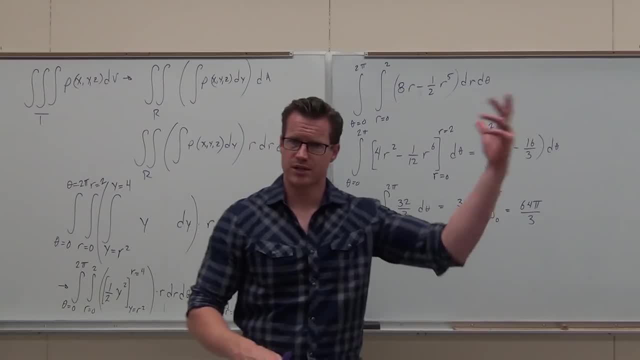 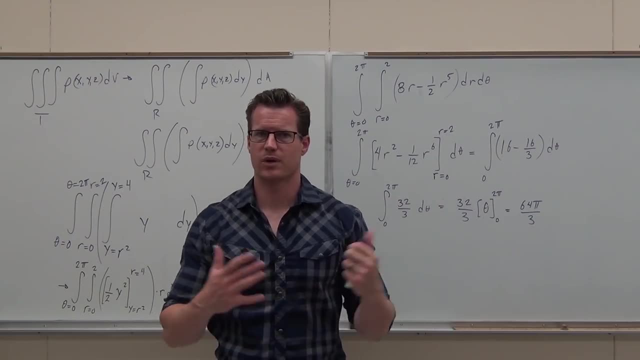 Mass. That's the mass. That's the mass of the region that I wrote on the board earlier. depending on the fact that the mass density function of that region is given by rho, x, y, z equals y. That's what that came from. 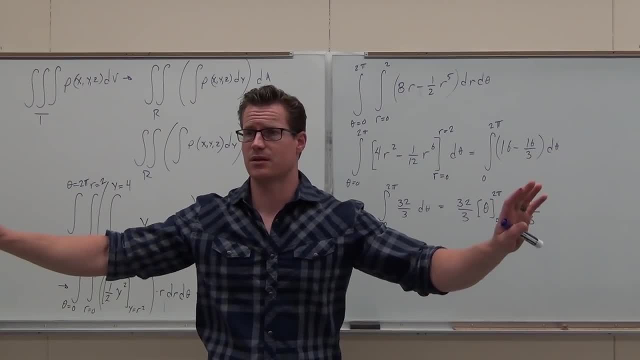 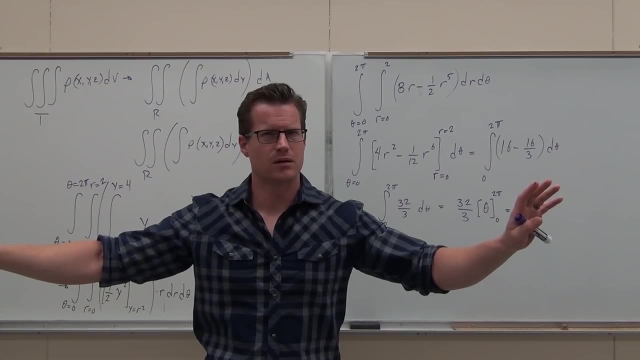 Do you feel like this has been explained well enough and you guys completely understand the concept? Concept Concept is big. Can you do all of it? What's your first step? again, R3.. R3, simple, And then you have a. 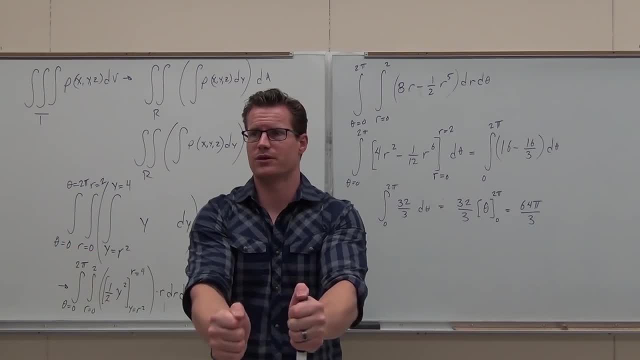 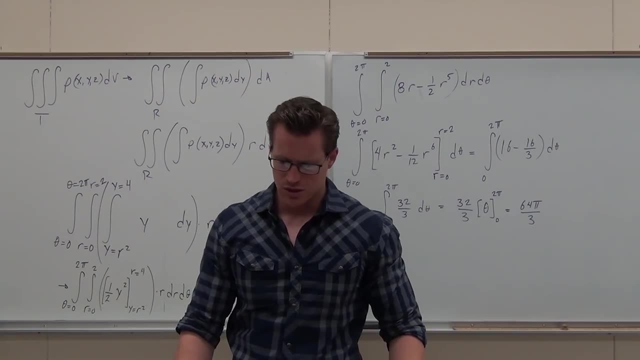 Double, Double, integral With the region And you define it however you learned in 14.2 and 14.3.. We're going to stop here for today. We're going to come back next time. We'll honestly just deal with a lot of set up, set into the problems. 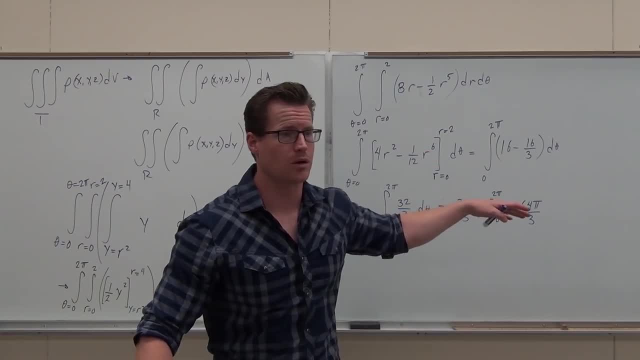 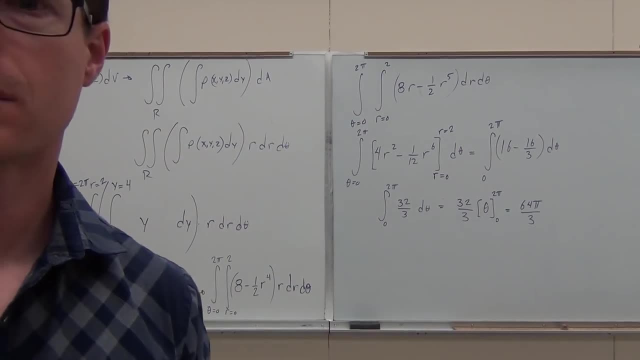 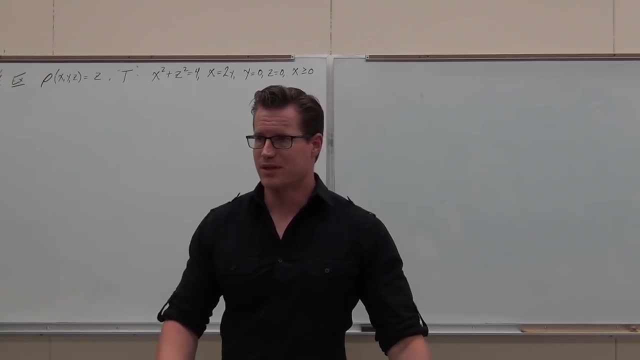 because that's the biggest thing. We're going to skip a lot of this. It just it takes too long, So we're going to worry about set up, set up, set up next time, All right. so welcome back. A few more examples and we're almost done with this idea. 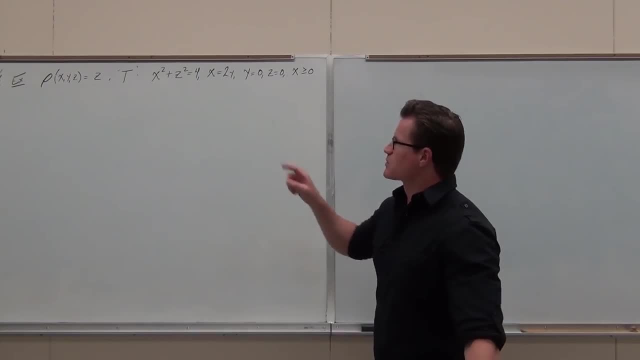 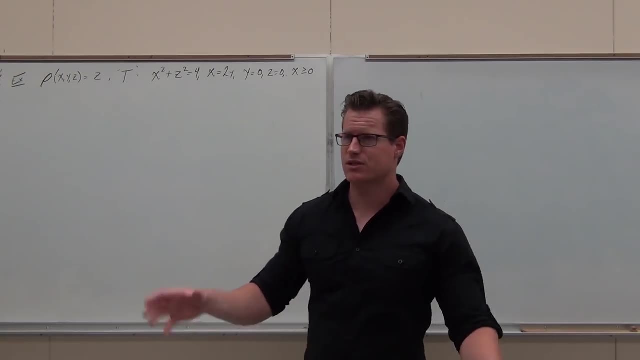 So we're going to focus on mostly set up and I want to set this problem up. If you recall from the triple integrals, we had a couple ideas about what these things did. What they can do is give us some measurement of like a volume idea under a 40 surface. 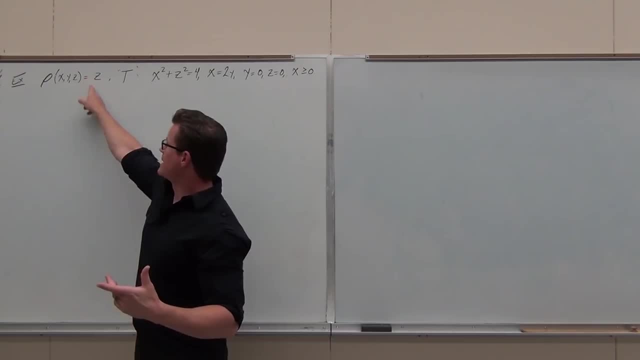 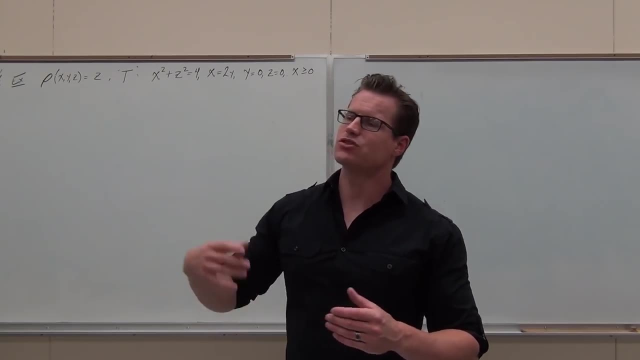 which is kind of weird. or if we have a mass density function for a region, what it will do, what these triple integrals will do, they'll find the mass of that region, And that's generally how we think about it. So the key here is: set up, set up, set up. 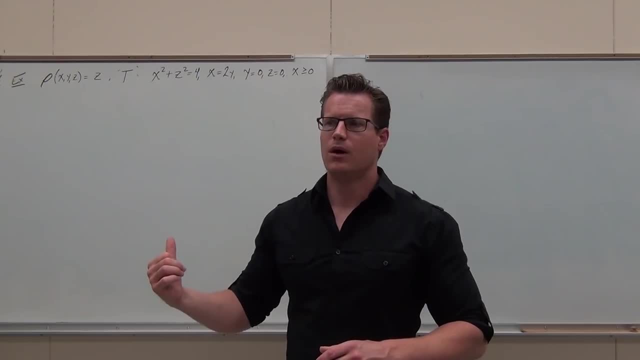 And I want to talk about this one. This is a very interesting problem. What we're going to do is we're going to set this up two different ways. We're going to look at the only two ways it really makes sense to do. 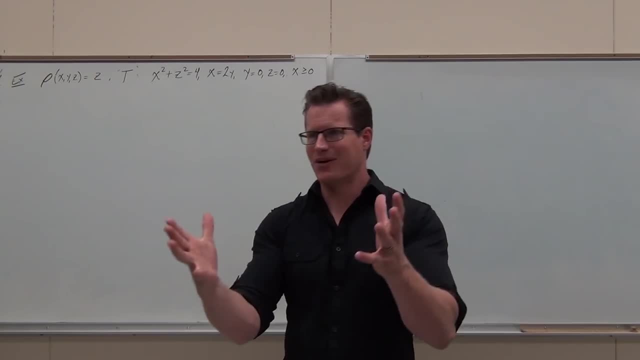 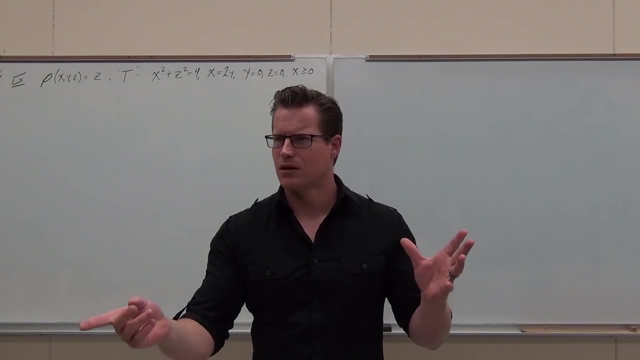 If you remember- and I hope that you, I need you to remember- what's the first thing you do for a set up of a triple integral, What do you do? first Say it again: R3 simple, R3 simple. So we choose either X simple or Y simple or Z simple. 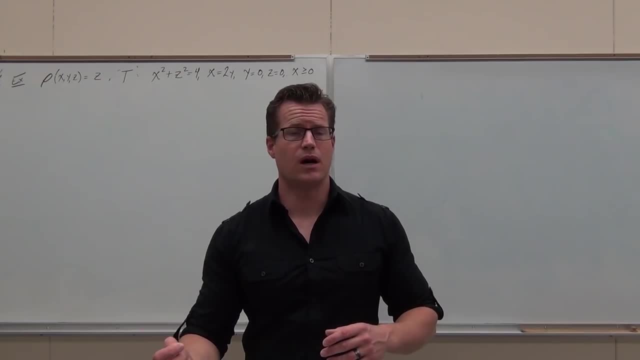 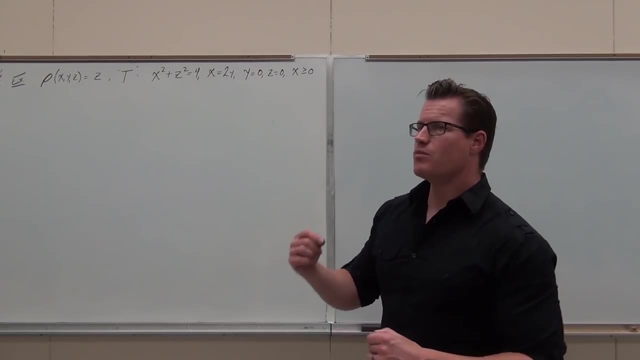 What's the one we typically try to? stay with? Z simple We try to, And that's the first one That's an option for us here. Y simple is also an option for us here. X simple not so much, and I'll explain why. 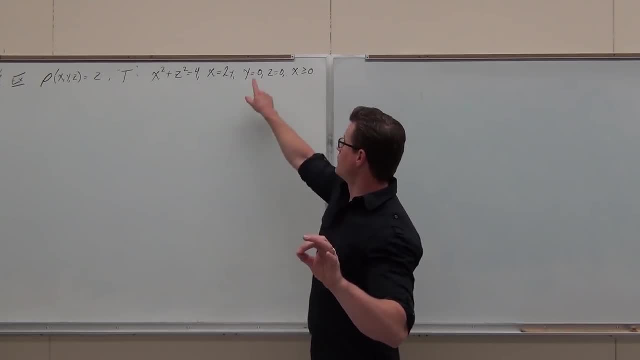 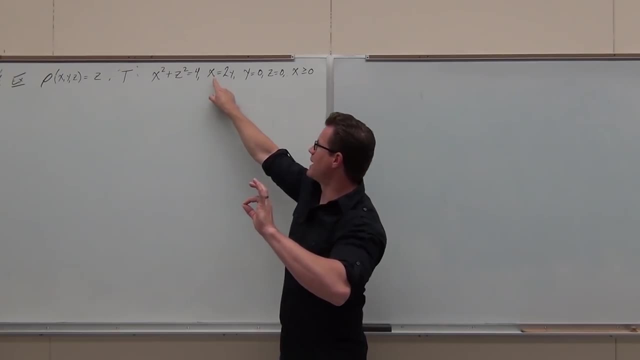 Y simple and Z simple will be okay, because I have a Y equals 0 and a Z equals 0. So Y simple, Z simple. that would be nice because I have a 0 at the bottom, like that. X simple. I'd have to go between two functions of different variables. 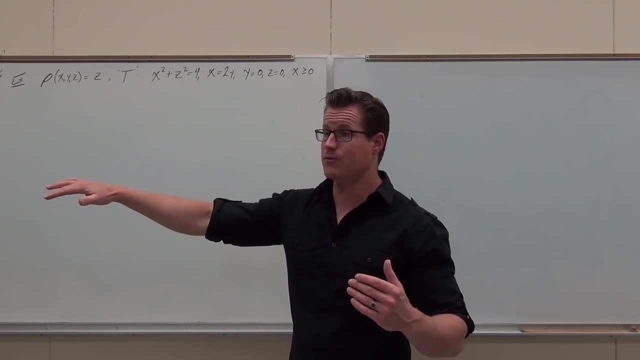 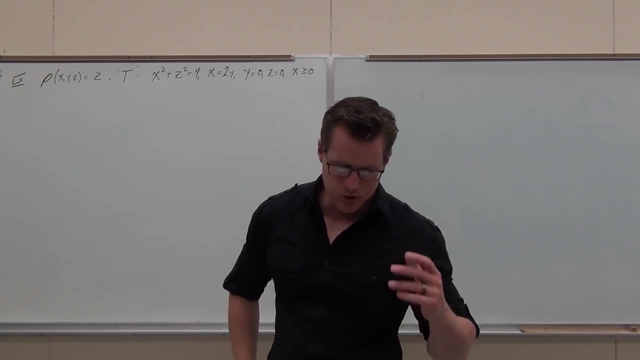 That would be a little bit awkward. So right now, I'd put X- simple off the table. I'd be focusing on Y- simple or Z- simple. Now that you understand what I'm talking about. So let's go, Let's go ahead and we're going to do, we're going to do Z simple first, just the setup. 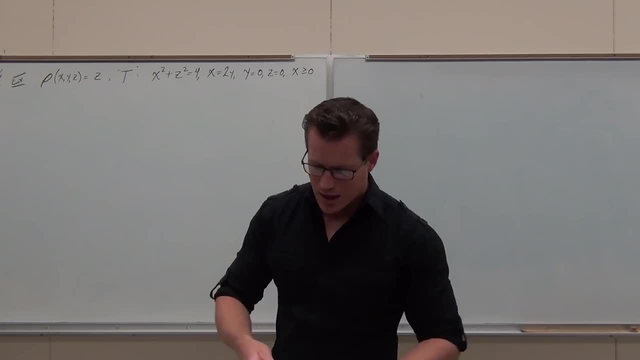 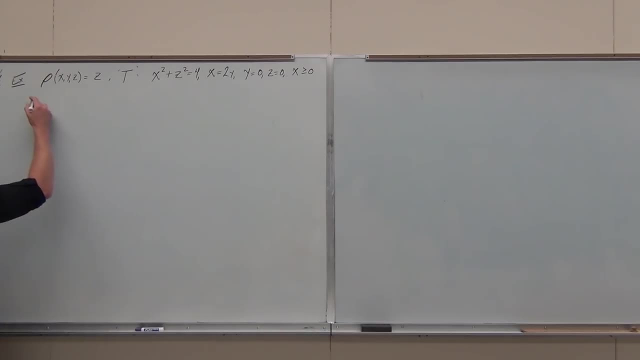 And then we're going to do Y simple and we're going to see how the setup changes. So let's focus on the Z simple. So, number one thing, any triple integral, we always do an R3 simple first. Then we're left with a region that's on a coordinate plane. 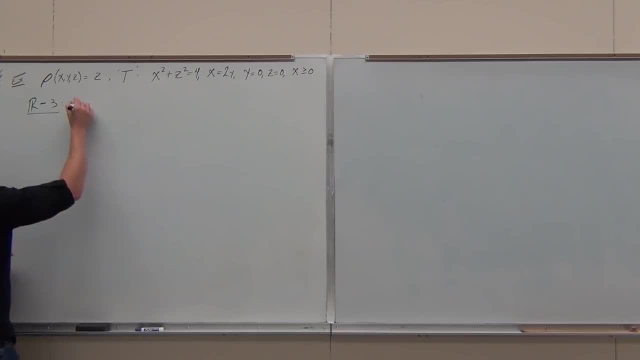 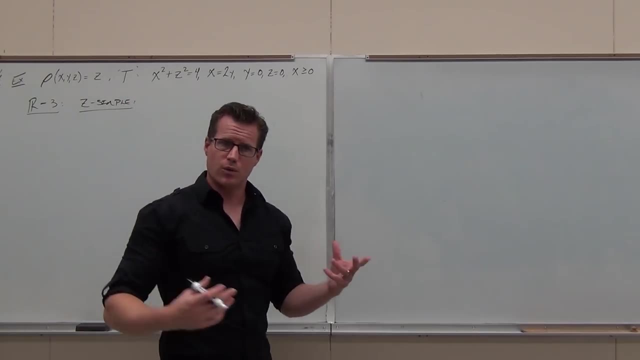 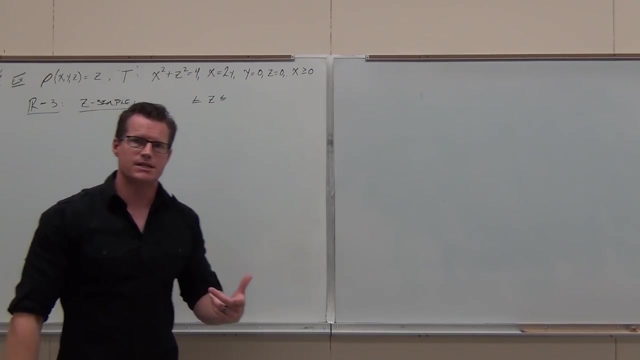 So R3 simple, Let's just try the Z simple for now. If we're going to do Z simple, then ultimately what we need to get out of it is Z being matched between two other functions. That's what we would need to get. 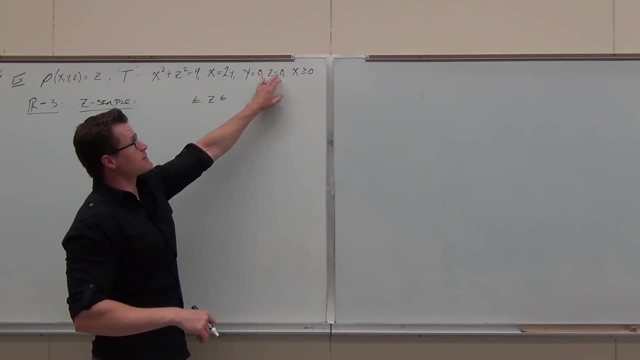 So let's look at our functions. I've got well, that doesn't have a Z in it, That's got a Z in it, That doesn't, That doesn't, That does. These are going to give us our two functions of Z. 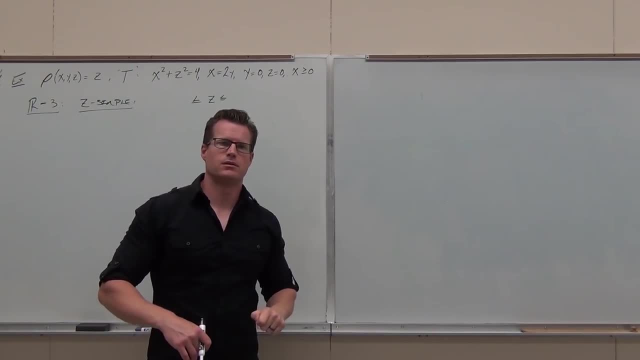 And now that you understand what I'm talking about, What's the smaller one? do you think Zero, Zero Generally? that's kind of a segment, A safe bet that zero is going to be your bottom bound between two functions in R3, simple. 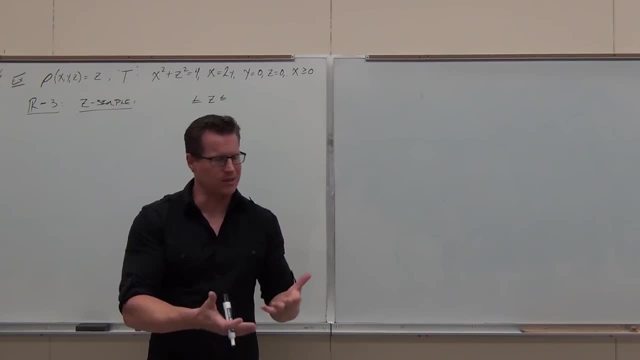 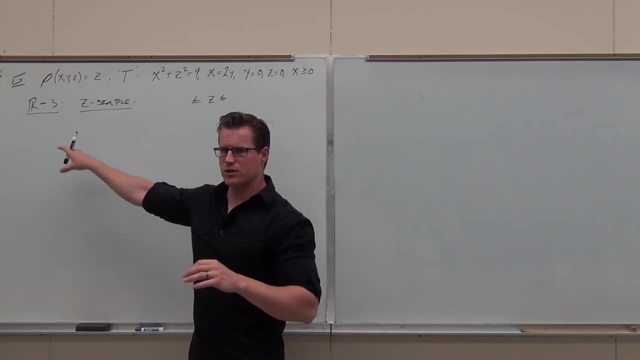 We typically try to keep in the first octant. That's generally what happens, or at least above the XY plane. If that's not the case, if you don't know the next step- and we did this last time- go down to your region, figure out your region and plug in a point. 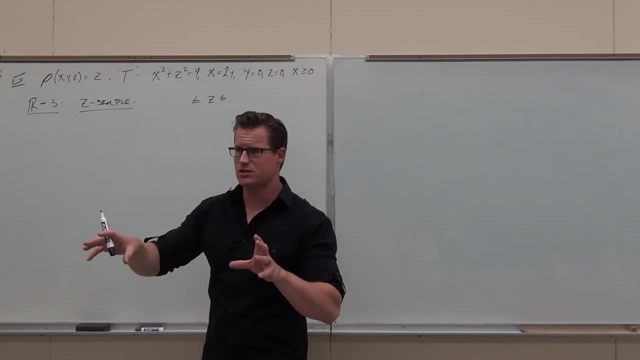 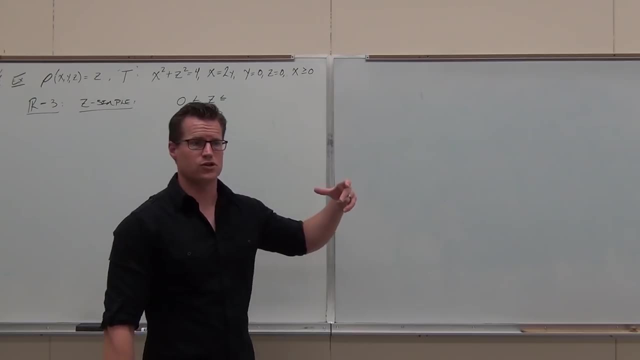 That will always tell you what's the bigger function of Z and what's the smaller. Does that make sense to you? We did it last time, So for right now, yeah, I'm pretty darn sure that Z equals zero is going to be our smaller of those two functions. 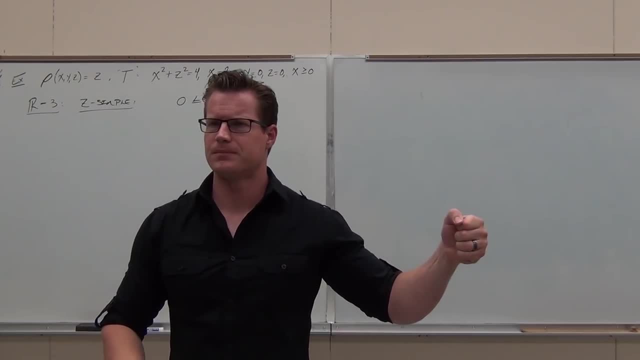 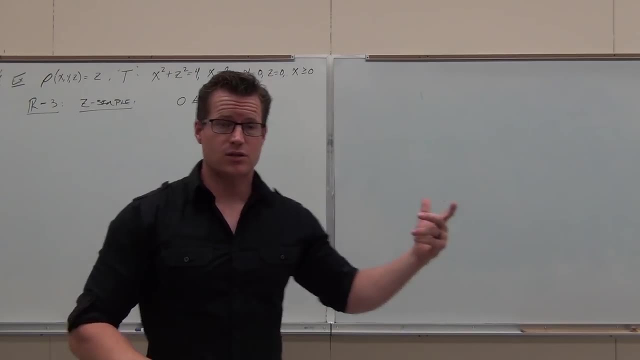 What would I have to do to figure out the bigger of the two functions? What would that be? You can say it louder, because I can't hear a darn word. you're saying Solve for Z and then plug in: Okay, Solve for Z and the only other one that has it. 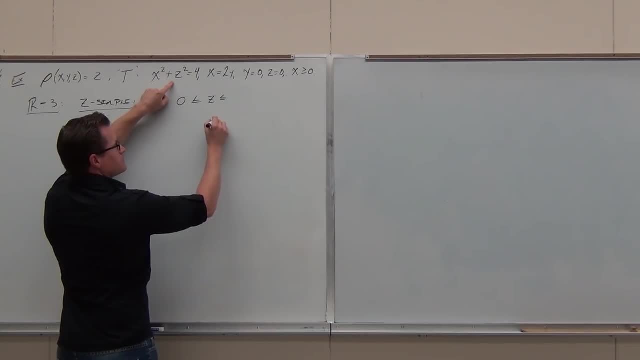 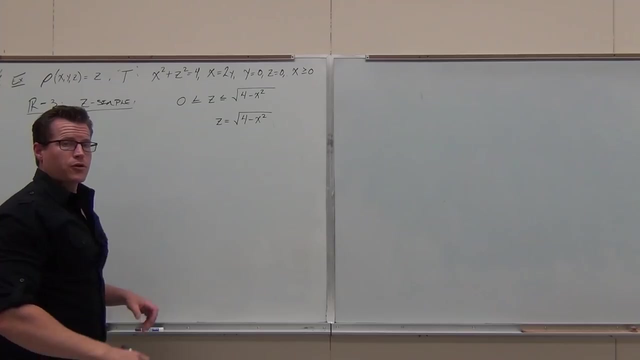 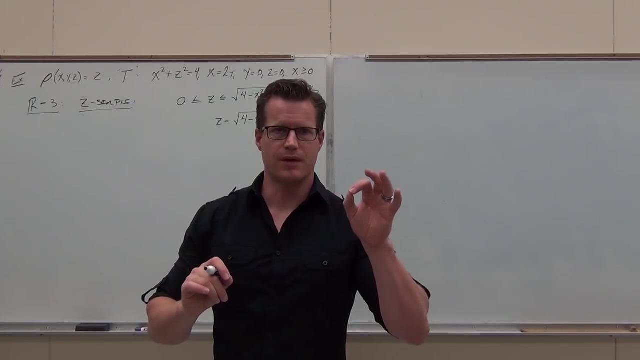 So Z would be well square root of what's in that square root. Four minus X, Four minus X. So for R3, simple. If we choose Z, simple, Z's got to be matched between zero and the square root of four minus X, squared heading. on that you're with me on that one. 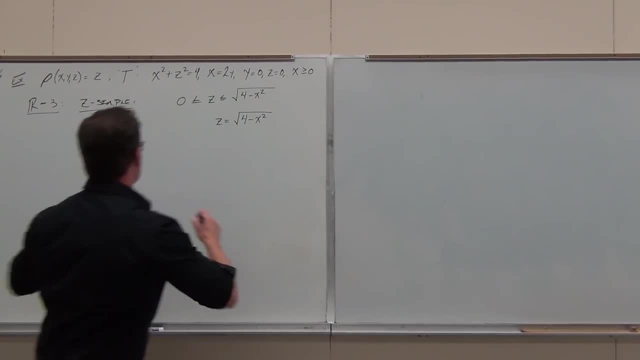 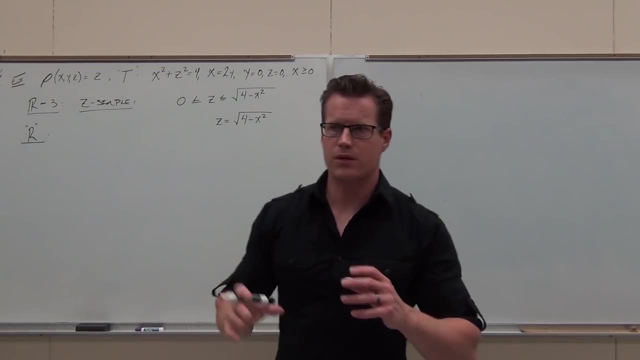 After the R3, simple. what's the next thing that we do? Come on quickly. So our region. I always like to list out the plane that that region's going to be on. So if I choose Z, simple, our region's got to be on what coordinate plane. 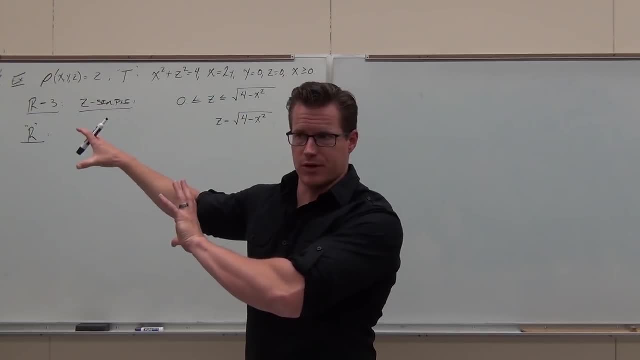 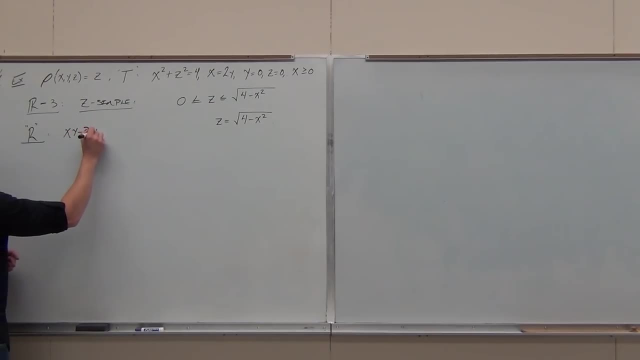 It's always on the plane. that doesn't include that variable. So if we have Z, simple we're on XY for sure. So our region's going to be on XY, XY plane. that's great. Hey, what do you do for regions? 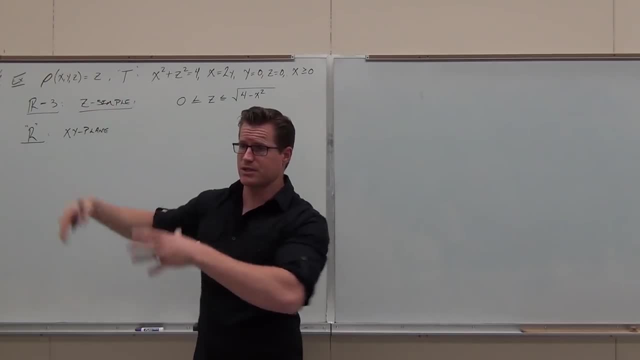 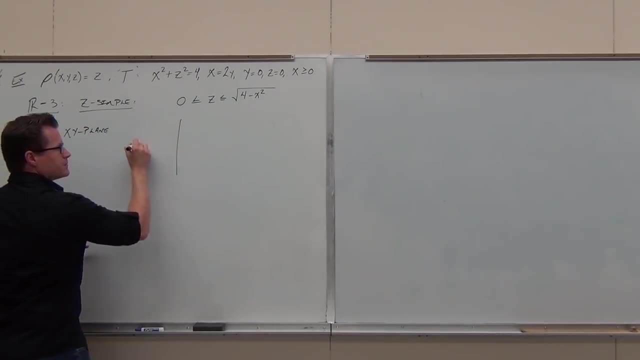 Like every time that you're setting up, now that we've got the R3, simple, we're setting up a double integral. you do what every single time: Draw a region, Let's draw it. So when we draw our region, Yeah, it's going to be on XY. 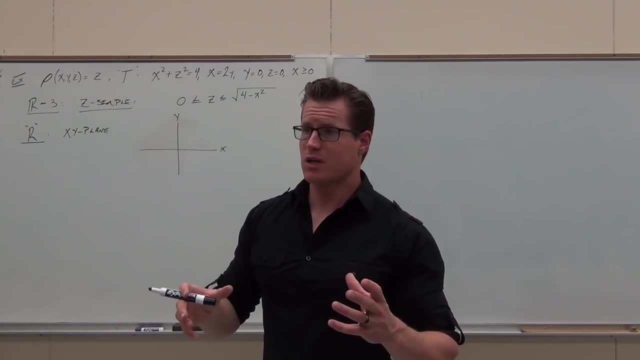 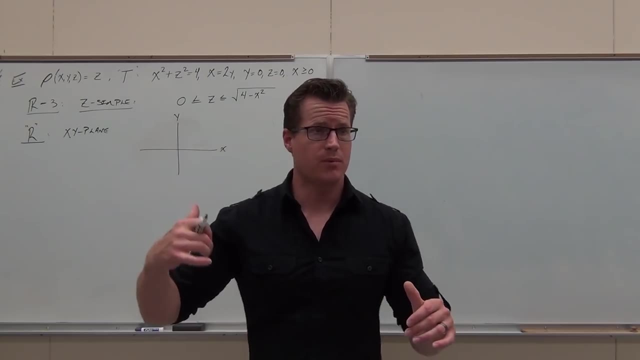 We're going to use all of these functions that actually make sense on the XY plane. So basically, anything that involves X's and Y's you can put on that plane. Z equals zero. well, not so much, because that says you're on the XY plane. 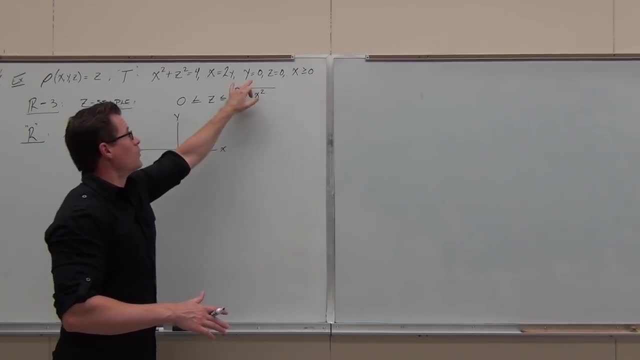 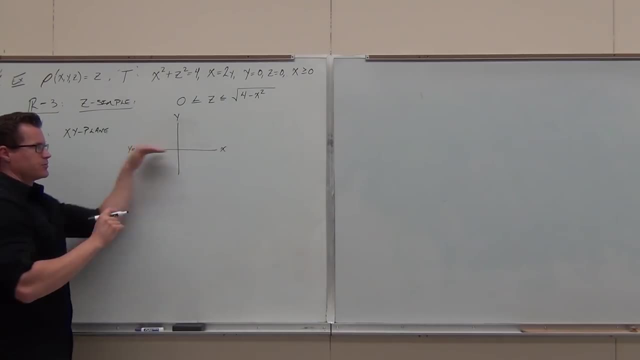 X greater than zero that we're going to use here in just a second: Y equals zero. that's relevant. What's Y equals zero? give us Y equals zero. So I know that already we have that line. We have X equals 2Y. 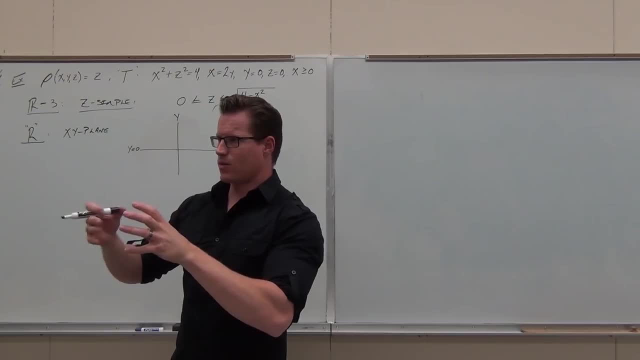 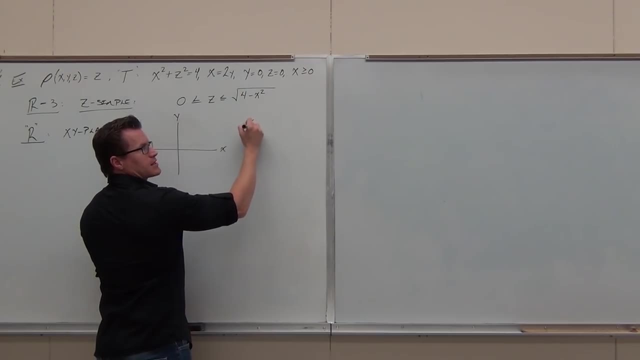 So we're going to draw that one X equals 2Y. since we have the X and the Y variables, it's pretty easy to draw. Me personally, I love things in terms of Y to graph them. So from X equals 2Y, I'd probably think about it just 1 half X. 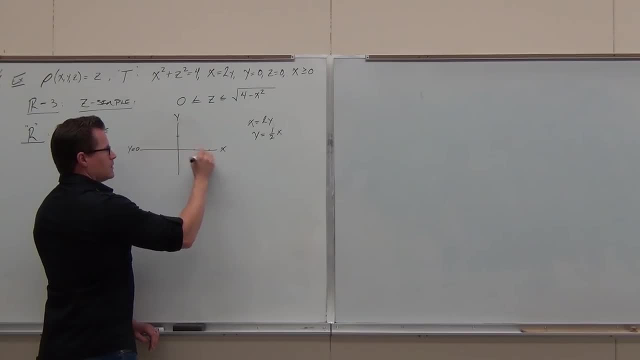 Well, We get that diagonal line. That's all that it gives to us. So we got that. on the XY plane, We got that Y equals zero. We have this. We're going to definitely be above X. sorry, to the right, of X equals zero. 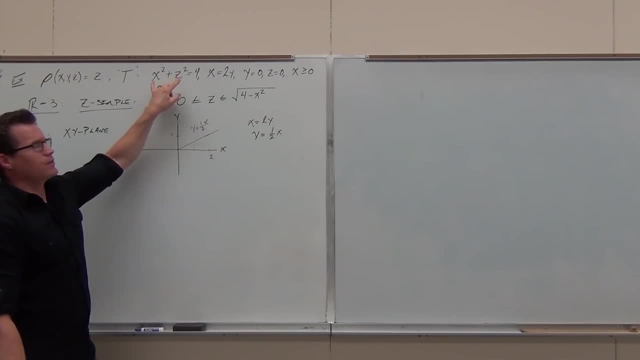 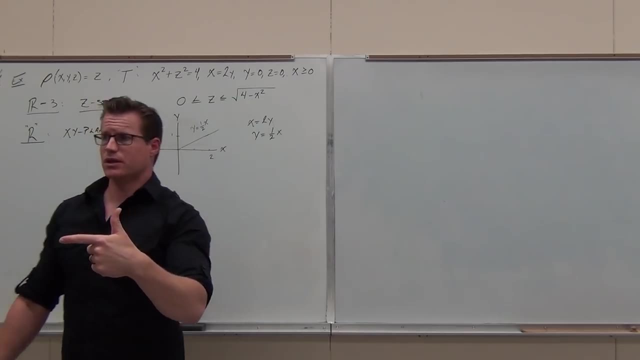 It's going to be that way. This gave us our diagonal line. Now, does that give us anything? Hey, if it has an X or a Y in it, it's going to give us something in the XY plane. The key here is, though: on the XY plane, what's the value of Z? 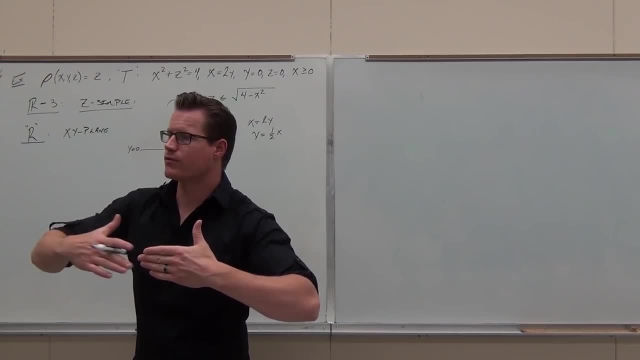 Zero, Zero. So when you're on that coordinate plane you need to zero out all of that, That R3 simple variable. So for us we go: yeah, this, that's great. This was, this is one of the lines. 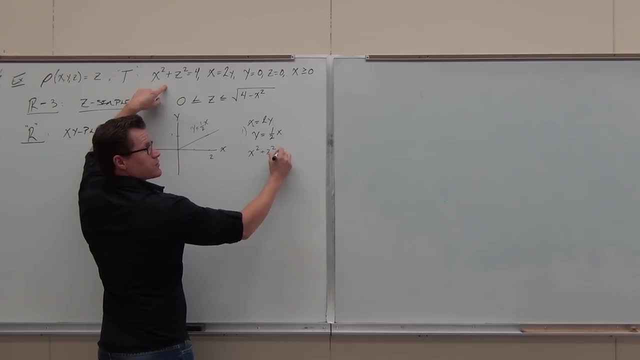 This right here, though. this is: X squared plus Z squared equals 4.. But hey folks, we're on the XY plane. Z is zero, And that gives us two other values. That gives us: X equals positive or negative, 2.. 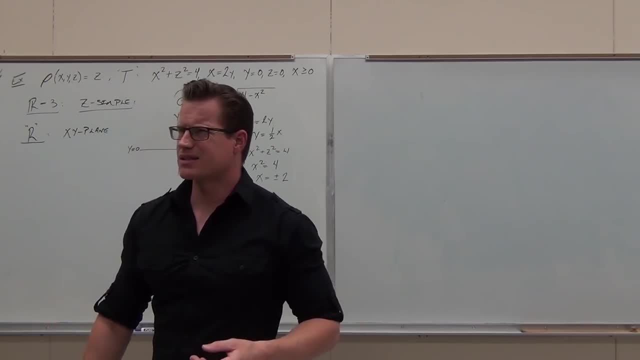 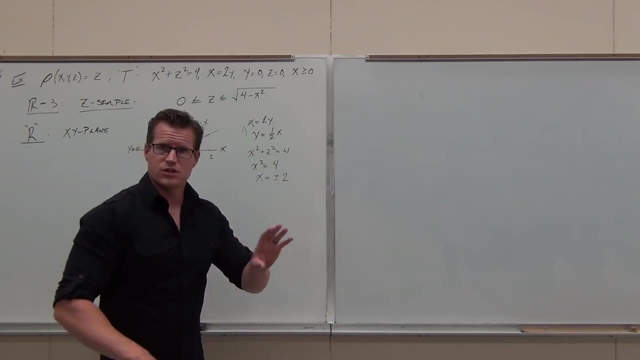 Well, hey, what are. what is that? on the XY plane, What is? X equals 2 and X equals negative 2? What's that? Yeah, those are our vertical lines. That's exactly right. Only there's there's one condition over here. 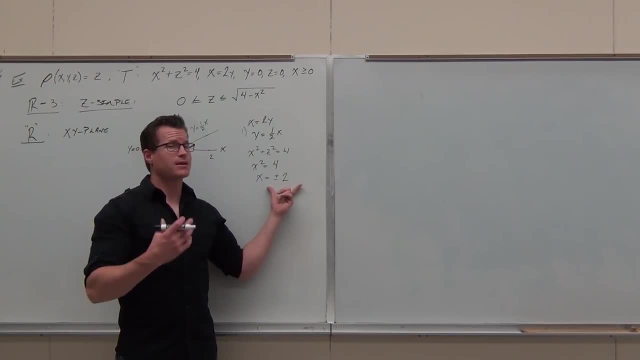 If X equals plus or minus 2, I have a condition that's going to eliminate one of these. What's that condition? Yeah, so I don't care about the one over here, This guy don't worry about it. X has got to be positive. 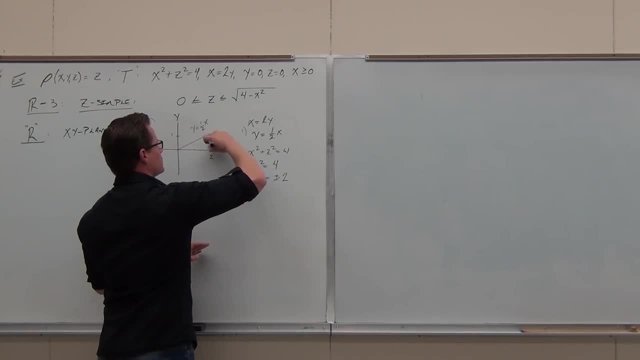 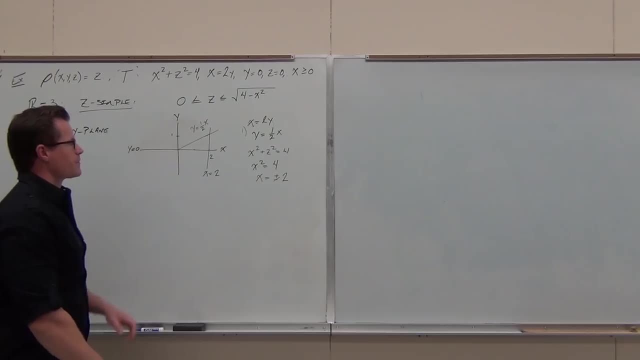 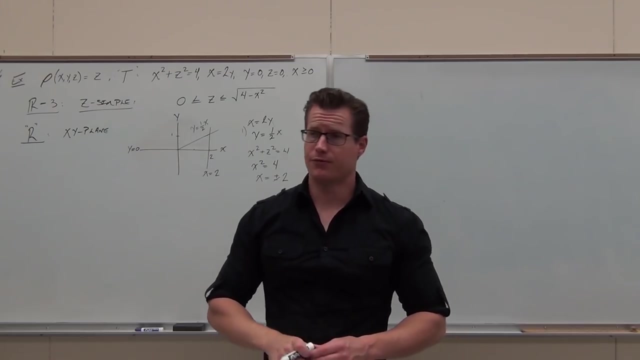 That's just giving me this vertical line at X equals 2.. I'm going to put that over here, Okay. So if you're the person who, man, you can't visualize that, I have no idea. Go down here first. 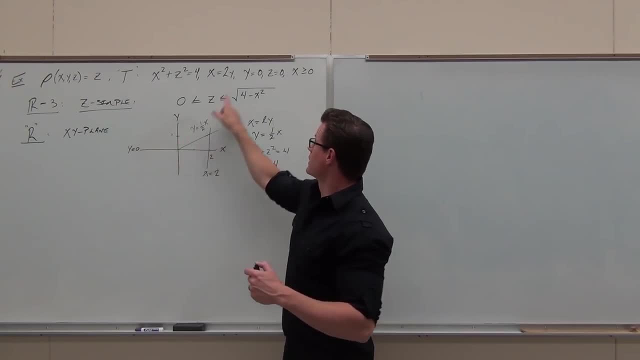 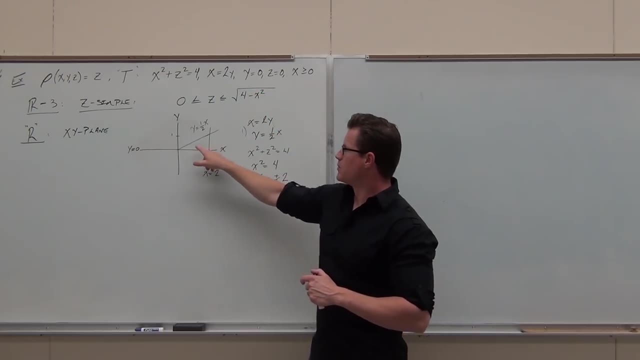 Take any point on the inside of this region and plug it into both this and this or this, and solve for Z here, which I'd already done earlier. Plug in any point on this region and it will show you what the higher function is. Does that make sense to you? 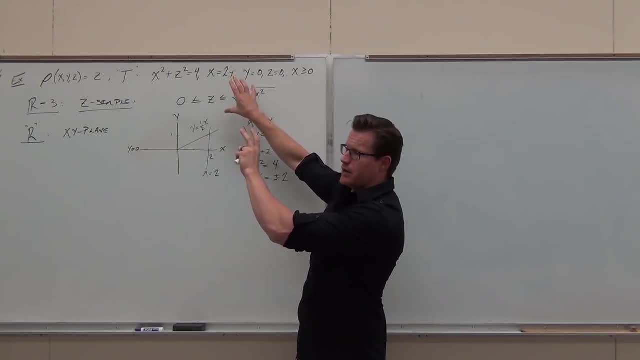 You can always come back and fill this in later if it's not good enough Intuitive for you. Fine, Do your region first, plug in a point to your z functions or your R3, simple variable functions, and it's going to tell you what's the bigger, what's the smaller. 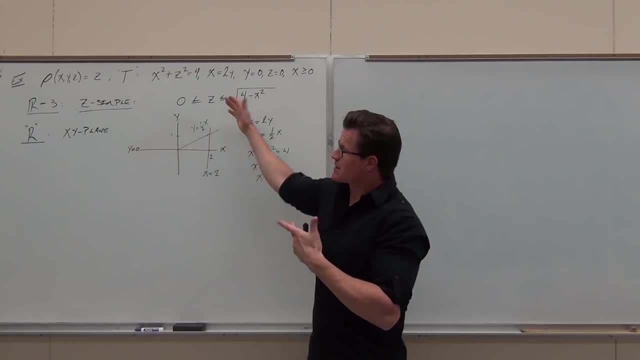 So fancy to understand that concept. Here we got kind of lucky. we got the zero. We know that's larger than zero, It's a square root. I mean it's going to be there. This right here we got our R on the x- y plane, no problem. 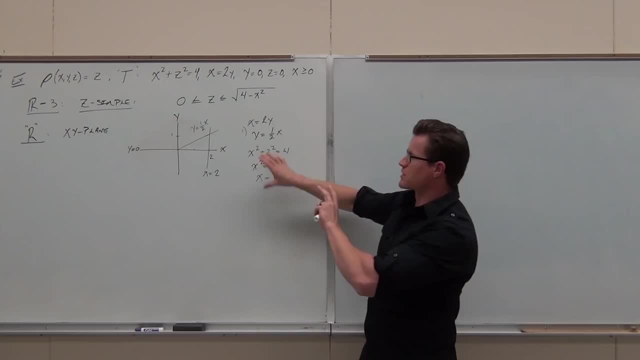 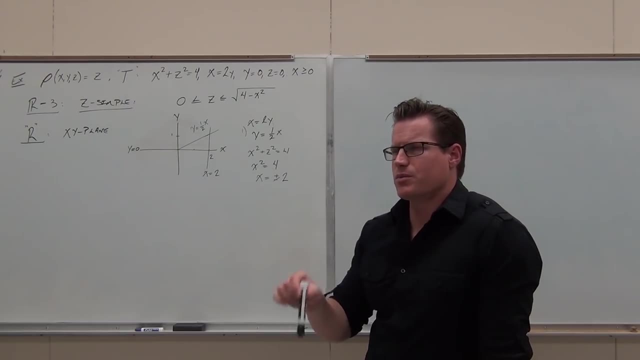 Anything involving x and y. we graph that We let z equal zero gives us some more lines up there, and that's our region. Now what direction? so we know that for our triple integrals, R3 simple takes care of the inside, the most inside integral. 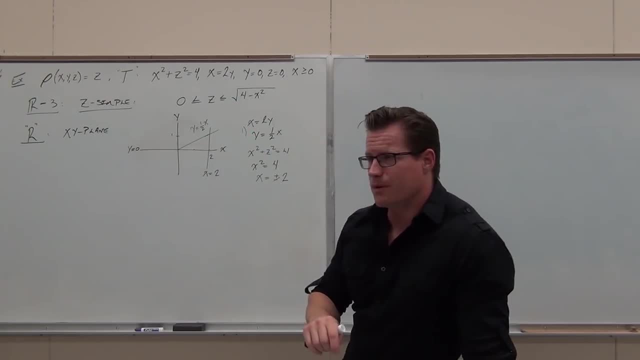 and then we get this double integral over a region That's our region and you get to pick whether you want to go along the x direction or the y direction first. Can you tell me what an appropriate choice would be? Would you want to go along the x direction, dx first or dy first? 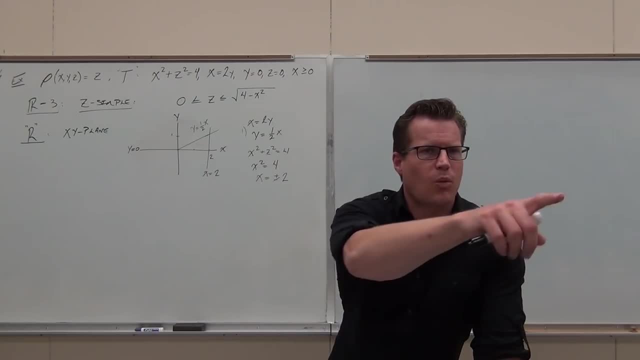 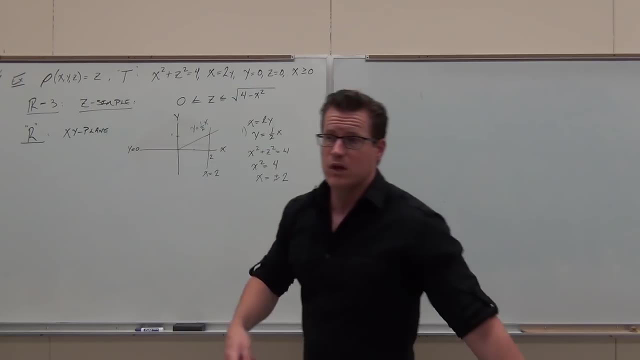 What would you do, Dy? Why, Why? Someone else besides you guys up here? why, Why, Why would you not want to go dx first? Let's look, If I went this way, if I did this, I'd enter my region by hitting this function. 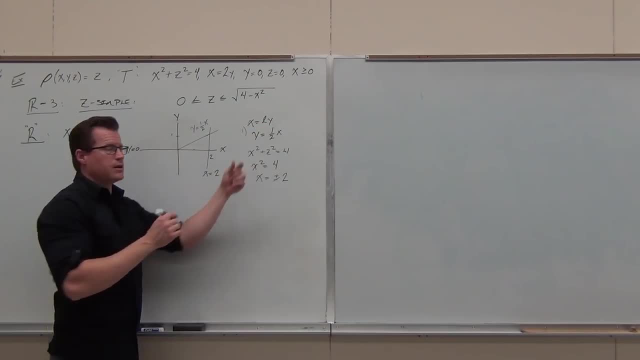 which would easily be solved for: x equals 2y. That's fine. And then I would end it by hitting 2. Doable, Very doable, And then, along the y axis, I'd go from zero to one, because this is the point 2, 1.. 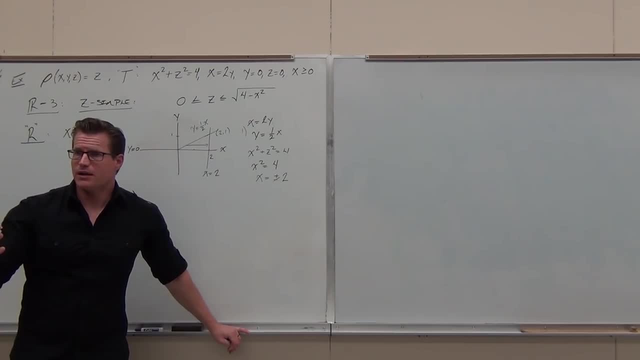 Does that make sense to you? That'd be fine. However, I'm not going to choose that way. Here's why. Here's why I always love, and it's nice because you have one function, one function. Do you notice how we're not switching functions? 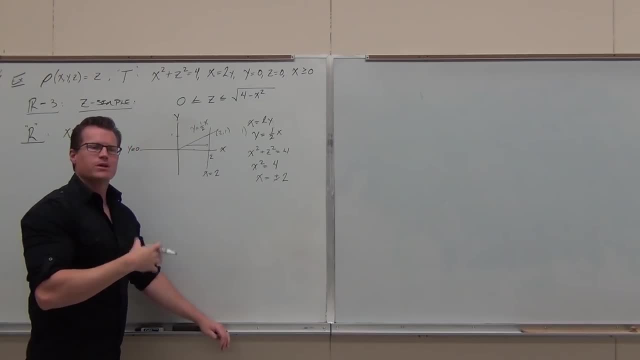 You guys see what I'm talking about. That's great, But I wouldn't choose that way. The reason why I wouldn't choose that way, can you see it? Why? Why would I want to do this way? first, dy first. 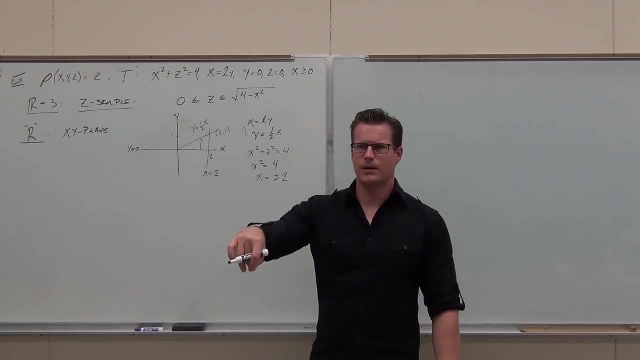 Now I'll tell you. it has to do with the lower function. What's the lower function? Zero, zero, zero. It's way easier to plug in zero, as it is another function. That's why, If I can do that and keep it between two functions and one of them zero, 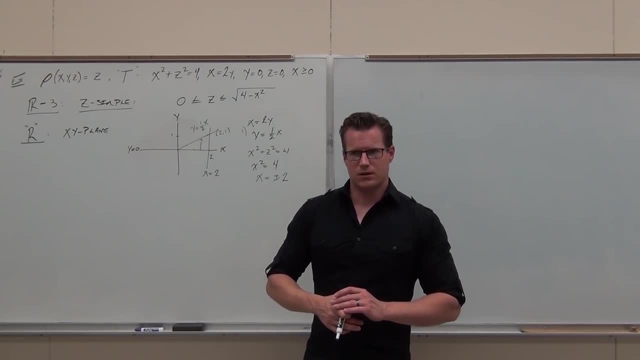 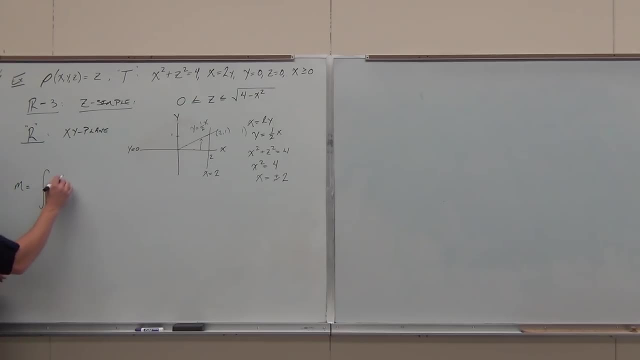 that's the better way to go. Does that make sense, Yeah or no? Yes, Okay, let's set this thing up So we're finding the mass. Always do our setup. first, Give yourself some room to do your setup, And we're going to end this thing with: well, r3 simple and then our r2 simple. 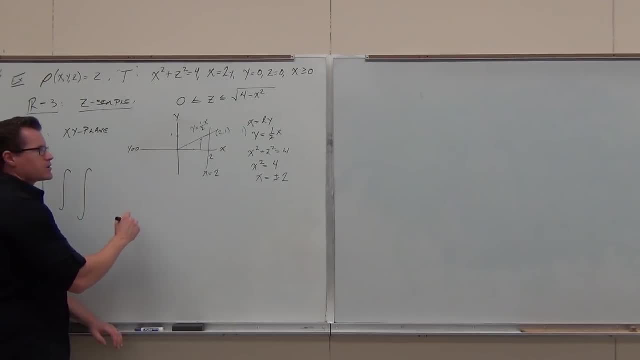 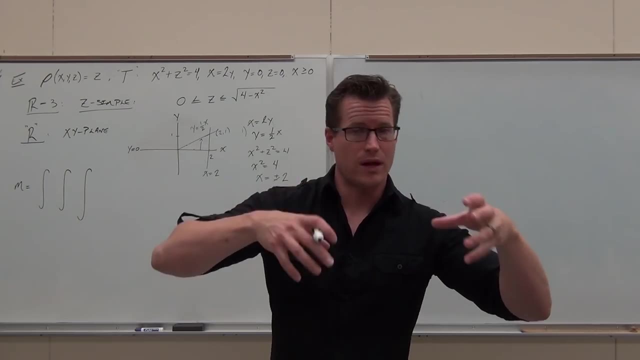 And then our constants. That's how we work it from the inside out. So what's the first thing? What was our r3? simple, Everybody come on. Our r3 simple was Zero, So we need d. what first? 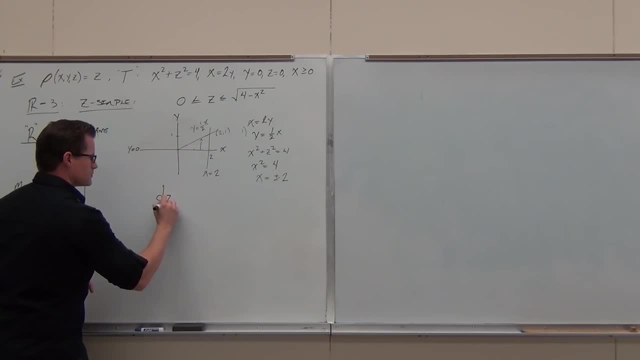 D. Okay, So from right here we got z equals and z equals The r3, simple, is always going to give it to you first. Everyone in class right now. what's my lower bound, please? Zero, zero. What's my upper bound, please? 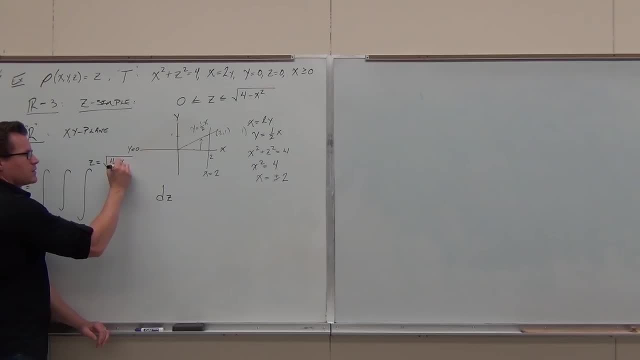 One minus two- Perfect, That looks great. I don't know if you're okay with that one Now, if you want to go an extra step on here, like I like to do before I set up the rest of it, I like to give myself some other inequalities. 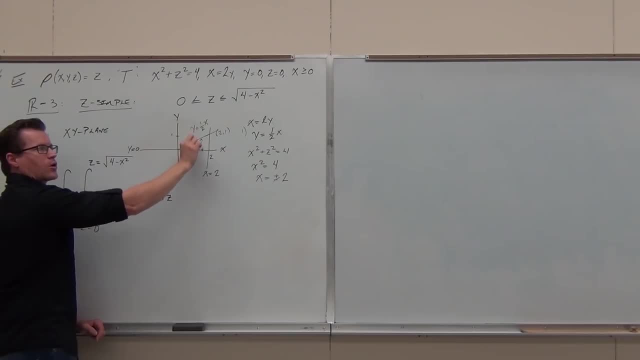 If I'm going to go along the y first, so that'd be r2, simple, On our region it's r2.. I'm going between zero and 1 half x And that also gives me something. Okay, And that also gives me something. 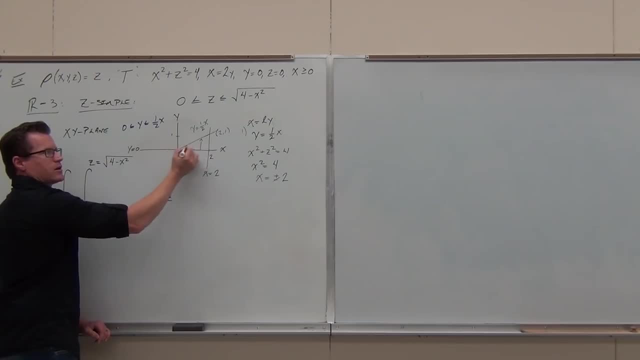 After I go between 0,, function of y equals 0, and y equals 1 half x, then I'm going to go across this region from 0 to 2 along the x axis. So same double integral set that we've always had. 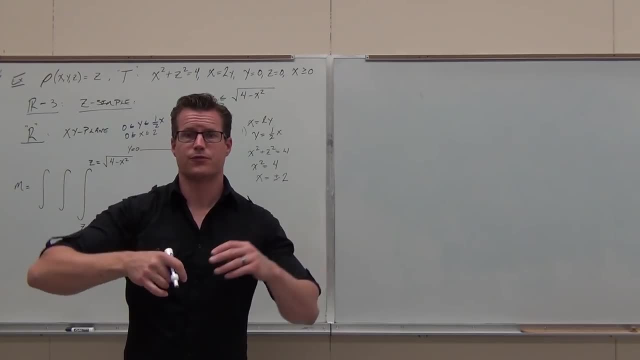 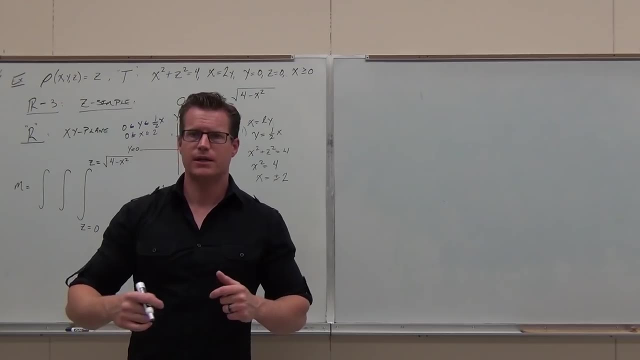 Go along one axis, then go along the other. The first axis- we call that R2 simple. The second axis: that has to be becoming constant, Always, every time, without fail, Head down, if you're okay with that one. 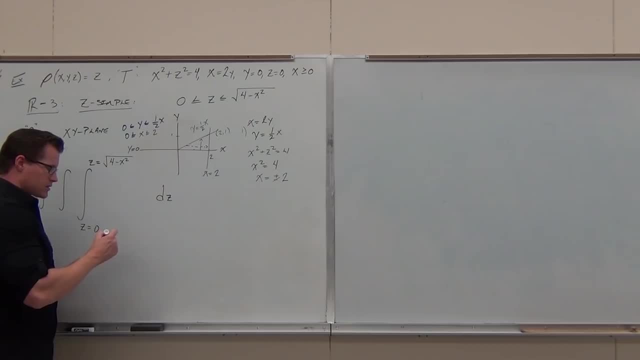 All right. so hey, now we can do the whole setup. The next thing: so if I did this and I did R3 simple, I now have dz because I chose z simple. The next one would be dx or dy. Everybody, help me, come on. 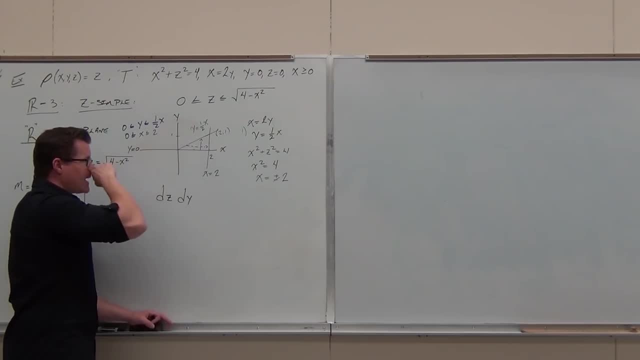 Because I chose to go through our two-dimensional region along the y axis and then we have to go from y equals that's where inequalities come in- 0 to y equals 1 half x. That's helpful. that's real nice. 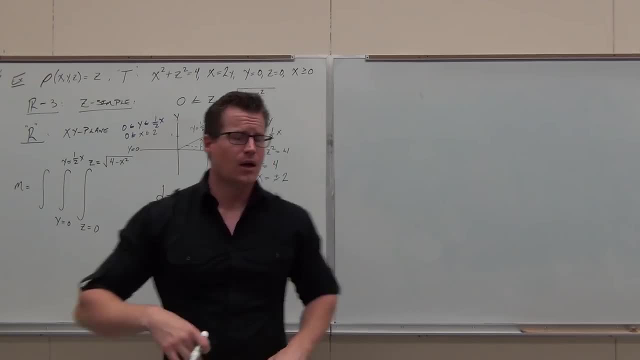 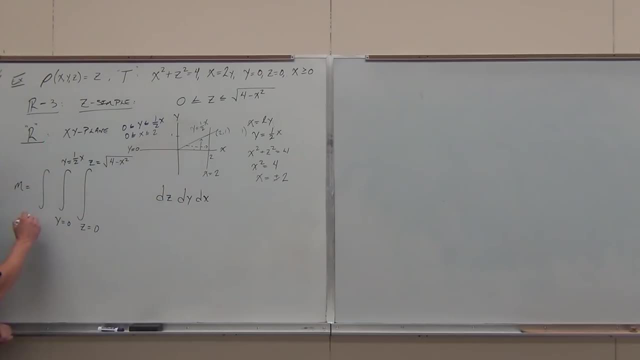 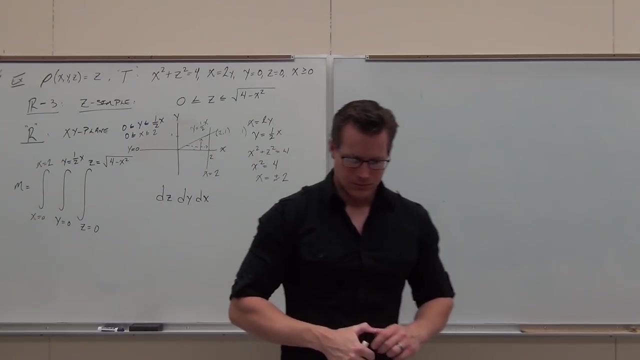 Drawing your inequalities automatically sets up your integrals from the inside out. Lastly, well, there's only one choice. I have to do dx. I know that my x's have to be constant. Sure enough, they are from 0 to 2.. 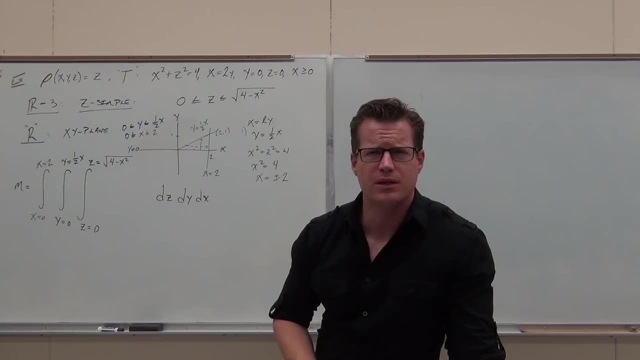 And it looks pretty good. to me. There's only one thing we're missing. What are we missing? Yeah, if we're going to find the mass, you've got to have a mass density function, which means here we're going to have what? 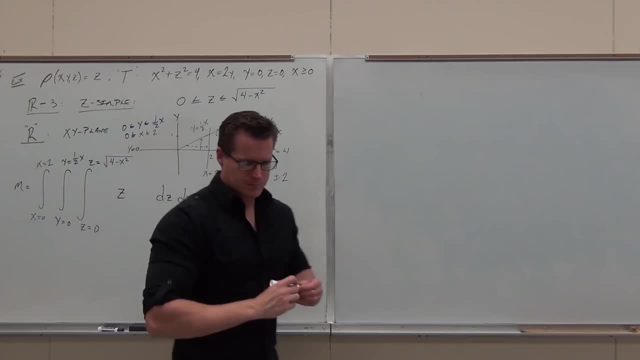 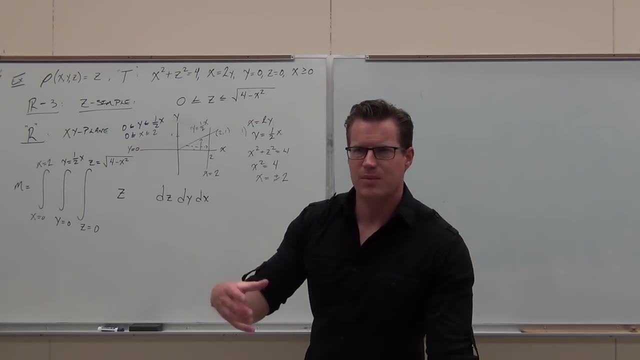 Zz. That's where I'm going to stop on this example. I want to see that you understand the setup. Do you understand the setup on the choice of z simple, where all of this junk comes from and how to get that triple integral? 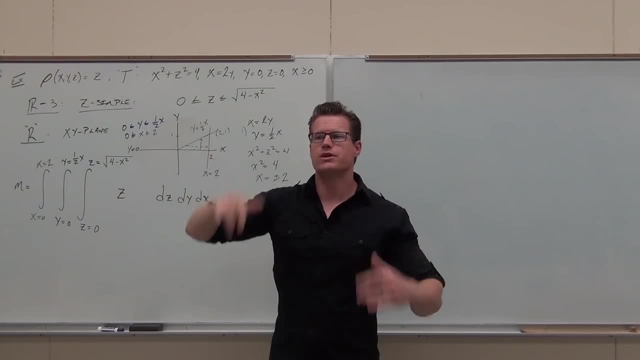 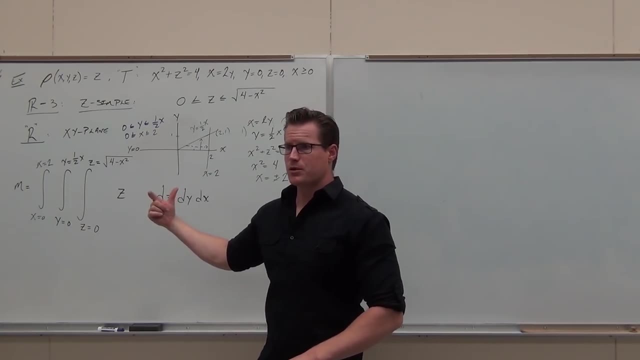 Show of hands. if you do, That's pretty much everybody. That's good. What would your next step be? Integrate. Integrate with respect to 1 half z squared. You plug in 4z, You get this squared. I'll show you that. 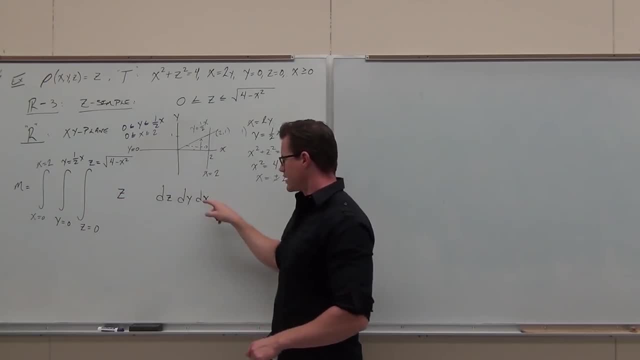 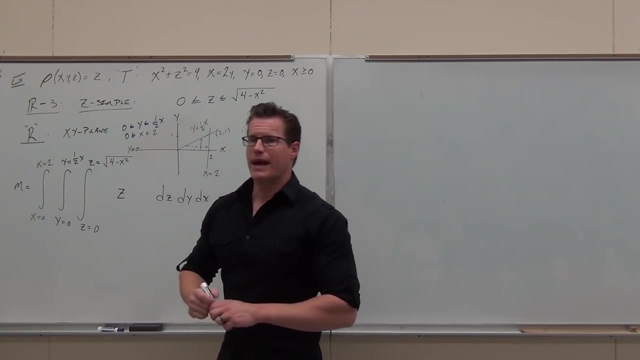 Then, with respect to y, plug in some stuff. Then with respect to x, plug in some stuff And you find the mass of that region. That's OK, That's an option. It's not a bad option. Your answer here is 1.. 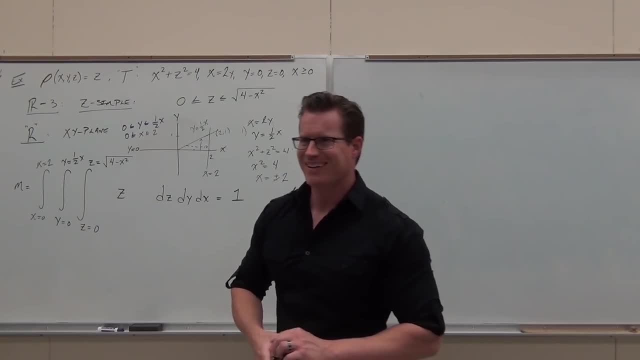 That's how fast I want you to do it. No, That's just the answer. Just look at it: 1. 1 and done. No. Now there is another choice here. I said x simple is not a great one because x simple. 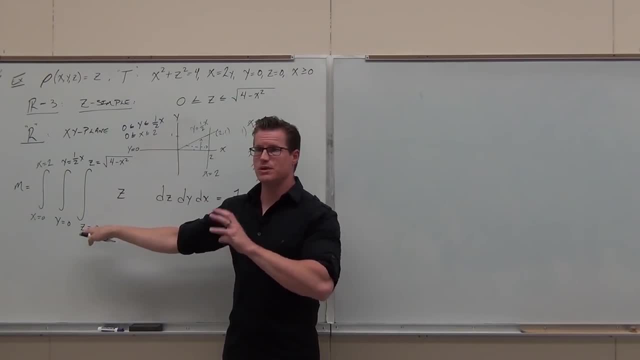 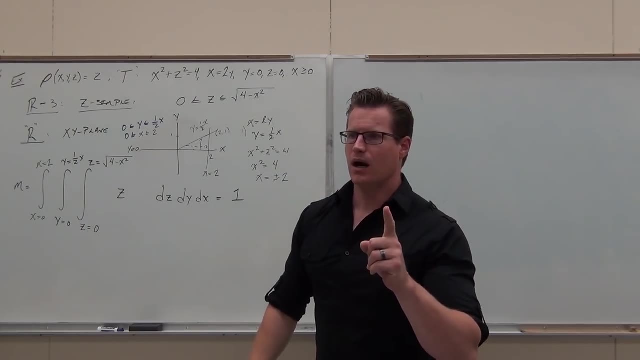 you'd be between two functions. I always love being between 0 and a function. If I had that choice, I'm going to make that choice every single time. But I want you to see y simple for one very simple reason: When we set up the integral, something special has to happen with it. 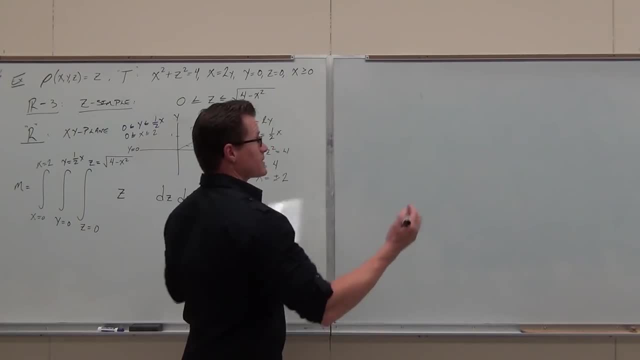 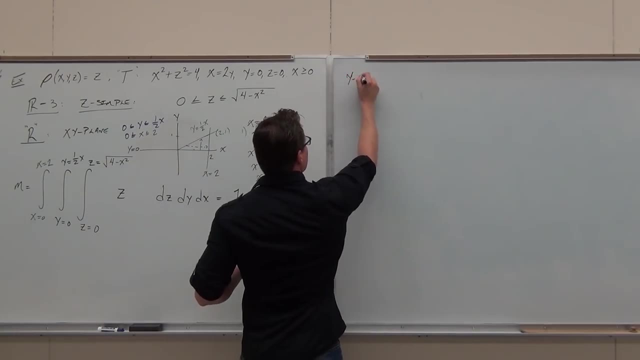 So I want to show that to you. So let's say that you get to your test. You don't see z simple, even though it's kind of a nice setup. You see y simple. Let's try that. So instead of r3 z simple, we're going to do r3 y simple. 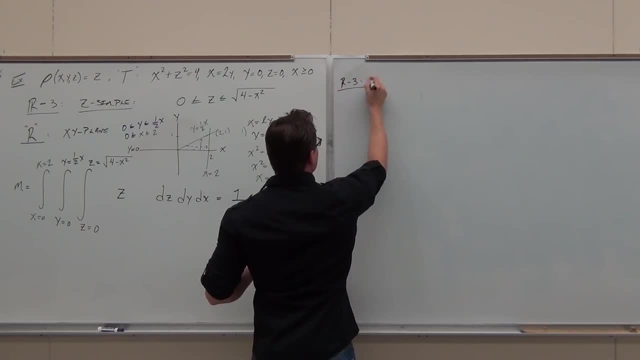 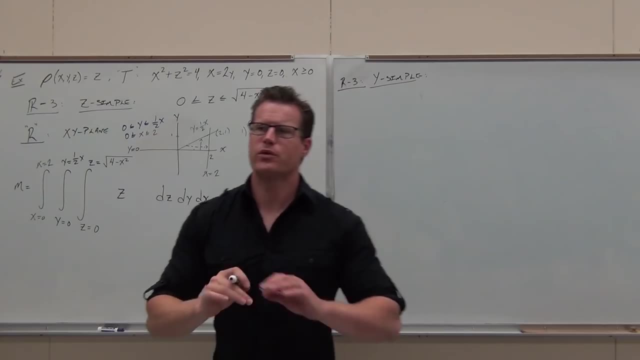 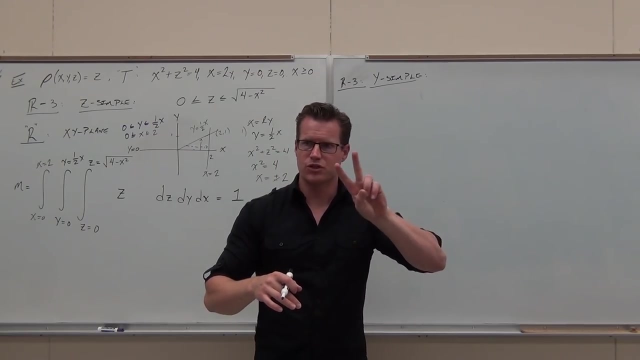 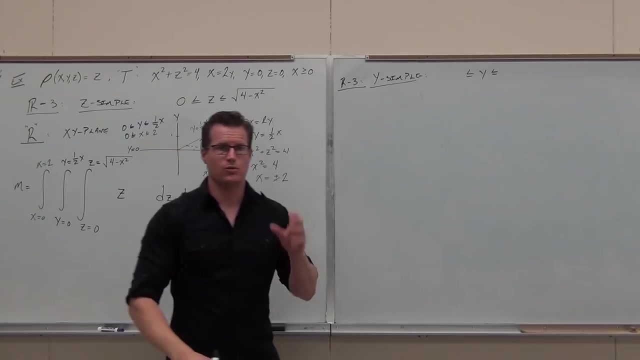 If we do y simple, that means we're going through a 3-D region, That's what we call r3 simple 3-D region. along the y-axis We have to intersect two functions where y equals something, So y is going to get matched between two functions. y equals. 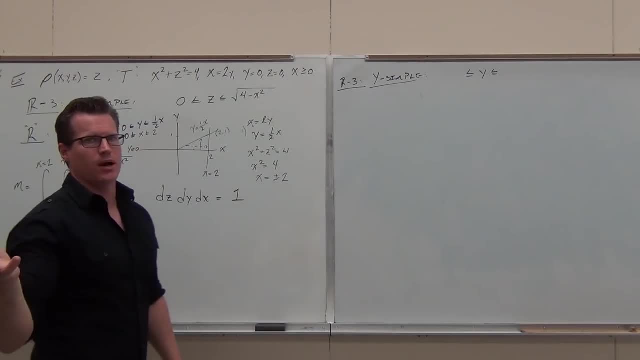 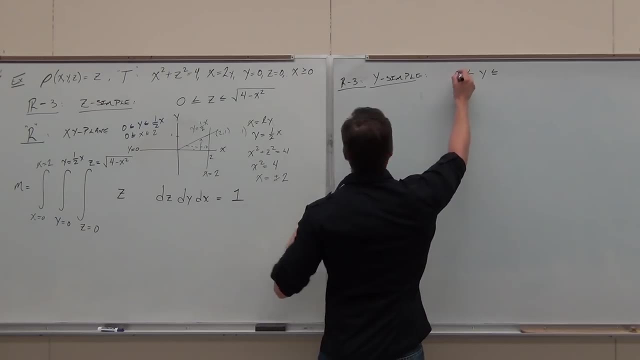 That's what we want out of this. One of them is really easy. Everybody right now what's one of the functions? y equals. That's why we picked that. That's why I'm not doing x simple. So I know y equals 0 gives me that bottom bound of 0.. 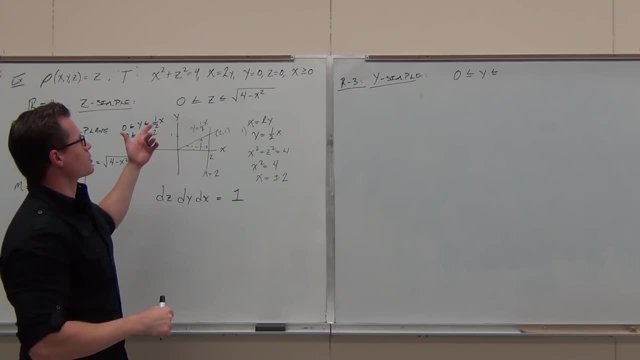 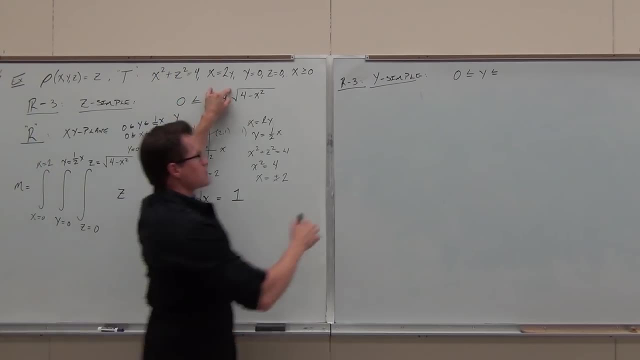 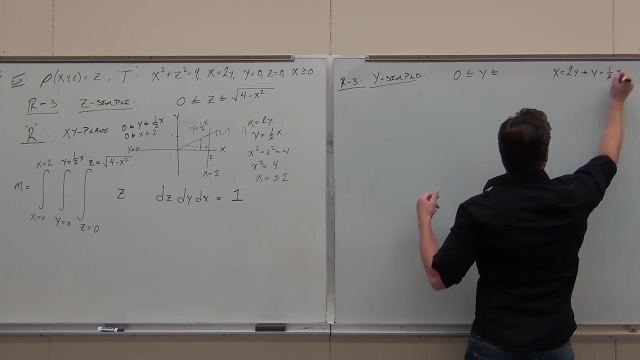 Pretty much, you can take that for granted most of the time. The other one, well, that's not a y, That's not a y That doesn't have a y in it, But that one does. So if I can solve this, then that gives me my other function, y. 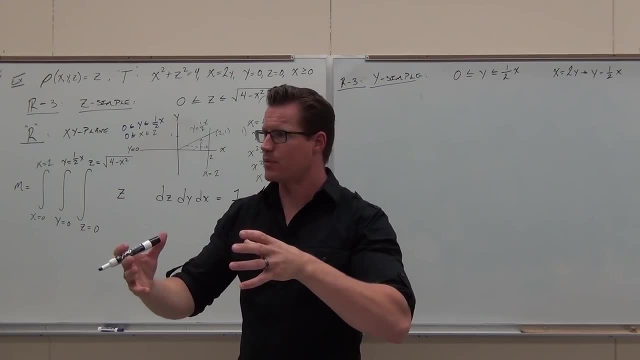 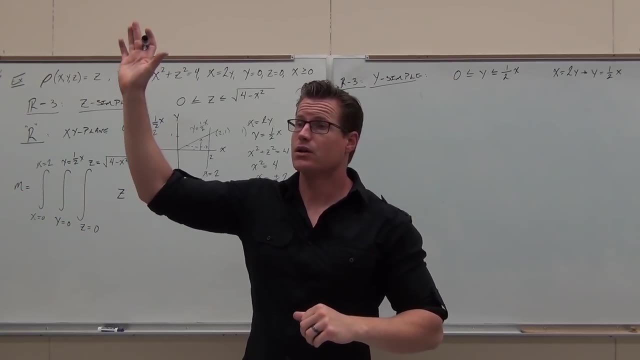 And I automatically have my inside integral set up. Instead of doing dz first, I'm going to do dy And I'm going to go from 0 to 1 half x. So if any of you feel okay with that one, Okay. so if we went y, simple on this. what's the region? 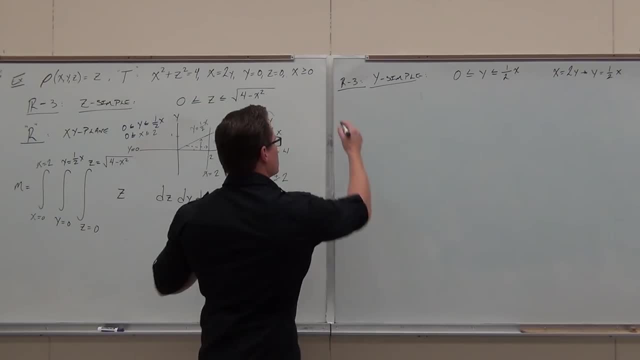 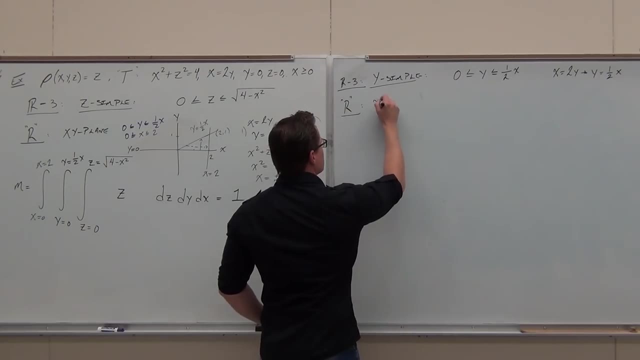 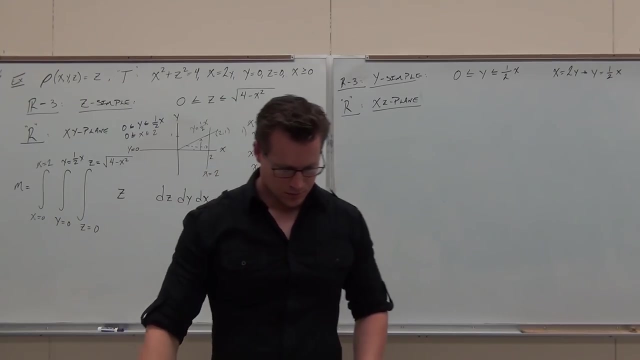 On what plane? Come on what plane? The xz plane. So for our r, we're going to have- yes, you're right- the xz plane. Every single time you have a double integral, you do what with the region? 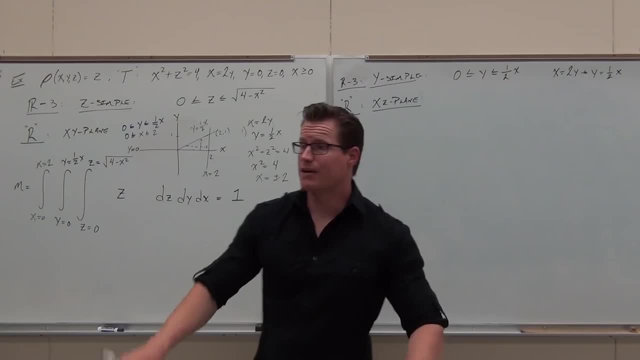 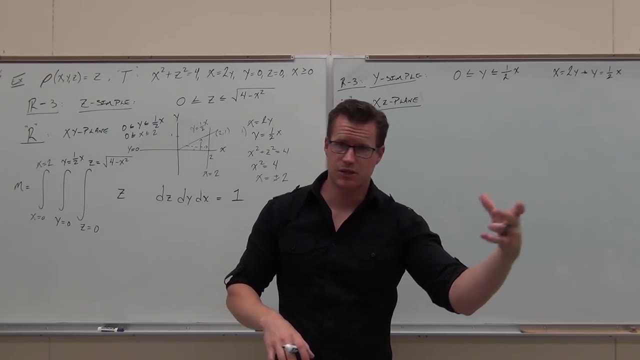 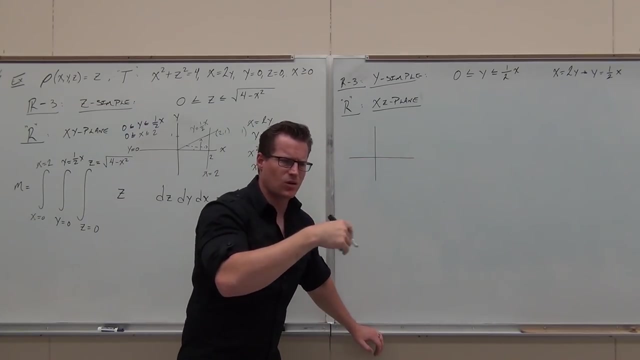 Graph. Let's draw that region, Let's do that. So everything that we have over here that involves whatever these two variables tell you, is going to be graphed on this plane right now, on the xz plane. Hey, what axes go where? 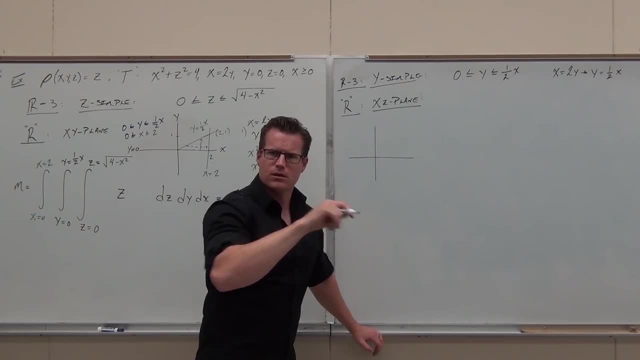 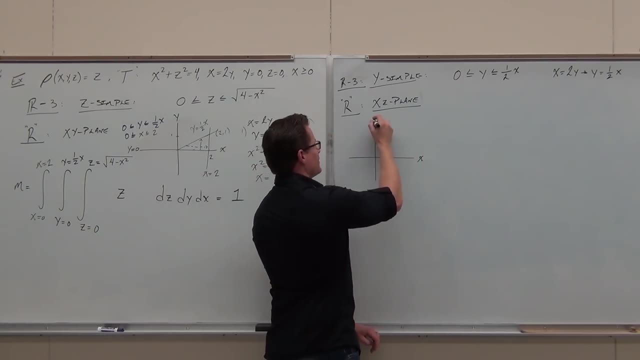 What's the horizontal one? What's the vertical one? The z one, Z is. Z is vertical. Sorry, You're forgiven, Don't let it happen again. Now let's see what's relevant. Is y equals 0 relevant. 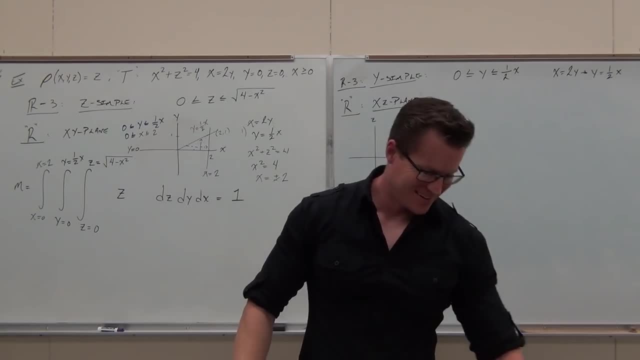 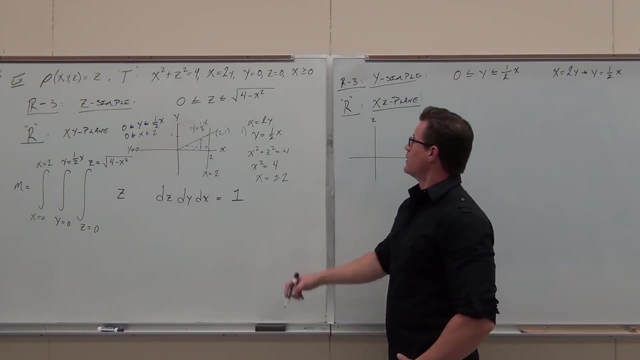 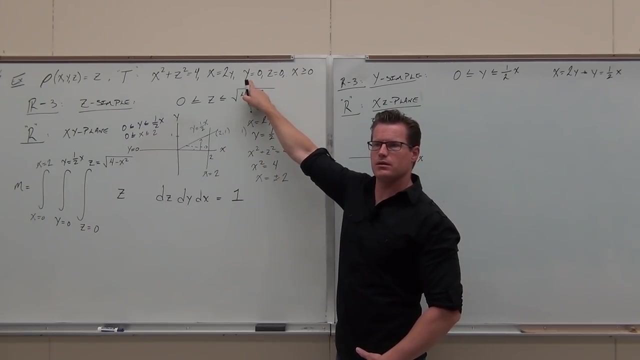 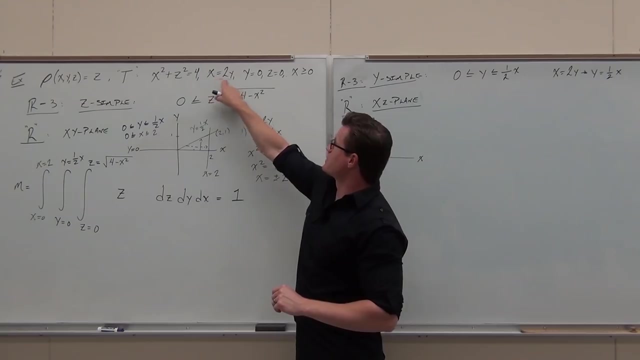 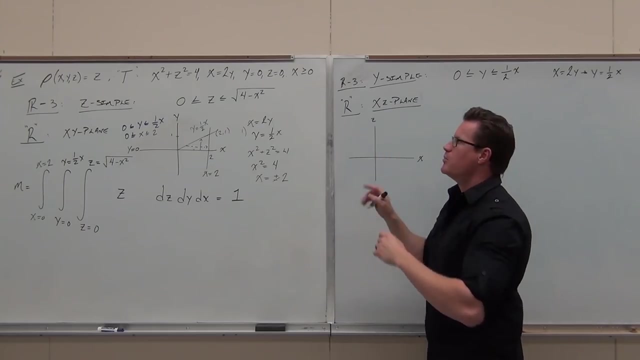 Yes, How is it relevant? It tells you you're on this plane. That's what y equals 0 said. Is x equals 2y relevant? Does it have one of these variables in it? Then it's relevant Everything. But here's the deal. 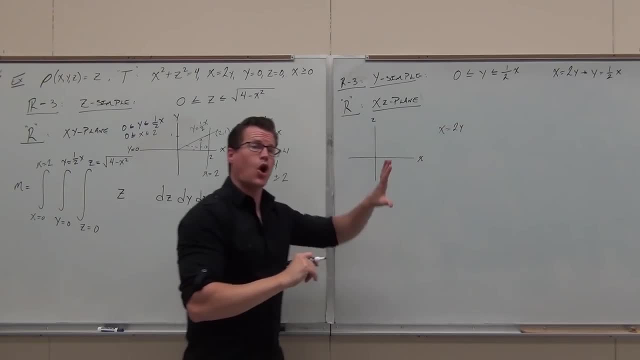 If x equals 2y and we're on the xz plane, it's very much like this, where z equals 0, we're on the xy plane. Now what is going to equal 0 out of that? We're on the xz plane. 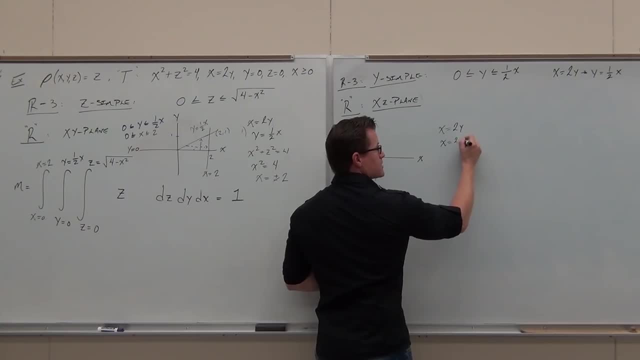 What's going to equal 0?? Well, we get x equals 2 times 0, because we are on the xz plane. Why is it going to equal 0?? We're on the xz plane. Why is it going to equal 0 on the xz plane? 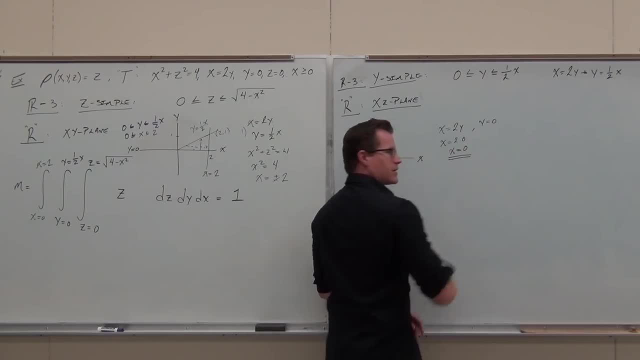 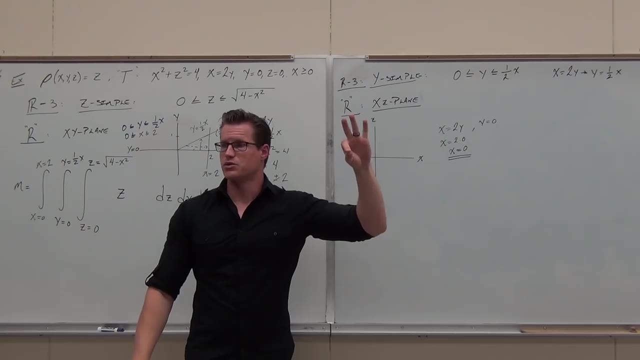 You're going to get x equals 0. This one thing right there is going to lead you to a better answer. If you have x equals 0, it's going to stop you from going all the way around a circle, which we can't do here. 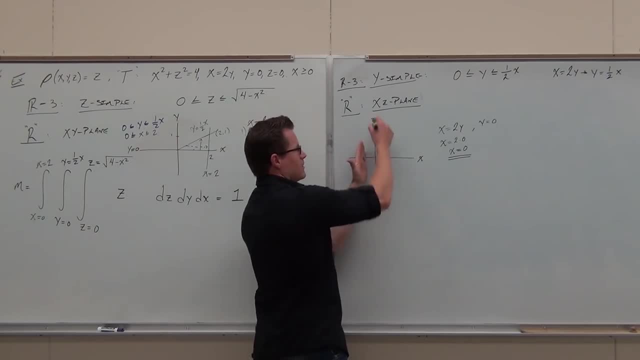 And you're going to see that in a minute. So x equals 0 says hey, we're stopping right here. This one would also do it. It says x has to be greater than or equal to 0.. Does that make sense? 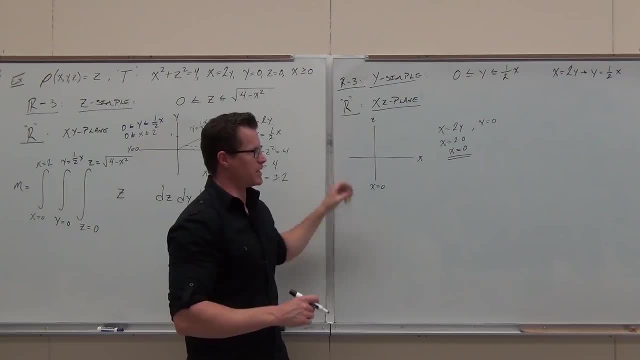 Most problems wouldn't give you that. I'm giving it to you so we don't have this other side to it. So that's one thing. We've got this on the plane. This one's also got to be there. What's z equals 0 going to tell you? 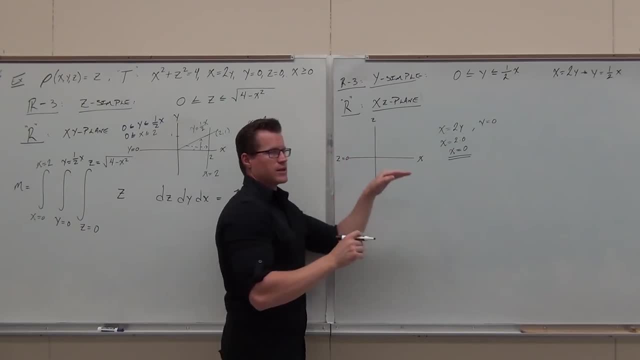 Yeah, it's going to tell you that we don't go any further than this. We're trying to find the region bound between here and here. Basically, that's in this first quadrant That one tells you. I'm not just over here either. 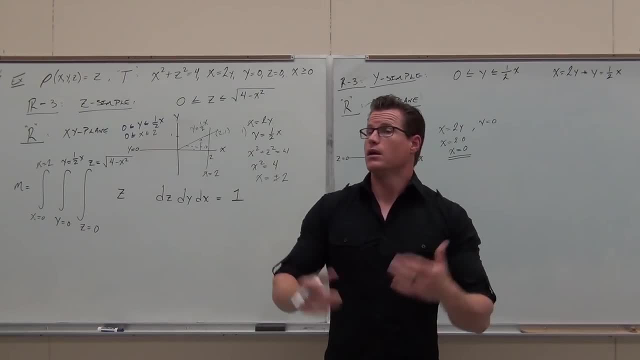 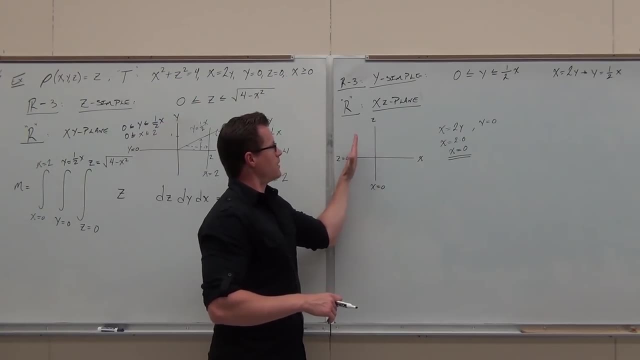 I'm only in the first quadrant And I don't know if you're okay with that one Now. we keep on going. That's also something, So we took care of this. That's saying we're positive of x equals 0.. 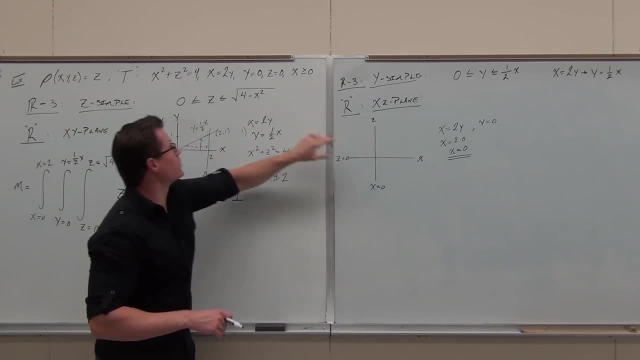 We have that That's giving us 4s on y. This says we're on the plane, This says hey, when y is 0, we have this: x equals 0. Kind of redundant here, but that makes it to the right-hand side. 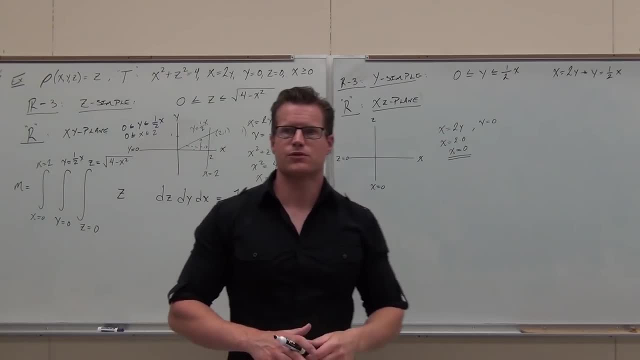 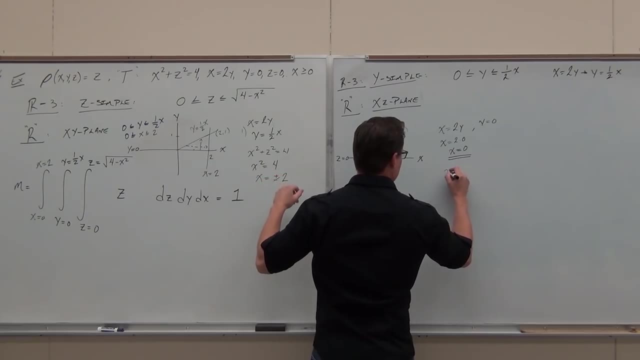 And then we have that guy. Can you graph: x squared plus z squared equals 4? Yeah or no? What's it? look like Circle, Since that's on this plane. that's a circle centered at the Radius of, For sure. 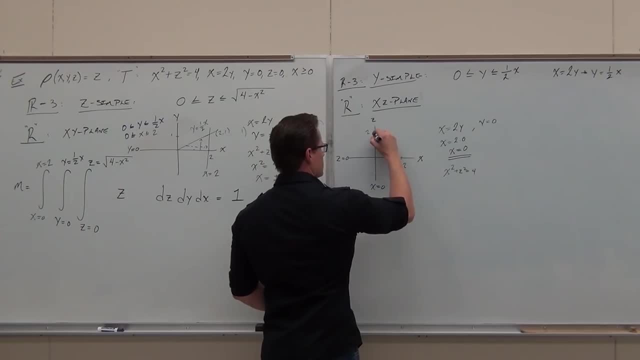 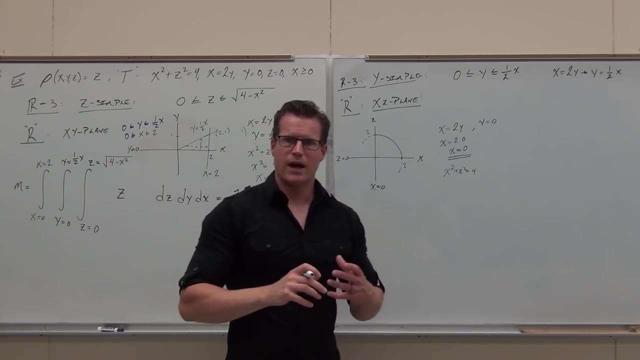 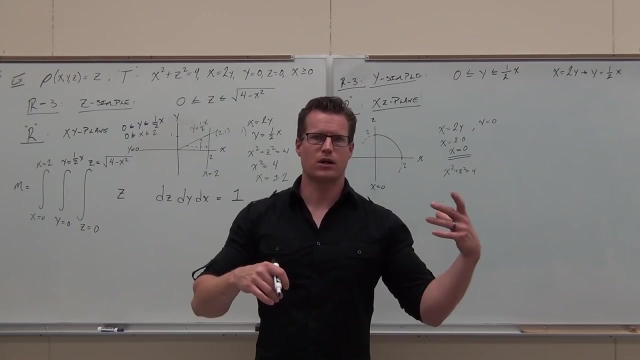 Radius of For sure. However, this is why it's important that you draw these freaking things. okay. If you just draw the circle and go from r equals 0 to r equals 2,, you're going to be absolutely fine. But if you go theta from 0 to 2 pi, you are not going to be fine. 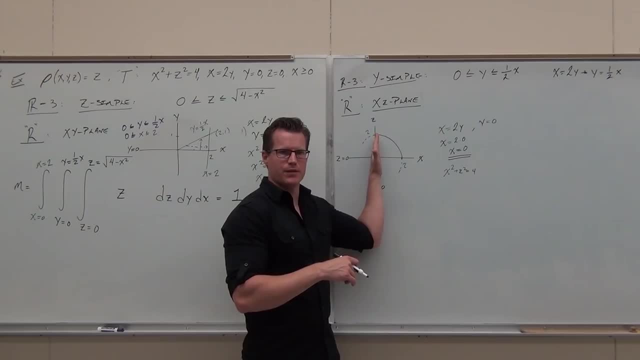 Do you see how this forces you to stop right there And you don't get to come back because x is greater than 0. This says the region that's bound by z equals 0 and x equals 0, and this circle is just this. 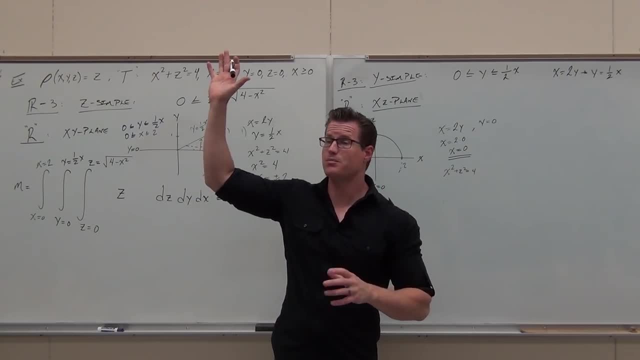 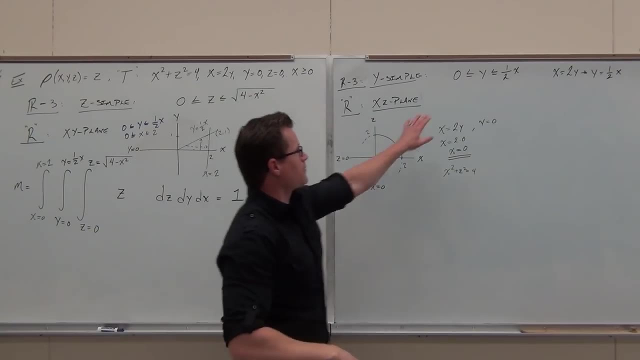 quarter of a circle. So it depends. if you understand that concept, That's a big deal. That's why we draw these things, That's why we graph them every single time. So let's see if we can do the setup. I know that I got the y. 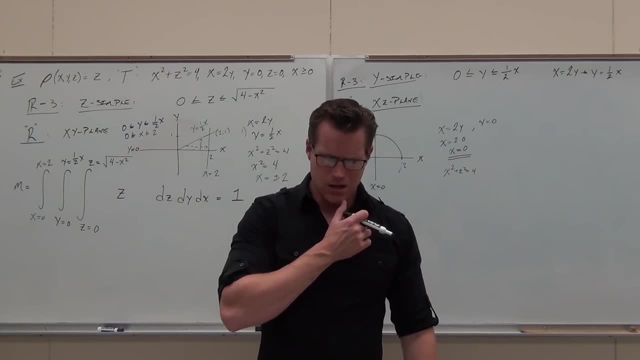 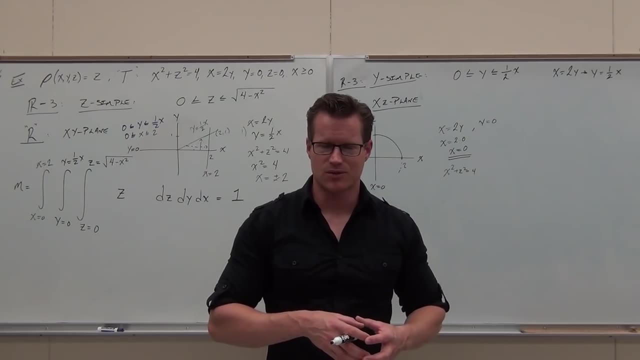 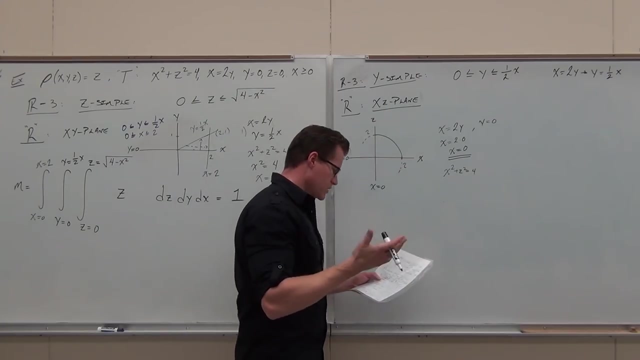 Wait a minute, What? I think I gave it away already. But what type of coordinates do we use for stuff that's like circles and stuff? Polar, Polar. Let's use some polar coordinates here. So if we got circular regions, why not switch this to polar? 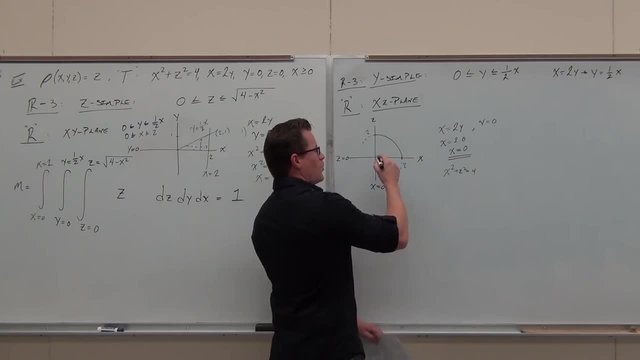 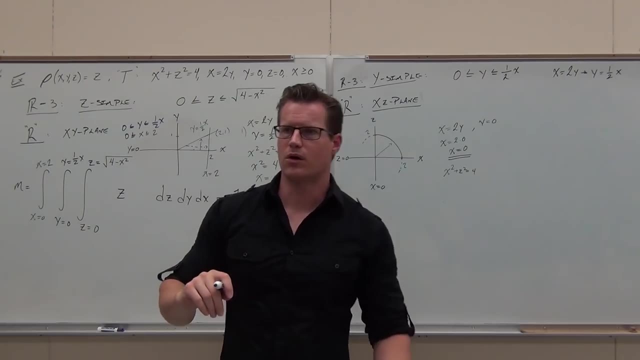 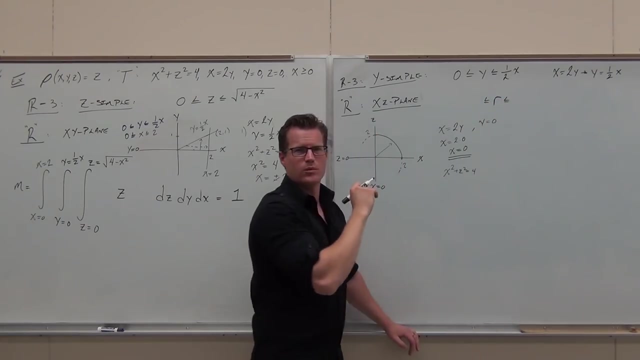 Well, if that's the case, then I want to be able to go from here through my region, from here to here. first, What always comes first, theta or r R R R, is going to be between what and what, please. 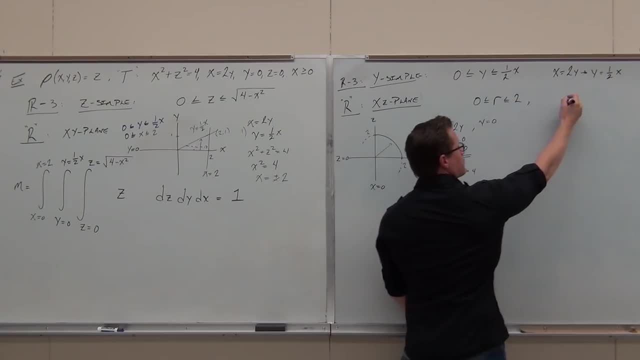 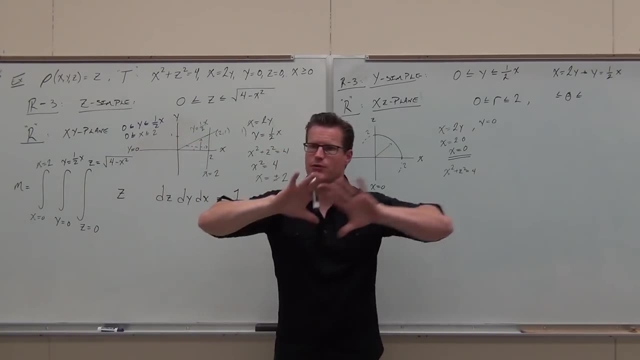 Z Z. After that we get theta Here again. why we draw the region, why we put everything up here on whatever coordinate plane we have, is so that you get this stuff correct. The setup is the most important point. Where does it start? 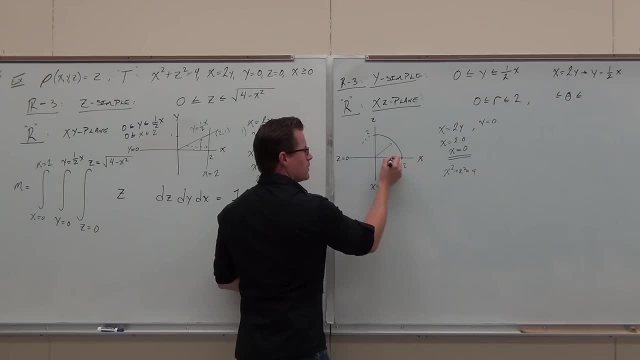 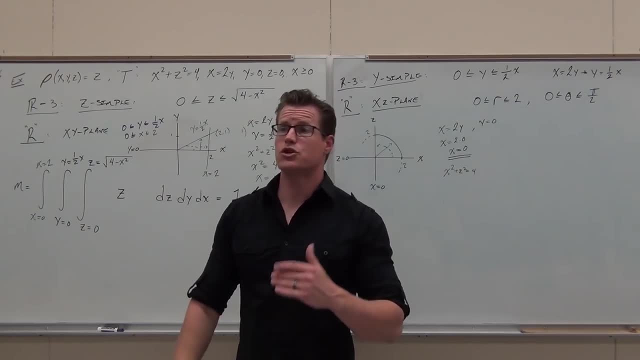 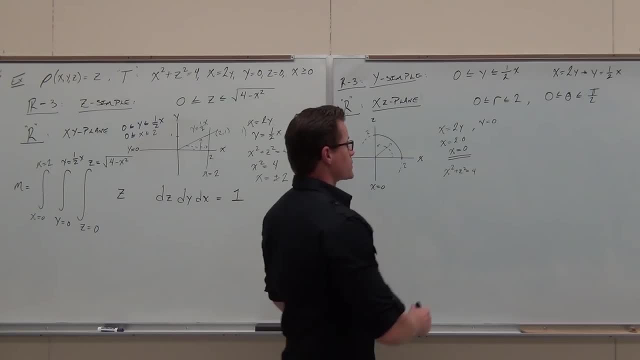 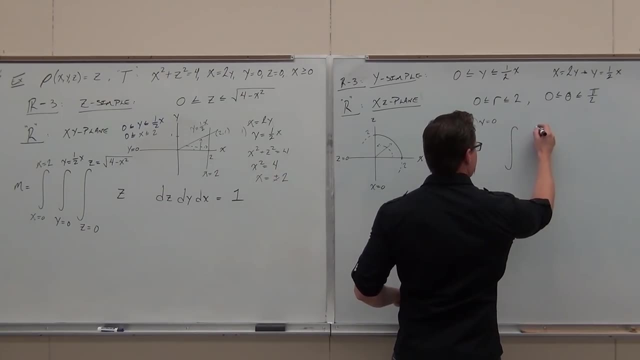 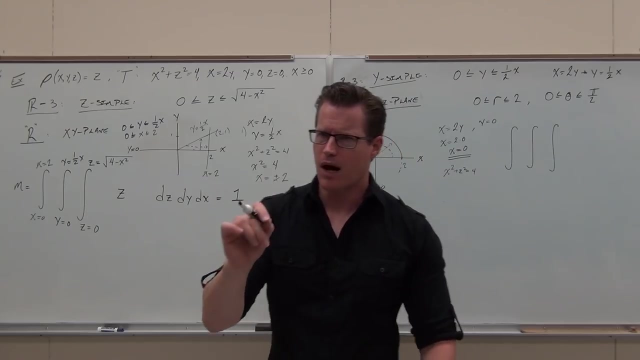 Are you with me? Okay, let's do the setup, then Triple integrals. now for this, We're going to go. well, what are we doing first? Are we doing dy, dx or dz Y? So you need a dy. 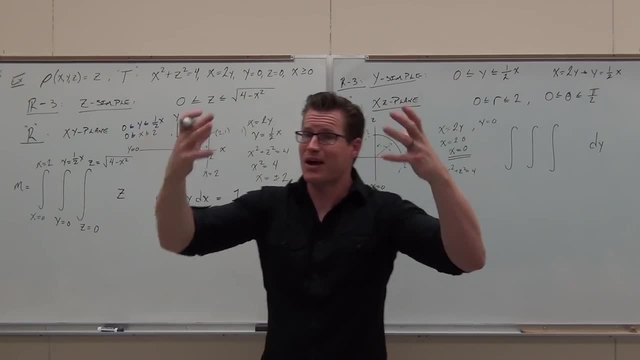 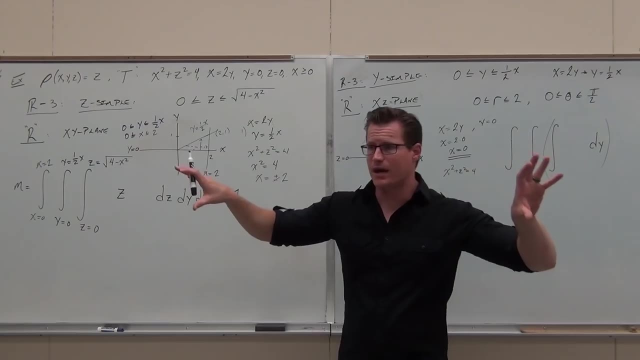 After that, well, that's just the R3, simple. After that we just have a double integral. So, this guy, you can put that in parenthesis and deal with the double integral basically independent from that. All it did was give you a region. 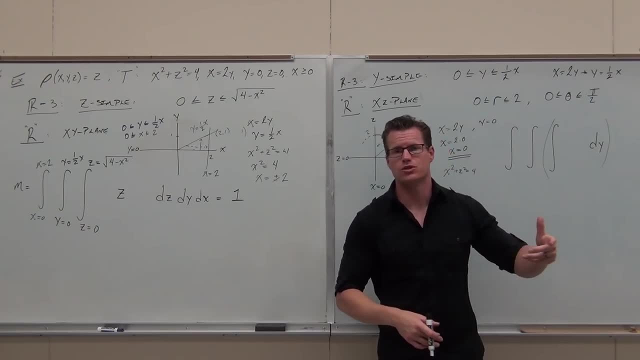 All we're doing is defining that region in terms of polar, because we had a circle. So, instead of having the dx, dz, what has to go over here for polar regions? everybody, What has to go over here? Rd, Rd. 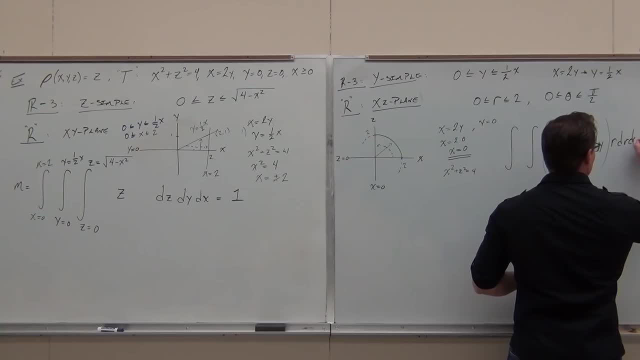 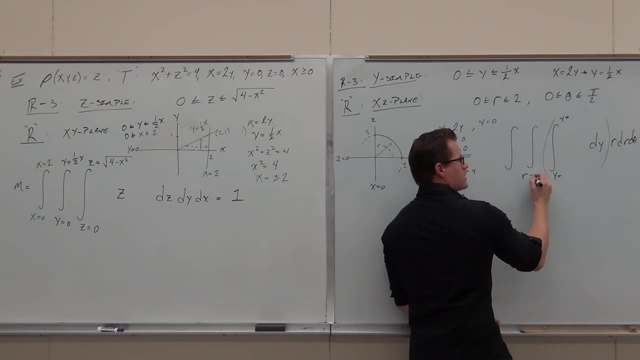 Beautiful Rd, Rd, theta. Okay. So I know that I want y equals here, y equals here. I want r equals here, r equals here. I want theta equals here and theta equals here, because we always match up our integrals from the inside. 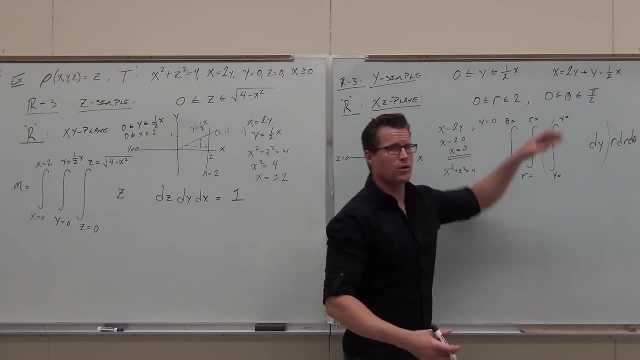 out with our variables, This one. if you've done the inequalities, you should be able to set it up. I want to see a proper setup. Go for it. I'm not going to give you long. We're all about setup. 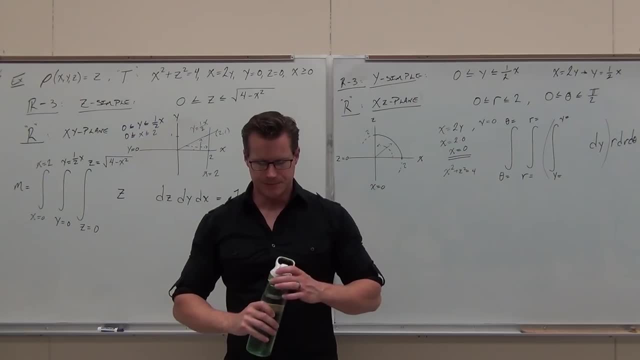 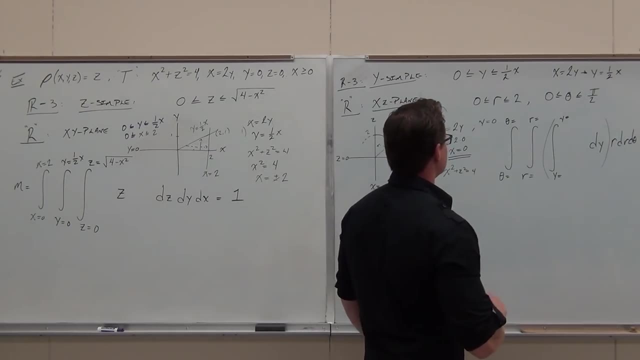 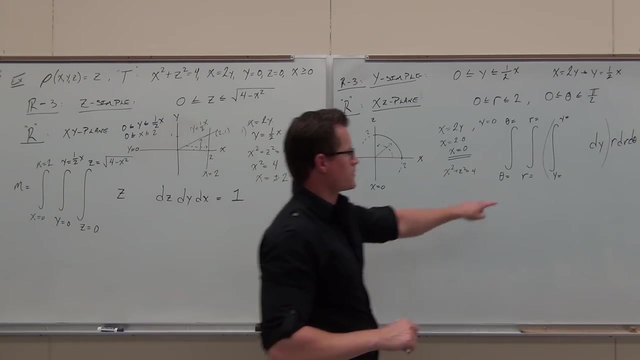 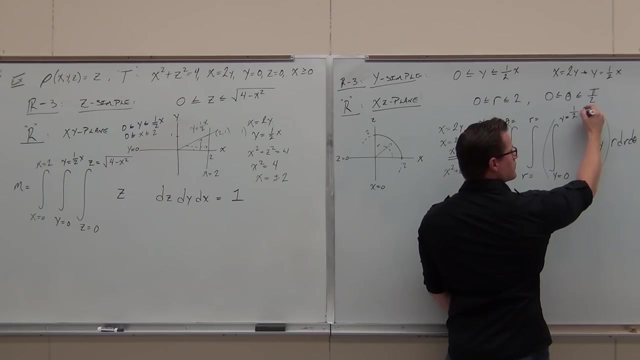 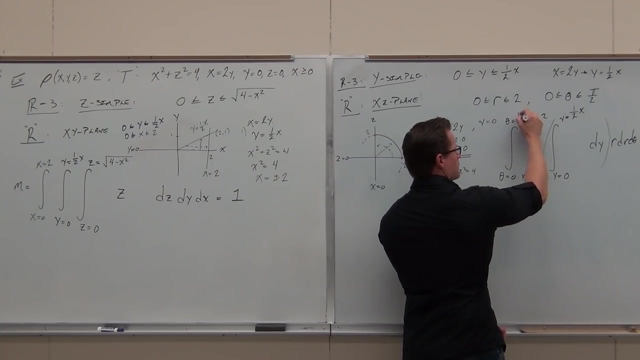 What goes here, please, Zero Zero. What goes here One-half? What goes here, please, Zero Zero. What goes here? Zero too, Here Zero. And That's the proper setup. we're missing one thing. 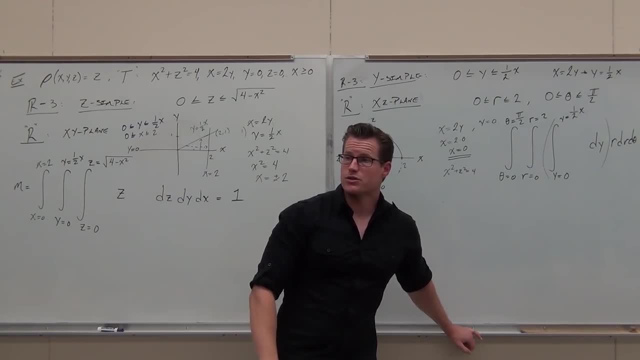 What's the one thing, Whatever the mass density function is. So in our case we had z. It's still the same z Man. that's it. That's the whole setup. I want to know if it makes sense. 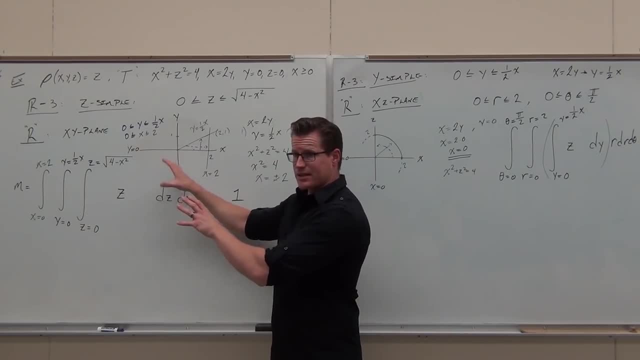 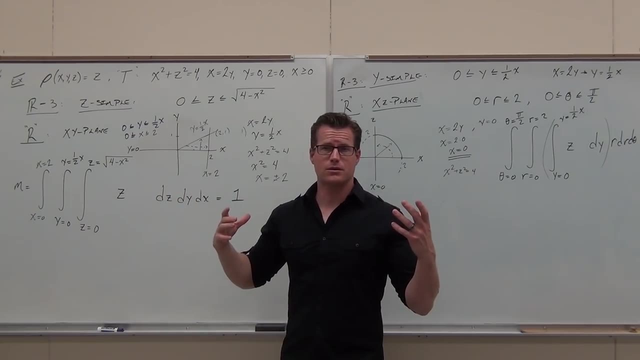 If you can see this as being a correct setup and this as being a correct setup, I'm a happy guy. Can you see them both as correct, As correct setups? Are they going to give me the same answer? Yes, They have to. 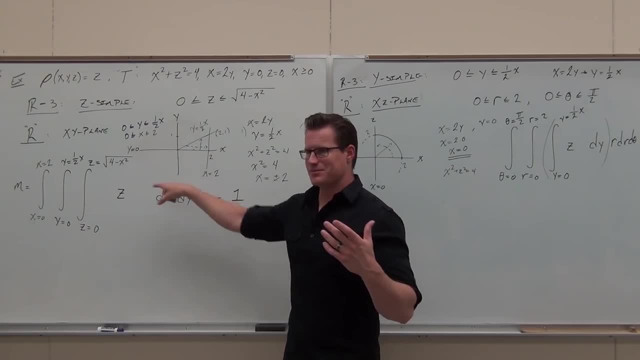 says they have to. I'm going to prove that to you. Well, you can take my word that that's one, But I'll show you over here. for one reason: Yes, Do we need to switch the y equal to one-half x in the term? 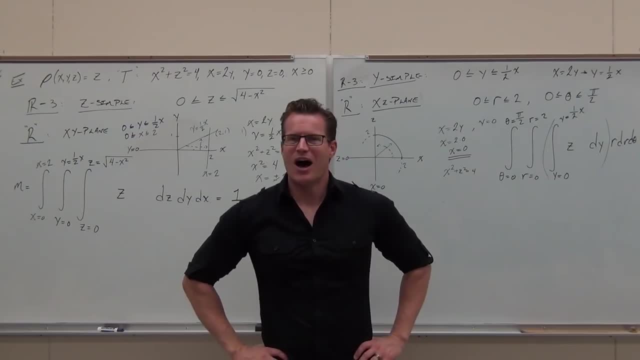 It's going to get to that. I promise I'm going to you like right now, But thanks for asking. I mean that's a great question, That's a perfect segue. Do you have to switch this stuff around, Listen? 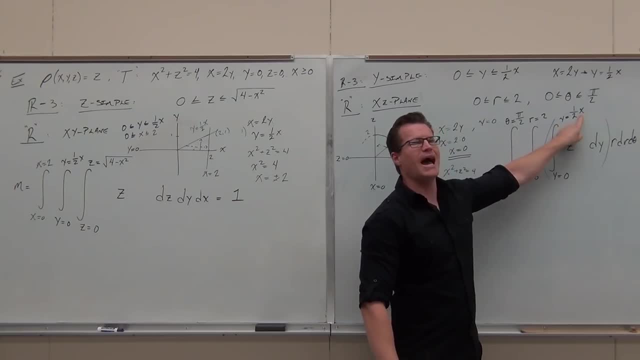 Listen carefully. This you will ultimately have to. You have to switch Why There are no x's Right? You're going to have to switch that to r's theta's. Hey, what is x? X is r. You can switch it right now. 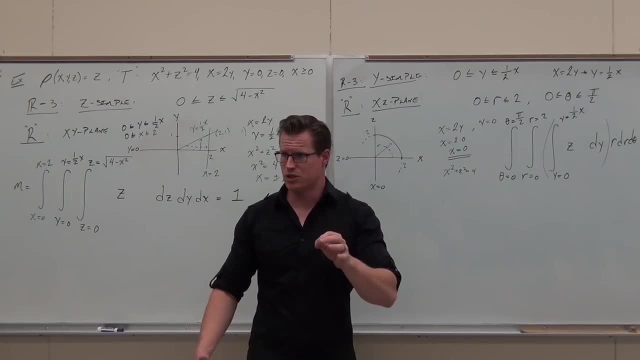 Could you have to switch it right now? No, you don't. You can switch it later, but you will be switching it. Some books make you switch it right now. Some books make you wait until later. It depends on the textbook. 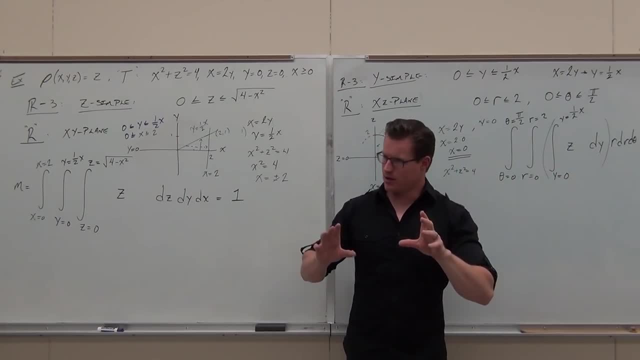 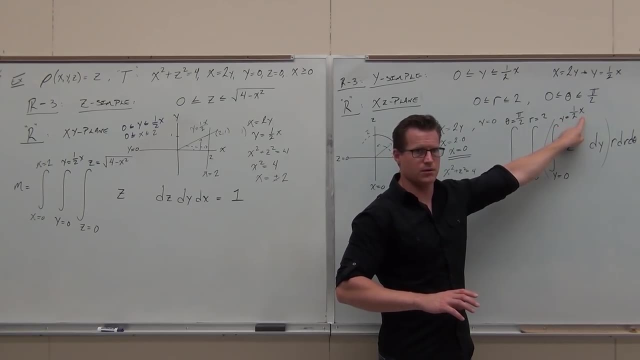 You can do either way. for me I don't care, But understand the concept. That's a big deal The way I've showed you. you should be switching that right now To r cosine theta. Does that make sense? 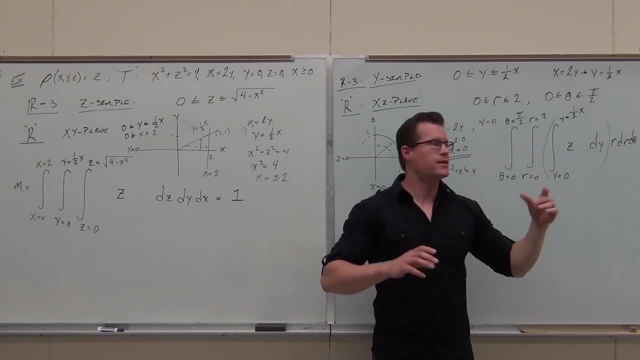 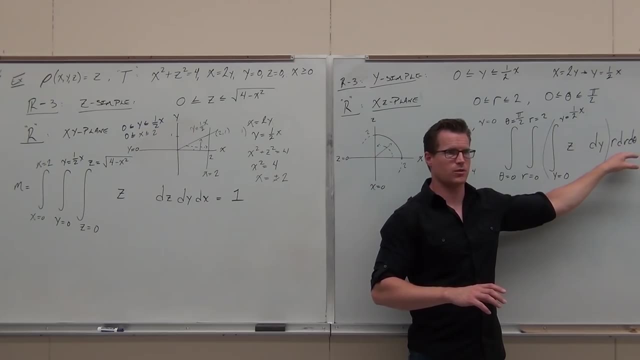 You should be doing that Because when you plug it in you're going to have r cosine theta. This variable has to match this. The remaining variables have to match these things. That's got to be there. Are you guys clear on what I'm talking about? 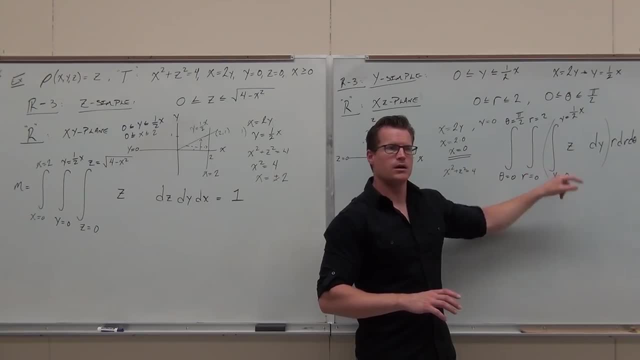 Now this one, Listen, This one. Sometimes you can get away with changing that now, and sometimes you can't. My encouragement to you is: integrate this first and then switch it. Okay, And then switch it when you have to. 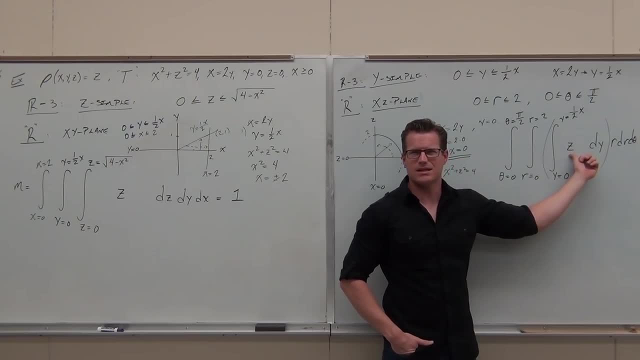 And the reason why I would say that is because if that had any y's in it at all, at least it probably won't. but if it did and you switched it right now, you wouldn't be able to integrate with respect to y. 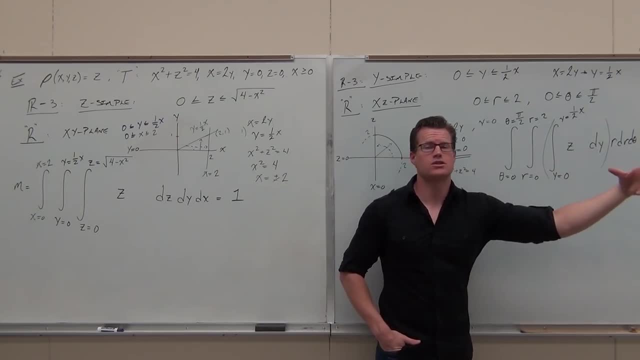 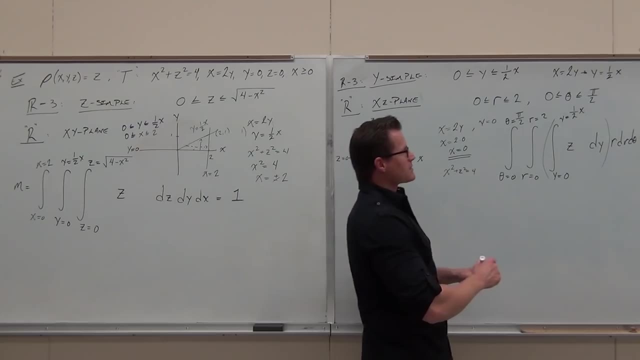 Does that make sense? So integrate this first and then change this stuff around. Does that make sense? So I'm going to start switching things so that you brought up a real quick point. So let's change this, You go well, x, no, no, I don't want the x. 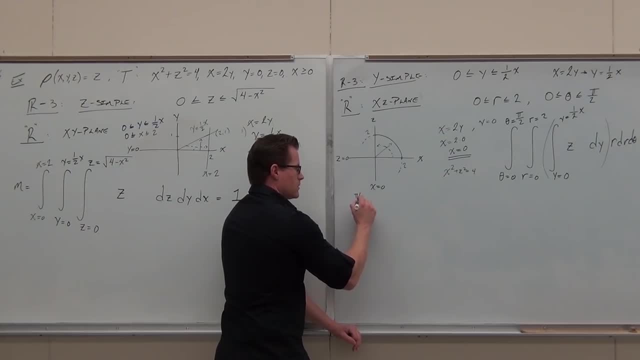 I want to make this 0 to pi over 2.. I want to make this 0 to pi over 2.. I want to make this 0 to pi over 2.. I want to make this 0 to 2.. I want to make this 0 to 1 half r cosine theta, because x is. 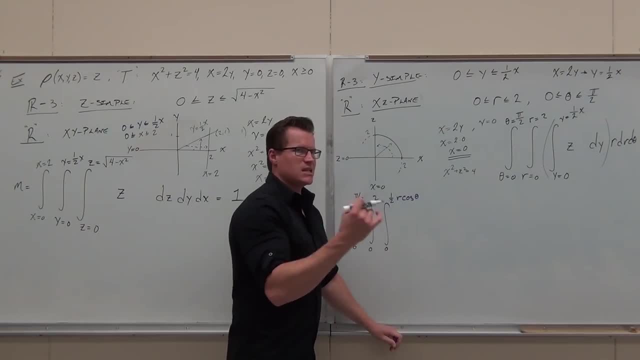 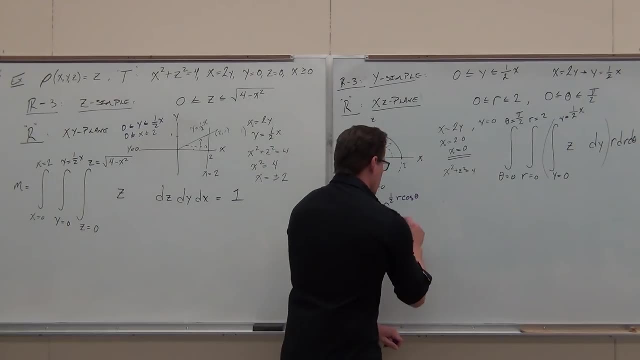 on the horizontal, and that's r cosine theta. for us, Z would be r sine theta. Is that clear? Not y Z? Then I have z dy. I'm going to do that one first, and then I'm going to have an r cosine theta. 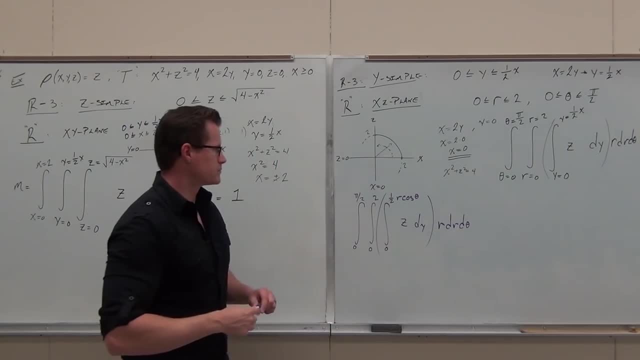 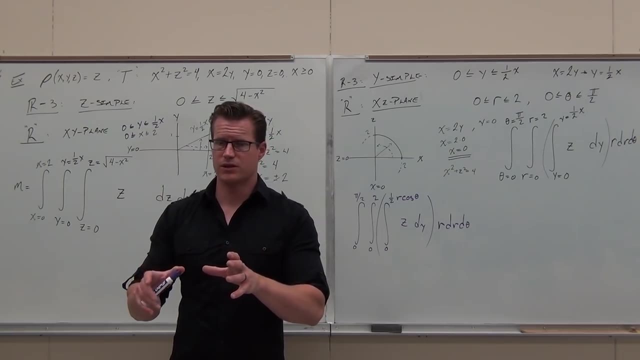 Z is going to be r d r d theta. Truly, do you understand the concept of what we just did, yes or no? Okay, So I'm going to go through it pretty fast. Hold on to your hats here We're going to integrate this thing. 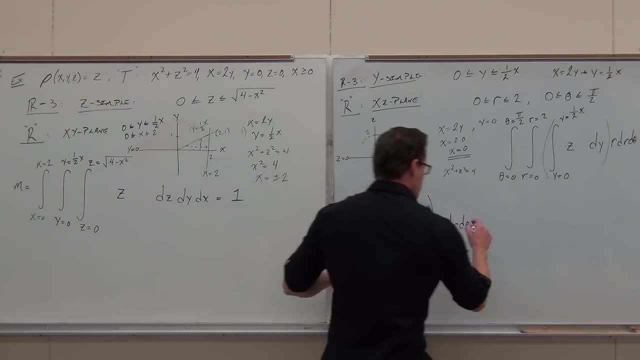 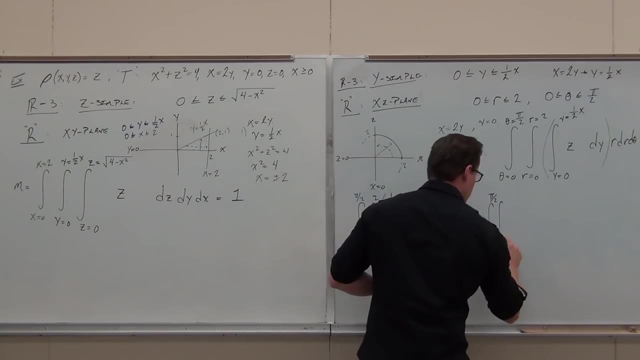 I want to show you some things that you should be doing and not doing. okay, So, first thing, 0 to pi over 2.. No problem, We're just going to rewrite these, this double integral out here, Integrate it straight to y. 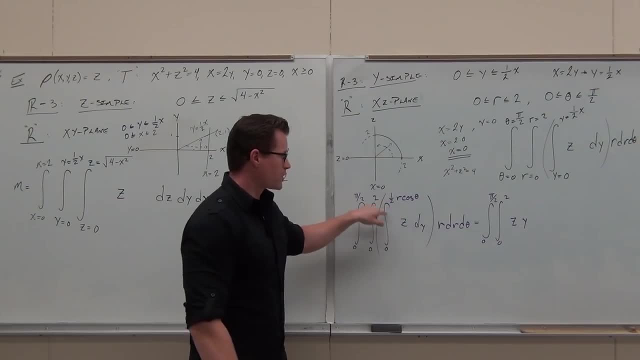 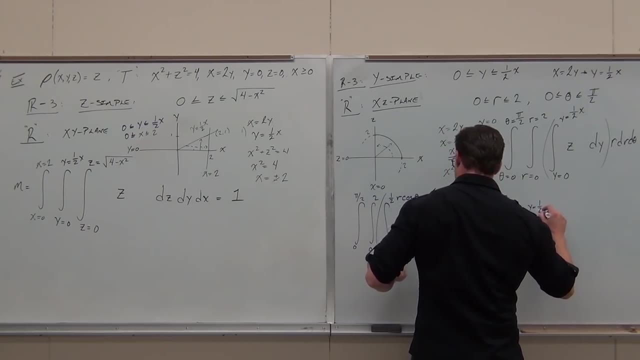 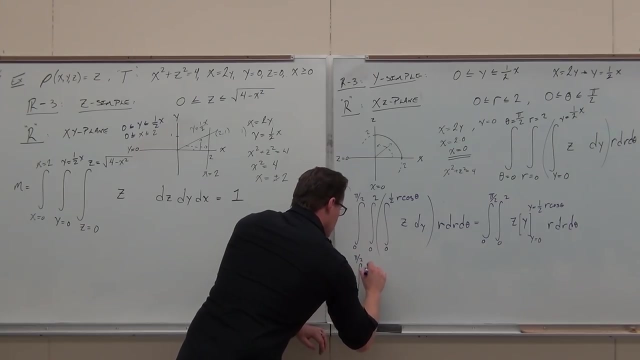 We get zy, And that's d r d theta. We also are going from y equals 0 to 1 half r cosine theta And then after that we're going to have an r dr d theta. Now we're going to plug that in. 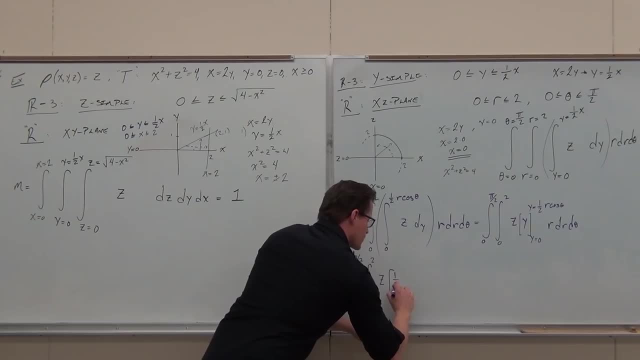 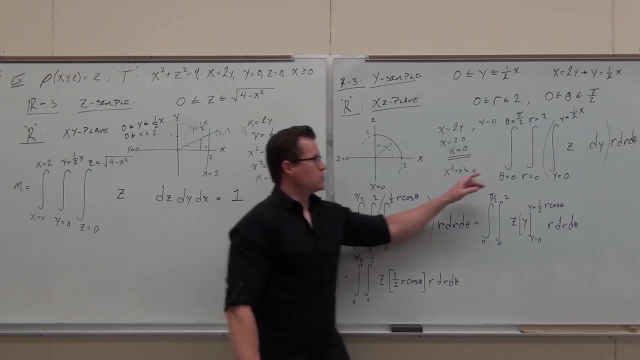 y equals. this minus y equals, that gives us just 1 half r cosine theta, r dr d theta. This is the point I'm going to make right now, though, Where you do have to match these up to your next variables, and that's exactly what we did here. 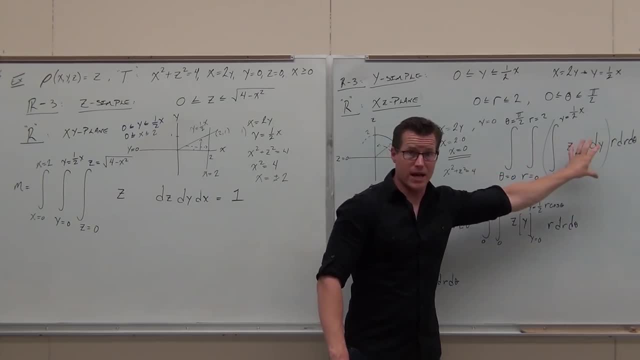 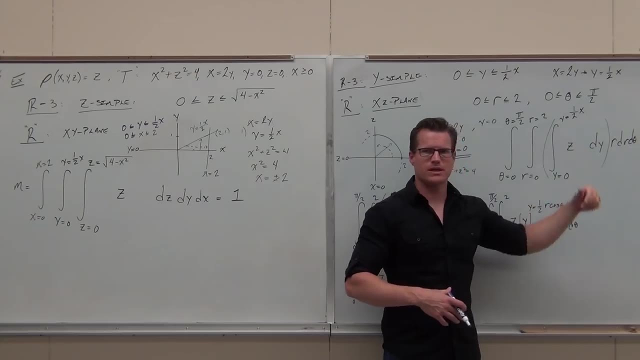 this z doesn't necessarily have to right away, Right away, In fact, I would encourage you not to, Just in case you have that variable, Just in case you have to integrate with respect to that z. Does that make sense to you? 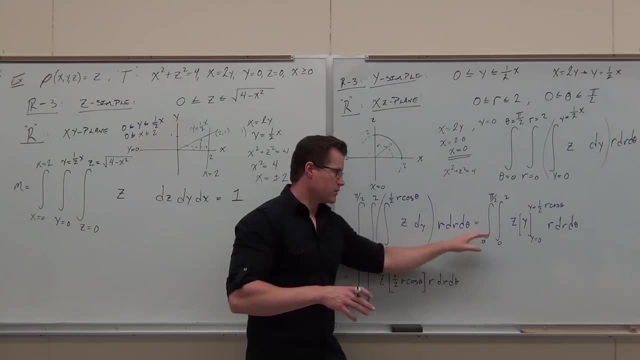 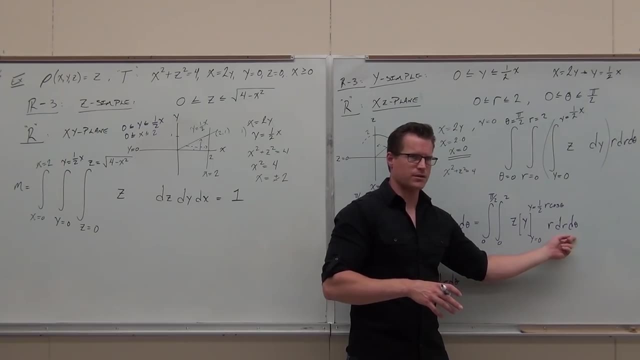 Just hold on to it. But then later on, when you get down to it, your evaluation, you get down to it and you go: wait a minute, wait a minute. All the rest of my junk has r's and thetas. 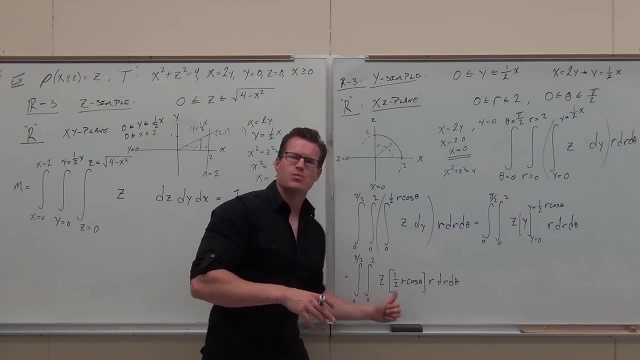 All the rest of the stuff has r's and thetas. This z is a problem. That's where you must change it. You must change it at that point. You can't go any further than right here before changing all your variables into the rest of these things- r's and thetas. 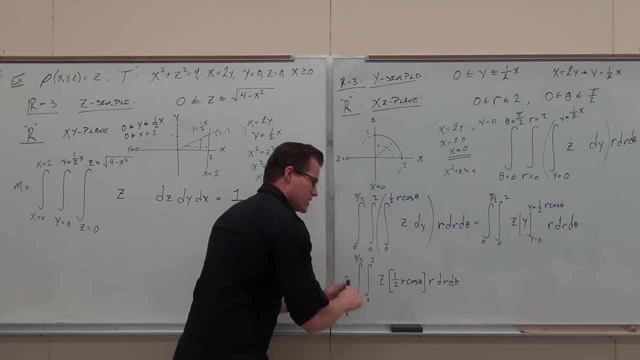 Does that make sense? So now we're going to go. well, how much is z? Z took the place of the y-axis. That's why we always write these in the same orientation: X and y, or x and z, or y and z. 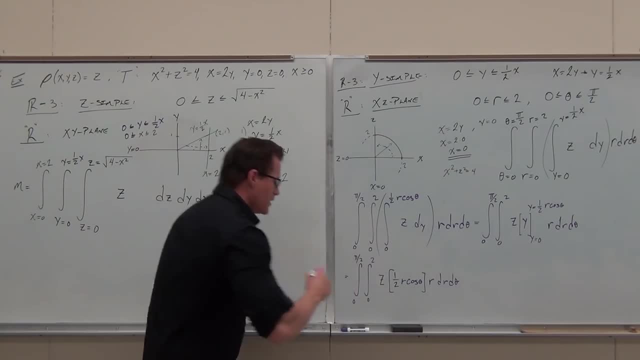 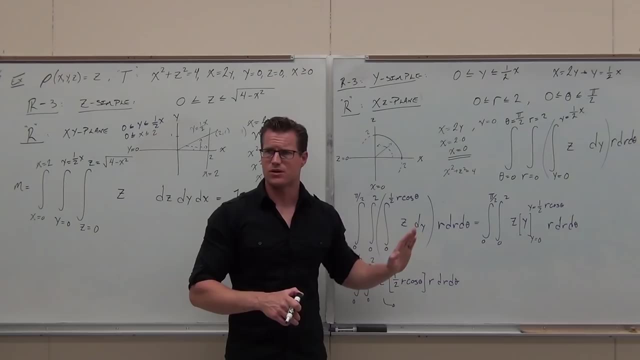 So we get the same relationships over and over again. This z now is going to be. well, can you figure it out? If x is r cosine, theta for horizontal y is r sine theta. Wait a minute. r sine theta is y. 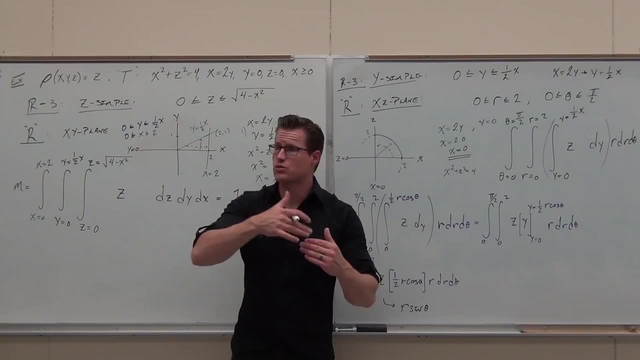 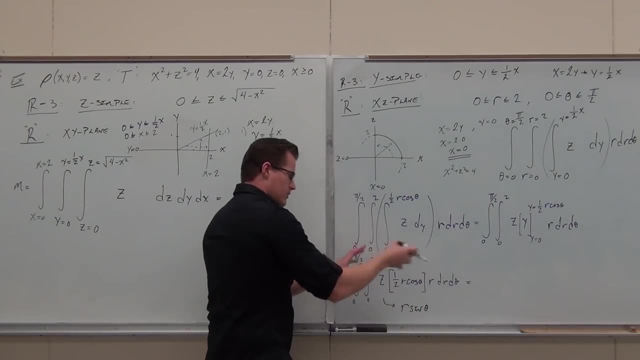 That's y, That's y. Well, it is. if we're on the xy plane, We're not. We're on the xz plane. That's why we get r sine theta out of that. So when we make that little transition, 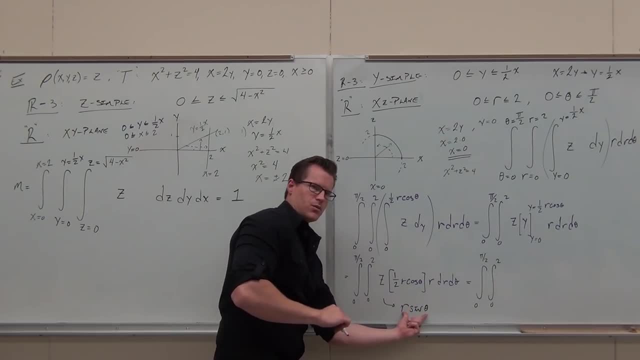 that z becomes this thing. I'm going to do all this at once. We get a one-half. We're going to have an r, an r and an r, That's r to the third power. We're also going to have a sine theta. 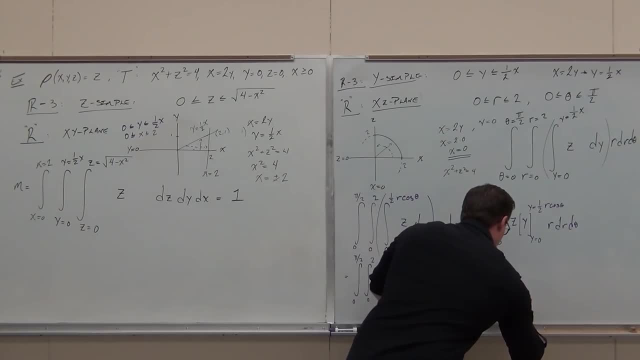 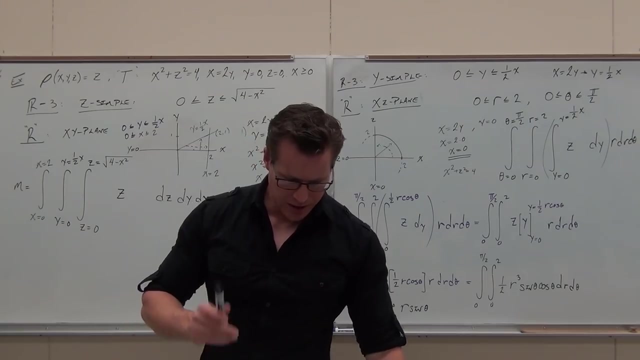 and a cosine theta. So we're going to get this one-half r cubed sine theta, cosine theta. Well, we took care of the r, so it's just dr d theta. I really, really, really want to make sure that makes sense to you. 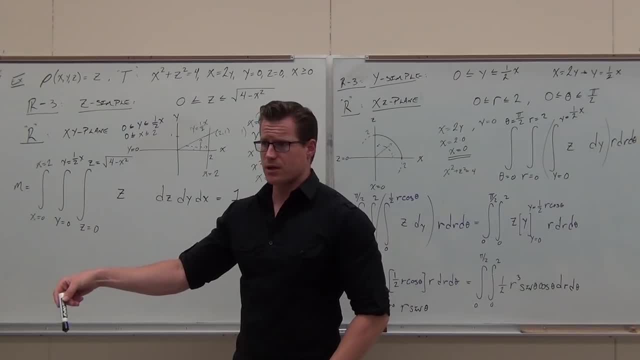 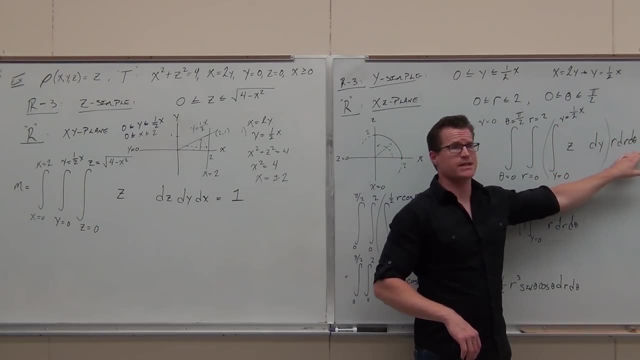 That's a big deal Where you change things and where you don't change things. in my opinion, In other books you can do it different. Me personally, I always make sure these variables match up to these variables. That is a big deal. 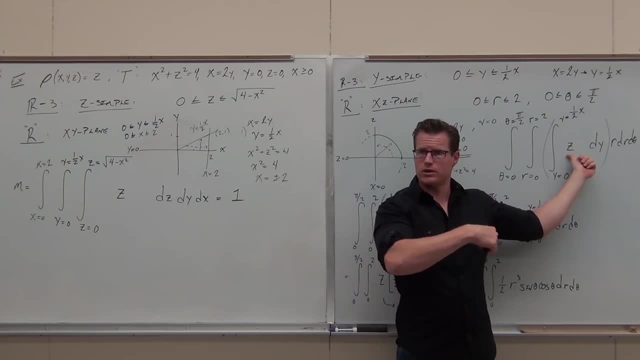 I don't change this right away. You could. In this example you could, because this is not a y. So if you really know what you're doing, like I'm going to change it now. fine, as long as this function does not have to do with that variable. 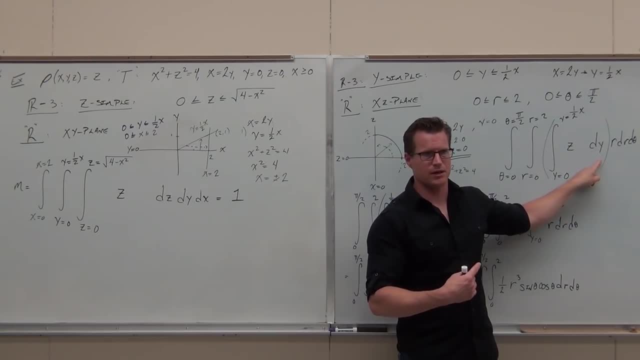 right there. Is that clear for you? That's a huge deal. I cannot stress that enough. Me personally, I wait, I wait and then I change it when I have to, When I'm done integrating all the certain variables I have. 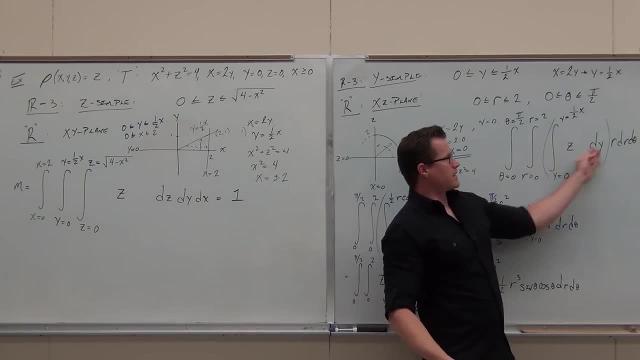 then I change it. You can say that here: Well, that's a z, There ain't no z's. Okay, Then you're able to change it. But if you have a y and there's some y's, you can't change it there. 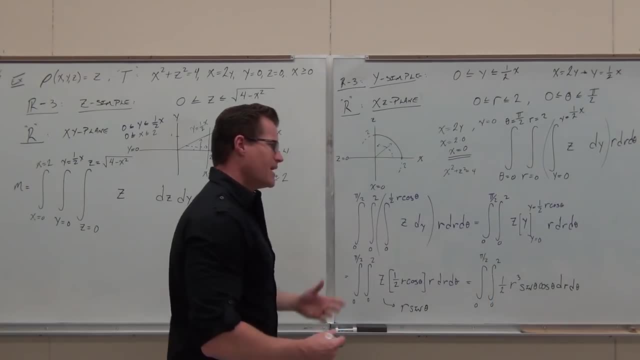 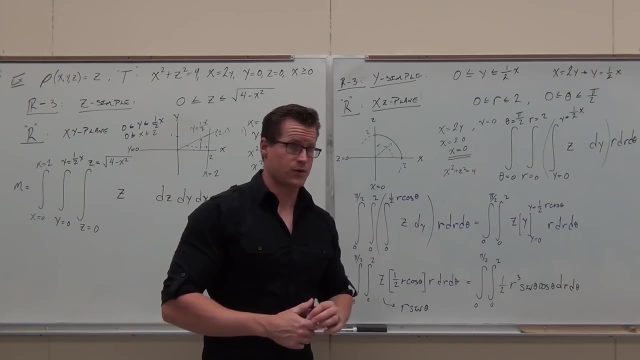 You've got to integrate first. Now, after this one, what would we do here? Integrate with respect to what r r first. Okay, So I'm going to have, I'm going to go right down here to get our r1.. 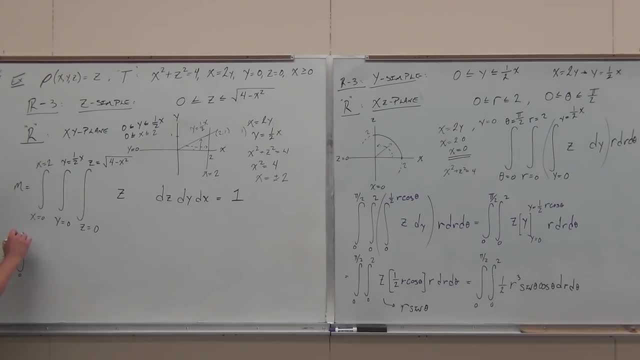 Sorry about changing sides of the board on you, So integrating with respect to r, we get this one eighth. r to the fourth, We're going to plug in for r 0 and 2.. And then we're going to have this: sine theta, cosine, theta d theta. 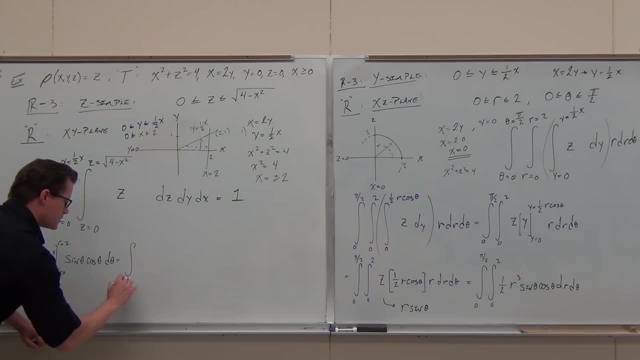 Well, that looks friendly: 0 to pi over 2.. If we plug in 2, we're going to get 16 over 8.. That gives us 2.. Plug in 0, we get 0. So we end up getting 2 sine theta d theta. 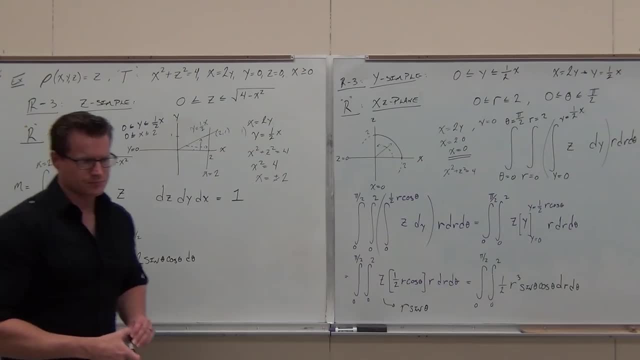 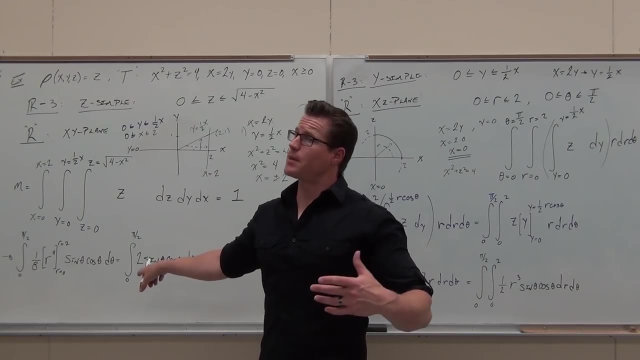 Cosine, theta d theta. Yes, no, That's really friendly. You have options here. You could do what. That's what most people think And that's fine. You can do it right now and get the correct answer. You could say: well, you know what. 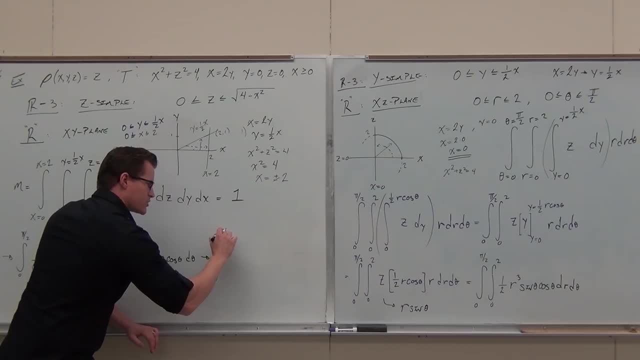 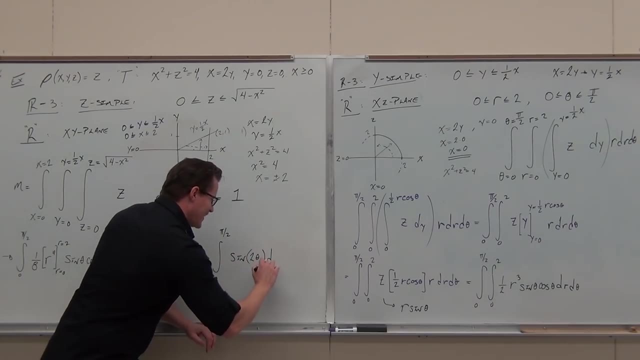 That looks an awful lot like this one identity that some of my trig teachers tried to get me to learn And I never did. It exists. Maybe you know it. That saves you some time, Because then, instead of a real u sub, you have a trivial u sub. 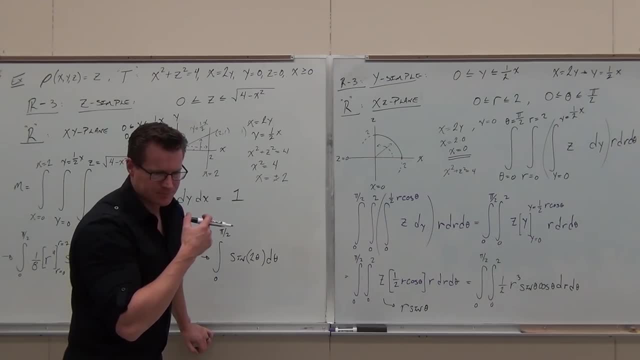 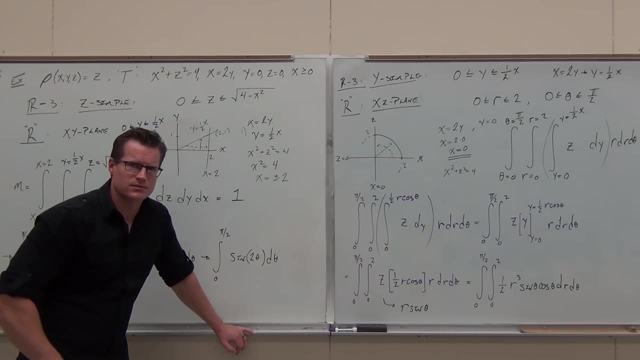 And you go. well, this thing right here, that's that. well, what's the integral of sine Negative cosine? And then this is the opposite of a chain rule. u sub is the opposite of a chain rule. So, instead of multiplying by 2, you divide by 2.. 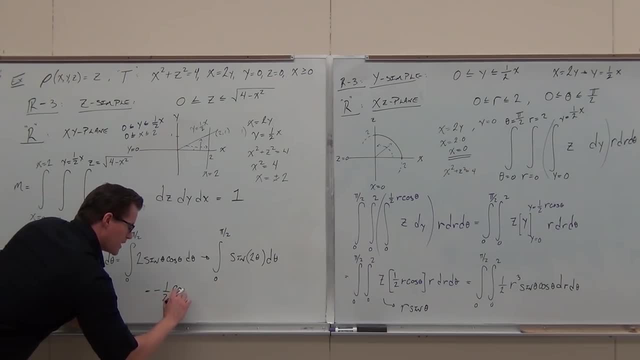 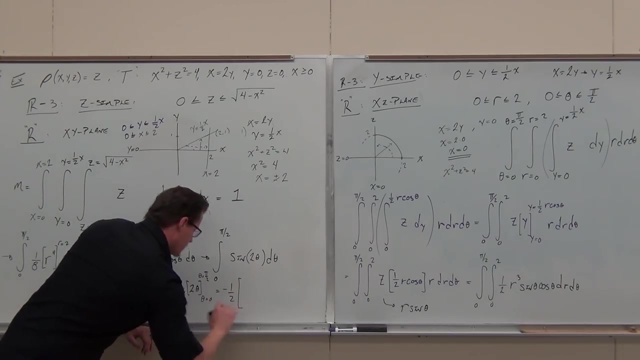 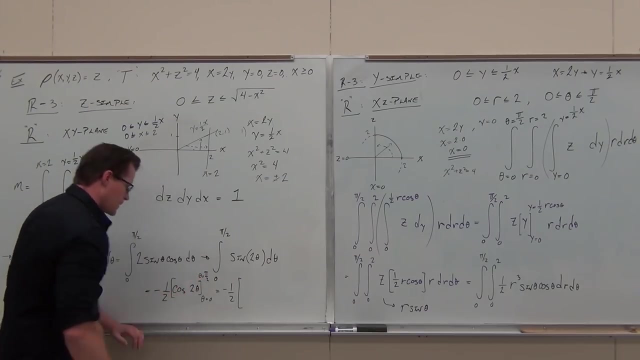 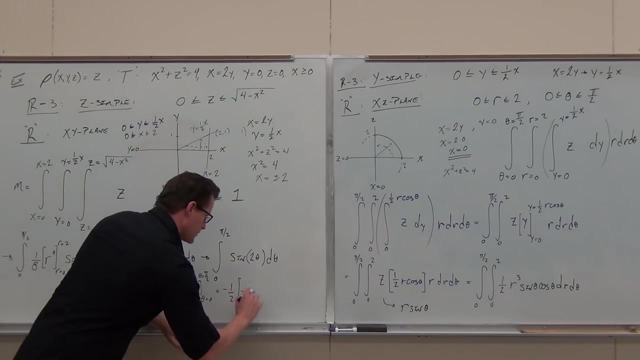 So this would give you negative 1 half, cosine 2 theta, And theta is going from 0 to pi over 2.. Which means we get negative 1 half And we get this thing: We got cosine of pi Minus cosine of 0. 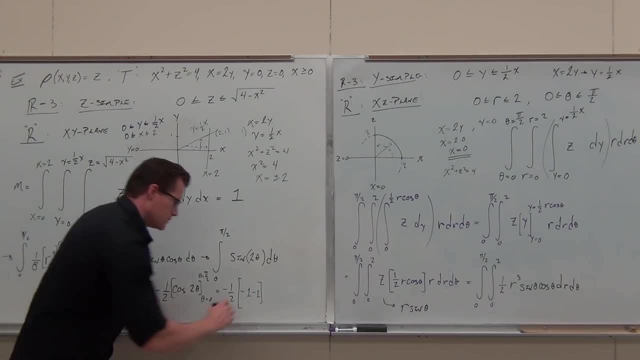 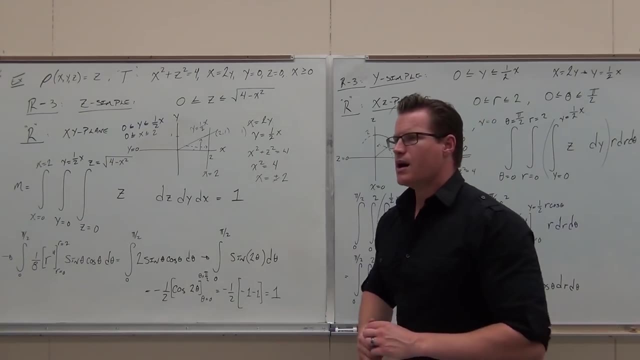 And we got negative. 1 half times negative. 2. Negative times negative is a positive, We get 1. Same thing. You get the same thing either way. The key here was identifying what the correct setup is. After that, integration pretty easy. 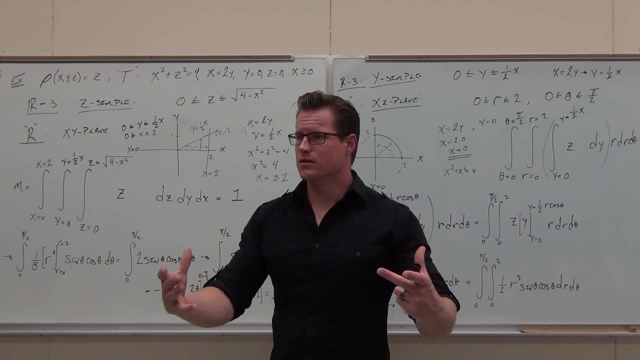 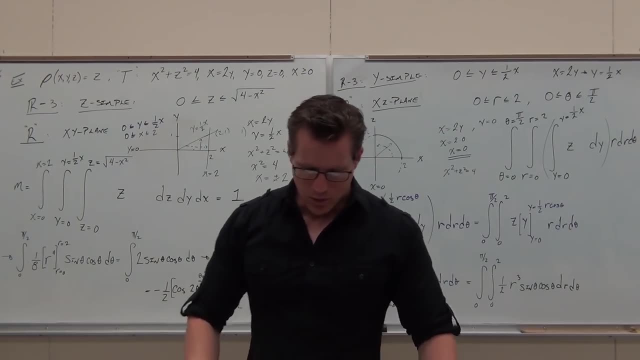 Honestly, you guys are smart guys and girls. You know how to integrate. So I want to make sure that you guys are OK on the setup. Show of hands if you feel OK with the setup. OK, We got one more. We switched gears for a little while. 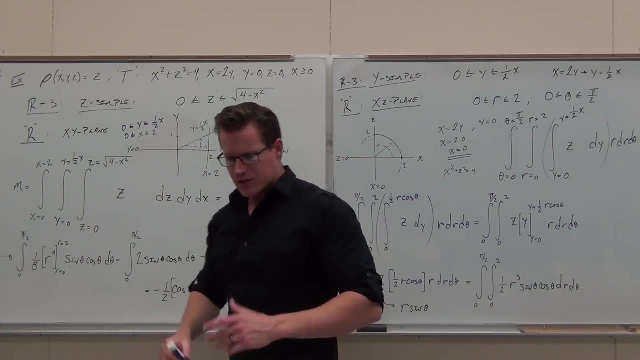 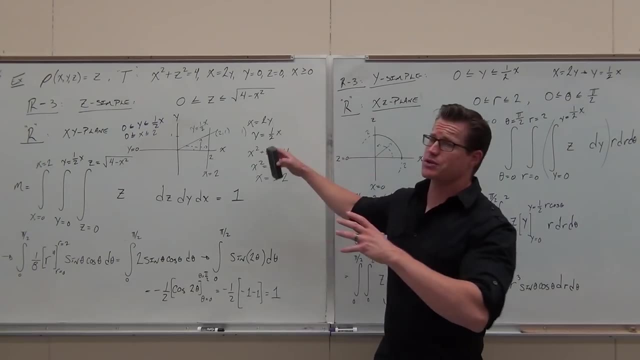 And then we're done with this section. So next, one kind of important Deals back with how you set up integrals across regions. Are there any questions at all? before we continue, Are you sure it's sinking in? You're on your head. 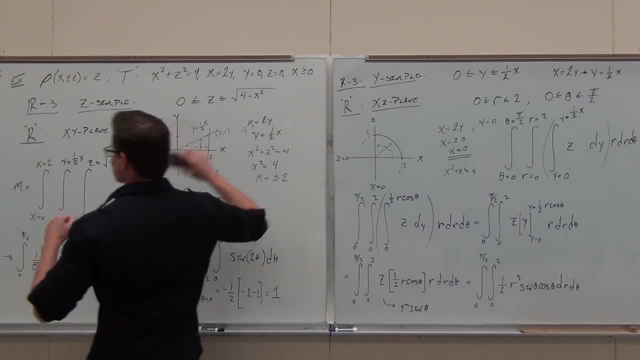 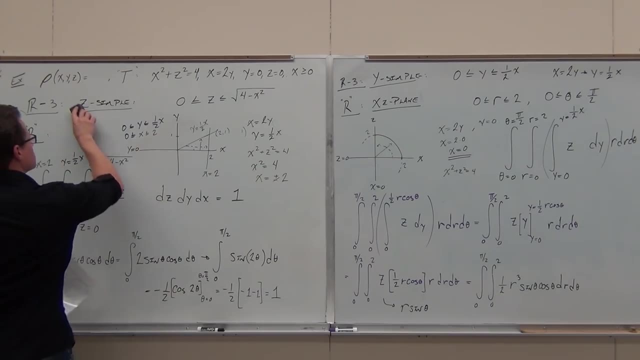 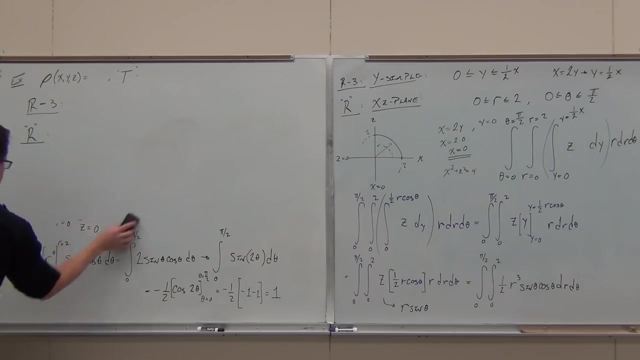 I want to make sure you all are with me. Yeah, OK, OK, So you're thinking about features of integrals. Are you still thinking of the code in eliminő, Tony? I think I'll let you take that up, Thanks. 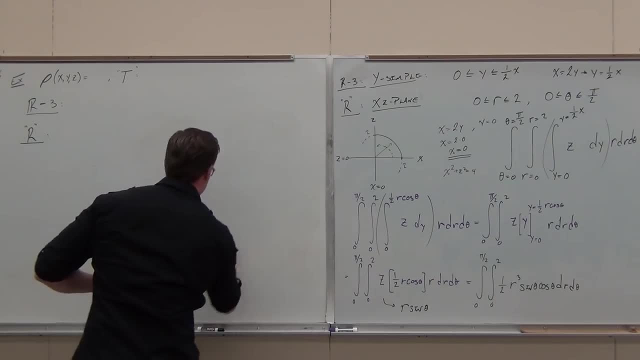 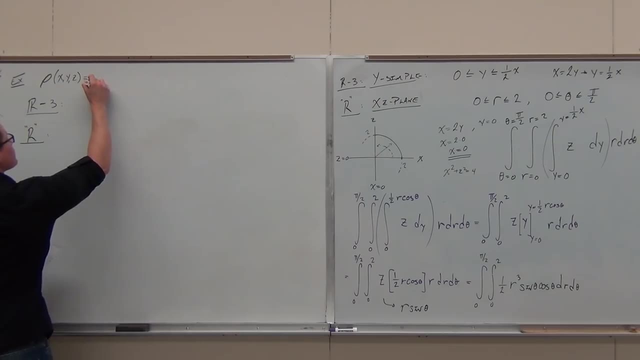 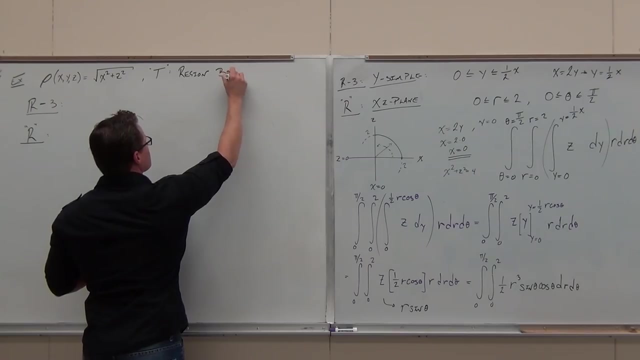 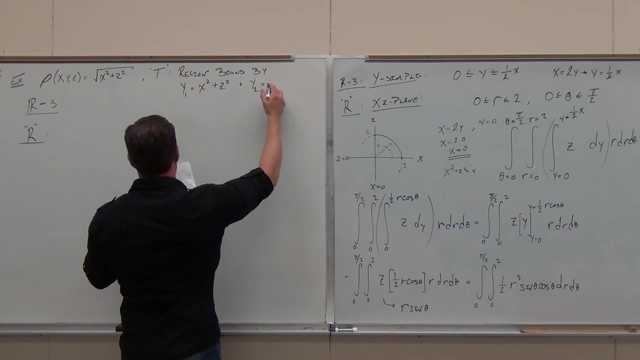 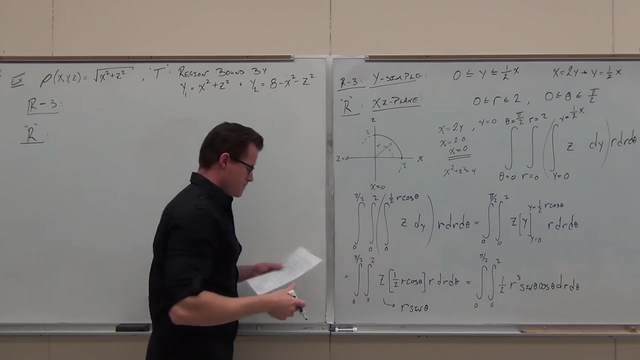 This last está bien, Steve, You two been playing around, Okay, All right, Sweet, Okay, what I want to do? same type of question. I want to find the mass of the region, mass of the 3D region. 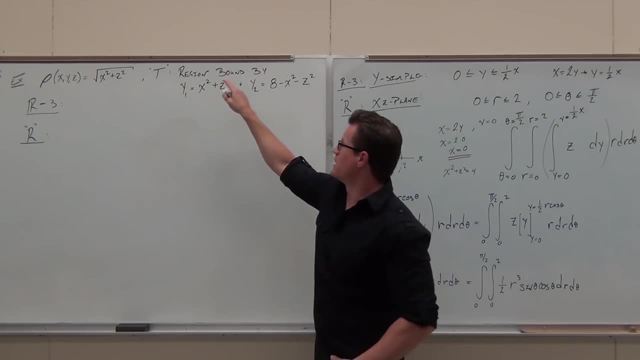 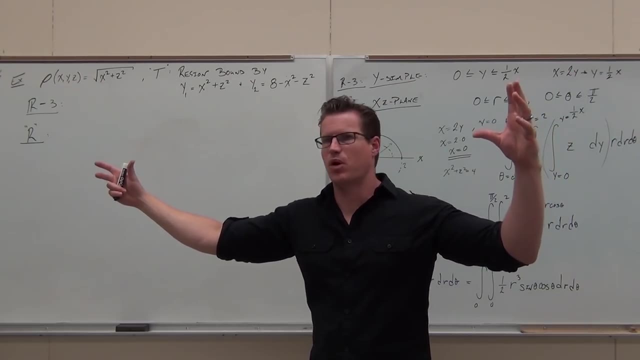 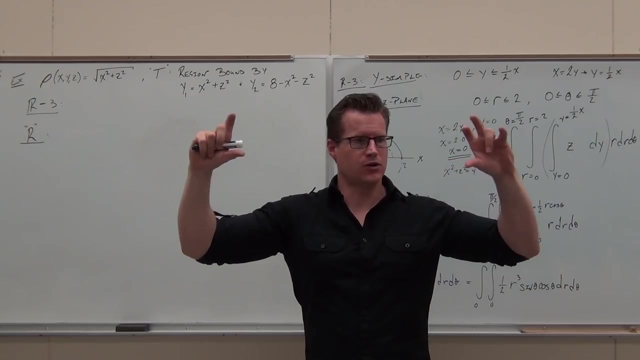 where the mass density function is at that one and our 3D region is bound by these two curves. Listen, I'll give you just an overlying concept that fits for basically any part of calculus, If you ever have to find the whatever bound by two functions. 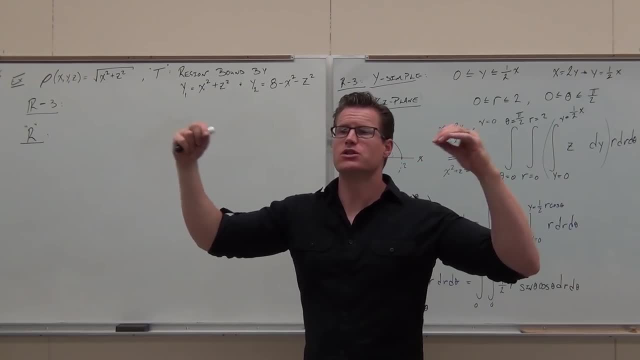 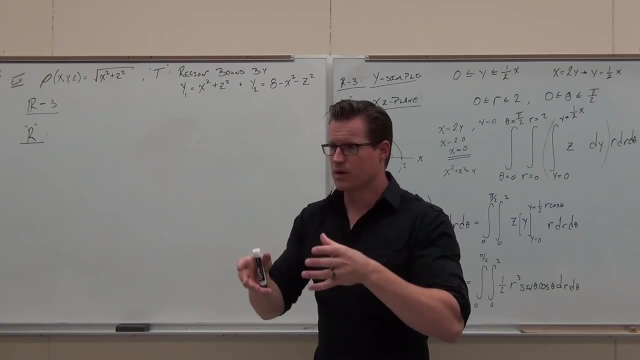 you need to find the intersection of those functions. If you want to find the area between two curves, you set the curves equal to each other. you find the intersection. If you want to find the volume under a surface bound by two regions, 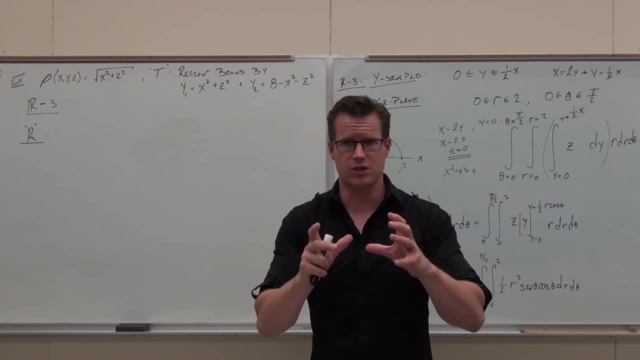 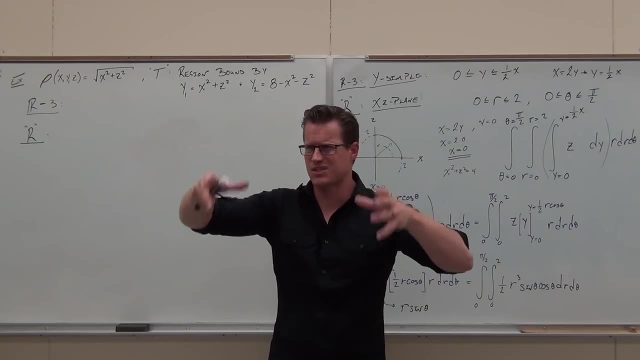 you set the functions equal to each other and you find this region. So when I'm not given stuff like hey, x equals 0,, y equals 0, some planes, some curves, some cylinders that define for you a real nice 3D region. 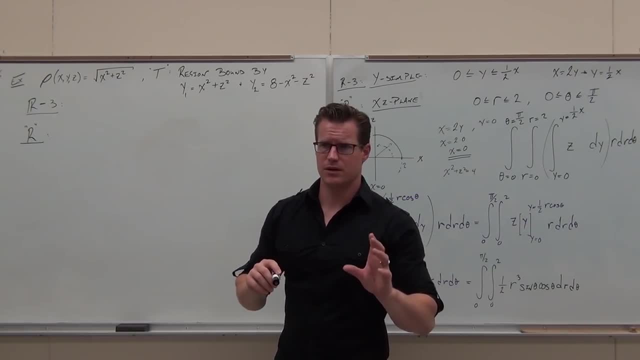 the idea is going to be this: Can I have your attention here real quick? I know you're writing stuff down, but the idea is this: If I set these functions equal to each other, it's going to give me an intersection. That intersection is going to be a curve. 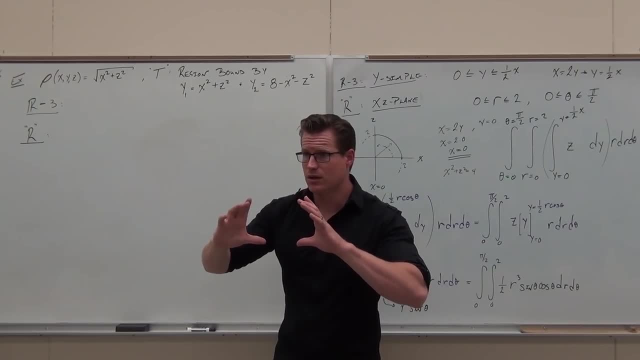 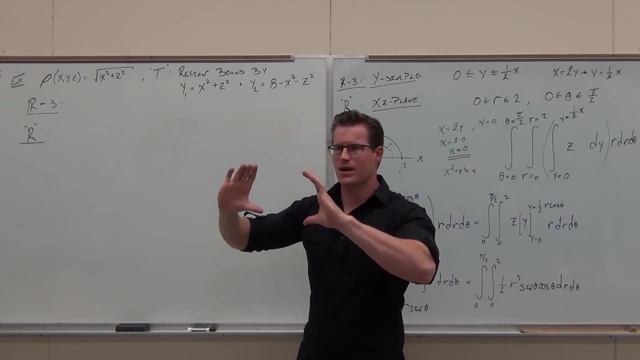 The intersection of a 3D region is a level curve. Does that make sense? So what this is going to do, when I set these equal to each other, gives me some sort of curve. That curve gives me this cylinder that contains this volume. 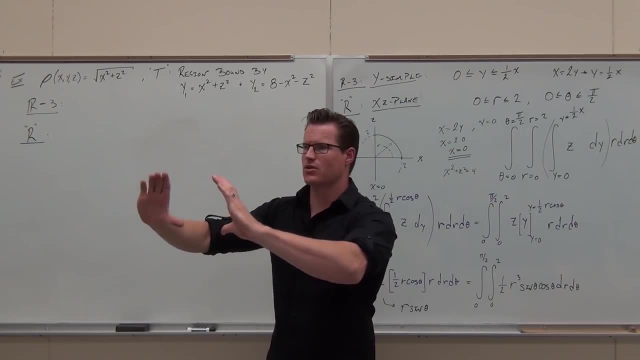 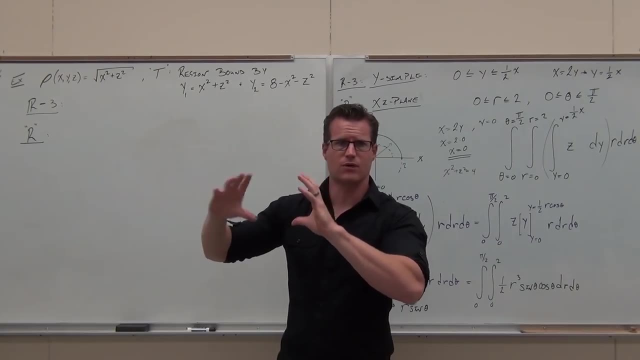 That's what's happening. It's giving me this thing that if I integrate across, it's going to have the volume inside of that level curve. It's like the outer bound for our 3D region. here our volume we're trying to find 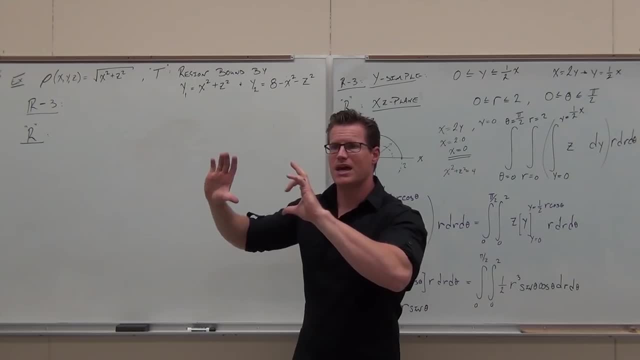 Does that make sense? So, find the intersection, Give us a level curve, Integrate over that level curve. That is the region that that 3D surface- sorry, 3D region- is going to be hanging over. That's the idea here. 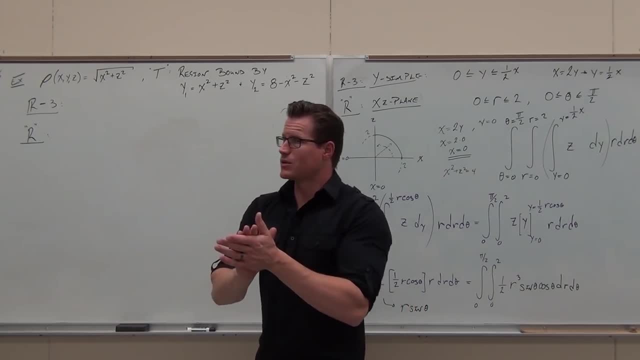 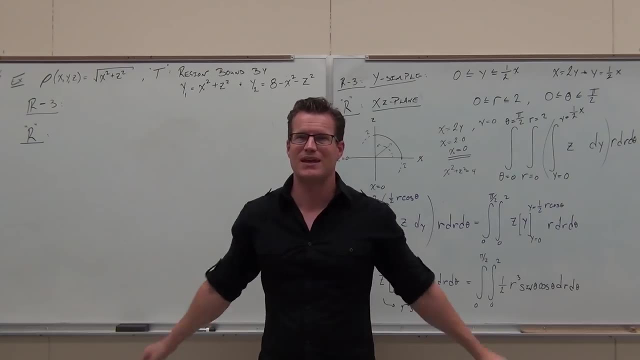 Head on if you're okay with that one. So now the first idea: set it equal to each other. But before we do that, you're going to pick right now whether you think we should be R3 simple, in X direction, Y direction or Z direction. 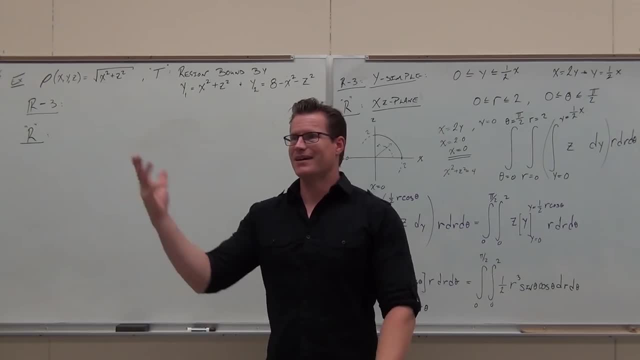 This one should be kind of obvious. What is it Y? Y, Because Y functions equal to Y. I mean por que? Por que es X, It's, they're equal to Y, They're literally equal to Y. That's a really nice choice. 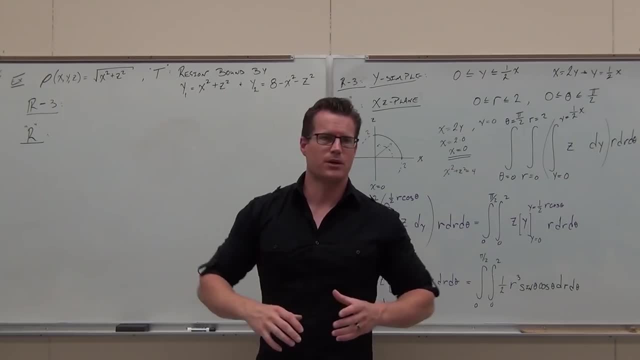 So if you have two functions that are automatically equal to Y, you're probably going to do Y simple. Does that make sense? We try to do Z simple all the time, but I mean, shoot, if they're just going to give it to you, I mean take it. 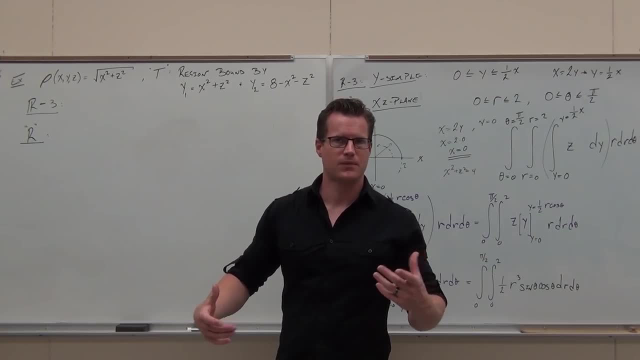 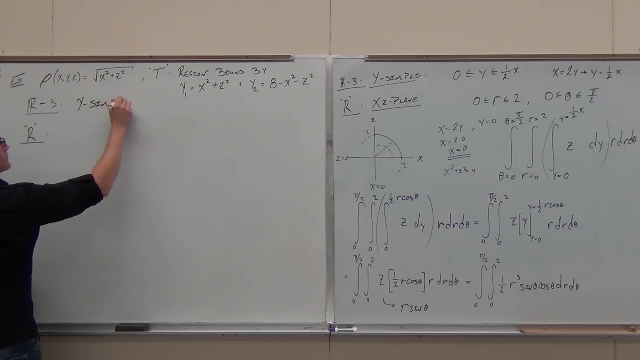 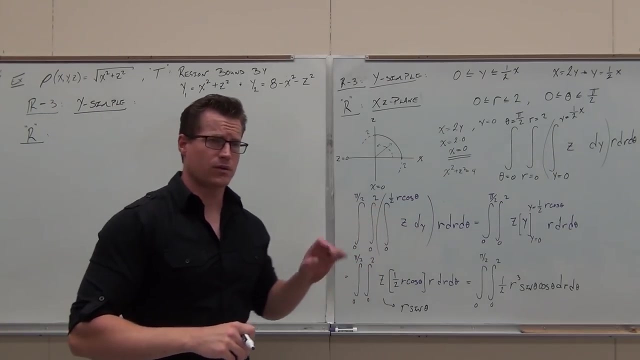 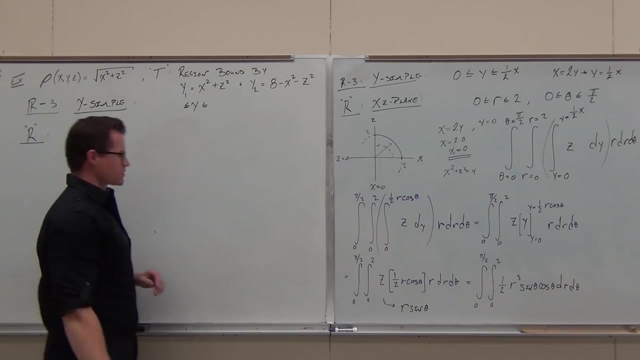 So this is going to for sure be Y simple Head on, if you understand Y literally. Okay. So if we're going to be Y simple, travel across a 3D region along the Y axis. first we have to match Y between two functions of Y equals. 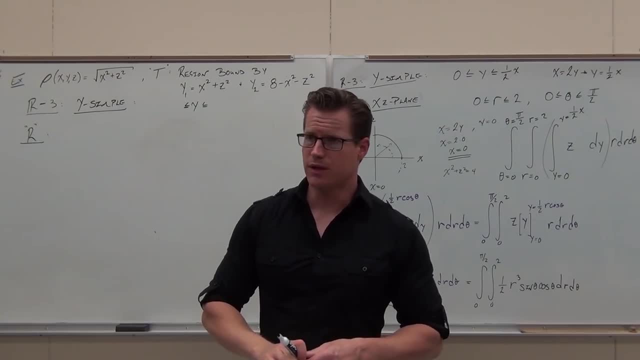 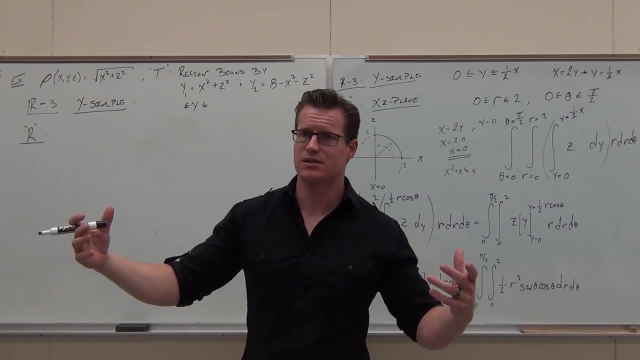 Now it's going to be up to you to either do this intuitively or hang on for a second to get the region. Me personally, I can do a lot of these intuitively because I watch section 11.6 and 7. 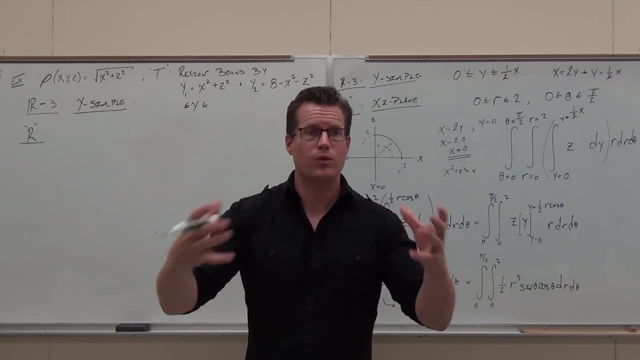 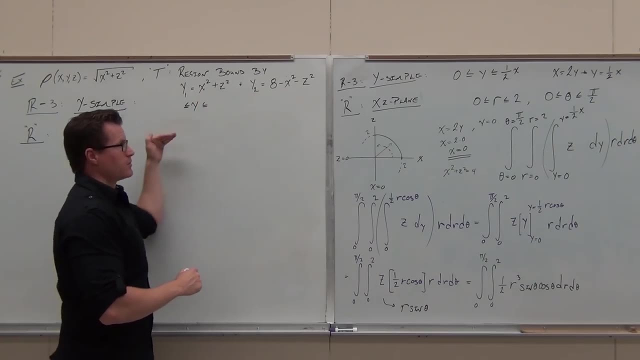 and know how to do polar coordinates and graph. okay, So I know what these surfaces look like. Okay, This surface that's intersecting the origin, This one ain't. I'm going from, on the Y axis, something that intersects the origin, something that doesn't. 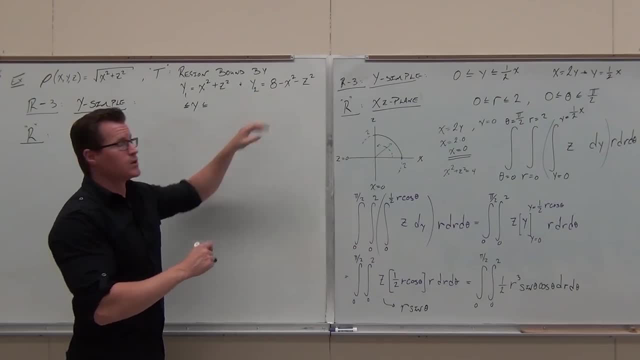 That's going to be the smaller of these functions and that's going to be the bigger. So right now I know that this is going to be X squared plus Z squared and 8 minus X squared minus Z squared. Wait a minute. 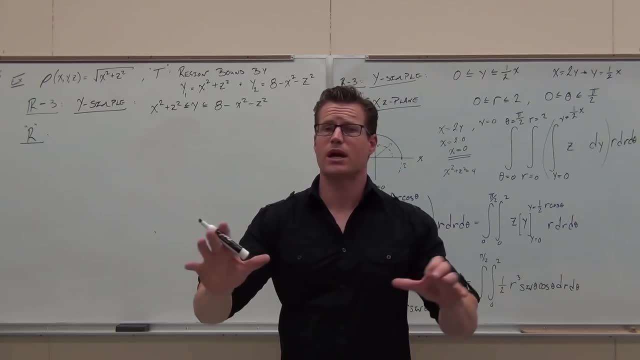 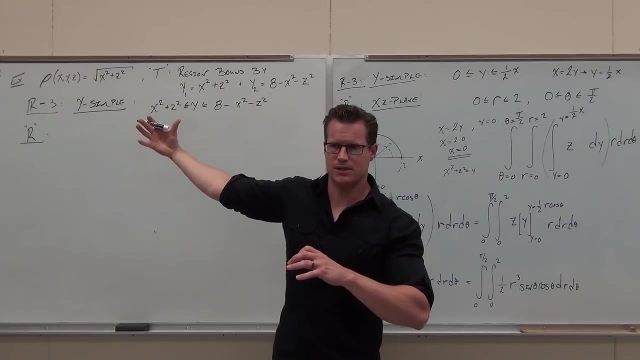 I don't know how to do that. I'm not intuitive, I can't picture this. That's okay. That's okay. You just won't get this right Now. you just wait a minute, You do the R and we come back to it. 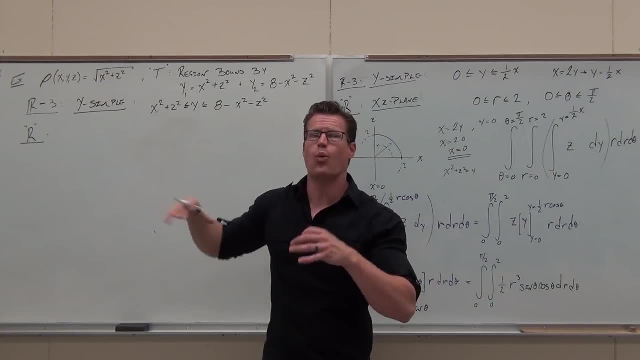 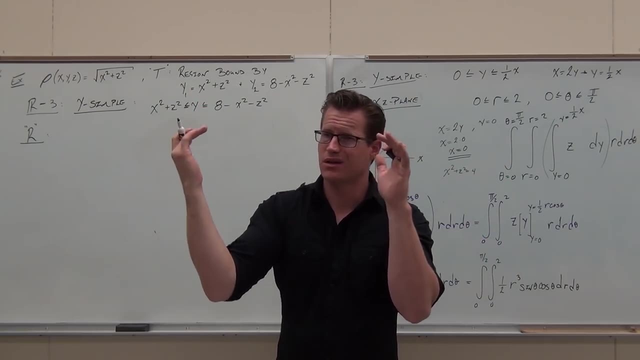 Does that make sense? I'll show you that in just a second. The key right now is understanding why we are doing Y-symbol. Do you understand why? Okay, Every time we set up a triple integral, we do the inside integral across R3-symbol. 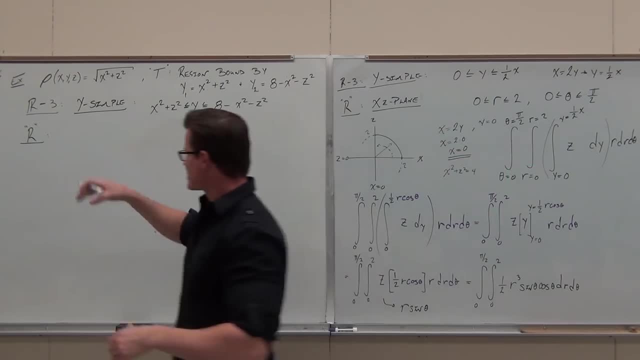 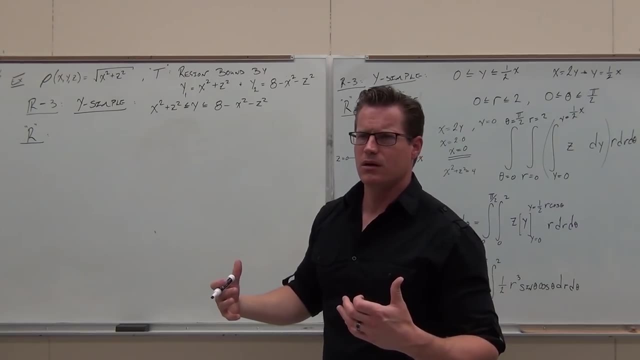 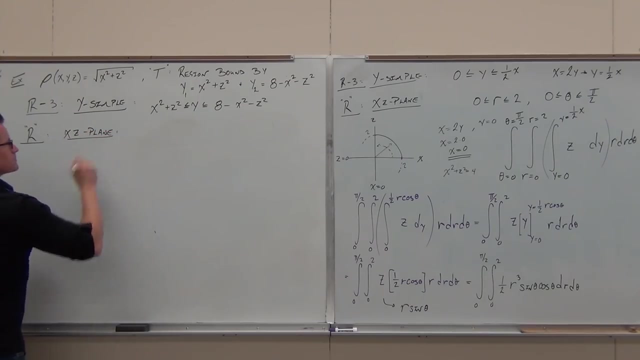 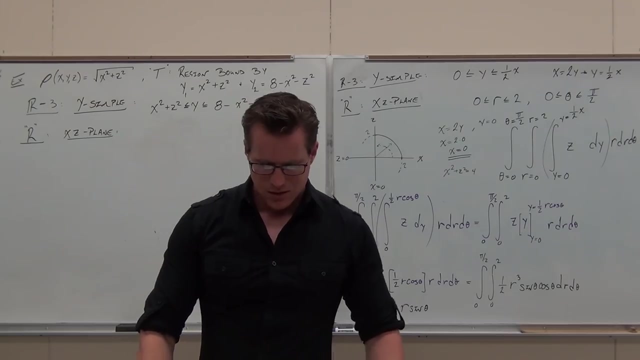 and then we have this double integral over a region on a coordinate plane. So let's set that up. If I did, Y-symbol, left side only, what coordinate plane is our region going to be on Secondary? The XZ plane? Okay, Now what's the region? 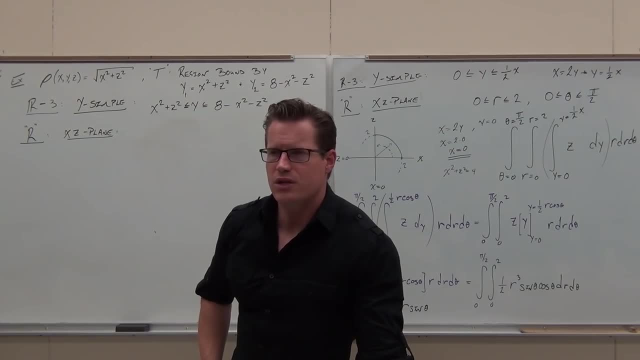 Listen, Listen. The region that we talked about at the beginning. you should be working right now. I don't want you doing the wrong thing. The region if you just put Y equals 0, and you just put Y equals 0,. 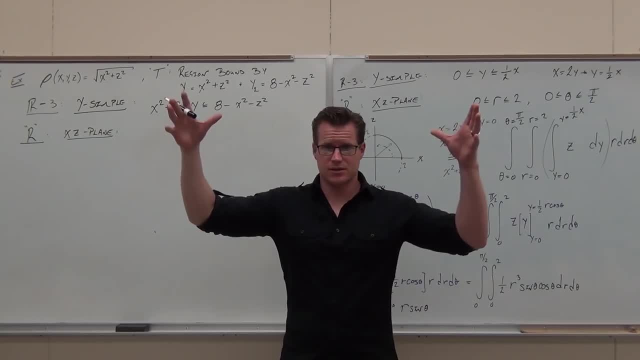 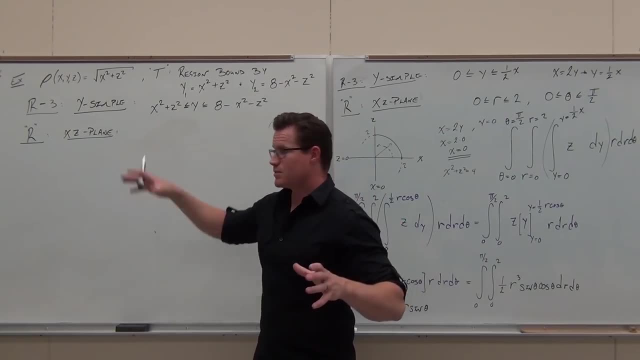 what you would find is that the XZ plane is going to be on the XZ plane. What you would find is where this intersects the Y axis at the origin. That's what you're going to find. You're going to find where this intersects the X- sorry, the XZ- plane at that, whatever that circle is. 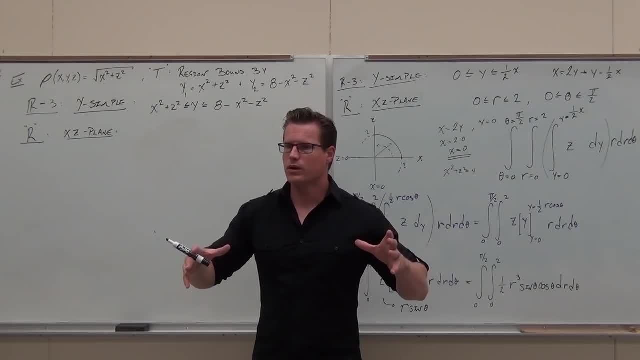 Okay, That's what you'd find. That's not what we're looking for. What we're looking for is that level curve that contains so, that big cylinder, that going along the Y axis, that contains the volume. So, if ever you have the region bound by these things, bound by two curves, 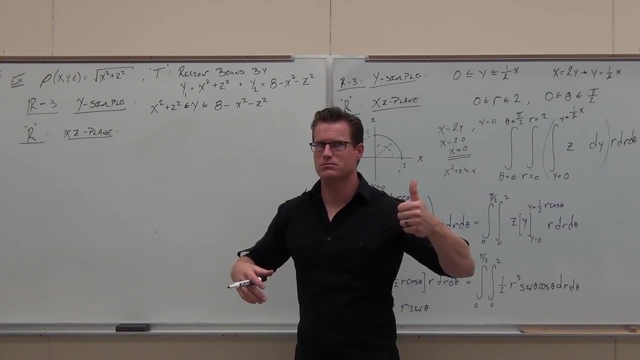 first thing you do in Calc 1, set them equal to each other. First thing you do in Calc 3, set them equal to each other. Find the level curve that will give you the region. If you set them equal to each other, the Y's are gone, will be on the XZ plane. 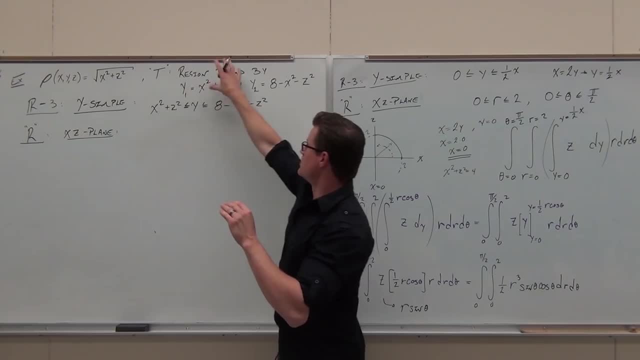 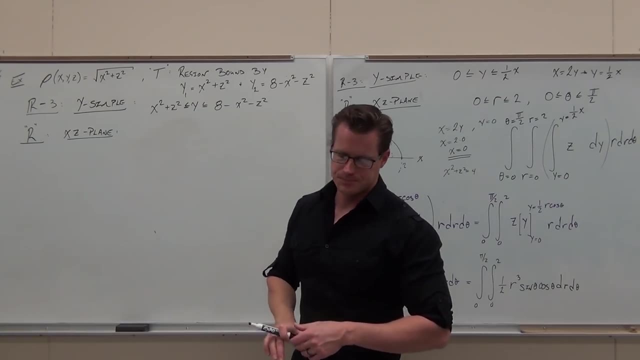 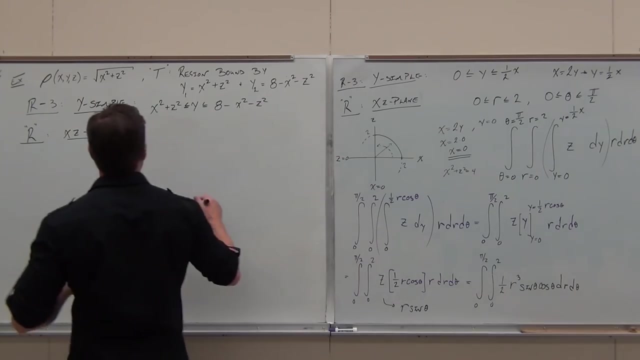 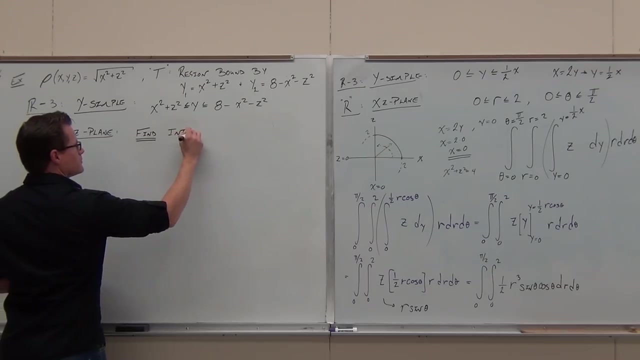 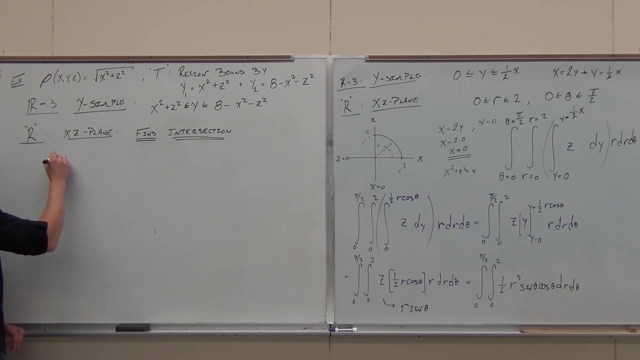 Does that make sense? So if you have region bound by, set the functions equal to each other and find the level curve, Why don't you try that right now? Set them equal to each other. That's all I wanted from you right now. 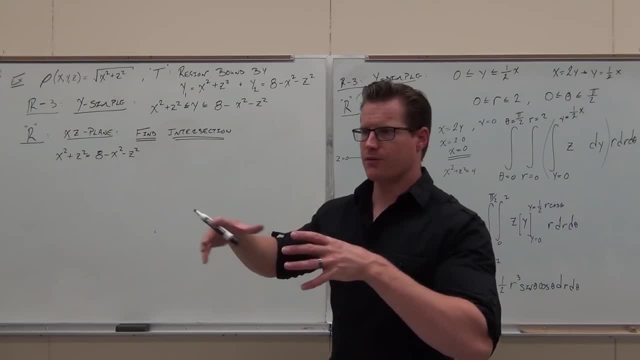 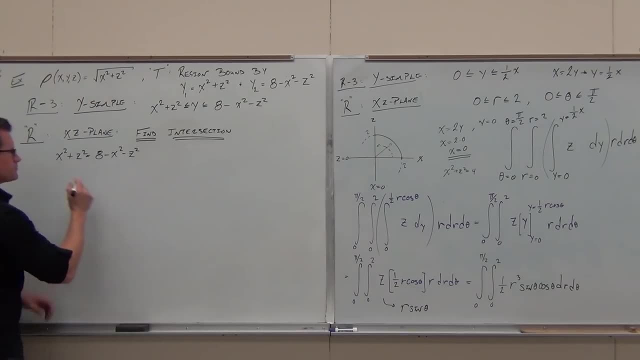 Did you set the functions equal to each other? Right now we're finding that That level curve that creates a cylinder that contains that 3D volume that we're trying to locate right now, the 3D region. By the way, you know you could do some fancy-pants math on this stuff. 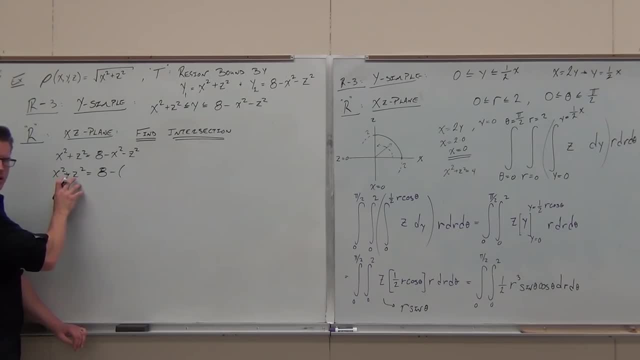 Make sure that you're looking for the squares, plus squares a lot, because if we're going to translate to polar, which that's really helpful, So do things like, factor out the negative. Don't be afraid to view this as one kind of one piece. 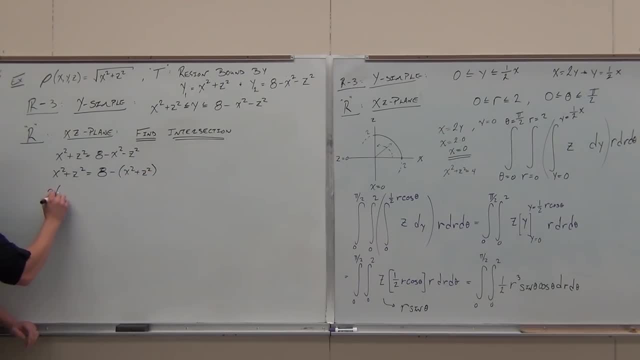 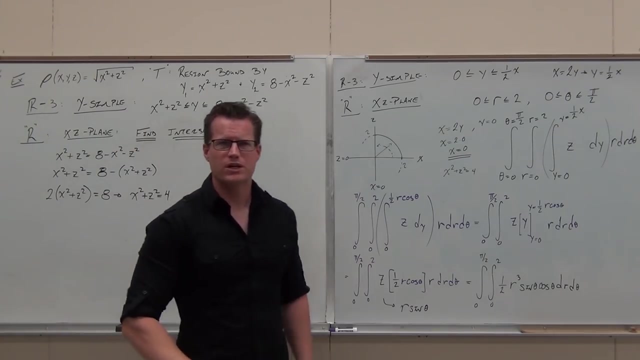 If I add this to both sides, I got one of them, I add another one. I got, I got two of them now. So some algebra technique. it really helps Divide by two. That's a really nice way to figure out what this region looks like. 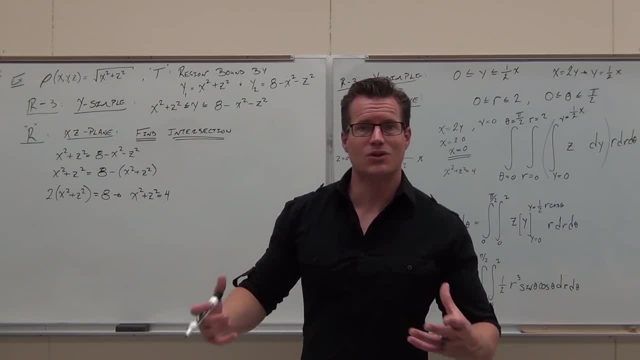 What's that region look like? Draw the circle: Is it a full circle? Yes, Yes, that intersection is. that's what's all matter. So what's what's nice about these, these regions that are bound between two functions? 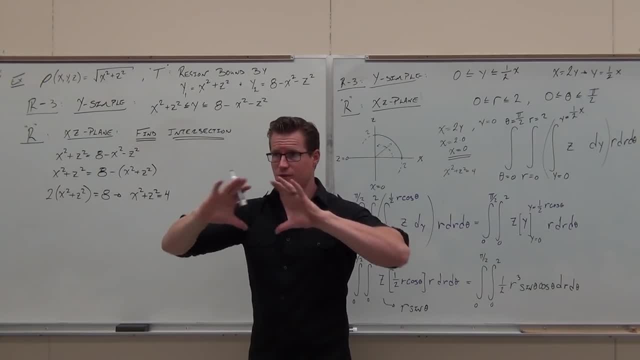 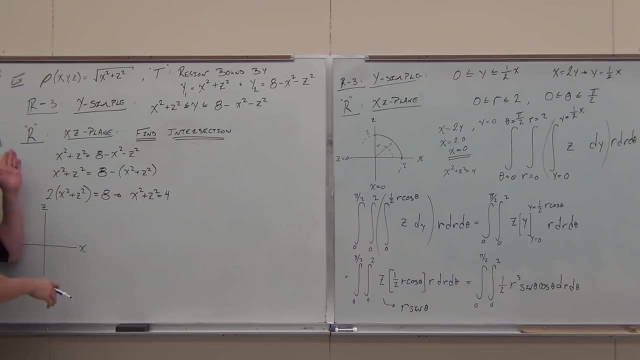 is. it typically gives us a nice level curve. So this level curve is is a full-on circle. Draw the circle. Draw it on the XZ plane, where Z is the vertical. It's got to be a circle centered at the origin with a radius of two. 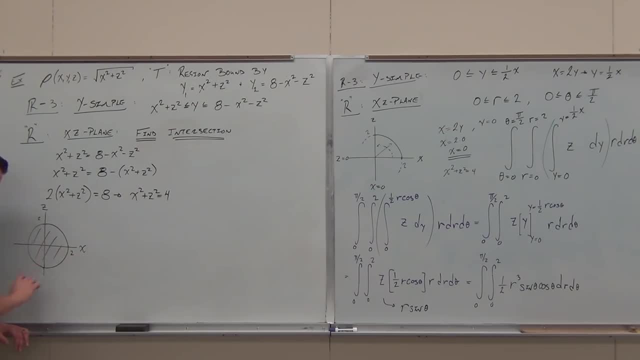 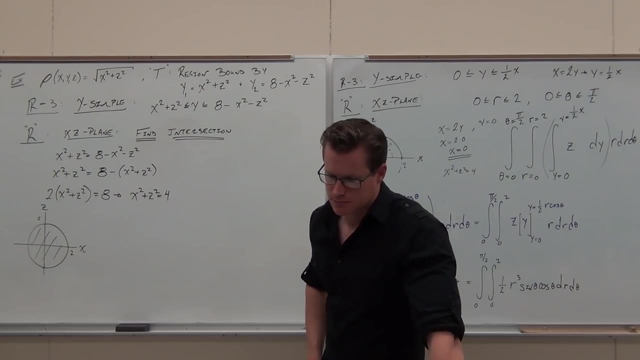 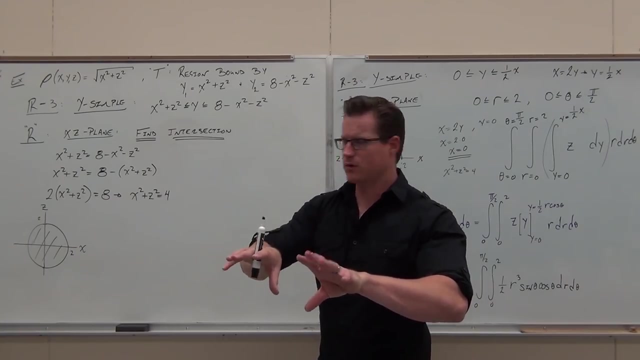 And the region is the entire circle. Okay, Since we're literally just dealing with a double integral now- and this is literally the only reason we have to worry about- would you do this in terms of rectangular, or would you do this in terms of polar? 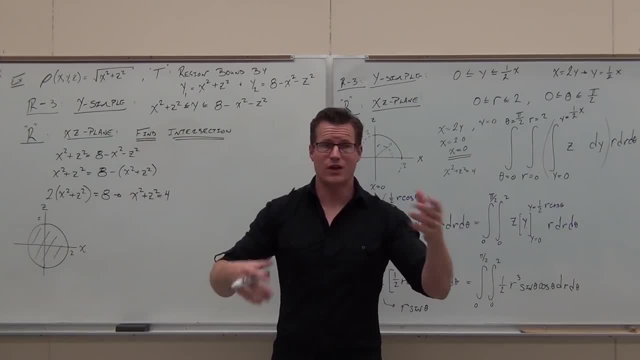 Polar, Why? Why? Why? polar Circle Circle. So if it's a circle and all we got to worry about is DR D theta, Let's define our R and let's define our theta. Let's do it right now. 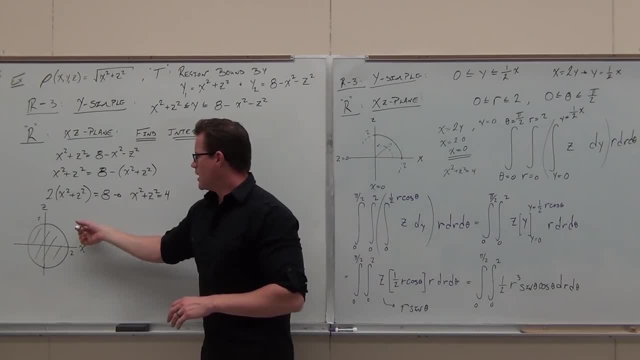 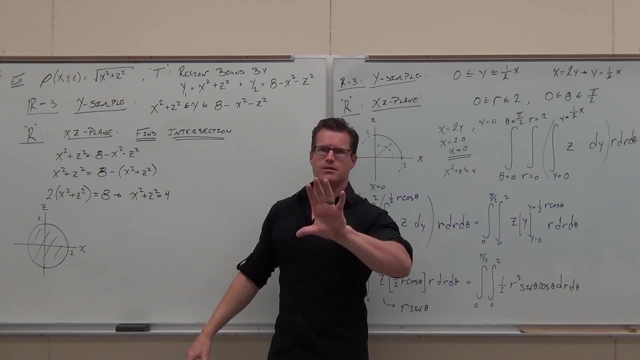 I've already got Y between two functions. We'll talk about R between two functions, Okay, And we'll talk about theta between two constants. By the way, stop, stop, pause. I need to make sure you see this at this point. 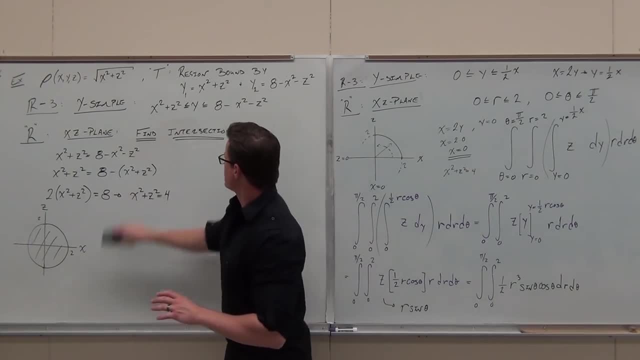 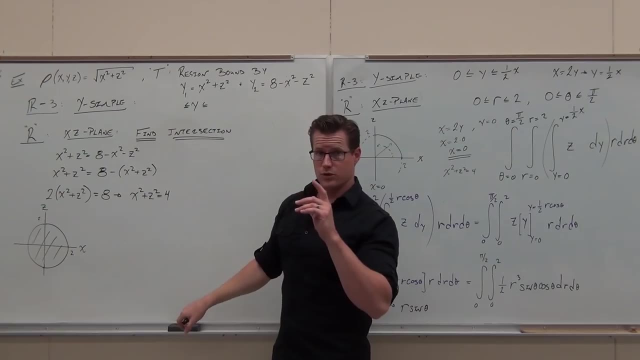 If you don't have this right now, I don't know what this is. If that was you like, ah, you told me you were going to tell me, This is where you would find it. So you know that you're going to be between two functions of Y, because we have Y equals. 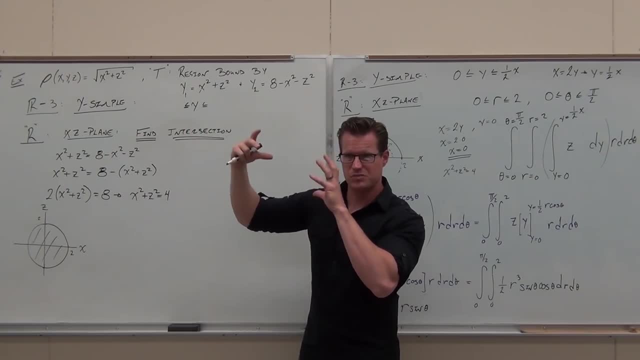 That's called Y, simple across the 3D space there, If you find your R on XZ, Okay, Okay, XZ plane, yes, set your functions equal. Find the intersection That gives you that level curve that's going to contain. 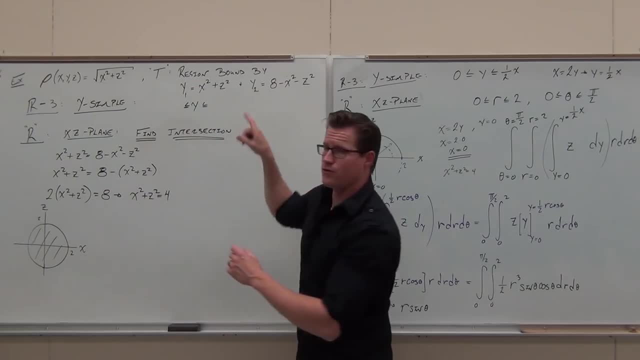 This thing's going to shoot out there. Okay, It's going to shoot out there. It's going to contain the volume between those things. That's what it's going to do. That's why we find it. We integrate over this area. 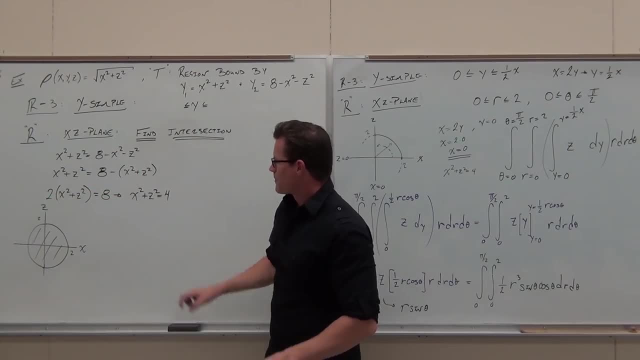 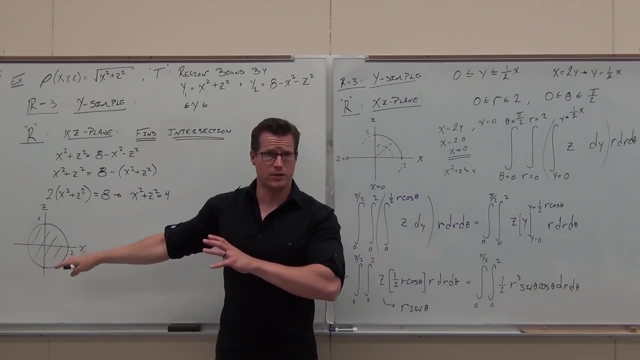 We find the volume of that. That's brilliant. But as soon as you find this region, if you were not able to intuitively tell me what's smaller and bigger, this is where you do it. So, on the XZ plane, find a point on the XZ plane. 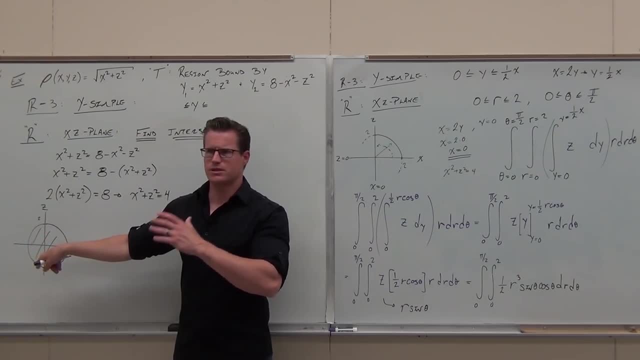 On the inside of your region. Give me a good point: Plug in 00. if you can Do that, So plug in something inside there, though Not on the edge. Inside, Doing an edge is going to be equal. Don't do that. 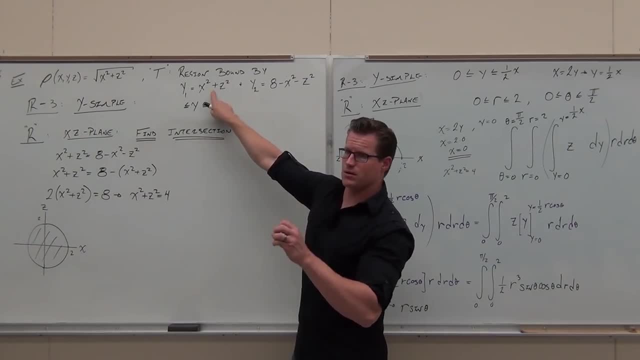 Inside. So plug in 00.. If I plug in 00 here, I get 0.. If I plug in 00 here, I get 8.. Which one's bigger? Well, 8.. Let me tell you that is the larger of the function. 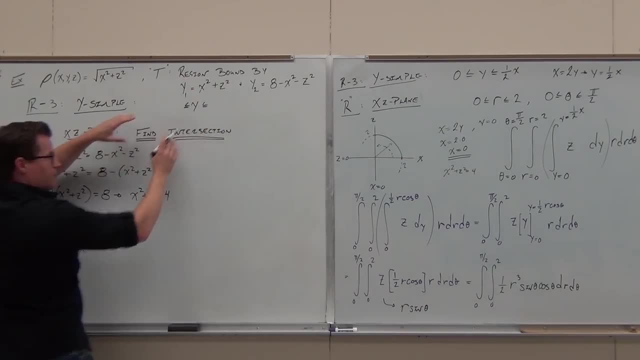 So if you weren't able to find it at first, now you go. well, that gave me 0 for some point on the inside. That gave me 8 for some point on the inside of this region. I don't care about what's outside. 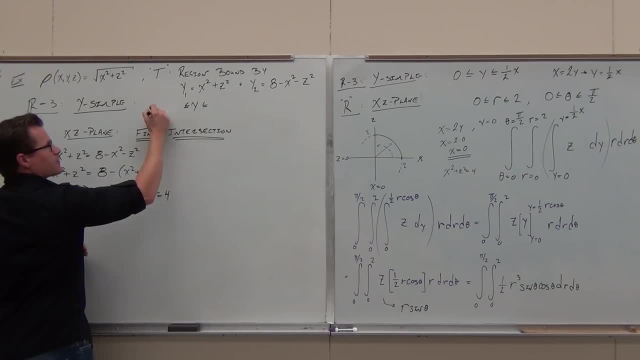 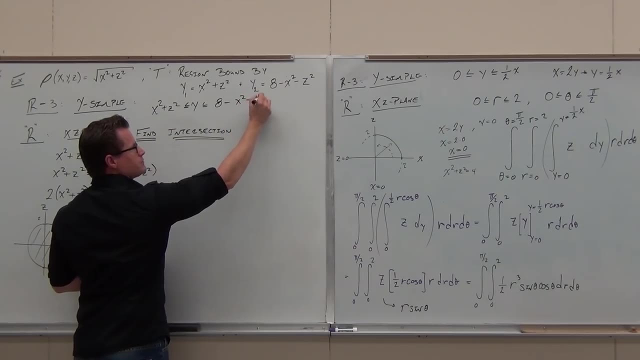 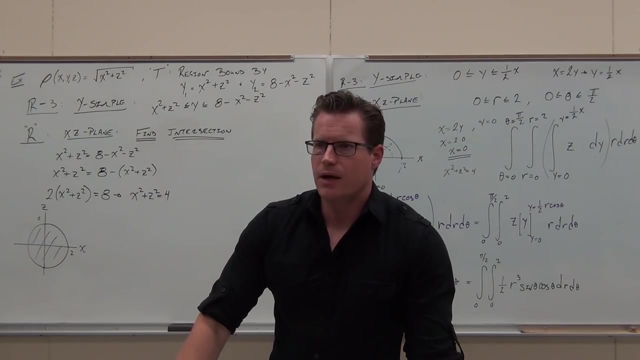 care about just points inside, not on the region, just inside. therefore, this is the smaller of these two functions and that gives me the high one, and alone that's the best whole idea. now I'm gonna go a little bit deeper on your understanding here. okay, check this out. do you remember when we found volume between two? 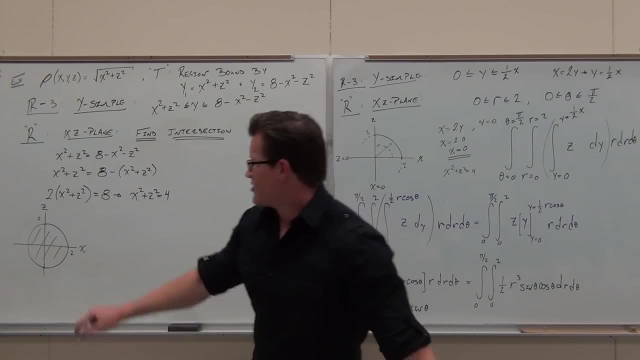 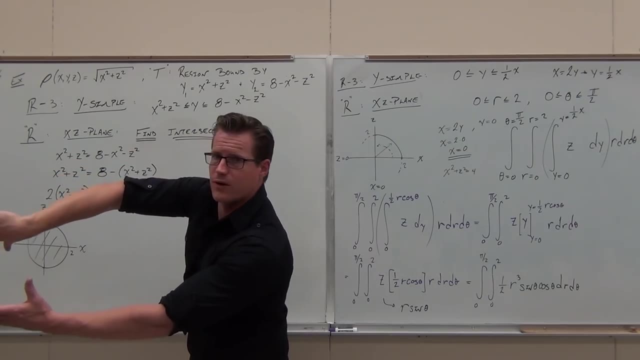 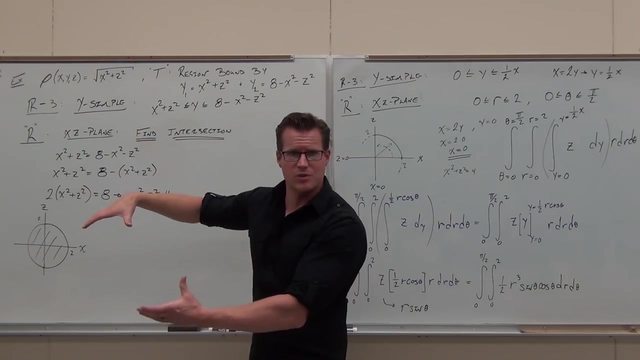 surfaces. you found the intersection. the intersection created the region, and then what I talked about was: you're taking the cylinder out, you're intersecting a smaller function and you're intersecting a larger function and you're subtracting the volume bottom from top. do you remember doing that? the 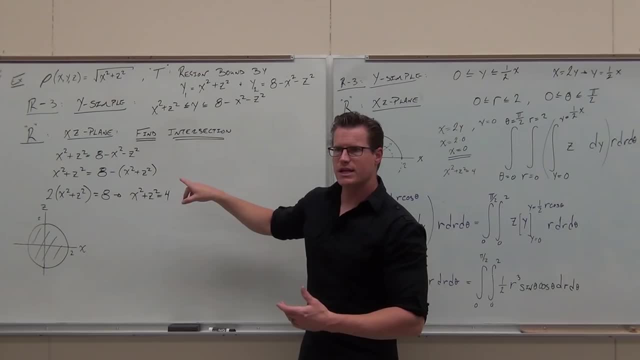 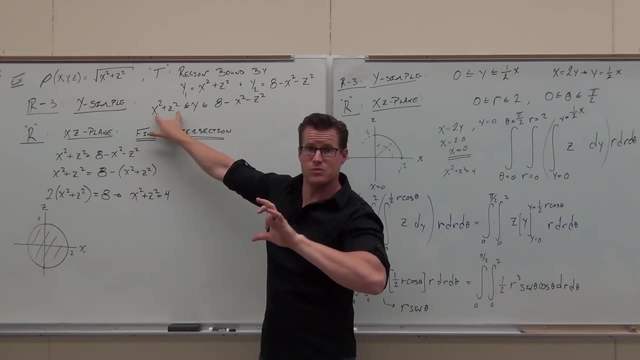 intersection port. for that reason, when you do your, your integral setup, do you recognize that that is going to be what? you plug it on the top, that is what you're gonna plug in on the bottom and you subtract them. that's exactly what's happening. you're literally doing the same thing, but you find intersection to. 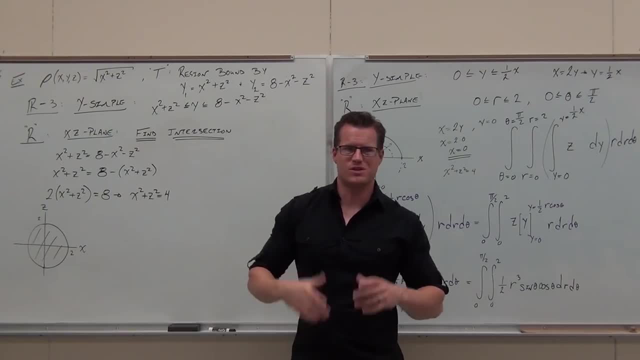 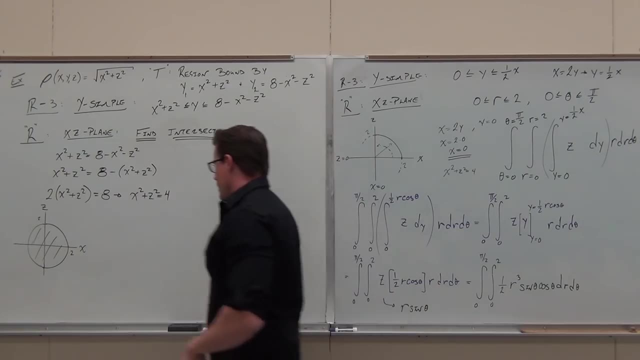 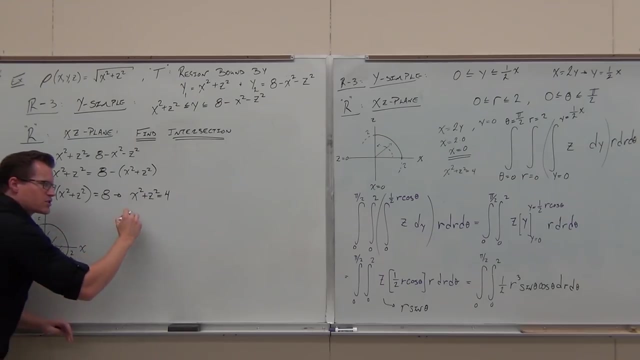 give you that cylinder so that you can subtract those volumes. in this case is mass of the region. but that's a second idea. you guys get that, that idea, okay, so now we're on it, let's go ahead, let's start changing this. we know that if this is our circle, we can certainly change this into polar. 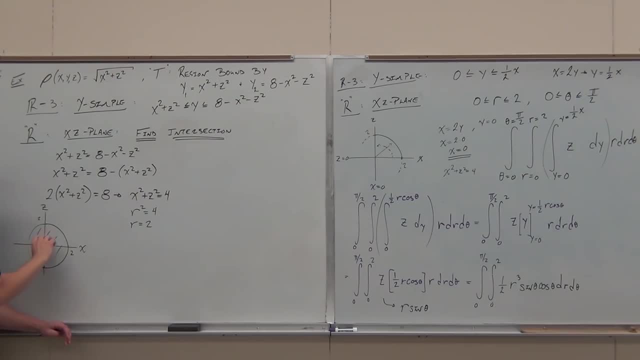 it tells us that, instead of going from zero to a function of X and Z, I now have well circle with X and Z. I now go from the origin to A radius of 2.. That tells me that I'm going from 0.. I'm going to start going a little quicker through here. 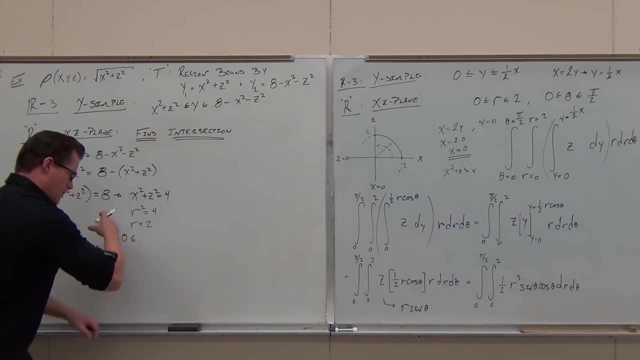 because I know we've done it many, many times, So I'm not going to be asking you for a lot of this, but if you're confused, you by all means stop me. So I know that polar function. this is I'm going. 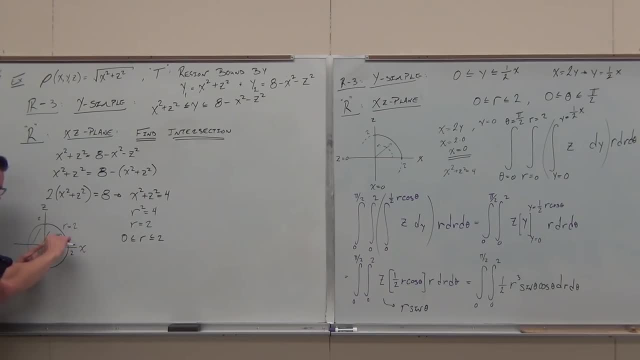 through the region from 0. So I keep my region immediately, and then I end at r equals 2.. I'm also going full circle on this thing. So that's 0 to 2 pi. If not, if you're with me. 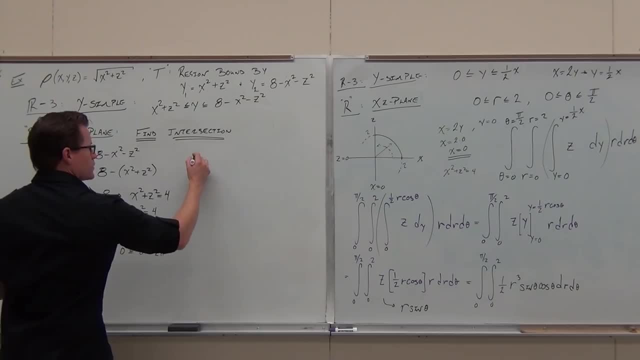 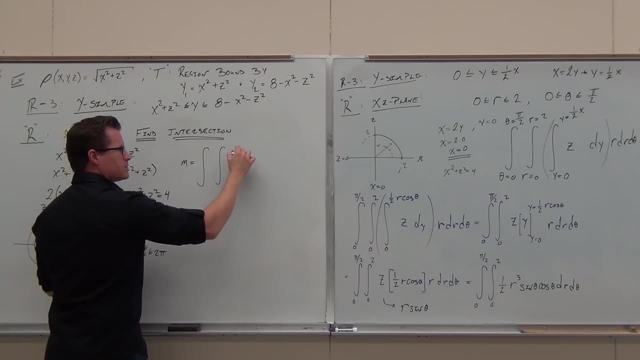 Okay, so we start changing, So we start setting up our triple integral. So, for a triple integral, I know that our mass- that's what we're finding here- Mass is going to start with a triple integral of our mass density function. 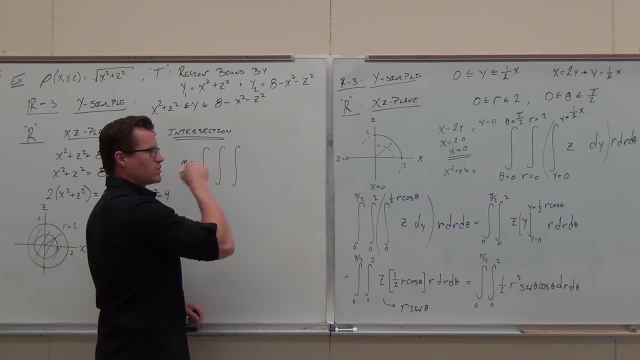 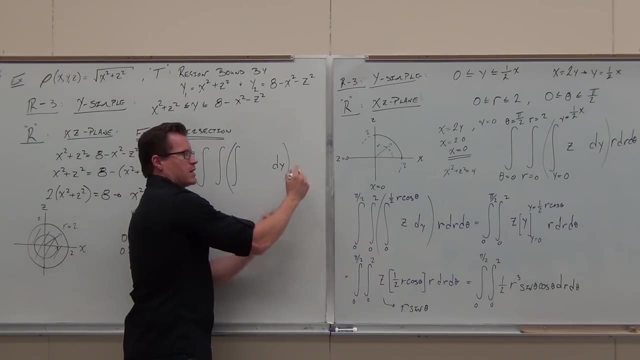 We're going to do that in a minute, But I know that I'm going to do: oh, what simple, what simple did we do? I need to set up my first integral, And then I know that my region for my double integral is polar. 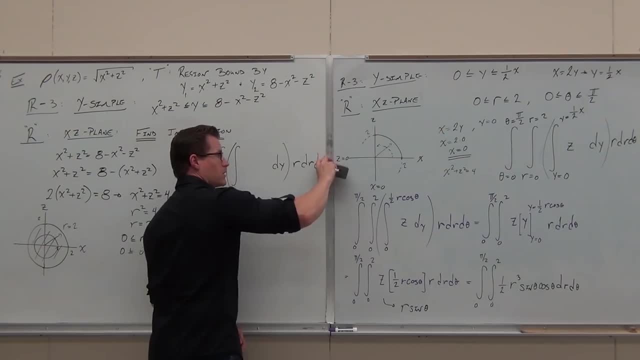 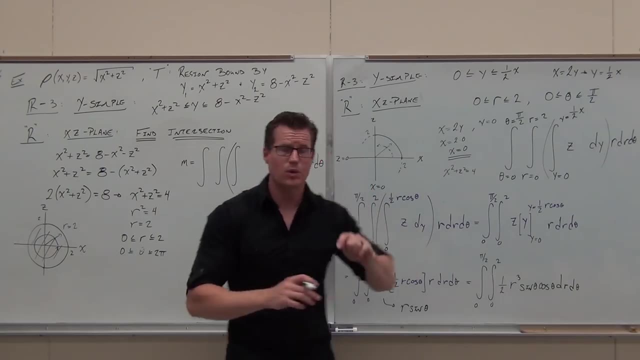 So I need to set this up. If I can write it correctly, it is basic integral, r3 simple. That's y simple. Then I've got a double integral. It was over a polar region, So I have a polar double integral after that. 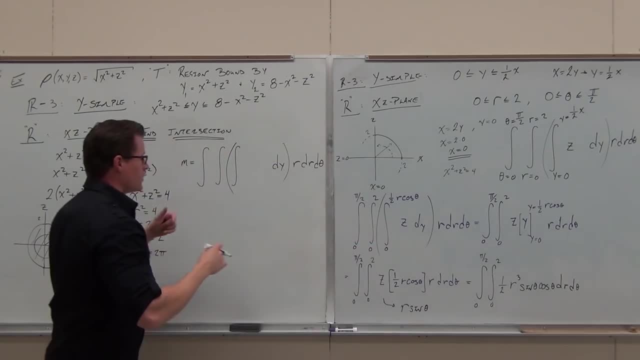 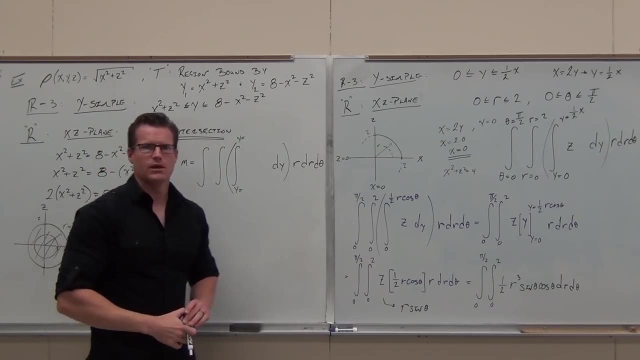 So you understand the concept there. That's the big deal. Now, now keep on going. This guy has to be y equals the small function to y equals the big function. Are you listening? You still have your attention. Do you remember over here how we had a little snafu? 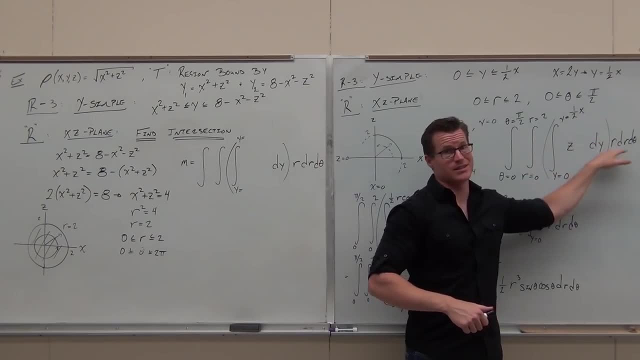 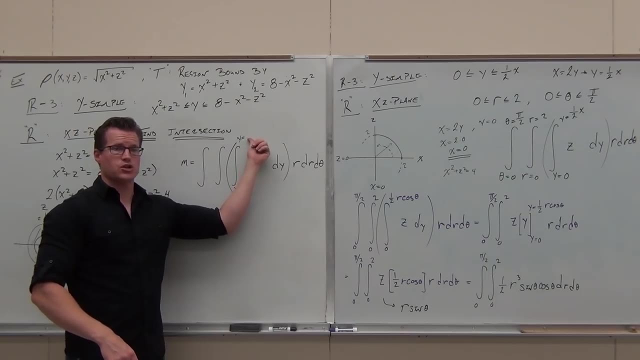 We had this one half x and went: ah, that's not over here, Let's not let that happen this time. So right now, if I'm going to go between y equals a function and y equals a function, I want to make sure I define it right. 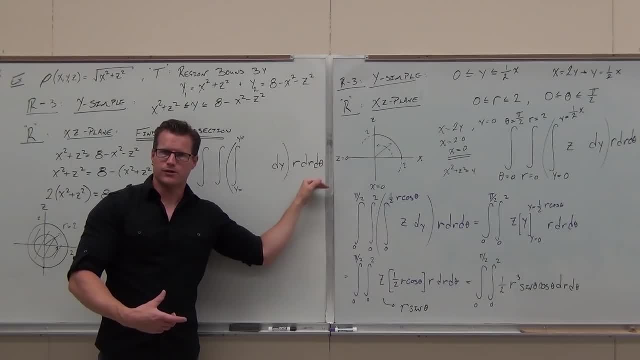 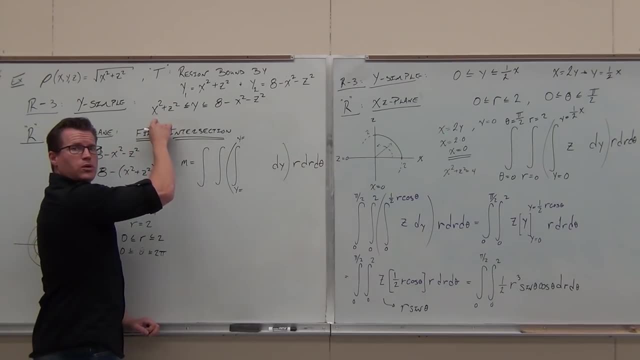 now, in terms of whatever these are, a polar function. So let's, let's, let's change this thing. So, up here, can you change this Into something that's polar? Yes, What would it be? R square, r squared. 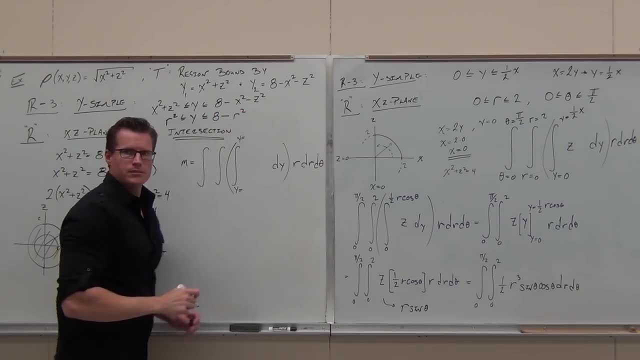 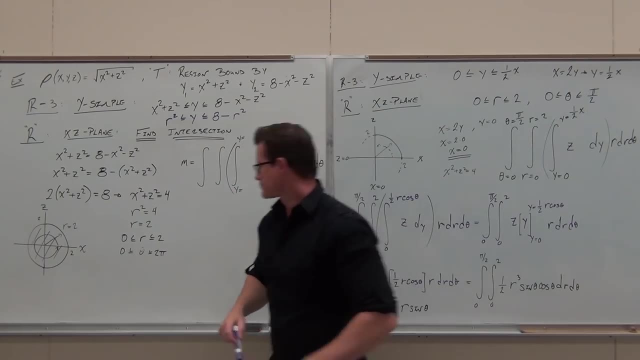 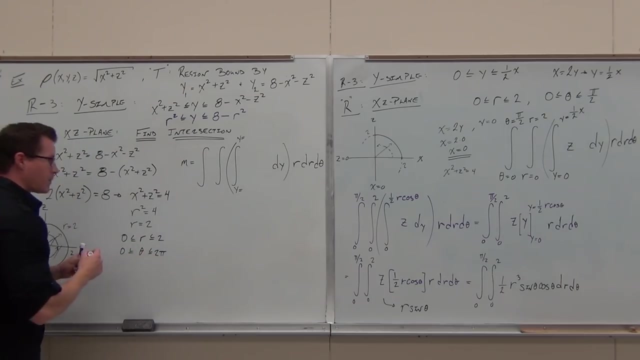 And this guy would be 8 minus r squared. And now, if you're okay with that one, You can also check your work right here. Plug in zero for your radius. That's zero, That's 8.. Good, So I know, because I got an integral. that's right to y sure, I got y equals and r y equals. 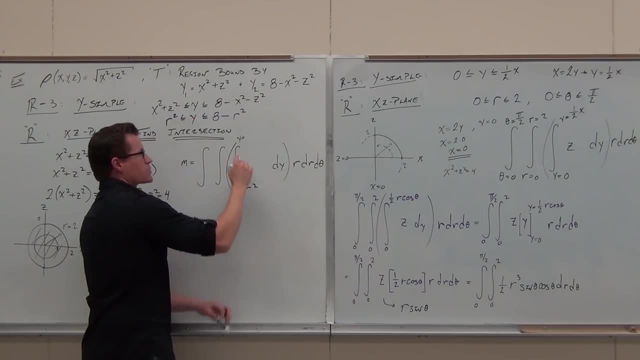 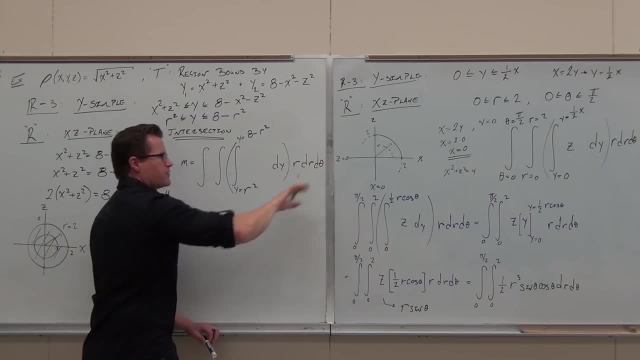 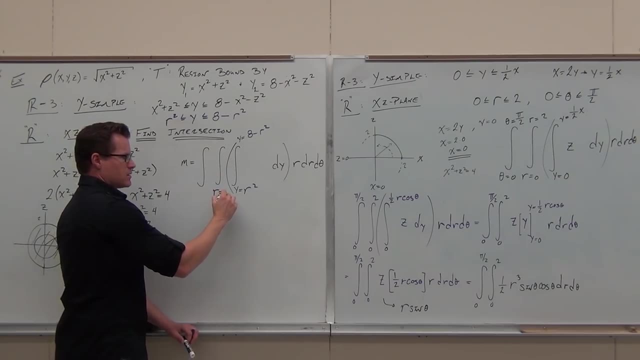 now, so that my integral matches up with the rest of my variables. That's what I want Now. the rest of it: r equals. what's r equal here And here, please? And theta equals. And here We're going to double check: y? y equals r, r equals theta, theta equals. I have an inequality. 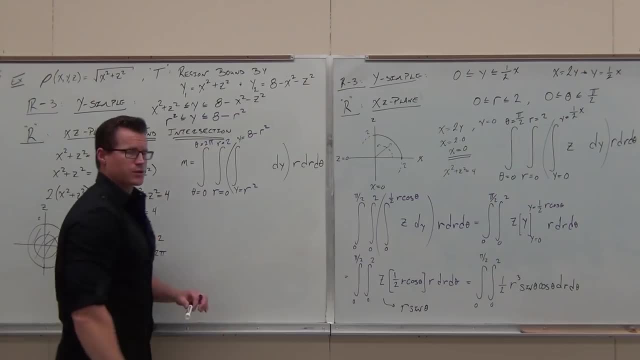 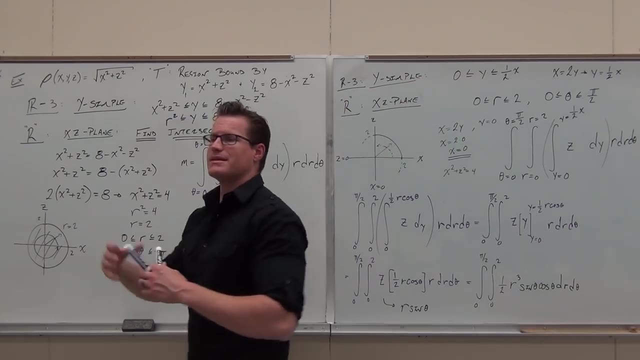 set up small to big, small to big, small to big. It looks great, with one exception. What goes on the inside of that right now, please? Whatever it is, Whatever the mass density function is, So in our case, yeah, thanks for the r. 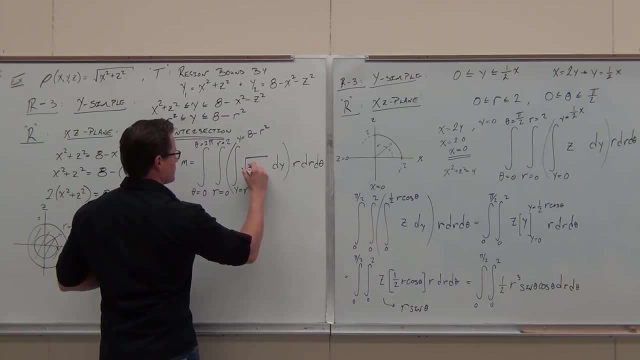 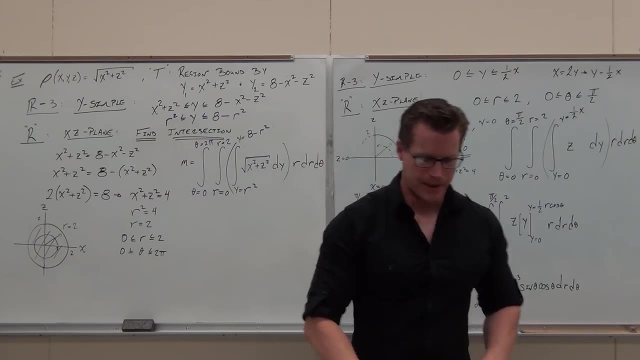 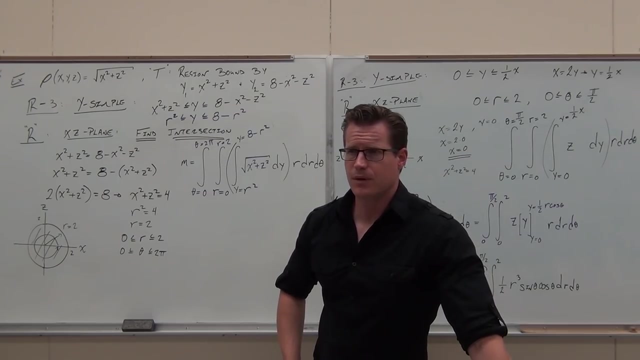 Uh-huh, you're not missing anything. That's got to go there, That's got to go there. I need to know if that makes absolute sense to you, yeah or no? You sure No. I told you before. I just told you that you really should integrate this with respect. 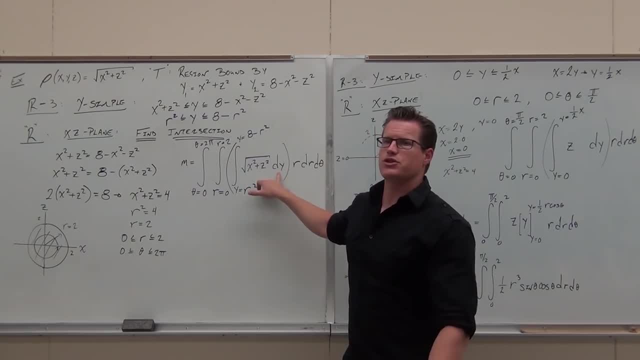 to y without changing stuff first and then plug in y. but I'll show you how to cheat at this a little bit. If this does not have that variable, you can change it whenever you want, Because right now think about this for a second. 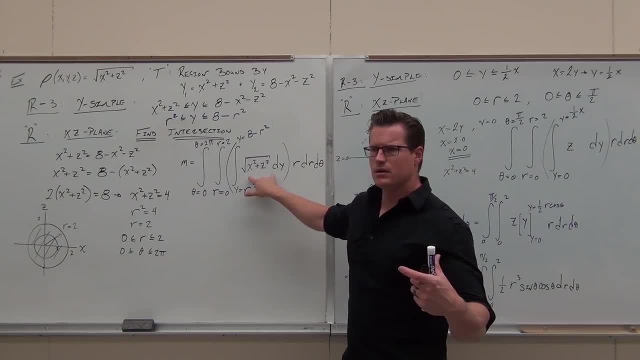 Would this all be a constant with respect to y? That means you could pull it out. You could even pull it this way, like that r, so you could group it. Okay, If this has that variable, if this has d, whatever variable is here is in there. 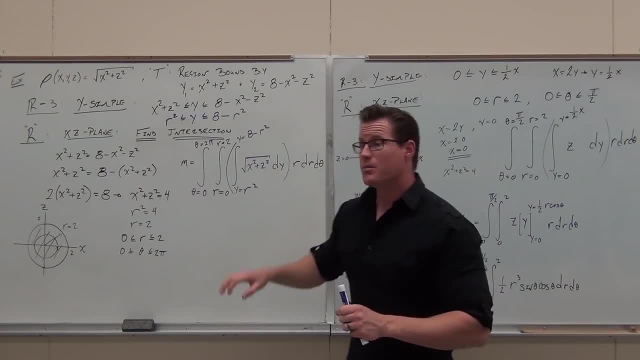 you can't change it, do not change it. avoid changing it at all costs. You can't do that. But if your function does not have this variable in it, you can change it whenever you want. You just have to know what you're doing. 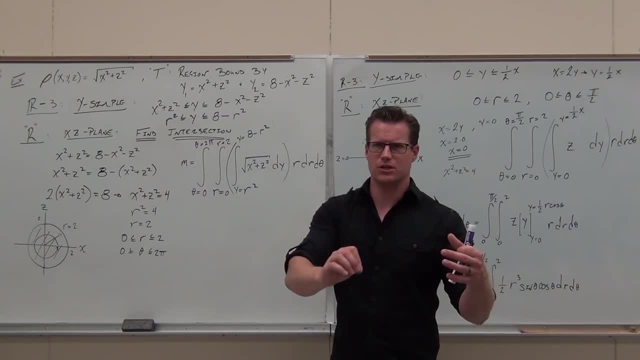 Does that make sense? Do you understand when you can change it and when you can't change it? Yes, If this variable is anywhere in that function you can't, You have to integrate first. If this variable is not in that function, you can change it right now. 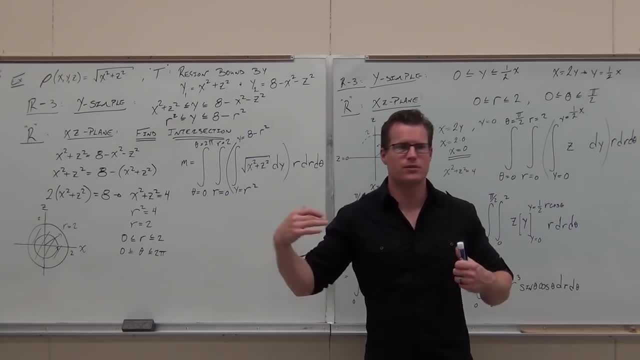 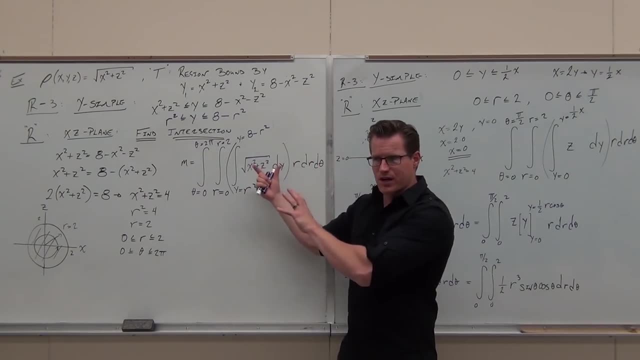 So let's do that, just so I can show you How did how this method works. I've already shown you when, how to you don't have to change it. Now I'm going to show you how you can change it if the variable is not related to your d. 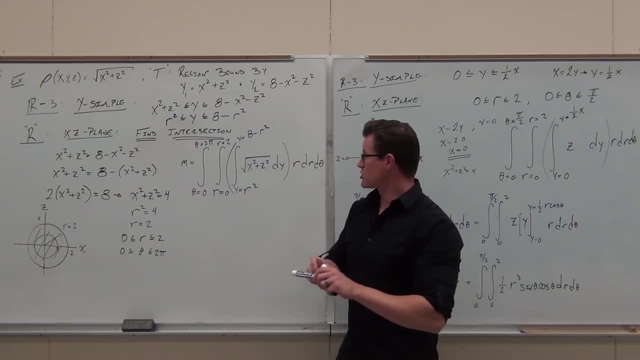 whatever r is, three symbol is: Does that make sense to you? So let's, let's change this here. I love changing stuff. that's square root of x, squared plus, I don't care whatever squared, What's that going to give you? 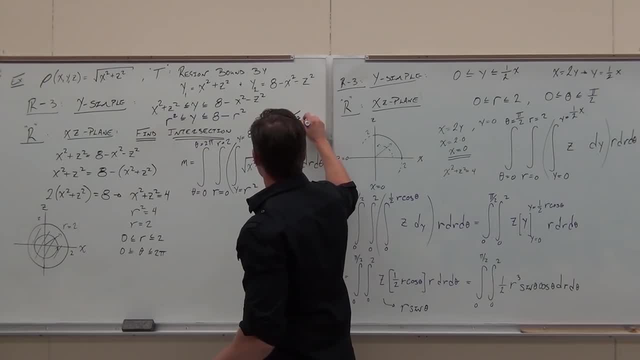 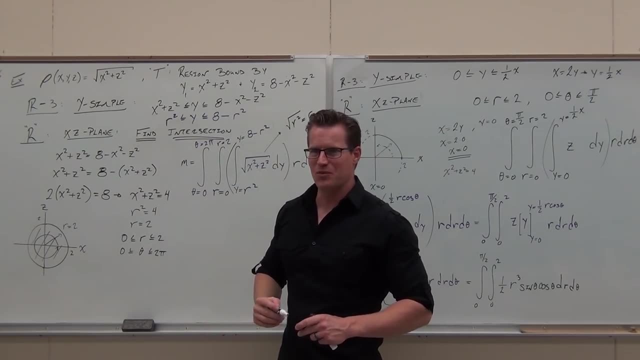 R R, Yeah R R. I watched Pirates of the Caribbean this weekend. so it's my birthday, I get to do what I want. Pirates of the Caribbean: Boom, Rrrr, No, Huh. Saturday. 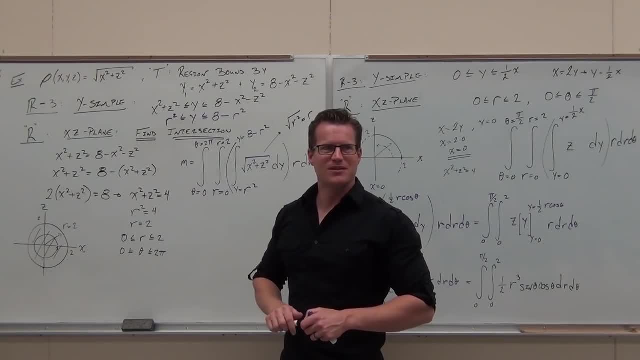 Saturday was my birthday. It was for real- My wife's birthday. I turned like 27,. so, Yeah, In my dreams- I don't know if I'd want it either- Say what Like the 10th time. 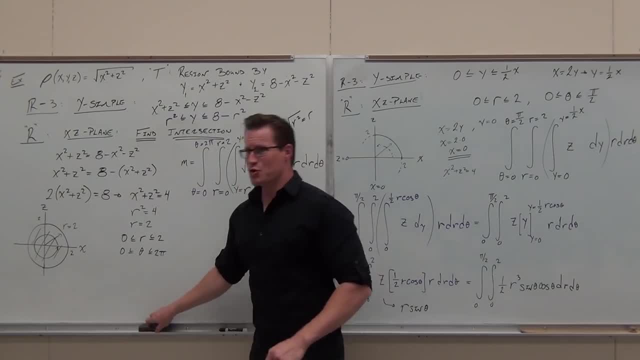 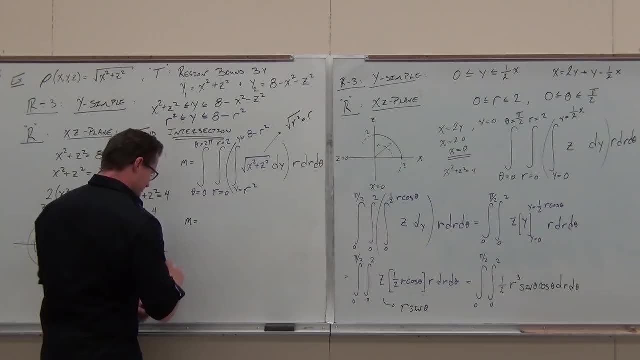 10.. You shall not. Oh, I've used that one already. The question was: am I in my 40s? Yeah, I'm 83. I age really well. Strict diet of quinoa and steroids- That's a lie. 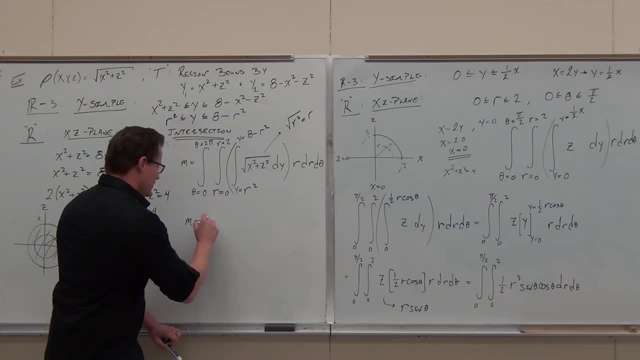 That's a lie, I'm just joking. Don't take steroids. They do weird things. Ask my uncle. He was Mr America. Look him up. Gary Leonard, For real Mr America, Although he, yeah, Yeah. 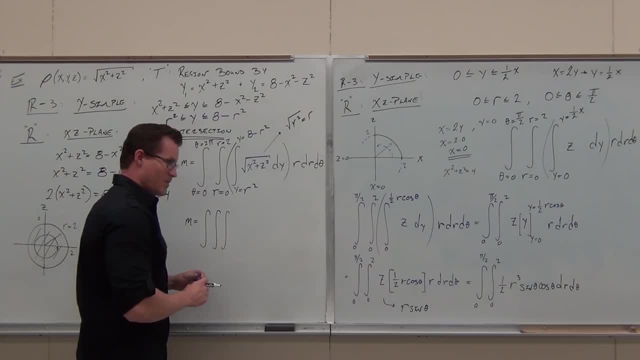 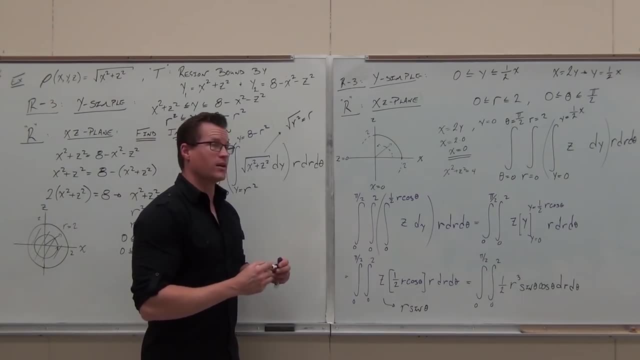 For real, I don't know. Taught me everything I know about not taking steroids. Yeah, No, he's massive, But he was. He's still in great shape. I don't actually think he took steroids, But around the time of the 80s a lot of bodybuilders did. 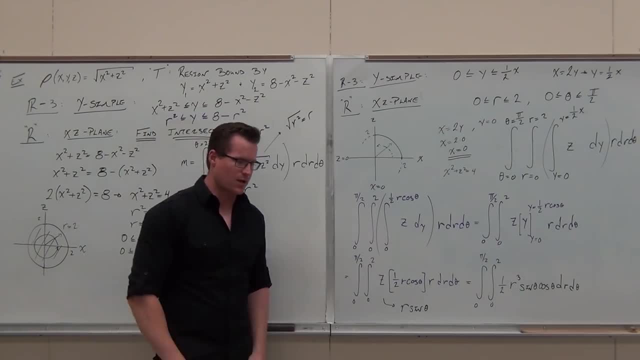 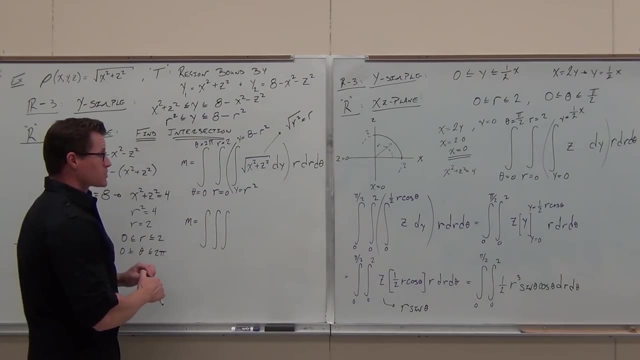 It's what they did. They took steroids to recover, And they'd also take uppers to work out as hard as they could. Not good man, Not good. So let's do our triple integral, the complete setup. You can change this if this variable's not in there. 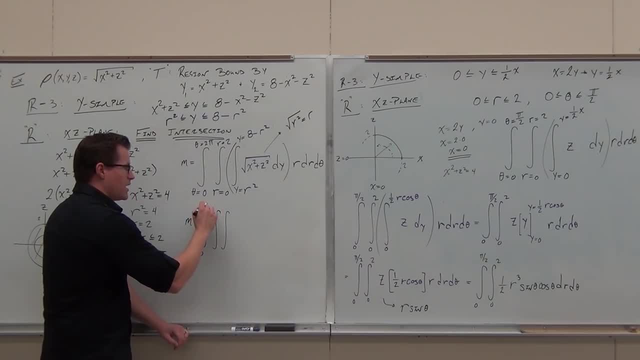 So we're sorry, we're back on track. It's sidetracked. Zero to two pi. I don't ever do that, do I? Zero to two? This, this don't change. This is still r squared to eight minus r squared. 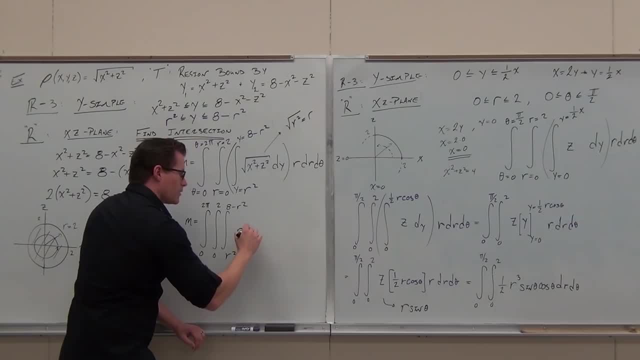 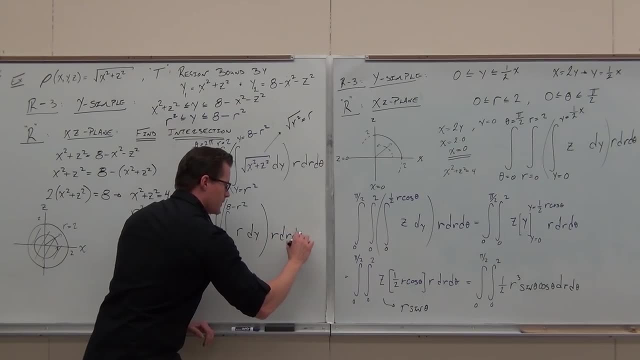 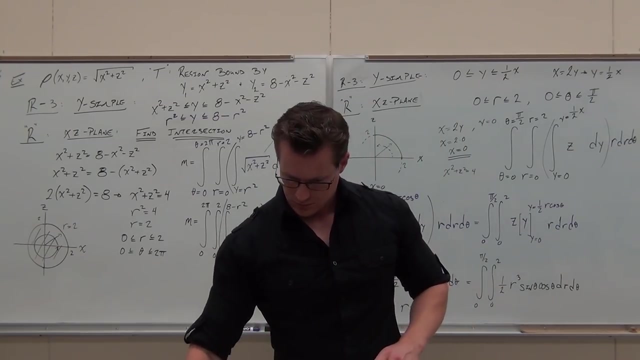 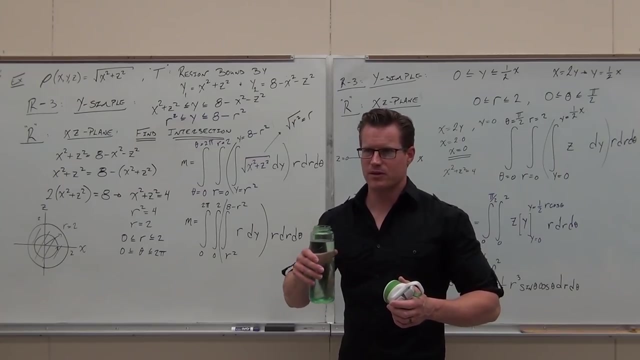 But this you can change. This is now r dy. We'll do that first. Then we won't forget our r? dr d theta. This is your chance to practice. I want you to do that integral. Go for it. You know, I was joking about the steroids thing, right? 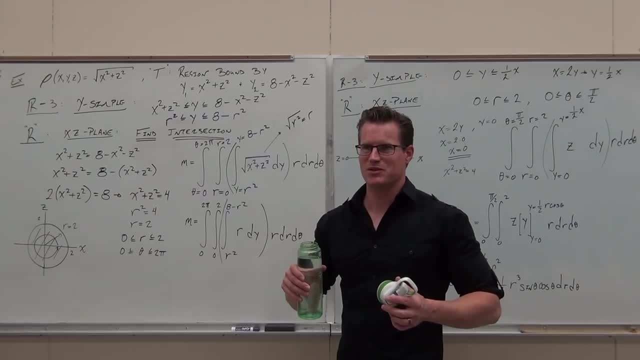 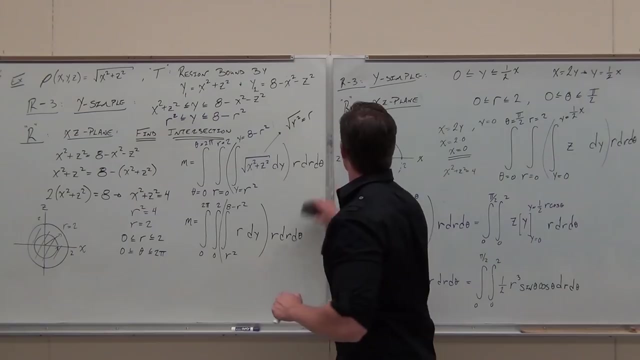 Okay, That's, that was a joke. Maybe it was a joke in poor taste, But it was a joke. Goodness, Not a little bit. Okay, No, Thanks. Okay, Go görüşür 25, compete for top 30.. 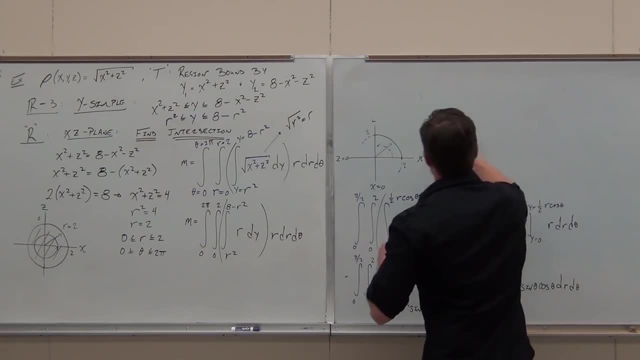 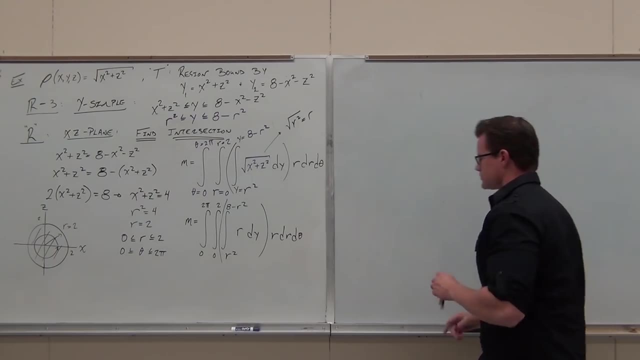 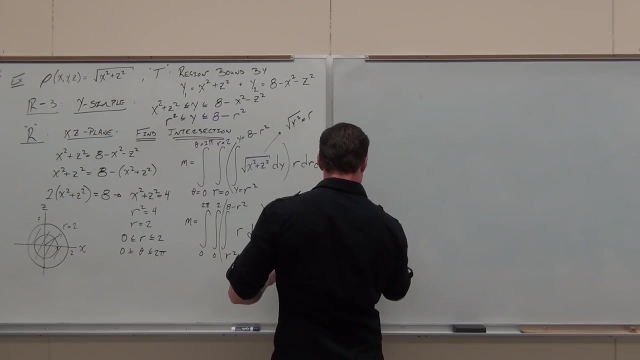 We won't Understand this2018 National Sports Championship, but we and the people behind us and the choices of the women in the position and the basketball team of Ford and we will go. We're both good. It's okay, Thank you. 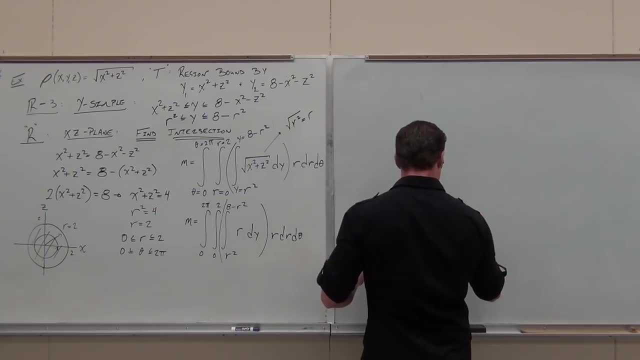 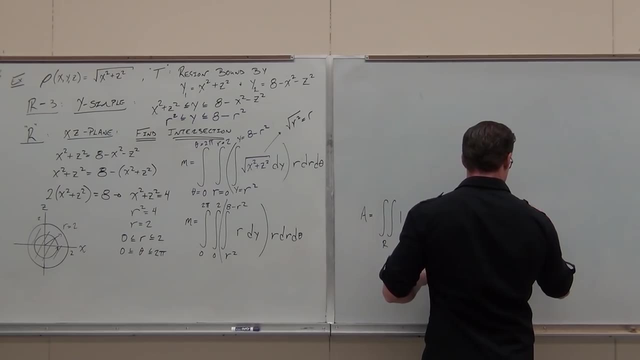 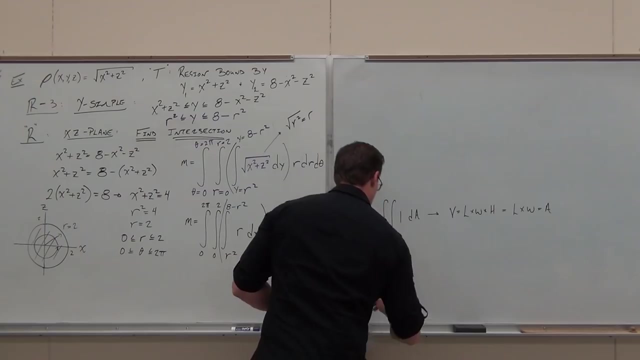 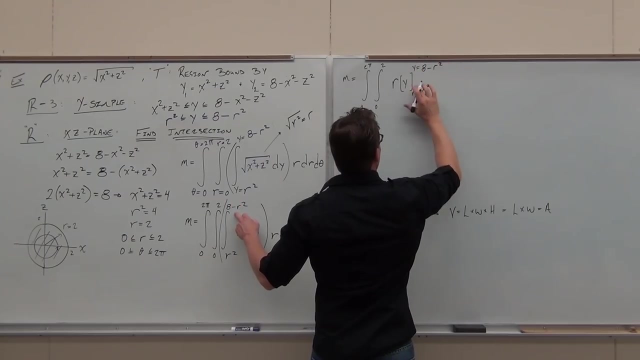 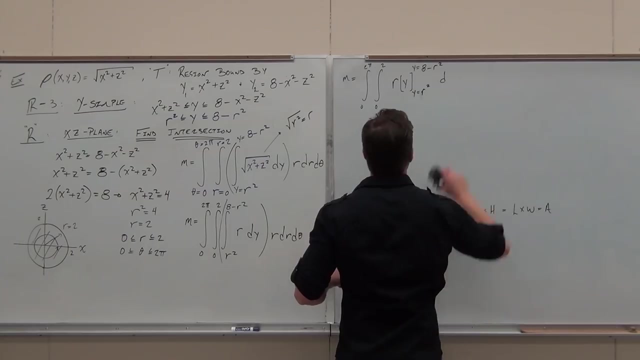 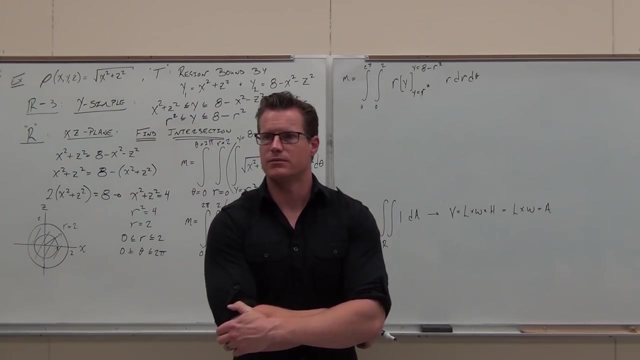 Bye for now, Bye, Bye. Come on, Don't do that, Don't do that. Thank you, Thank you. How did you make it that far? Did you integrate with respect to y and get at least a y up there? 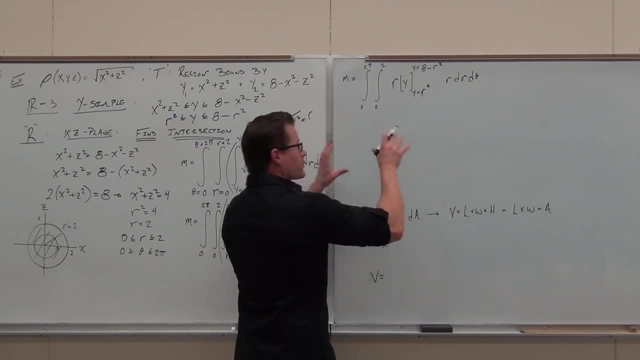 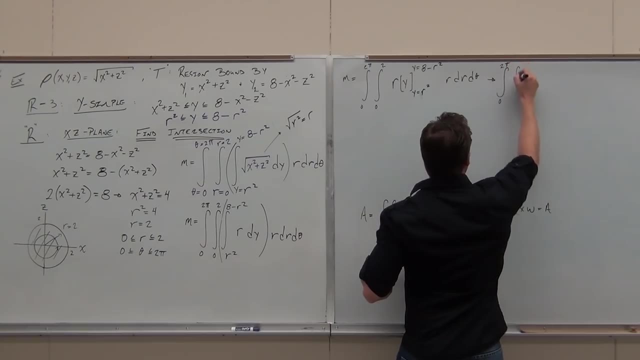 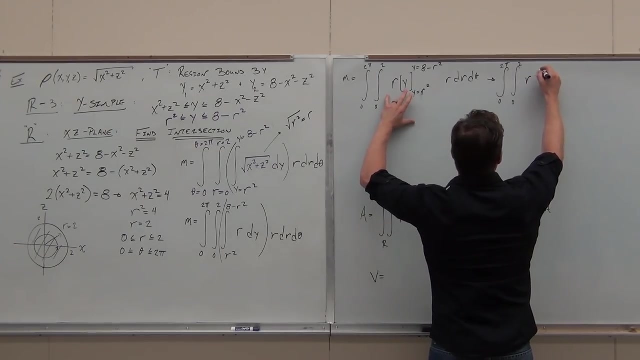 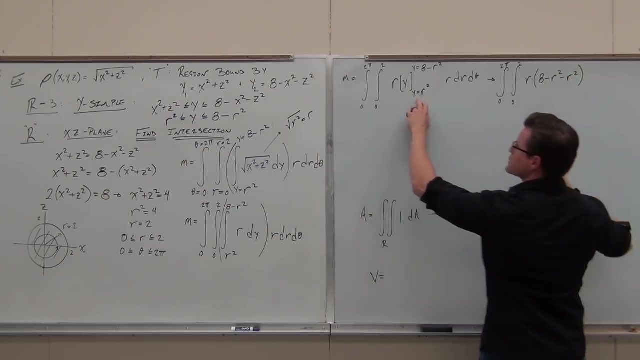 Plug in for the y. Okay, we can do that. Just don't forget your rd, rd, theta. That's important, Thank you. So here we have our Thank you. You can see it too. You can see the outside function minus the inside function. 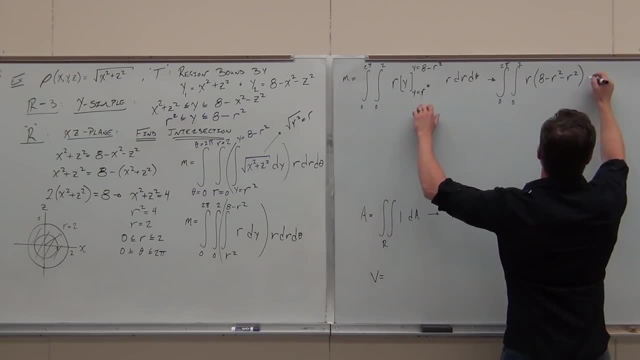 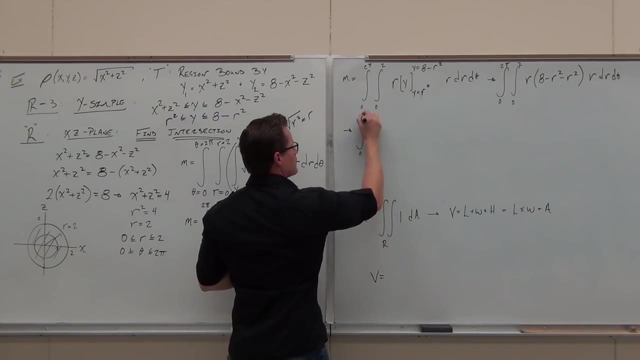 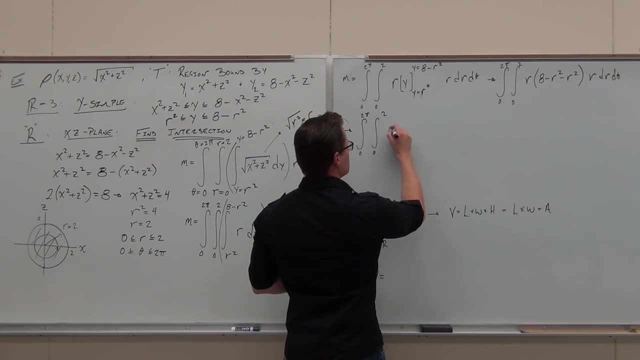 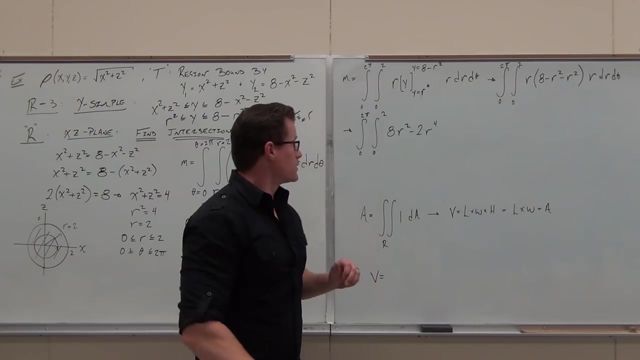 That's taking the subtraction of the volumes there. Maybe simplify a little bit before we continue. Looks like we have 8r squared, 4u, 2r to the 4th. I believe I did it right. Double check me though. 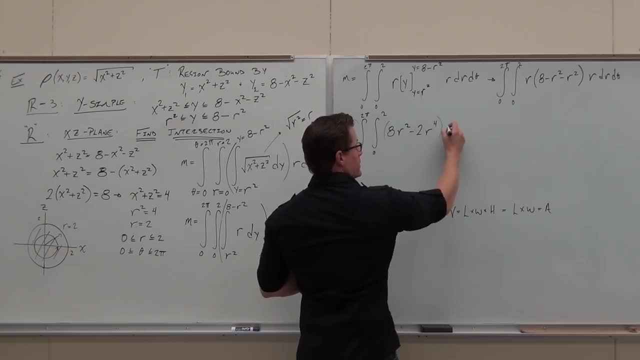 Did you guys get the same thing? Yeah, Now we still haven't even integrated with respect to r yet, but we have cleared out that r, That's r squared 8r squared minus 2r to the 4th. 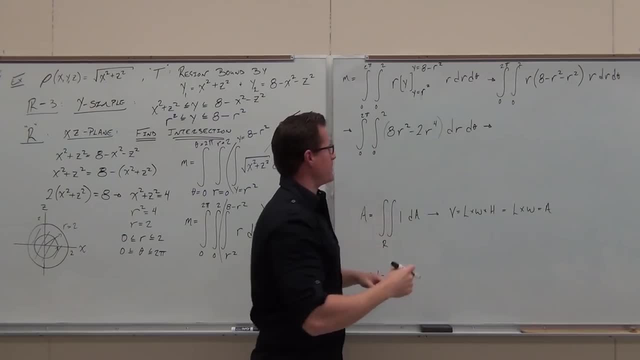 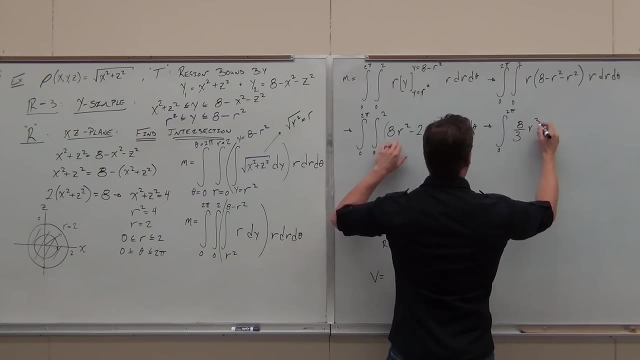 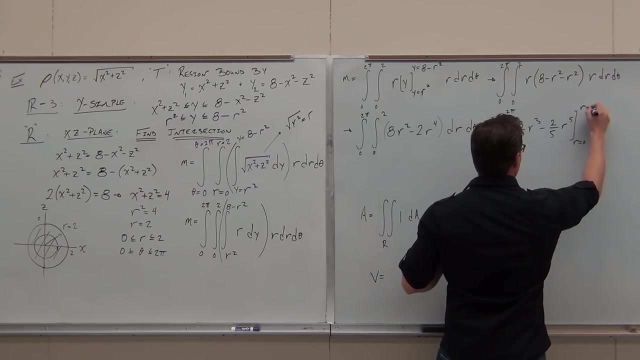 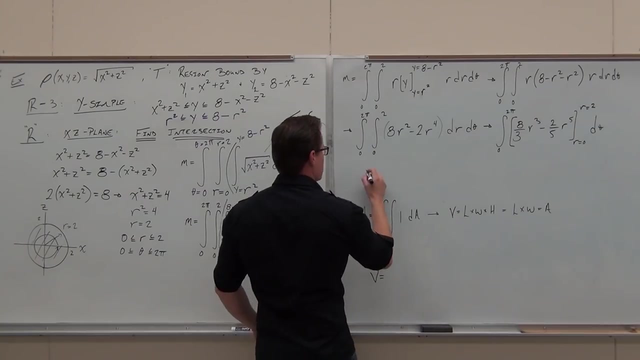 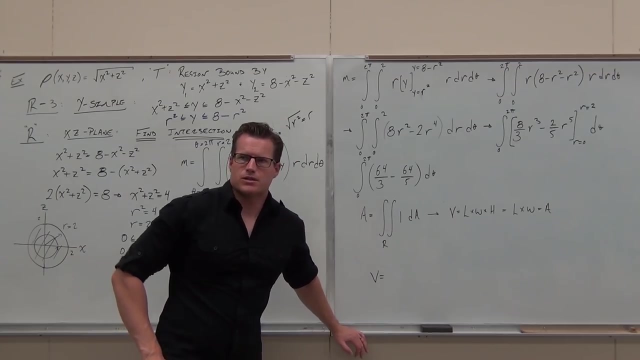 And then we do the dr d theta And it's pretty basic from here. Let's see: Plug in 2. Looks like 64 3rds minus 64 5ths. d theta, Blake, our, Our Listen. you're always welcome to combine like terms before you integrate. 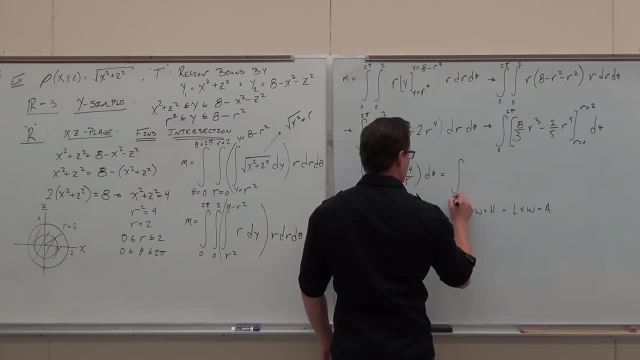 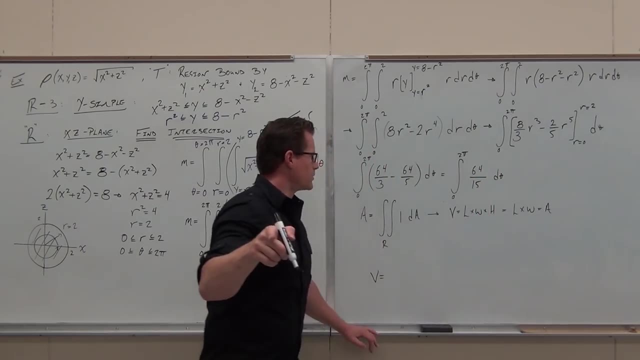 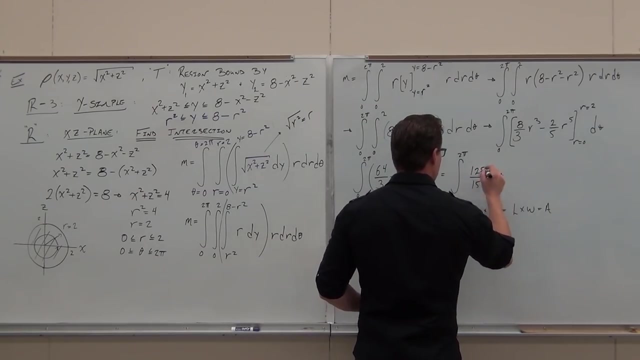 That's a really good idea, I think. Double check my work though: 64 15ths No 128.. 128.. Sorry It's a fraction, but I'm a calculator man. Best thing ever So cool. 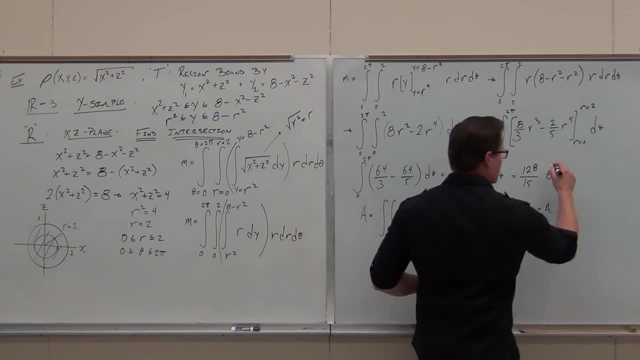 If we integrate a constant with respect to theta, we get theta. We plug this in: Theta equals 0 to 2 pi. Looks like we get 256 pi over 15.. I think that's pretty much it. Were you able to get it. 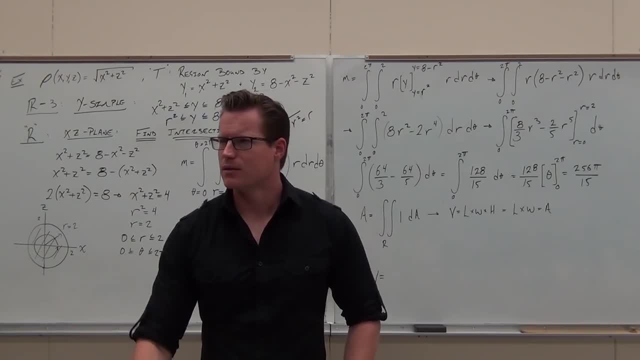 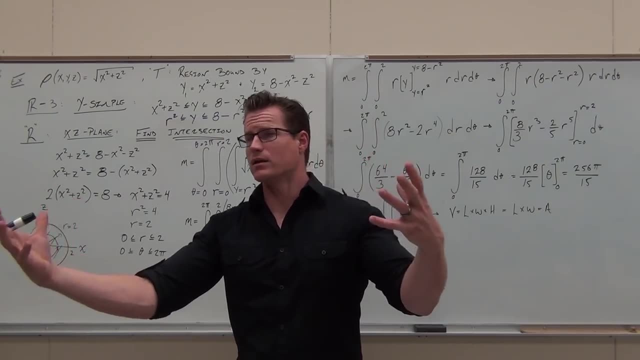 No, Now, what is it? What's that represent? Mass, Mass, Mass of what? Mass of what? Come on, Come on, Help me out. Mass of what? Mass of the thing, What thing? The mass of the region defined by. 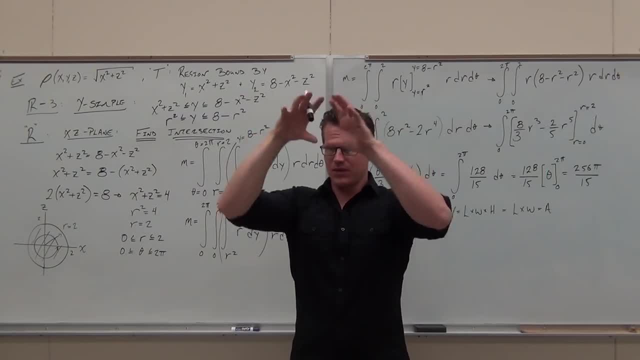 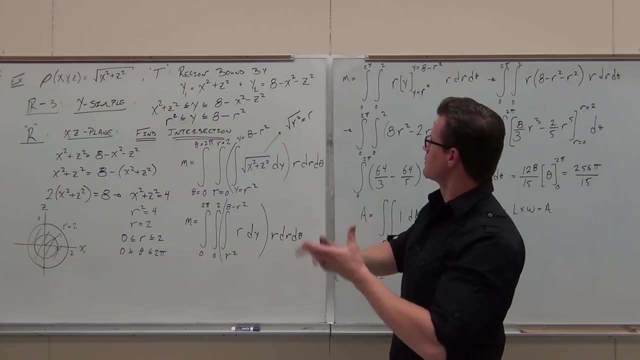 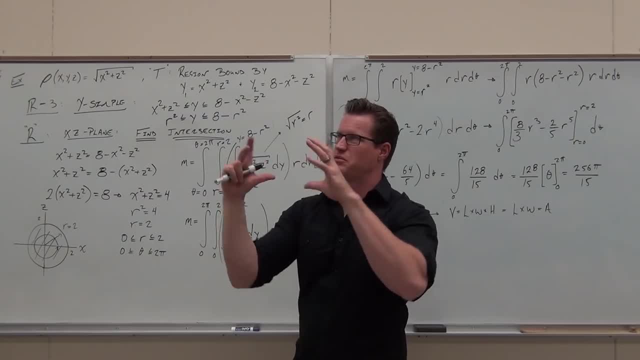 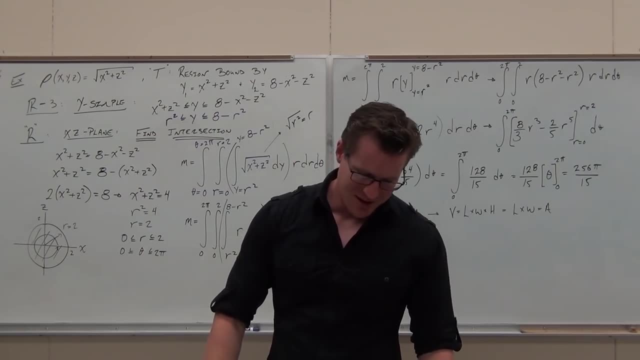 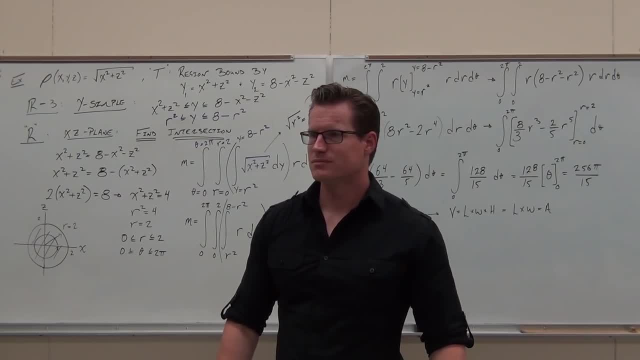 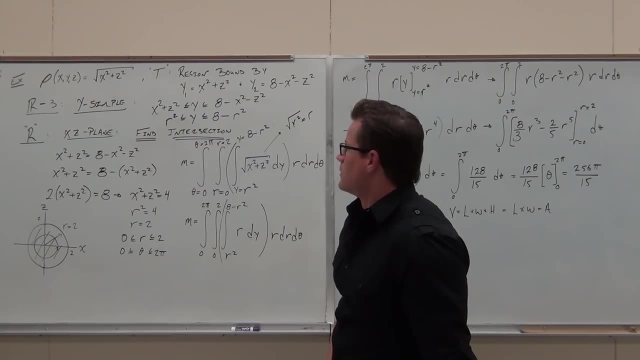 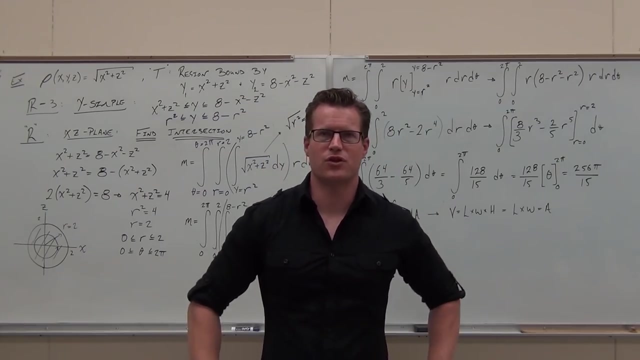 You sure, You sure you're sure? Or is that just an ice cream cone? Kind of like an ice cream cone? Yeah, Yeah, that's all. I just have to draw it to really see. But that's the idea, That's what we're doing. 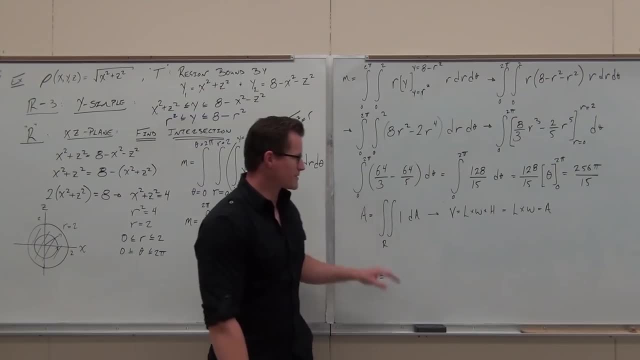 Now I want you to recall something here for a second. Do you remember how we had this little sidetrack? We said: wait a minute. What if you don't have a function in there? What if you have just one? And you double integral over r with respect to the area. 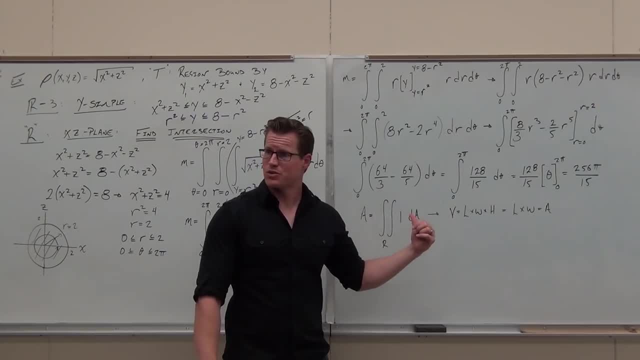 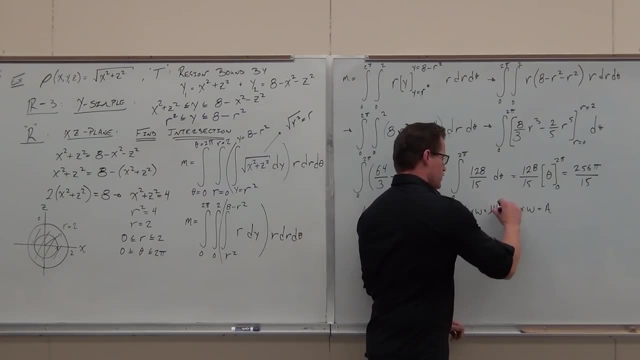 times one basically just gives you the area of the region. Do you remember doing that? Well, the reason was it was volume. is the basic idea: Length times width times height? What if your height was one? Well then, you just get length times width. 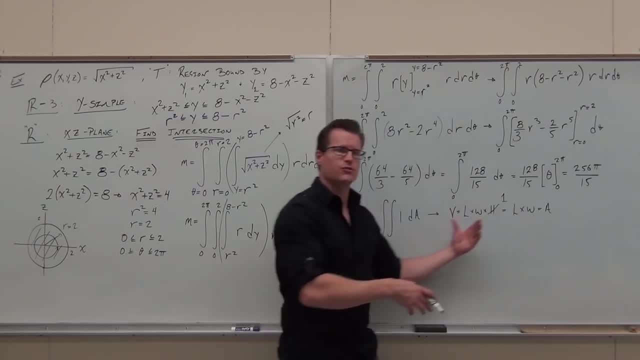 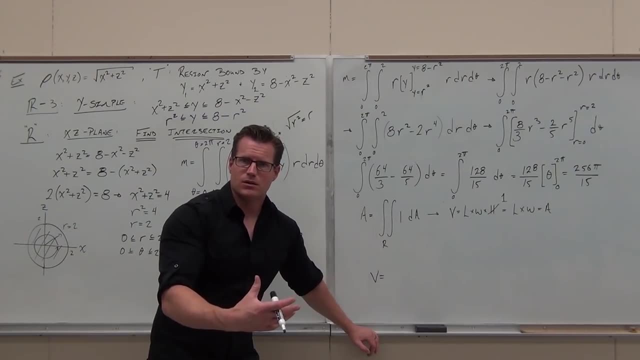 But that's exactly what area is, And that's a really basic explanation for how this works. I proved it a while back, We talked about it a while back. Well, now let's go further. Can we do the same idea with volume? 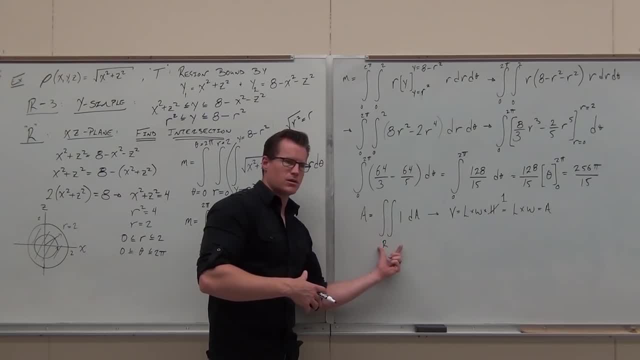 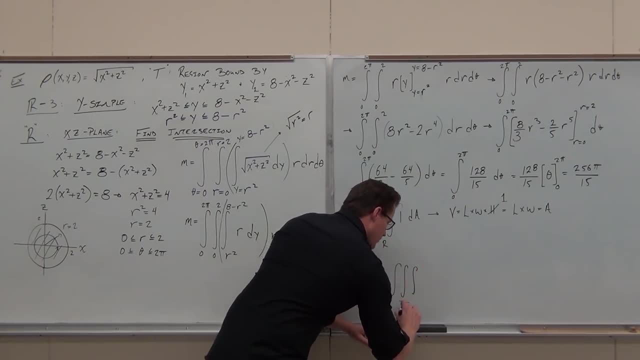 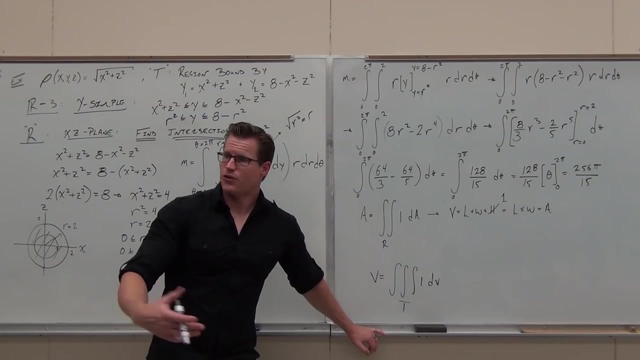 If a double integral over a region of one gives us area, then a triple integral over a three-dimensional region with a height of one, with respect to volume, is going to also give us volume. This is a different way to find volume, which is a really interesting thought. 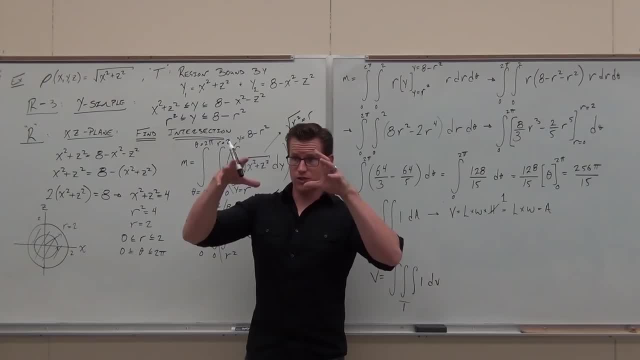 because we already had double integrals right. Double integrals over surfaces give us volume under the surface. Well, if we can define that region in three space and we just do a triple integral over the region, we also get the same volume. 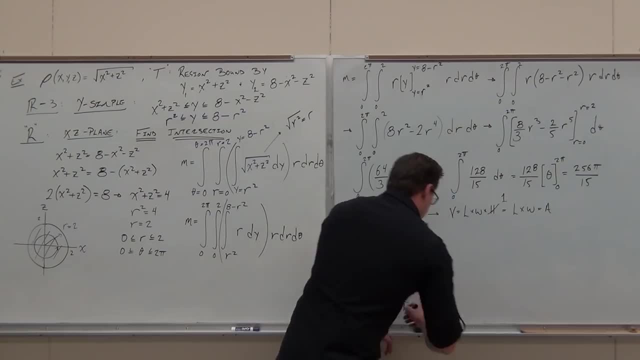 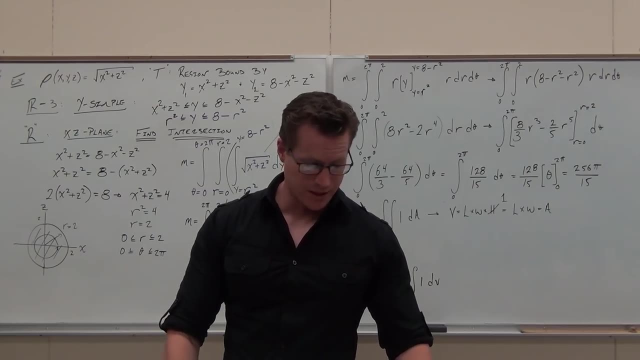 It's just a different way to find volume, a really interesting way, So we can do that as well. Let's try just two of these. We're going to focus. We're really really on the setup on these guys. We'll do that. 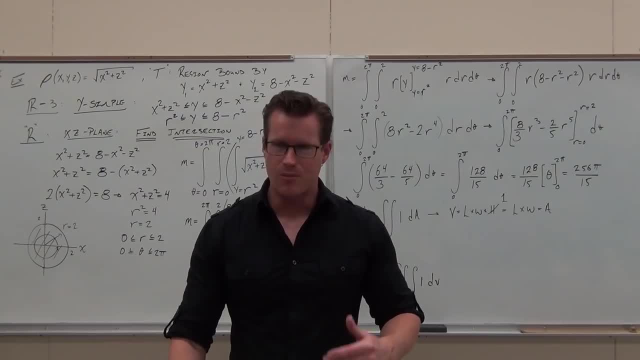 We'll come back. We'll talk about center of mass. We talked about a little bit of that in 14.4.. Talk about center of mass, and that should pretty much wrap this section up. Tell you what. Let's take a break now. 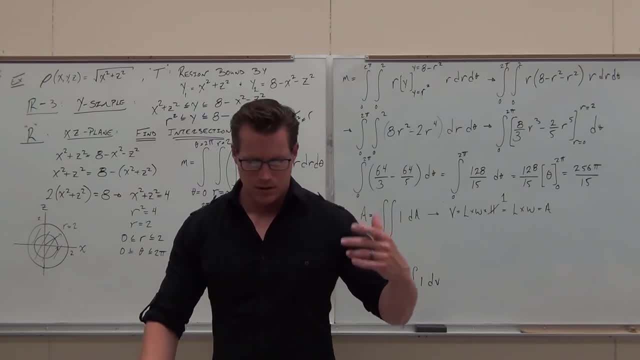 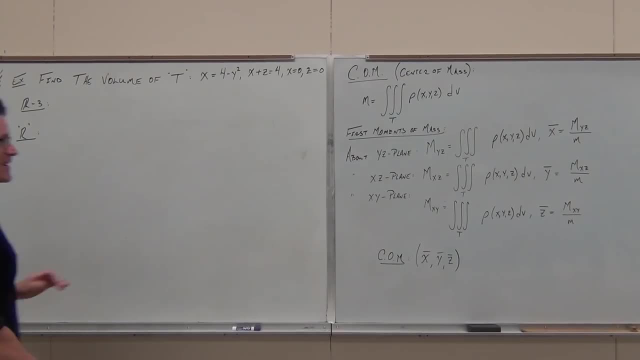 We'll come back and talk about how we apply this to some of our regions. Good math, So this is a little bit later. Right now we've got to practice that last concept. I put on the board over here saying, hey, you know what? 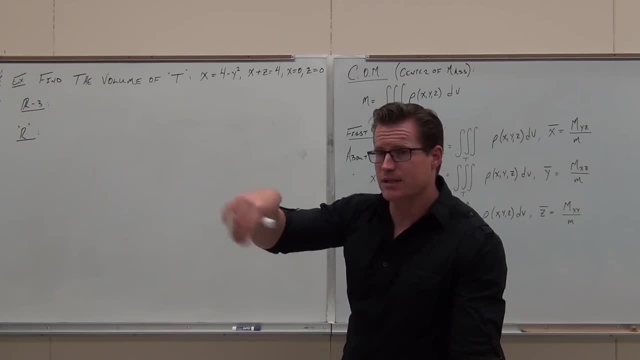 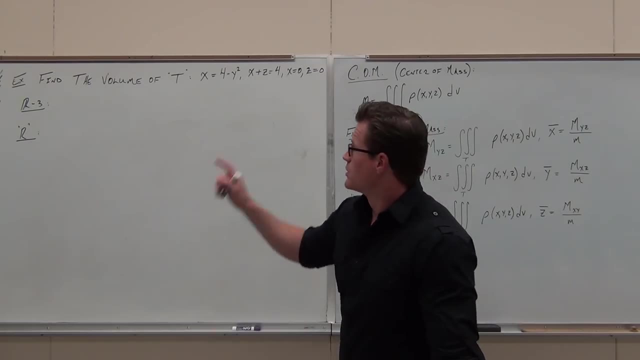 Just like we can find area of a region with a double integral, we can find volume of a 3D region with a triple integral. just kind of little mathematical manipulation that we do. So we're going to find the volume of this region, right. 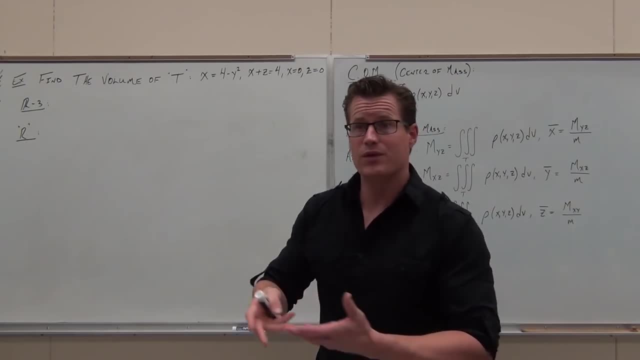 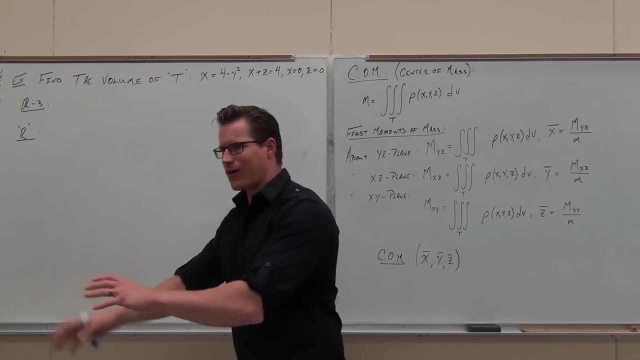 there. This is not a region between two functions, So this is a little bit nicer. You don't have to find intersections, All we have to do is determine R3 simple, then the R on whatever plane we have, and set up a triple integral. 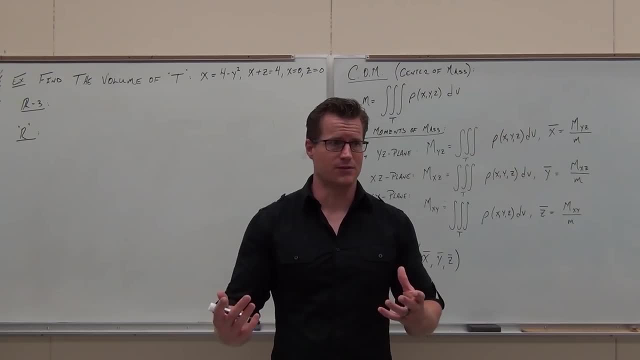 It's, in fact, even easier than that, because I don't have a mass density function. I'm not asking about the mass. We're switching gears, We're asking about the volume right now. So, number one thing, let's check it out. 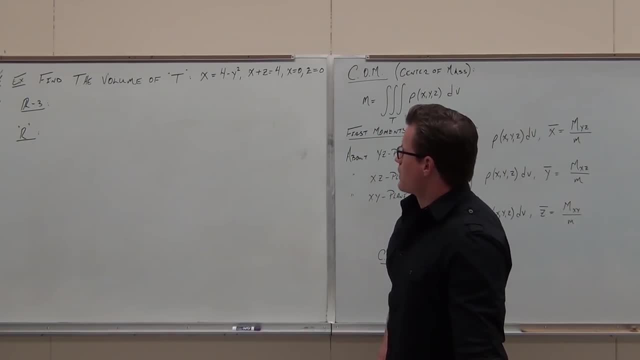 We do R3 simple. What would you choose as R3 simple? There's actually two choices here. What would you choose? X, You could choose X. Why. Why could you choose X and be OK? You already know And I like the zero. 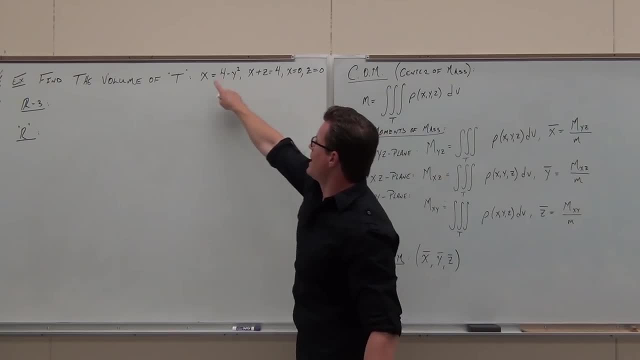 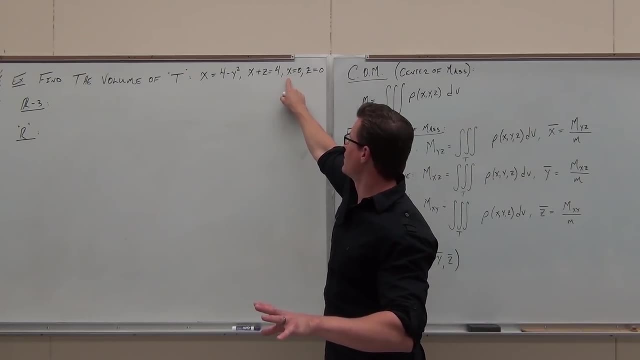 I like that X gets a little bit funky because I have X and X and X. Does that make sense? That's a little hard to deal with. Might not be the best choice. How about Y? simple No, because there's only one Y: That. 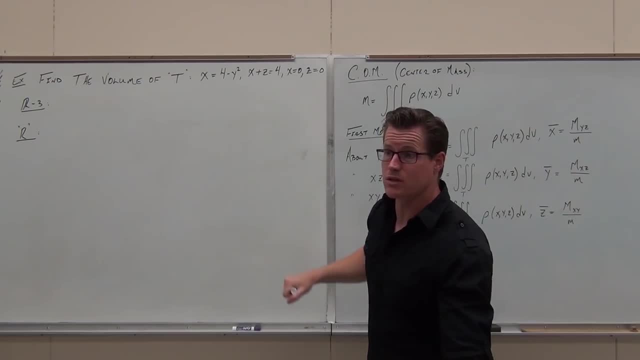 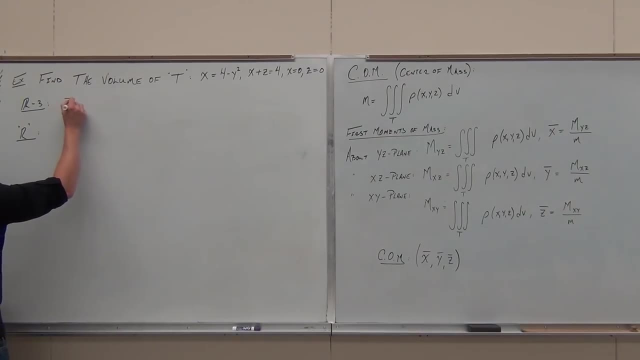 would not be a good choice. You'd have to break that up into two different functions to do it. I don't want to do that. So what's the correct choice? Z, simple, Z, simple, So definitely Z. simple Keeps our region nice. 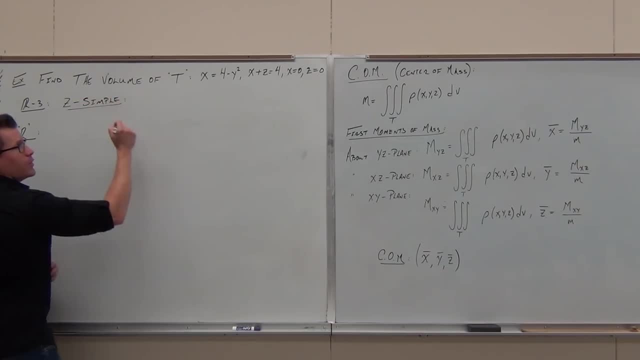 No ambiguities here. Z simple is the way to go, which means I'm going to have to match Z between two functions of Z equals. I already know the small one. What's the small one? Zero. What's the large one? 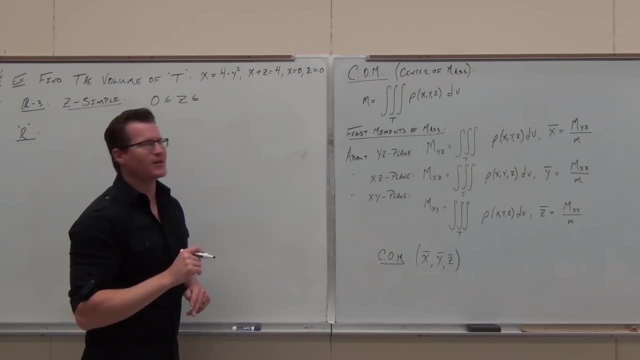 The other one, The other one? Yes, very good, What other one? That one? Well, there's only two functions that have Z's in it. That's what makes it nice: You limit your choices. So from here I know that Z equals 4 minus X. 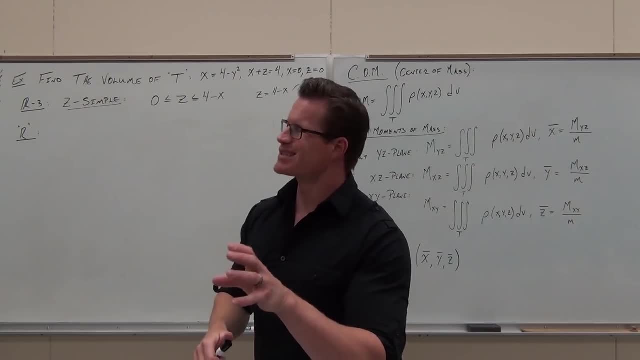 That's going to be the upper function Again. if you didn't know that, if you couldn't see it, zero is nice because it kind of makes the choice for you. If you didn't know that, what would you be doing right now? 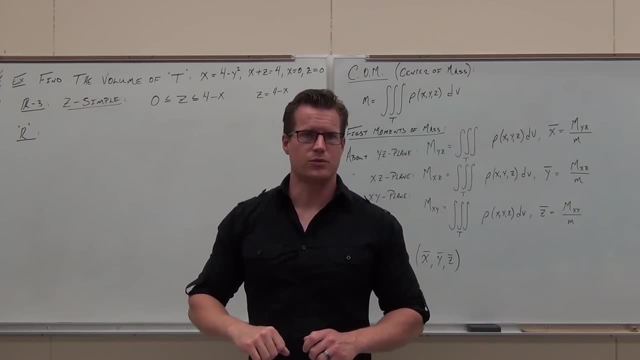 Before you set this up, what would you do? Draw the region. You've got to draw the region Now, right now. speaking of the region, if we chose Z simple, the region everybody's going to be on what coordinate plane? 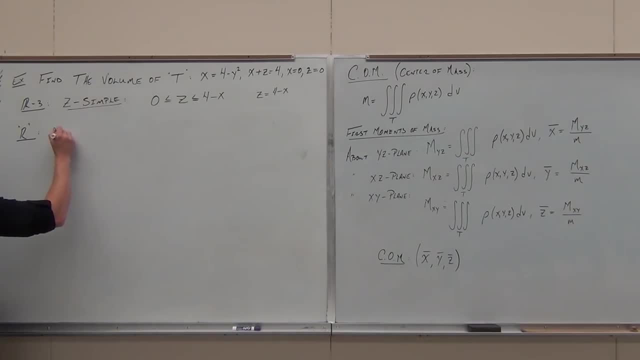 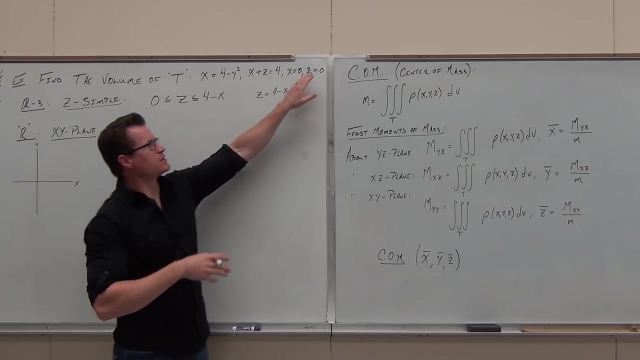 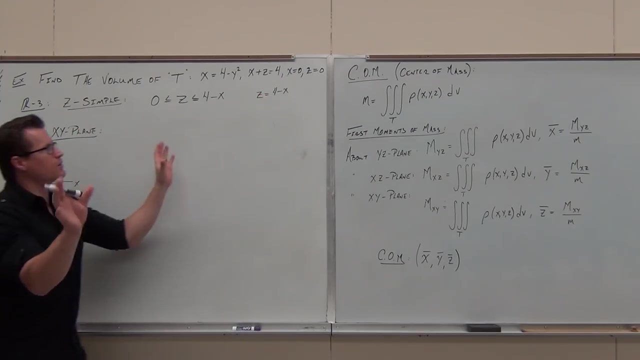 X-O-L Always draw it. So we use everything to put this on the X-O-L. The X-Y plane- Z equals zero- means we're on the X-Y plane- X equals zero. That's the Y axis. We label all of this stuff. 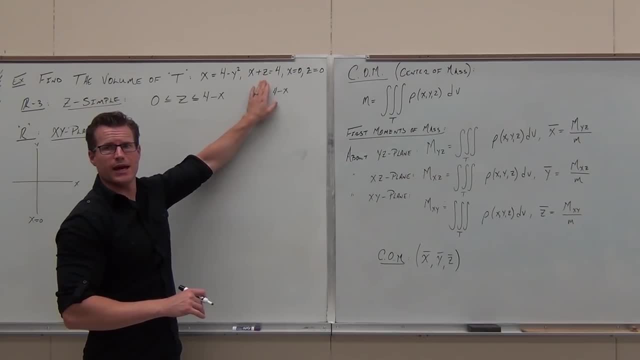 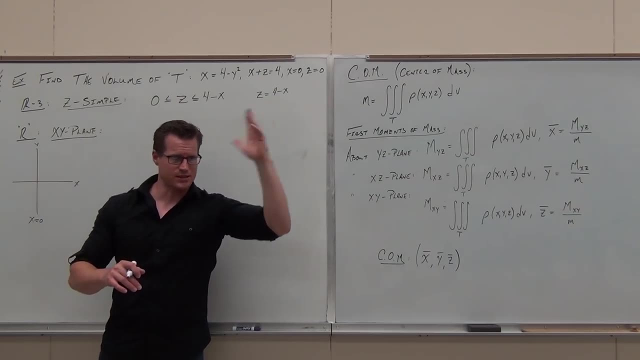 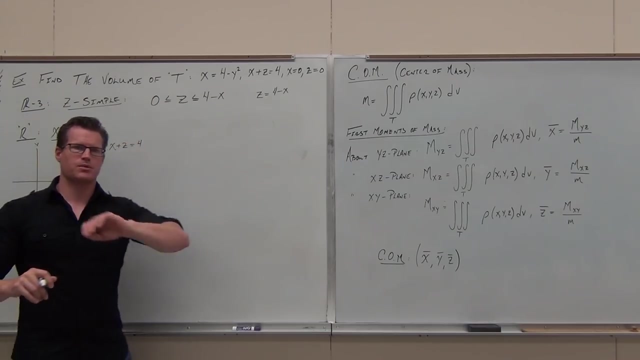 Hey, how about this one? Is this going to be relevant for the X-Y plane? Everything with X's and Y's in it is relevant. Even if it gives us just constants, it's relevant. So if I have X plus Z equals 4 and I'm on the X-Y plane, what's the value of Z on the? 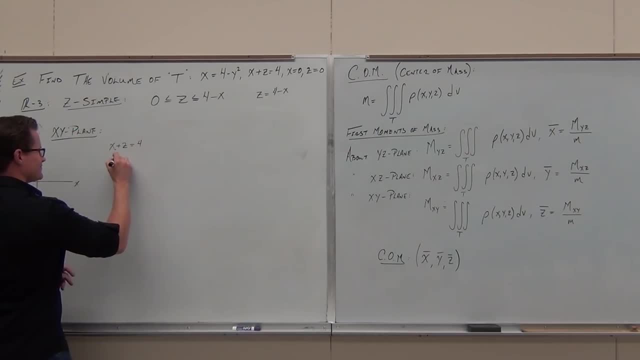 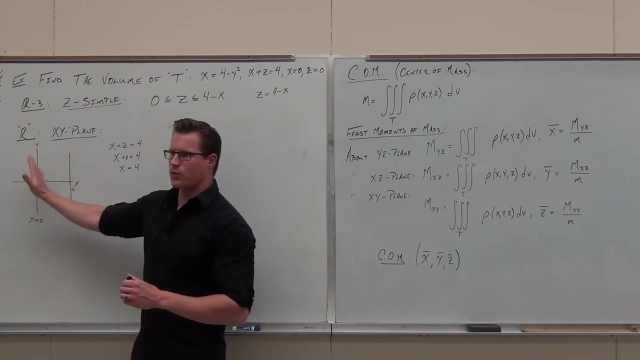 X-Y plane. Zero On the X-Y plane. This gives us another line. So I know right now, right now, that I can't go any further than between zero and four along the X axis. That's important. I know I can't go outside that. 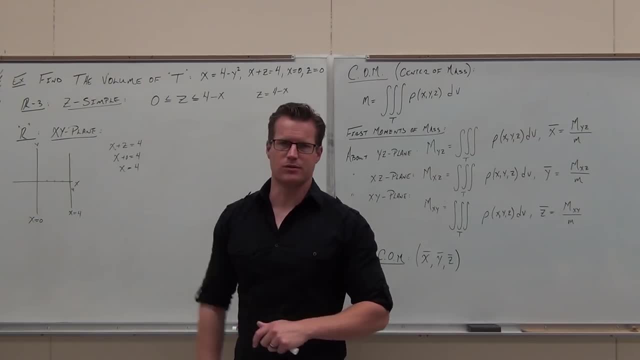 So probably, if I do D-X last, I'm going to be on the X-Y plane, Almost guaranteed. But we're going to draw the rest of it. There's one more to draw. Oh hey, that's kind of nice. 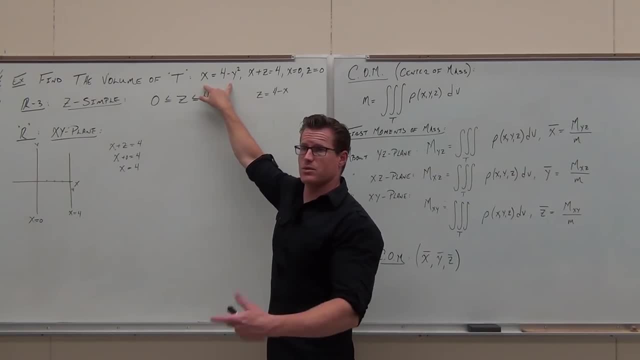 This is why we chose Z simple. The other reason: Because that's a really nice simple shape on the X-Y plane. That's a cylinder along the Z axis. It has a nice shape on the X-Y plane. What is that shape? 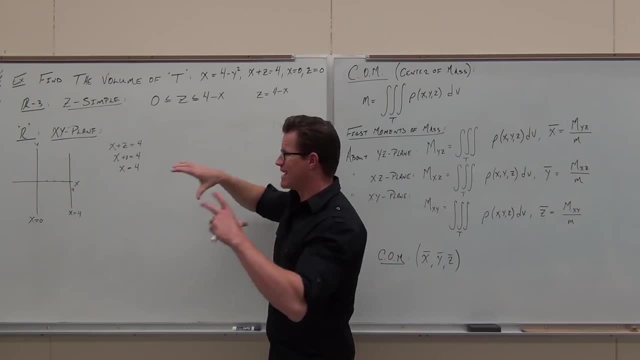 Parabola: Yeah, It's a parabola shifted- Oh dear. Two. Do you know how to draw that? Yeah, That's a type two parabola shifted- Oh dear. Do you know how to draw that? 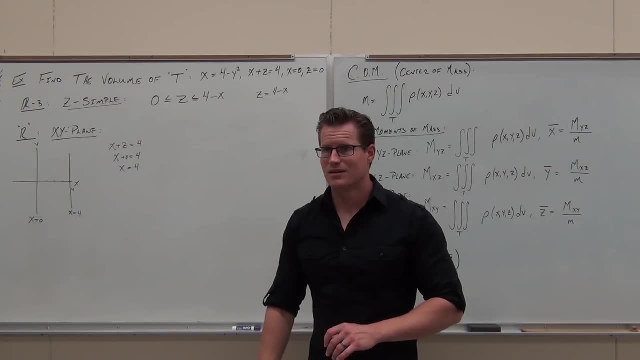 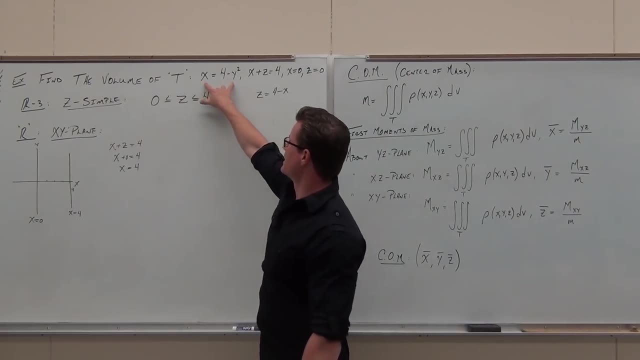 Yeah, That's a type two parabola shifted. Oh dear, Do you know how to draw that? Yeah, That's a type two parabola shifted. Oh dear, Do you know how to draw that? Yeah, That's a type two parabola. 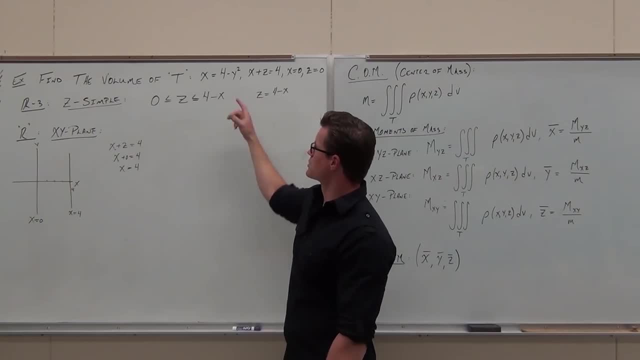 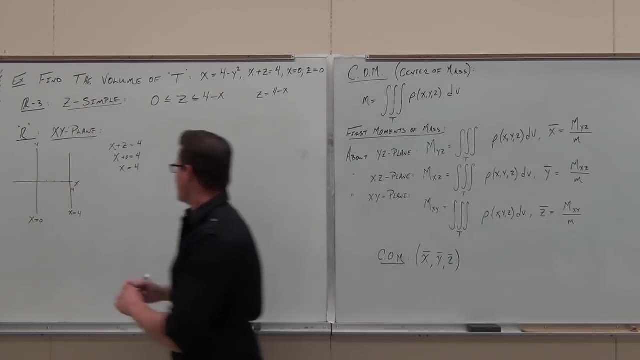 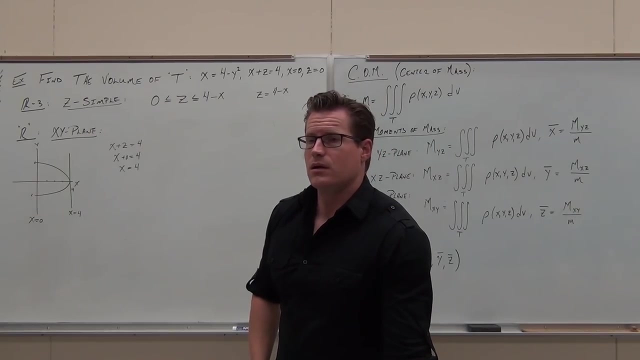 It's depending on Y, So it's a parabola that's opening towards the negative X axis, shifted positive four along the X axis. That parabola looks like this: You guys, okay with that one, Are you sure? Now You might want to know where that intersects the Y axis. 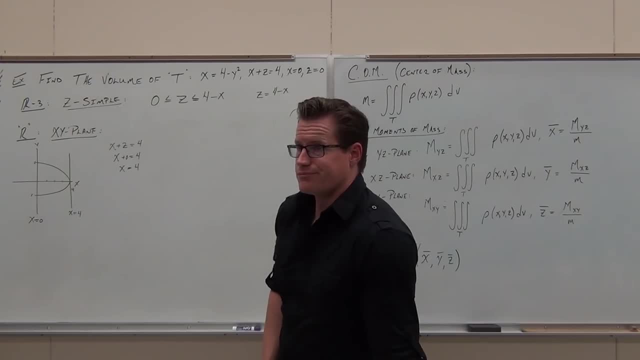 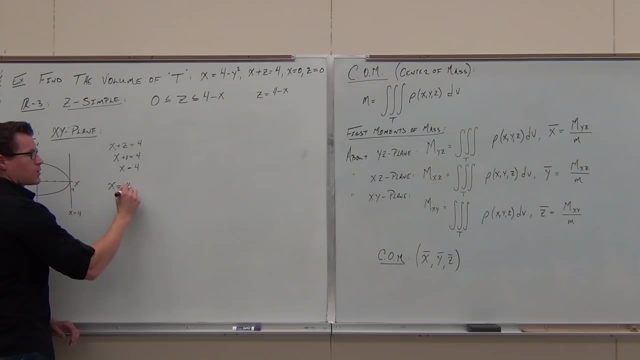 How would you figure that out? Yeah, If you know the X is zero and you know that these things are going to intersect. so X equals four minus Y squared. you go. well, where does that intersect? the X equals zero. Zero equals four minus Y squared. 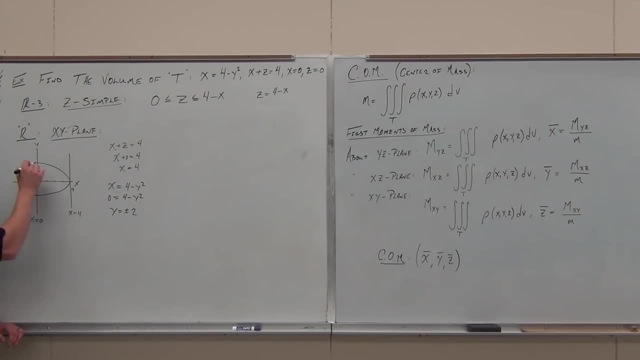 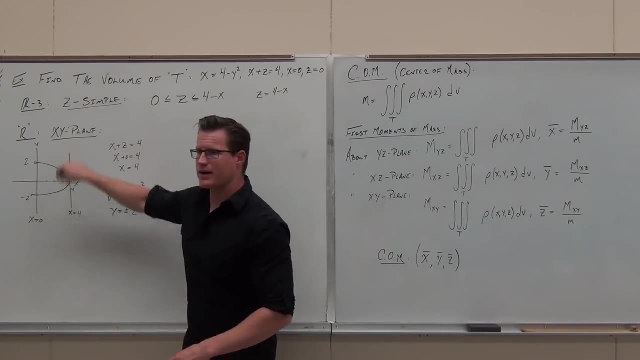 Y would equal plus or minus two. So down here negative two, up here positive two Should have answered with: okay, with that one. That's our region. Now, did this play a big part in defining our region? Well, no. 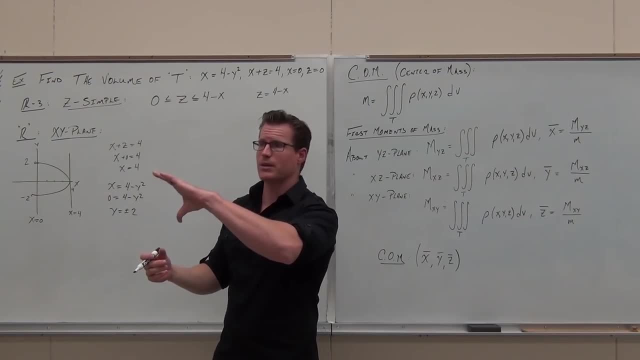 Not really, But you put it on the graph because it might. If this had been an upward opening parabola, it certainly would have. Does that make sense? Put everything on there and then you look at the region that's bound by whatever functions. 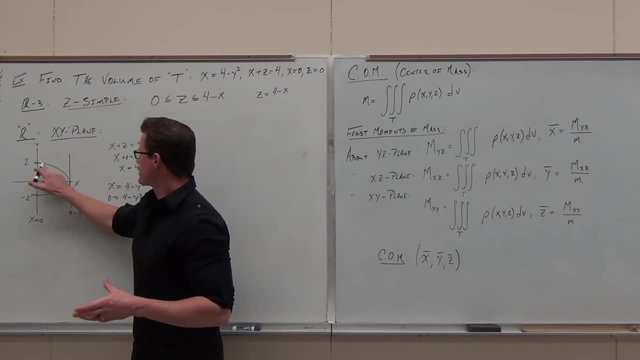 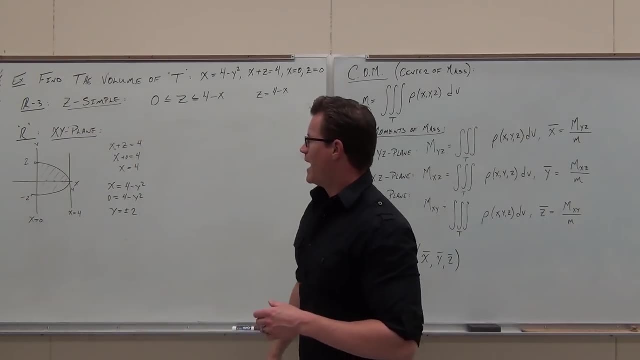 you just put on your coordinate plane. Right now, this is our region, right there. Now here's my next question: What point would you plug in to determine whether this is right? Would you plug in the point zero, zero, No. 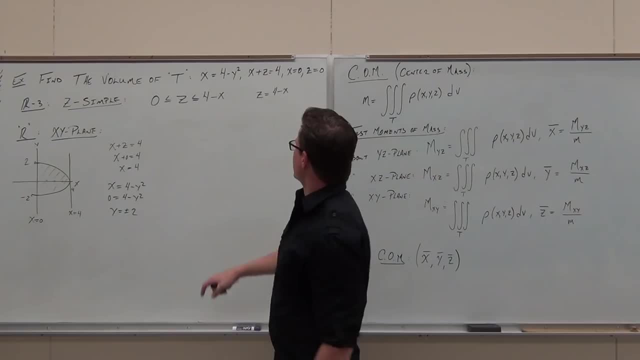 No, No, not so much. I wouldn't want to do that. What I would plug in is something like zero one and see if that works. If I plug in zero one, well, X is just one, I get three. 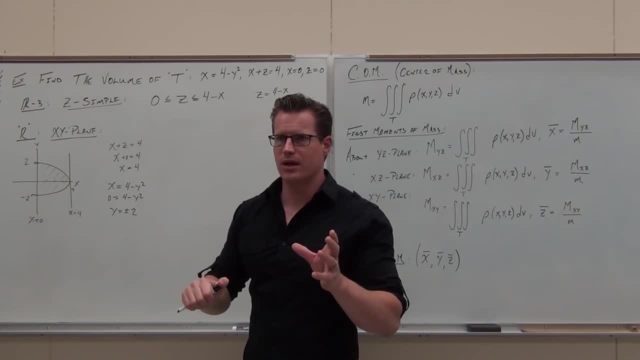 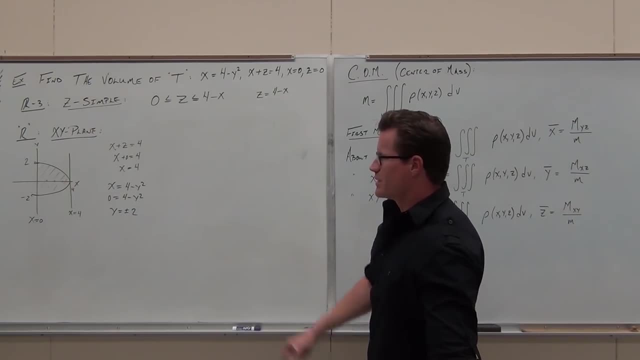 I get zero. I know that that's in the appropriate orientation and not if you're okay with that one. Okay, So I guess you'd plug in zero. So it would have worked there also if you had that cylinder going up. So anything else. 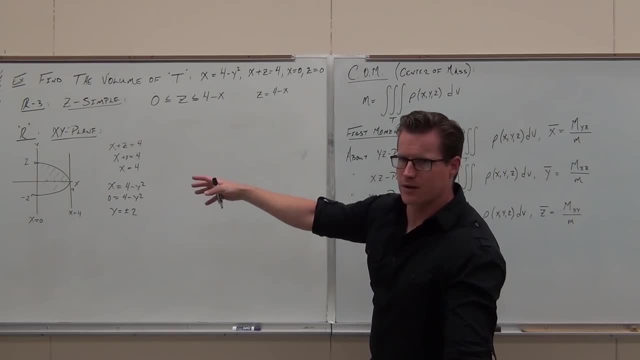 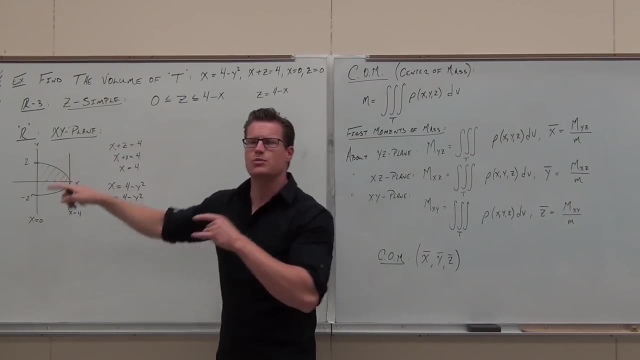 Usually you want to pick something on the inside of that region. That goes without fail if you pick something inside a region. So I know I'm going to be setting my triple integral with dz. first You tell me What's the appropriate choice for the R2 symbol. 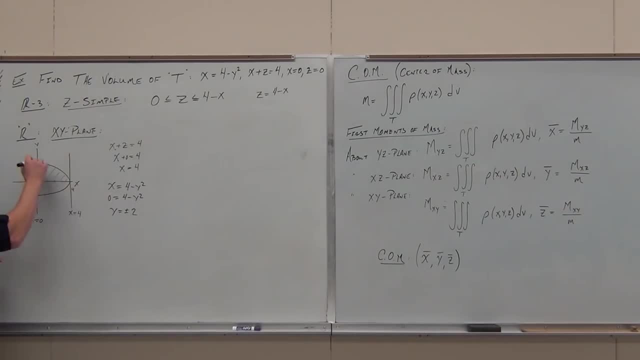 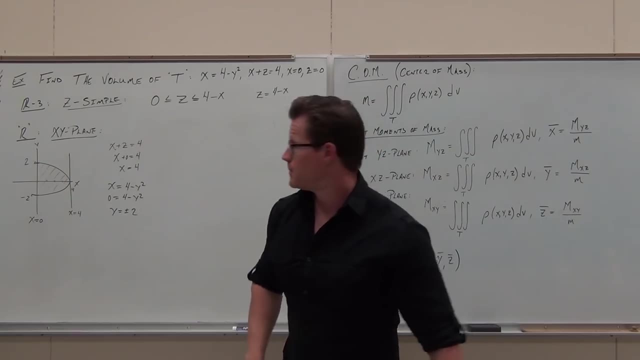 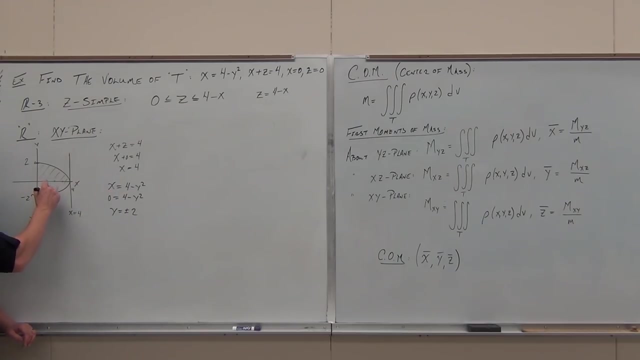 Would you want to go along the y-axis first or along the x-axis first? What would you want to do If I did the y? do you remember how this is given by one function? If I did the y, If I did that first, how would you go between one function? 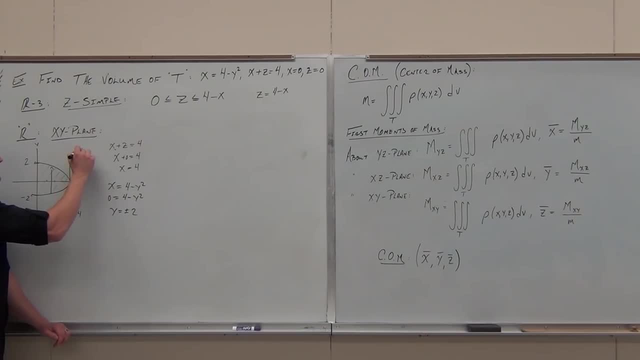 You'd have to break it up. You'd have to solve this, for y equals square root. from here, y would equal square root of four minus x. Does that make sense? Let's see, Have I done that right? Subtract: square root. 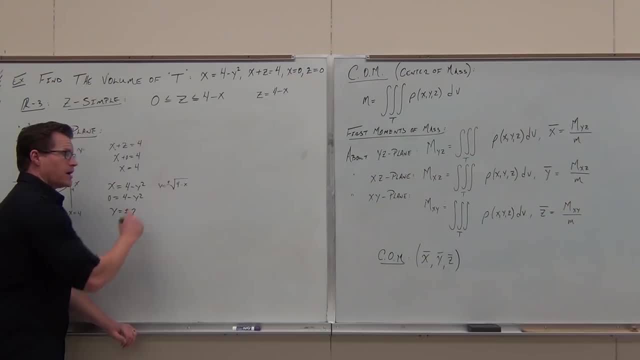 You have to do that. plus or minus You could do it. Is that going to be fun? No, Maybe that's not such a good choice. Also, I'd have to be plugging in two functions. I also don't want to do that. 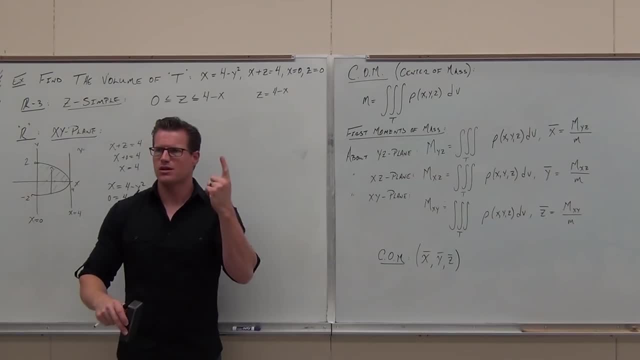 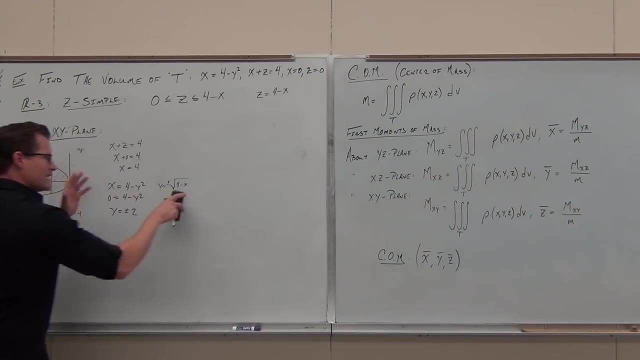 So when we start breaking up functions to go along a certain direction, try choosing the other direction, Try choosing the other axis and see if it goes better. Does that make sense to you? Yeah, So here? yeah, I really don't want to do that. 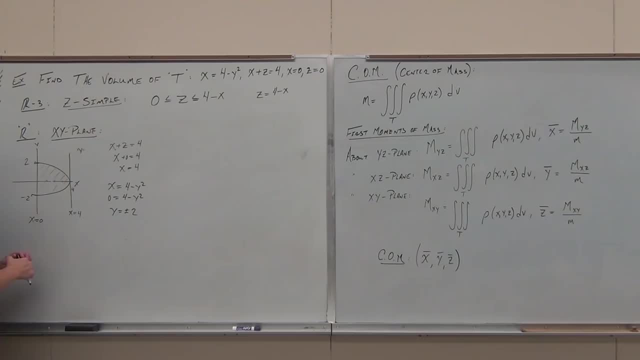 I really don't want to go along dy first. I'd like to go along dx first. No, No, I'd like to go along the x first. I'd like to go along the x first, Which means that I have this function. x equals zero. 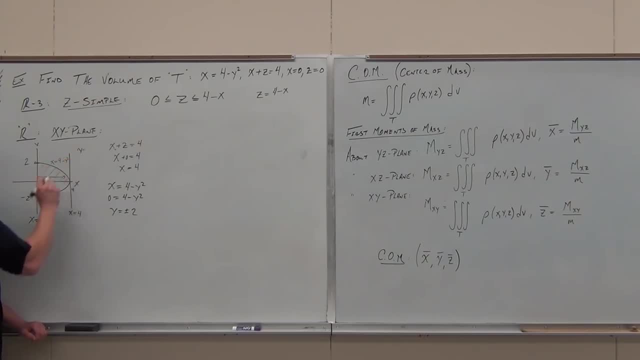 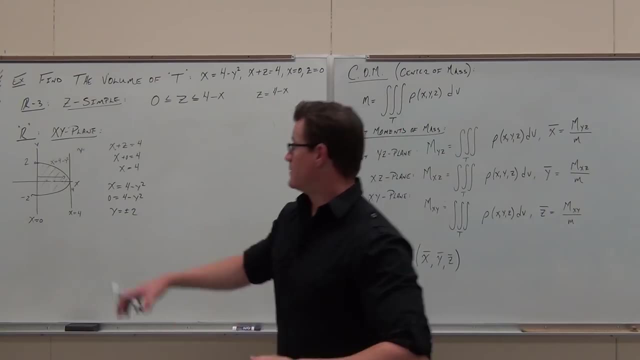 I've got this function. x equals four minus y squared. That's a much nicer way to go. Does that make sense to you? Yeah, You sure. So I had z simple Cool Mash z between two functions. I got it. 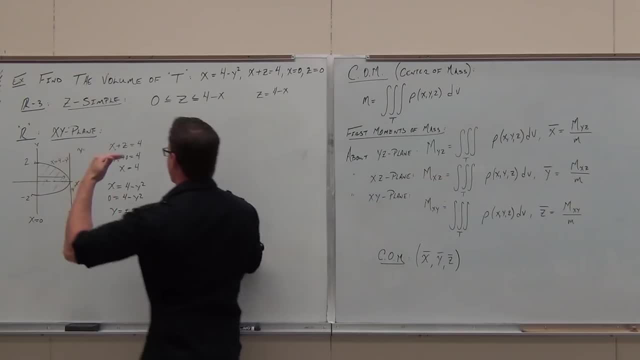 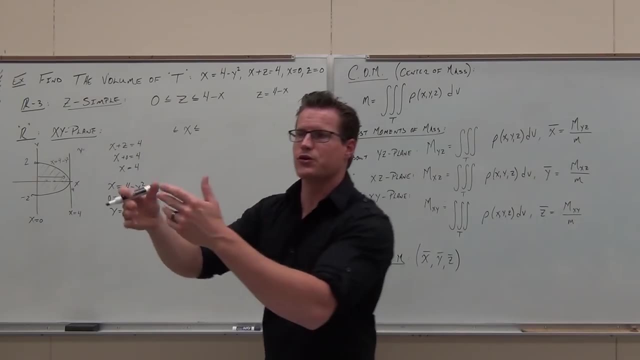 Go across the 3d space, Then I'm going to go along the x direction. That means I've got to mash x between two functions. two functions of x equals what's the first one? come on, help me out what's the first one, as I'm going through the region, what do we get to? that's why I 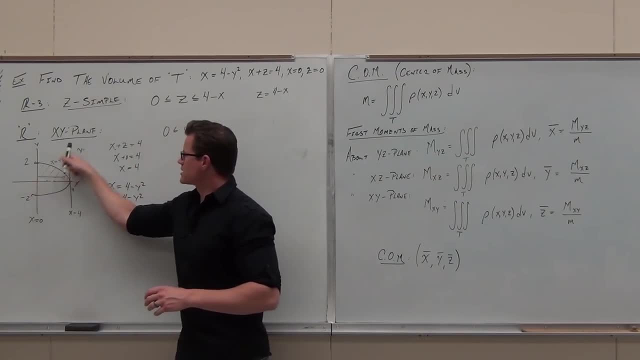 put everything on the ground zero. I don't make it to the x equals 4. I'm bound by this one. I'm bound by when I reach the far end of my region, 4 minus y squared every single time. hey, truly, show hands, feel okay with that. now I also. 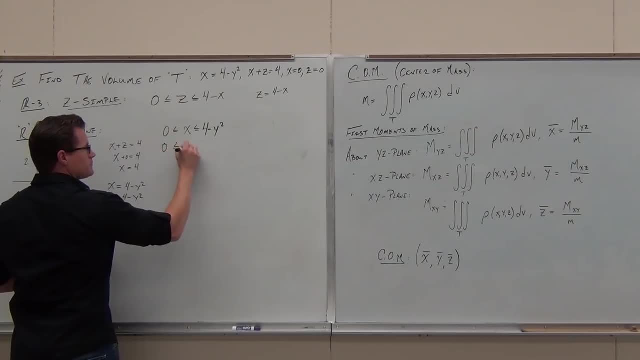 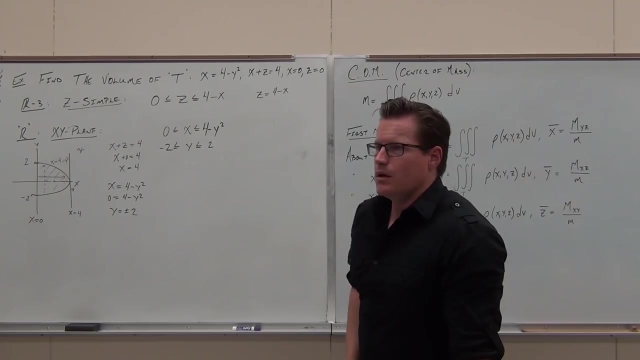 have to go between constants for my Y and if you look at it along my y-axis I hit the region at negative 2 and a maximum of positive 2. so anytime we're set of a region- r3 simple first, we typically pick Z simple. who can make sure regions kind of nice if it's given to you like all y equals? 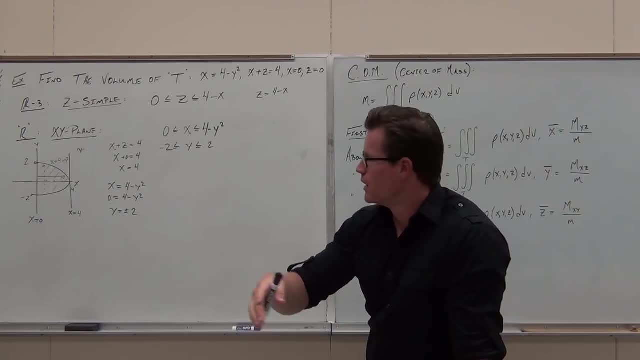 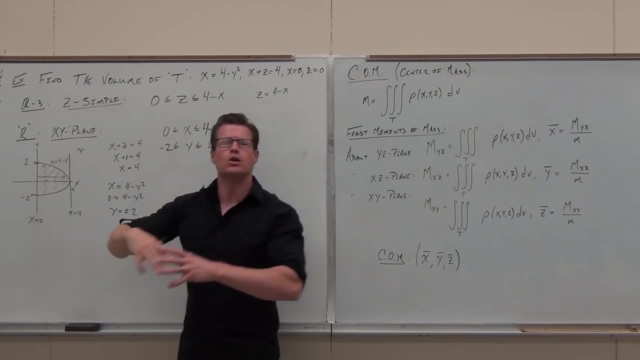 or x equals, then fine, of course, pick those y or X simple. after that we draw a region of whatever coordinate plane does not involve your r3 simple variable, no problem. draw everything that you can look at, the region that's bound between the curves, and then set up a really nice. 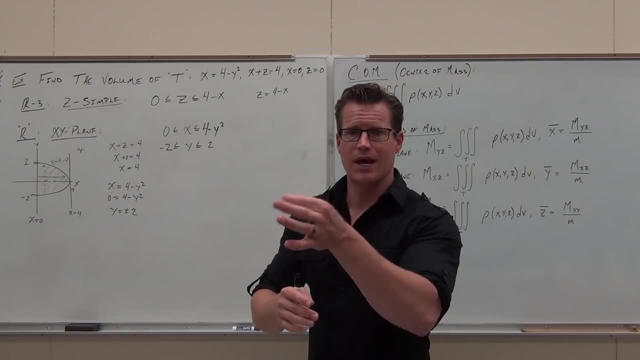 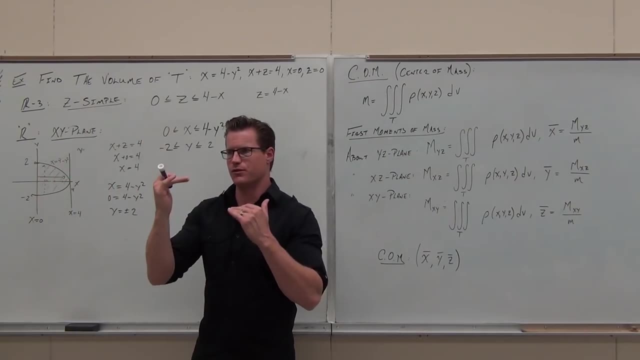 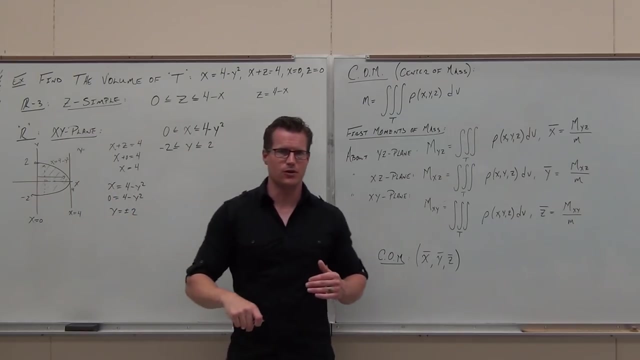 r2: simple, something, hopefully, that goes between 0 and a single function. that's what you want. don't start going in directions that force you to break up functions and two different functions. that's horrible, because if I did this- sorry, if I did this first- I'd go between two kind of nasty functions, both of 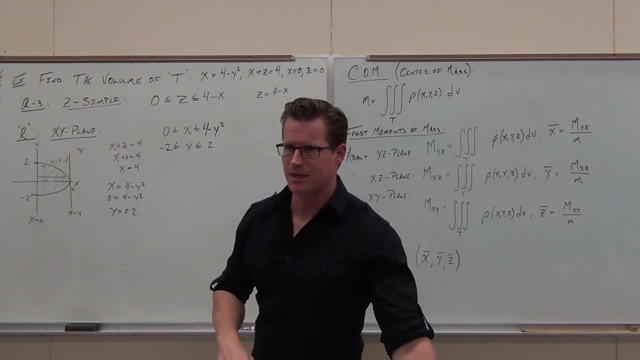 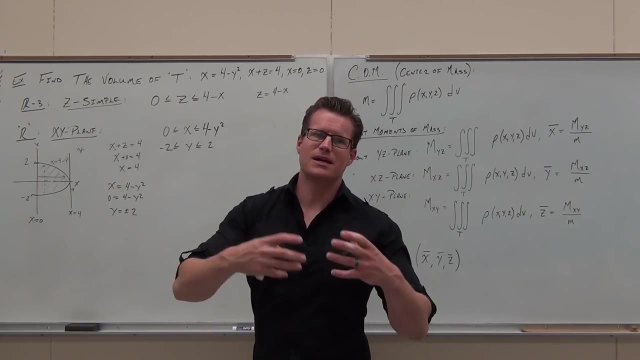 which have square roots. that sucks. don't do stuff like that. does that make sense? so keep it as simple as possible. that's why they call it Z simple. that's why they call it Z simple. right, it's not, but it does make it nice if you can go between 0 and 1 function. 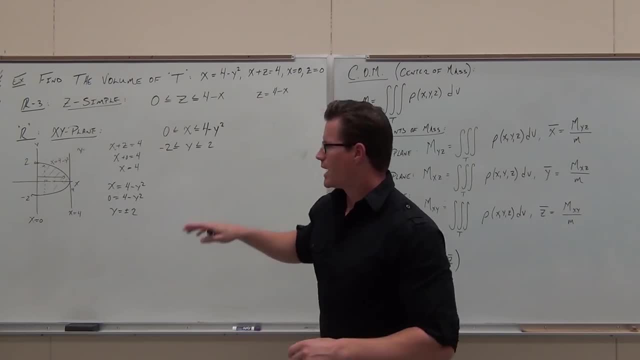 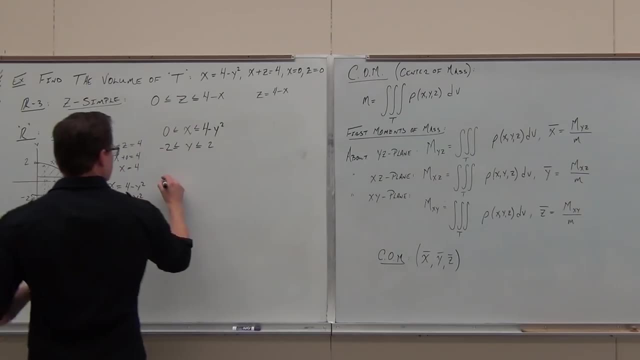 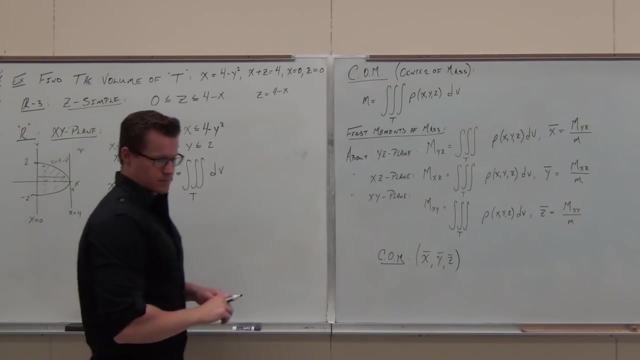 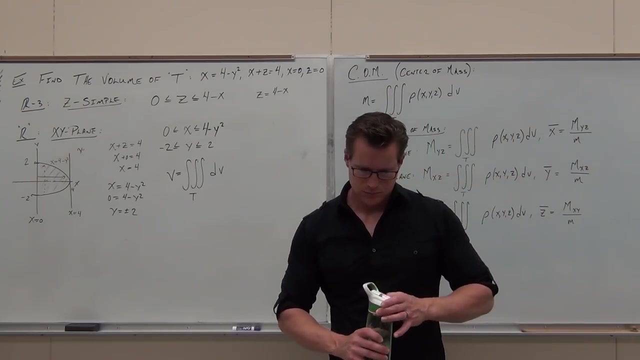 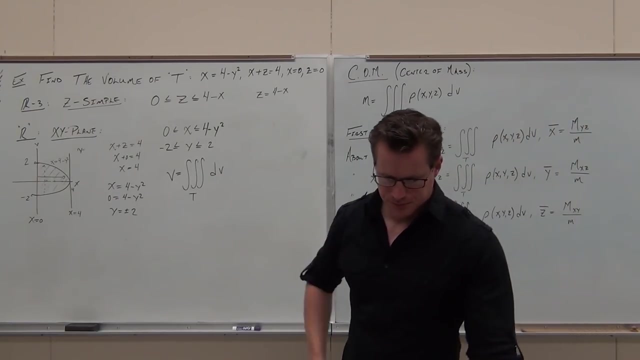 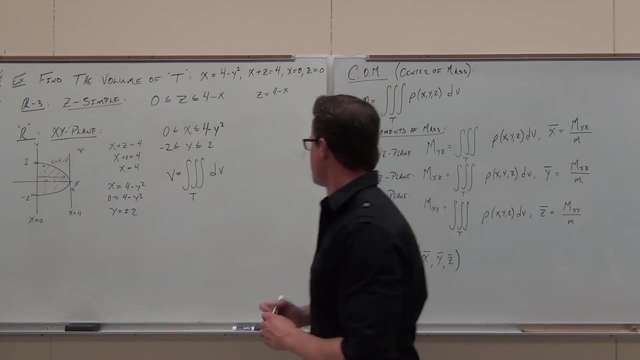 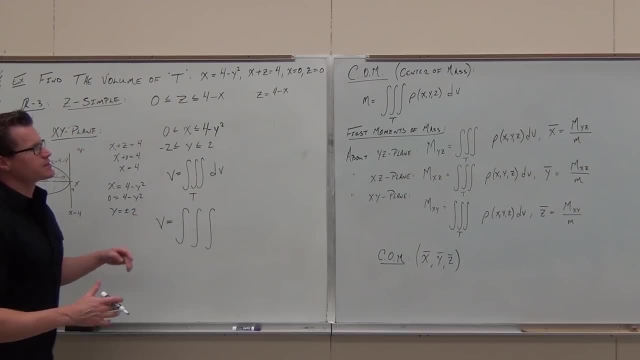 you, you set the south. i know that I have to do dxtYNC but it all depends on how you easy. but it all depends on how you choose to do your year to your symbols. r3 simple choose to do your sm peine, your sin fools. R3 simple said I need a dc first. 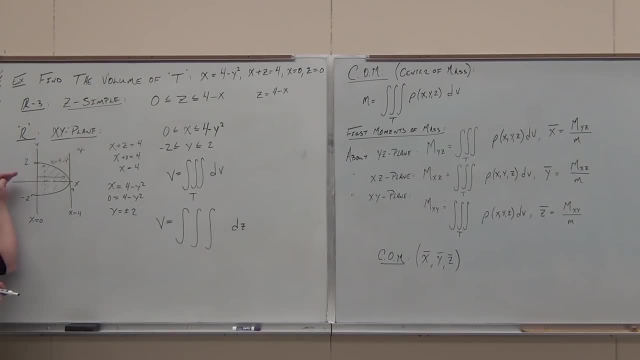 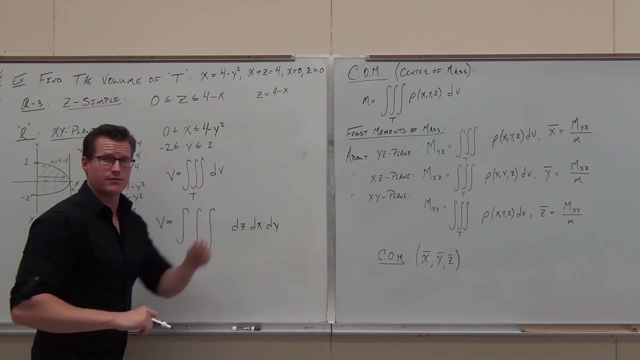 after that i will go along that region if your, if you choose to combine your region, of course, two of the X and c and y are c with z, equals to z, equals to z to the union, and then uidnow, that's fantastic. then it just used bus. 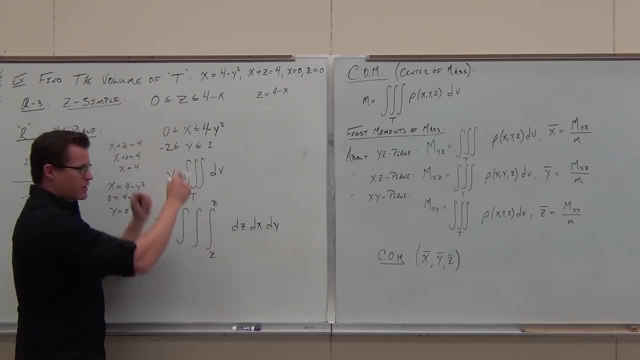 We have Z equals to Z equals. It should have an inequality up there somewhere: X equals to X equals. You should have another inequality up there And then Y equals to Y equals should have another inequality. It should be between functions at most, functions at most and then constants at most. 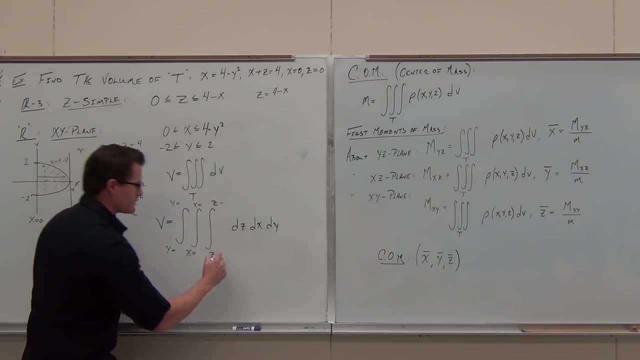 That's how these things are all set up. So here Z, we got 0,, 4 minus X, For X we have 0,, and then 4 minus Y squared, And then for Y we have negative 2 to 2.. 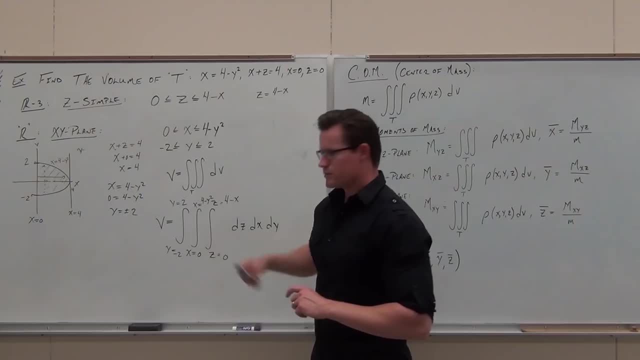 Now, next question for you guys: What goes there? 1. 1. Nothing, Because that's the whole nature of this volume. If I take the volume, if I do a triple integral over a region with a height of 1 in four dimensions, 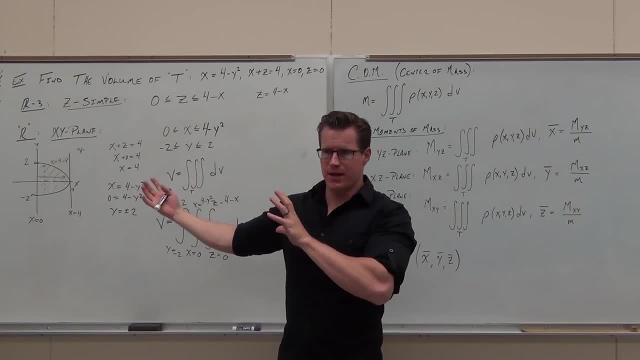 what we're getting is this: 4. It's a three-dimensional thing. that's numerically not unit, numerically equal to the volume of that 3D region. That's what we're doing, just like the area over a double integral. 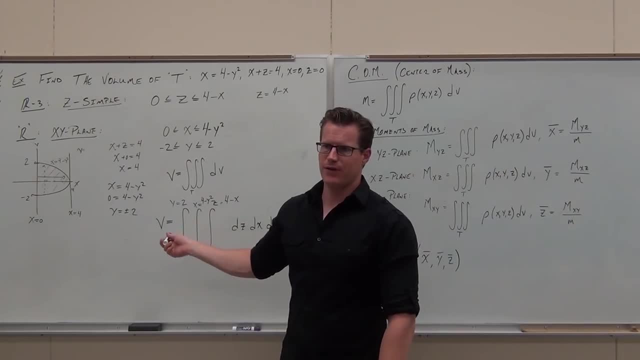 Same thing Now. could you do that? if I asked you, to What would your first step be with respect to? you're just going to get a Z, Then you're going to plug in stuff for Z and integrate with respect to X. 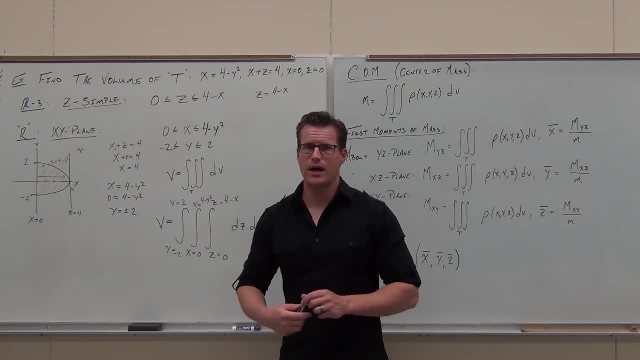 You're going to plug in stuff for X and integrate with respect to Y. You're going to plug in stuff for Y. Bless you, I really don't want to go through the whole. I'm not going to do any of the motions of doing this triple integral. 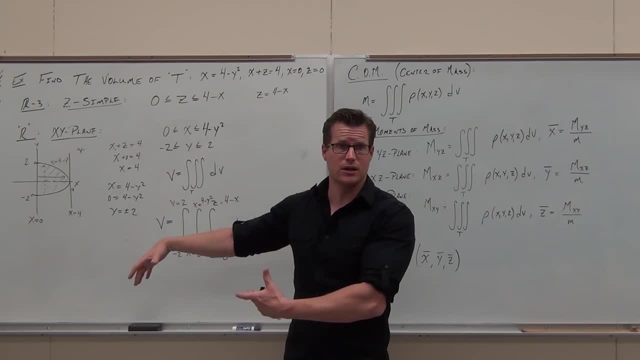 Would you guys be okay if I the setup was the most important thing? Would you be okay if I just give you the answer and you try it later? The answer on this thing. if you want to check it later, you know what to do. 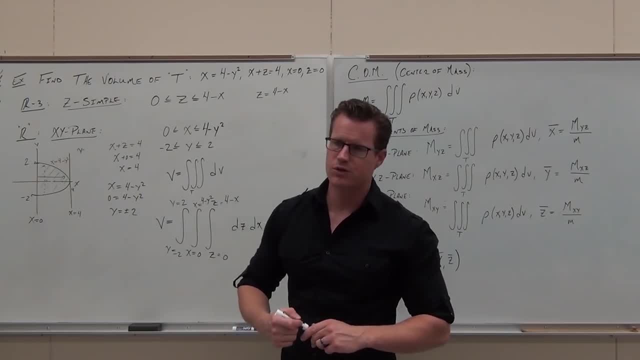 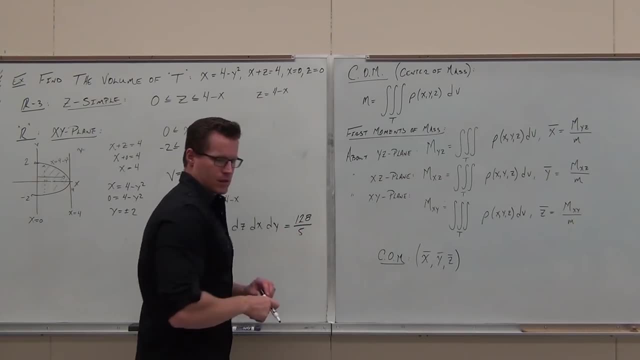 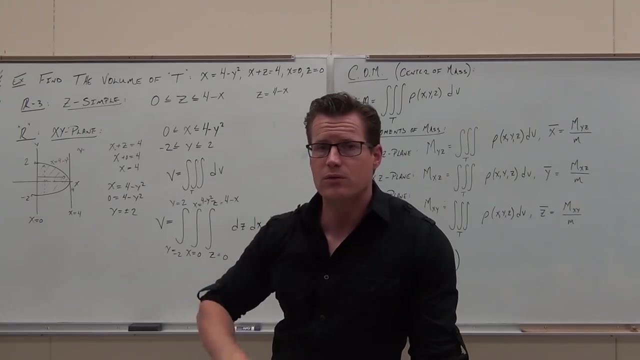 Z, plug in for Z. X, plug in for X. Y, plug in numbers. You're going to get 128 over 5.. Here's the thing I want to make absolutely clear. Do you feel confident on setting up a triple integral right now? 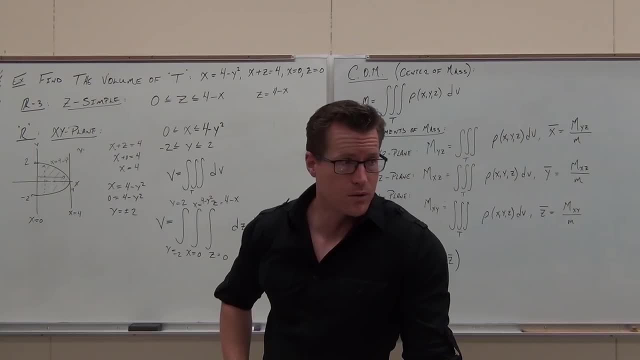 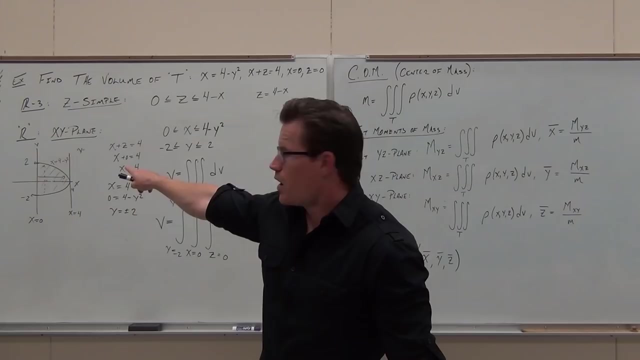 What's your first step? R3, simple R3 simple- X, Y or Z. Pick the best choice. After that, you do what? A region on a coordinate plane. Then you draw that region And you determine whether it's polar circles and stuff or nonpolar rectangular equations. 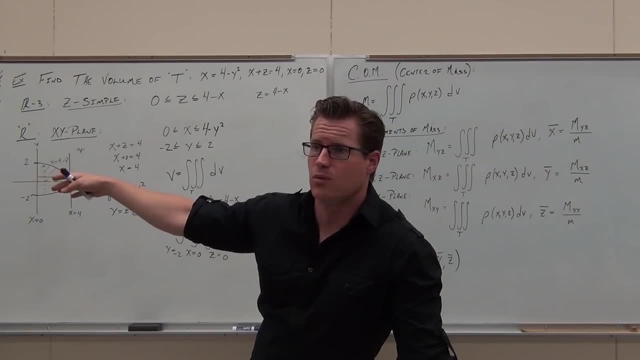 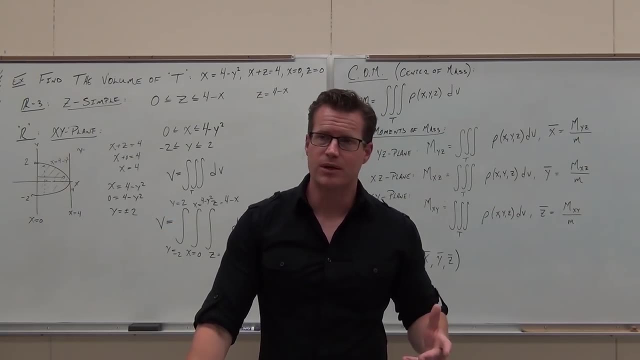 And you choose the appropriate direction- Either along the X or along the Y- You set up your triple integral And then it's all easier after that. I do have one more example. I don't really think I want to do it. You guys seem to be getting this really well. 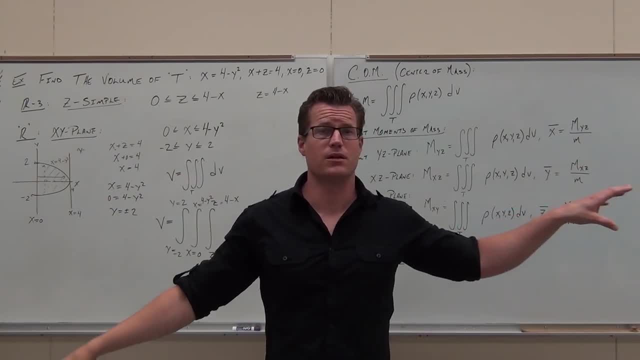 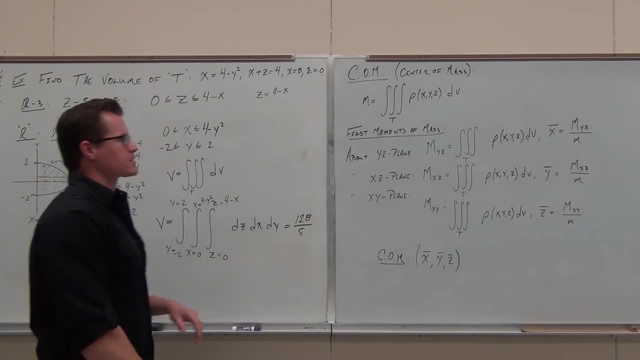 Do you guys want to skip that one and go on to this stuff, Or do you need another example? You feel okay with that? Okay, so let's move on. The last thing: We talked about this in 14.4.. We did it, though, with planes. 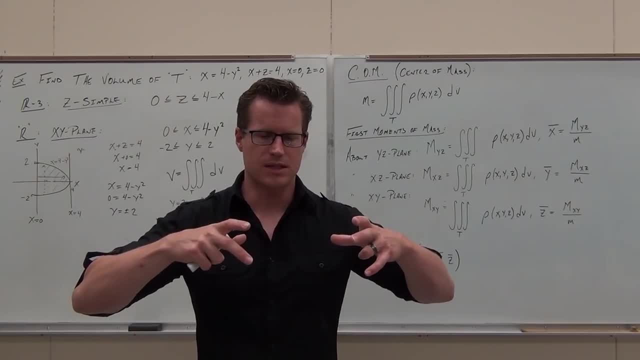 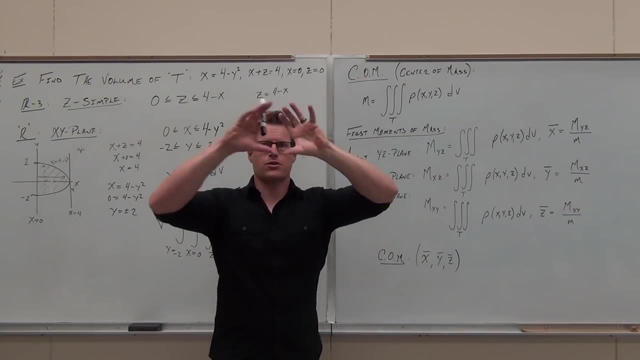 Things that were like two-dimensional Regions on planes. Now we're going to talk about three-dimensional. So we still can find the center of mass. We can find the mass of a three-dimensional region. We've already done the first part. Actually, that's exactly what we've been doing this whole entire time. 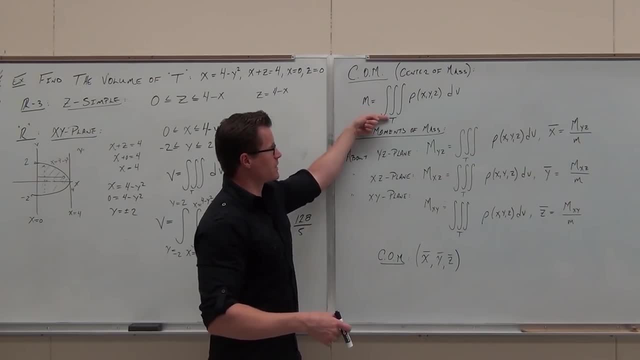 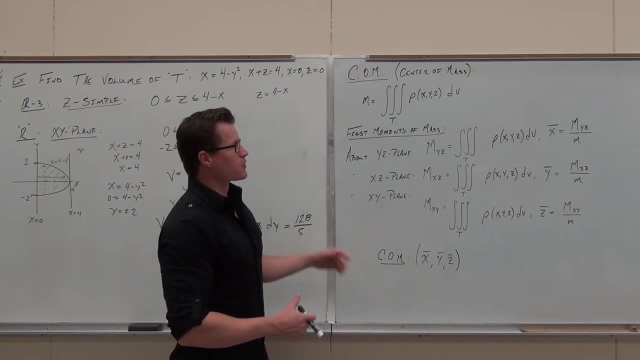 We said: hey, what's a triple integral? We could think about it as the mass of a 3D region. if we're given a mass density function, That's literally what we've been doing the entire time. The rest of it says: well, the first moments of mass look really similar. 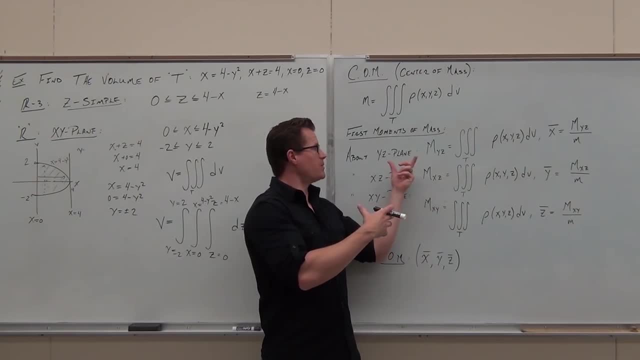 It's just, I don't have double integrals, I have triple integrals. I'm not going about an axis, I'm going about a plane. now, And you see the pattern. If I want to go about the YZ plane, I'm going to call that the first moment about the YZ plane. 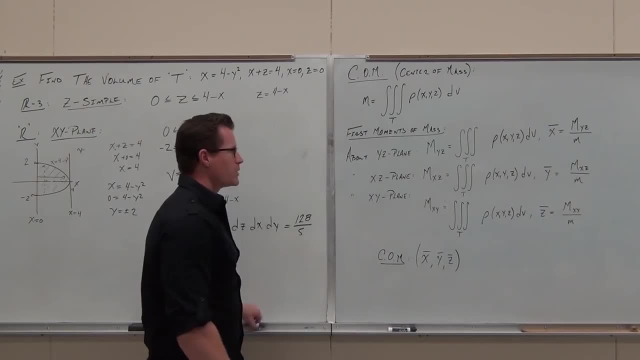 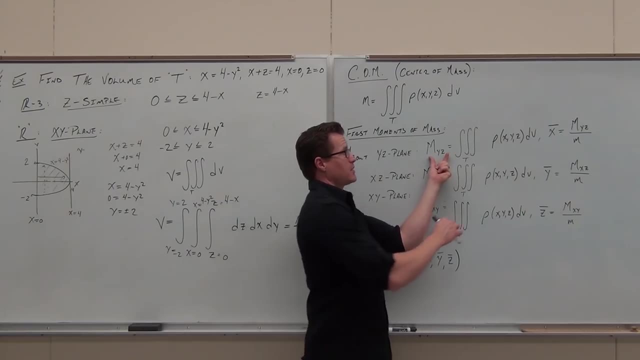 And what we learned about last time in 14.4 was that all of the variables are opposite of what you have here. So if I'm going about the YZ plane, look at the board so you don't get confused in your head. 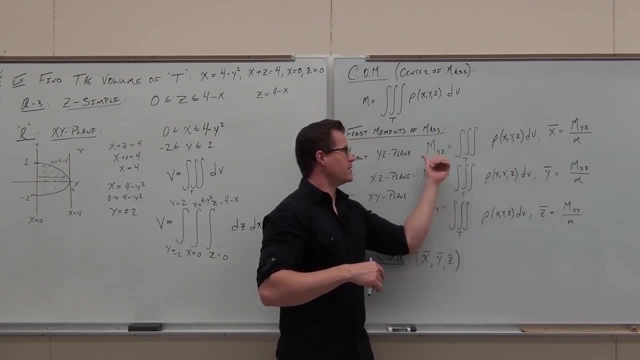 This is literally just the same thing as mass. Do you guys see it? If I want to find the first moment of mass, we compare that to how far away the mass density is along the axis perpendicular to the plane. So perpendicular to the YZ plane, that's X. 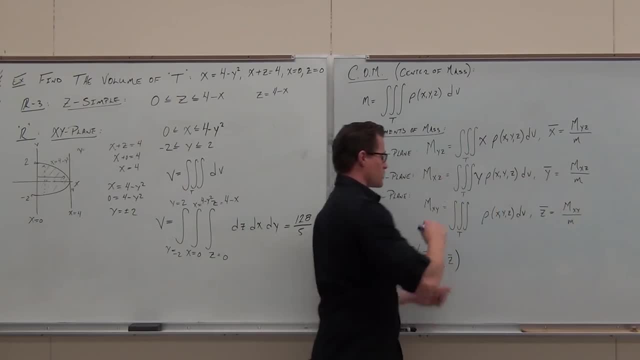 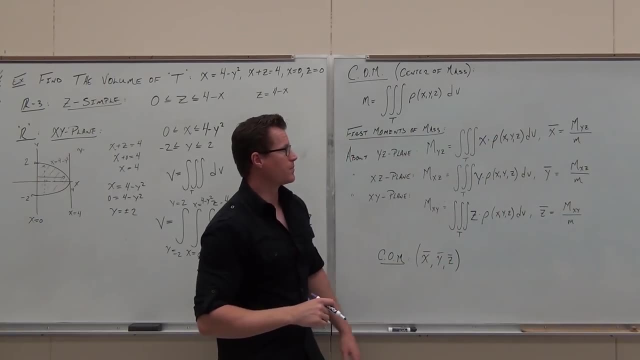 That's an X direction. Perpendicular to the XZ plane, that's a Y direction. Perpendicular to the XY plane, that's a Z direction. They look very, very similar to stuff we've done in 14.4.. And then, if you remember, the center mass idea was: hey, you take the first moment of mass. 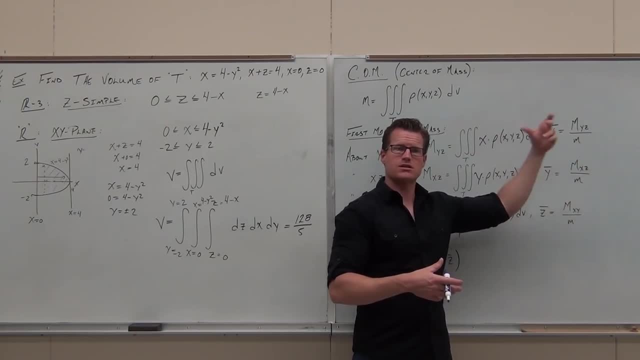 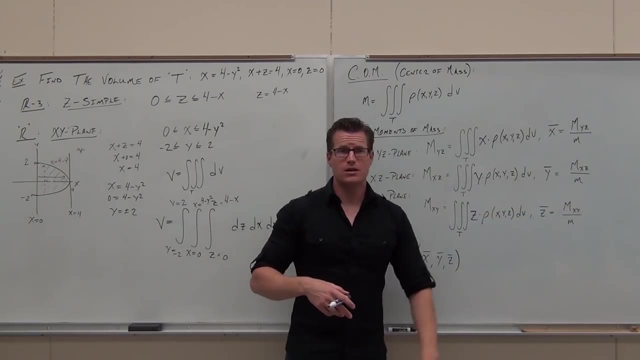 divide by the total mass of that region and you get this kind of average Along the X axis, Same thing for the Y axis, Same thing for the Z axis, And if you put it all together you get the center mass of a 3D region. 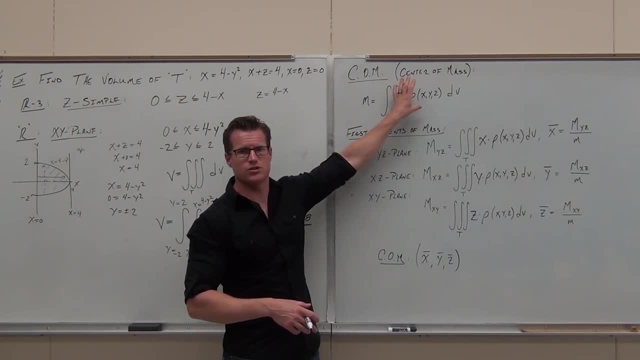 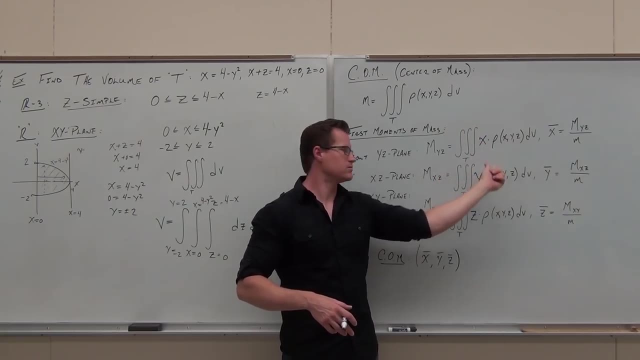 That's it. Have we done this before? Oh yeah, This is what triple integrals are. We've done that. a ton, This is exactly the same thing, exactly the same setup. You just tack on an X, a Y and a Z. 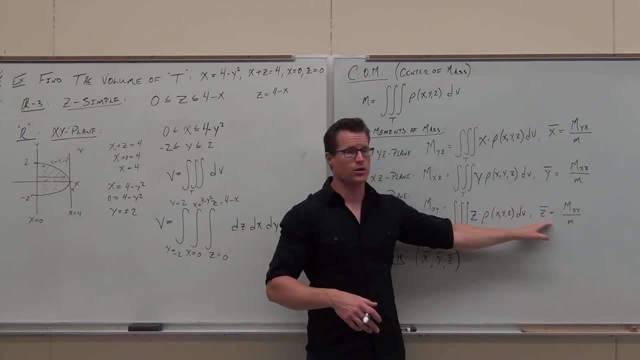 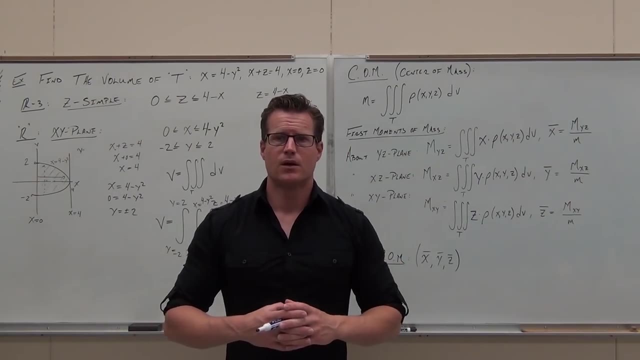 and it gives you the X, the Y and the Z coordinates. if you divide by mass And that gives you the center mass. That's typically how these things are used- is to find center mass of a 3D region. We're not going to do any examples of this in this section. 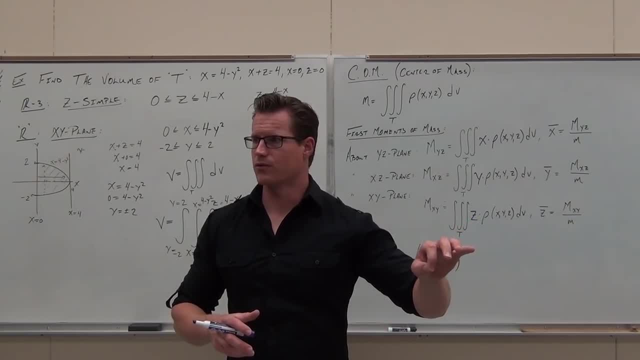 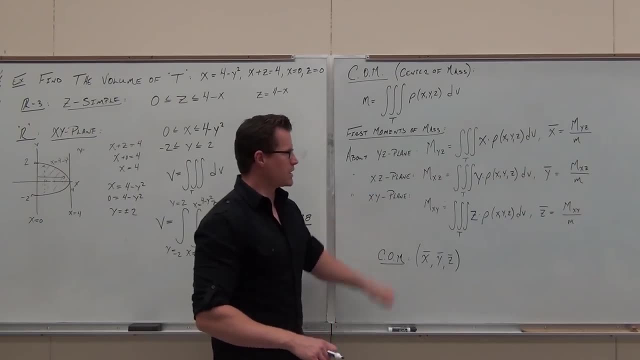 but in the next section you're going to get a shot at doing this. We're going to find the center mass with some triple integrals. We also have, like, on top of this stuff we also have second moments. You guys remember talking about second moments of inertia, all the inertia stuff. 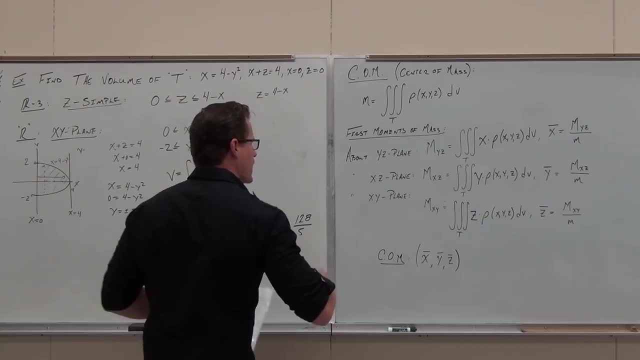 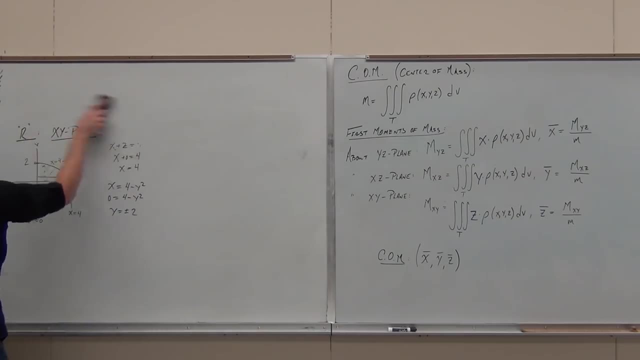 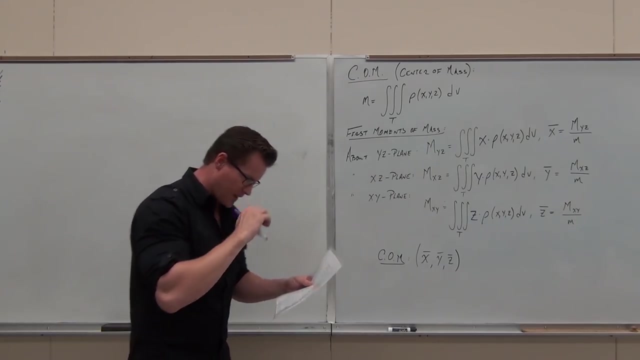 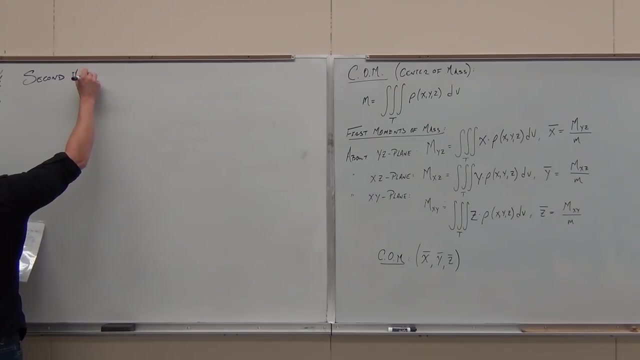 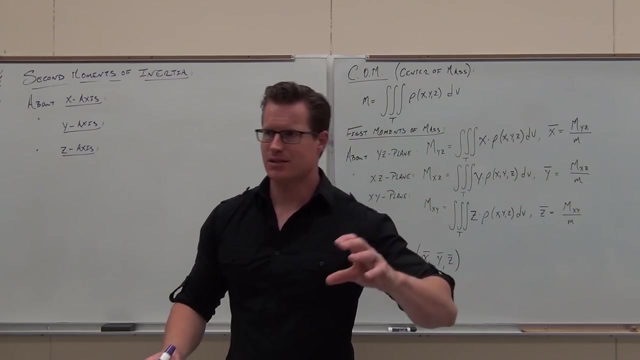 We also have that. It gets a little more hectic. but I'm going to talk about the second moments, Second moments of inertia and we'll do one pretty much just setup problem and go through it. So second moments of inertia. So with the second moment about the X axis, 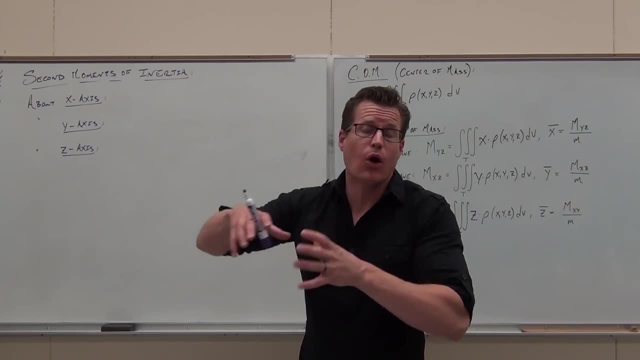 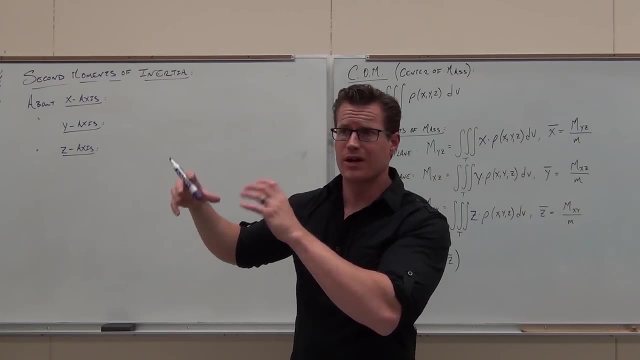 that's basically saying how hard is it to get this 3D thing moving about the X axis? The larger the number, the harder it is to get it to move. It's the same thing with respect to the Y axis and the Z axis. 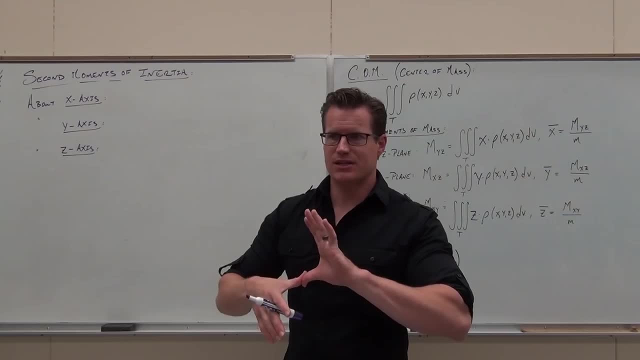 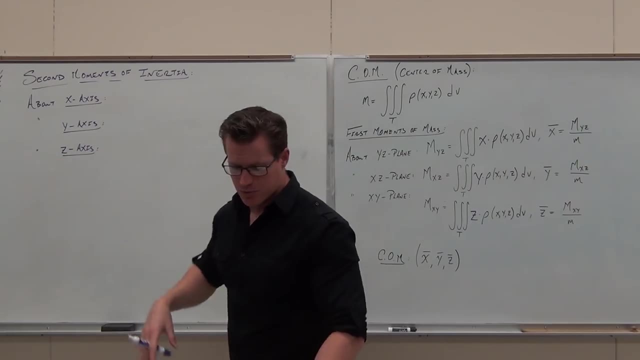 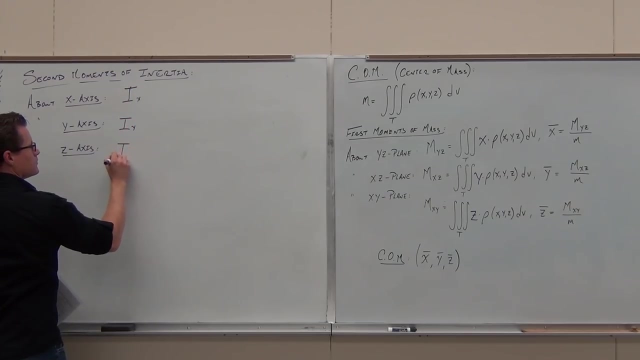 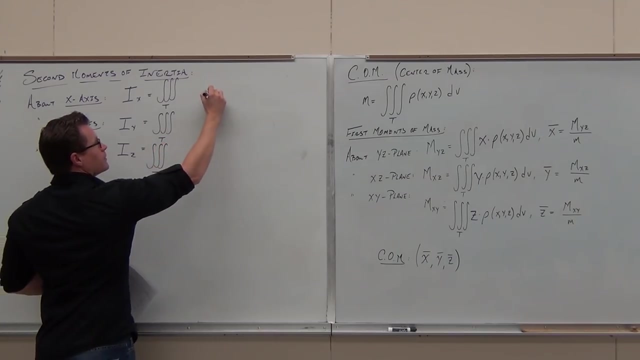 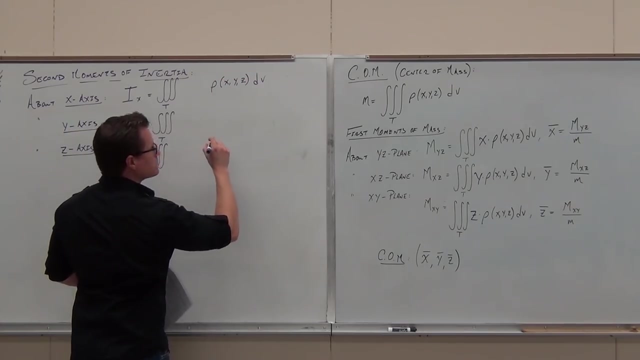 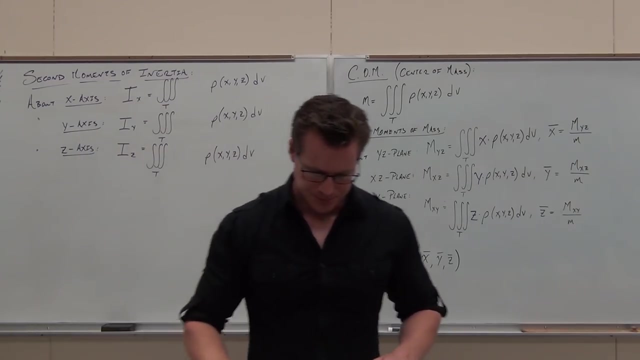 We also had this idea that if we're talking about the X axis, it's using the two different variables to compare this. You're still going to have a mass density function, but inside of our triple integral that we create here, we're using some kind of this. 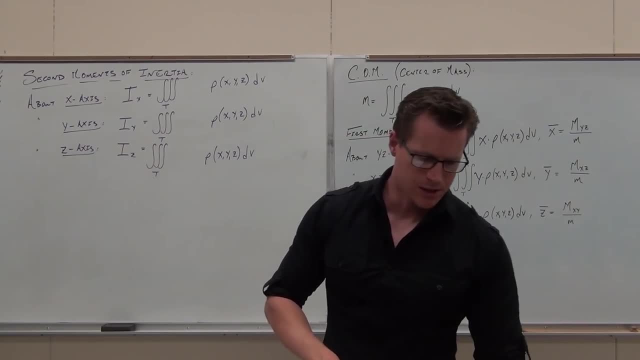 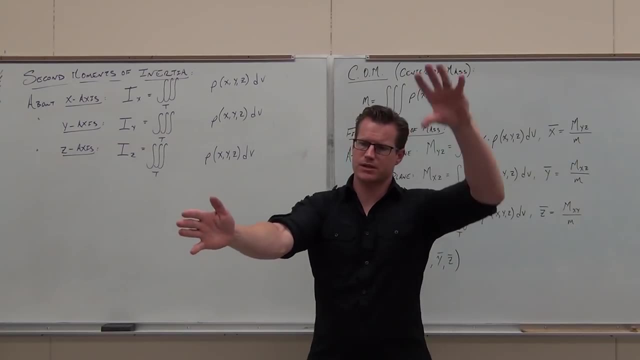 I'm not going to go through like a rigorous proof or anything like that for this. I just want to get the idea in your head. if I am talking about this 3d mass, that's away from the x-axis, and I'm trying to say how hard is, is it to get? 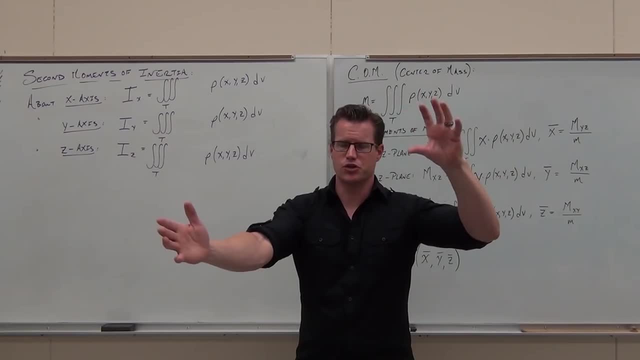 this 3d mass to move about the x-axis. to get it started, that's an inertia concept. well, I have two measurements. I've got how far it's away from the x-axis in the x-direction and in the y-direction. does that make sense? I've 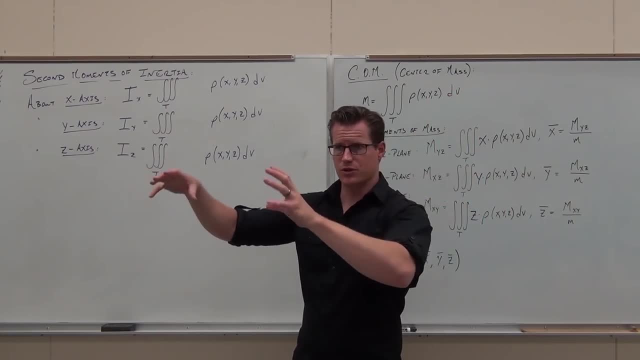 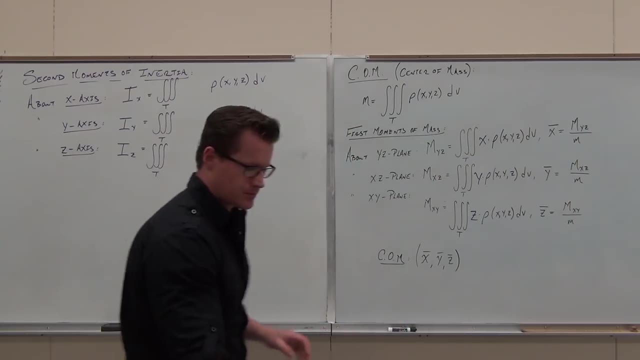 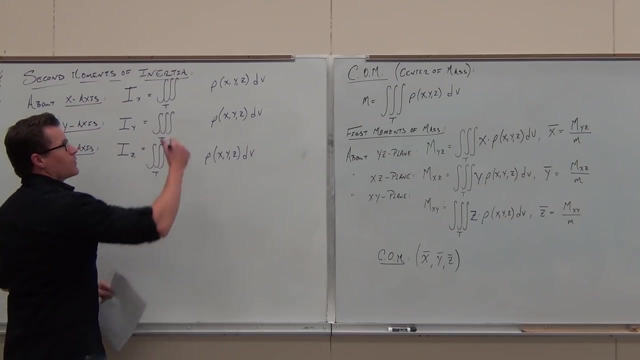 got. I've got two of them. if you compare that to the, the moments of inertia for 14-4, there was only one of the variable along there. okay, but here we got, we got two. we're gonna have the other two variables not on this axis. so and oh by. 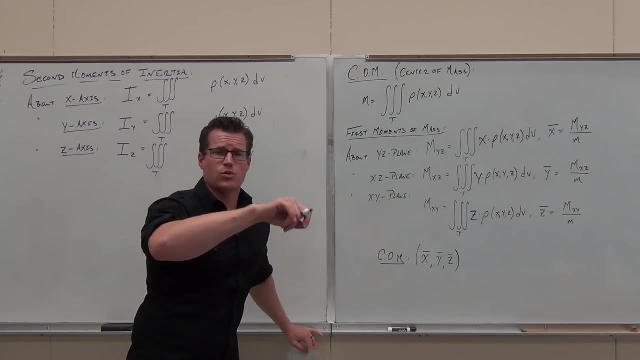 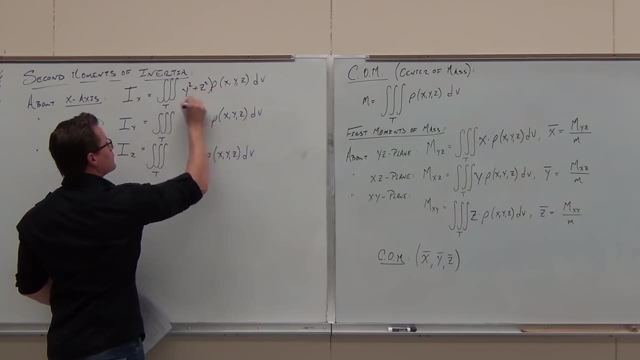 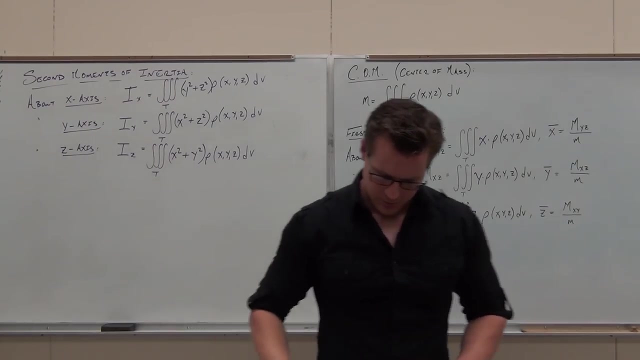 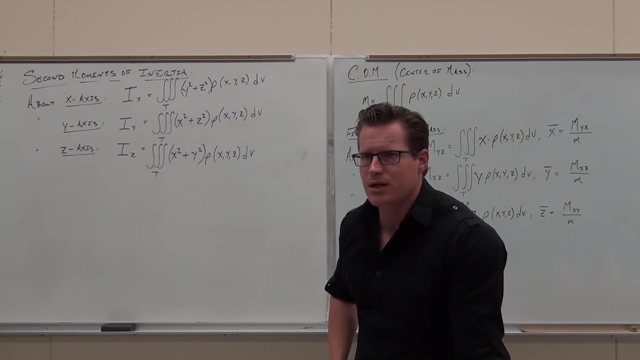 the way and the moments of inertia from from 14-4. they were all squared. they're squared here also. you let's how you find the second moments of inertia. we're gonna do one kind of quick example about how to do this and then we'll be. we'll be good to go, if you. 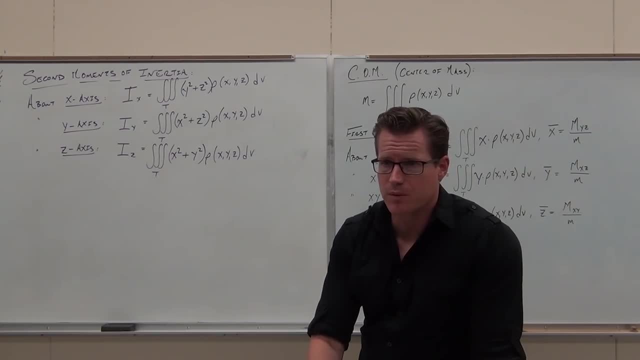 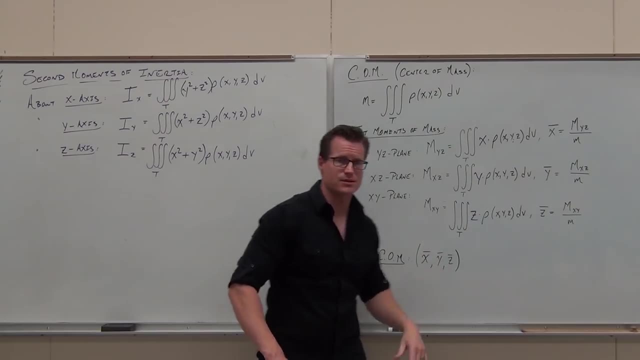 need a refresher. go back and look at the 14-4 stuff about moments of inertia. you're gonna see a lot of some similarities between first moments of mass, where the separation of the unit comes from, how we get this where the center mass is. 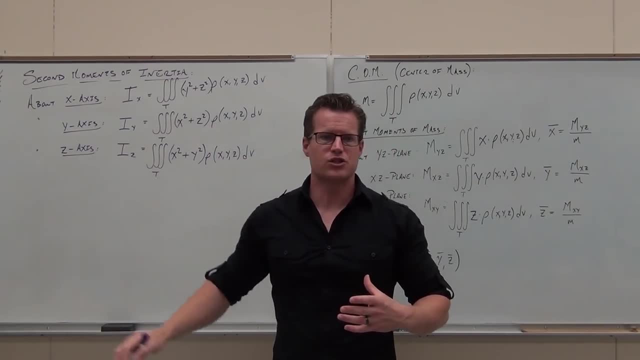 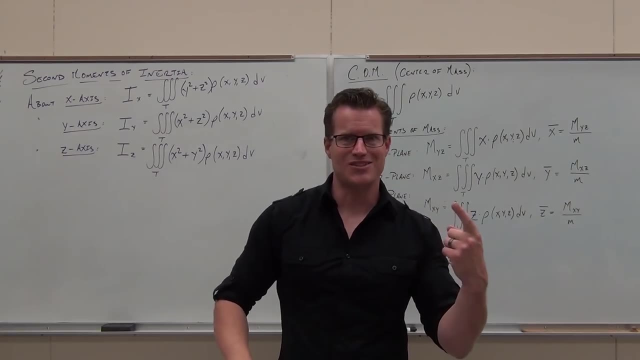 and what the moments of inertia are. They look very, very similar, Are they super hard to do? Well, there's two things that make these things difficult. One is the setup of the region, but you guys know how to do that, right. 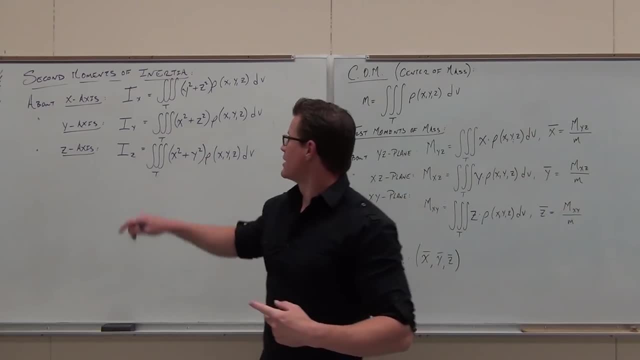 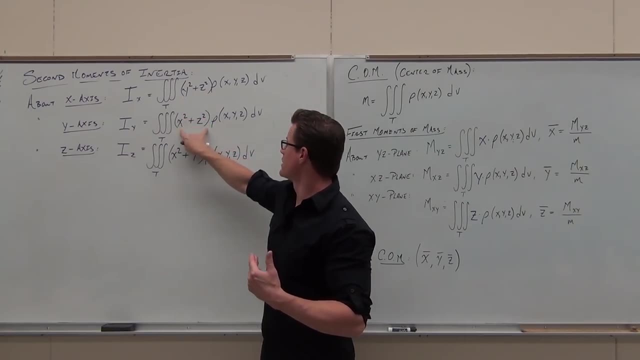 Setup the region. that's the hardest part. The second hard part is when you start tacking stuff on in here. this can make your stuff freaking crazy, okay, So you start doing this and then you have a mass density function. this can get some nasty, nasty triple integrals in there. 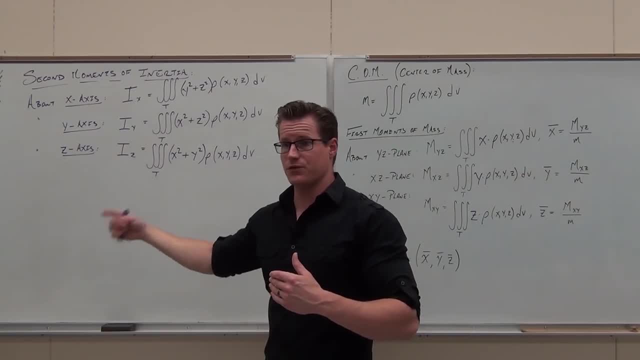 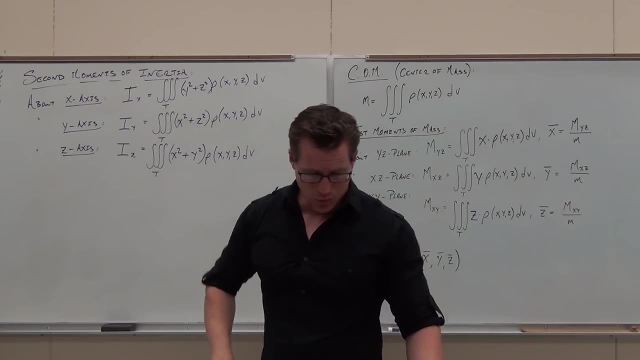 not because the region's hard, but because you're starting to integrate with lots of different variables and you're plugging in and you're distributing like crazy. Does that make sense? So that can make it difficult. Let's try one example. 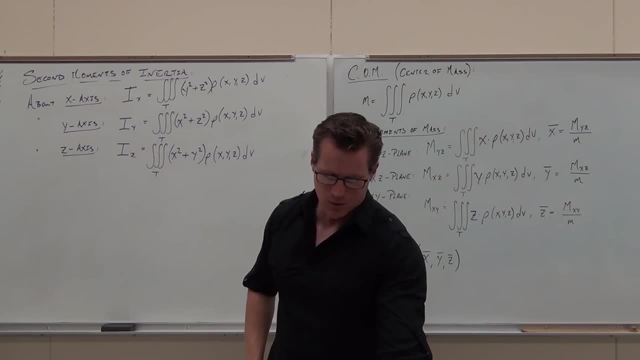 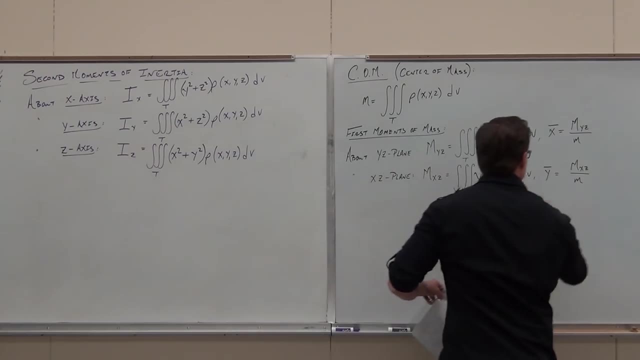 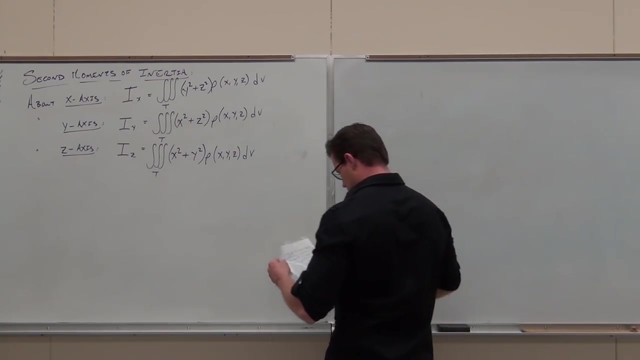 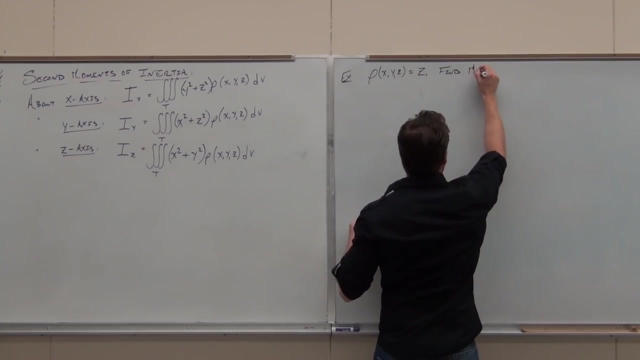 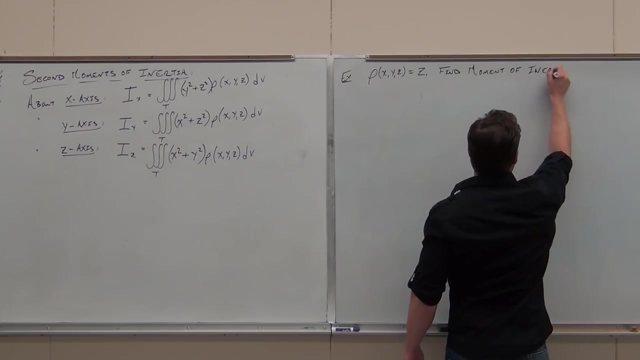 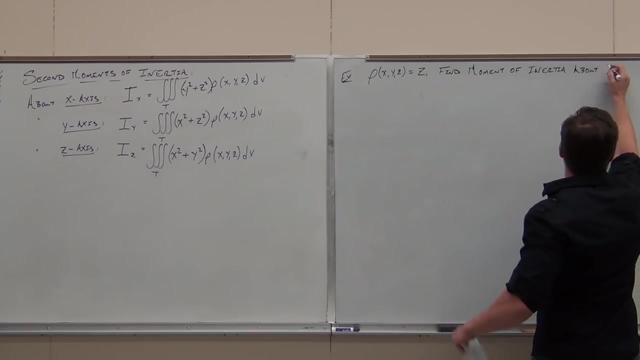 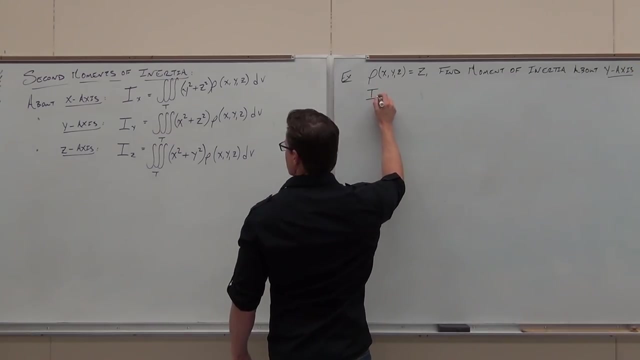 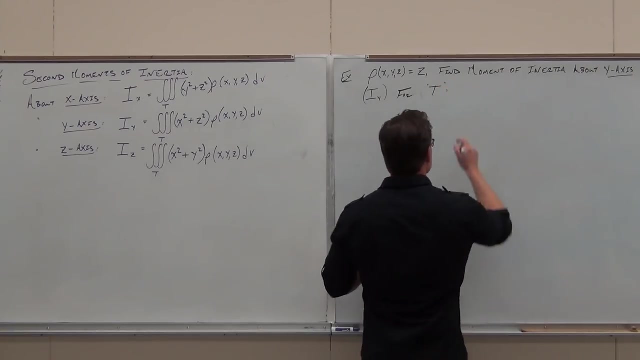 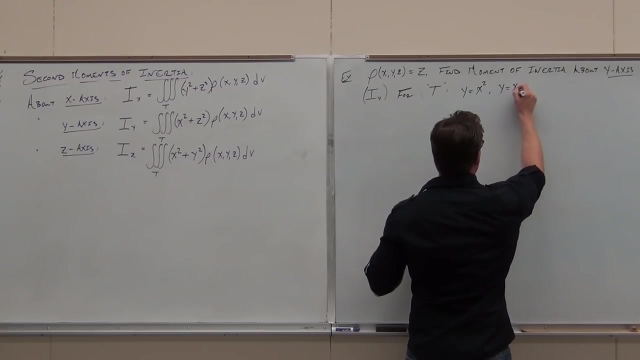 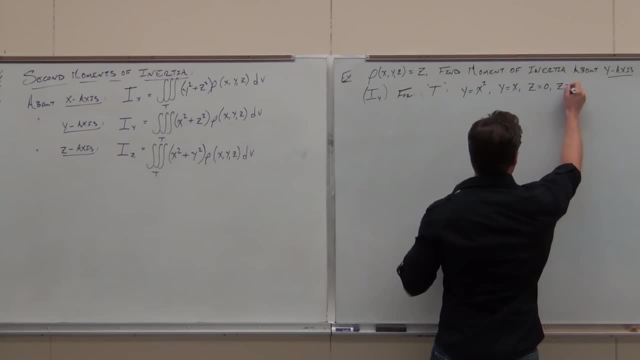 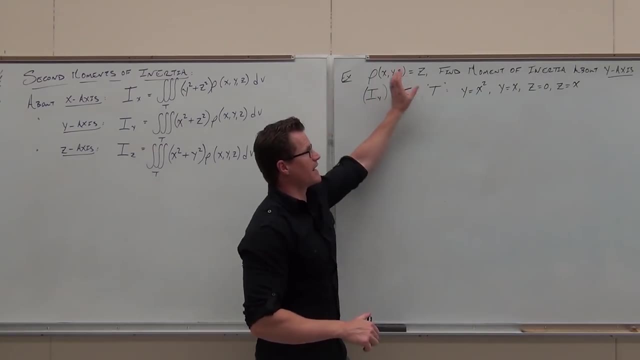 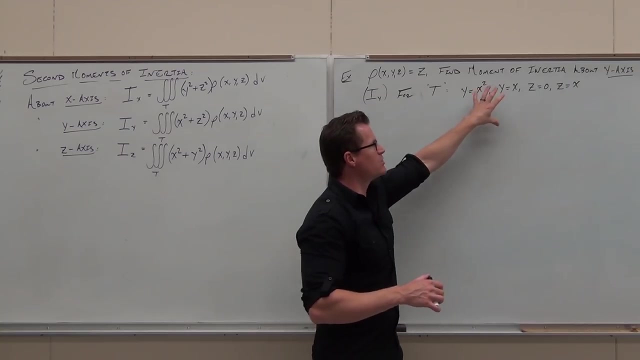 So I've given you a mass density function that's related to this 3D region. This thing's gonna create a region for us. What we're looking for is how hard is it to get this region started about the Y-axis given. 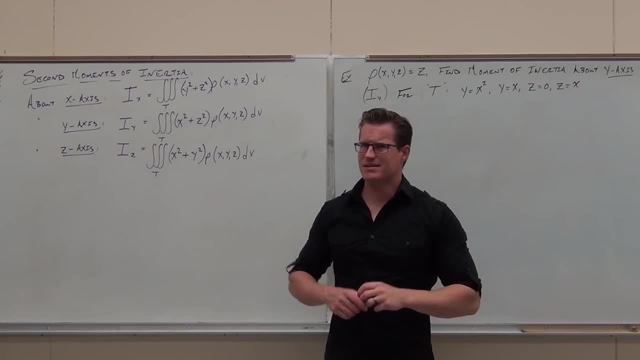 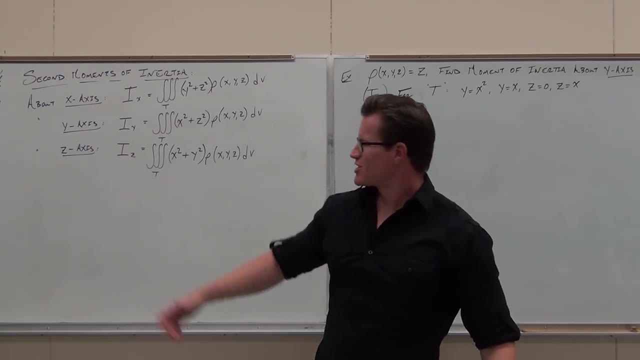 that it has that mass density function. Does that make sense? The mass increasing as we go along the Z-axis? That's what that says to us. Okay, well, it's just a setup, Man. it's just a setup of a triple integral. 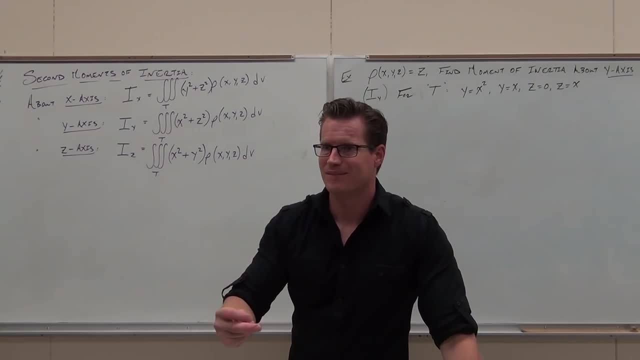 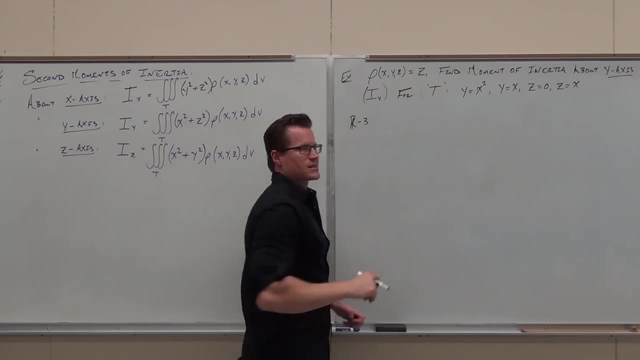 What's the first thing you do with the setup on a triple integral every single time. What do you do? R3 simple. Let's set up R3 simple, So write that down. Listen, I don't want to make this harder than it is. 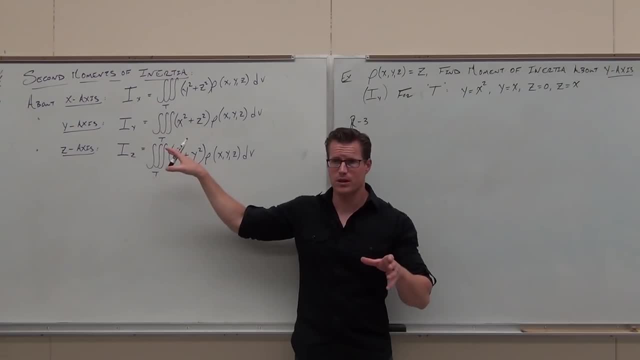 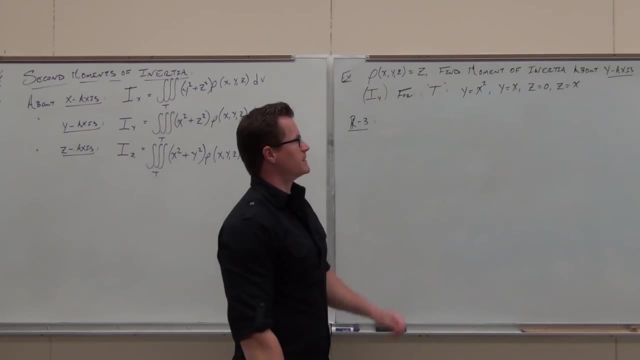 Do you guys recognize that? this is exactly the same concept? You just have a formula and you've got to add some extra variables onto there. Yeah, It's the same thing. So R3 simple. oh man, you've got two choices here. 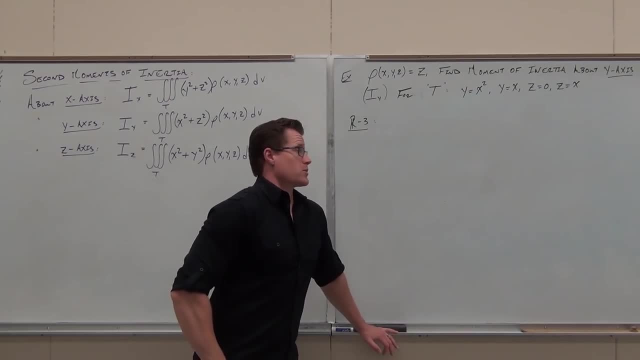 two choices, what's a? what two choices could you do? You could do all three, really, if you wanted to. What could you do? Y and Z? Z simple. you could do Y simple. you could even do well. 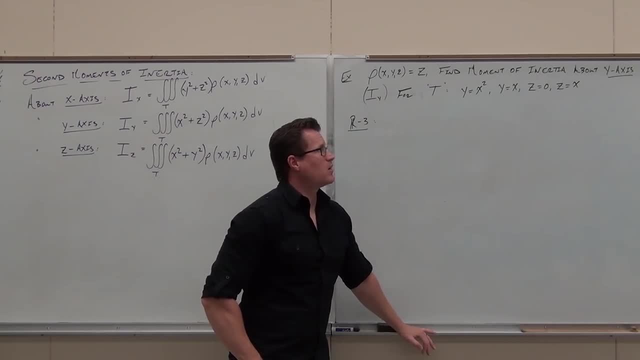 X simple would get a little funky because you have three of them, but it's probably between Z simple and Y simple. What's the better choice between Z simple and Y? Y is Z simple, you're right, but why The zero? 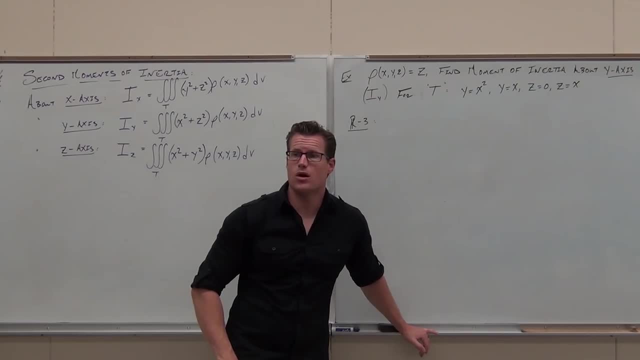 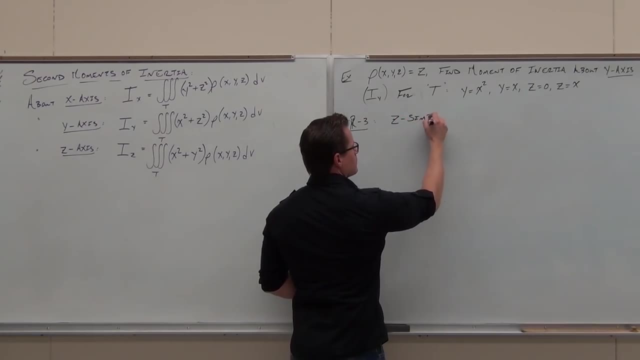 I love the zero, love the zero and that keeps our region kind of easy to draw on the XY plane and we can draw those things really nicely. So let's pick Z. simple, That means that Z is going to get matched between two functions. 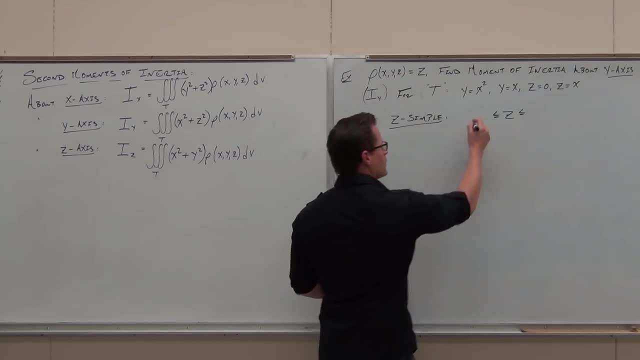 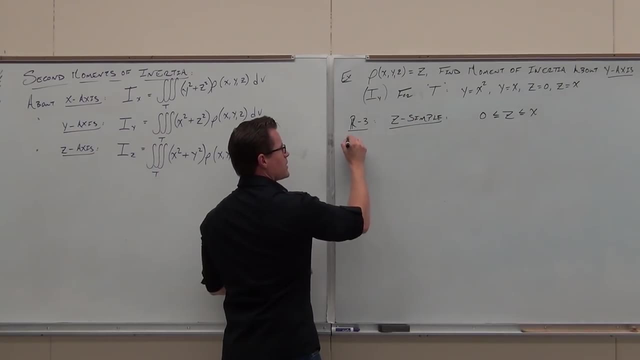 of Z equals. you tell me what the smaller one is: Zero. What's the larger one? It's literally given to you. use that. that's so nice. So if we're doing Z simple, you all need to tell me. 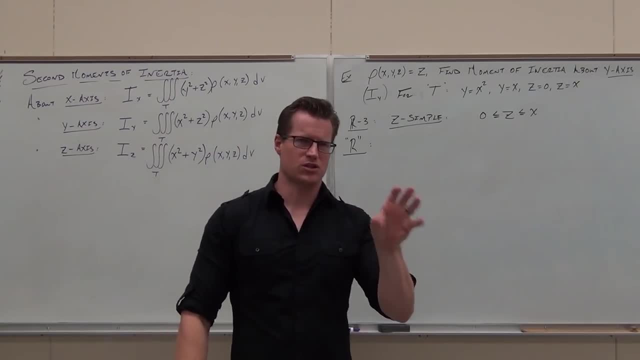 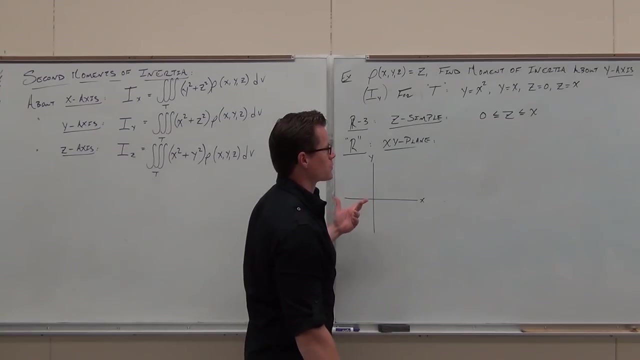 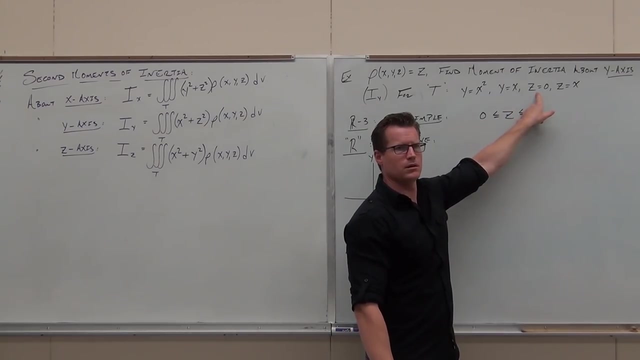 what is the region? what coordinate plane is the region on X, Y, Y? We should draw this every single time. If we draw that and we go, okay, well sure, oh man, is that relevant? No, that's telling us that we're on the XY plane. 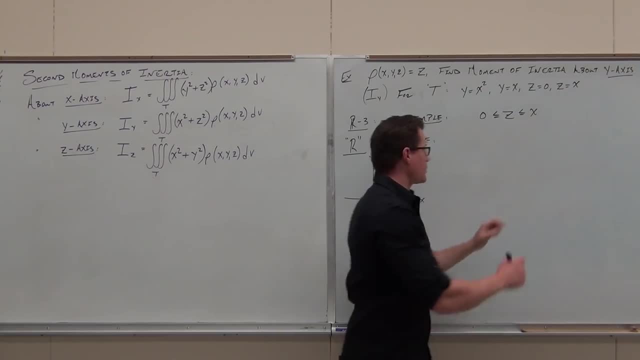 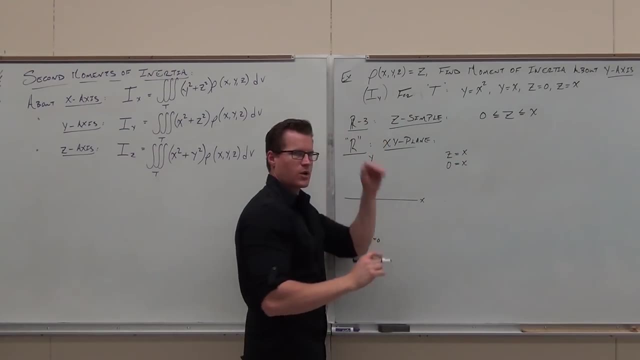 Is this relevant? Yes, because on the XY plane, Z equals X becomes zero equals X. Okay, so that's X equals zero. That's giving us a Y axis. That's already helping us just a little bit. at least it's giving us something. 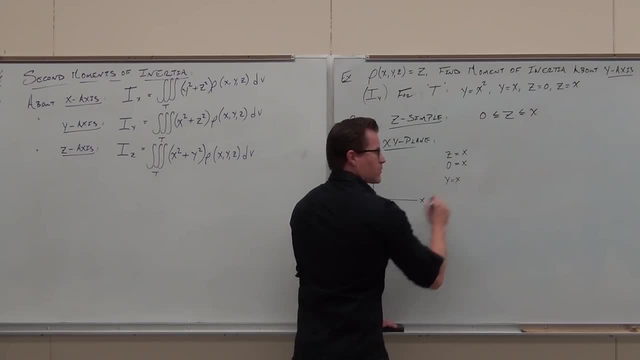 Next up. so that's one. How about Y equals X? Is that relevant? Oh, that's certainly relevant. That's literally a line on the XY plane, so let's draw that line, And then we have this Y equals X squared- also relevant. 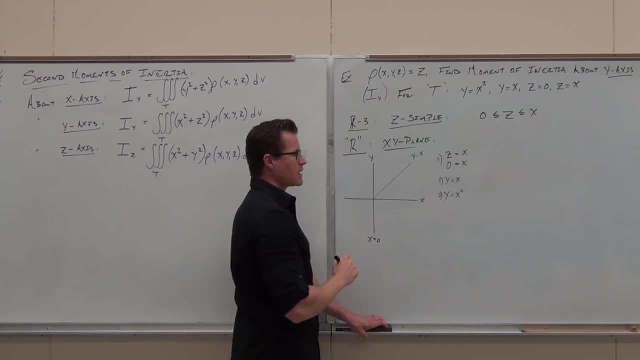 So one, two, three lines that we get out of this thing: Y equals X squared. well, that's That Over here is not relevant. It's not creating any additional region for us on the left-hand side, so just focus on quadrant one right now and now that you're okay with that one. 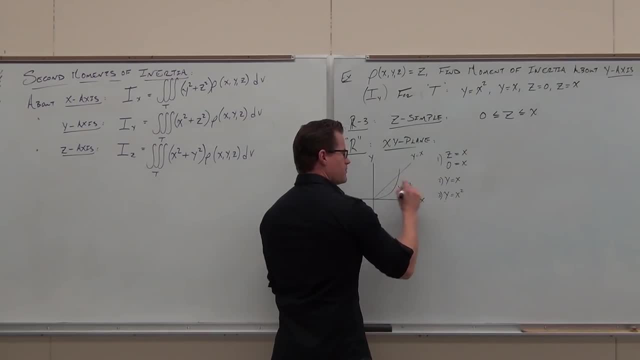 So our region is this guy. We've got Y equals X and Y equals X. squared Man. it helps to draw those regions. It literally shows you everything you want. Now what would you do? We've already done Z simple. The next thing I need to do is pick an R2 simple. so, somewhere across this region, either along the Y, 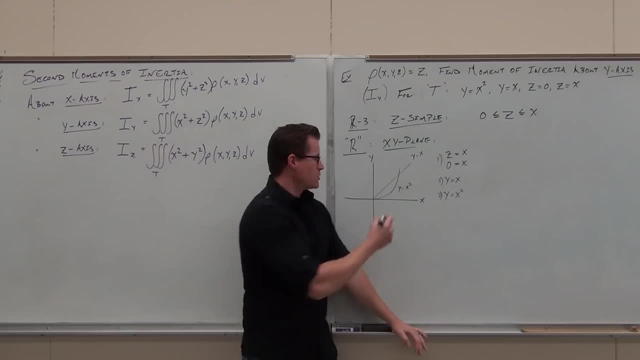 or along the Y, Along the X? What's the appropriate choice? Would you go DX along the X or along the Y? What would you do? Y, Y? Why would you go along? You're right, but why would you go along the Y? 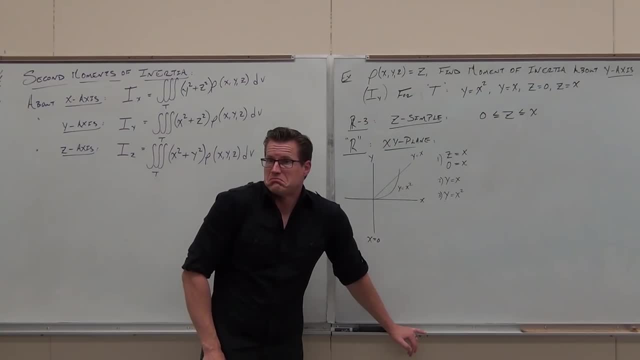 I don't know, It's already there. yeah, If I had to solve it for X, it'd be kind of annoying because I have some square roots. I had to plug in some square roots. Do you want to do that? 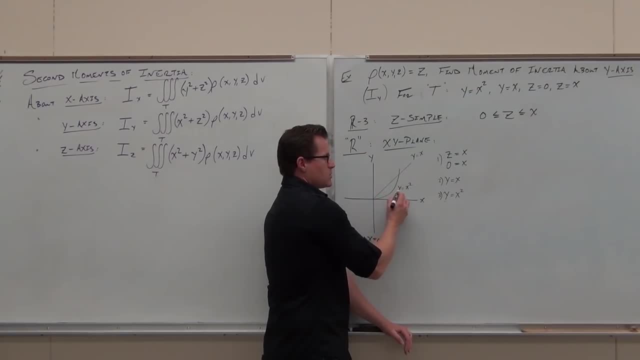 Well, I don't either. You could. You could do it, You could go this way, But you'd have to solve for X. If this one's already solved for X, it's kind of universal, But this one would suck. 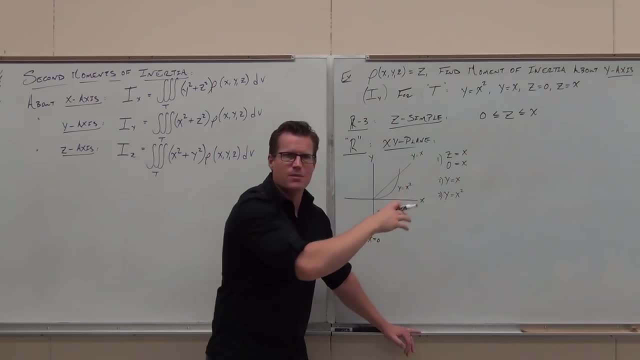 You'd have that plus and minus square root of Y. You'd pick positive square root of Y, but you'd have to plug it in square roots. Do you guys want to plug in square roots? Then stick a. yes, I love square roots. 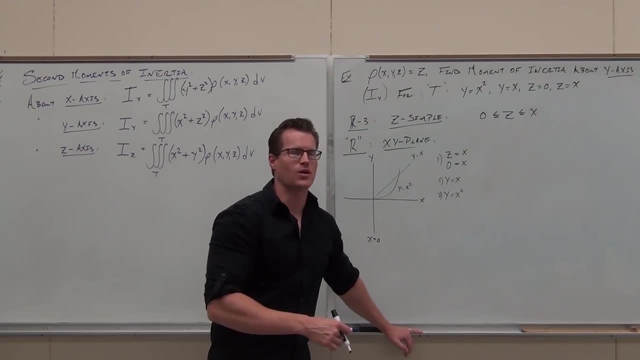 I love one-halves over one-halves X to the- oh sorry, three-halves over. whatever it is, I don't want to do that because I don't want to have to solve for X, because that's annoying. 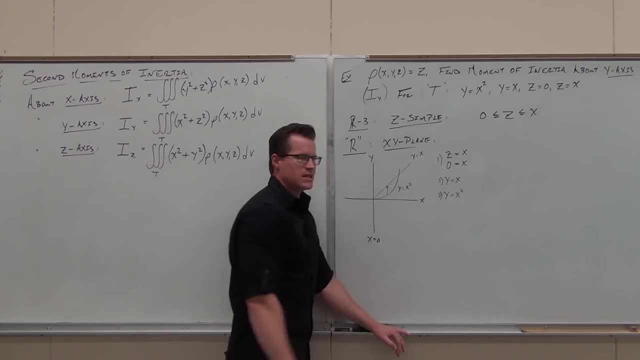 So for the R2, simple: let's go DY first, Let's go DX, Let's go between two functions of Y. That's what that means. So our two functions of Y. what's the smaller of those two, please? 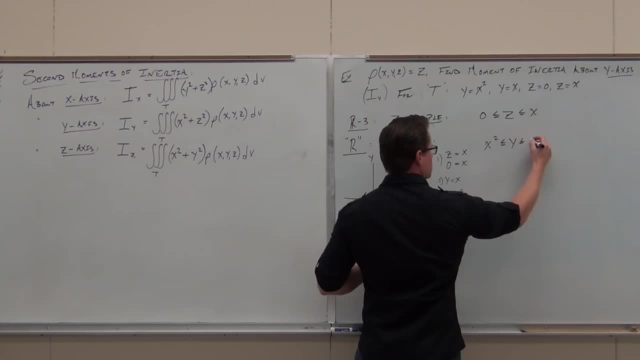 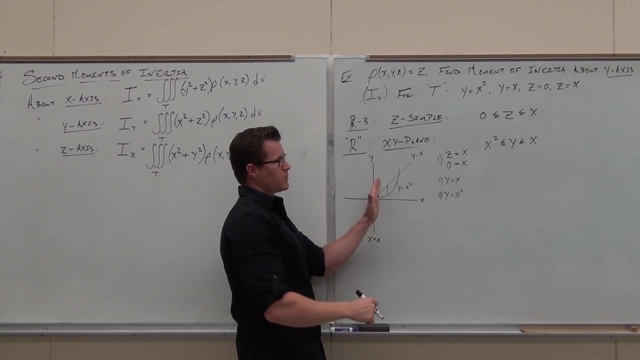 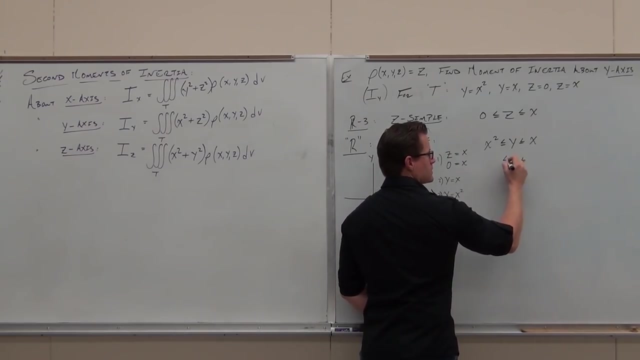 Square root of X Larger. Now, if I do that, if I go along the region R2, simple between two functions of Y, that leaves me with my constants along the X. So I need X to be between constants. What, oh wait, what constants are? I don't see any constants. 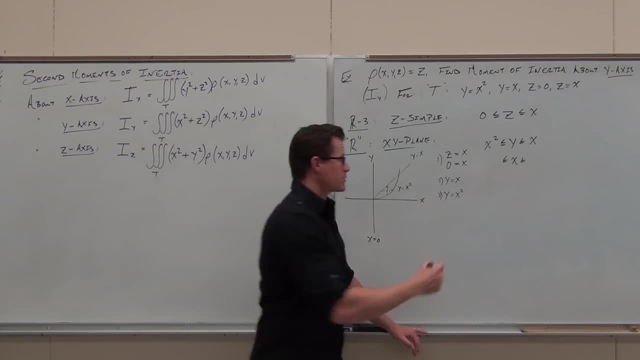 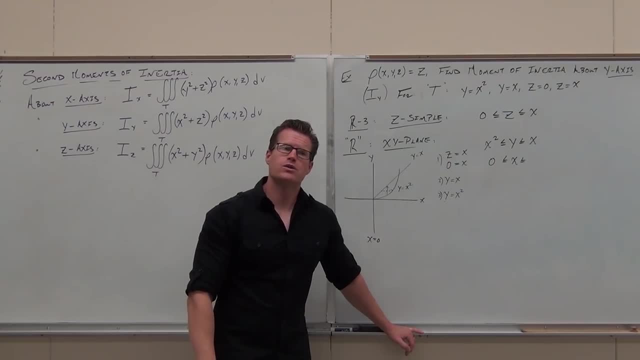 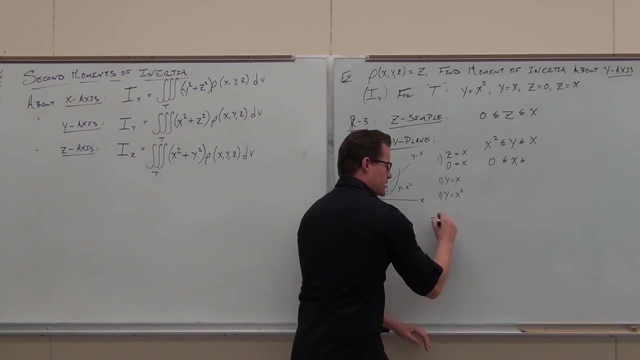 So I'm going to do that, So I'm going to do that, So we go okay. well, if I set these things equal, so set them equal. subtract X: X minus 1, I know that X equals zero and X equals 1.. 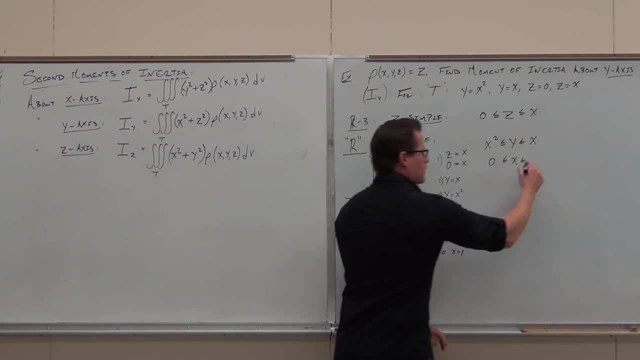 That gives me my constants. If that's 1, 1,, which it is- then I get zero 1, I don't know if you're okay with that one. What I want is a, a perfect setup on the function. So And I want to make sure I want there, I want that when there's something common. so I'm going to make sure that I'm on the one and you're not getting the multiple like if there's one or two nest in the same raised group. 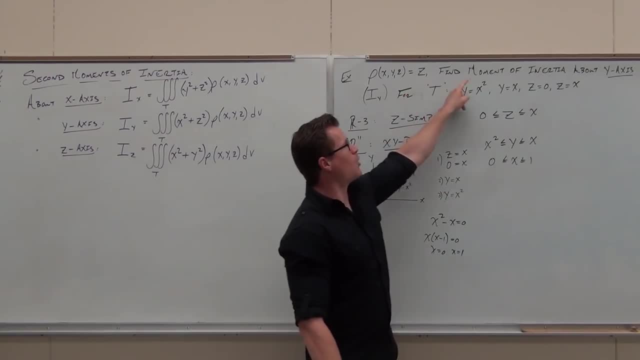 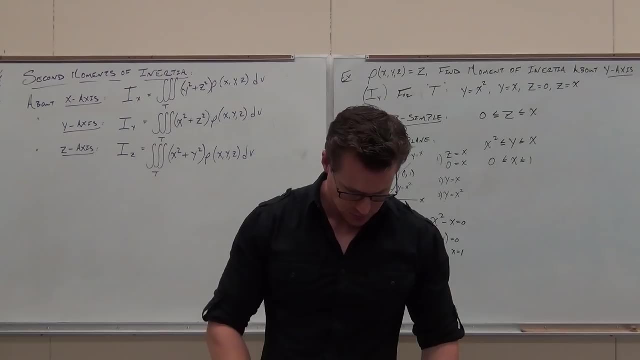 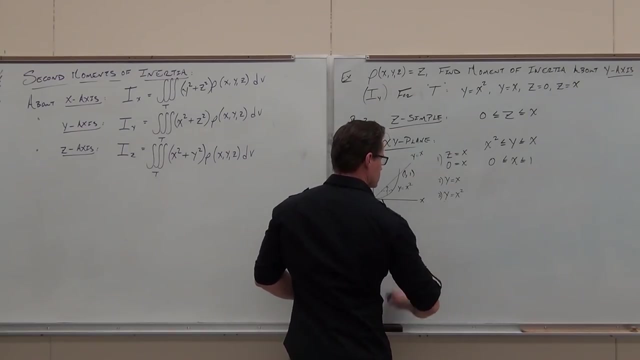 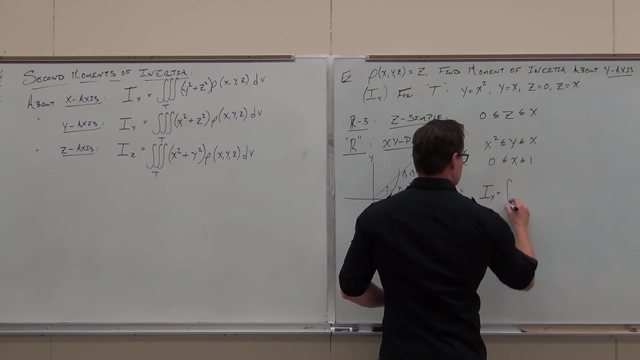 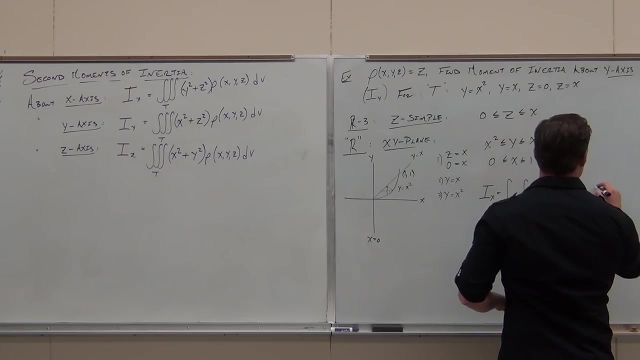 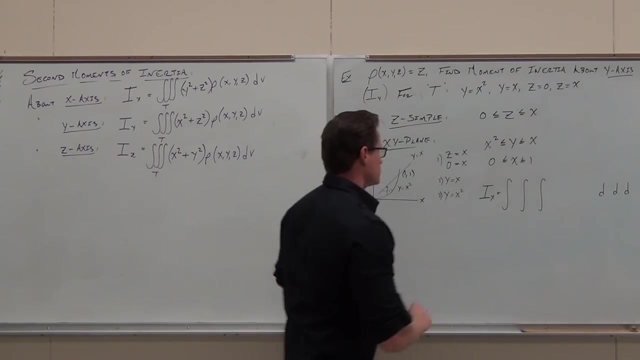 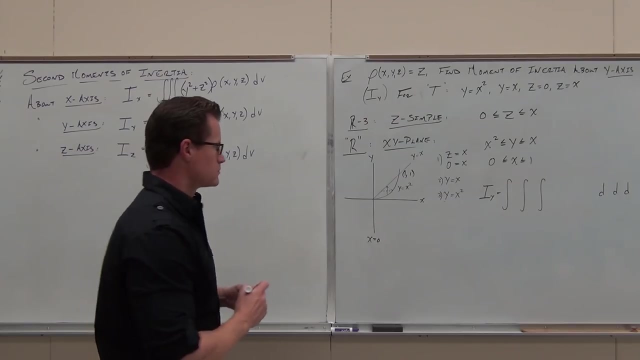 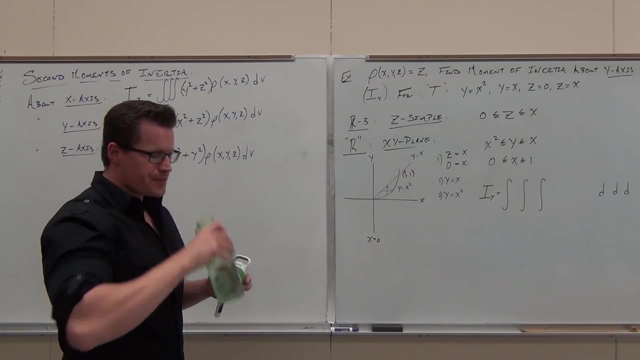 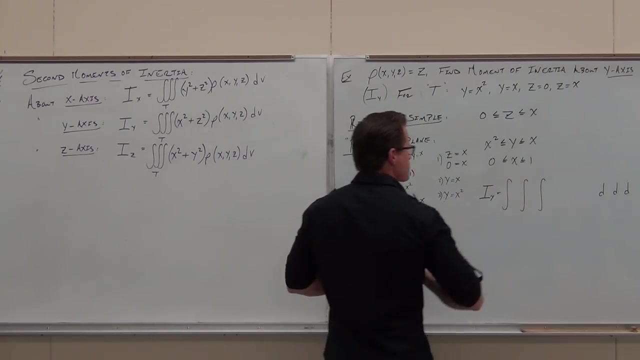 Perfect set up of your triple integral. Again we're finding the moment of inertia. second moment of inertia about the y-axis. So you look at the formula: set up a perfect triple integral formula. That's what I want, All right. 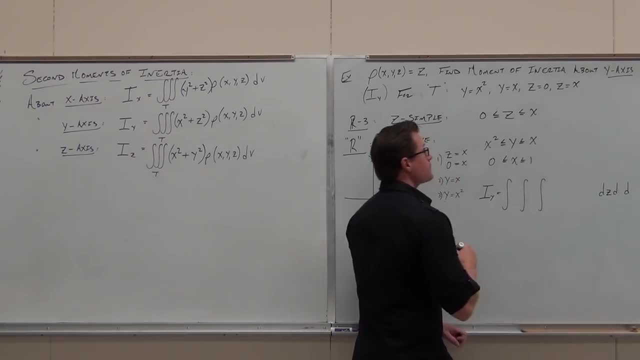 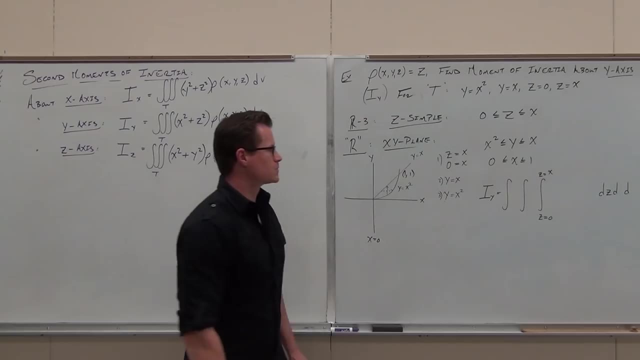 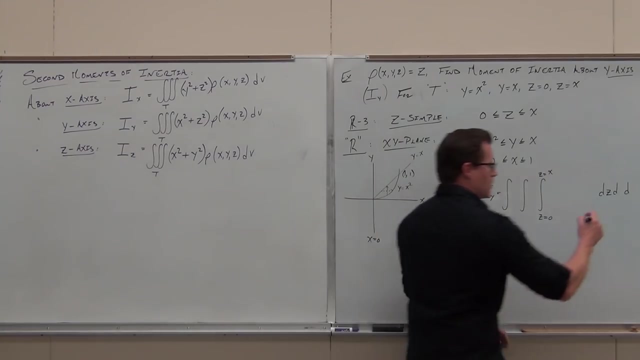 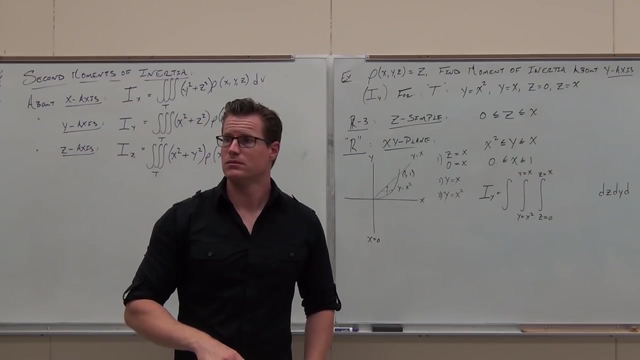 So z simple, dz first between 0 and x. R2 simple was along the y, so dy. y equals between x, squared and x. All right, Did you remember? Did you make it that far so far? Yes, yes. 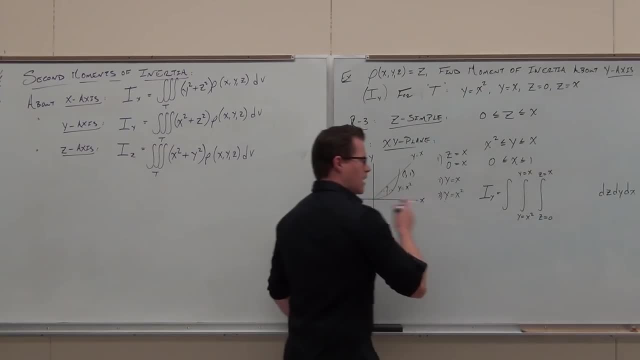 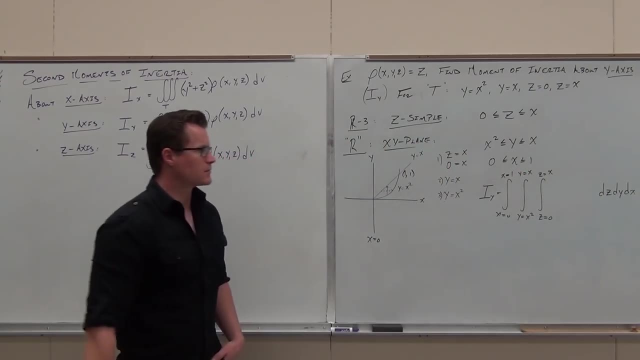 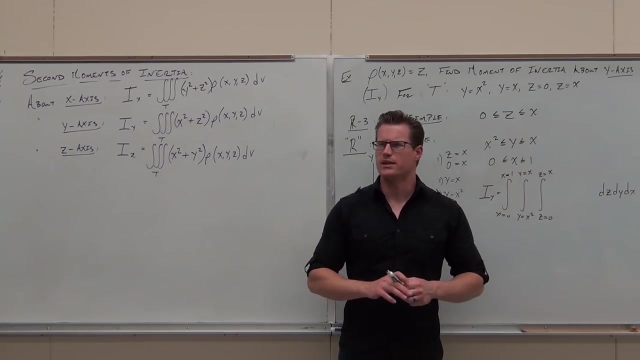 Last one: Constants. Rx is our last one. Constants from x equals 0 to x equals 1.. Hey, that's the region. By the way, if I left it right here, if I left it right here and integrated from this right now, what would it give me? 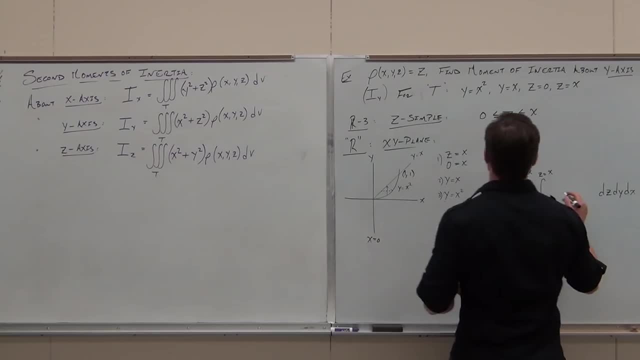 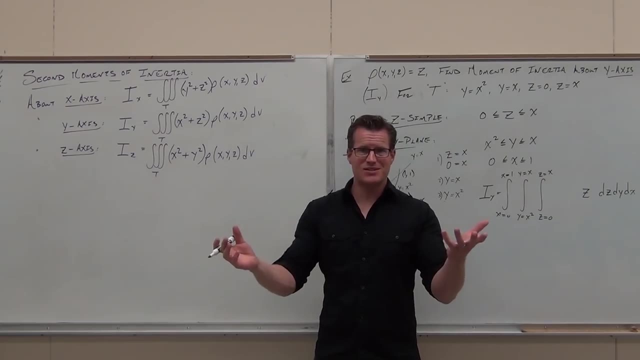 Yeah, that's right. Give me the volume of the region. If I did this And integrated, If I integrated with that, what would it give me Mass? That's right, That's the mass of the region. And now to find the second moment of inertia, about the y-axis. 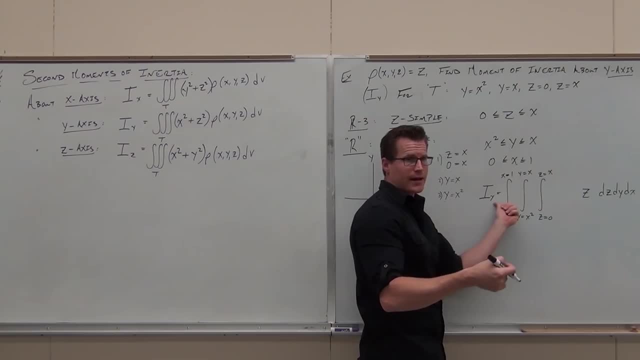 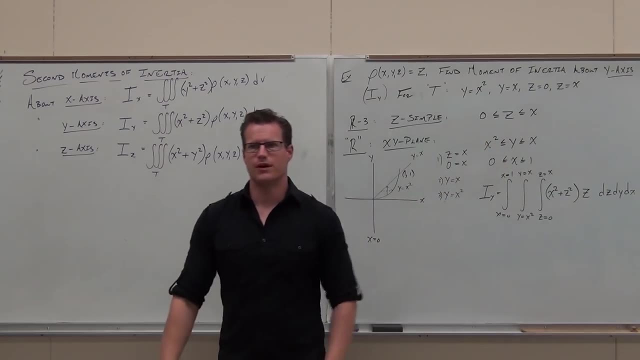 I need to have the other two variables squared and added. So I need to have x squared plus z squared in there as well to find the second moment. That's the correct setup. I need to know if you all got that Show of hands, if you did. 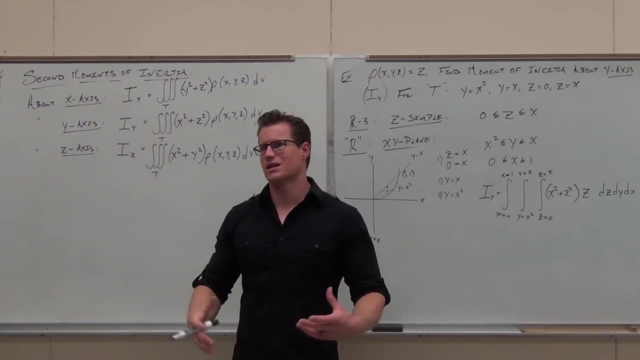 That's fantastic. Again, I'm going to leave it to you. This one's kind of an easy one. What's the first thing you're doing? What's the first thing you're doing on this problem? before that, before you integrate? 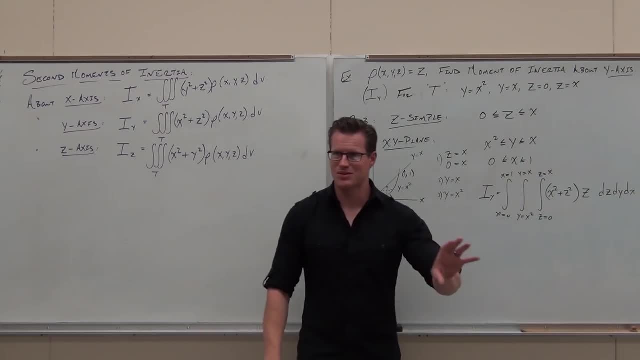 Don't do a u-sub here. Don't waste your time doing a u-sub. Okay, Please don't do that. Distribute, Distribute, Distribute. Don't do u-subs with power ones. That's like a universal. 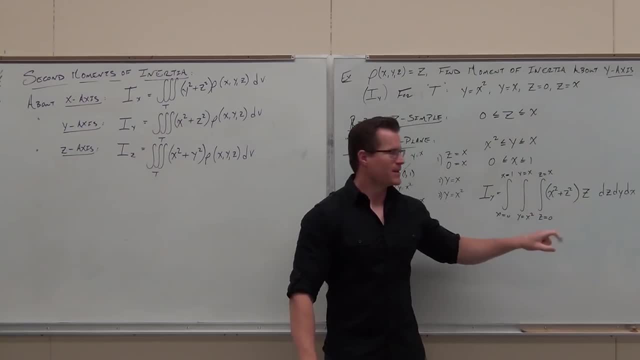 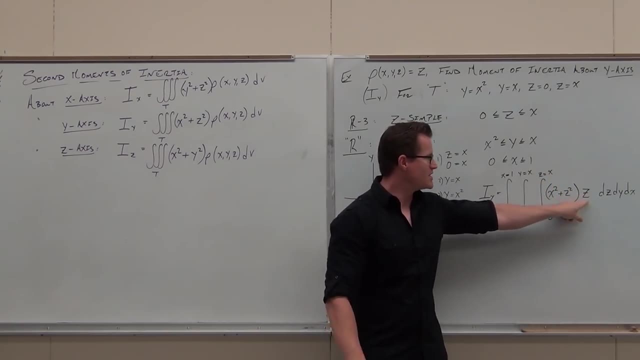 That's like a face punch your test? Okay, Don't do that. If you don't have powers here, do not do u-subs, because it's easier to just distribute that and do basic, basic integration. Does that make sense? So do I need to do it? 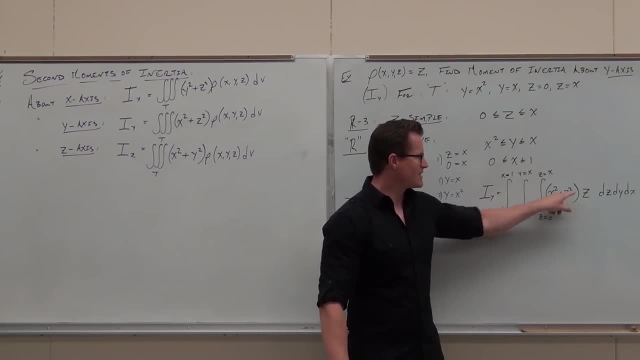 No, Distribute this. That's x squared z. This is x to the third. Integrate with respect to z: You're going to get a one-half, You're going to get a one-third z squared z to the third. blah, blah, blah.